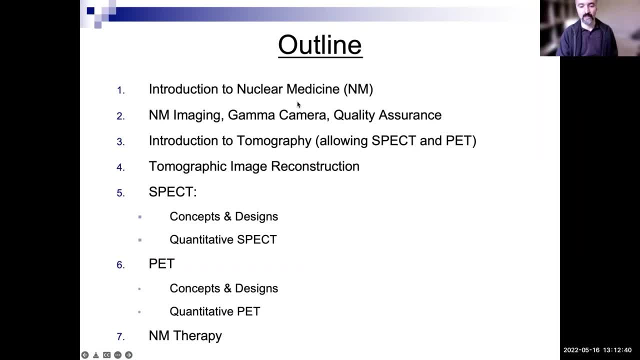 Please feel free to stop me anytime. And looking at how imaging is done in nuclear medicine. what is a gamma camera? quality assurance aspects, what is tomography? how do we do tomography, especially Nuclear medicine that leads to SPECT and PET imaging. how do you do reconstruction? and some of these you'll see overlap with what you might have learned so far on CT, for example. 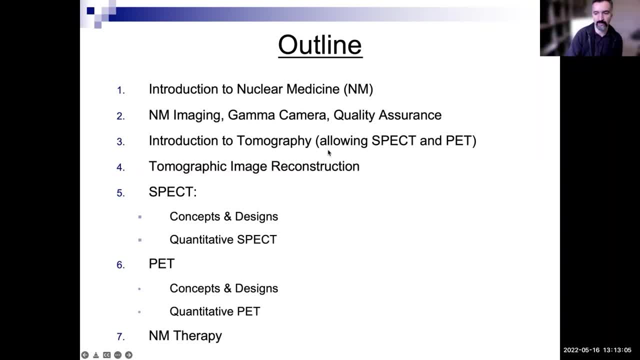 Some of the concepts, some of the core concepts, but of course they're very different in some other sense. whereas because in our field we were dealing with emission Whereas an emission tomography, whereas in CT imaging you're dealing with transmission tomography because the source is outside the body, whereas in nuclear medicine the source of radiation is inside the body, 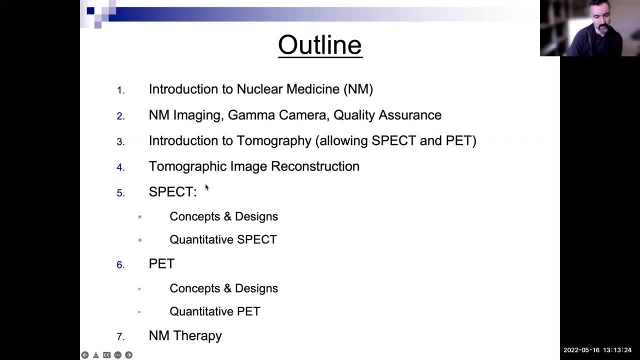 So we're going to talk about that a little bit later. So we're going to talk about that a little bit later. So, SPECT imaging, PET and finally, the very exciting and emerging or re-emerging field of nuclear medicine therapy, also known as radiopharmaceutical or radionuclide therapy. 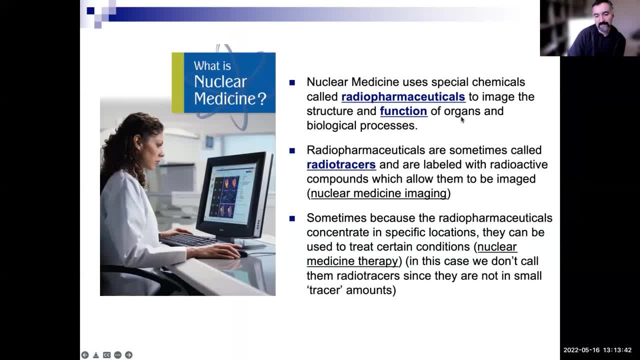 So nuclear medicine? you know basically what is it And you know we're dealing with radiopharmaceuticals that are used to image the structure and especially you know what's the valuable point: is the molecular. And you know we're dealing with radiopharmaceuticals that are used to image the structure and especially you know what's the valuable point: is the molecular and the functional aspects of the body, of organs and biological processes. 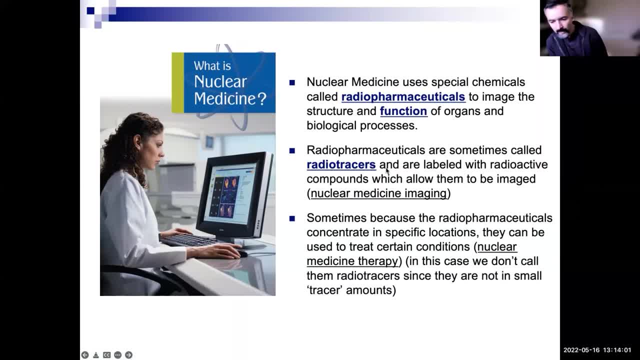 They're sometimes called radiotracers, you know, because they're injected in tracer in small amounts. but this is for imaging In therapy. you shouldn't be calling them radiotracers, because you're not supposed to be injecting small tracer amounts. 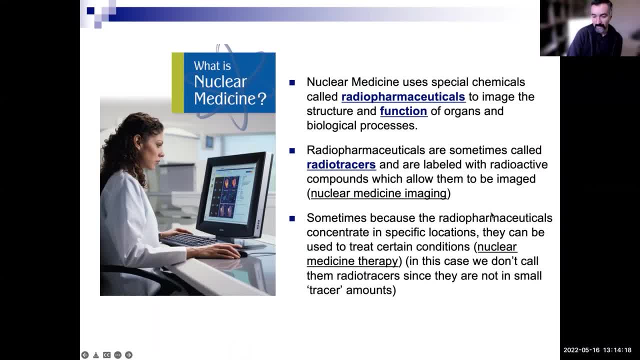 You're supposed to be injecting large amounts And if they're really concentrating well in specific locations or in certain, for example, tumors or cancer cells that express certain proteins that you're binding to, then you really do want to be injecting a lot. 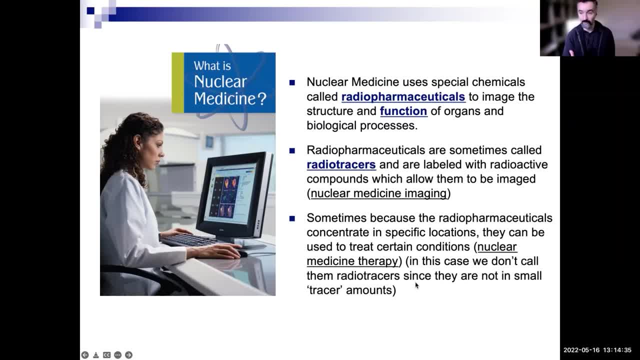 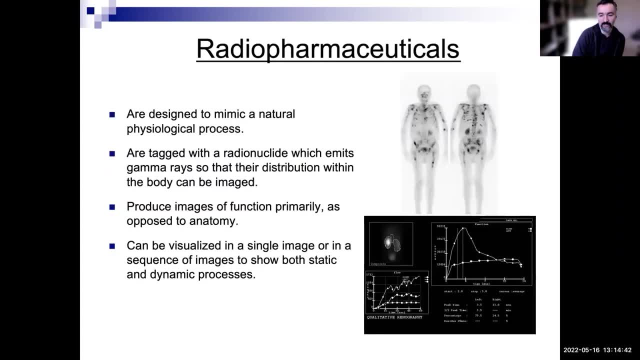 And so in that case we just call them radiopharmaceuticals, for example, because you want it to sit there Instead of imaging. you want it to bombard the tumor, for example with high doses. So both sides are very active: imaging and therapy. 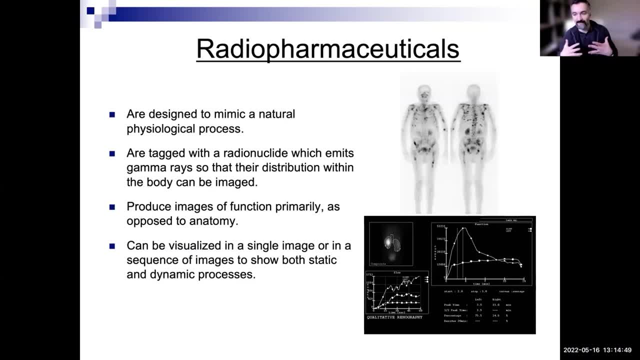 And therapy in the past. you know, half a decade is just undergoing tremendous growth, A lot of exciting results, which I'll be talking about. So radiopharmaceuticals are designed to mimic a natural physiological process, So they're tagged with a radionuclide that emits gamma rays and produces images of function as opposed to anatomy. 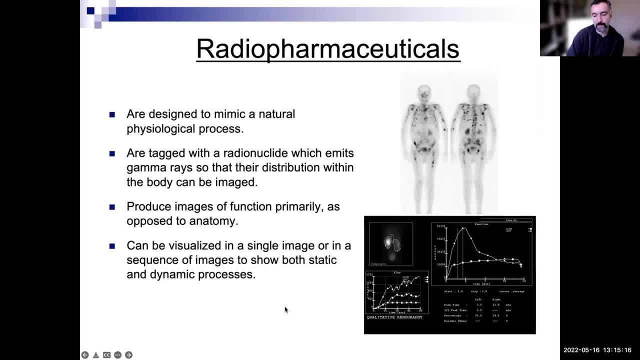 And so this could give you a single image or it could give you dynamic images. For example, you could get a dynamic image of a certain organ and track how the uptake in the organ, for example, changes. So this would be dynamic image. 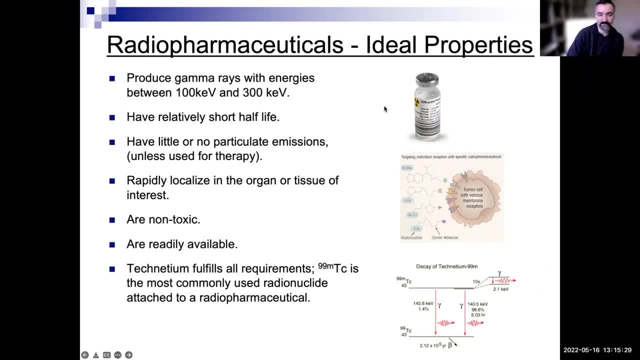 So what would be an ideal property of a radiopharmaceutical? Ideally, you would like it to have these energies between maybe 100 to 300 kiloelectron volts, Because if it's below this then it's scattering in the body left and right and it's not making its way to the detectors. 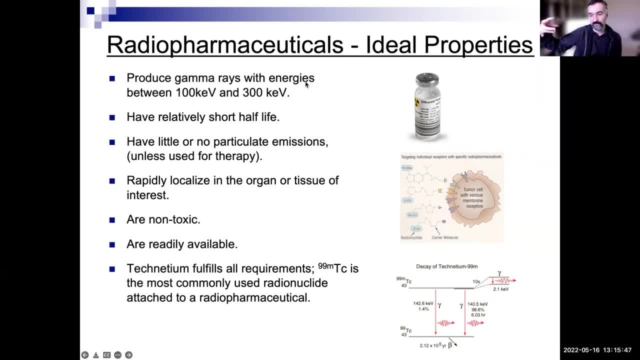 Whereas if it's more and more energetic, then it becomes more and more difficult to capture it. And you have to build thicker and thicker crystal, giving you more and more experience. And you have to build thicker and thicker crystal, giving you more and more experience. 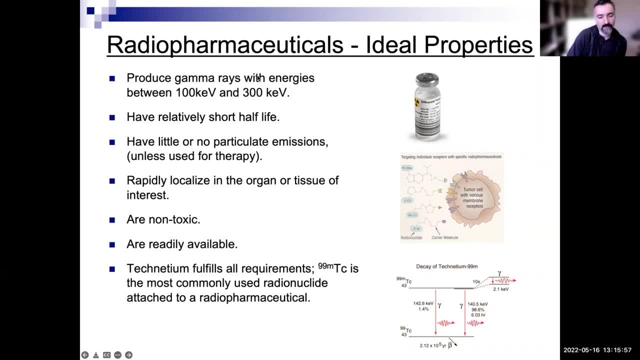 And therefore the sensitivity would come down. You would like it to have a relatively short half-life. You don't want it to be too short, because then transportation becomes difficult. You know figuring out by the time it's produced, but until the time you inject it into the body it's going to take a while. 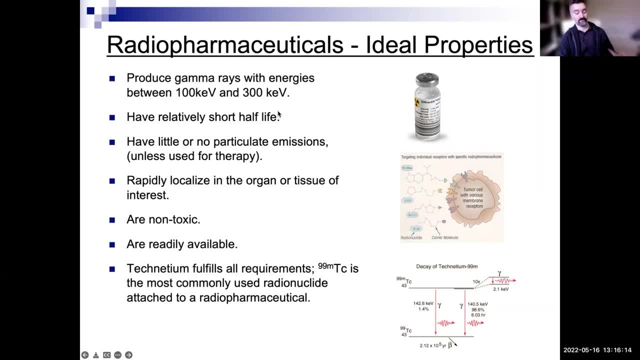 You don't want it to be too long either, because you're injecting it into the body. If it sits there forever, then you cannot inject too much and therefore you're not going to get high-quality images. You don't want it to emit particles. 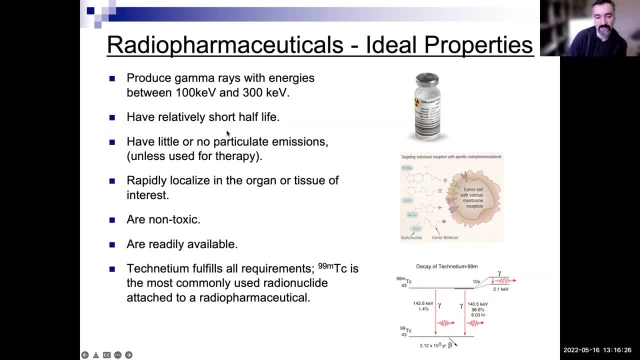 You don't want it to have particulate emissions, because if it emits particles, the particles are going to be actually harming the body. Except, again, if intentionally you're using radiopharmaceuticals for therapies. In that case you definitely do want them to have particulate emissions. 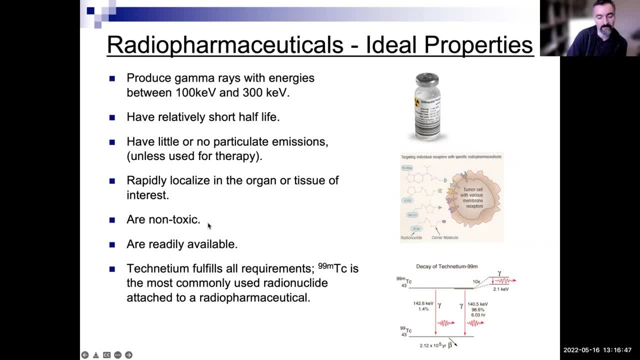 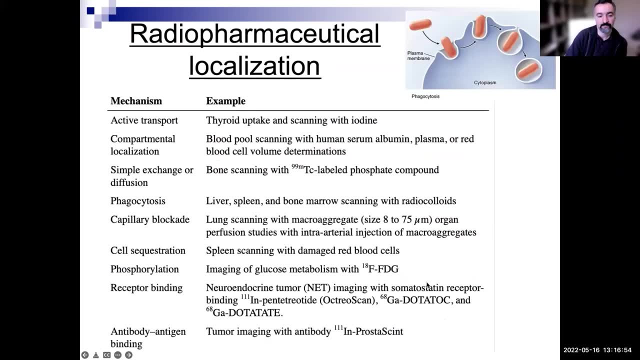 You want them to rapidly localize. You don't want them to be toxic. So for imaging radiopharmaceuticals, technetium really fulfills Technetium. we'll see in a bit. it has a six-hour half-life and an energy of 140 kiloelectron volts. 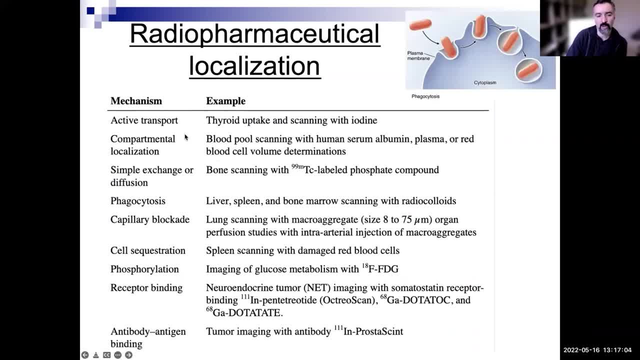 We'll see that in a bit. So radiopharmaceuticals localize in the body using different phenomena mechanisms. Active transport is one of them. Diffusion Phagocytosis is one: Cell sequestration- We're going to see an example of this where you used to do splint scanning with damaged red blood cells. 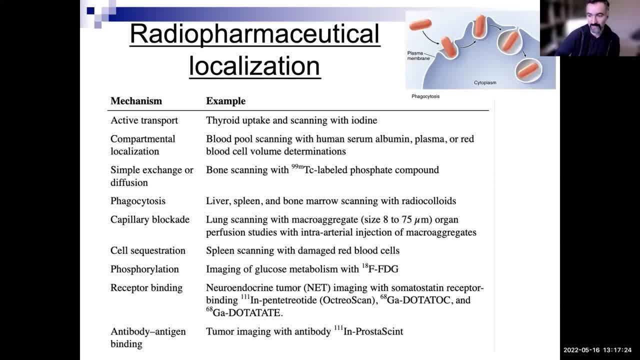 You damaged red blood cells, You put them into the body And because the splint is supposed to deal with that, it accumulates in the splint. It's kind of a very cool phenomenon Just showing the amazing range of things you could do in nuclear medicine imaging. 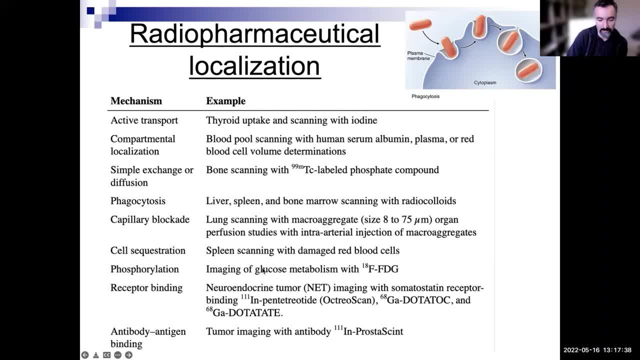 Phosphorylation. So along the glycolysis pathway, like here, we have fluorodeoxyglucose. You can sort of think of it as radiolabeled sugar, sort of right, And in that phenomenon you could be imaging the body's metabolism. 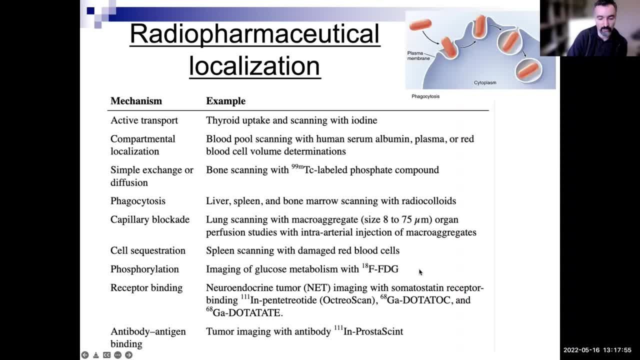 which is what we're doing. PET imaging using fluorodeoxyglucose, Very, very commonly used Receptor binding, is very, very popular these days- Neuroendocrine tumors, for example- and antibody-antigen binding is also another phenomenon. 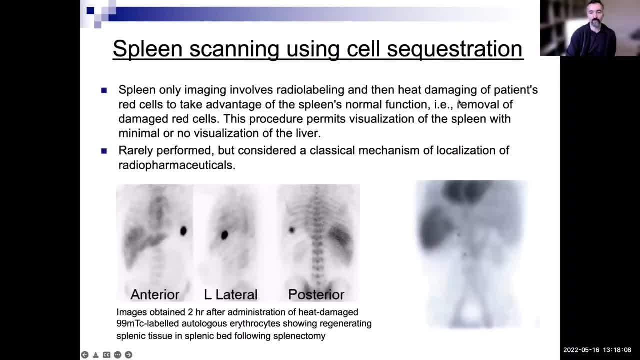 So the promised example of splint scanning. So if you heat, damage some red cells and then inject them into the body, well, the splint's normal function is to remove damaged red cells, right? So you start, Start, Start, Start seeing an accumulation in the splint. 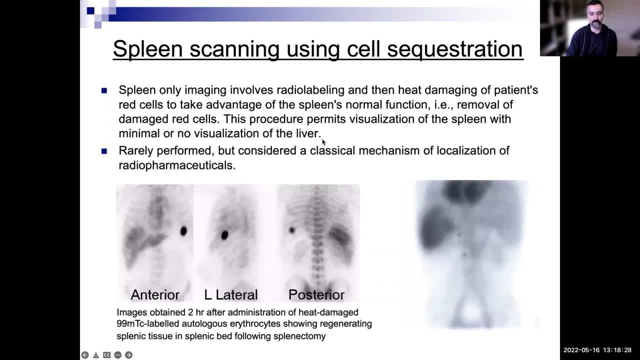 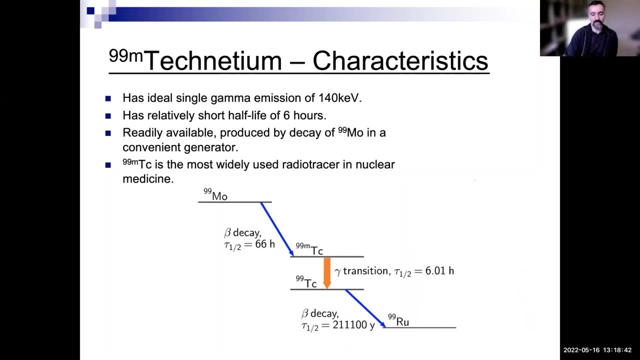 So that's a very cool idea that used to be used to image the function of the splint. Just showing you that the sky's the limit in terms of the kind of things you could do in nuclear medicine imaging Stegnetium again. 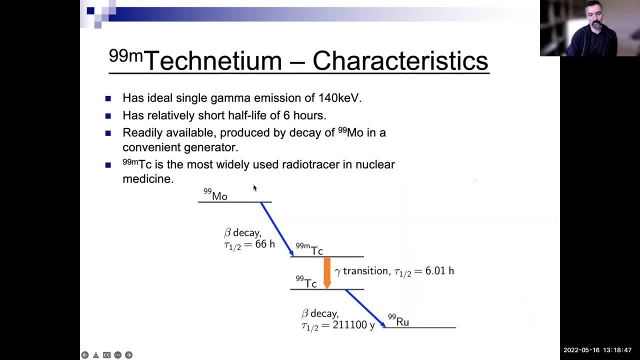 So you start with the parent isotope, right? So the parent in this case would be molybdenum-99.. It emits into stegnetium-99m, which you can think of it as like an elevated state of stegnetium-99.. 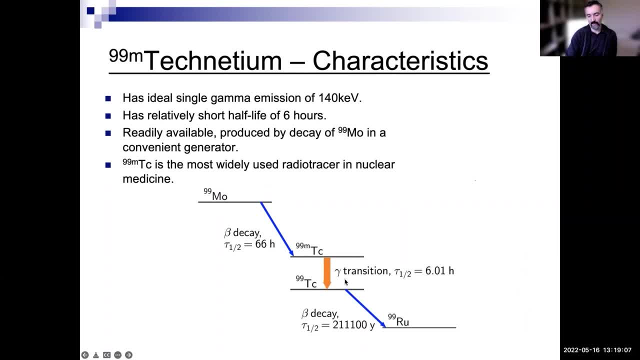 And then it emits to stegnetium-99.. And that phenomenon, that transition takes about, or the half-life is six hours and the energy is 140 kiloelectron volts, So it's kind of ideal. Now, how are these radionuclides actually produced? 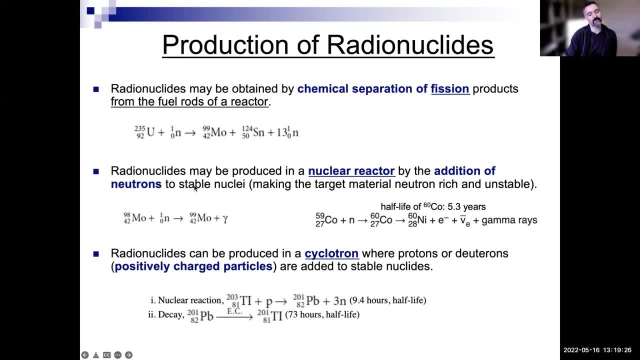 Without going into too much detail, just remember there's really three ways that are used. One is to use fission products. You've heard of fission from the few rods of the reactor. So you have a large molecule and somehow you break it down. 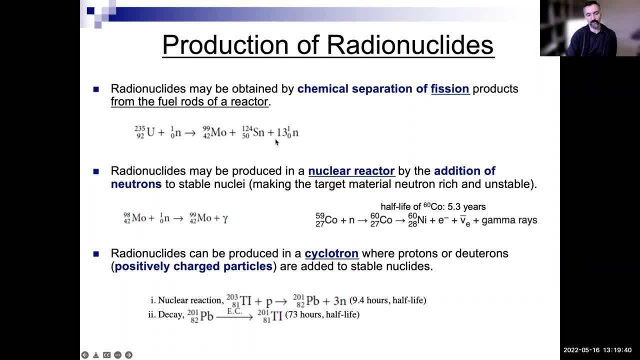 That's what fission is. You break it down into two smaller molecules, And so this is our isotopes. So in this case, you're having uranium being broken down into molybdenum-99.. Right, Molybdenum-99.. 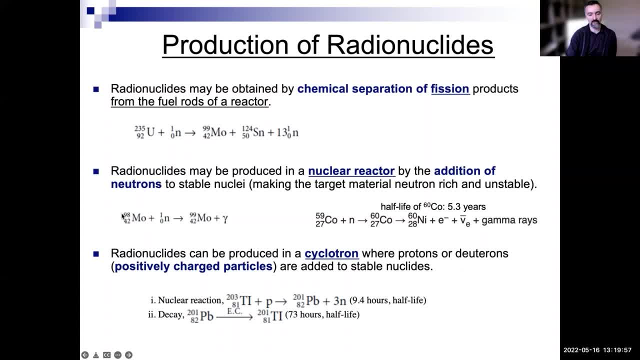 There's another way to produce the exact same thing. In that case, you start with something else like molybdenum-98, and you add neutrons to it. And that's what nuclear reactors are, because in nuclear reactors you are, through whatever phenomena that you're doing- you're producing more and more and more neutrons. 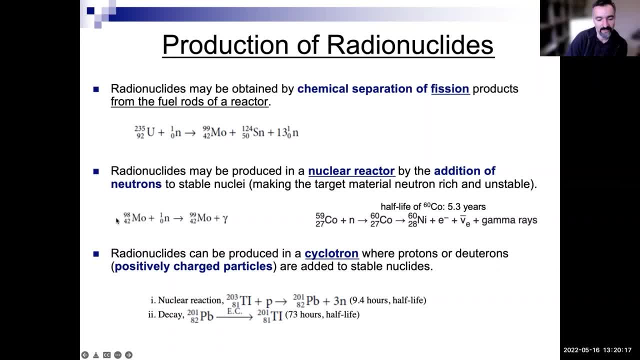 So you have lots of neutrons that can be used to attack other radionuclides, and those then can produce other radionuclides, So this is called. so this is another phenomena where through which molybdenum-99 is produced. 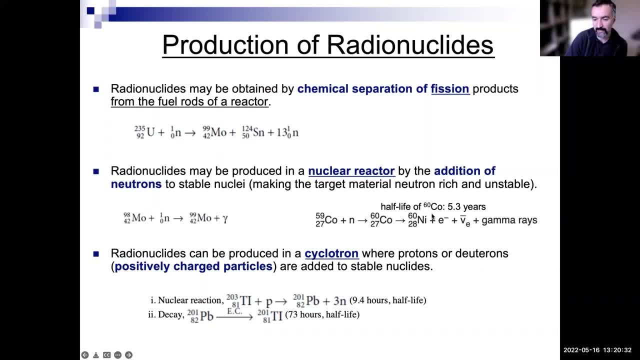 Interestingly, you might have heard of cobalt-60 in external beam radiation therapy. Before LINACs and linear accelerators, which are the norm these days, people used to use cobalt-60.. Even right now in Vancouver, we have one example that I know of where instead of LINACs, they're using cobalt-60.. 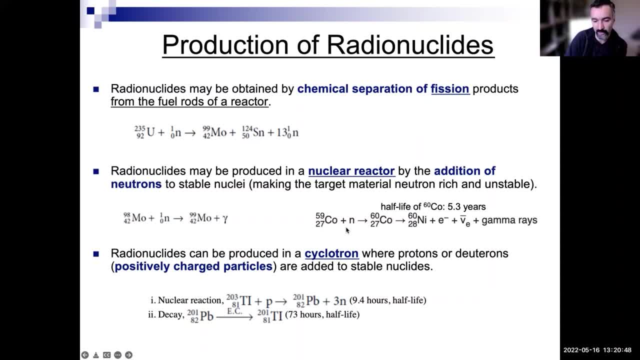 So how's cobalt-60 produced? Well, you take cobalt-59, you add a neutron to it and then you get cobalt-60. Which is a very long time, A long half-life of five years. Obviously, you can't- you know that's not, you cannot- inject that into patients. 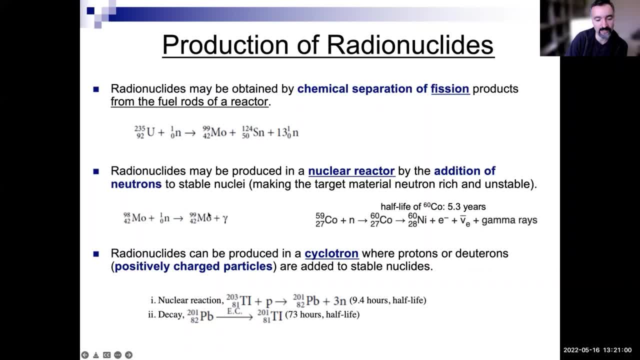 This is for external beam radiotherapy, But molybdenum-99, in this example, has a half-life of around 66 hours. And finally, you can use cyclotrons, which are much more affordable devices than nuclear reactors. So you here, you're adding protons right, or deutrons, which are positively charged particles. 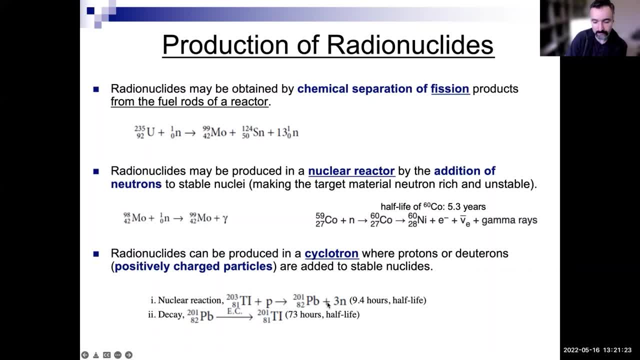 You're adding them to something- In this case thallium- to produce something else. So finally you end up with this kind of a thing Like you start with something else. It's one kind of an isotope of thallium. 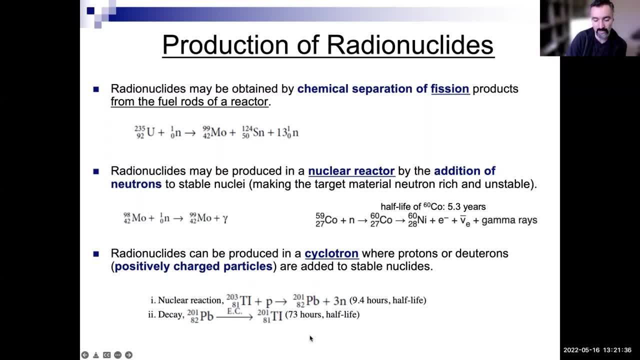 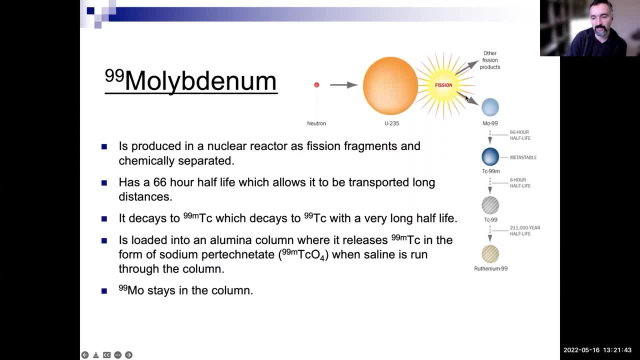 And you finally end up with this kind of thallium which is actually used in cardiac imaging in SPECT. So molybdenum-99- is this parent right that we saw? One example was when you break down uranium-235 into molybdenum-99.. 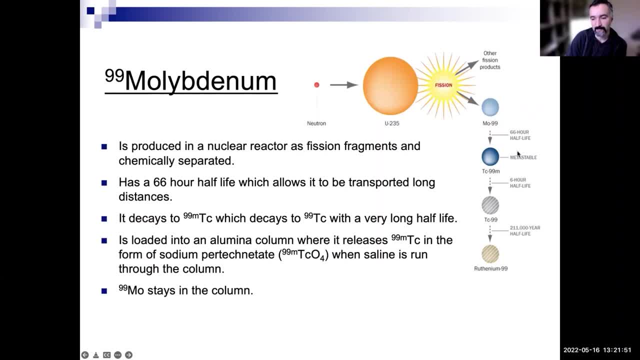 And then you ship it to places, And then You get technetium-99m And you need to separate these two from each other. There's a half-life of 66 hours, So transportation can be done relatively easily. So how do you actually then separate these two from each other? 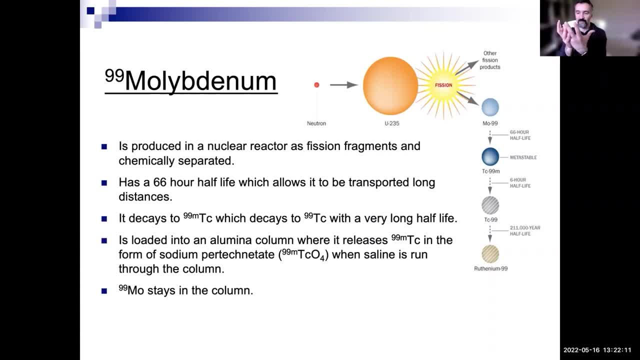 It's like the parent and the daughter are together. How do you separate the daughter, which is technetium-99m, which is what you want to inject into patients? How do you separate that from the parent? Well, to do that, you use generators. 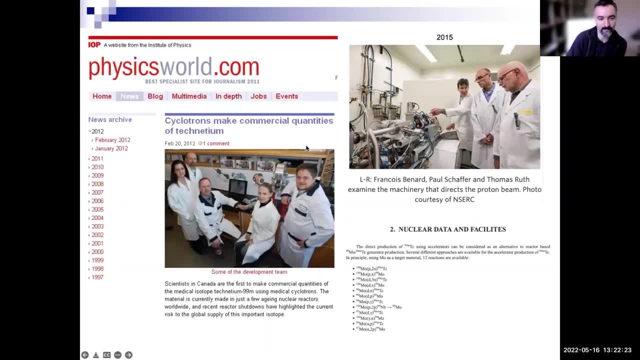 So let me show you an example of that. Actually, before I show you an example of that, I want to emphasize to you that molybdenum-99m can also be produced using other means, Not just using nuclear reactors, but using cyclotrons, which is sort of a very interesting invention that was, for example, really promoted and done in Canada. 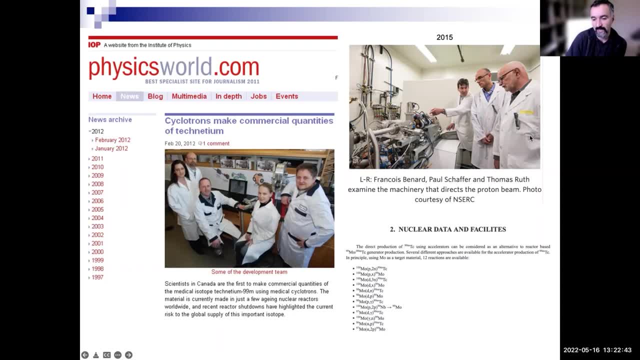 Here are examples of fantastic colleagues here at BC Cancer Agency: Dr Benard, Dr Schaefer and Dr Ruth, who were kind of involved in this amazing project. So, because of shortage of you know sources available, using nuclear reactors for example, because there's only a few centers in the world, sometimes there's shortages. 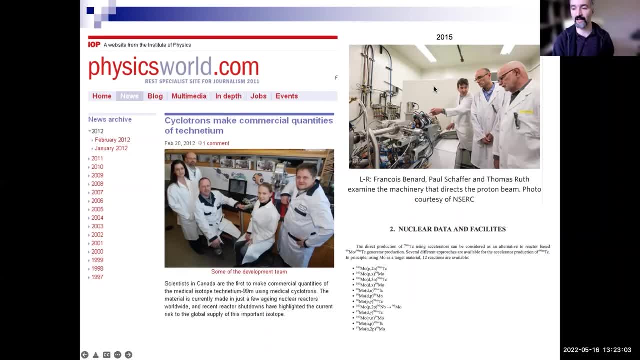 Well, guess what? Cyclotrons are much, much smaller. Every center can have its own, or many centers can have their own cyclotrons to produce this. So this is some innovation that continues to be a work in progress and in discussion. 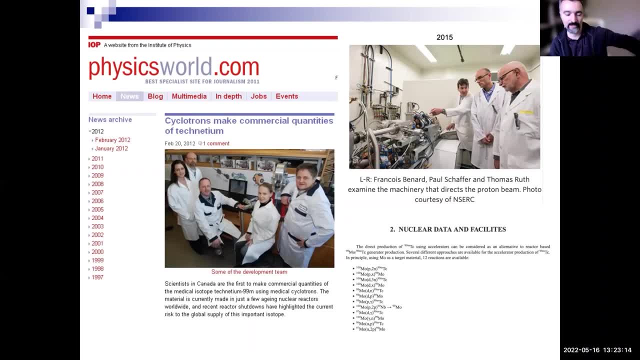 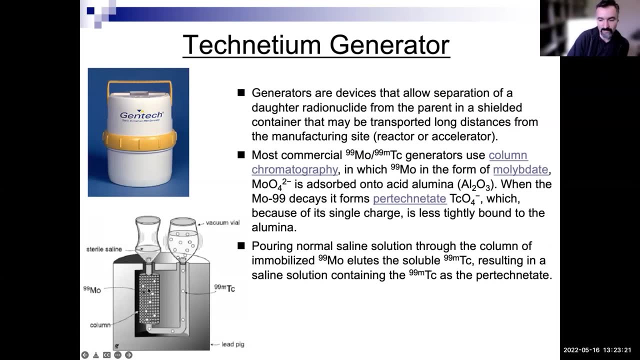 Should one be using the conventional ways or should one be switching to cyclotrons? So technetium generator, Pretty much think of. okay. so you have these things, these materials, the alumina, acid alumina, right. 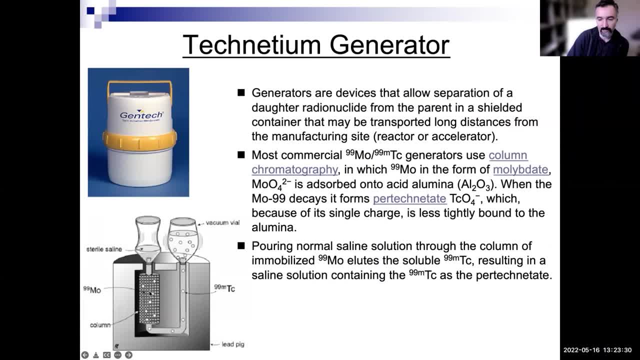 Aluminum oxide basically, And they're porous and they're highly absorbing. So you load the molybdenum, which has created an ion, highly charged ion, two negative charges in here and it just cannot pass through, Whereas the daughter that is created from this 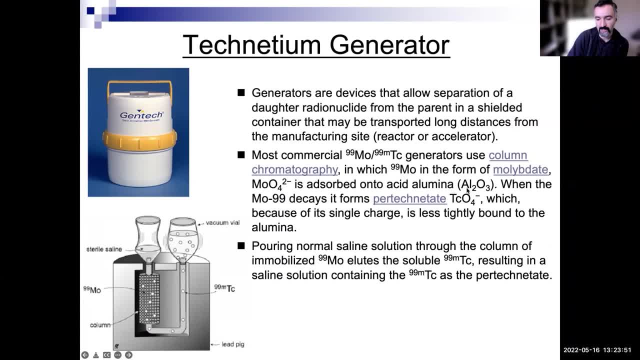 Is technetium which in an ionic form becomes pertechnetate, but it only has a negative one charge, not negative two charge, and it more easily passes through here. Especially when you do saline, you basically pour saline. 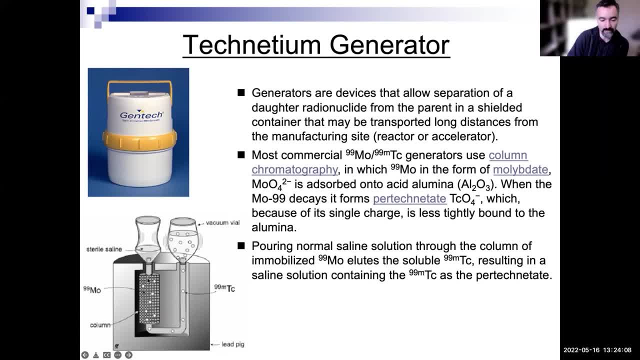 And so, basically, the daughter is able to pass through here, but the parent gets trapped. Just kind of tragic, I guess. right, The daughter makes it, So the daughter makes it And you care about the daughter, not the parent in this example, right? 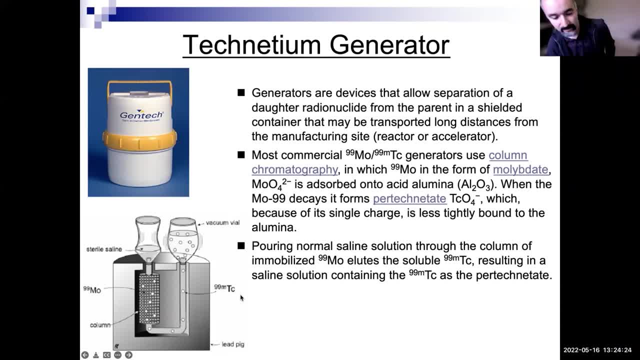 So you want technetium-99m to be separated from molybdenum-99.. You definitely don't want to be injecting this into patients if it's got a long half-life, whereas this is a short half-life- six hours. 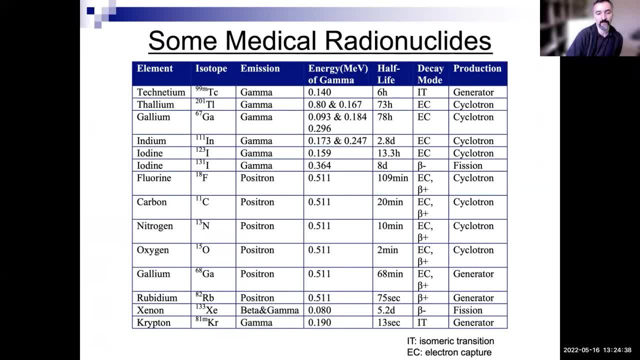 And there you have it. Now. there are many different isotopes. There are, in fact, over a thousand radioisotopes that are out there. Well, a fraction of those can be used in existing scans, Existing scanners and devices. 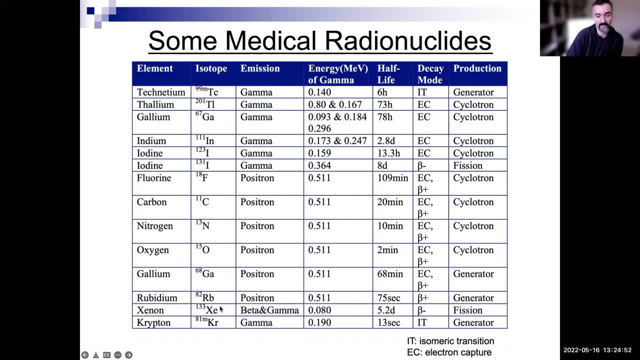 But there's actually a lot of them that can be used. Here's an example: Technetium thallium gallium- right, So you make your way down here- And these emit either gamma rays- so single photon, So this allows you to do planar- or spec imaging. 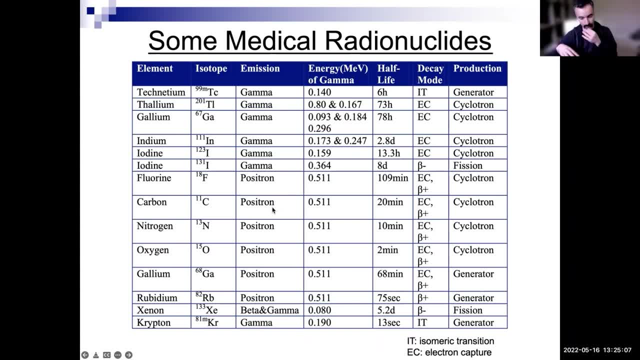 Or they emit positrons And, as you'll see in later parts of the lecture, positrons can combine with electrons and they produce two gamma rays going in opposite directions. Two photons, not one photon. That allows you to do PET imaging. 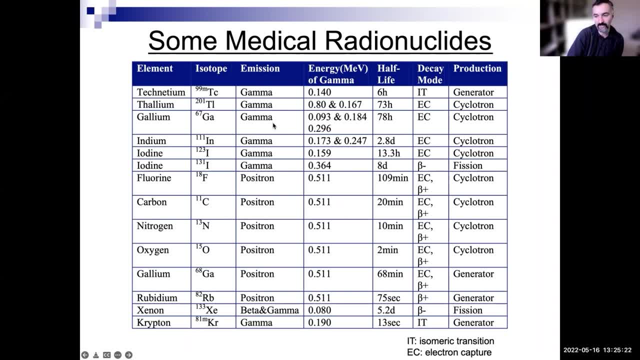 So anytime you see gamma rays it's for spec or single photon, planar imaging or planar imaging. So single photon can give you either planar imaging or spec tomographic imaging. Or you could do positron emission And that gives you two photons. 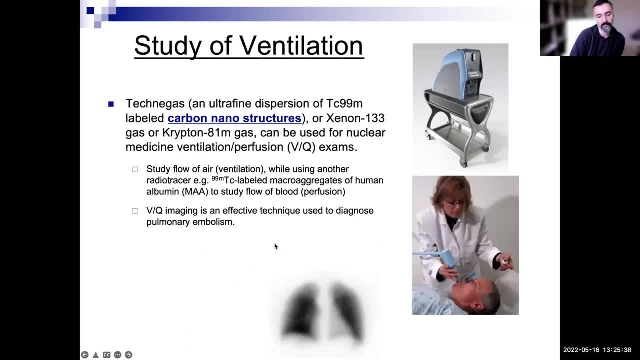 And that allows you to do PET imaging, as we'll see later. So many different things that you could do. Often these are injected into patients, But here's a counterexample to that. We've got technigas, just as an example. 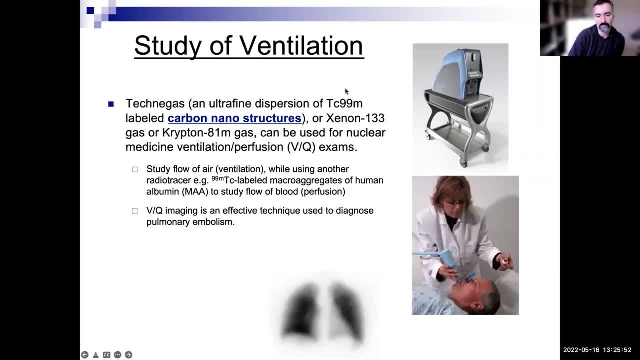 This could be technetium labeled, Or it could be also inert gases like xenon or krypton that are actually inhaled Right And so that can be used for ventilation studies to study the flow of air in the body, And you often inject that with a pair radio tracer. 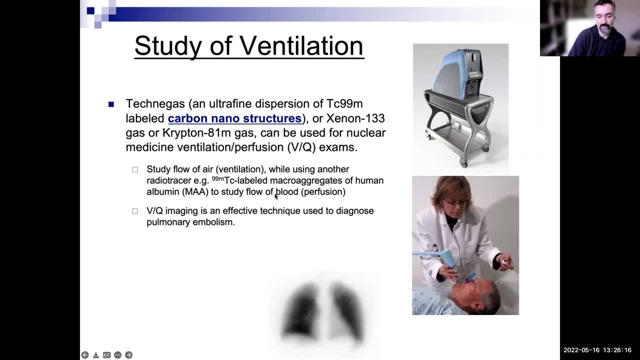 In this case, for example, MAA MAA is mentioned to study flow of blood. So you're studying both: flow of air, that's ventilation, and flow of blood, that's perfusion. So that gives you a ventilation perfusion exam, which is very valuable, as you know. 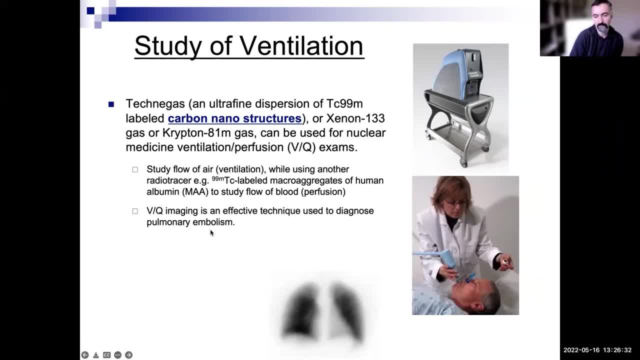 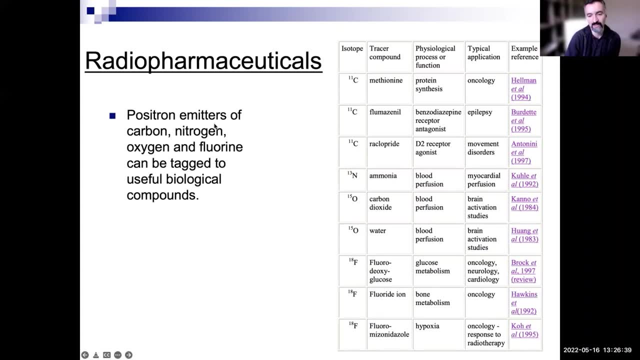 For example, used to diagnose pulmonary embolism. Here's an example of some radiopharmaceuticals in PET, You know the ones that emit positrons, And so examples are carbon, nitrogen, oxygen, Oxygen and fluorine, And these are labeling certain molecules. 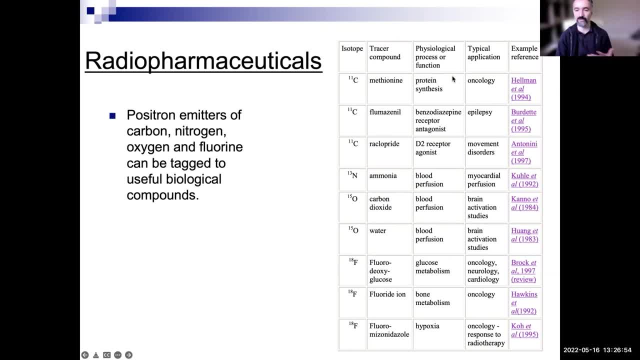 Because these molecules end up measuring a certain physiological process. So many, many different things can be measured. You could measure hypoxia, You could measure perfusion, You could look at the receptor binding in the brain, Et cetera, et cetera, et cetera. 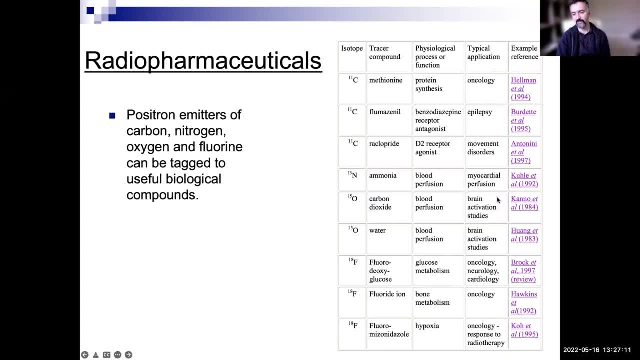 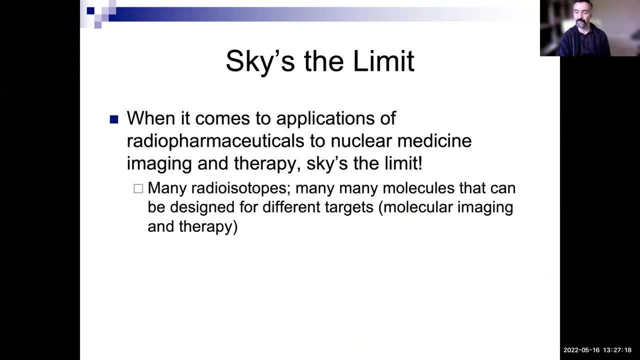 Many different applications: Oncology, Brain imaging, All kinds of different applications actually- Neurology, cardiology, et cetera. So sky's the limit. actually, Nuclear medicine is tremendously exciting Because we're looking at molecular imaging, functional imaging, physiological imaging. 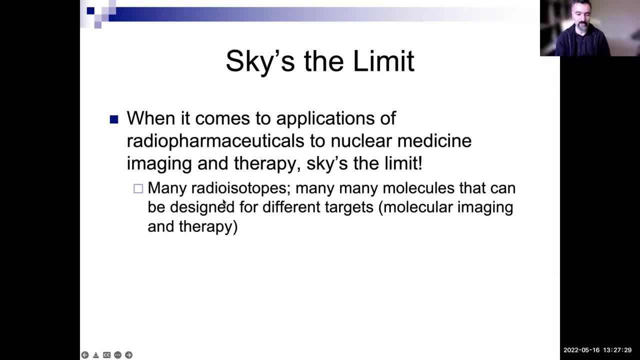 And, as I mentioned, we have so many isotopes that are out there And a respectable number of those can be used in nuclear medicine. And what's more is that those can be used to bind to Many, many, many, many different kinds of molecules. 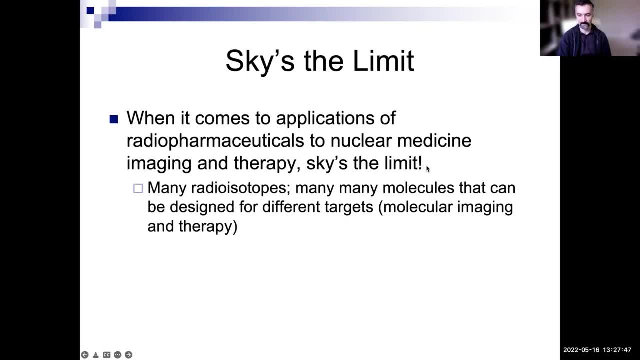 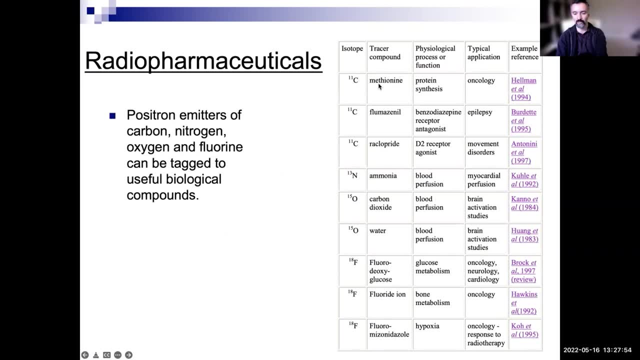 Each of which could be measuring different things. Okay, So carbon-11, in this example, can be used to label totally different molecules Which are measuring totally different things. So it's very, very exciting actually, The kinds of things that you can do. 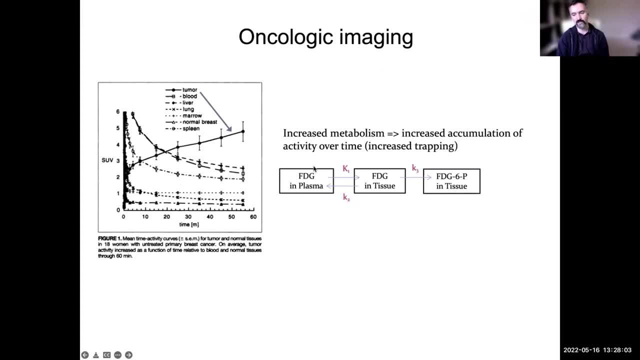 So here's just an example on oncology: Fluorodeoxyglucose. This is radio labeled sugar. Well, there's increasing uptake in a tumor Because of the increased metabolism. Because of the increased metabolism, Whereas in normal organs it comes in and then it leaves. 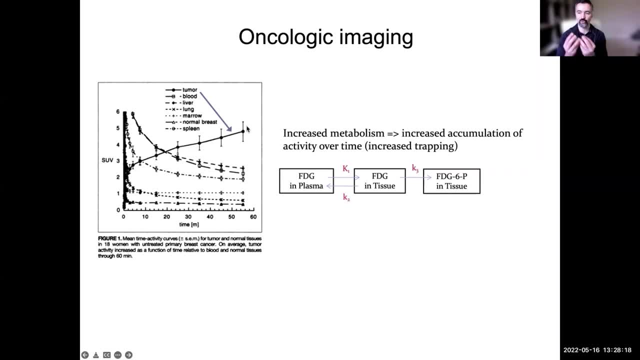 Whereas because of this process of phosphorylation it kind of gets trapped in highly metabolic tissue, Specifically tumors. This is a phosphorylation step: Fluorodeoxyglucose phosphorylates into fluorodeoxyglucose 6-phosphate And it just gets trapped and accumulates in the tumors. 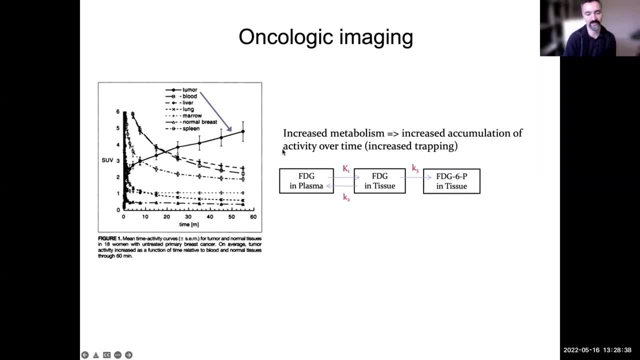 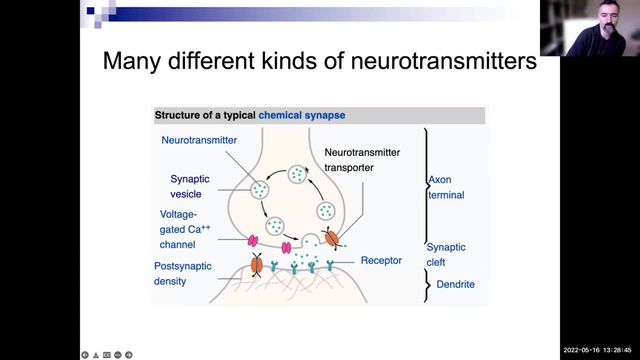 This is the bread and butter of PET imaging in the clinic these days, But again, this is not limited to just oncology You could do. First of all, as you know, there are many different- over 100 different- neurotransmitters, right? 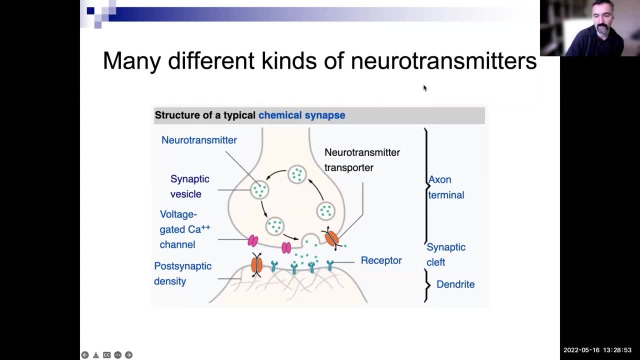 And you could try to study these. And neurotransmitters are interacting with receptors or transporters And therefore you could be studying the. You could be studying neurotransmitters if you're able to, For example, create certain molecules that bind to receptors. 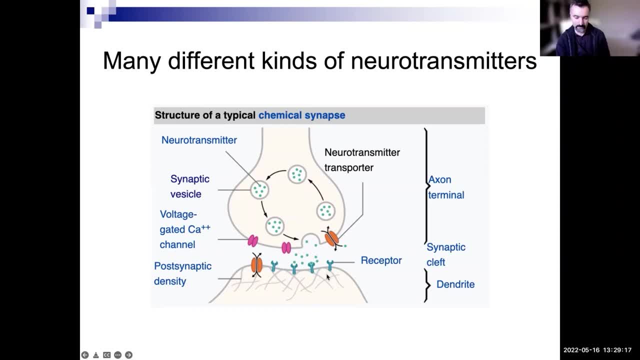 Imagine you've got dopamine receptors, D2 receptors. If you create certain molecules that compete with dopamine, that also binds to dopamine receptors, you could be, for example, indirectly measuring how much dopamine is in this space. So you could be labeling receptors or transporters and therefore studying the dopamine levels. 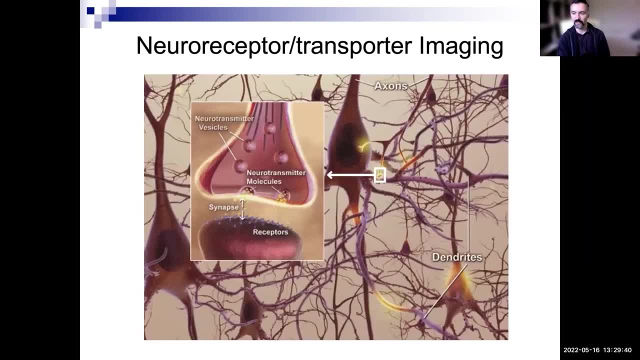 For example, this is very, very popular. This is commonly used in Parkinson's disease and others. So here again you could be doing imaging of the neurotransporters or neuroreceptors And through that, studying many different aspects of neurotransmission. 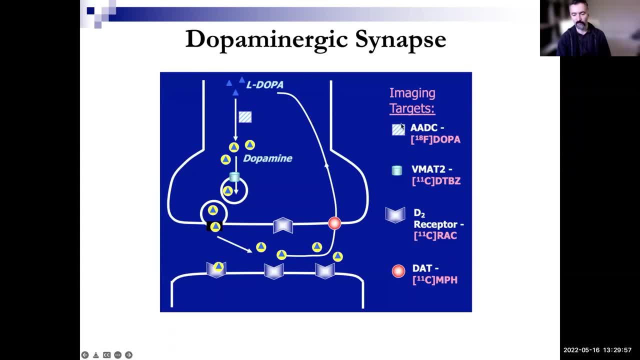 Just showing an example, Many things commonly used in different diseases, including Parkinson's disease, as I mentioned. So you've got dopamine that is being delivered through the vesicular monoamine transporters. So you could be imaging that Or you could be studying the dopamine levels. 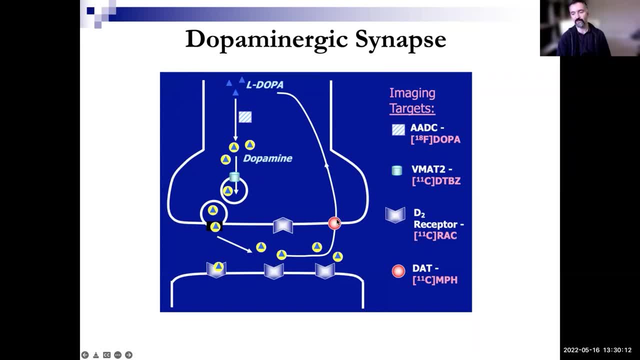 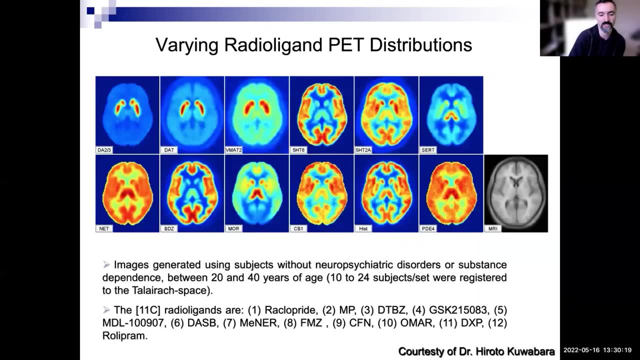 Or you could be studying the dopamine receptors, Or you could be studying the dopamine transporters And, through that, studying what's happening to the neurotransmission in the brain. You know what is going on with the brain of a Parkinson's disease patient. 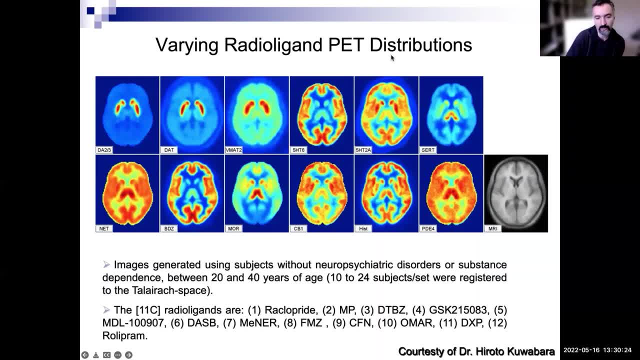 In those years when I was at Hopkins, we were looking at a lot of different things, different aspects, different radiopharmaceuticals for brain imaging. So here are many different examples of imaging: dopamine receptors, The dopamine transporter, The vesicular monoamine transporter. 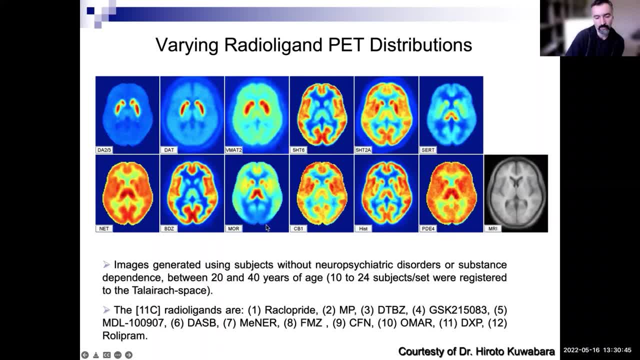 Serotonin, Mu, opioid receptors, The cannabinoid receptors, The so-called marijuana receptor, Many, many different things, And so you could be studying those using different radio-labeled molecules. Like, in this case, for dopamine receptors, you could be using Ractopra. 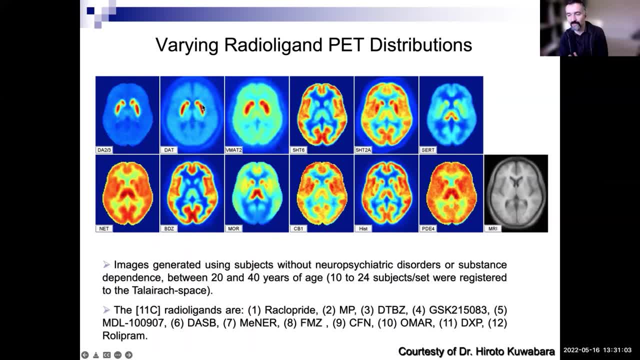 Or methylphenidate for this Again. so for different neurotransmitters and different neuroreceptors And neurotransporter phenomena, you could be using different molecules. So it's very tremendously exciting And you could be studying this. Cardiac applications. 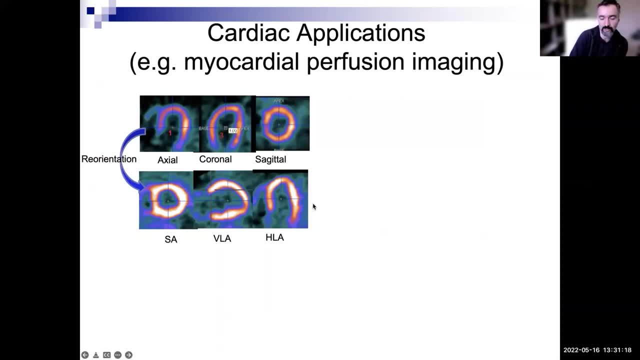 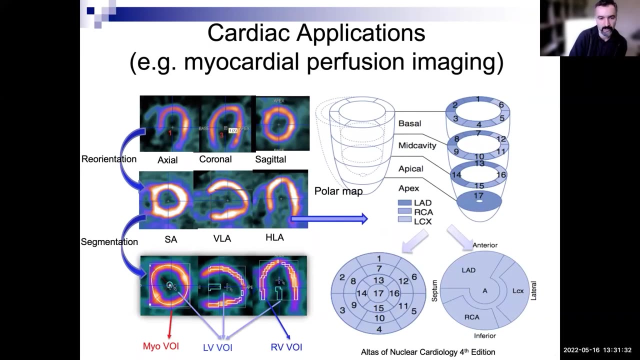 Myocardial perfusion imaging is very, very popularly done, as you know, in our field, In nuclear medicine imaging, So I won't go through those details, But there's tremendous value, as you know, in myocardial perfusion imaging using SPECT, for example. 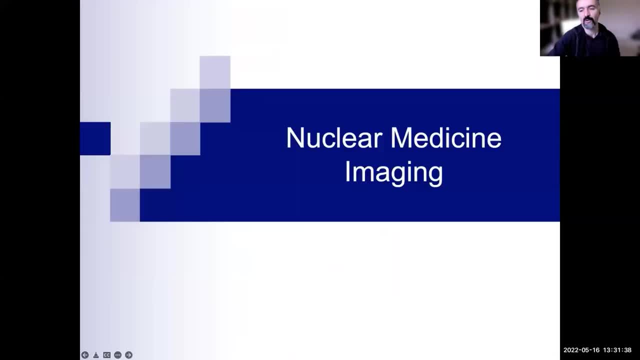 And PET imaging. Okay, So let's actually talk a little bit more about this. How do we do nuclear medicine imaging? Any questions so far? Feel free to stop me, please. You can see that I'm quite excited about this field. 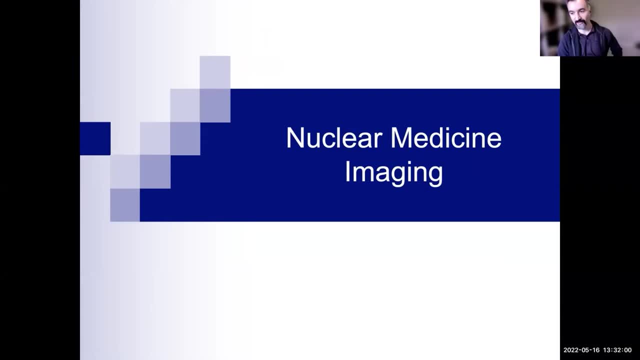 Because I feel that it's often underestimated. You're more than welcome to come and visit our facilities. I'd be delighted to show you around If you still haven't seen the imaging facility here we have at BC Cancer Particularly to nuclear medicine, imaging and therapy. 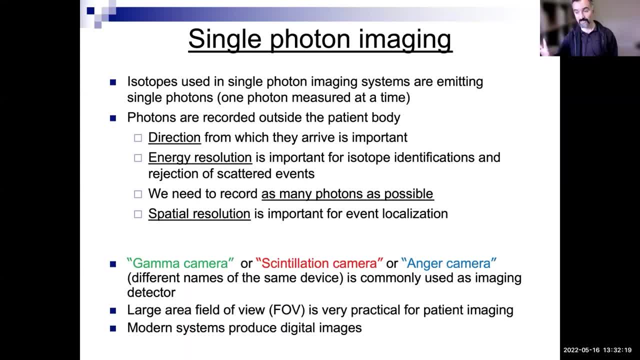 So let's talk about single photon imaging. PET imaging is dual photon imaging, Anti-parallel photon imaging- There's two photons, But let's talk about single photon imaging. That gives you planar imaging, Gamma imaging And also, in the case of tomography, it's going to give you SPECT imaging. 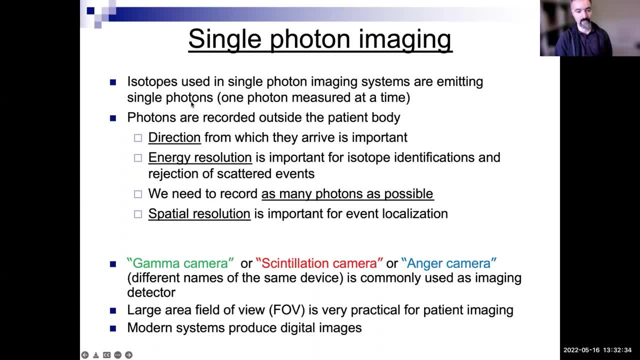 So isotopes are emitting single photons. here, Photons are recorded outside the body. You've injected something or inhaled something. Something's in your body And the photons are exiting your body. The gamma rays are exiting your body, So they have a certain direction. 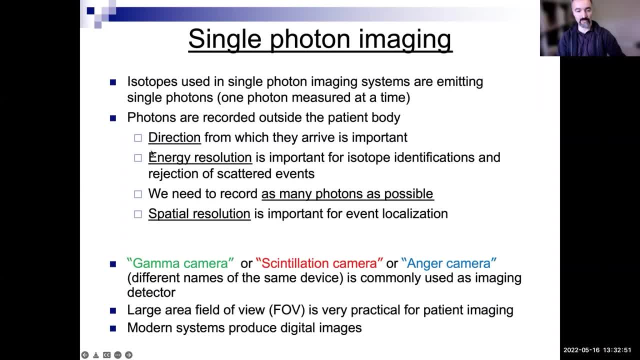 They have a certain You need to have a certain, You need to have the proper energy resolution to be able to know what the energies are of these things, To remove things that have been scattered, That are complicating things, And you really need to be recording as many photons. 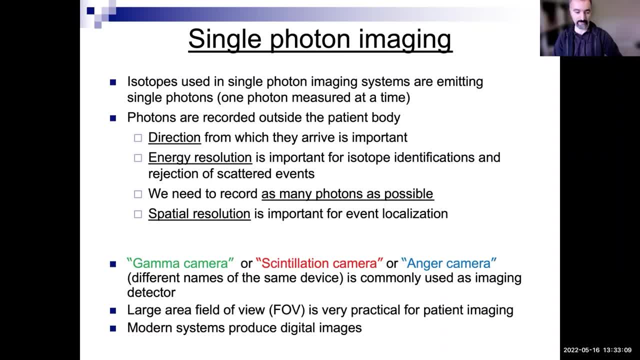 Because you know otherwise you're going to get very noisy images. So this thing is called a gamma camera or scintillation camera, An anger camera. You're going to be learning more and more in this presentation about why we call this a scintillation camera. 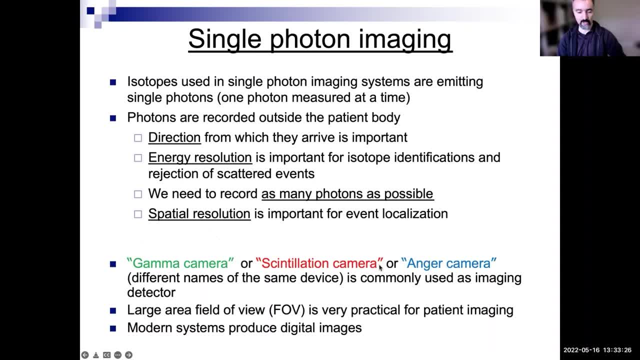 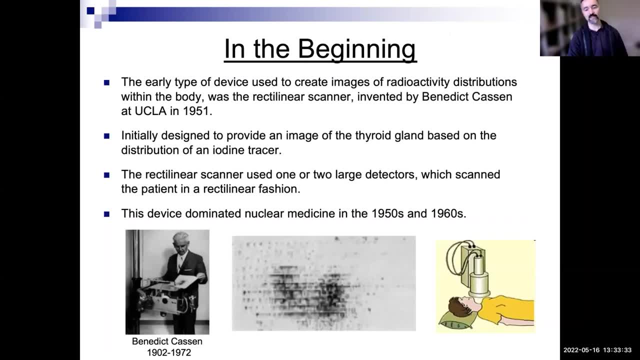 Why we call this anger. Anger is the name of a person. Why is it called the anger camera? What did Mr Anger actually do? So let's talk about these more. At the beginning, We didn't have a gamma camera in this sense. 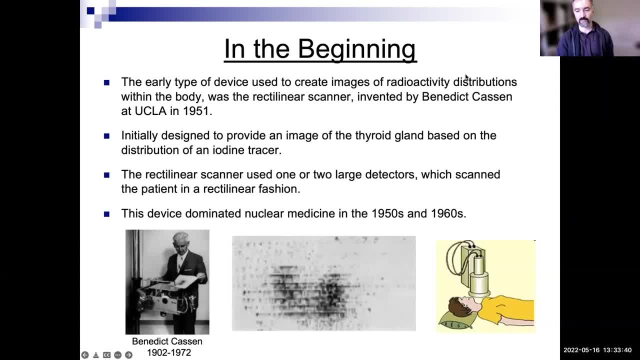 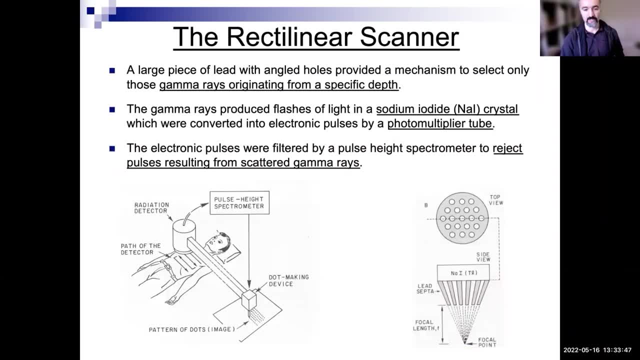 And what we used to have. There was this invention by Benedict Casson at UCLA, Where basically he was, He had this kind of a design where he was only imaging a single point. So it's not good enough, at the same time to be imaging a field of view. 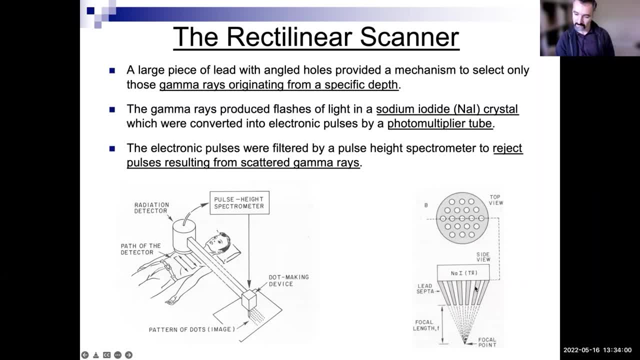 But only imaging a single point Where all these collimators are focused on this point. So all photons coming out of this point he would have been able to see. So if he's doing that, then he has to be moving this over the body in order to image. 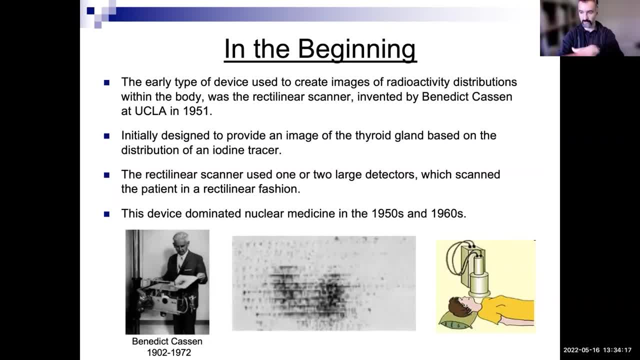 Because at a given time he's only able to acquire a single point in this field that is in front of us. So he used to use one or two large detectors, Maybe one at the top of the body, one at the bottom of the body. 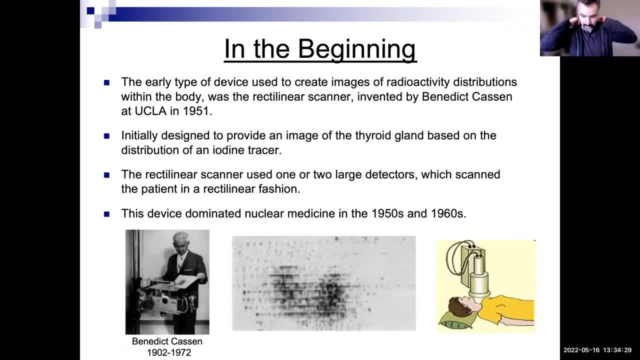 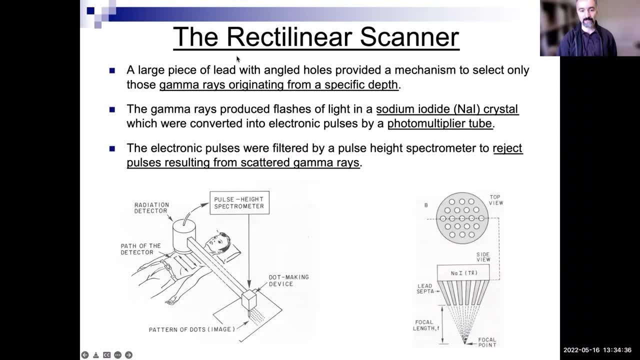 And this dominated nuclear medicine in the 50s and 60s. So again, It's a large piece of lead basically. So the scintillator, the thing that is able to actually detect these gamma rays, That's sodium iodide, for example. 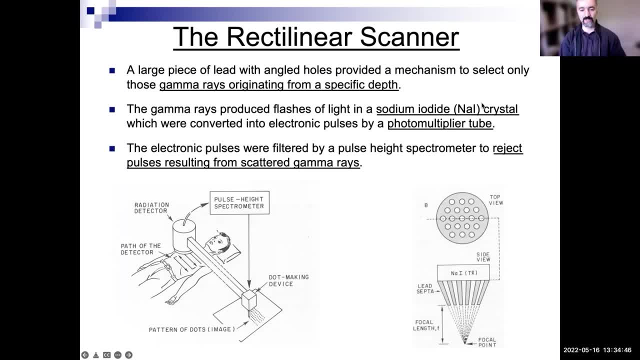 That's a scintillator, It's a crystal, a scintillator, But at the front of it you've got these focused lead collimators That are sort of saying: I can only measure things coming from this point, Anything else from this here, here, I'm not going to measure. 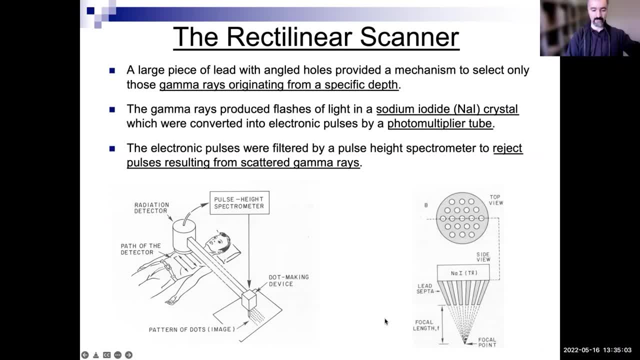 Because my collimators are going to reach this point. I'm going to check it And then again it's rectilinear, So you kind of move like this, Back and forth, back and forth, Until you cover the body. So section imaging. 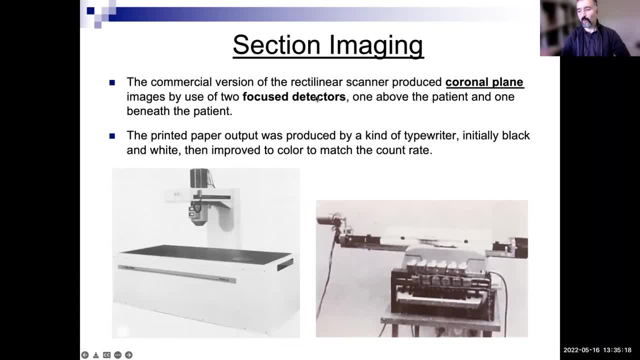 So this used to produce a chronoplane. This is very old stuff. It's just a historical thing. Thank God we don't do this anymore, But this is the historical innovation that, of course, we've built on top of. But let's talk about 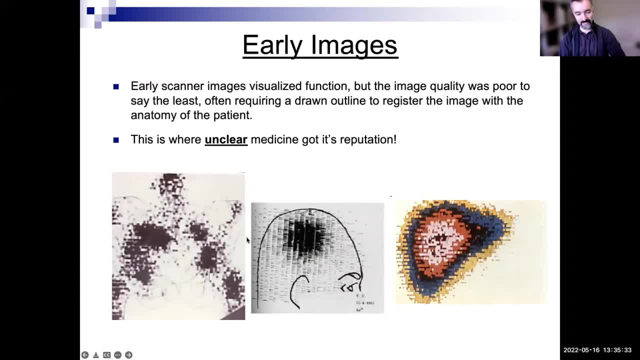 These are the kind of images that we used to get. You see, the feel of a rectilinear sort of going through, And this is actually why there is this joke that nuclear medicine is just playing with the letters. here is unclear medicine, Because the resolution was not good enough. 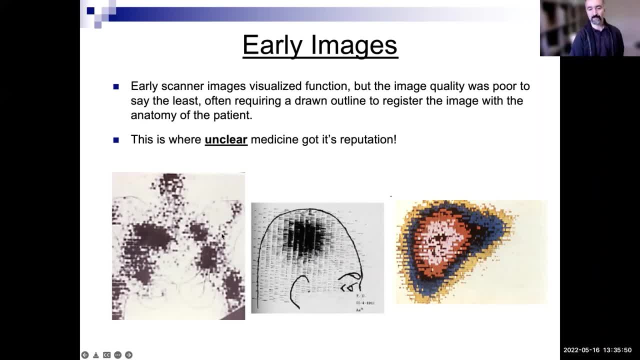 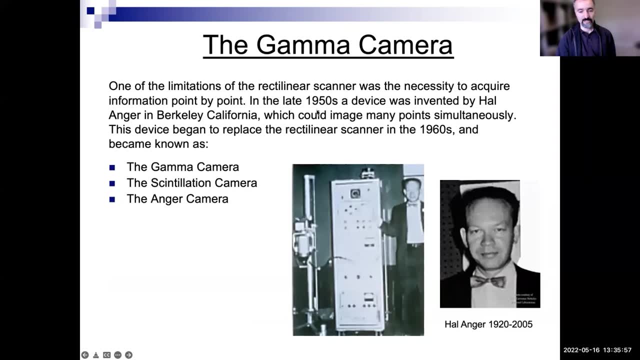 I mean, this doesn't look good at all. right, But we had a major invention by none other than Mr Hal Anger, Who invented in the late 50s something in Berkeley, California, That we are now calling the gamma camera or scintillation camera. 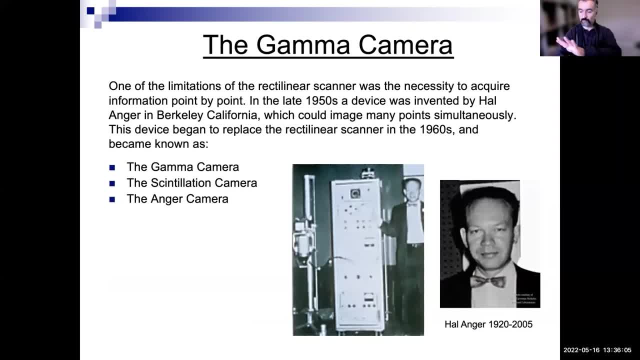 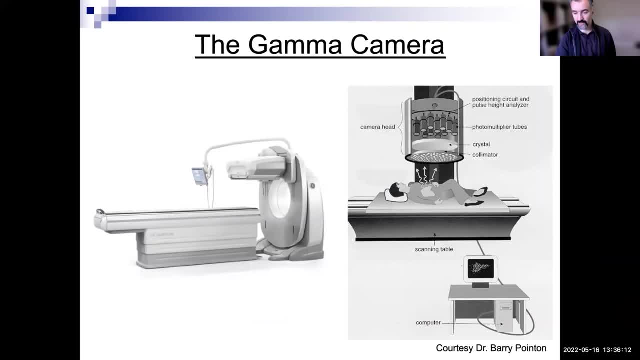 The beauty is at a given time, it's imaging the whole plane, The whole field of view, Not just a single point. So how did you do that? And this idea, to this day, is being used, So let's go through that. 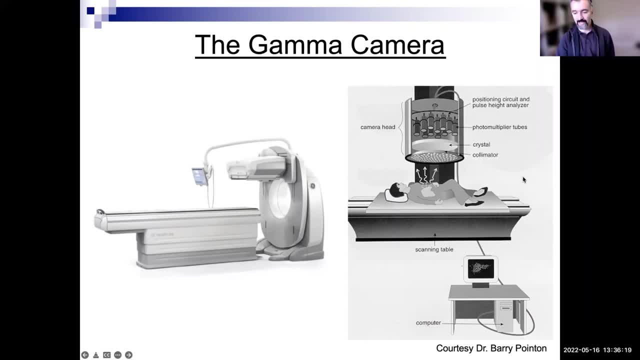 The gamma camera. How does it work? If I have to break it down, I would say: these are the steps. Here's the patient. You've got a collimator, Not like those focused collimators I mean. So it's a collimator that actually is parallel often. 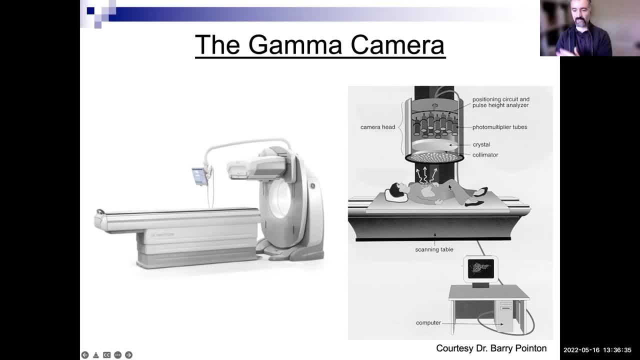 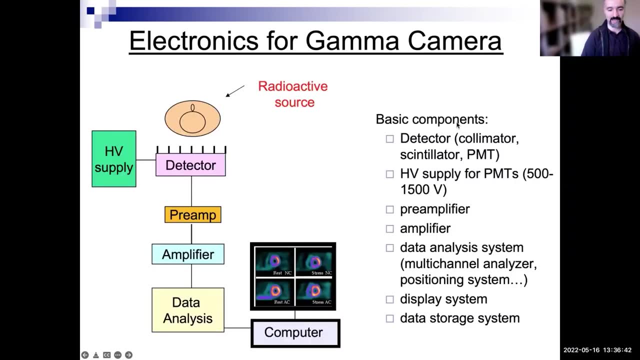 So anything that is going at 90 degrees or give or take can enter it. You've got a crystal, You've got a photomultiplier, So how does this actually happen? So let's look at it another way. You've got the patient. 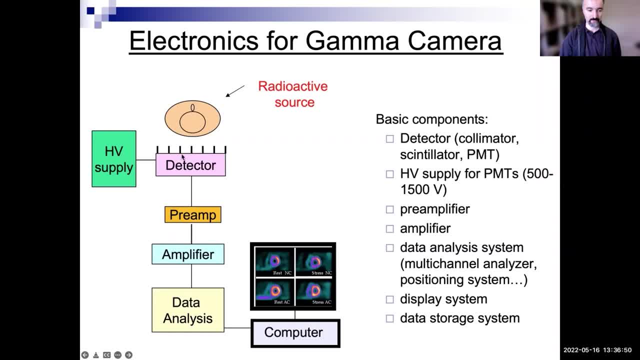 You've got these parallel collimators, You've got the detector or the crystal or a scintillator, And after the photons pass through these collimators it's going to detect them, And then you have some electronics at the back that amplifies the signal, converts these. 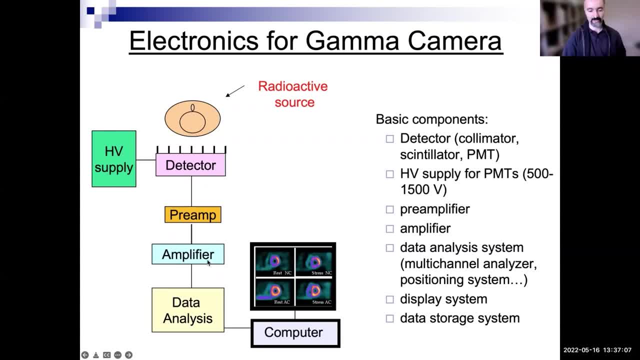 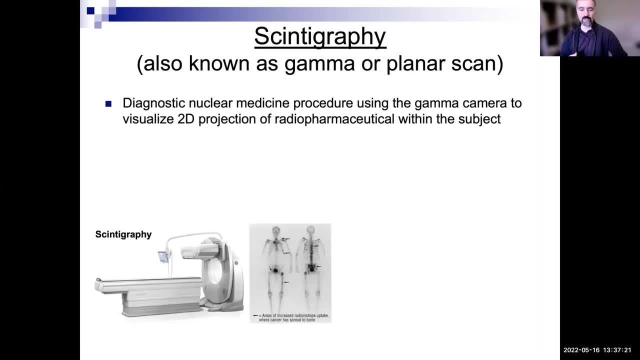 Essentially, this gamma ray is being detected, ultimately into electric signal that you obtain. Yeah, So you've heard of the term scintigraphy, also known as a planar scan or a gamma scan. Yeah, gamma or planar, Basically it's planar. 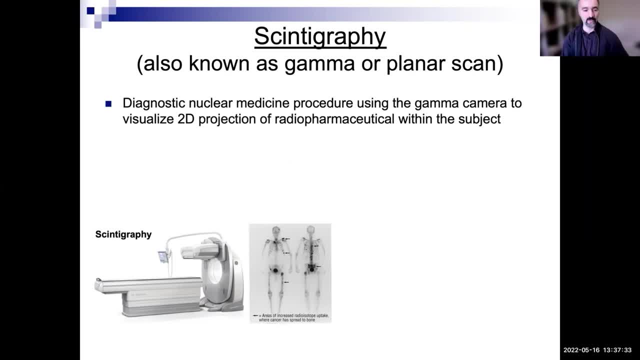 It's like the equivalent of an X-ray, So this has been used for diagnostic imaging, for example to visualize a 2D projection. So it's analogous actually to plane or projectional X-ray radiography- Very analogous- The difference being that here the source of the radiation is inside the body. 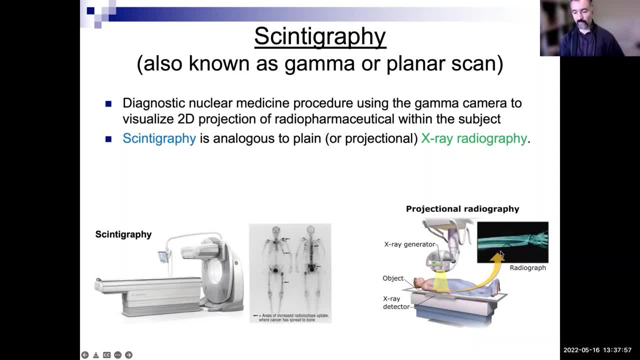 Whereas in X-ray radiography, as you know, the source is outside the body, passes through the body, But it's very analogous to it. So that's scintigraphy for you. The difference is that again in our field, in nuclear medicine, we're dealing with emission. 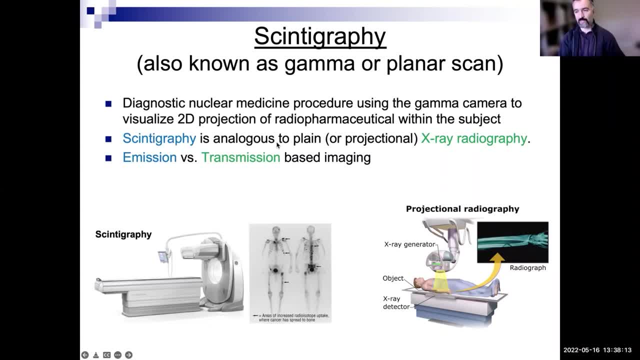 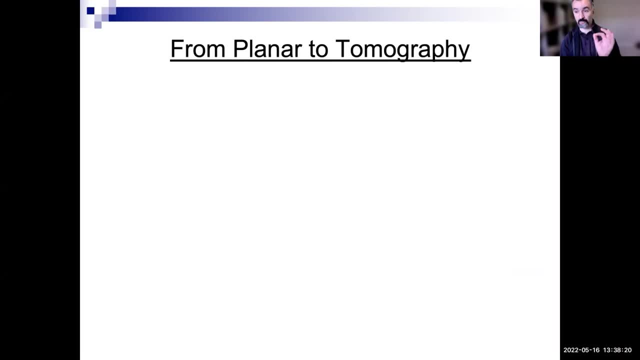 Whereas in X-ray imaging we're dealing with transmission, because the source is outside the body. But we want to move. If you want to move from 2D imaging to three-dimensional imaging- three-dimensional imaging that you actually visualize depth- then you need tomography. 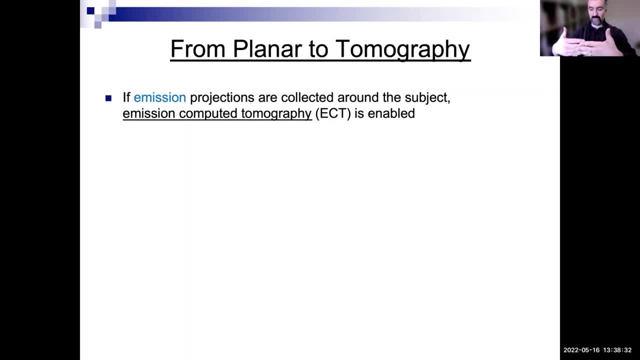 So in this case you're not just acquiring at a fixed angle, You're going to be rotating around the body, so you're acquiring at different angles. So this is called emission computed tomography. You've heard of computed tomography CT. 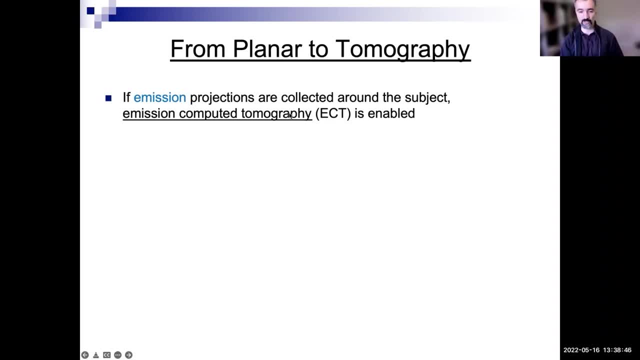 But in our field we call that emission computed tomography, To emphasize that again, the source of the radiation is inside the body. So for emission gamma rays this leads to single-photon emission computed tomography or positron emission tomography. 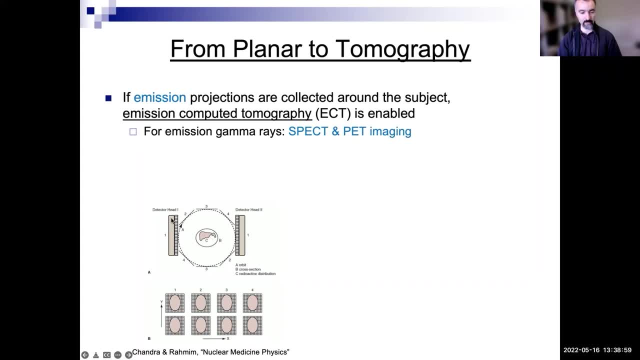 And again you've got the radiation coming from inside the body. You've got planes, And the planes can, for example, rotate around the body- spectra, image. But if it's transmission projections that are collected, well, that's transmission, computed tomography, or commonly known as just as computed tomography. 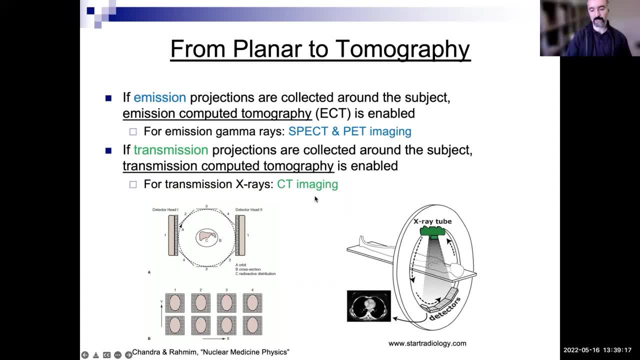 So if you're dealing with X-rays, then we call that CT imaging. So again, it's very analogous. Synthegraphy is analogous to planar imaging, whereas PET and SPECT imaging are analogous to CT imaging because they're tomography. 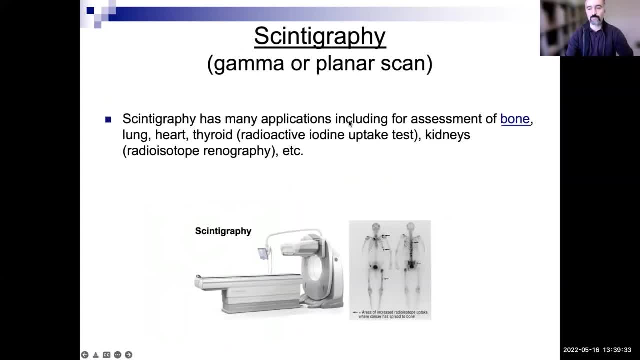 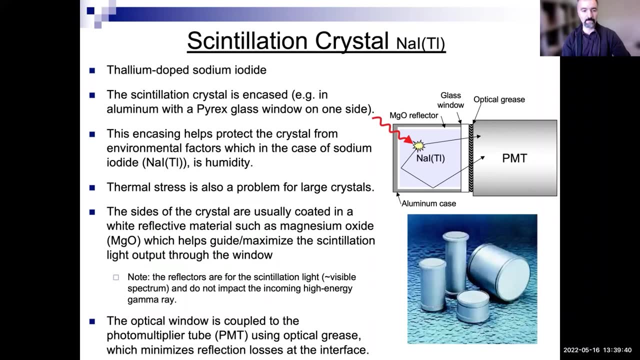 So it has many applications for assessment of bone, lung, heart, thyroid, kidneys- many different things. And let's talk about the crystal itself: Crystal or the scintillation crystal. This crystal is the crystal that you see on the right. 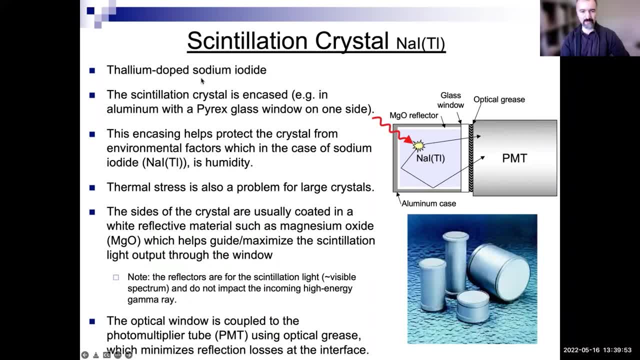 Because I'm assuming you saw, on the left, my video one year ago. I was talking about this crystal and you saw in the video one year ago that it contains a protein and it's basically a phytochemical that contains a protein. So you see, it contains a protein. 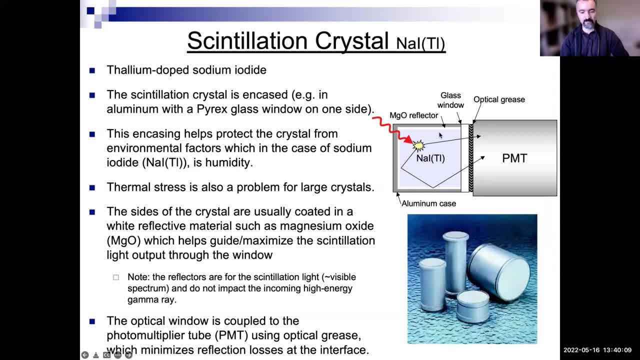 and it is with a phenotypal. it's a methyl phenotypal, that is a phytochemical, that is a phenotypal. So this crystal here is a phytochemical with reflexive material, because once a photon comes in, 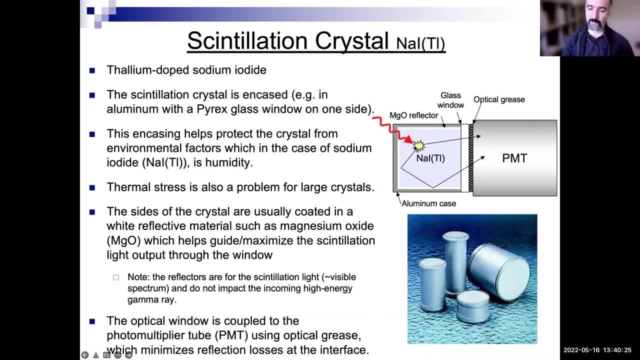 sorry, a gamma ray, gamma ray. once the gamma ray comes in here in the crystal, it creates so-called scintillation. just hanging there with scintillation is almost to really boil it down. it means you absorb that really high energy radiation. 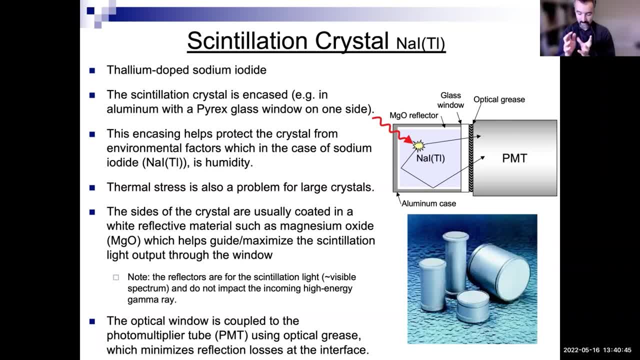 gamma ray coming in, 140 KV, for example, coming in, you absorb it through some kind of molecular excitation and then that molecular excitation comes back to the sort of the base level and it emits much, much lower energy photons. 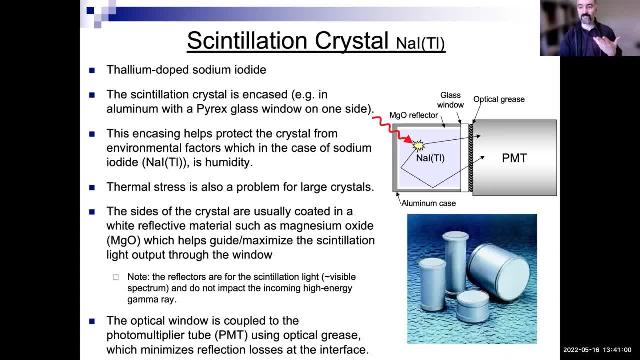 but many of them, And so it scintillates right, You can actually see it visually- And so these much less energetic photons. they may start going in different directions, so you may be coding this so that they're not leaving the system. 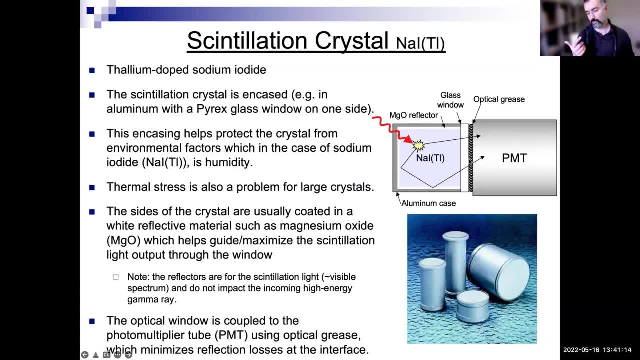 but they end up in the PMTs. And what the PMTs do is that they absorb those photons, those scintillation lights, and they amplify, they convert them to electric signal. We'll get there Just hanging there, hanging there. 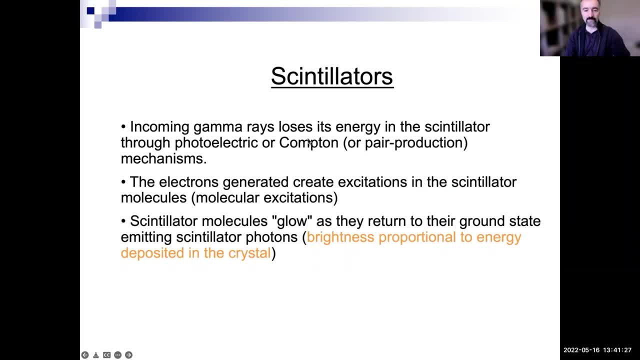 So scintillators, how do they work? You have incoming gamma ray, which is highly energetic, that loses its energy in the scintillator through certain mechanisms, and those mechanisms end up exciting the molecules of the crystal And those molecules as they're excited. 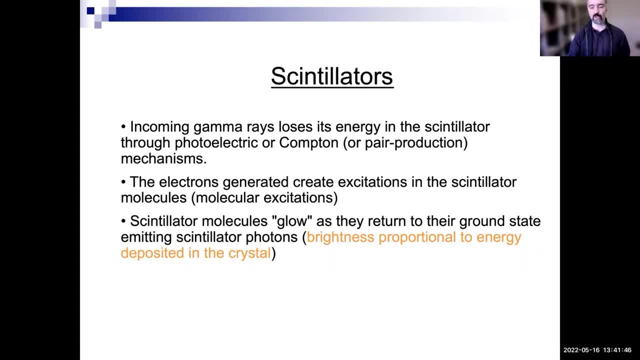 when they come back to the ground state, they glow, And that glow is the brightness of it. The number of photons they emit is proportional to how much energy it was, So you can actually know what was the energy of the photon that I just absorbed. 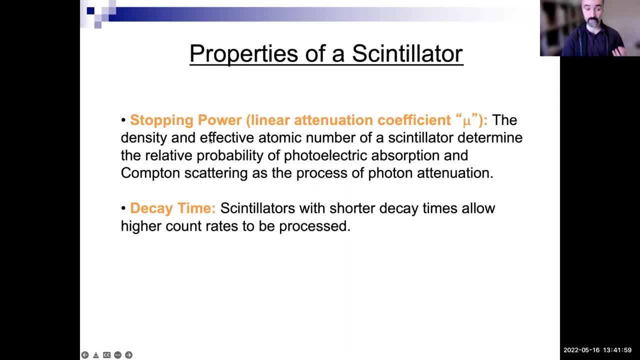 So what are some important properties of a scintillator? Well, they have to have very good stopping power. They're very energetic. Hundreds of kiloelectron volts coming in- hooray. You gotta be able to stop them. So you gotta have dense material. 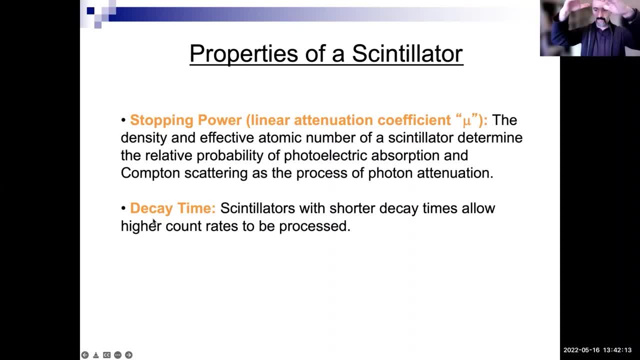 You gotta have something that when it glows or when it gets excited, and come back to ground state and glows, that doesn't change anything. It doesn't take too long, Because if it takes too long it's almost like the processing time is too long. 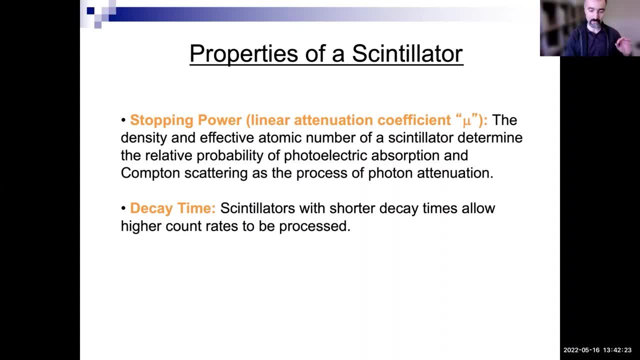 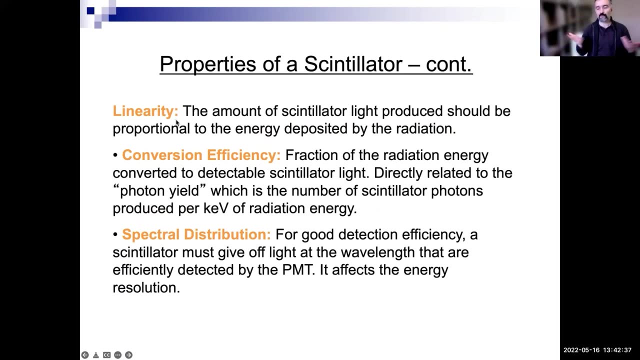 So I'm not open to more events coming in. So you want it to decay quickly So you're able to accept more events coming in. Linearity is a technical alternative. You kind of want to be able to map what was the energy of the thing that came in. 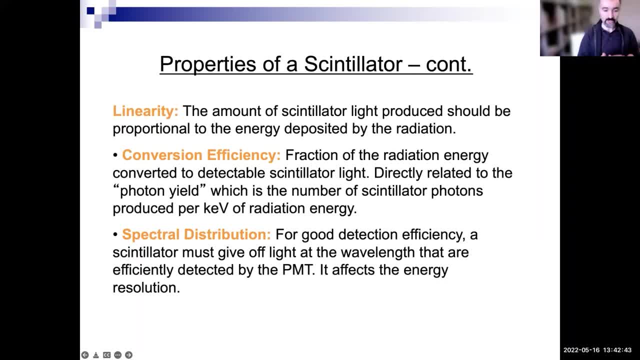 Conversion efficiency. Not only do I want to absorb you, I also want to convert you into scintillation light- lots of it- So I'm able to detect and know how much was the original energy. It has some good spectral distribution, meaning the energy resolution should be good. 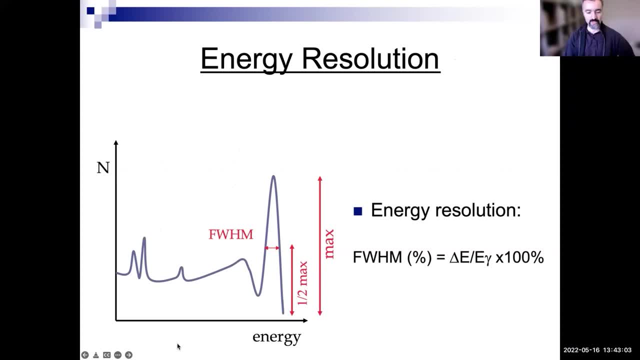 So let's show you some examples. So this is the energy of the incoming ray. This is the number of this could be here, for example, the number of photons at different energies that you're detecting. The original source was here, But what you end up getting is not just a single spike. 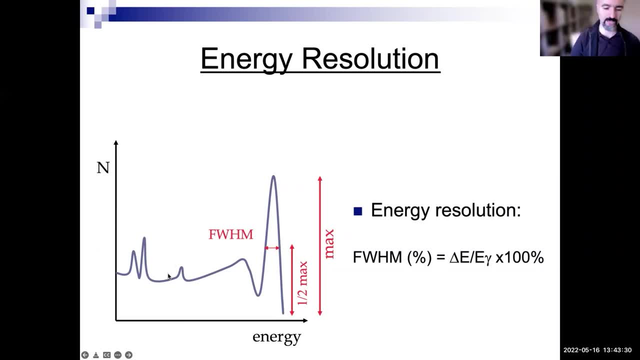 You're getting a whole range of stuff that are kind of strange, Like I really don't want to be seeing stuff here because my incoming energy was here, So I do get a bit of a broadening. That's like the energy resolution of the system. 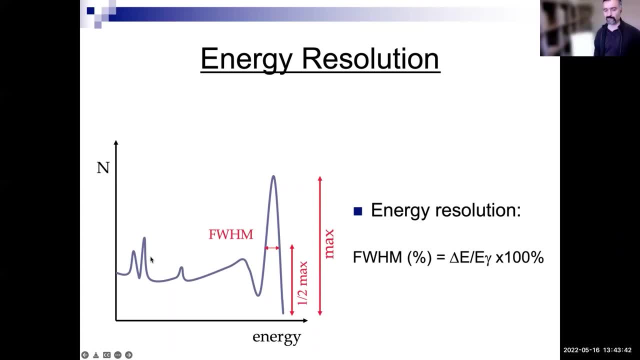 But what are all these things here? These are all the unwanted stuff, But we'll come back to that. But the energy resolution is this: You want this to be as small as possible. The percent full width at half maximum ought to be as small as possible. 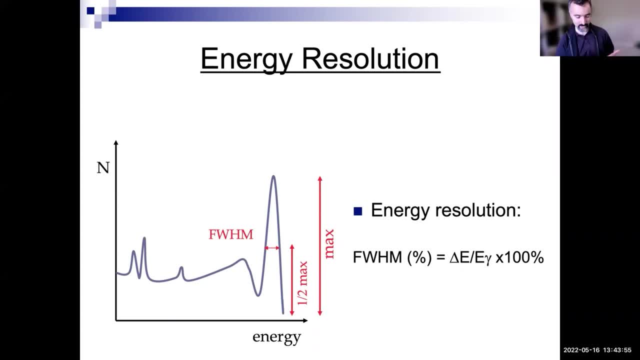 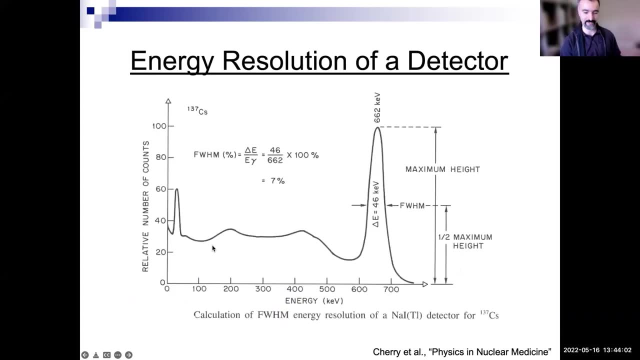 because that allows you to really know what was the original energy very well, so that you can reject all these weird unwanted scattered events. Okay, so you measure the width at half of the maximum. In this case it's 46.. So 46 divided by 662, if it's, the original source was 662.. 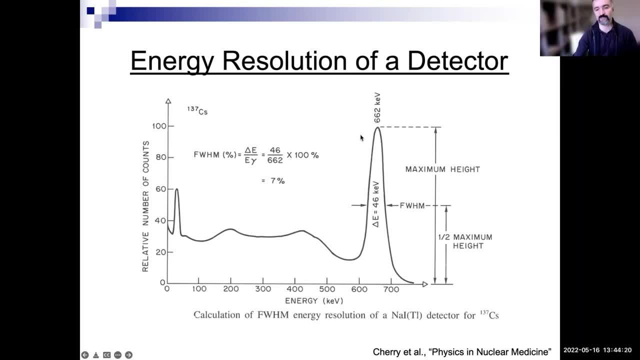 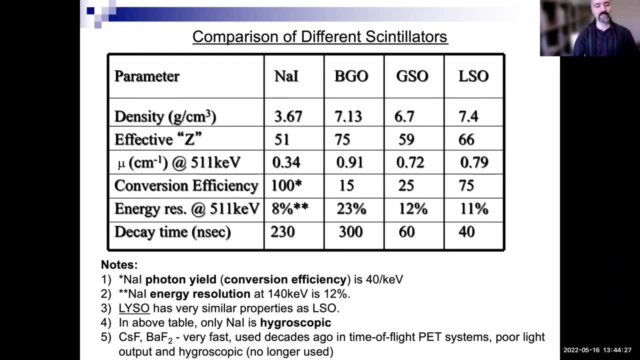 And this example tells you that this kind of energy and with this kind of a whatever detector, I have a resolution, energy resolution of 7%, which is actually pretty good. So many different scintillators are out there: Sodium iodide I kept mentioning, used for seeing a photon. 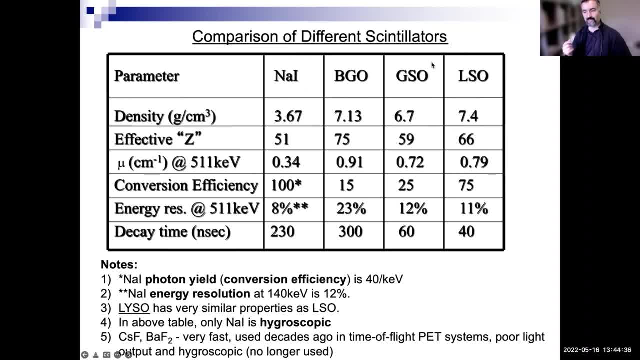 But these are example of scintillators using PET imaging, because PET the energies are much higher and you need better scintillators. So, but you see how the density is here, but whereas for PET we really need to use denser material. 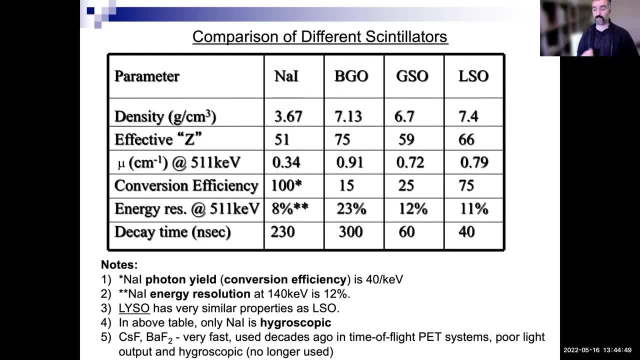 because we wanna stop that really energetic light, And that's why one reason PET scanners are more expensive is you gotta have denser material, You gotta have more expensive crystals to absorb the light. The effective Z or Z number is important. What else do I wanna really mention here? 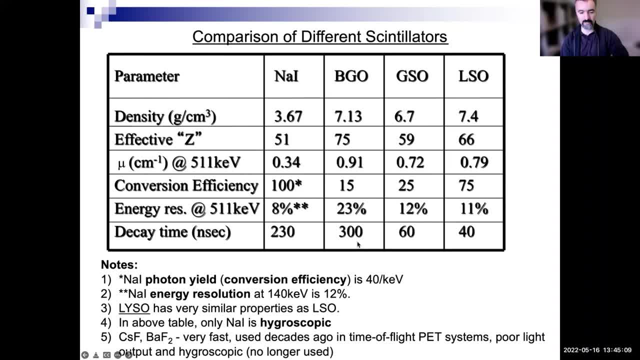 The energy resolution looks there typically in this kind of scale. Look at the decay times in nanosecond. So like, for example, LSO, which is very nice, right, Because it's not taking too much. It's almost like the processing time is not that long. 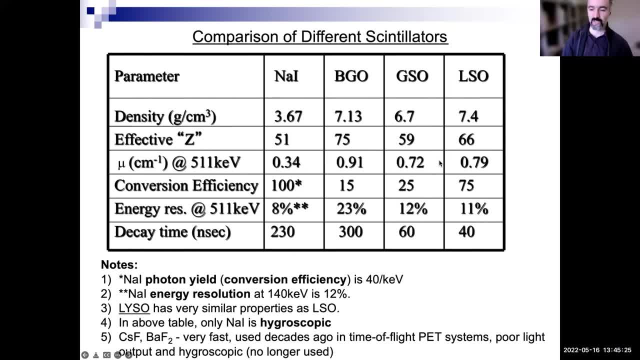 And the attenuation coefficient. essentially, you see how it changes. So obviously these things are better than sodium iodide at this very, very high energy, which is the energy in PET image. So this is why sodium iodide is not a good crystal. 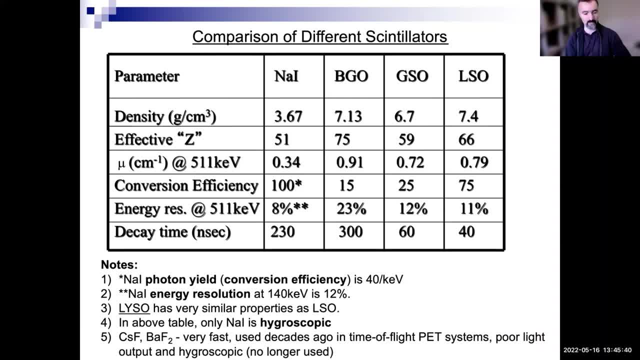 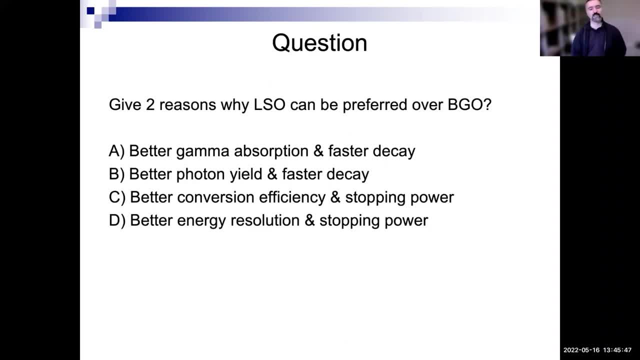 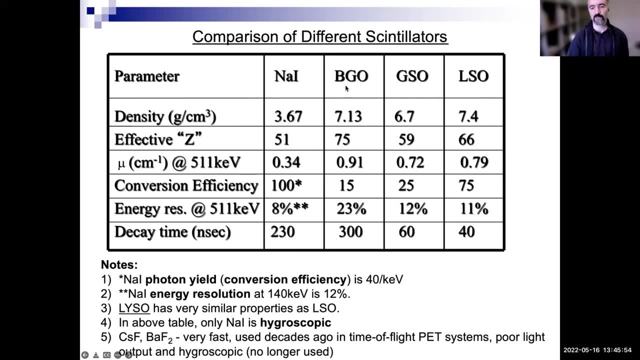 for PET imaging applications, but it is great for, you know, for speccing a full-time imaging. So if somebody was asking you, give two reasons why LSO is preferred to BGO In PET imaging. people used to use BGO. 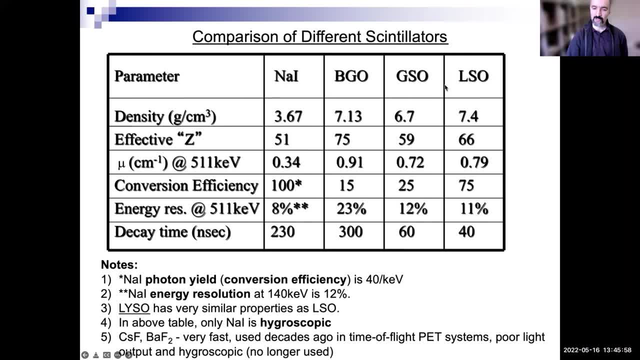 but then they started using LSO. Let's look at it together. What are two reasons why LSO is better than BGO? You see, the densities are almost the same. Effective Z values are not that different. At the same time, the attenuation coefficient is almost. 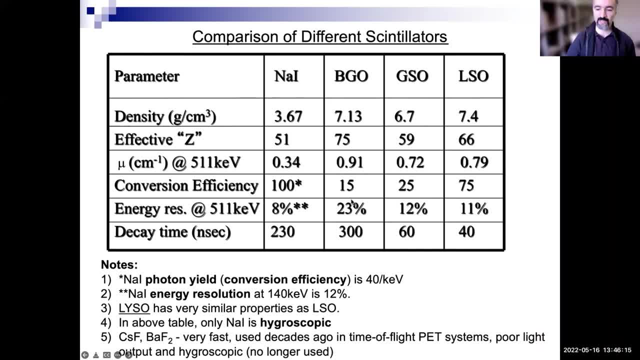 in fact slightly even lower, but there is this number that is really higher, the so-called conversion efficiency, which says let's take sodium iodide as the reference. You know the number of photons that are emitted in this scintillation phenomenon. 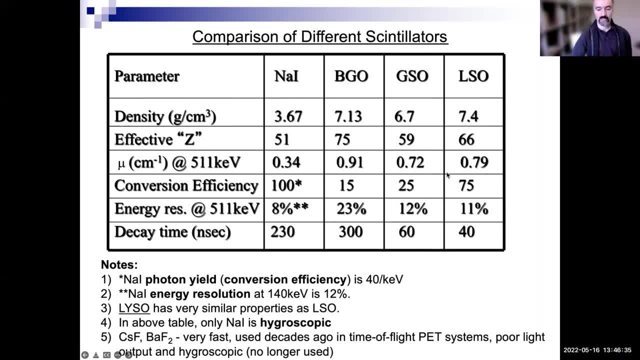 Well, LSO produces a lot more photons. So the photon yield, or the conversion efficiency, essentially iodide is. for every kiloelectron volt you produce 40 photons. So if it's 140 kiloelectron volts, 140 times 40,. 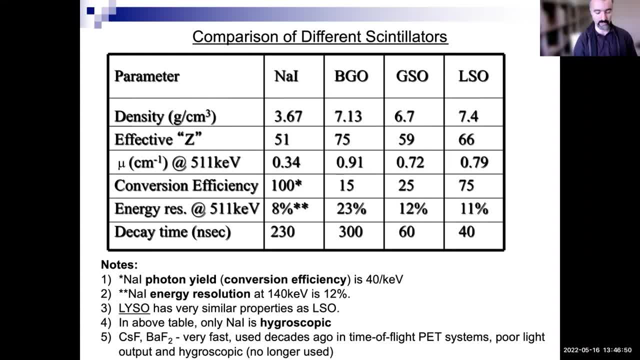 that's a lot of photons that you produce, right? So 140 times 40 is around five 6,000.. So for every single ray that comes in, this produces about 6,000. So let's call that a hundred percent, like, just as reference. 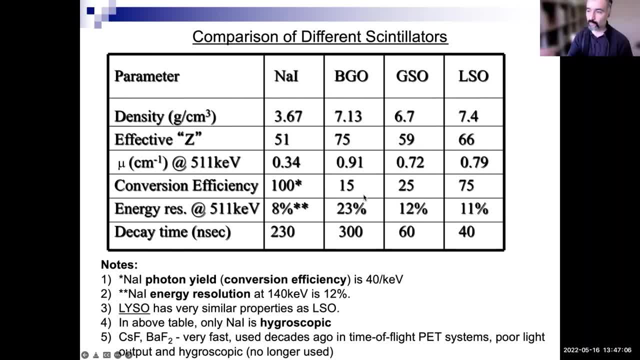 LSO produces a lot more than BGO, So a lot more photons are created. So that allows you to do better imaging, better signal, less noise. So that's one advantage. The other advantage is you see the energy resolution smaller because there are a lot more photons created. 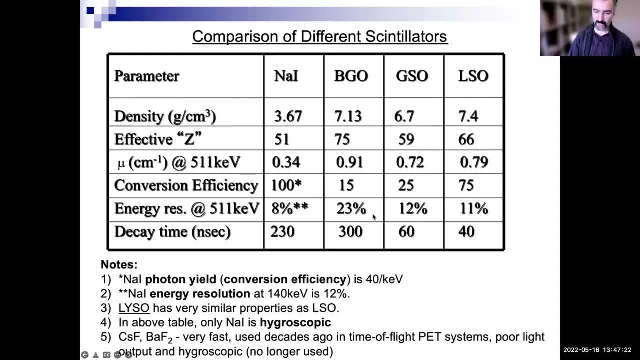 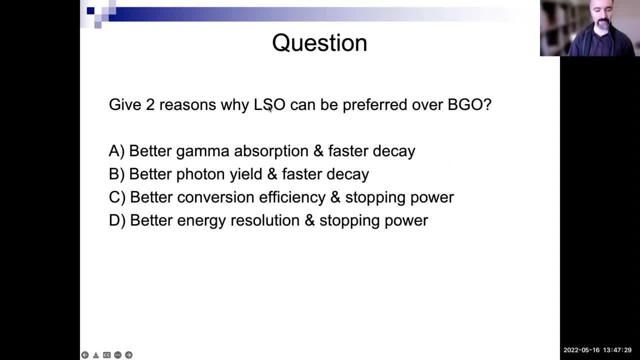 turns out to actually give you better signal to noise ratio, better energy resolution. So the correct answer here would be better See Better conversion efficiency and not stopping power. So the stopping power is That's okay. Yeah, Good guess. 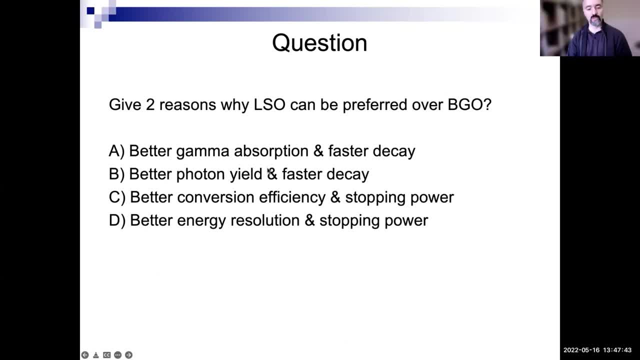 Good guess. Faster decay, that's right. So the absorption is not better, The stopping power is not better, but the photon yield, what it produces, is better and it is faster. Was that Tracy? Thank you for answering. So- It was Ally. 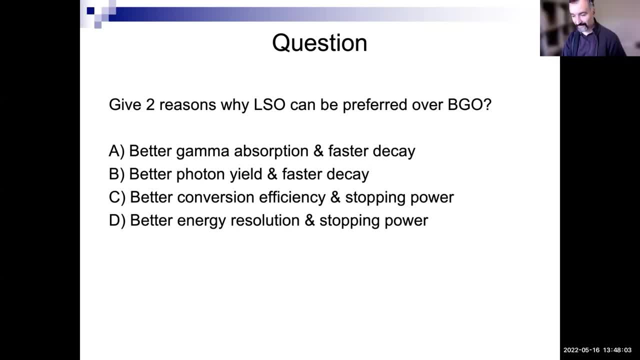 Oh, You're what You're with Ally. No, it was me Ally. Oh, Ally. Oh, I'm sorry, It's okay. Okay, um, thank you for that. thank you for for for answering. so b, okay, so multiplier two, so what. 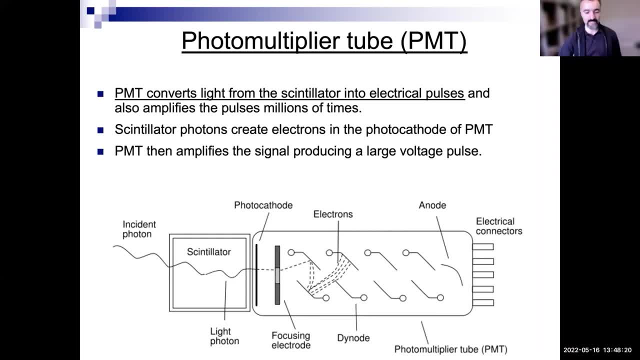 what on earth are pmts? so pmts once you're producing scintillation light. so again you stop the really high energy photon, convert it into this much, much lower, but lots and lots and lots of photons. well, photons are entering here, but you want to get a signal that is electric. 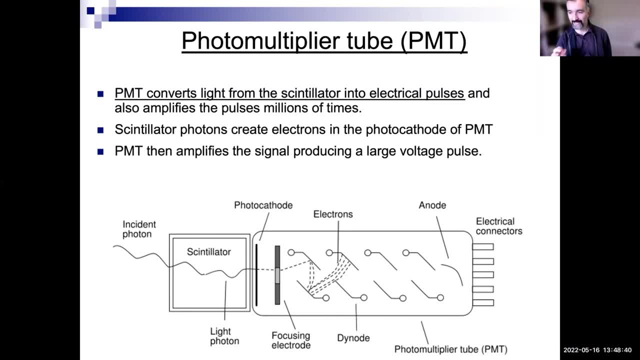 not photonic. like the electric circuits work by electrons, not by a photon. so then you, you use a pmt for that. the pmt takes the incoming light, has a photocathode that basically uses a photoelectric effect. that photon comes in, you let uh, electrons go out. this is a photoelectric effect, this is. 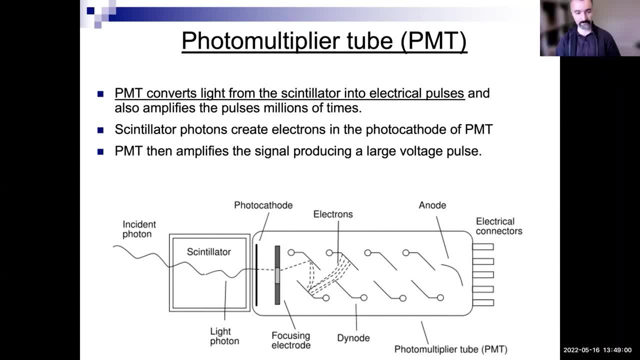 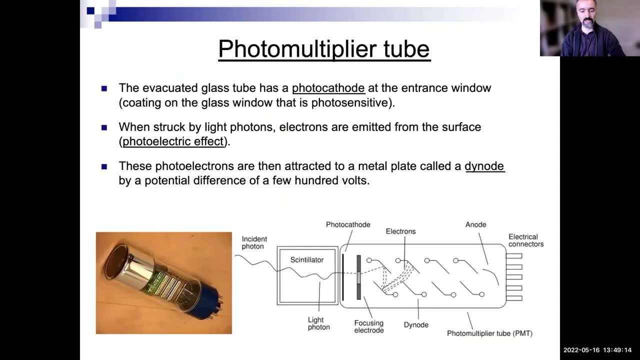 what einstein won his nobel prize for, because he studied that effect. um so, um, so you produce these photons, and then you have these, these dinodes that amplify the signal. okay, so, so here are examples of the pmts. and again, so, so, so you have a photocathode and then, when struck by light photons, the electrons are emitted from the 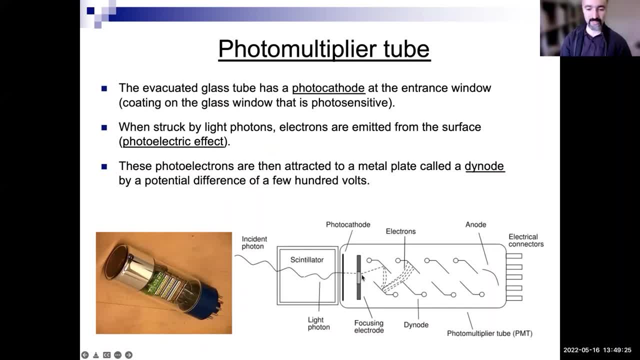 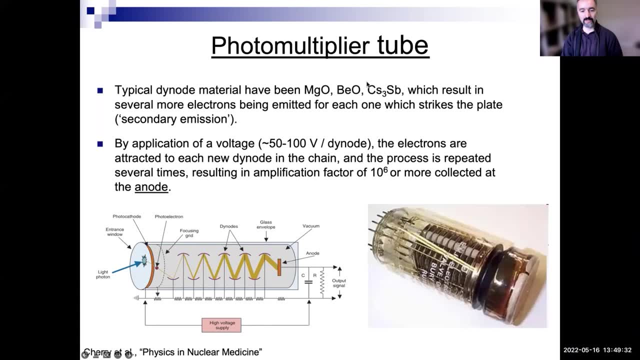 surface. so this is a photoelectric effect. and then these photoelectrons are then attracted to these metal plates which are called dinodes, and the dinodes amplify them. now, typical diamond material, like examples here. essentially, through this example, here is a photoelectron. it's something called secondary emission, it's a phenomenon, it's. 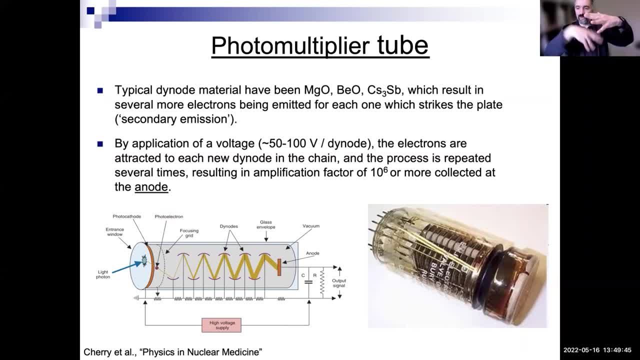 like you've got this surface. you hit it with a single electron, it releases like three, four, five times as many electrons. it's a secondary emission electron to electron, but it's amplified electrons. so you enter here, let's say, with a single electron, amplified, amplified, amplified, amplified, amplified, until here you get this substantial signal, that is. 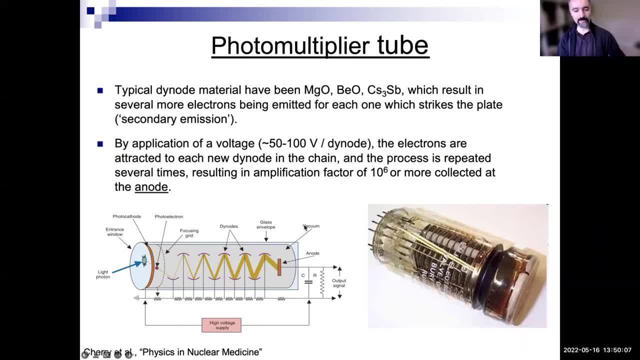 detected, because if you only have a single electron emitting, you couldn't. that's, that's not going to be enough signal. so so this is the second emission that we have right now. but PMTs amplify, And so you apply a lot of voltage, like you, let's say 50 to 100 volts per di nodes. 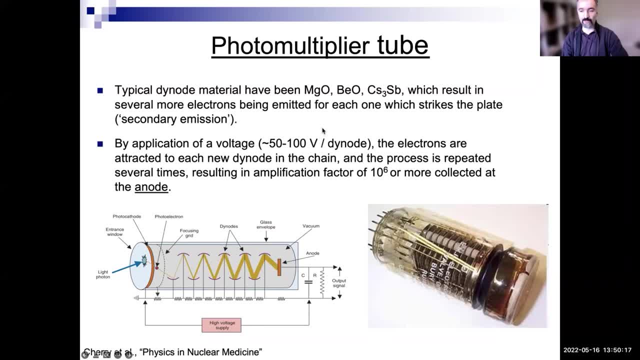 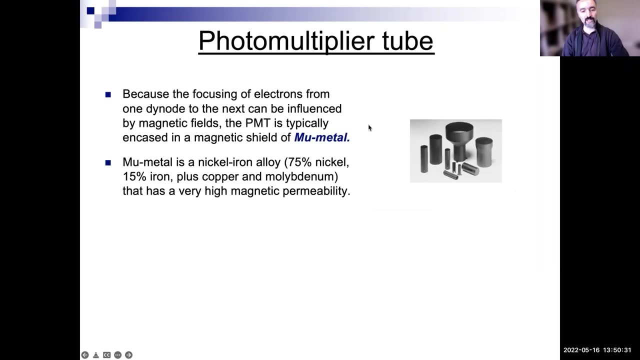 So if you have like 10 di nodes, you're gonna need like a thousand volts here, So you need high voltage supply. Okay, so you get significant amplification. Now one of the issues is that PMTs can be influenced by magnetic fields. 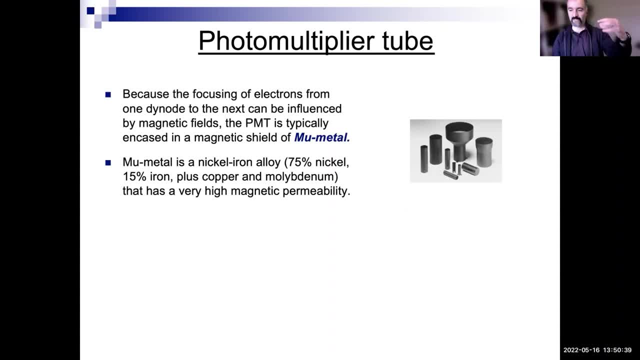 Why? Because, remember, you've got electrons moving. If an electron is moving and there is a magnetic field in there, the electrons can be distorted in their movement. An electron in the middle of an electric field can move in weird ways, Or actually there's laws for that. 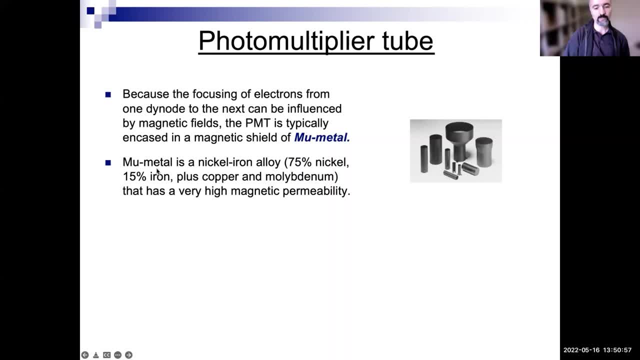 So they tend to use so-called mu metals, which is kind of- here's an example- like nickel, iron alloy As an example to increase the permeability, Or sorry. so yeah, so here's a measure of the permeability. 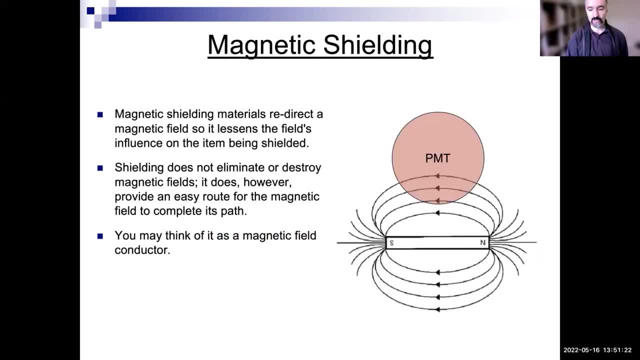 Yeah, yeah, they have very high permeability And what they do is that if you have a magnetic field, for whatever reason here, once you use these, they kind of redirect the magnetic field along this direction, So they lessen the field's influence. 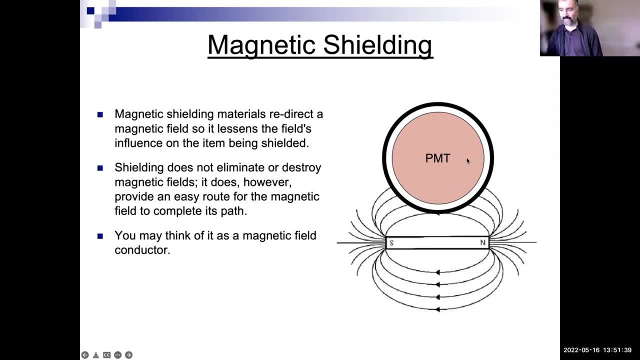 on the items. They kind of shield the PMT from the Earth's natural magnetic field and other things nearby. Now they cannot do magic if there's just too much magnetic field. If you do PET-MR imaging, which is something people do, 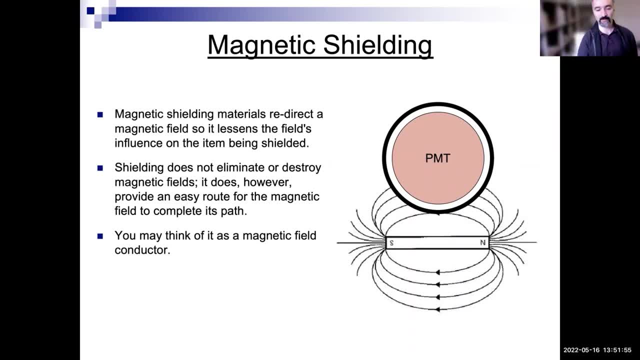 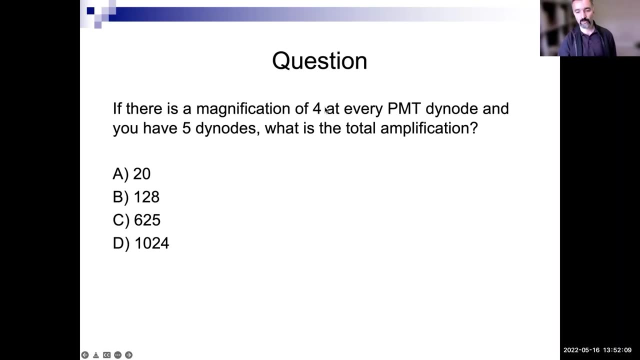 then this is not good enough, Because a magnetic field like one, two, three Tesla is not gonna be. it's too strong for this, But for lower ones it's good enough. So here's a question for you: If there is a magnification by a factor of four, 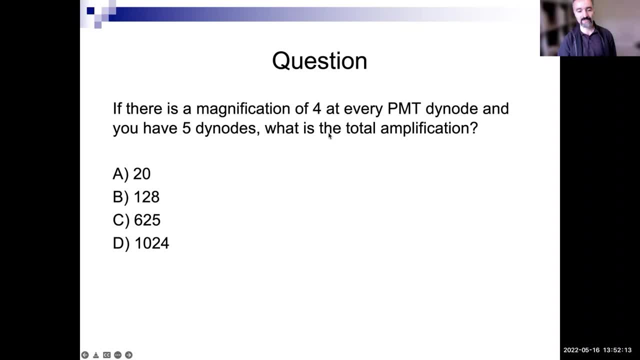 at every PMT dinode and you have five of them. what is the total amplification? How would you do this? Even if you don't have a calculator, how would you do this? Is it like four to the five? So is it four to the five or is it five to the four? 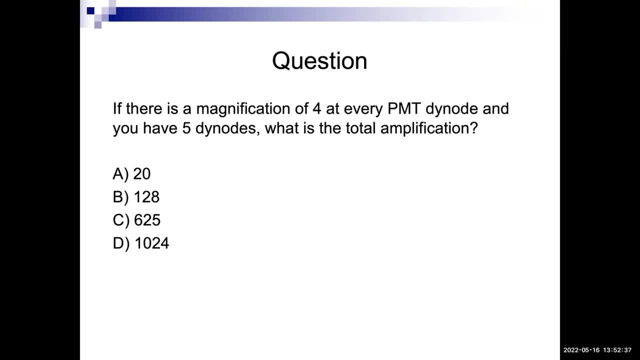 Which one is it? Five thirds and a half? Can I know? Oh, You might've said it right. Five to the, I don't know. five to the four. No, I think you said it right before, Because it's like at every dinode, it gets multiplied by four. 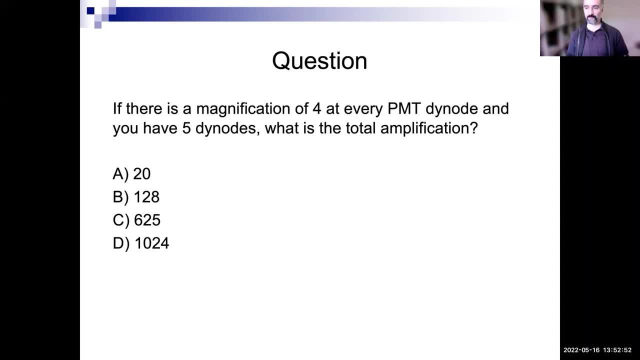 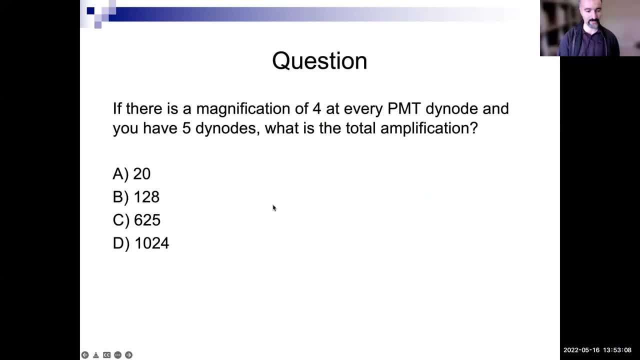 Yeah, so D. Yeah, So it would be D exactly. So the answer is D, Because four to the power of five is a thousand. But this is just a number. In reality it's quite more. In reality. it's more like not a factor of a thousand. 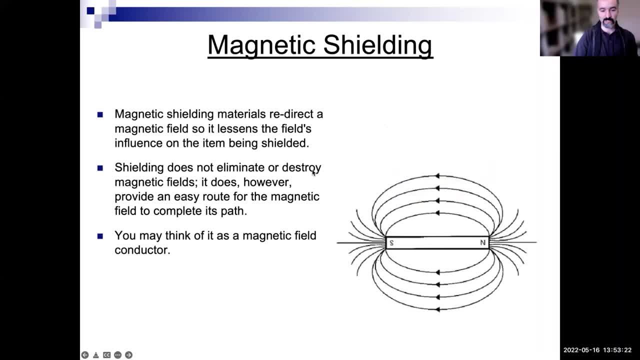 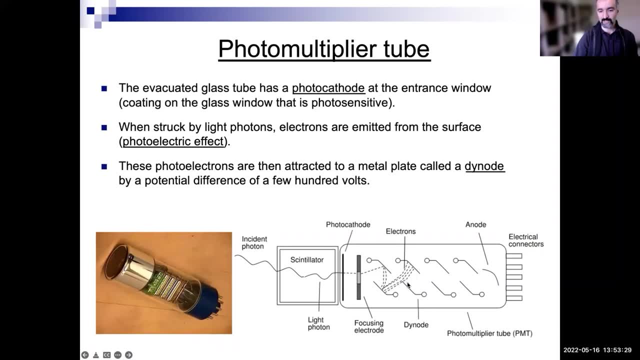 but it's more like a factor of a one million, Because you have more than five dinodes, you have more like, let's say, 10. And the amplification is actually more than a factor of four. That was just a toy example. 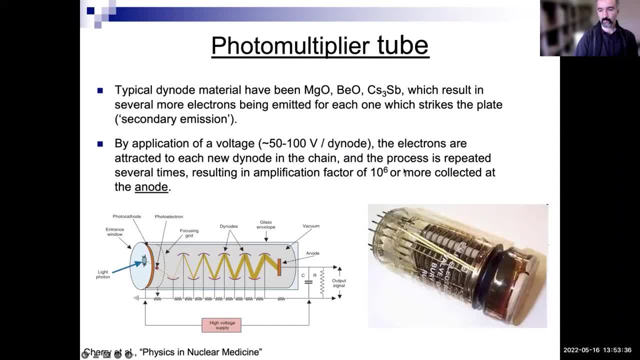 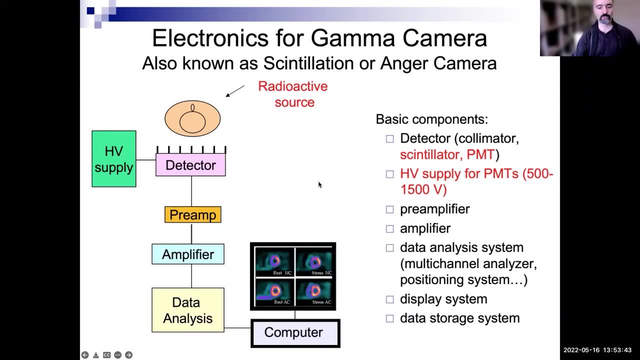 But really the amplification tends to be around a million Or more, But this toy example it was around a thousand. Okay, so thank you for that. So, okay, so we've talked about the scintillator, the thing that stops the original high energetic gamma ray. 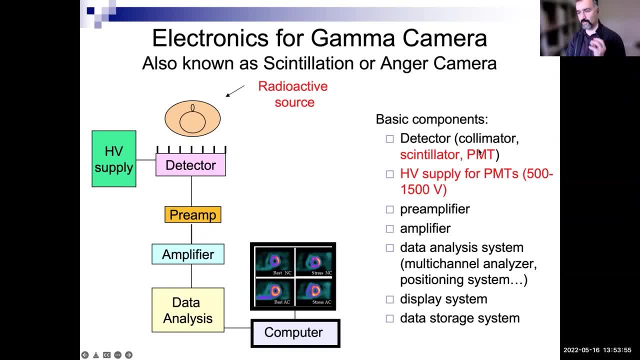 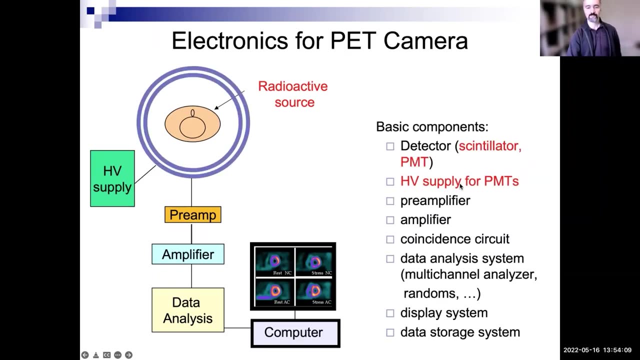 conversed to scintillation light, PMT, which converts that to electrons and gives you high level electricity or electric signal And the voltage supply that's needed to achieve that- around a thousand volts. But let's not talk about other stuff. 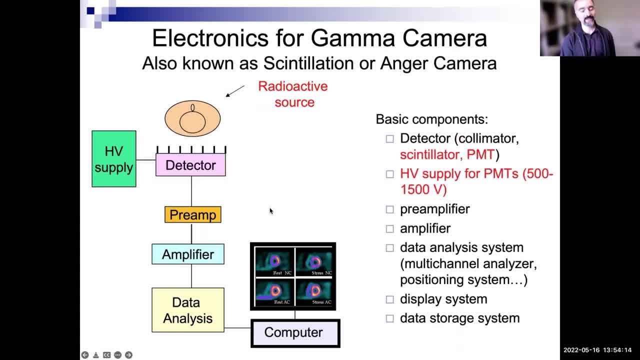 I noticed that this is for gamma ray, For PET, it's very similar. The phenomena is the same, except in PET we don't have like a detector like this that rotates around the patient. You'll see why we have to do this in SPECT. 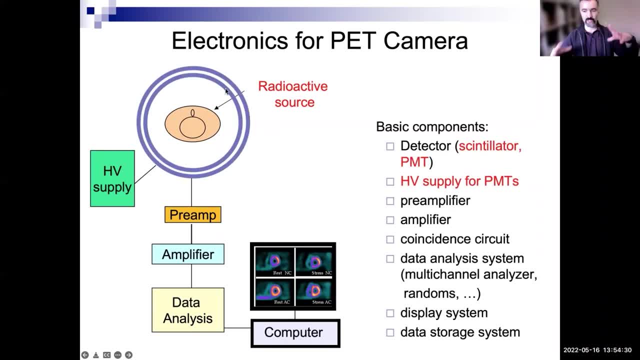 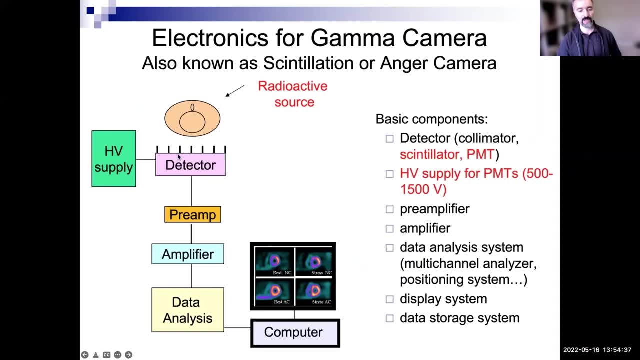 But in PET you can actually build detectors all around the patient like your ring. Even in SPECT you could sort of do it with certain new novel designs. But traditionally in SPECT you've had a planar detector which rotates around the patient. 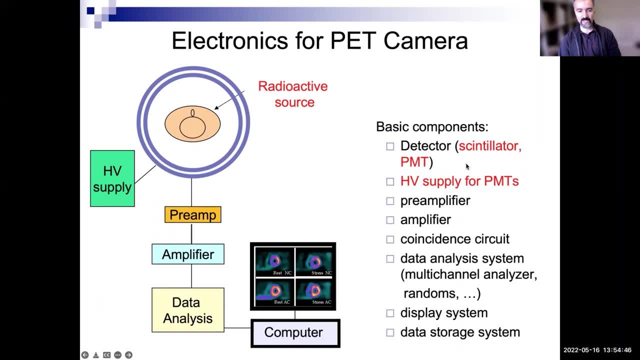 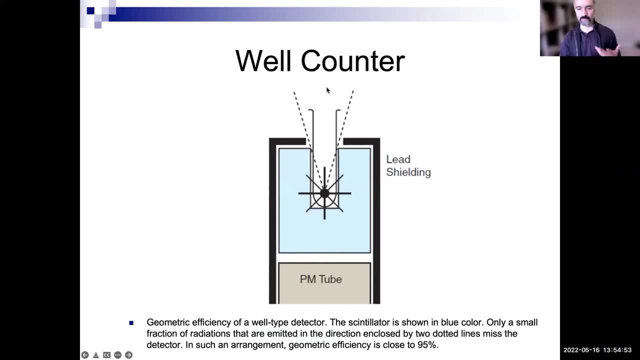 Whereas in PET you could surround, But the ideas are. the rest of it is the same, And also the principles of a well counter are highly related to this. What's a well counter? It's a very high sensitivity device to measure low amounts of. 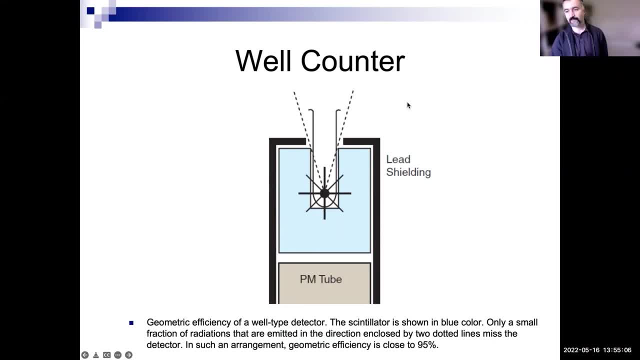 low amounts of radioactivity. Let's say you do blood count, blood sampling. Imagine you've injected radioactivity into the body of a patient and you just want to measure how much radioactivity there is in their blood. So you take little small samples, blood samples. 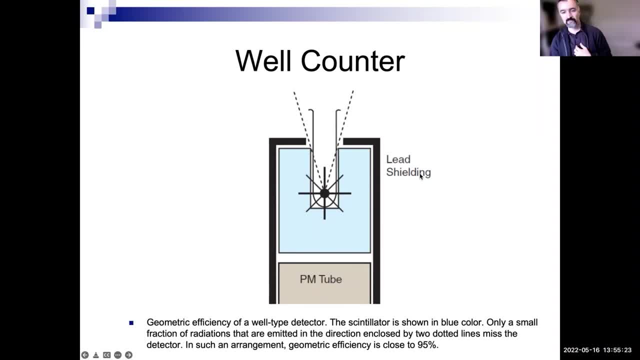 So there's very little radioactivity. So how do you measure that? So you have this so-called well counter. It's a well, But this whole thing is a scintillator- One big, massive, highly sensitive, highly sensitive scintillator. 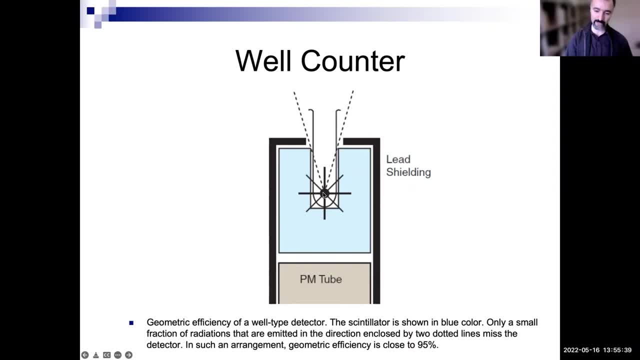 You dig a hole in it and you put your radioactivity here. Well, it's so sensitive to this because almost all photons emitted, all gamma rays emitted, except the ones that are directly exiting the well counter, are going to be measured by it. 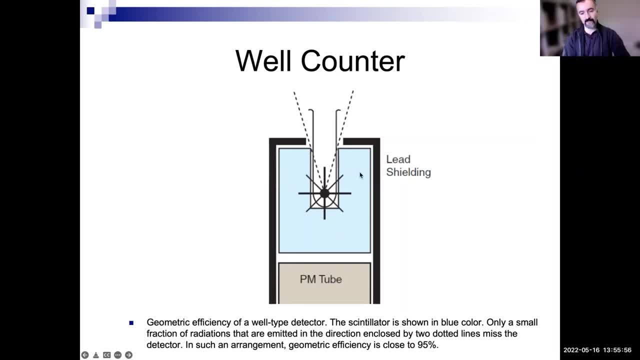 So guess what? This is going to be highly sensitive, But the principles are the same. So you've got a scintillator and then at the back of it, you've got a PMT, a PM2, a PMT. 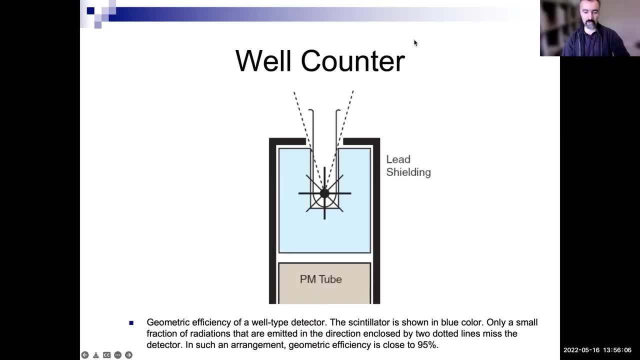 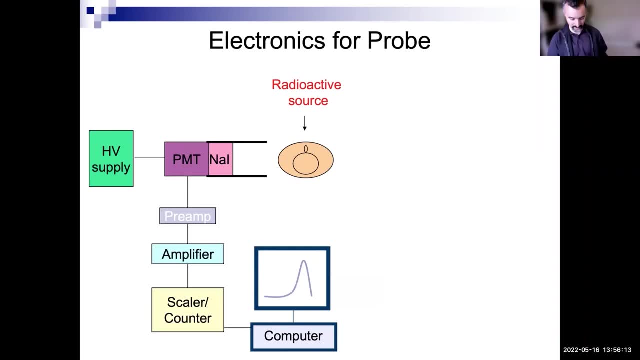 So the electronics for a well counter are also in a sense similar. And finally probes, so-called surgical probes. Imagine you've injected a patient something just to see how much stuff is in this particular tumor or to detect where the tumor is in the body. 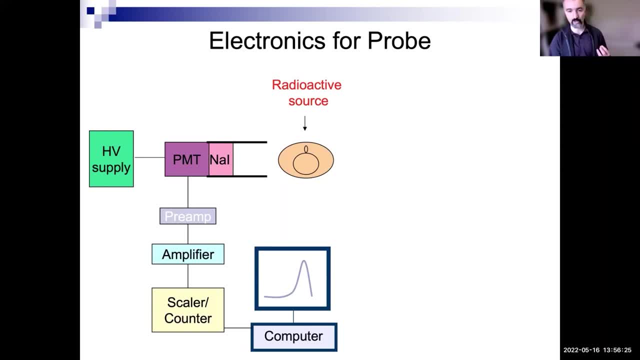 during the operation or to see whether you've successfully removed all of it. So probes are these things that I'll show you, but the principle operation is the same. The only catch is you're not surrounding the patient, It's just a single crystal. 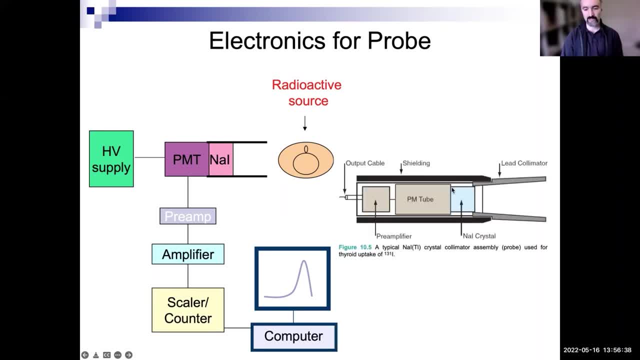 And this single crystal in the probe is basically matched to a PM2, to a PMT, and in the back of it you have got electronics. So it's a very similar thing, but you're just having this probe that you move around. 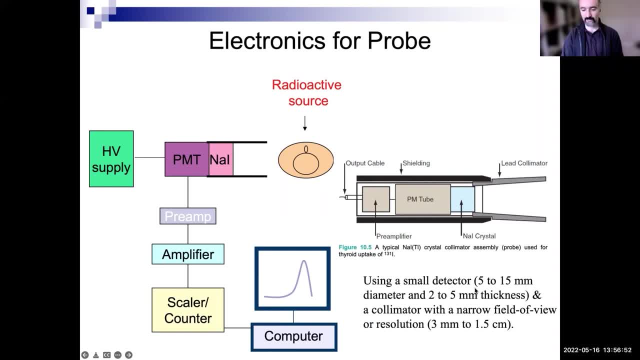 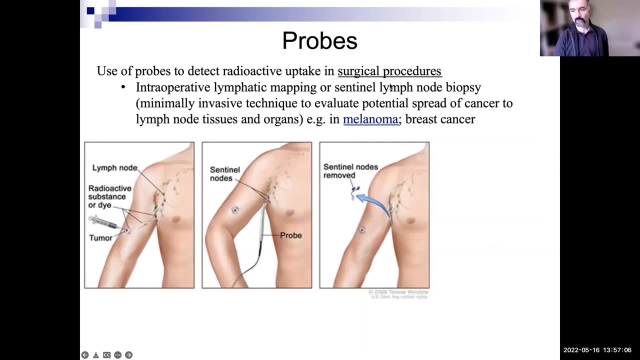 and see what's going on. So again, small detector and a collimator here, just so that you get only photons coming from a certain angle, not from outside of the field of interest. So probes, of course, are exciting. So nuclear medicine is not just about scanners. 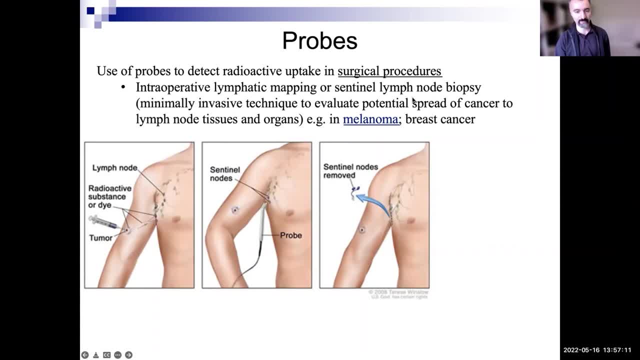 that we're used to, The probes are quite valuable Surgical procedures. you could do lymphatic mapping, or known as sentinel lymph node biopsy, which is minimally invasive. looking at things like melanoma in this example- and this audience is very familiar with that- 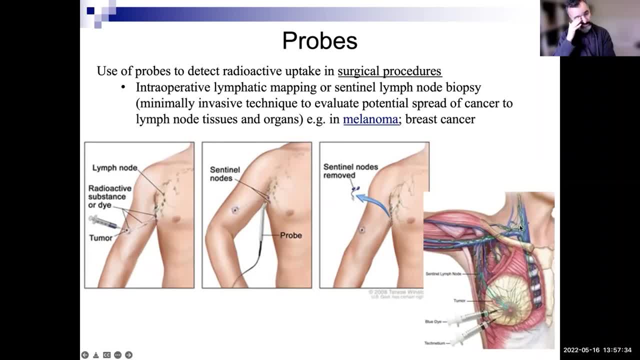 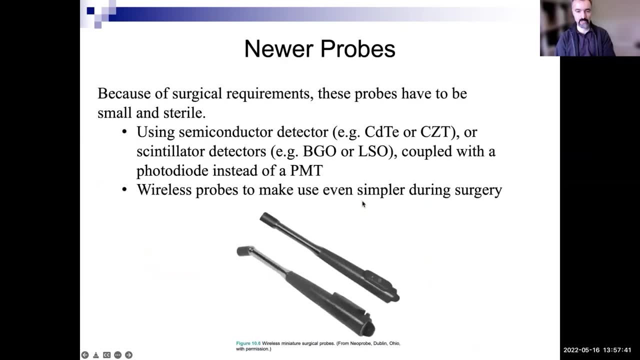 or looking at breast cancer. So it's a very, very valuable technique. You've got the probe here sort of making measurements of the sentinel nodes, And newer probes are moving towards other kinds of detectors, so-called semiconductor detectors, which are more expensive. 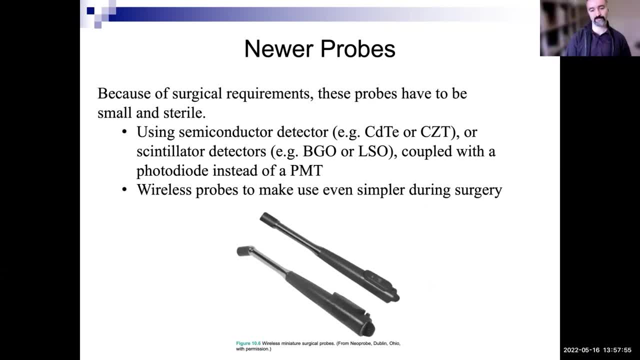 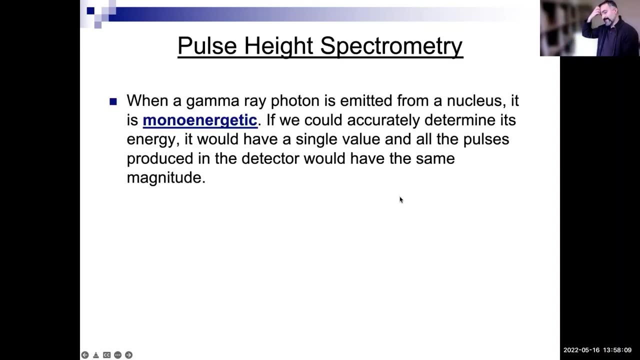 but you only need a single detector. So even if it's more expensive, it doesn't really matter for a single detector. So people are moving from scintillation detectors to semiconductor detectors, but the principle of operation is the same. Okay, so let's talk about some more details. 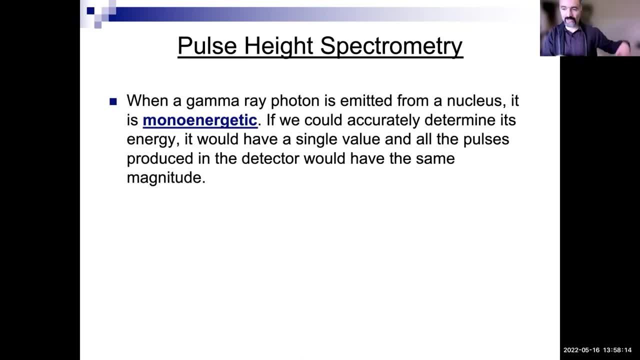 Remember how I said: you've got all these weird events, low energy things that you measure, and you really don't want them. Well, how do you even measure them And how do you eliminate them, Like imagine a photon or gamma ray in your body? 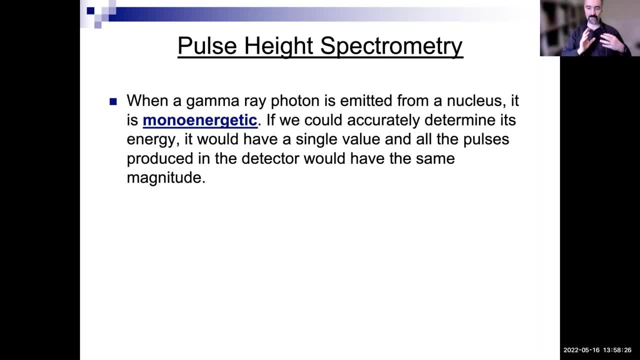 before it leaves your body, it scatters in your body and which lowers its energy, and you end up detecting something coming from the wrong angle because it got scattered. It could totally deceive you. How do you eliminate such an event? So you need to be measuring the energy. 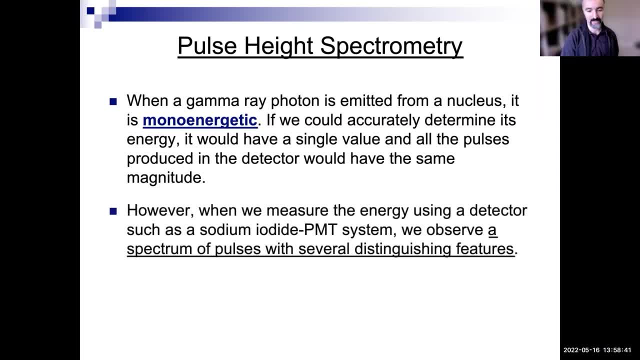 of the gamma rays that are coming in. So how do we measure the energies of the gamma rays? So, in fact, the truth is that we can, as I just mentioned to you before, because the number of photons that you get generated from a scintillator is proportional. 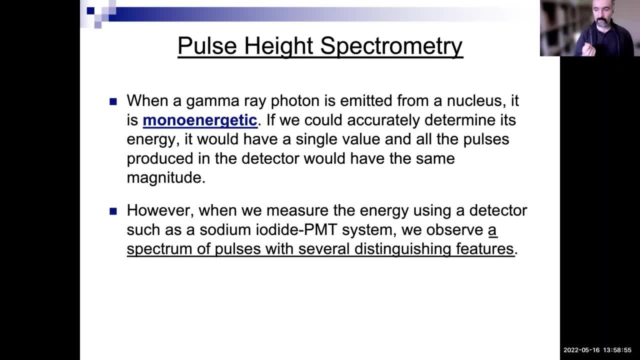 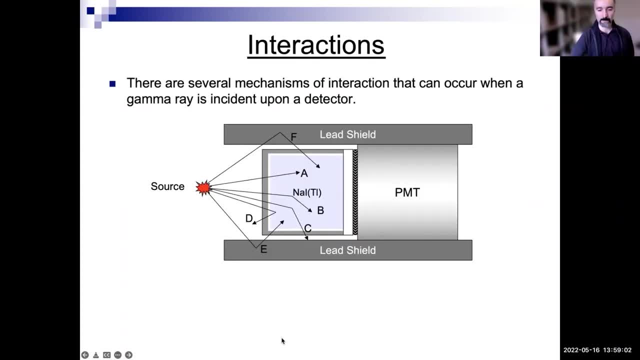 to the original energy, So we can measure the energy. But another question is: why do we get so many different energies? What does that distribution even look like? So let's understand all these phenomena that are going on. So imagine you've got a source. 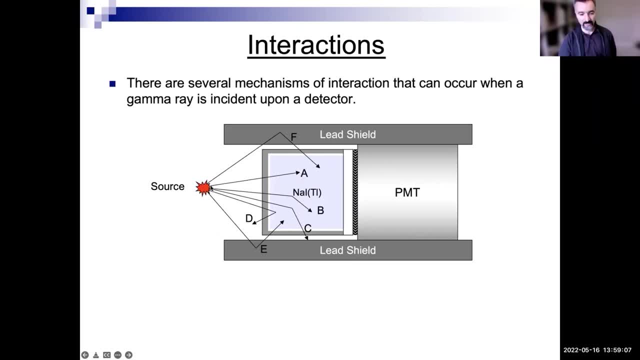 that is entering the crystal. This is your scanner. Well, ideally this thing enters here. All of the energy is absorbed, Scintillation, light's produced and great. But there's a whole bunch of other things that can happen. For example, you could enter the crystal. 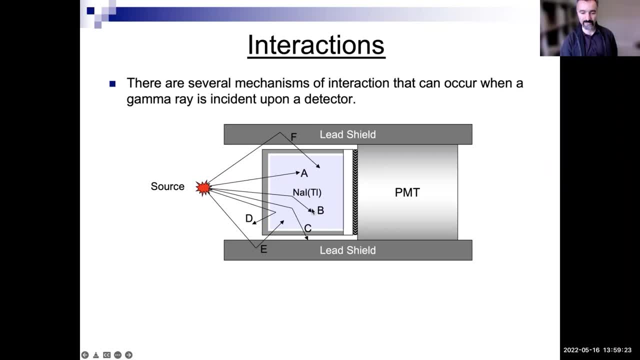 but you're not fully absorbed by the crystal. You scatter, but then you're absorbed here. Well, that's okay, because these two events are still absorbing the same detector. But what if you entered the crystal and some of your energy, of that highly energetic photon? 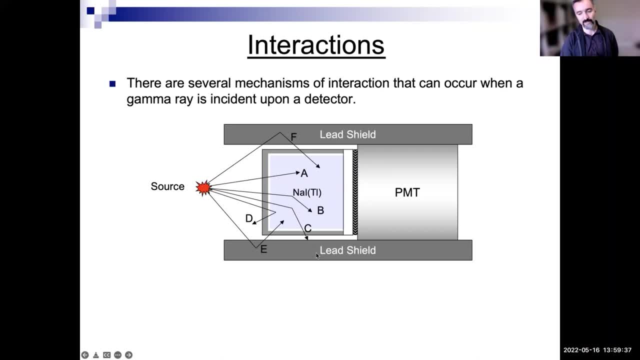 is absorbed, but not all of it, and the rest of it leaves the detector. So you've only acquired or captured some of the energy. You've lost the rest. So you're going to look at a lower energy photon. You're going to think that the original gamma ray 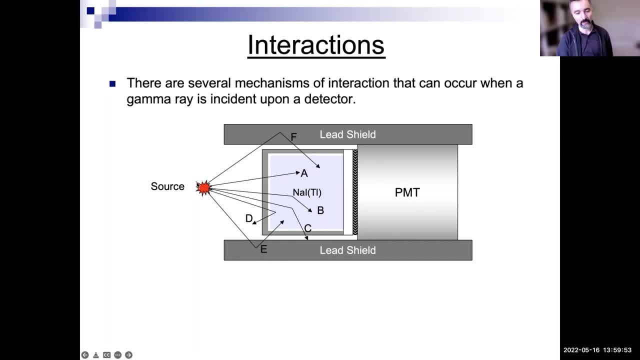 had lower energy than it actually did. It's going to mislead you. Or what if, before you enter the crystal, you enter some kind of a shield around it, you scatter, and then here you have a lower energy gamma ray that's coming in and therefore you're mislead? 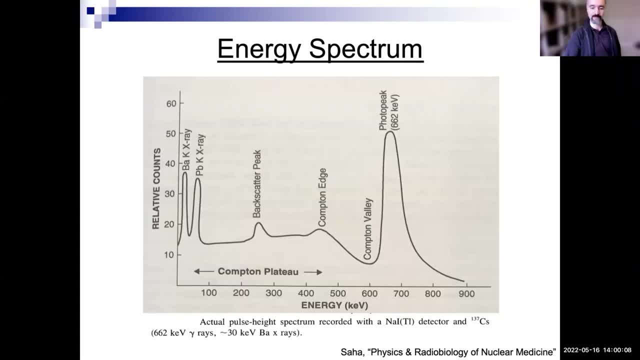 So many opportunities to be mislead, But guess what? We can eliminate most of them or many of them. So imagine questions welcome. Imagine that you've got an original gamma ray that has 662 kiloelectron volts in this example. 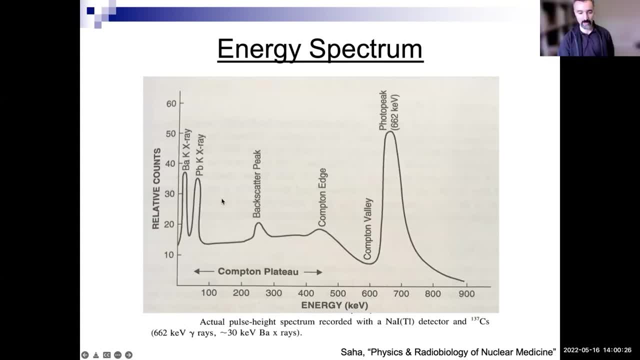 This is what you actually measure, which is mind blowing at first, But it's okay, We're okay, We're going to deal with this. So you have all these weird things showing up, whereas you really only expected to see something at 662.. 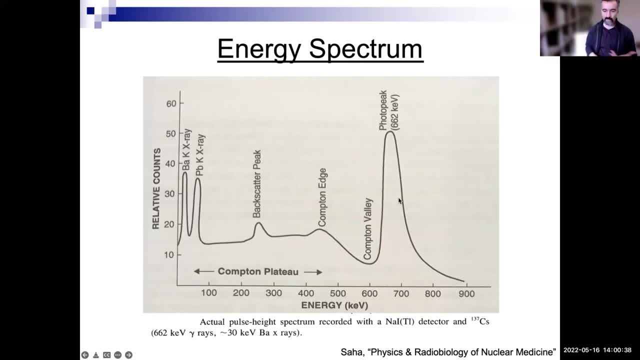 Sure, we see a little bit of broadening, simply because nothing is perfect, right, We have limitations, we have noise, So you're going to get a little bit of noise, But, okay, we wish we only measured this, but we've got a whole bunch of things here. 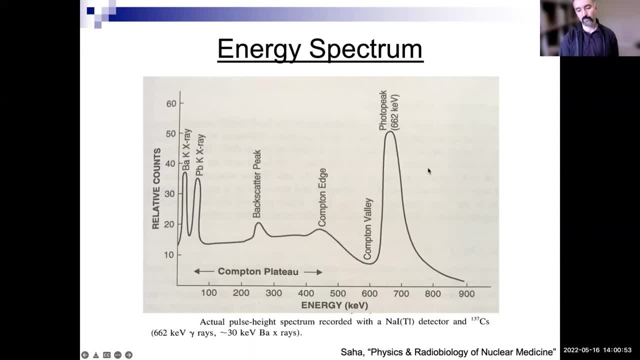 So let's try to understand what they are. But the good thing is, at the end of the day, we could put upper and lower energy bounds and reject all these events. Let's first try to understand them. So here you see, things like x-rays, okay. 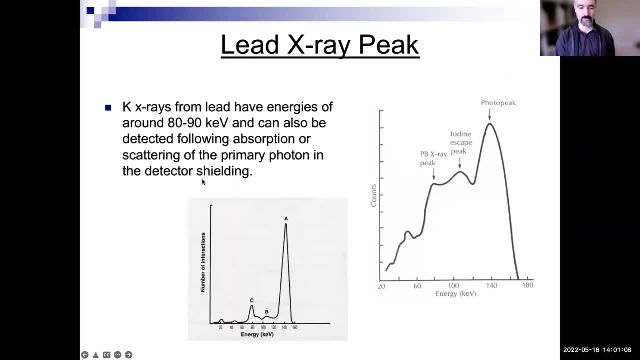 So these are not actually gamma rays. Some of these are x-rays- We'll see that in a second- K-shell- x-rays, for example, from lead. Okay, so remember, you have lead shielding and you have lead shielding and through absorption of stuff through the lead. 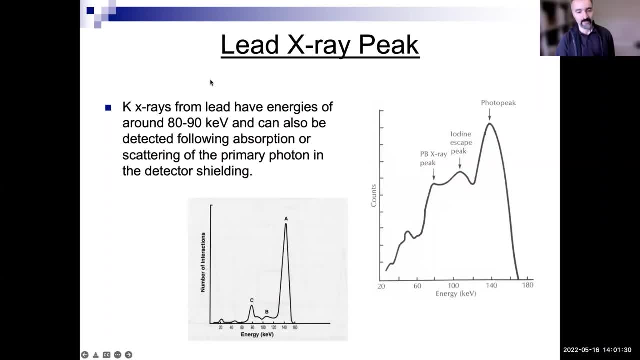 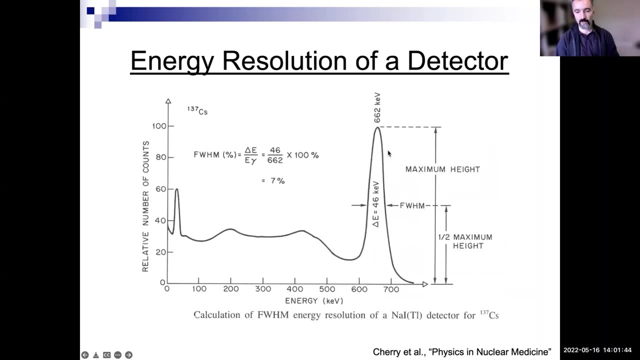 you may release x-rays, So that can totally mislead you. So you've got sodium or lead- sorry lead x-rays here, for example in the range of 80 to 90. So that could be the speed here. Energy resolution: we already talked about. 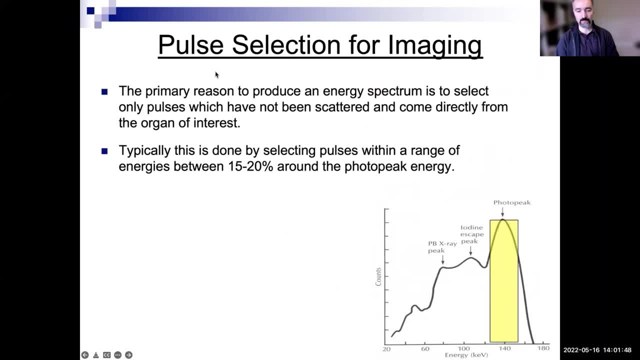 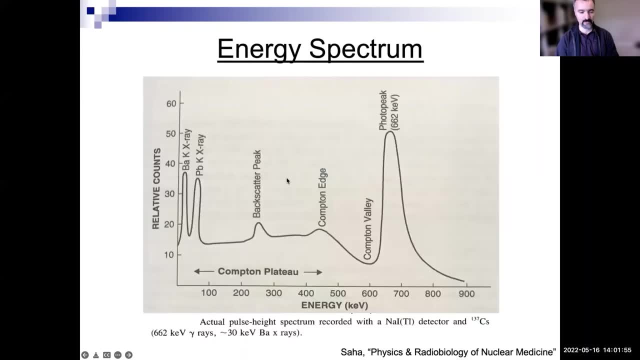 so I won't go over that. You can be putting there's other things. Oh, do I go over it? No, actually, let me go over some details here. So this is the lead x-ray that I just mentioned to you. 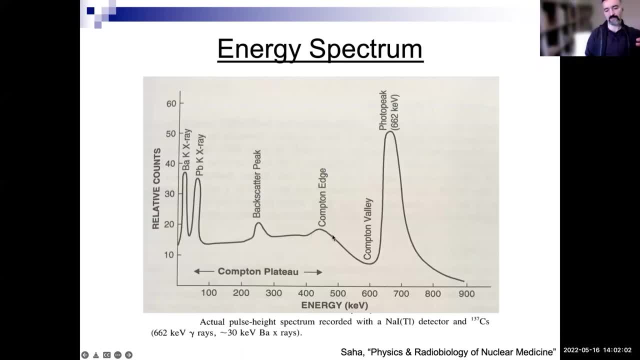 There are things like so-called content edge You could be, or a backscatter peak. You could be, for example, entering the crystal and being backscattered and only conveying and releasing part of your energy. okay, So if that happens, depending on the angle, 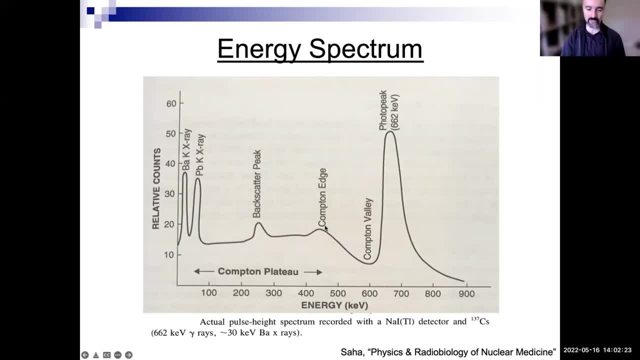 by which you scattered, you could get a range of energies that are in this range. This is the maximum value. We call that content edge. This is the lowest that you could, for example, be having In this example. So content edge and the backscatter peak. 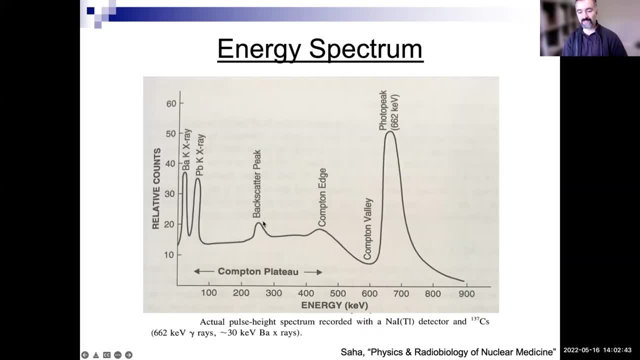 Okay, so backscatter peak. I won't go through the details, but basically you could be because of scattering, you could be getting events that are in this area. whereas you could, you should be declining those events. So to do that, we would put a energy spectrum. 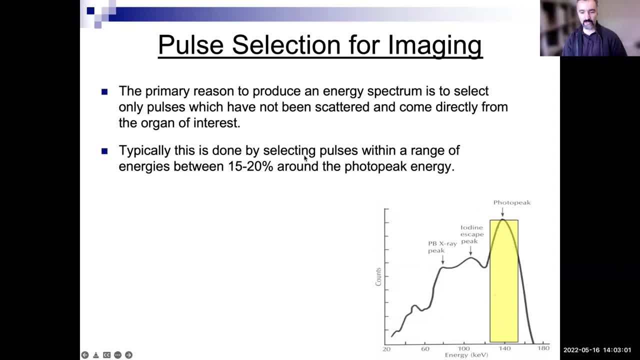 or put a upper and lower Energy range, For example. we would say I only will be accepting a 20% window around my photo peak, 20% And nothing else I will accept. So all these stuff I will be rejecting. 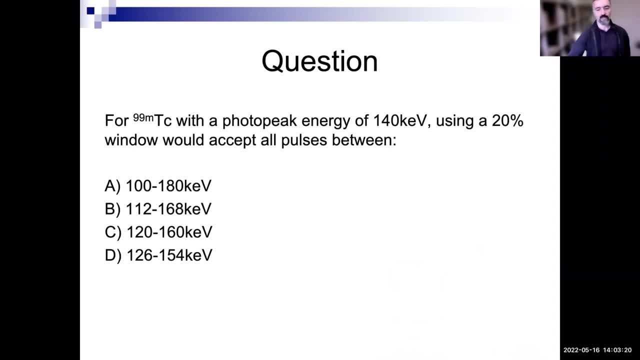 So here's a question for you. Let's look at Technetium 99M, which has a photo peak energy, which is the incoming gamma ray energy of 140 kilo electron volts If I put a 20% energy window on it. 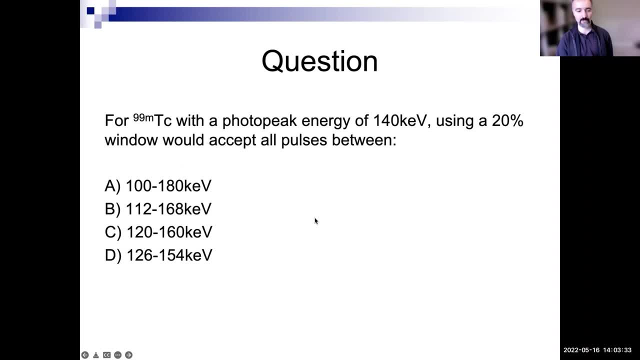 what is the range of energies that I'm accepting? Which one of these four is it? Can you work it out? It would be B, So it's always, of course, with me. now you're learning. I'm asking three questions. 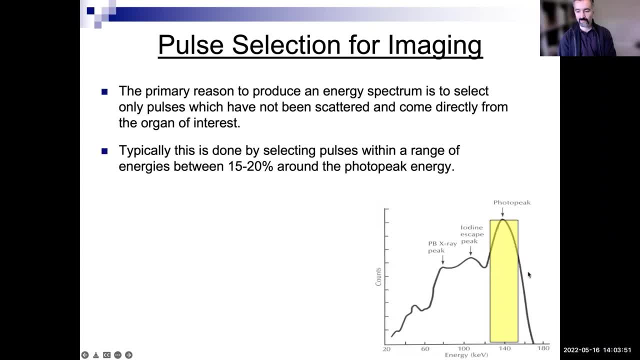 The 20% is from the upper to the lower, So it's not from the middle. So it's really more like when I say 20%. when we say 20% we mean 10% at the top and 10% at the bottom. 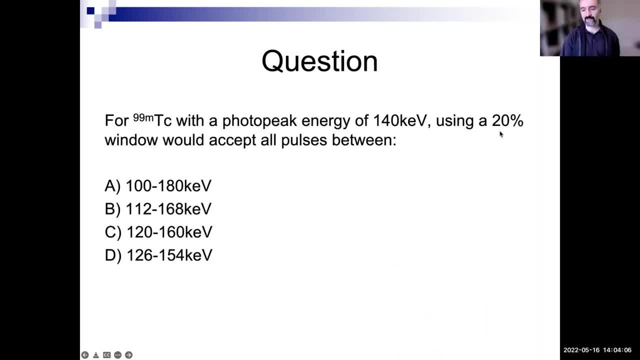 You know what I mean? Oh, okay, Yeah, Yeah. So, because of that, 10% of 140 is 14.. So it would be 140 plus 14 and 140 minus 14.. So it's actually D. 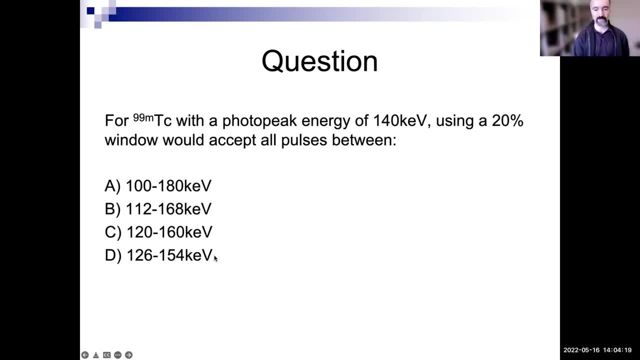 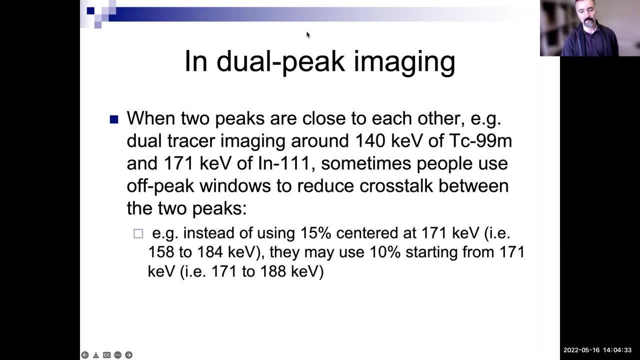 So these are gonna be the energies we're gonna be accepting. We won't accept anything else. Okay, So we could be doing things like dual peak imaging, So, for example, when you could be injecting two different- this is the beauty of gamma single photon imaging. 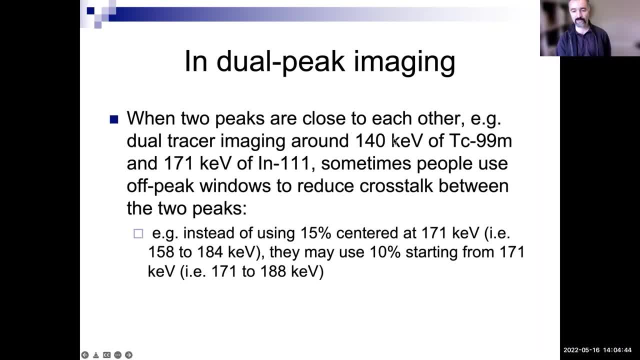 You could be injecting two different things into the patient with different energies. Let's say, technician 99M has a photo peak at. you know, the main energy peak is at 140 kV, whereas Indian 111 gives you 171.. These are two different energies. 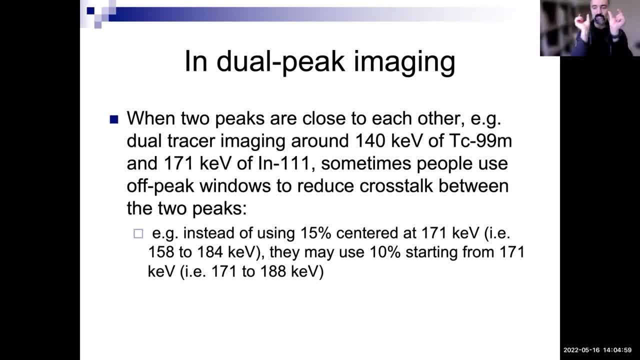 So you could be putting two different energy windows simultaneously in the patient And you could be imaging two different radiopharmaceuticals that are co-injected, for example, which is amazing. But you gotta be careful, because if the peaks are too close to each other, they may cross contaminate. 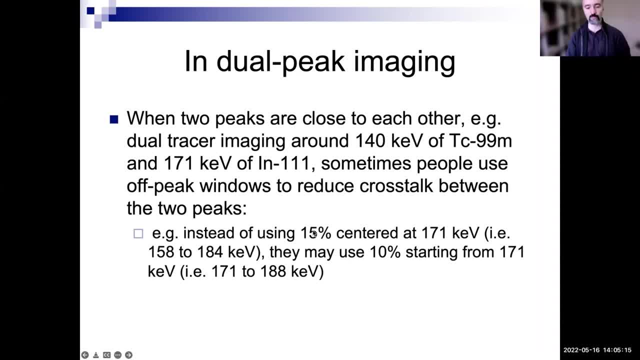 due to the blaring energy resolution. Sometimes people, instead of putting like a 15 or 20% energy window centered, they might put it like left centered or right, or instead of centered at the peak, they would put it a little bit to the right center. 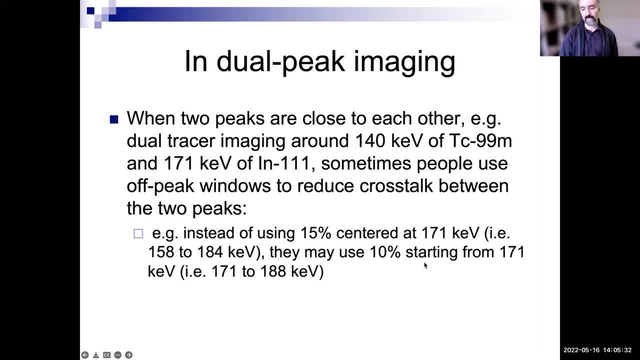 A little bit to the right or a little bit to the left. In this case they would put a 10% from 171, all the way above it, So not below it, so that there's less contamination, Just as an example. 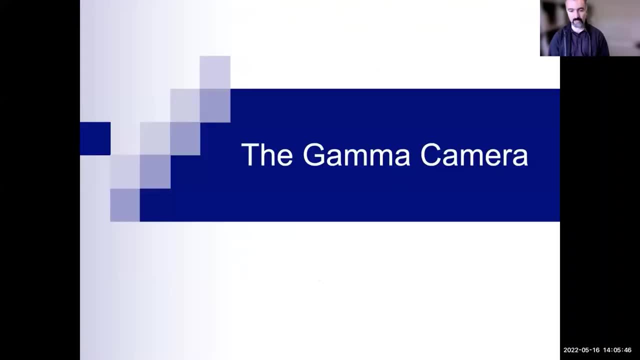 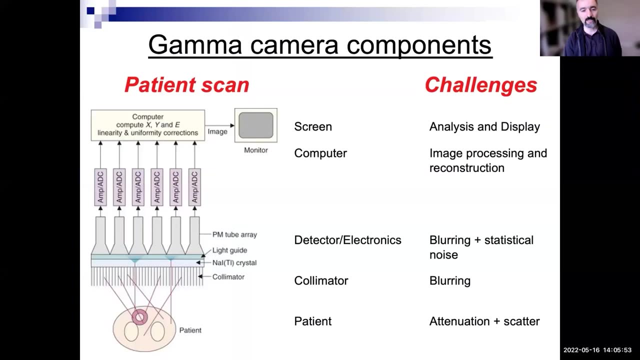 Okay. So let's go through this. We can take a break a bit later. So the gamma camera has a number of principle operations. We've already really talked about this. I'm just going to keep mentioning some of these. We need the okay. 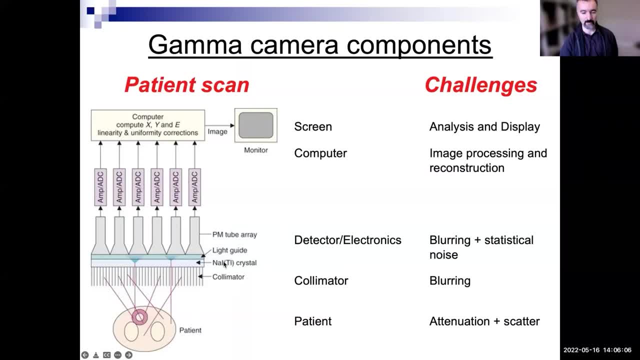 We haven't talked about collimators much, but we've talked about the crystal or a scintillator. We've talked about the fact that you need a PMT, a photomultiplying tube, and the backend electronics. We haven't really covered that much. 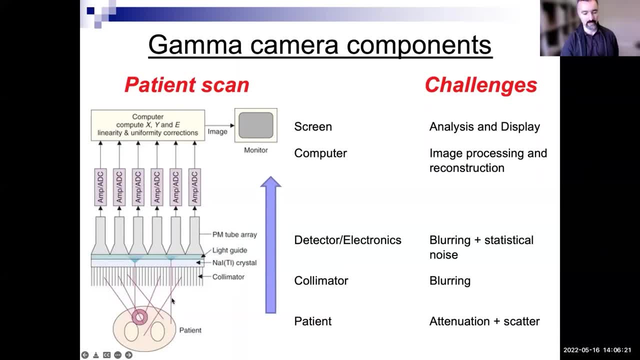 So we're moving this way right, The patient is here. Collimator basically blocks photons that are coming at bad angles. Doesn't want to be confused. It only accepts photons coming at 90 degrees. And we talked about PMTs, So there's a whole bunch of electronics. 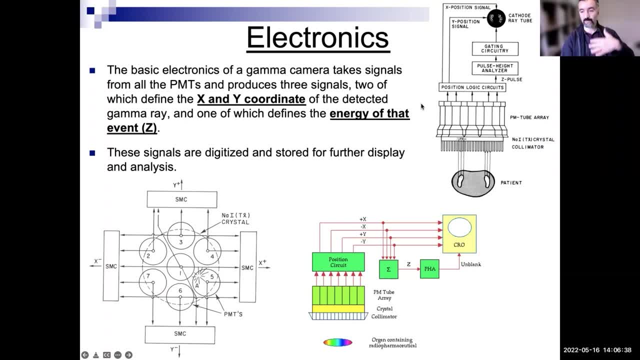 which I really won't go into. you know essentially. imagine that at the end of the day you've got your PMTs and you can really figure out which PMT obtained your signals. So you know the X and the Y coordinates. you would know. 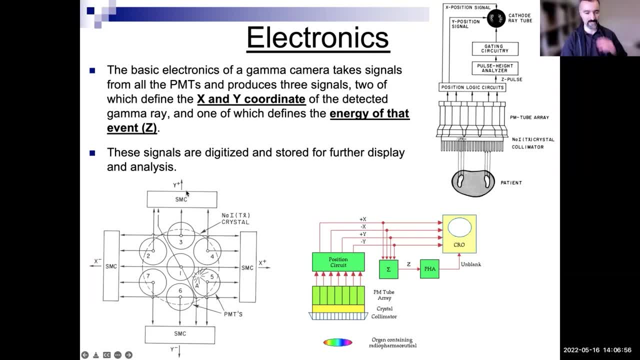 And when you know the X and Y coordinates, so we call those X. forget about this. X minus, X plus, Those are just old things. You know electronics literature, but just X and Y. you know the coordinates. you know where which PMT obtained the signal. 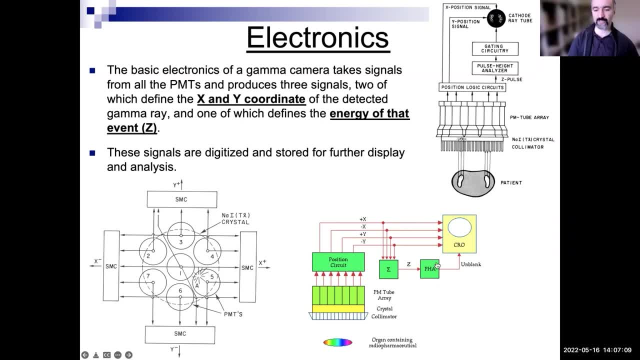 and the Z or the Z signal is basically, it's not the Z coordinate, It's just the energy. X, Y, Z, X and Y are the physical coordinates. Z is the energy, you know the energy. So the beauty of anger. 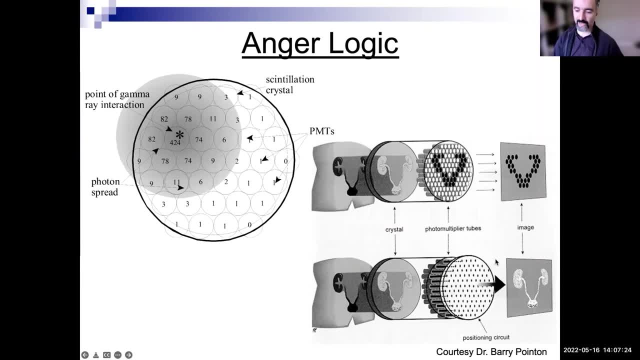 and this is one of the key contributions of Mr Anger which really allowed this to happen. The beauty of anger logic. of course you know what exactly is it. Conventionally, this is what you would get, For every PMT would have to be paired with every crystal. 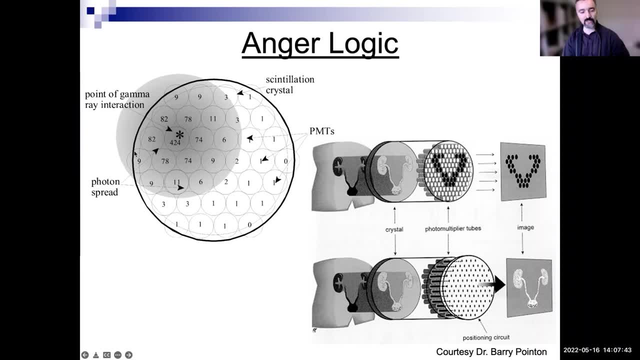 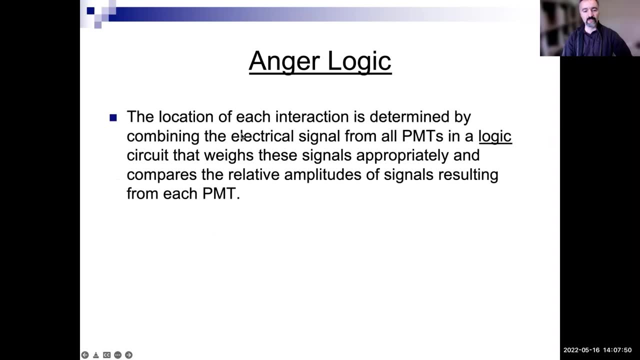 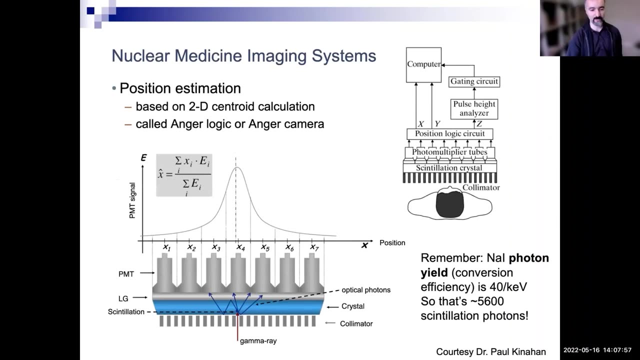 And so you get this kind of resolution, But with anger logic you get a much, much better resolution. So how does it actually work? The location of each interaction is determined by combining signal from multiple PMTs. So think of it this way. 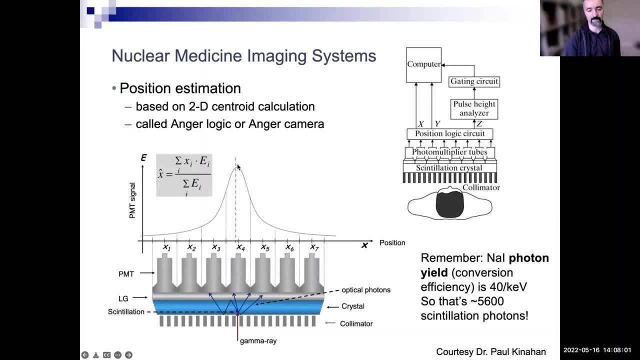 Imagine the original source of light was here. The scintillation crystal is producing a lot of different signal, but guess what? Not all of it ends up in this central PMT. Some of it ends up going to these nearby ones. Now, normally you wouldn't like to. you're like. 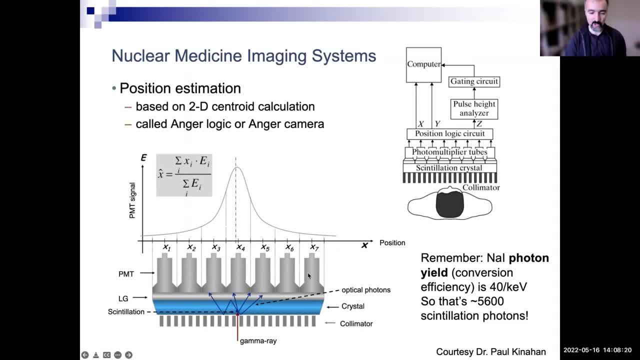 oh, that's not good. They're ending on different PMTs. but this is good because you could take the signal from all these PMTs and averaging them and figuring out what is the exact position even within a PMT. Normally you wouldn't know where within this PMT. 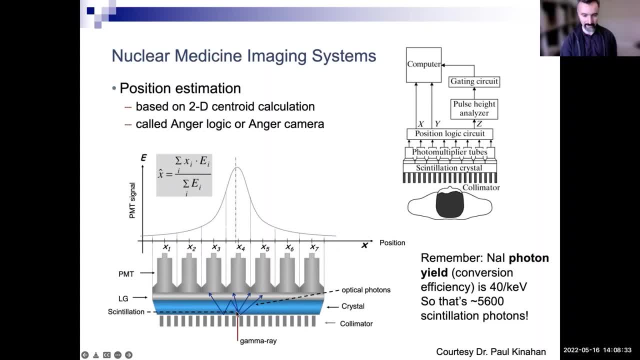 you detected your signal here Like: this is your event. Look at this event. Normally you wouldn't know where along the PMT you got the signal, but now, because some of the signal remember, you may have four or five 6,000 different photons being generated. 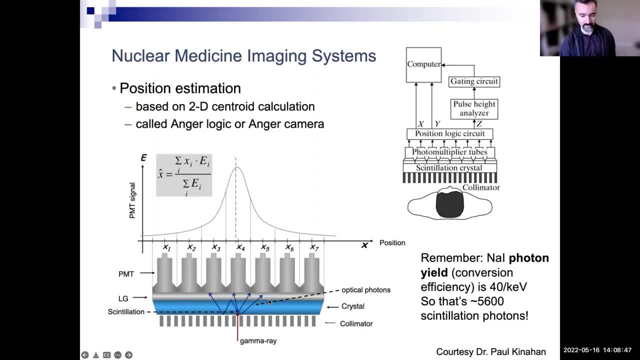 from a single gamma ray coming, While some of them end up here, some of them end up here, And when you average them and weight them, you would know where exactly within this PMT you obtain this. So this is anger logic. It's kind of a very cool technique. 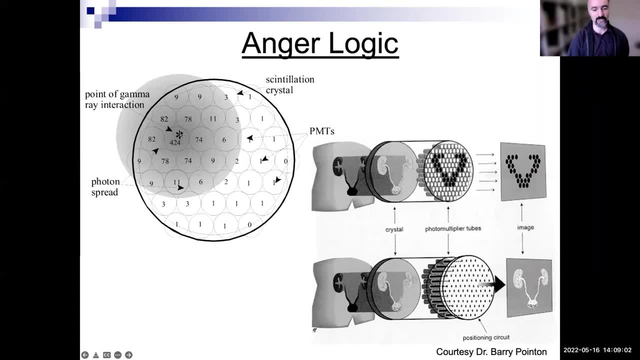 So, again going back to this, this original signal is coming from here, So most of the photons end up in this PMT, but some here, some here, some here, and by averaging all these energies and weighting them, you would actually sorry. 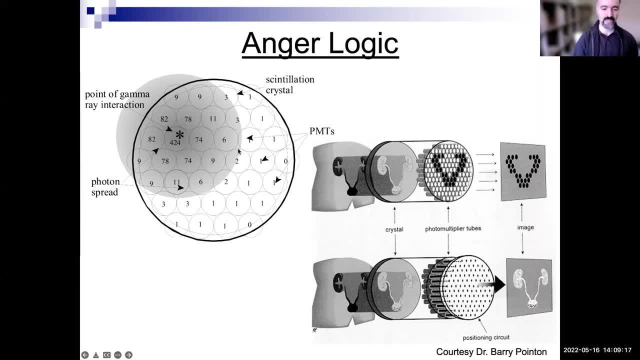 by measuring all these PMT signals and weighting the amount of signal you receive, you can actually identify where, within this PMT, this event is aligned. So you go from a resolution of one PMT, which is not impressive at all, to a sub PMT resolution, where you can get much, much finer. 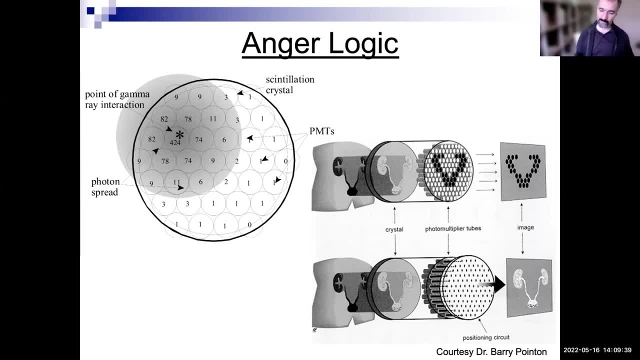 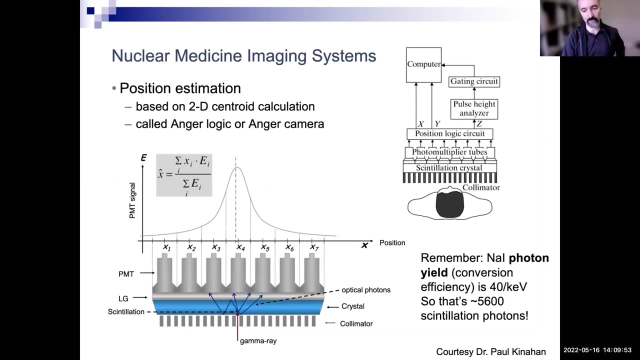 So I thought anger logic where you use nearby, it's counterintuitive. actually, You let the signal spill to nearby PMTs too, not the one-to-one mapping. So with the help of this community of PMTs and averaging, you would know finer details about where the original signal. 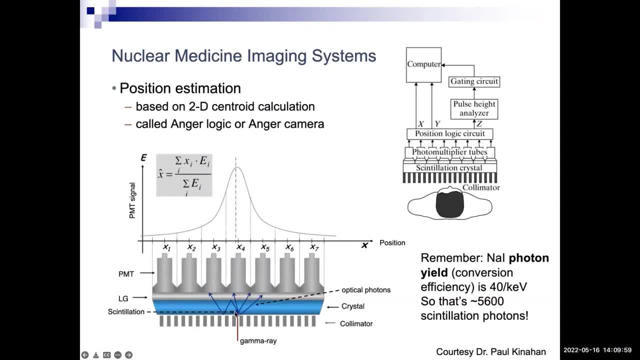 was Again. just to emphasize: if you start from here, it's much less likely you're going to get a signal in this PMT, much more likely you're going to get them here. but by averaging this you can sort of figure out. 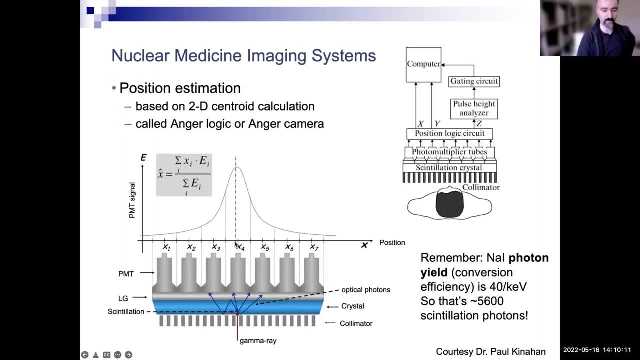 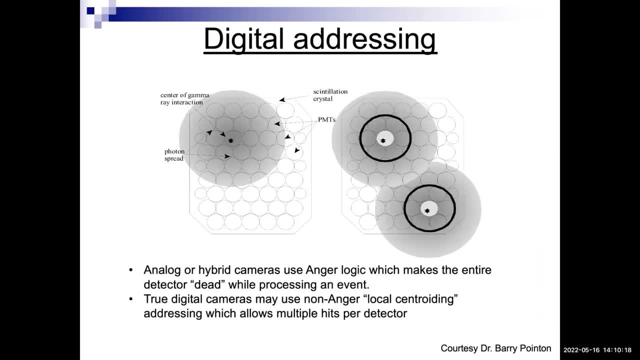 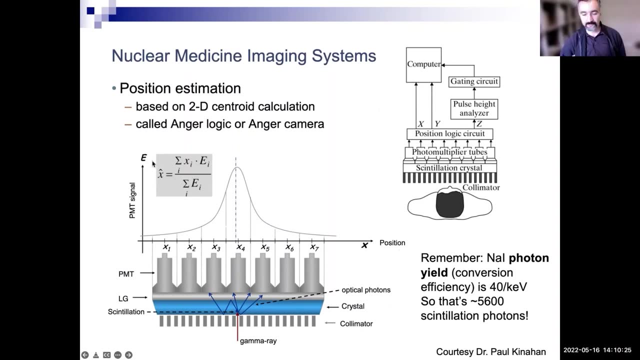 oh, I'm slightly here to the left of the center which you wouldn't have been able to measure. So this just to clarify. so you're taking like dead center of the average, You're taking the dead center. What do you mean by dead center? 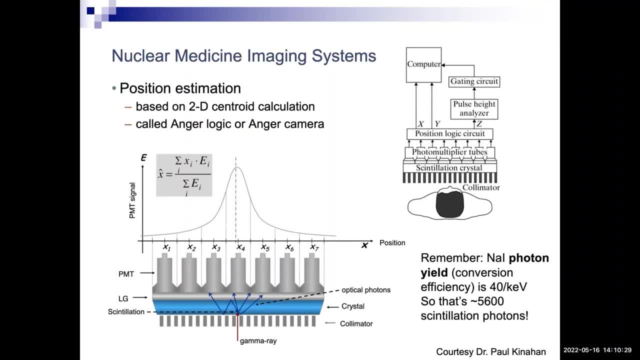 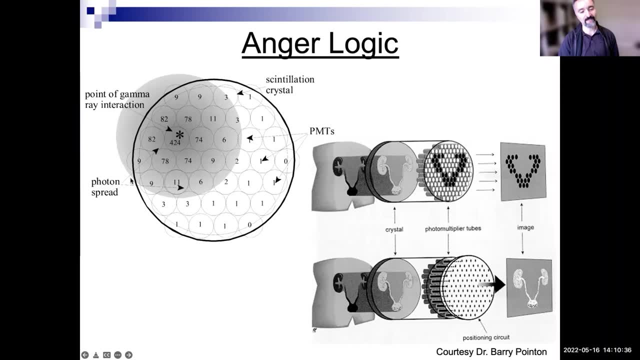 I don't know, I just going off of the image that you were showing with the circle in the middle Here. Yeah, So you actually average all this signal and it would tell you that in fact, it is not at the dead center of PMT. 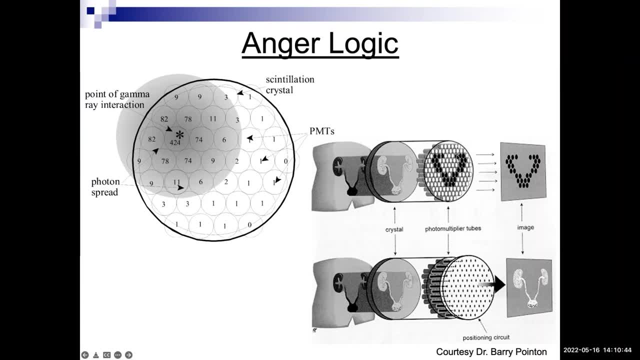 that it is slightly off of the center, Okay, And that's why you can go from a resolution of not knowing where within the PMT you are to actually knowing where within the PMT you are. Okay, It's kind of a funny, bizarre thing actually. 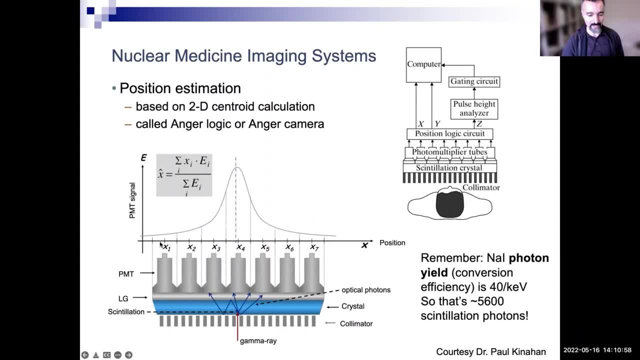 Like: look at this signal here. If I'm getting all these different signals, imagine I'm getting 10 photons here, 20 photons in this PMT, 40 in here, 60 here, 35 here. If I average those, and if I average all those signals by the position of the PMT and the energy or the number of signals I got, I would conclude that I was not at the exact middle of this PMT, but I was slightly to the left of it. 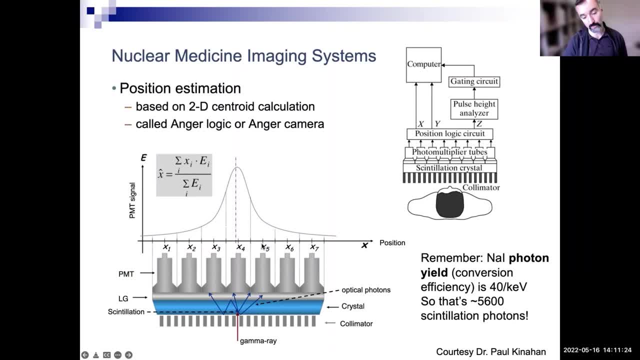 Because this PMT next to it got a little bit more signal than this PMT to the right of it. Right, Okay, So that's kind of a cool thing. Sometimes in life you get something that looks worse, but it's actually better. 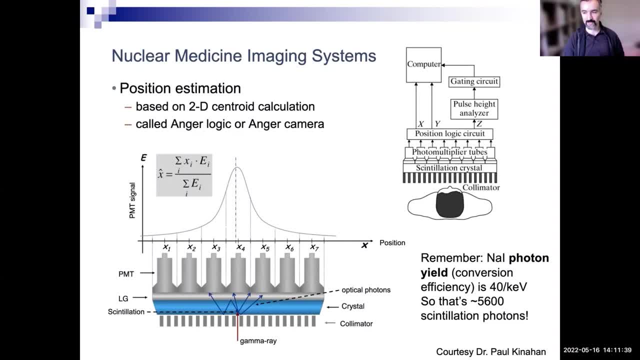 These things are spilling to nearby PMTs. How can this be better? But it is better because nearby PMTs are giving you more hints about what's happening. I mean that's a bad analogy, But imagine you've got nosy neighbors and you've lost something in your home. 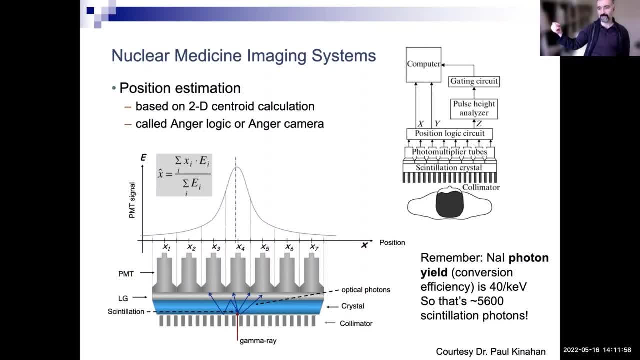 You don't know where on earth it is, but your neighbor to the right hears your cell phone better than your neighbor to your left. So you conclude that my cell phone is not in the middle of the house, but it's more to the right of the house because my neighbor is listening or hearing a bigger sound. 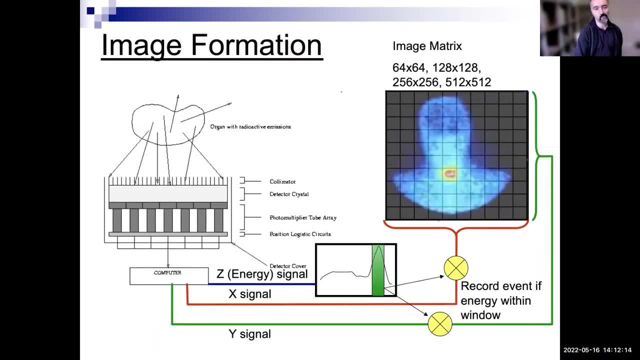 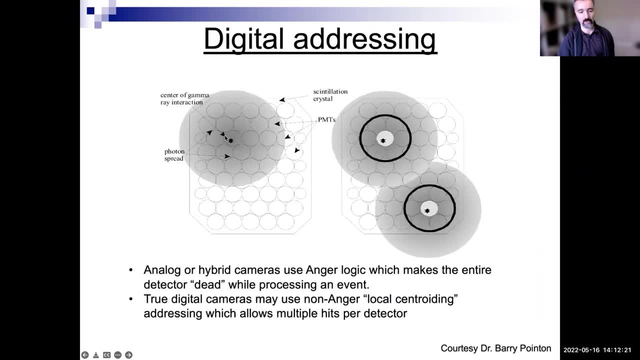 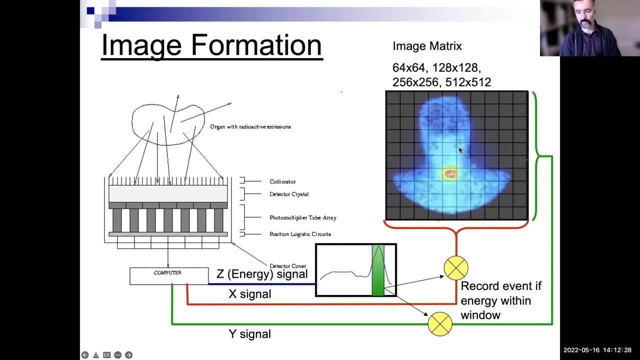 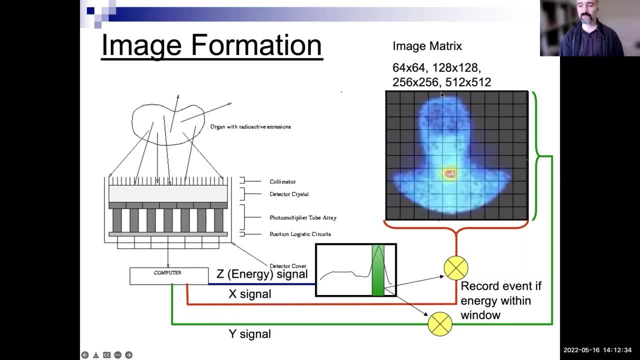 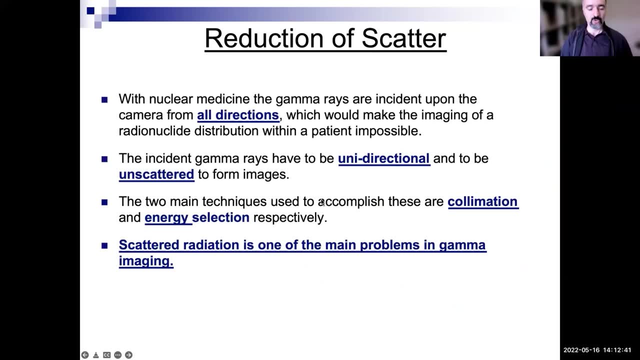 And it depends, of course, on the number of pixels that you have. The more pixels that you have, the finer the resolution, et cetera, et cetera. So, given the fact that we can measure the energy of the signal, because the more the energy of the original gamma ray, the more scintillation that is being produced, the more the glow. 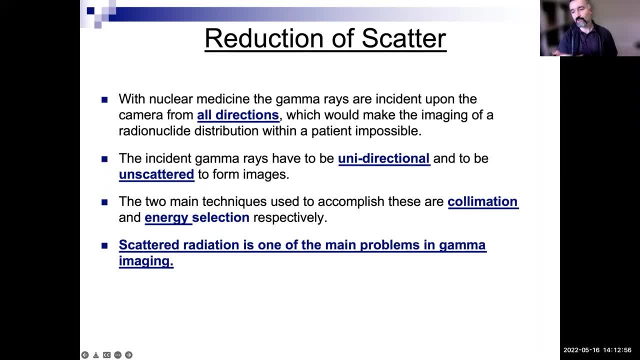 You can actually eliminate some low, Low energy value. Like you know, you really should not be measuring 50 kiloelectron volts Like this. original event was 140 kiloelectron volts. At best it might have become 10 or more or 10 less because of, you know, limitations in signal to noise ratios. 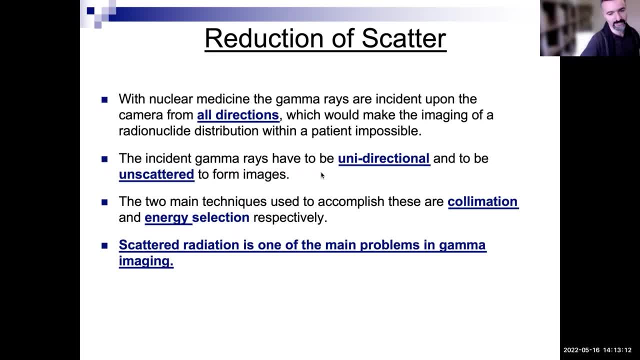 But it should not be 50 kiloelectron volts. So you will be rejecting all events that are too low in energy. So you can do energy selection. Now, how do we pick directionality? So let's talk about that a little bit more. 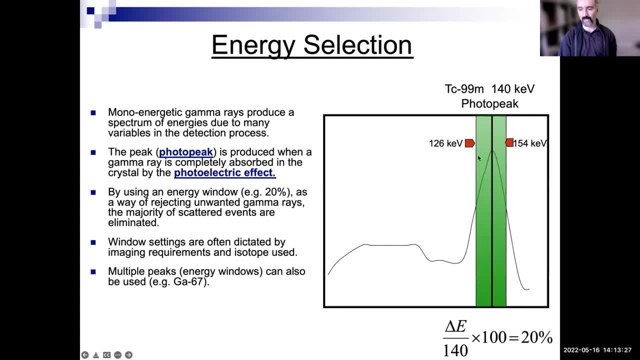 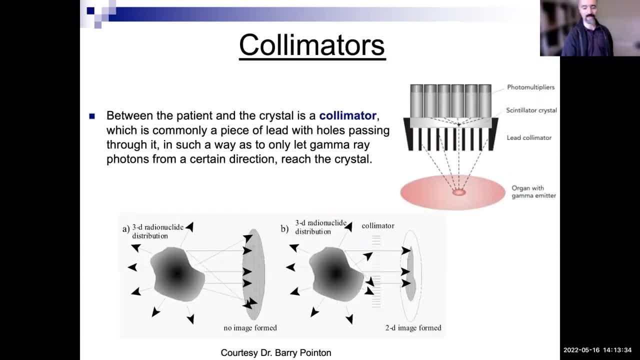 Shortly. But again you would put an energy window around this and eliminate all these other signals that are coming in. But let's talk about collimators. Collimators allow you to control the energy. Imagine you've got a source here. Collimator tells you or allows this photon to pass through, but not these ones. 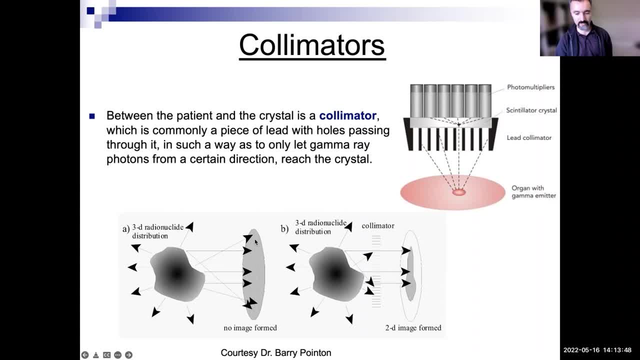 And why is that? Because imagine you don't have any collimators And you've got this is your source of. This is like the human. Let's imagine this is like some tumor in the body or some organ in the body that we thought. this is a detector. 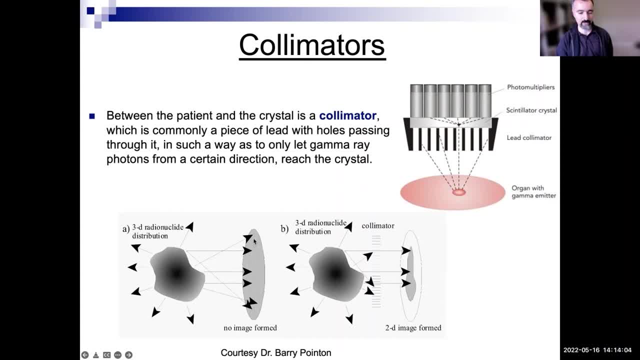 Well, any signal from anywhere in this organ could go in any direction and create this big blur And you don't know where what came from, where you cannot visualize this. but if you would collimators that say: I will only accept if you're coming at exactly 90 degrees- give or take a few degrees, I can better map where this event came from. 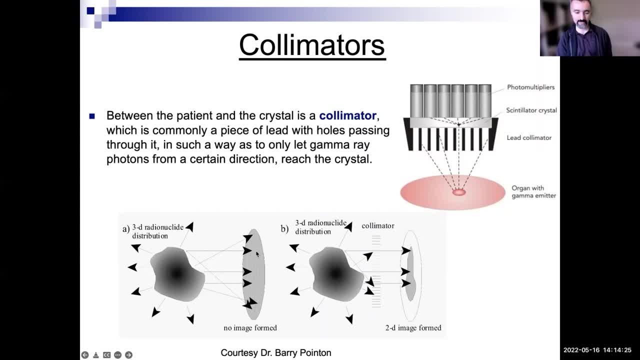 I can back, project it and know where it came from. But here, if I detect something here, I don't know where it came from. It could have come from this angle. It could have come from this angle. This angle doesn't allow you to do things. 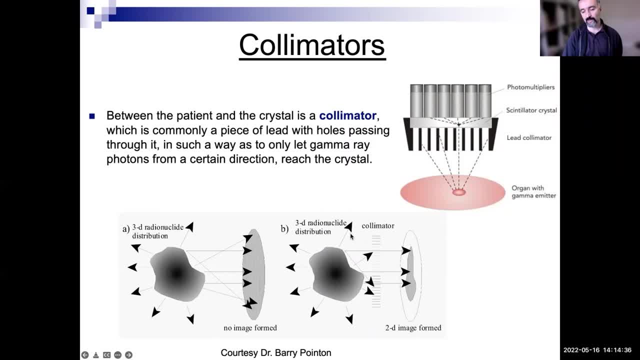 So, unfortunately, you have to do a bit of a sacrifice. You have to put a collimator. Collimators are good because they only accept certain angles, but they're bad because they kill a lot of signal. This event has some value, but we had to kill it because we want to only constrain this to things coming at normal angles. 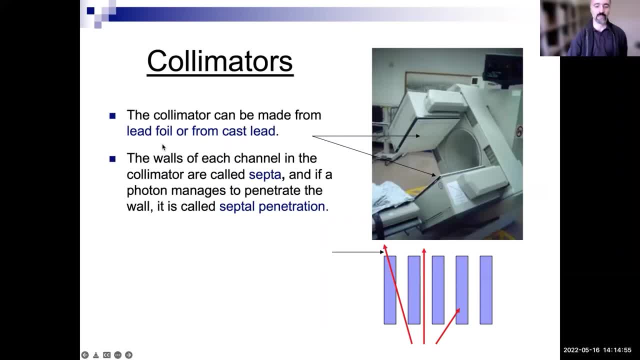 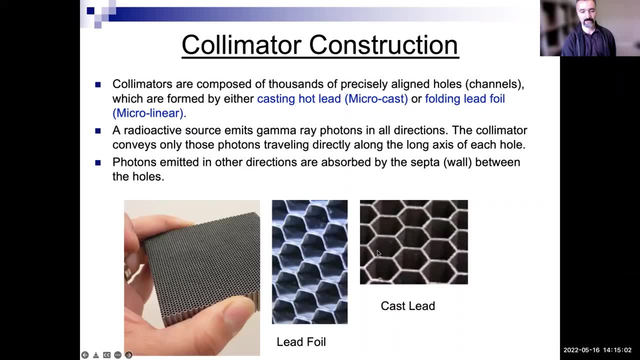 So collimators are very common. They're they're They're made commonly from lead, whether it's lead foil or cast lead. So here's lead foils, cast lead. we won't go through those details. The walls of the collimators are called septa. 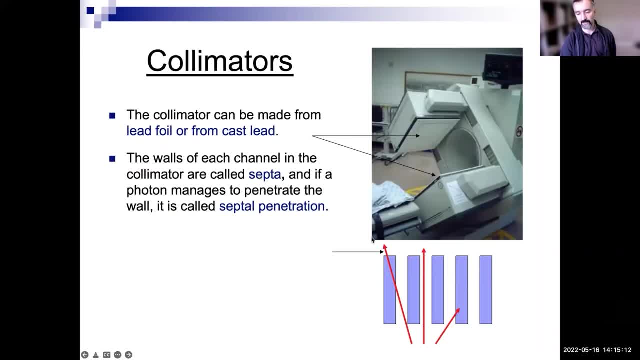 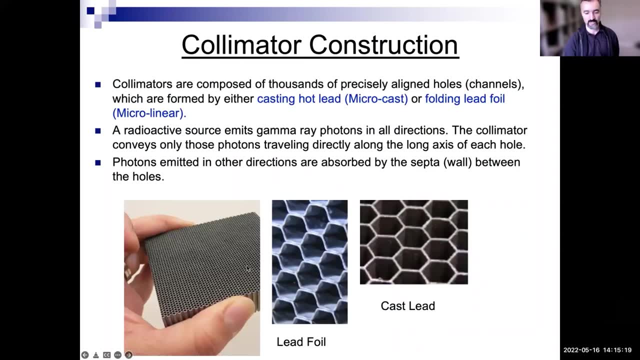 Sometimes signal unfortunately does penetrate the septa, so that's a limitation. but you want to keep that to very low percentages. So here's an example of collimators I can imagine if something's coming from above it will only make sense. 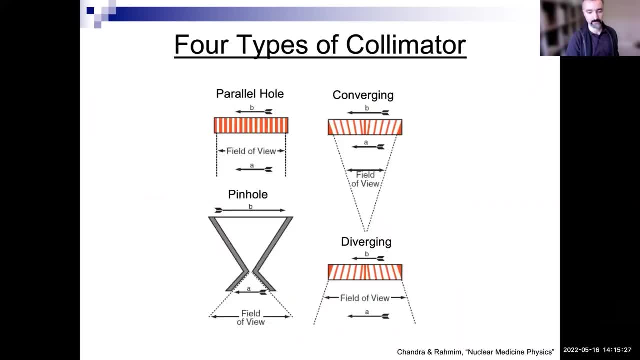 If it's really above it but not going at an angle. we do have other kinds of non-parallel whole collimators, like converging, if you want to look at a small field of view and make a big image of it to get better resolution. because looking at smaller things, kind of like the original Casson thing, the scanner, but that was focused on a single point. 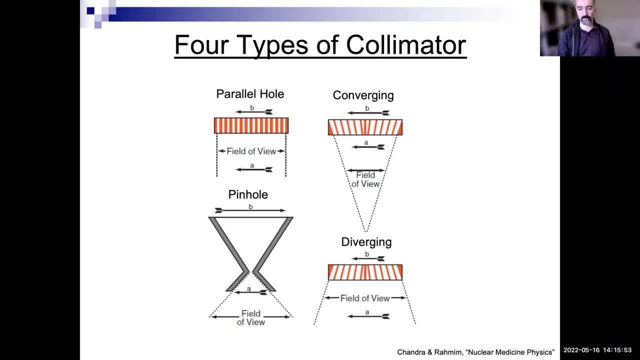 This is focusing on, like a part of the small organ, for example. You could have diverging too, like: imagine if and people really don't use this anymore, but imagine you want to image the entire body in a single detector, So you could do that. 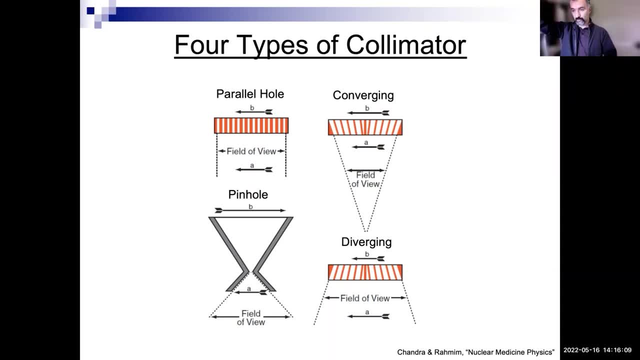 Nowadays because detectors have become bigger and bigger. if you really want the whole body, you just do multiple scans. There's also pinhole collimators, really used a lot in small animal imaging, for example, but also in brain imaging, where you could get really significant amplification. 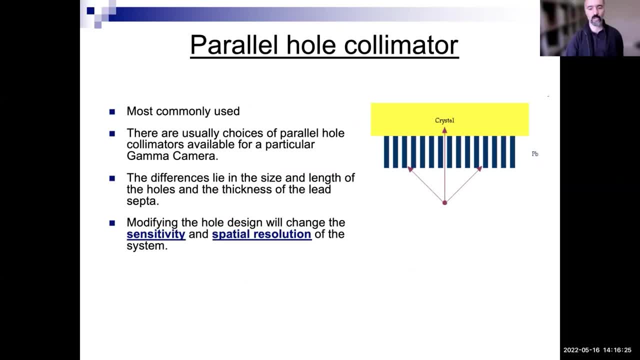 Won't have time to go through these details, But parallel whole collimators are the most common. You'll be seeing. this is where a lot of the quality assurance is happening, with and without these collimators. The size of these holes and the length of the collimators is going to really have a lot to say about the sensitivity and the resolution of the system. 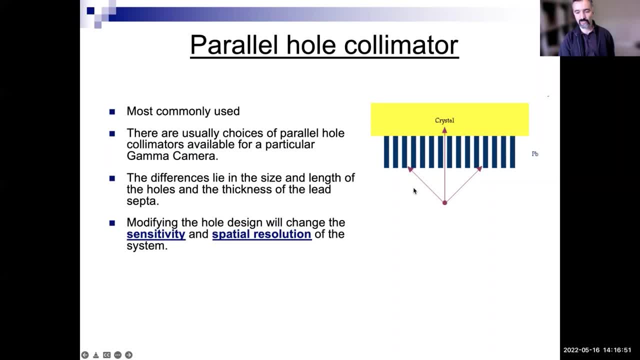 So I'm going to ask you a question: If I make the collimators longer, do you expect the sensitivity of the scanner to drop or to increase? What do you think? Making collimators longer- which means almost more intrusive, more hardcore in some sense, like what, because it's well, I don't want to say it- would it? would it allow you to accept more events, or longer? 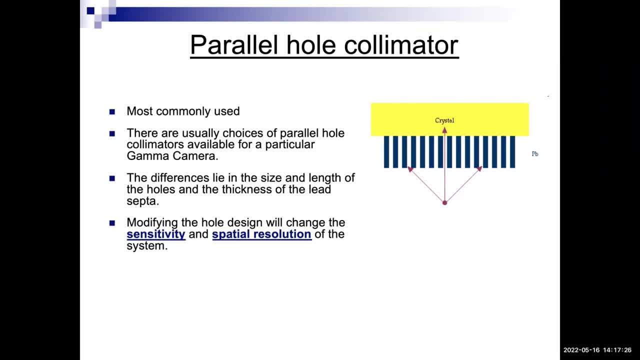 Would it allow you to accept more events or longer? Would it allow you to accept more events or longer? Would it allow you to accept less events? You'd accept less. Yes, So it lowers the sensitivity. So then you would ask: why on earth would you ever want to do that? 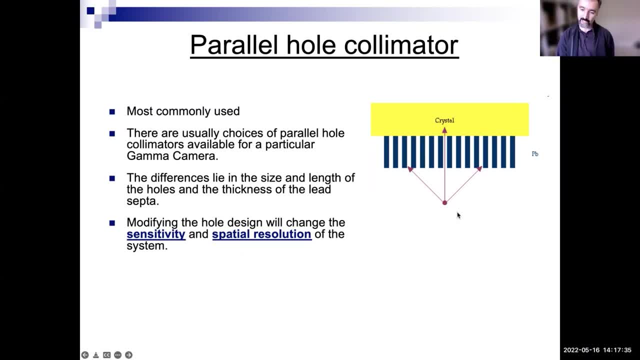 Because it turns out it improves resolution. Because, because it turns out that if you make this even longer, if an event is slightly at an angle and normally might have made it to here, if you make this longer, even that won't be accepted. 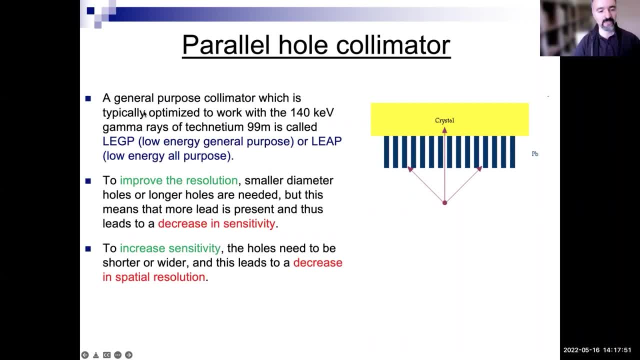 So it actually makes the resolution better. Just hanging there with me, a general purpose collimator is what we typically use with this energy, So we call that low energy general purpose or low energy all purpose leap. But to improve the resolution, 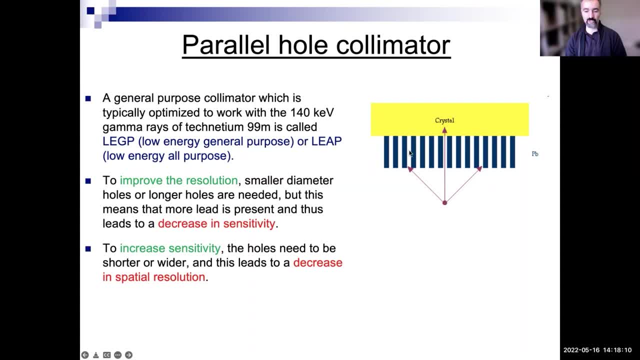 we could do a number of things. We could make the diameter smaller. you could imagine why that would make the resolution better, because in resolution, smaller is better If you want to make the point source appears smaller. Or you could make the holes long. 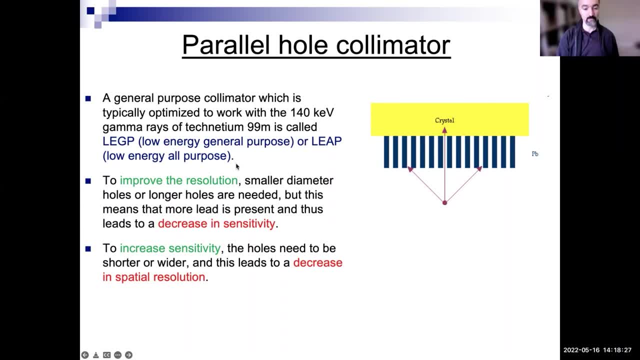 longer, which is what I was just telling you. But both of those results, both of those mean that you're using more lead shielding, as you're making the hole smaller- some thicker lead or longer lead- and that kills more signal. So there's always a trade off. 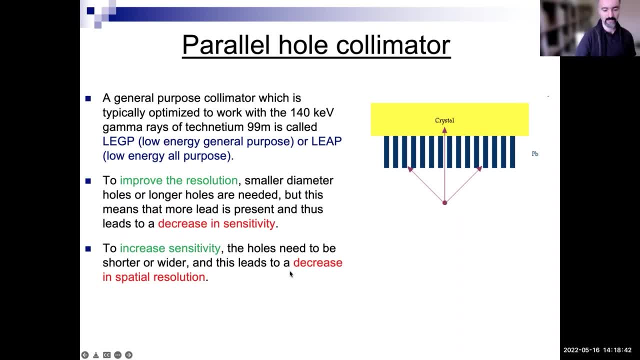 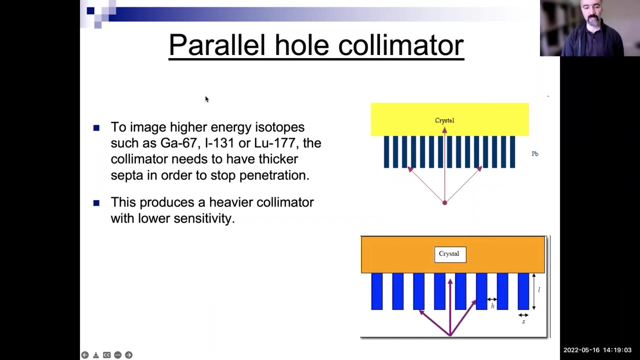 between resolution and sensitivity. So to increase sensitivity, the holes need to be shorter. Right, the holes need to be shorter Or wider, And that results in a decrease in resolution. So there's a trade off. And if you wanna image like high energy isotopes, 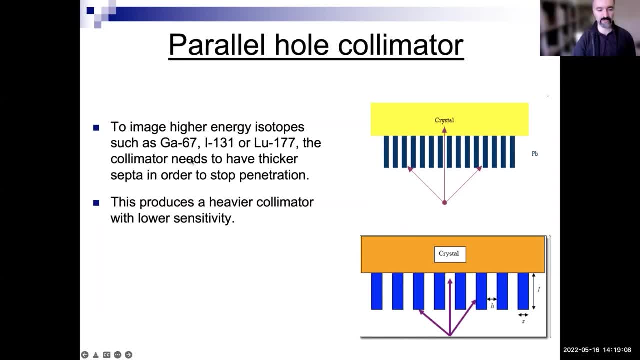 things that are not at 140, but in 200s or 300s. you need to be having thicker septal, because sometimes these highly energetic photons can penetrate, So you make the septa thicker. If you make the septa thicker, 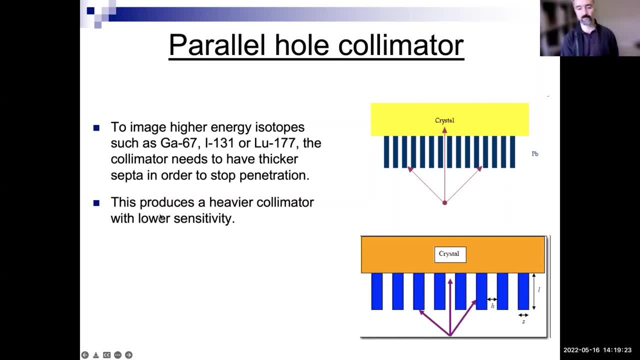 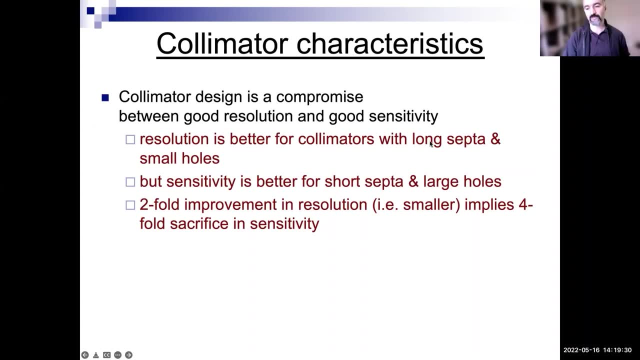 it's a heavier collimator and lower sensitivity, because again, you're killing more and more signal. So there's always a trade off. But if you wanna remember this, basically resolution is better for collimators with long septa and small holes, but sensitivity is better for short septa and large holes. 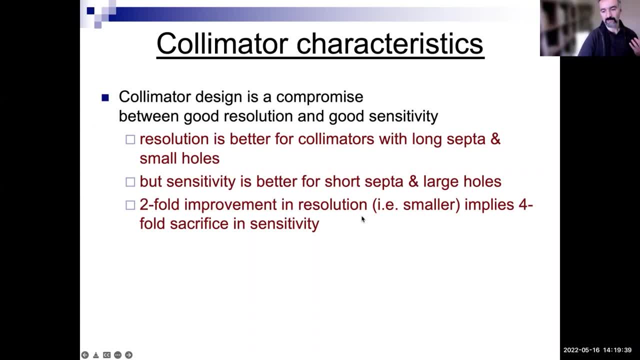 And turns out a twofold improvement in resolution, meaning getting two times smaller, which means two times better resolution means you have to sacrifice four times in sensitivity. We won't show the math here, but just remember it If you wanna improve the resolution. 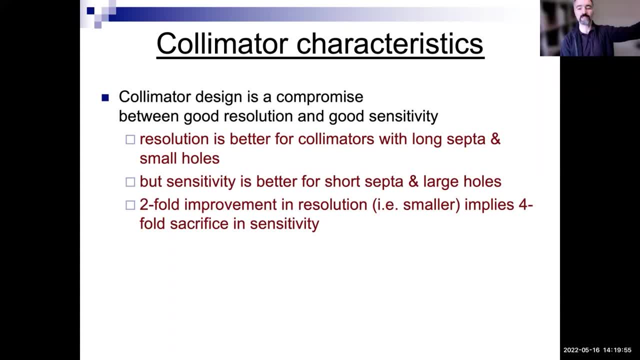 like: if you wanna go from four millimeter- like one- sorry, one- centimeter- resolution to five millimeter resolution, right. so if you want to go from 10 millimeter resolution to five millimeter resolution, factor of two improvement resolution, you're going to have to kill four times as much signal, which is not great. there's a trade-off. 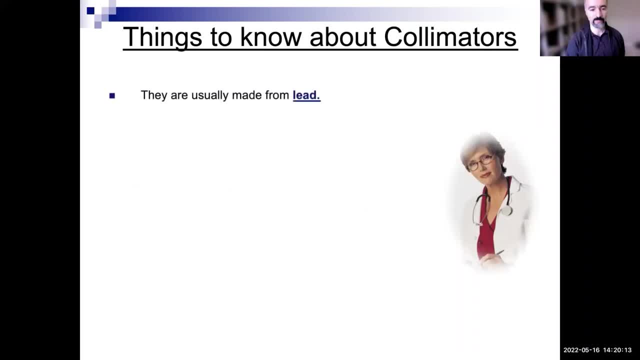 so things to know about. collimators are usually made from lead, typically hexagonal. the lead strips between holes are called septum. parahole collimators project the same object size. they're looking parallel, they're not converging or diverging, and high energy radionuclides require higher energy collimators, meaning thicker septum. 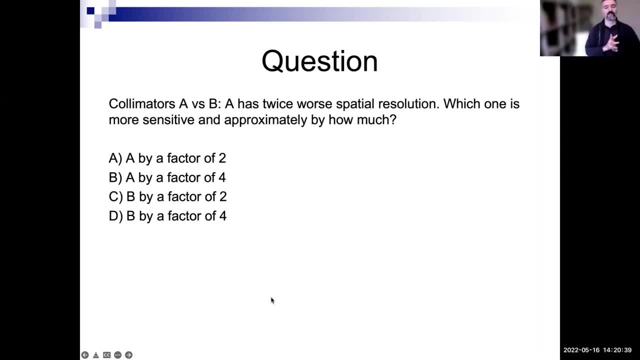 so let's, let's try to answer this. you got a collimator a versus b. a has twice worse, poorer spatial resolution. you got a collimator a versus b. a has twice worse, poorer spatial resolution. you got a collimator a versus b. a has twice worse, poorer spatial resolution. 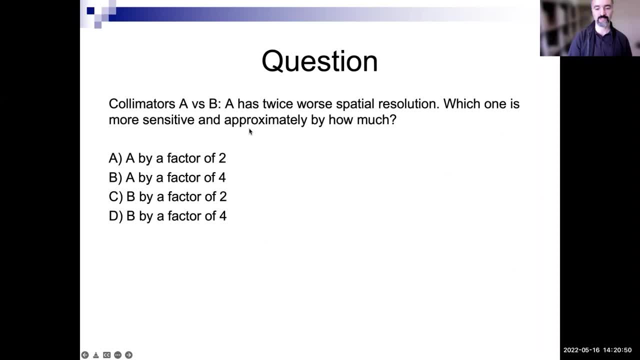 which one is more sensitive, and approximately by how much. a is worse or b in terms of sensitivity, or, sorry, which one is better? which one is more sensitive? a, oh no, hang in there. hang in there. a is worse. spatial resolution. so it's more sensitive, yes, but by a factor of how much, uh. 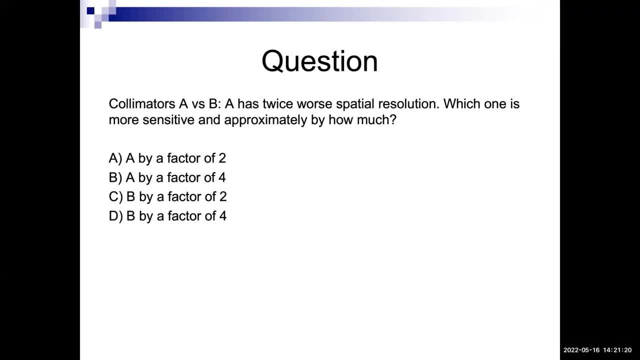 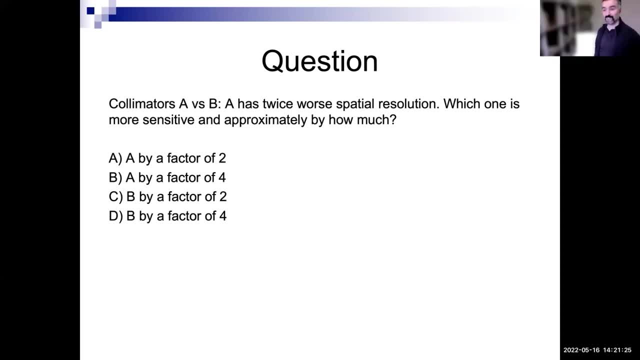 twice the worse. uh, i i think my twice the worse. uh, i i think my factor of two, but i i probably missed it twice, factor of two, but i i probably missed it twice, factor of two, but i i probably missed it twice as the twice, because it's twice twice. 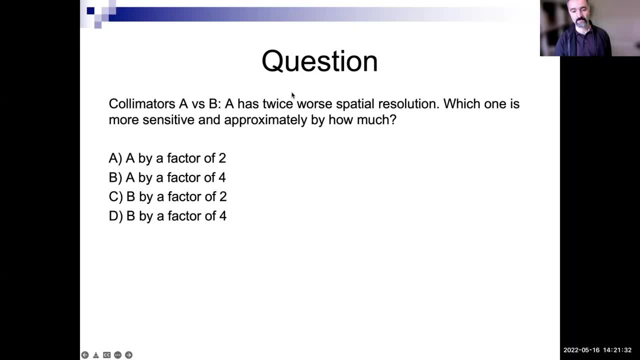 as the twice, because it's twice, twice as the twice because it's twice twice. if this is twice as worse, if this is twice as worse, if this is twice as worse, this will be four times as worse, right? this will be four times as worse, right? this will be four times as worse, right? because we said here: 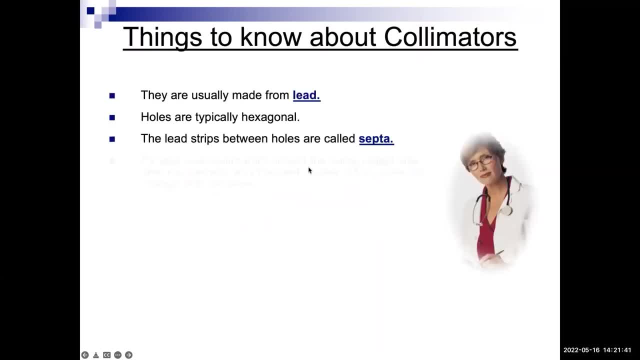 because we said here. because we said here: a twofold by two, this will be fourfold. a twofold by two, this will be fourfold. a twofold by two, this will be fourfold. yeah, yeah, okay. so the answer therefore: yeah, yeah, okay. so the answer therefore: 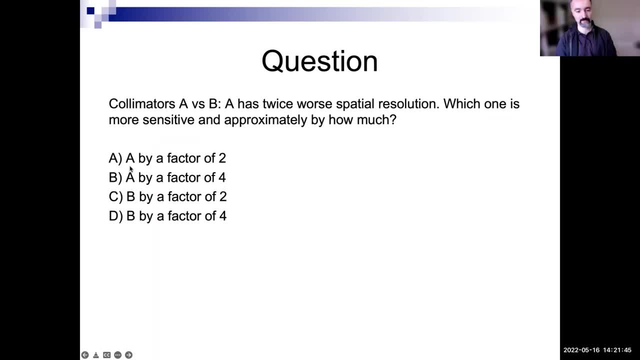 yeah, yeah, okay, so the answer therefore: thank you for that ali. the answer is: thank you for that ali. the answer is: thank you for that ali. the answer is therefore therefore: therefore: b a is worse in resolution, but it's. b a is worse in resolution, but it's. 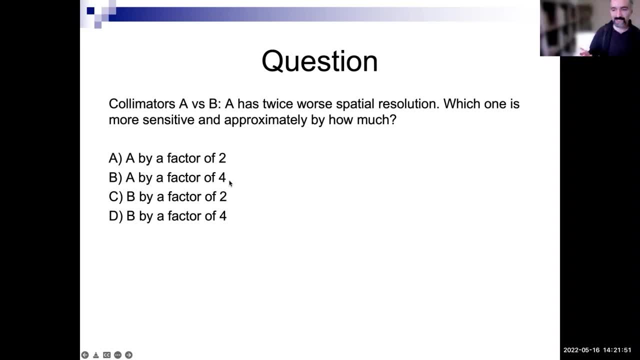 b a is worse in resolution, but it's better in sensitivity by a factor of four, better in sensitivity by a factor of four, better in sensitivity by a factor of four. so it depends on the application right. so it depends on the application right. so it depends on the application right. if your application cares about. 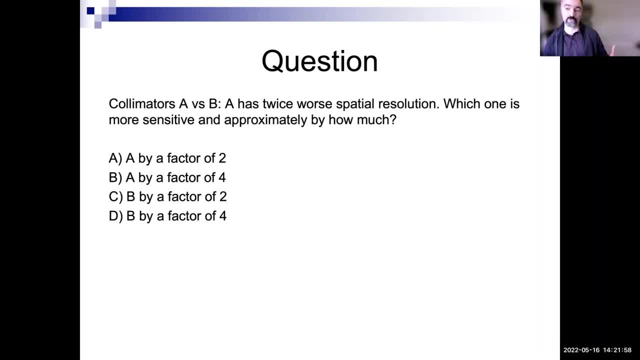 if your application cares about, if your application cares about resolution, then you got to give up on resolution. then you got to give up on resolution, then you got to give up on you're going to get more noise. but if you're going to get more noise, but if 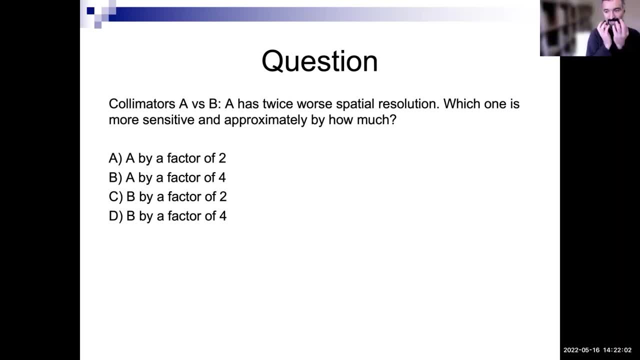 you're going to get more noise. but if you, your application really cares about you, your application really cares about you, your application really cares about the signal, the quality, the amount of the signal, the quality, the amount of the signal, the quality, the amount of signal, the signal, the reduce noise levels, then you might be. 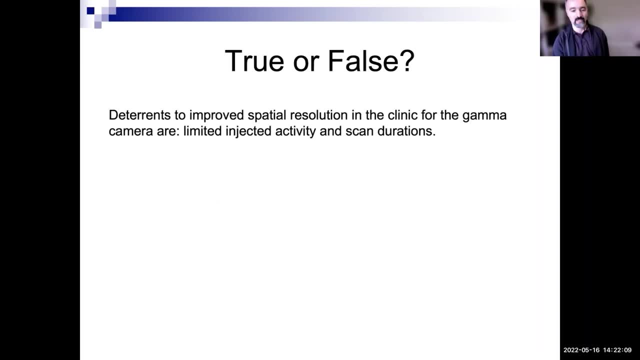 signal the reduce noise levels, then you might be signal the reduce noise levels, then you might be getting getting getting poorer resolution um, poorer resolution, um, poorer resolution, um. so here's a question: is this true or so? here's a question: is this true or so? here's a question: is this true or false? deterrence to improved resolution. 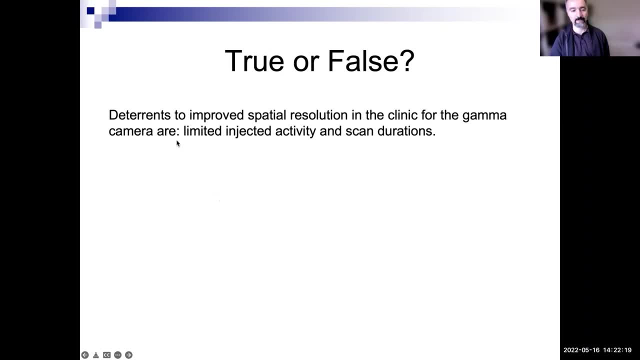 false deterrence to improved resolution. false deterrence to improved resolution or special resolution in the clinic or special resolution in the clinic or special resolution in the clinic for the gamma camera are limited. injected for the gamma camera are limited. injected for the gamma camera are limited. injected activity. 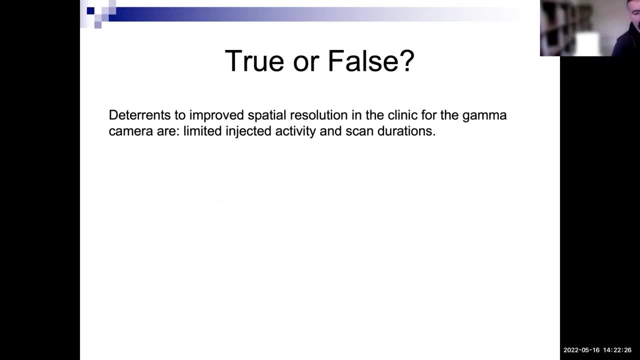 activity. activity and scan durations: is it true and scan durations: is it true and scan durations? is it true that a deterrent, an impediment to us, that a deterrent an impediment to us, that a deterrent, an impediment to us getting better spatial resolution in the. getting better spatial resolution in the. 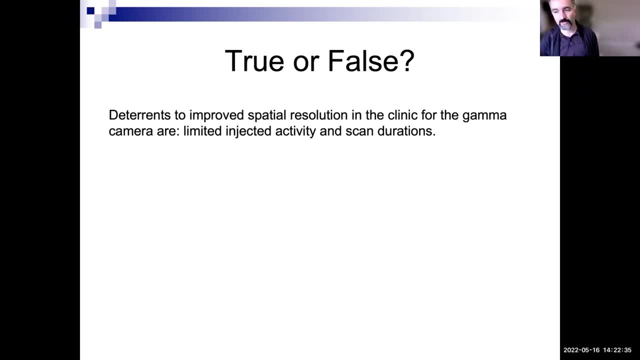 getting better spatial resolution in the clinic clinic. clinic is that we can only inject our patients? is that we can only inject our patients? is that we can only inject our patients with a certain amount of signal and we with a certain amount of signal and we with a certain amount of signal and we can only inject them for a certain or? 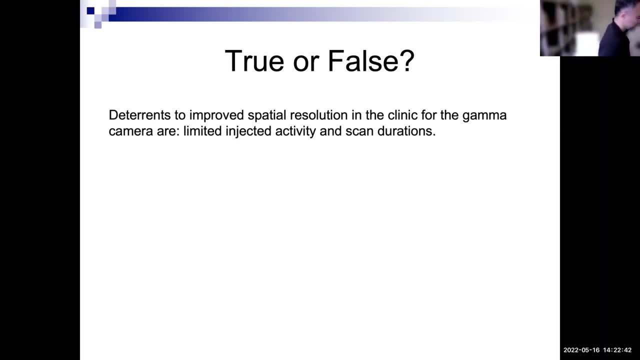 can only inject them for a certain, or can only inject them for a certain or limited duration of time. is this true? limited duration of time: is this true? limited duration of time: is this true or false? what do you think? it's a weird compounded question, i think. 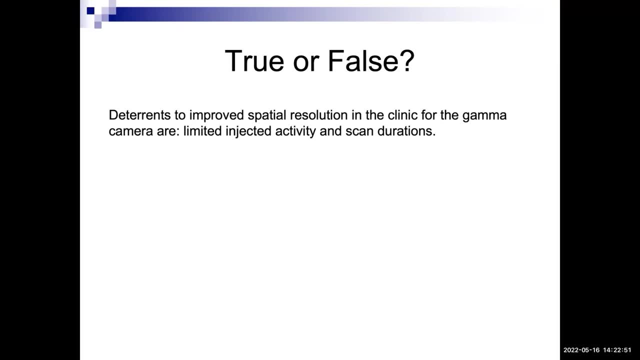 it's a weird compounded question. i think it's a weird compounded question. i think it's false. it's false. it's false because it has more to do with the, because it has more to do with the, because it has more to do with the collimator. 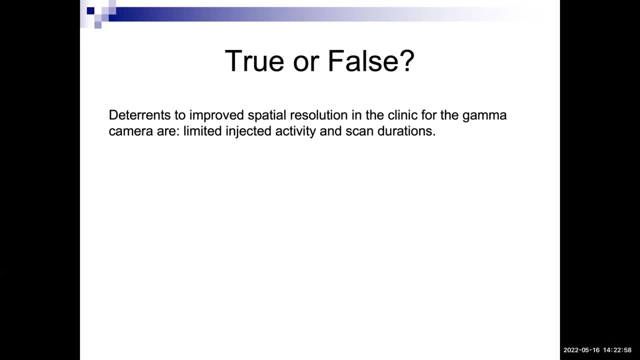 collimator. collimator- right, so? so, let's, let's work through this, right, so, so, let's, let's work through this, right, so, so, let's, let's work through this. uh, uh, uh, if you want to get improved spatial, if you want to get improved spatial, 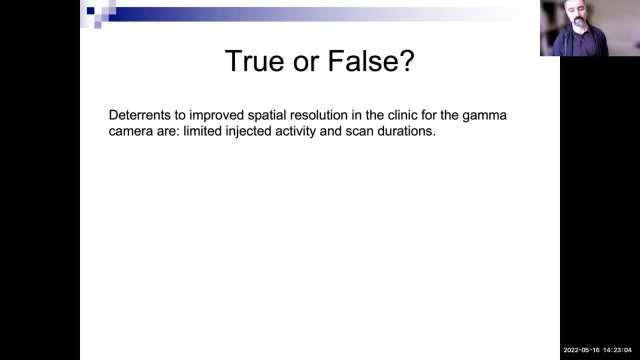 if you want to get improved spatial resolution. resolution, resolution, what, what? what does it mean in terms of column or in? does it mean in terms of column or in? does it mean in terms of column or in terms of sensitivity? terms of sensitivity? terms of sensitivity: it means that the sensitivity will be. 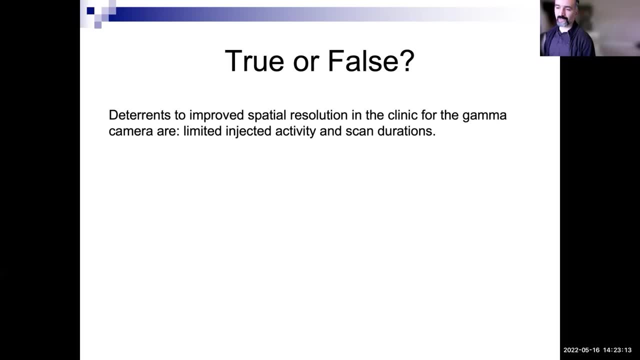 it means that the sensitivity will be. it means that the sensitivity will be not as good. right, but imagine if you are not as good. right, but imagine if you are not as good. right, but imagine if you are allowed to in, allowed to in, allowed to in to image a patient for a very long time. 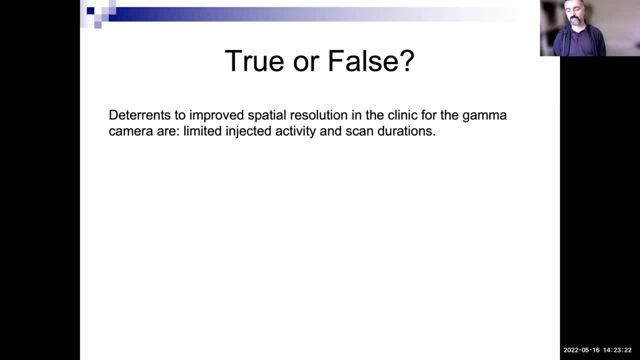 to image a patient for a very long time. to image a patient for a very long time, even though sensitivity in this device, even though sensitivity in this device, even though sensitivity in this device is poor, but since you're getting more and is poor, but since you're getting more and 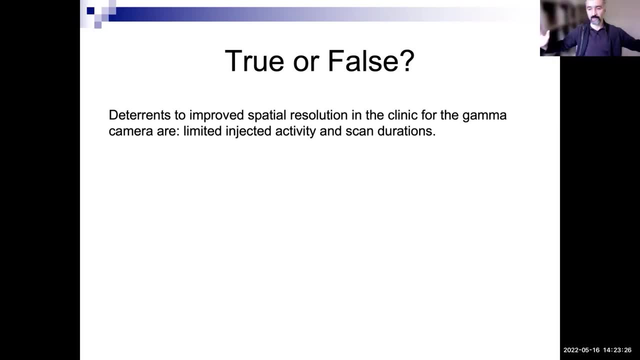 is poor, but since you're getting more and more and more signal, because you're more and more and more signal, because you're more and more and more signal, because you're imaging over a long time, you can imaging over a long time, you can imaging over a long time you can. you know safety concerns, you can inject. 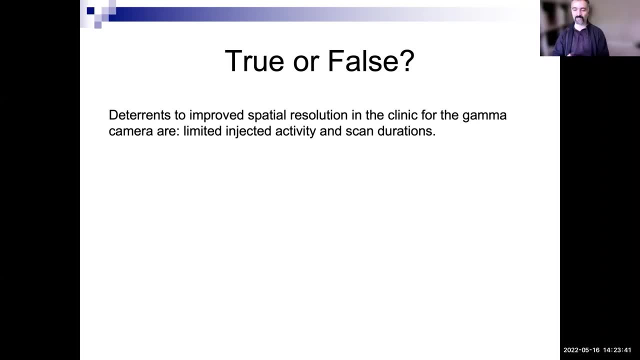 you know safety concerns. you can inject. you know safety concerns. you can inject as much. you could make up for the loss as much. you could make up for the loss as much. you could make up for the loss of signal by just injecting more into of signal, by just injecting more into. 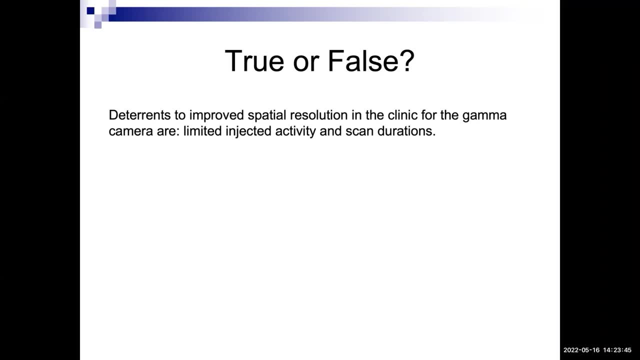 of signal by just injecting more into the patient, the patient, the patient okay so technically, some way that we okay so technically, some way that we okay so technically, some way that we amplify the signal to noise ratios in, amplify the signal to noise ratios in, amplify the signal to noise ratios in patients. so 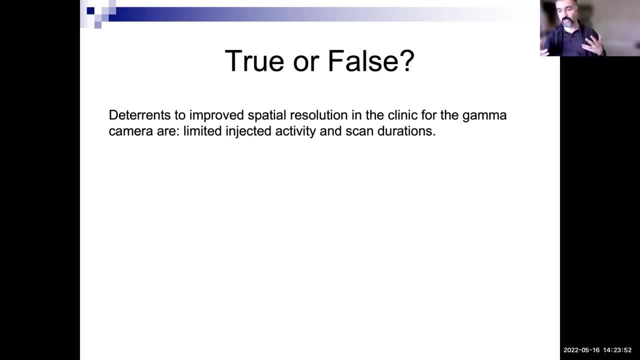 patients, so patients, so we make up for the fact that we don't. we make up for the fact that we don't. we make up for the fact that we don't have great sensitivity. sometimes is we have great sensitivity, sometimes is we have great sensitivity, sometimes is we just inject them more, or just inject them more. or just inject them more. or we scan them for longer, but there's a. we scan them for longer, but there's a. we scan them for longer, but there's a limit to this. you cannot inject the limit to this. you cannot inject the. 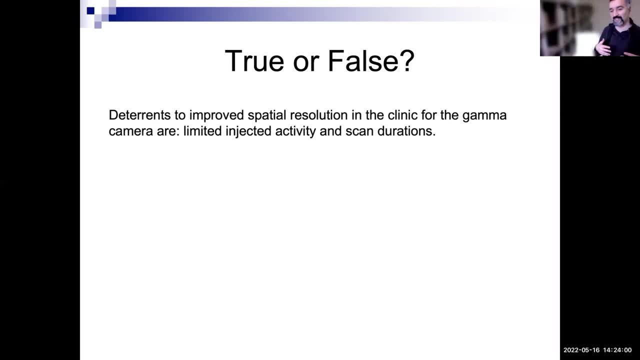 limit to this. you cannot inject the patient too much. patient too much, patient too much, way too much, and you cannot scan them way too much. and you cannot scan them way too much and you cannot scan them for way too much for practical reasons, for way too much, for practical reasons. 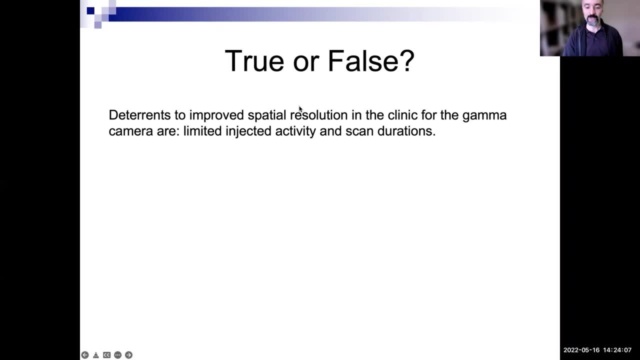 for way too much for practical reasons. therefore, if these concerns were not, therefore, if these concerns were not, therefore, if these concerns were not there, there, there, we could be getting very good spatial. we could be getting very good spatial. we could be getting very good spatial resolution because- because we could be- 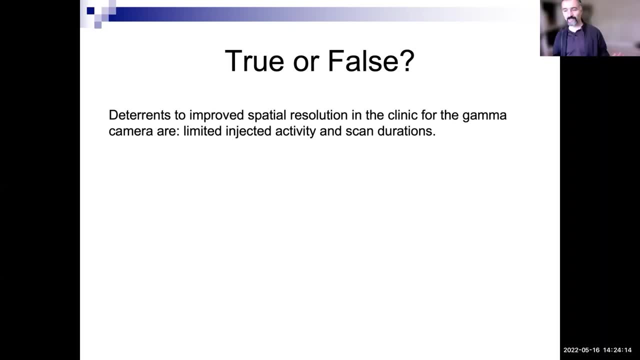 resolution. because because we could be resolution, because because we could be designing collimators that are awful in designing collimators that are awful in designing collimators that are awful in terms of sensitivity but fantastic in terms of sensitivity, but fantastic in terms of sensitivity, but fantastic in terms of spatial resolution. and we would 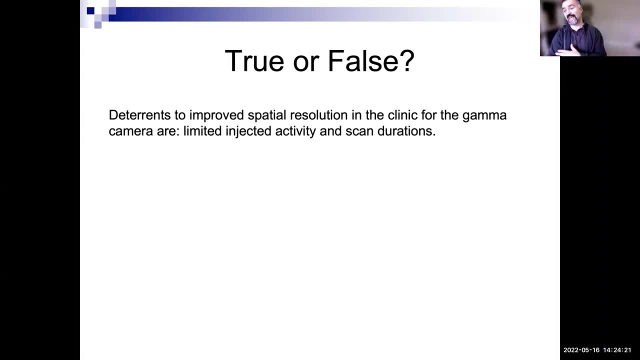 terms of spatial resolution, and we would terms of spatial resolution and we would make up for that terrible make up for that terrible make up for that terrible sensitivity by just scanning forever, sensitivity by just scanning forever, sensitivity by just scanning forever. we can't do that, we can't do that. 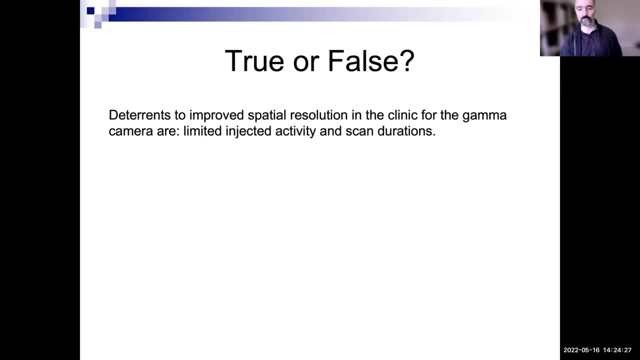 we can't do that. so this sentence it's a convoluted. so this sentence it's a convoluted. so this sentence it's a convoluted sentence, but it's actually true sentence. but it's actually true sentence, but it's actually true um. 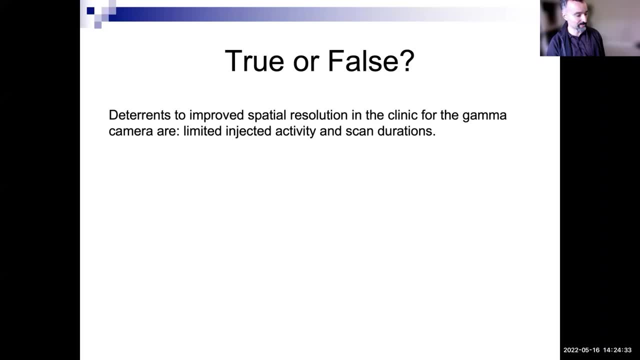 um, um, and that's why you, you might hear that, and that's why you, you might hear that, and that's why you, you might hear that there are some mri protocols of, there are some mri protocols of, there are some mri protocols of, uh, carcasses, uh, or things of the sort. 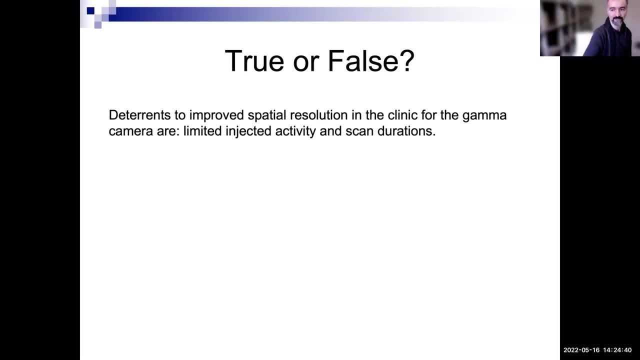 uh, carcasses, uh or things of the sort. uh, carcasses, uh or things of the sort, but they get amazing spatial resolution. but they get amazing spatial resolution. but they get amazing spatial resolution because they scan the carcass for like. because they scan the carcass for like. 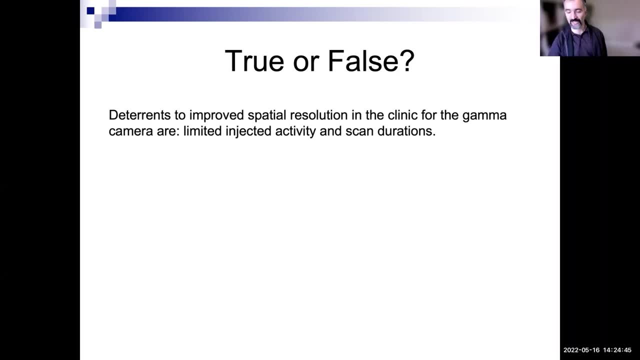 because they scan the carcass for like 12 hours or 14 hours overnight mri scan. 12 hours or 14 hours overnight mri scan. 12 hours or 14 hours overnight mri scan. you get like, you get like, you get like sub millimeter resolutions that are. 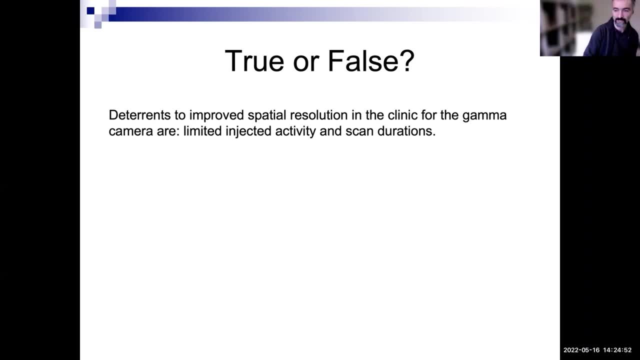 sub millimeter resolutions that are sub millimeter resolutions that are mind-blowing, but you can't do that with mind-blowing. but you can't do that with mind-blowing, but you can't do that with real life patients, real life patients. 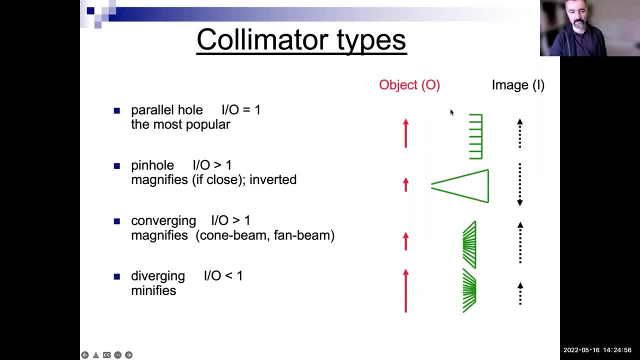 real life patients. okay, and collimator types are different. okay, and collimator types are different. okay, and collimator types are different. as i mentioned, there's parallel ones. as i mentioned, there's parallel ones. as i mentioned, there's parallel ones, there's pinhole, pinholes and converging. 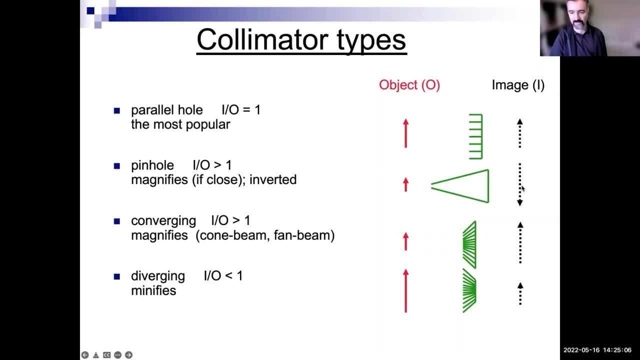 there's pinhole pinholes and converging. there's pinhole pinholes and converging have somewhat similar properties in the have somewhat similar properties in the have somewhat similar properties in the sense that they make the image of, the sense that they make the image of the. 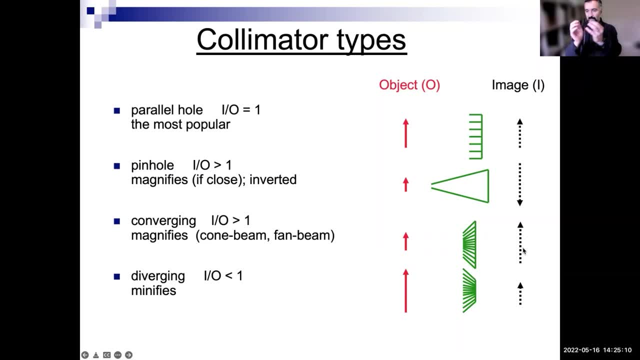 sense that they make the image of the object, object, object bigger, bigger, bigger they make the image bigger. therefore they make the image bigger, therefore they make the image bigger. therefore they have better resolution, like even in. they have better resolution, like even in. they have better resolution, like even in. that kind of detail can be amplified. 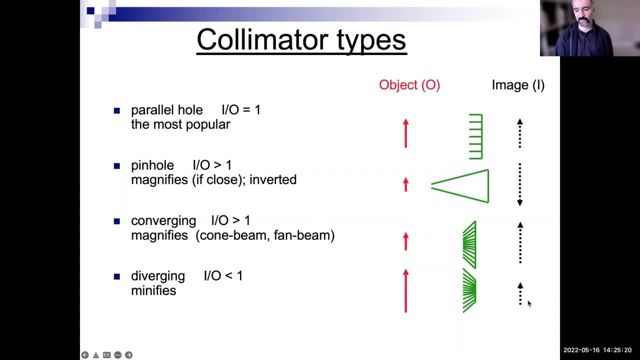 that kind of detail can be amplified. that kind of detail can be amplified. diverging the ratio of the image to the. diverging the ratio of the image to the. diverging the ratio of the image to the object is actually less so you could be. object is actually less so you could be. 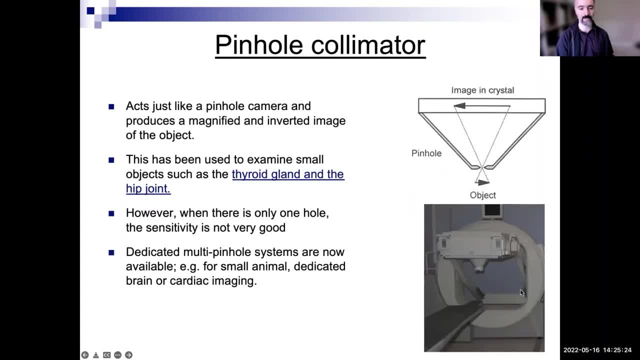 object is actually less so you could be imaging like a whole body in a single imaging, like a whole body in a single imaging, like a whole body in a single small detector. depends on the small detector, depends on the small detector, depends on the application, application, application. just a quick uh comment about this. and 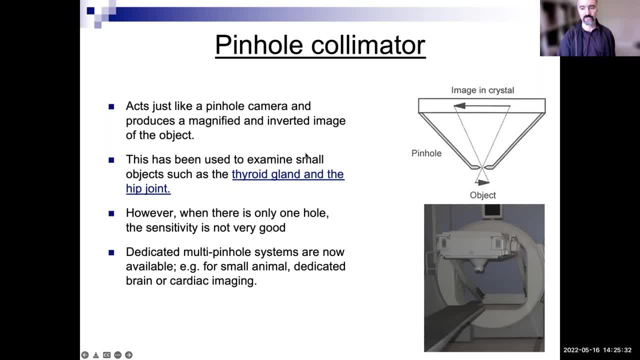 just a quick uh comment about this and just a quick uh comment about this, and then we're gonna, then we're gonna, then we're gonna take a break. pinhole collimators are: take a break. pinhole collimators are take a break. pinhole collimators are like a pinhole camera, actually like 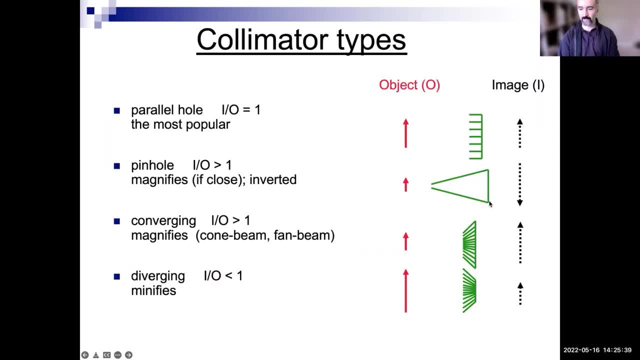 like a pinhole camera actually. like like a pinhole camera, actually. like. you've heard of pinholes, they do. you've heard of pinholes, they do. you've heard of pinholes. they do. invert the image unlike everything else. invert the image unlike everything else. invert the image unlike everything else that we're having here: pinhole. 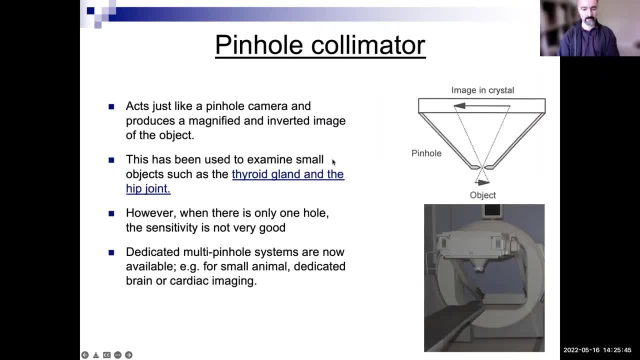 that we're having here pinhole that we're having here pinhole kilometers. invert the image, but that's kilometers. invert the image, but that's kilometers invert the image, but that's okay, okay, okay, um. so this has been used in the past to um. so this has been used in the past to. 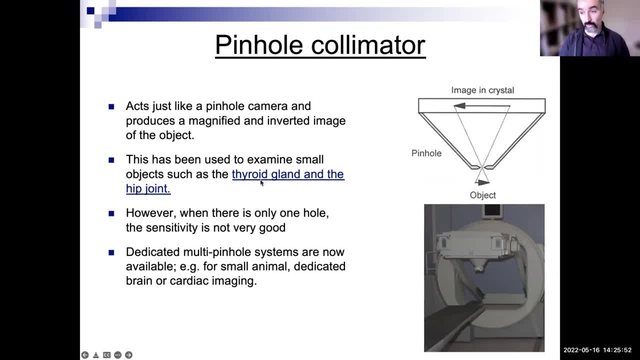 um, so this has been used in the past to examine small objects. because you really examine small objects, because you really examine small objects, because you really tune into an object or a small animal, tune into an object or a small animal, tune into an object or a small animal- tremendous applications actually in. 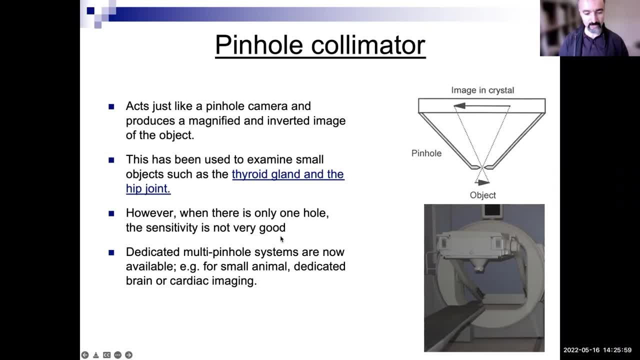 tremendous applications actually in tremendous applications, actually in small animals in pre-clinical imaging, small animals in pre-clinical imaging, small animals in pre-clinical imaging. and now there is increasingly multi, and now there is increasingly multi, and now there is increasingly multi pinhole systems where you don't cover. 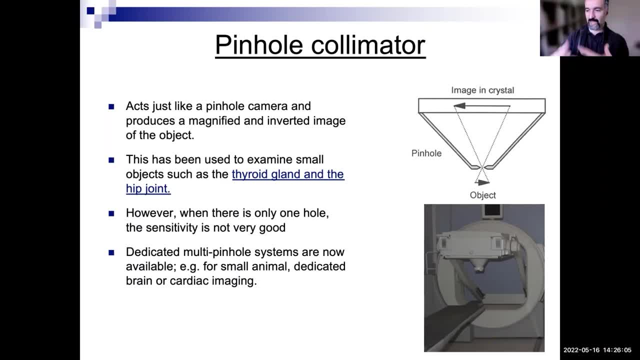 pinhole systems, where you don't cover pinhole systems, where you don't cover just a single small area, you cover just a single small area. you cover just a single small area. you cover multiple areas and you patch them in a multiple areas and you patch them in a. 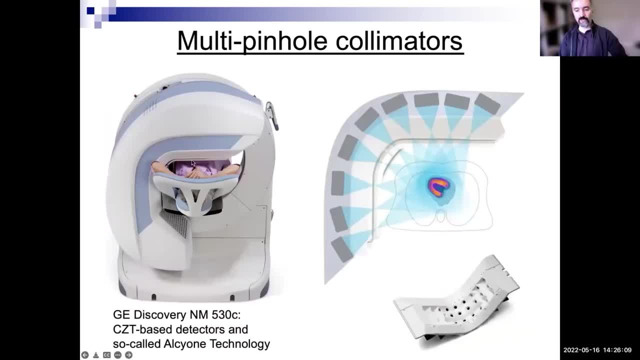 multiple areas and you patch them in a sense together, sense together, sense together. so so there are really great um i so. so there are really great um i, so so there are really great um. i mentioned brain applications, but also um mentioned brain applications, but also um mentioned brain applications, but also um. you know, cardiac, dedicated cardiac, you. 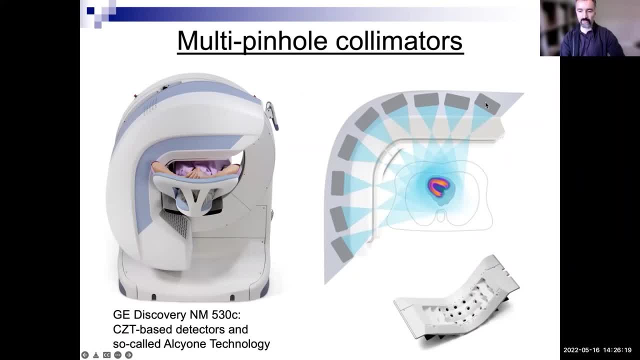 you know cardiac dedicated cardiac. you you know cardiac, dedicated cardiac. you could do using the concept of could do, using the concept of could do using the concept of pinholes, where, using each of these pinholes, where, using each of these pinholes, where, using each of these pinholes, you might be covering different. 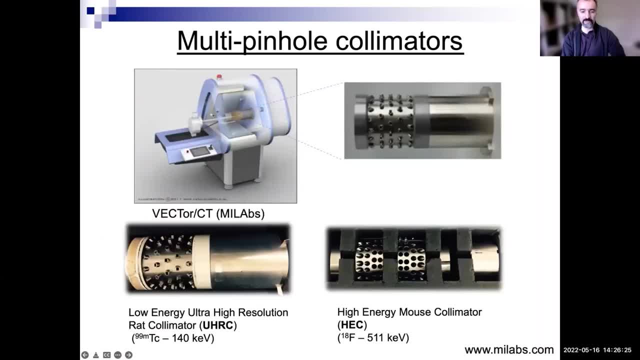 pinholes. you might be covering different pinholes. you might be covering different parts of the parts, of the parts of the the body um small animal imaging. when the body um small animal imaging. when the body um small animal imaging when you're inserting the animals in here. 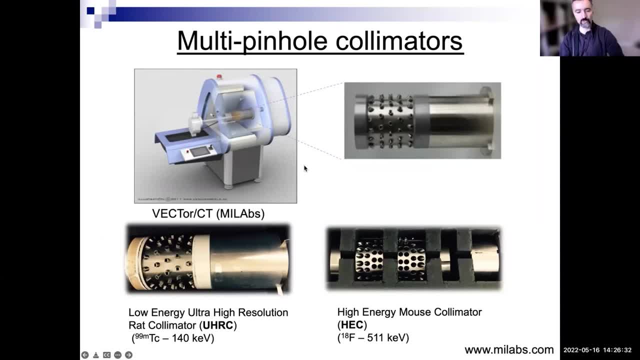 you're inserting the animals in here. you're inserting the animals in here. in holes are covering different parts of. in holes are covering different parts of. in holes are covering different parts of the body: the body, the body. super high, you could do amazing stuff. super high, you could do amazing stuff. 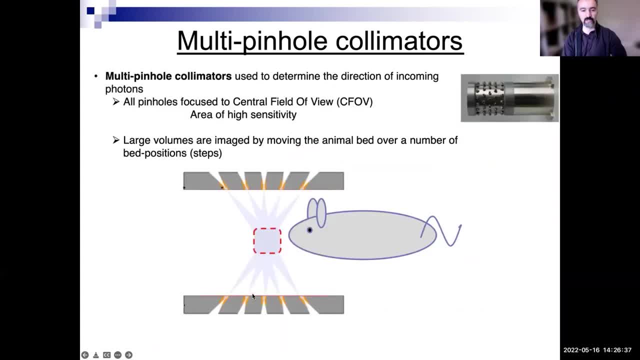 super high. you could do amazing stuff with super high resolution imaging, with, with super high resolution imaging, with, with super high resolution imaging, with spec, spec, spec, right. so here's an example. you could be right. so here's an example. you could be right. so here's an example. you could be doing like multi-bed imaging, moving the. 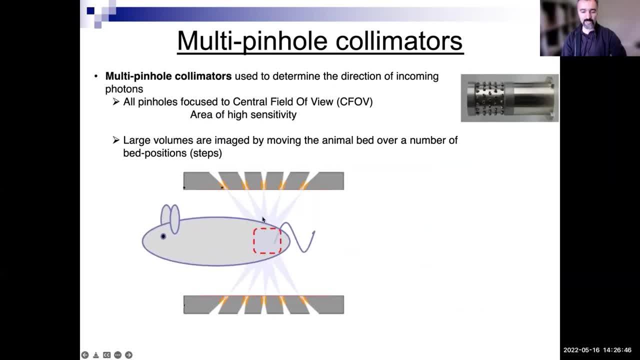 doing like multi-bed imaging: moving the. doing like multi-bed imaging: moving the, the mouse or the rat at different, the mouse or the rat at different, the mouse or the rat at different positions where it's being scanned by positions where it's being scanned by positions where it's being scanned by different pinholes, and getting very, very. 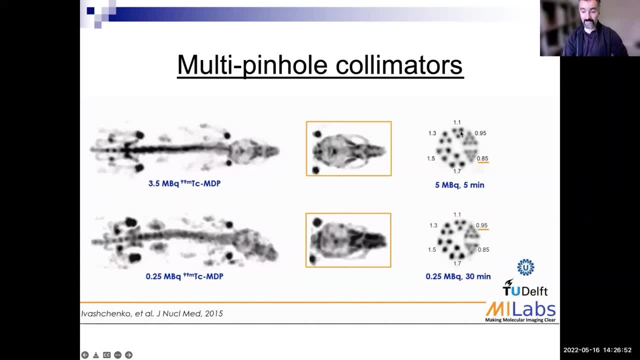 different pinholes and getting very, very different pinholes and getting very, very good resolution, good resolution, good resolution, like amazing resolution. sometimes you like amazing resolution, sometimes you like amazing resolution. sometimes you could like- and these are old images, so could like, and these are old images, so 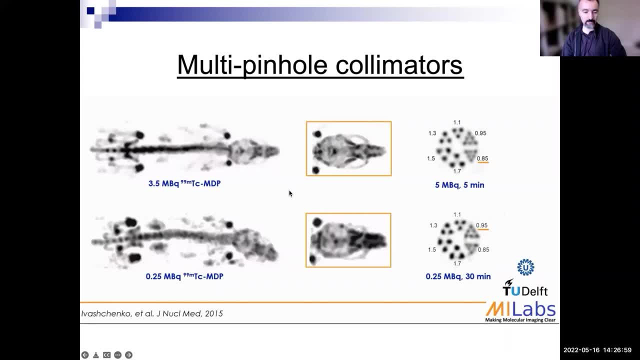 could like, and these are old images, so sub sub millimeter, small animal imaging. sub sub millimeter small animal imaging. sub sub millimeter, small animal imaging. capabilities, capabilities, capabilities um, um, um and spanning beyond you know to primates to and spanning beyond you know to primates to. 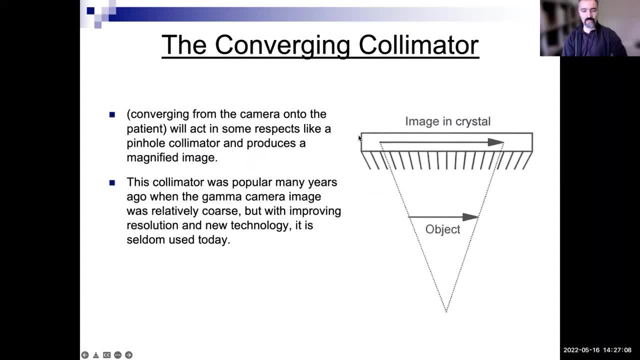 and spanning beyond, you know, to primates, to brain applications and things like this brain applications and things like this brain applications and things like this and the converging collimator um and the converging collimator um and the converging collimator um somewhat related to a pinhole it used to. 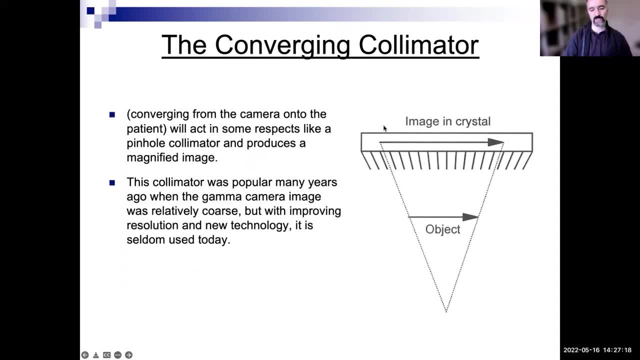 somewhat related to a pinhole. it used to somewhat related to a pinhole. it used to be popular. be popular, be popular, but nowadays because the resolutions of, but nowadays because the resolutions of, but nowadays because the resolutions of these um collimators. sorry of the. these um collimators. sorry of the. 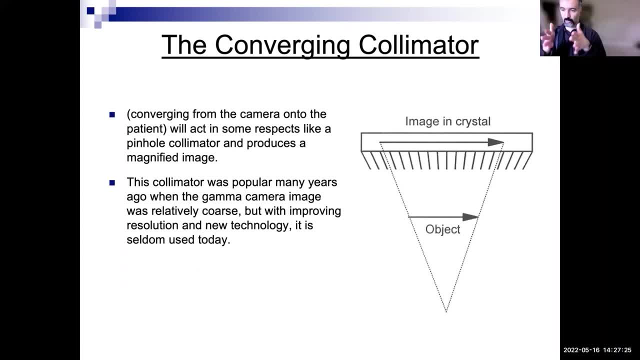 these um collimators, sorry, of the just general resolution of, of even just general resolution of, of even just general resolution of of even parallel hole, parallel hole, parallel hole. you know scintillator systems? have you know scintillator systems? have you know scintillator systems have increased. people do this less often. 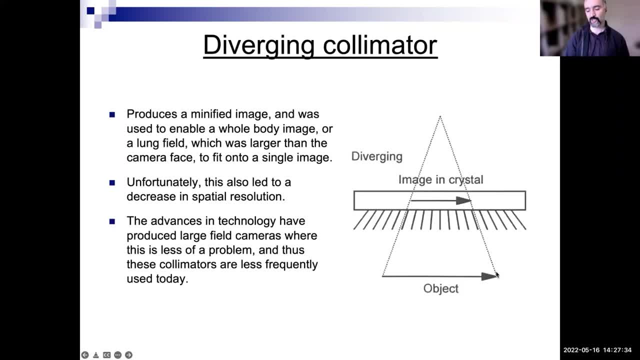 increased people do this less often. increased people do this less often. and diverging again, i mentioned you could. and diverging again, i mentioned you could. and diverging again, i mentioned you could. be imaging a large object in a single. be imaging a large object in a single. 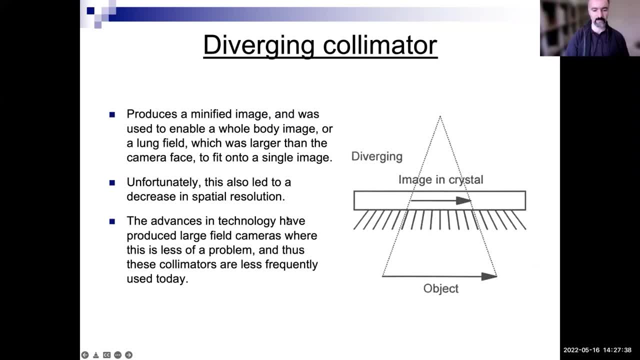 be imaging a large object in a single scan, but again not used that much scan. but again not used that much scan. but again not used that much. because in new technology you just make, because in new technology you just make, because in new technology you just make the detectors bigger and bigger and just. 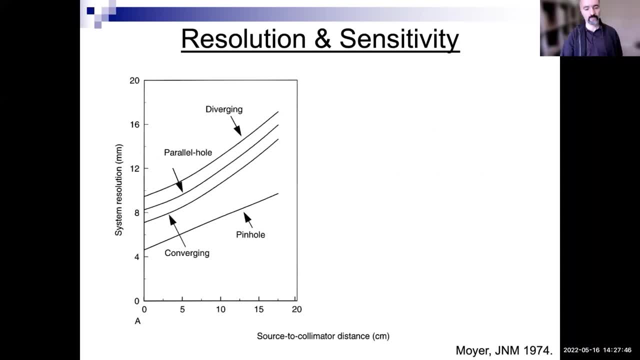 the detectors bigger and bigger, and just the detectors bigger and bigger, and just scan in a couple of bed positions, scan in a couple of bed positions, scan in a couple of bed positions. so if i were to plot this, so if i were to plot this, so if i were to plot this, um. 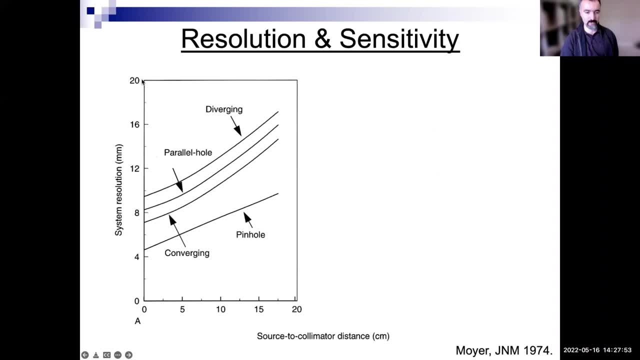 um, um. there is a resolution of a. there is a resolution of a. there is a resolution of a gamma camera depends on the distance of gamma camera. depends on the distance of gamma camera. depends on the distance of the source, the source, the source through the collimators. 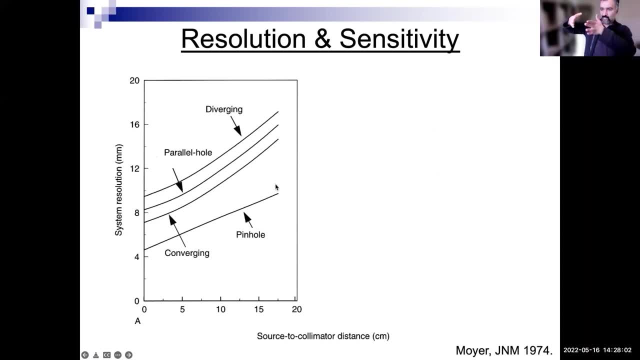 through the collimators, through the collimators, the farther away that you are, it turns, the farther away that you are it turns, the farther away that you are it turns out you get poor resolution because out you get poor resolution, because out you get poor resolution because there's a chance that 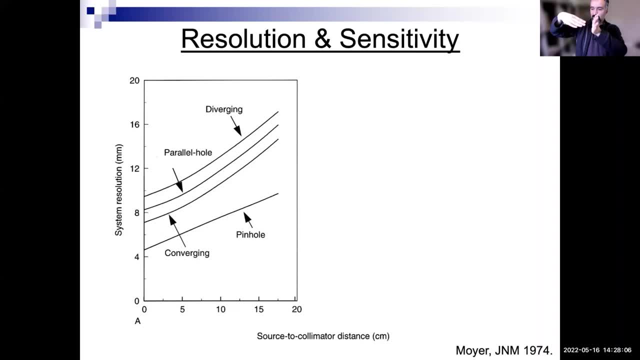 there's a chance that there's a chance that slight angles, even if you're not exactly slight angles, even if you're not exactly slight angles, even if you're not exactly 90 degrees and you're 90 degrees and you're 90 degrees and you're a bit tilted, you're going to make it. and 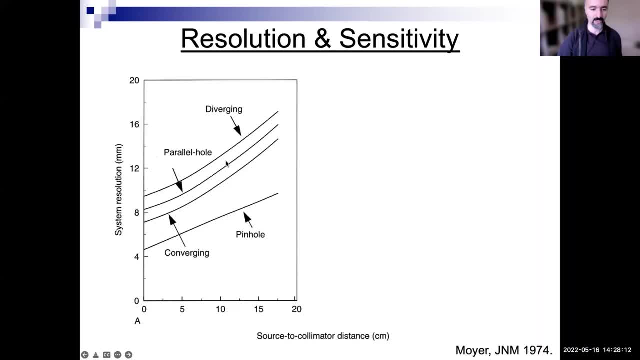 a bit tilted, you're going to make it, and a bit tilted, you're going to make it, and therefore you're going to, therefore, you're going to, therefore you're going to mislead the system so as you get away, mislead the system so as you get away. 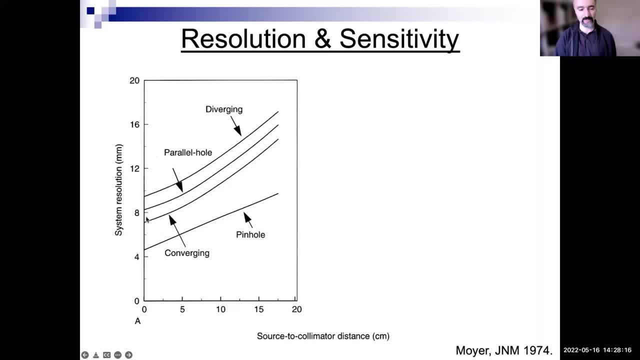 mislead the system. so as you get away from the, from the, from the surface of the collimator, you're going to surface of the collimator. you're going to surface of the collimator, you're going to get poor and poor resolution. get poor and poor resolution. 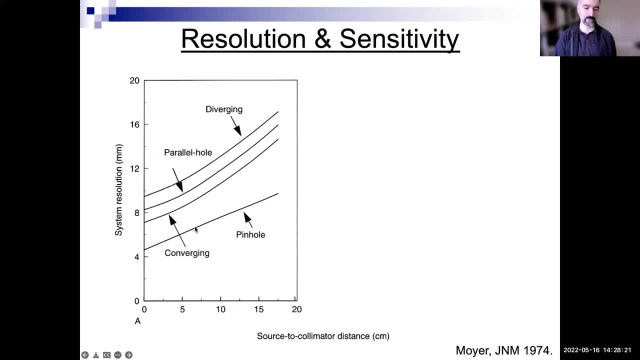 get poor and poor resolution. you can sort of see that the resolutions, you can sort of see that the resolutions, you can sort of see that the resolutions have typically been around, have typically been around, have typically been around. you know we're talking about a scale of. you know we're talking about a scale of 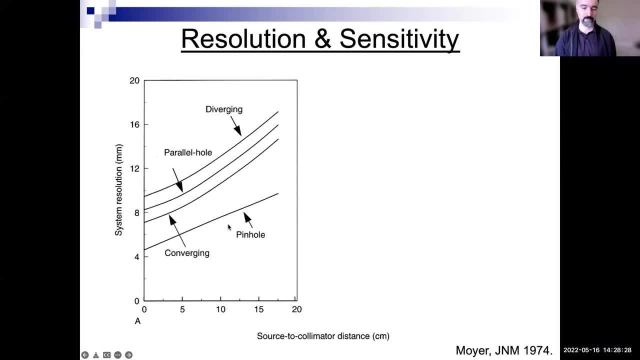 you know, we're talking about a scale of, let's say, one centimeter, let's say one centimeter, let's say one centimeter. okay, okay, okay, of course things are getting better. um, of course things are getting better. um, of course things are getting better, um, but yeah again, why is that happening? just, 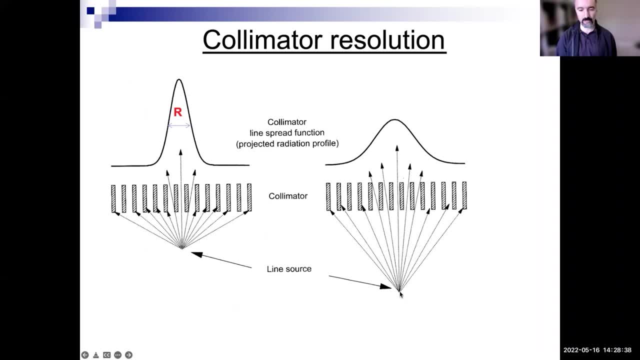 but yeah again. why is that happening? just but yeah again. why is that happening? just look at these. imagine you got a point. look at these. imagine you got a point. look at these. imagine you got a point. source here and point source here. source here and point source here. 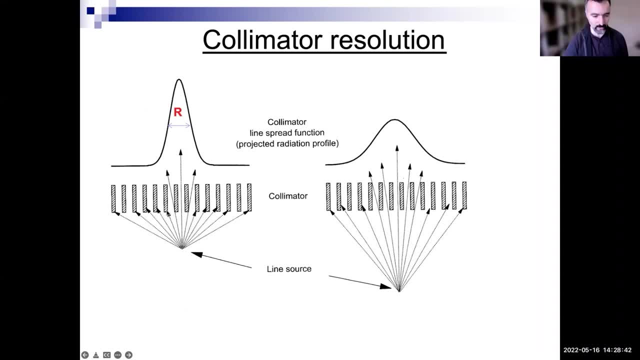 source here and point source here: this point source, it turns out. this point source, it turns out, this point source, it turns out. these two, these two, these two events will be rejected by it. events will be rejected by it. events will be rejected by it here, these two events, just because of 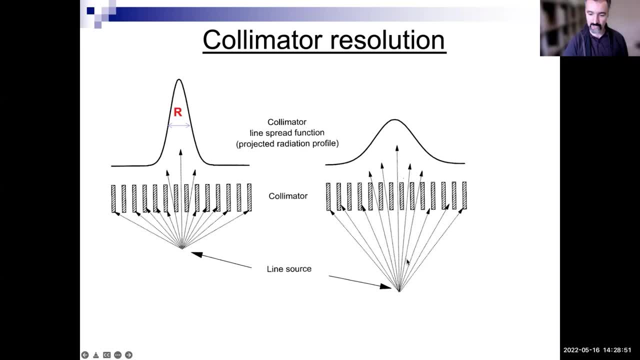 here these two events, just because of here, these two events, just because of angular like geometry will be accepted. angular like geometry will be accepted. angular like geometry will be accepted. so a slightly wider deviations from 90, so a slightly wider deviations from 90, so a slightly wider deviations from 90 degrees will be accepted. 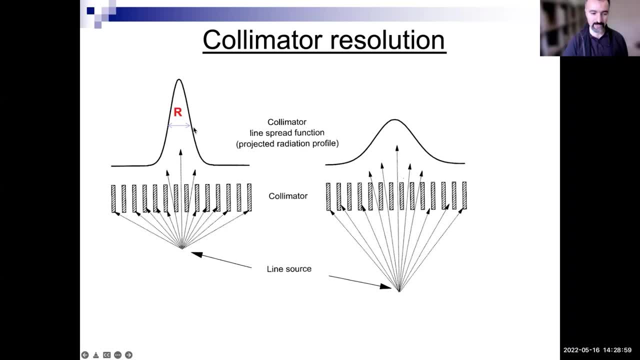 degrees will be accepted, degrees will be accepted. so, even though here you will be rejecting so, even though here you will be rejecting so, even though here you will be rejecting all these and only accepting a small all these and only accepting a small all these and only accepting a small range of deviation from 90 degree from in. 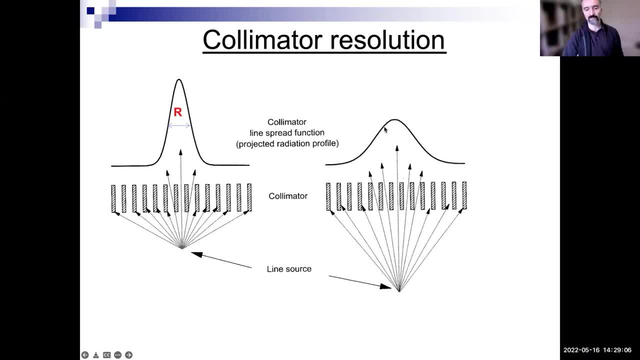 range of deviation from 90 degree from in range of deviation from 90 degree from in normal perpendicular. here you give it a normal perpendicular. here you give it a normal perpendicular. here you give it a little bit more, little bit more, little bit more. therefore, as you get farther away from 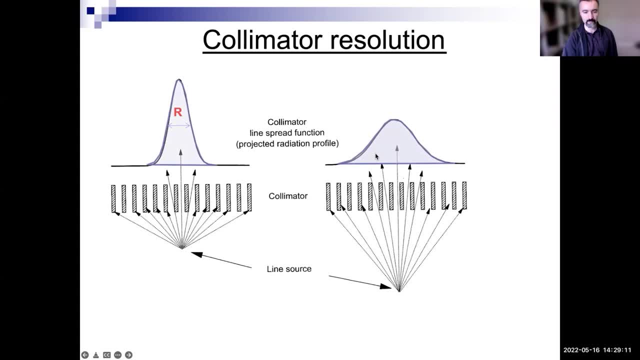 therefore, as you get farther away from, therefore, as you get farther away from collimators, your resolution gets poor, and collimators, your resolution gets poor, and collimators, your resolution gets poor and poor, poor, poor. um, and i want to show you this too, this um, and i want to show you this too: this: 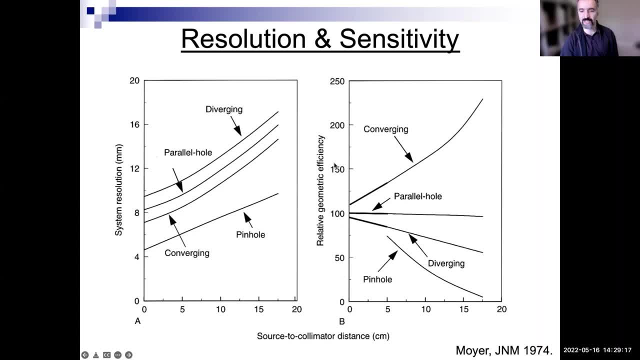 um, and i want to show you this too- this is a plot of not resolution, but just is a plot of not resolution, but just is a plot of not resolution, but just efficiency or sensitivity as we were. efficiency or sensitivity as we were. efficiency or sensitivity as we were talking about. 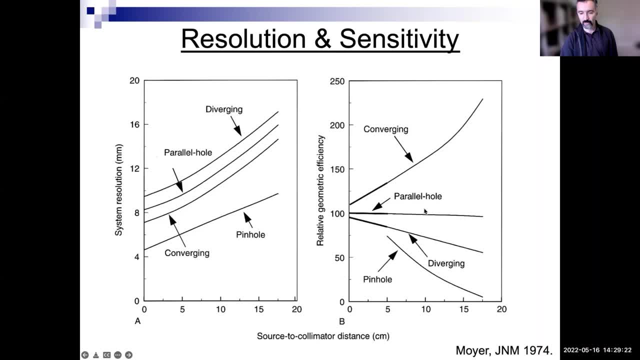 talking about. talking about. there's a bit of a difference here in. there's a bit of a difference here in. there's a bit of a difference here in. a parallel hole collimator doesn't matter. a parallel hole collimator doesn't matter. a parallel hole collimator doesn't matter if you're close to me or farther away. if you're close to me or farther away. if you're close to me or farther away from me, sensitivity is a sensitivity from me. sensitivity is a sensitivity from me. sensitivity is a sensitivity. the events are coming at 90 degrees i. the events are coming at 90 degrees i. the events are coming at 90 degrees. i don't care if you're close to me or don't care if you're close to me or don't care if you're close to me or farther away from you. i'm going to be farther away from you. i'm going to be. 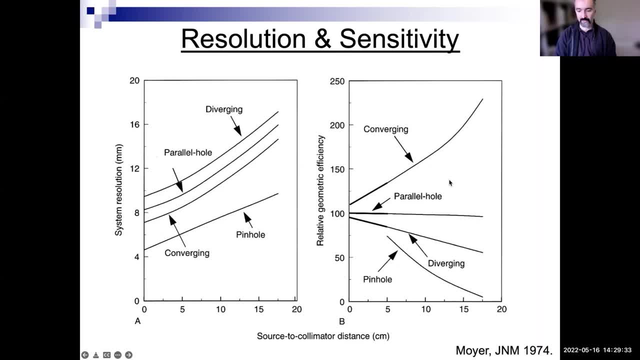 farther away from you, i'm going to be able to see you able to see you, able to see you. but it turns out that um in. but it turns out that um in. but it turns out that um in in a, for example, diverging, or a in a, for example, diverging or a. 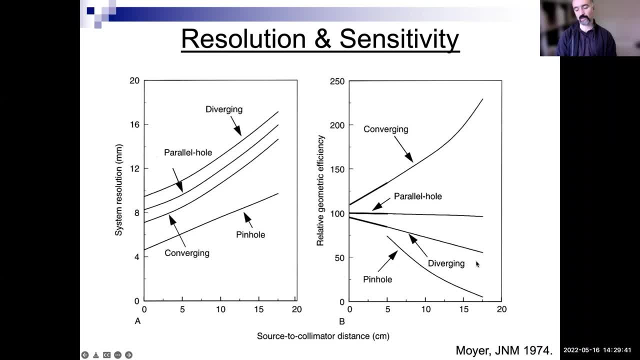 in a, for example, diverging or a pinhole system. as you get farther away, pinhole system as you get farther away. pinhole system as you get farther away, i'm gonna have a do a poor, poorer job. i'm gonna have a do a poor, poorer job. 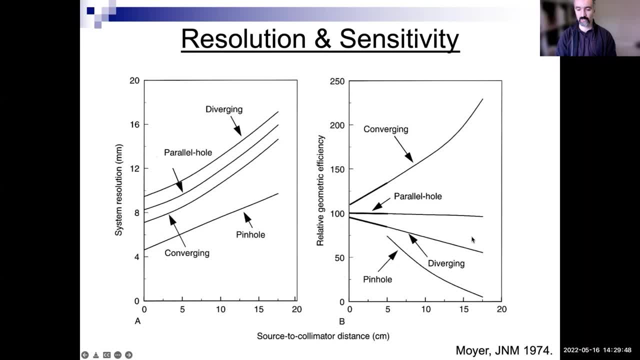 i'm gonna have a do a poor, poorer job. i've been able to, i've been able to, i've been able to to see you, um, to see you, um, to see you, um, yeah, so, yeah, so, yeah. so again, i'm just repeating same things. again, i'm just repeating same things. 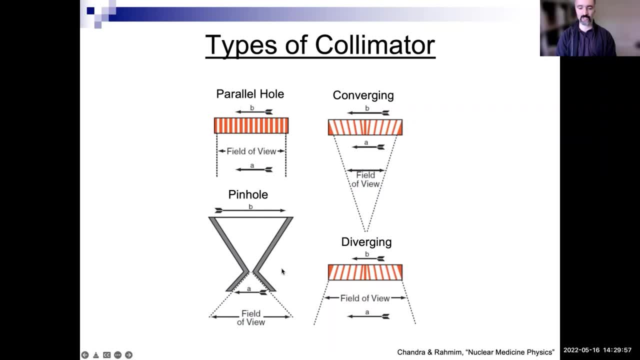 again. i'm just repeating same things: parallel, parallel, parallel, converging, diverging and converging, diverging and converging, diverging and pinholes- okay, you can sort of imagine it. pinholes- okay, you can sort of imagine it. pinholes, okay, you can sort of imagine. it might be hard to see, but you can imagine. 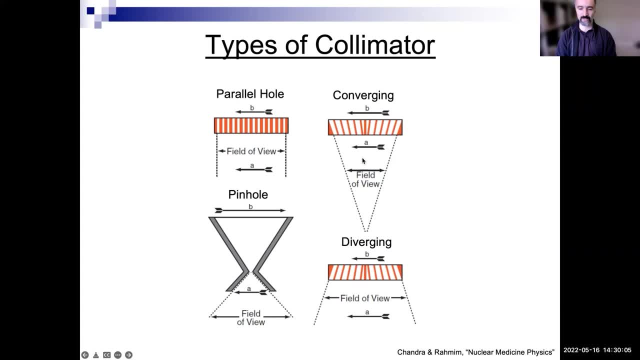 might be hard to see, but you can imagine. might be hard to see, but you can imagine that a point being here is going to be, that a point being here is going to be, that a point being here is going to be detected better than a point here. 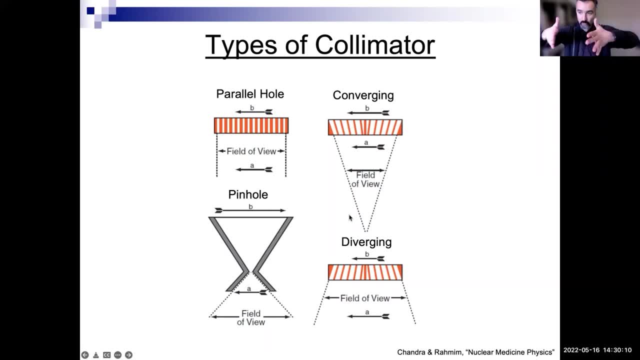 detected better than a point here. detected better than a point here. converging because, if you're here, all of converging. because if you're here, all of converging, because if you're here, all of these can, these can, these can have an eye towards you, whereas if you're have an eye towards you, whereas if you're have an eye towards you, whereas if you're here, some of these don't have an eye here, some of these don't have an eye here, some of these don't have an eye towards. so converging is kind of an. 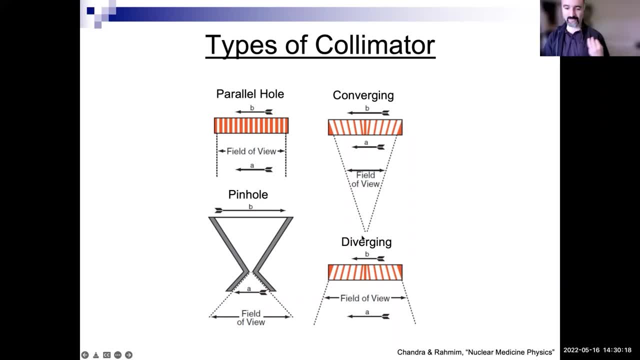 towards, so converging is kind of an towards, so converging is kind of an exception as it gets farther away. exception as it gets farther away. exception: as it gets farther away, your sensitivity increases, your sensitivity increases, your sensitivity increases. but that's an exception for the rest of. but that's an exception for the rest of, but that's an exception for the rest of them. that's not the case. and parallel them. that's not the case. and parallel them. that's not the case. and parallel doesn't matter if you're here or here or. 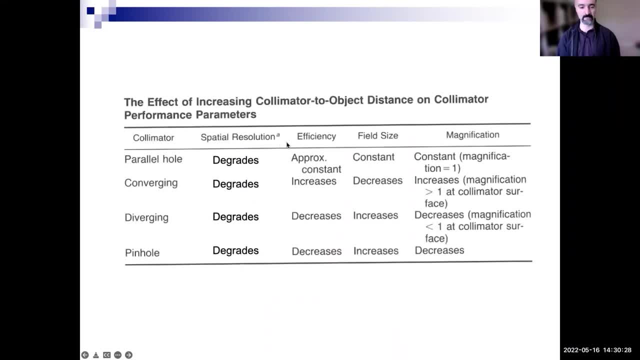 doesn't matter if you're here or here, or doesn't matter if you're here or here or here, i don't care, i'll be able to see here. i don't care, i'll be able to see here. i don't care, i'll be able to see. similarly. 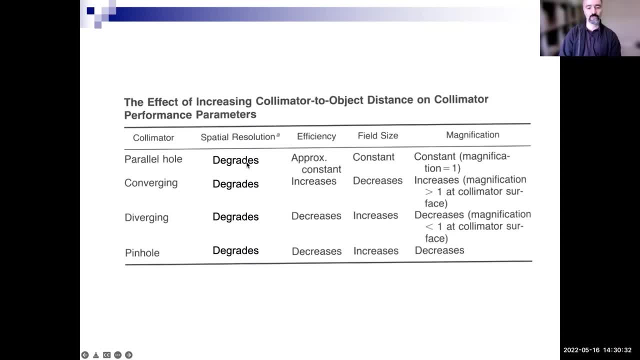 similarly, similarly so spatial resolution of a parallel hole, so spatial resolution of a parallel hole. so spatial resolution of a parallel hole degrades as you get away from it, as you degrades as you get away from it, as you degrades as you get away from it, as you have more distance to the collimator. 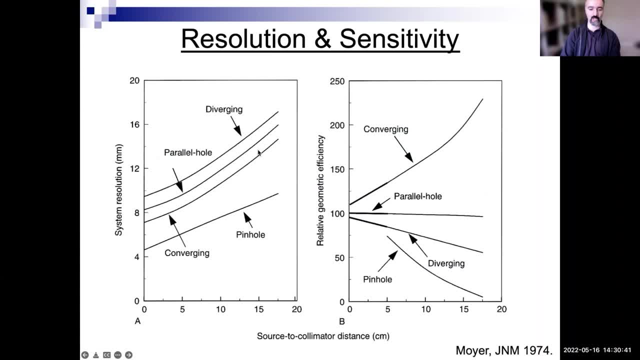 have more distance to the collimator. all of them degrade, as we showed here. all of them degrade, as we showed here. all of them degrade, as we showed here. all of them degrade, but in this case, all of them degrade. but in this case, all of them degrade, but in this case, parallel hole, the sensitivity doesn't. 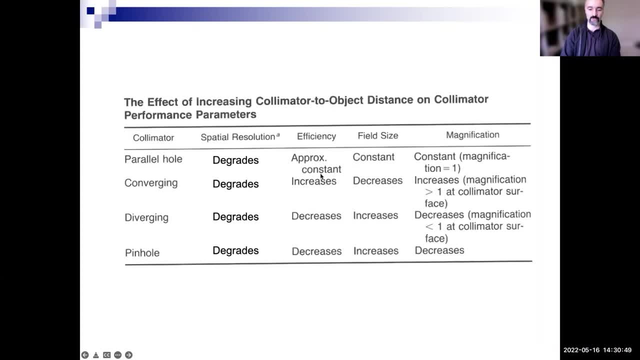 parallel hole. the sensitivity doesn't parallel hole, the sensitivity doesn't change. change change and converging improves, but the divergent pinhole the efficiency, but the divergent pinhole the efficiency. but the divergent pinhole, the efficiency. or the sensitivity decreases or the sensitivity decreases. 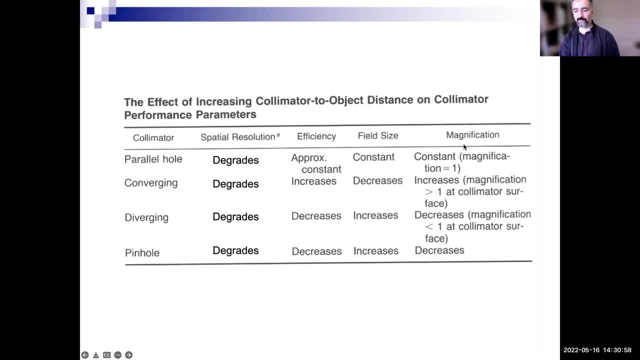 or the sensitivity decreases. and here's the magnifications in a. and here's the magnifications in a. and here's the magnifications in a parallel hole. there is no magnification parallel hole. there is no magnification parallel hole. there is no magnification but in converging and in. 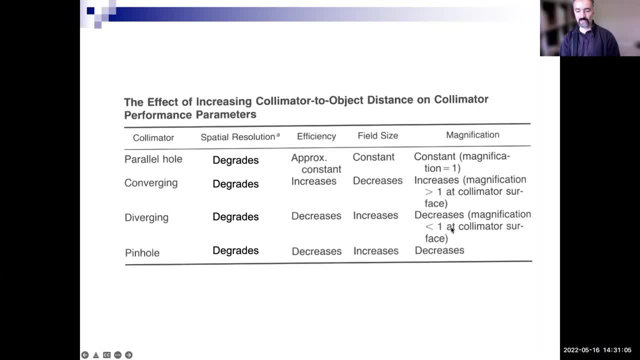 but in converging and in, but in converging and in. uh. in converging, there is a magnification. uh. in converging, there is a magnification. uh. in converging, there is a magnification. in diverging, there is a um. in diverging, there is a um. 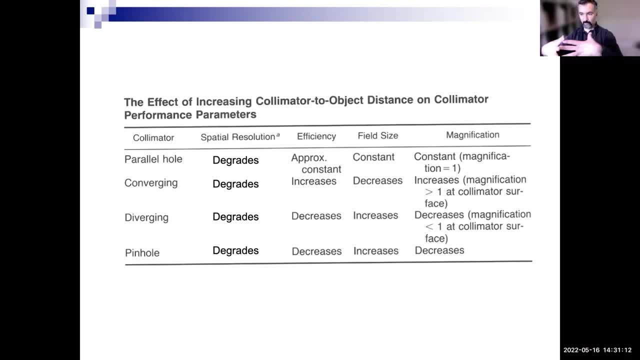 in diverging. there is a um, it's not a mic. uh, it's not a mic. uh, it's not a mic. uh, yeah, yeah, you're kind of suppressing it. yeah, yeah, you're kind of suppressing it. yeah, yeah, you're kind of suppressing it. now, pinhole depends how you think about. 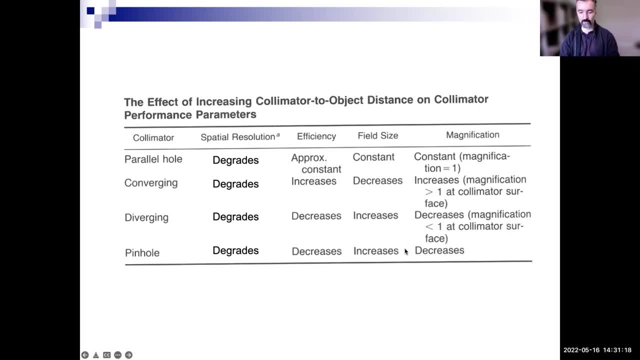 now pinhole depends how you think about now pinhole depends how you think about it. actually it actually. it actually depends where you are. it's a little bit depends where you are. it's a little bit depends where you are. it's a little bit complicated so i won't go through that. 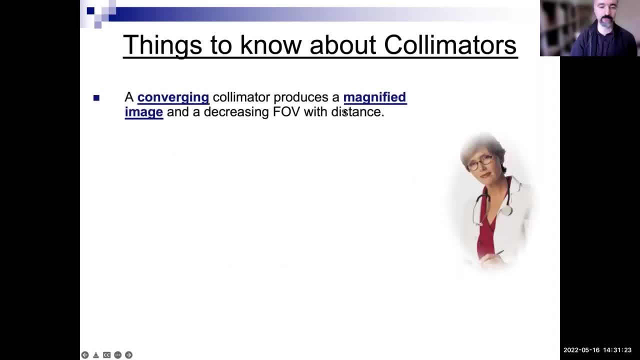 complicated so i won't go through that. complicated so i won't go through that. um, um, um. just summers. a converging columnar, just summers, a converging columnar, just summers. a converging columnar produces a magnified image diverging a. produces a magnified image diverging a. 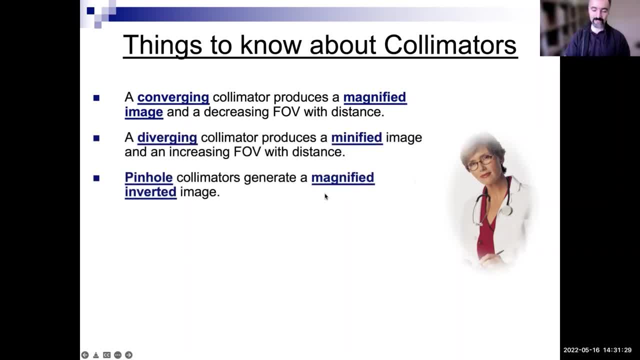 produces a magnified image, diverging, a minified image pinhole. minified image pinhole. minified image pinhole is an inverted image, is an inverted image, is an inverted image, but it's also magnified, but it's also magnified, but it's also magnified. uh, so uh. 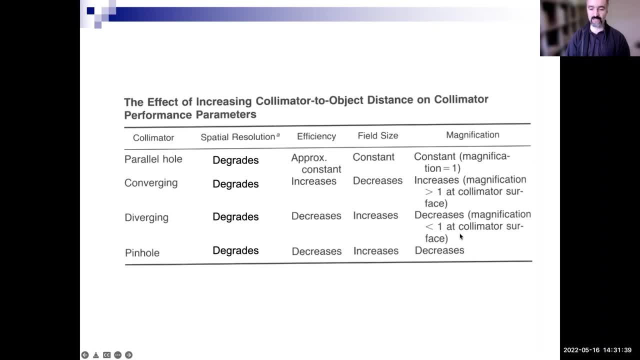 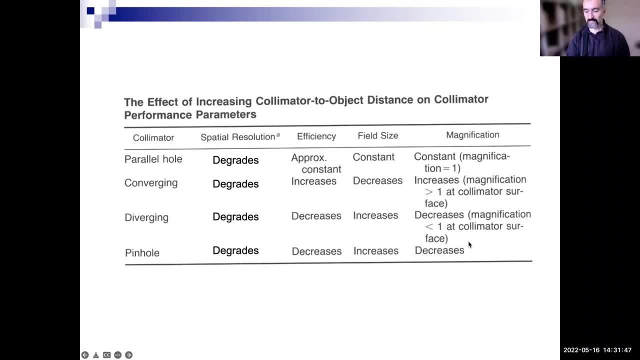 depends where you are. if you are really too far away, it could actually really too far away. it could actually really too far away. it could actually decrease it. but if you're at the right, decrease it. but if you're at the right, decrease it. but if you're at the right position, it could actually increase it. 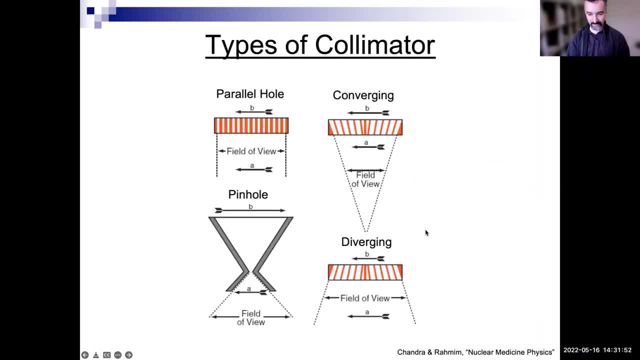 position: it could actually increase it. position, it could actually increase it. so this has to be fixed. so this has to be fixed. so this has to be fixed. uh depends on the context. actually, uh depends on the context. actually, uh depends on the context. actually, now that i have to tell you, i'll tell. 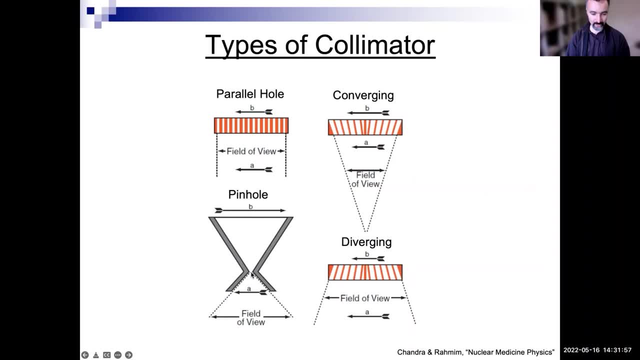 now that i have to tell you, i'll tell, now that i have to tell you, i'll tell you. if you're here, you, if you're here, you, if you're here, around here. you're clearly magnifying around here, you're clearly magnifying around here, you're clearly magnifying signal. 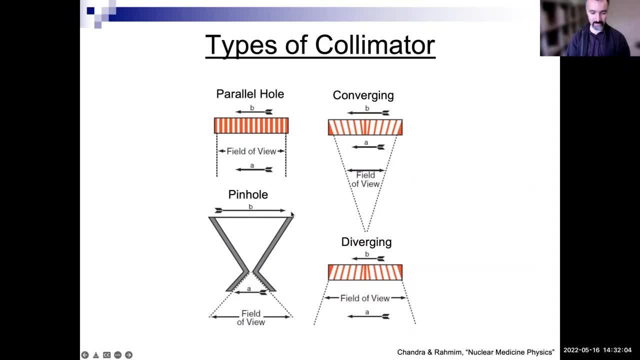 signal, signal, because imagine if you've got something, because imagine if you've got something, because imagine if you've got something that is this big. you're going to see it, that is this big, you're going to see it, that is this big, you're going to see it this big. but if you get too far away, you 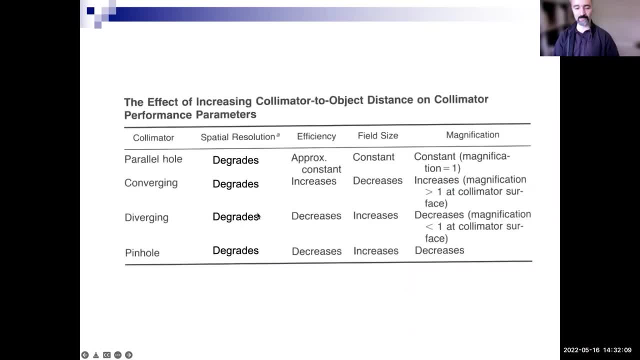 this big, but if you get too far away, you this big. but if you get too far away, you got a huge signal. you're going to get a got a huge signal. you're going to get a got a huge signal. you're going to get a smaller signal. so it actually depends. 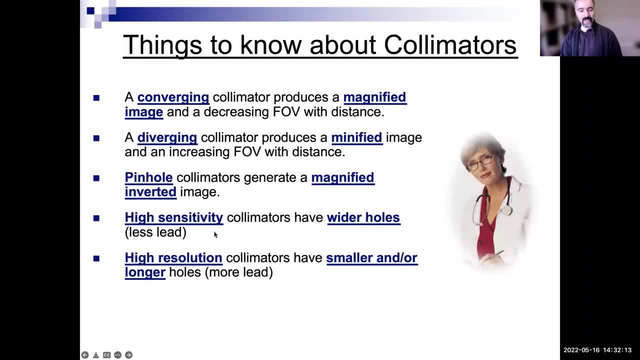 smaller signal, so it actually depends. smaller signal, so it actually depends where you are, where you are, where you are, okay, okay, okay, and high sensitivity columnars have, and high sensitivity columnars have, and high sensitivity columnars have wider holes and high resolution: wider holes and high resolution. 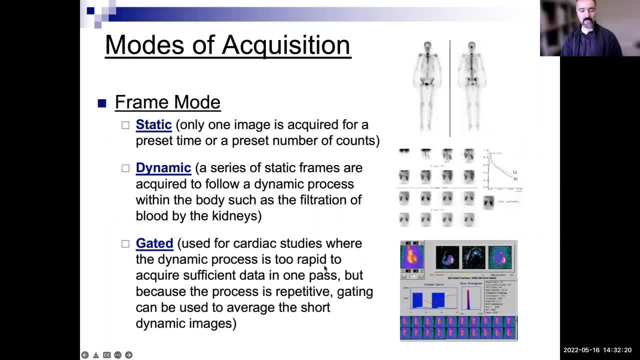 wider holes and high resolution. columns have smaller and or longer holes. columns have smaller and or longer holes. columns have smaller and or longer holes. okay, and finally the modes of acquisition. okay, and finally the modes of acquisition. okay, and finally, the modes of acquisition could be static. i already mentioned that. 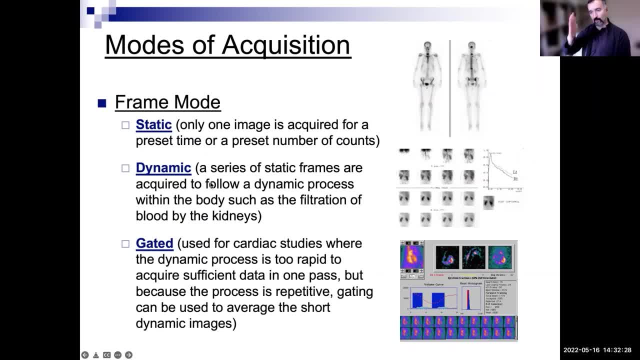 could be static. i already mentioned that could be static. i already mentioned that could be dynamic. so you don't acquire. could be dynamic, so you don't acquire. could be dynamic, so you don't acquire. just once you acquire over time and it. just once you acquire over time and it. 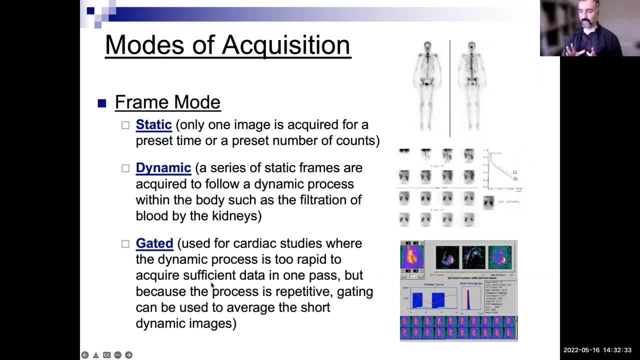 just once you acquire over time. and it could be gated like you look at a beating could be gated. like you look at a beating could be gated like you look at a beating heart and you get. let's say you'd heart and you get, let's say you'd. 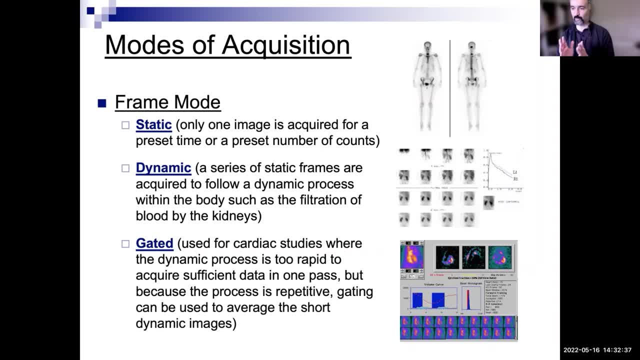 heart and you get, let's say you'd subdivide the beats of the heart into, subdivide the beats of the heart into, subdivide the beats of the heart into eight parts and you keep acquiring from eight parts and you keep acquiring from eight parts and you keep acquiring from different phases of it and you put them. 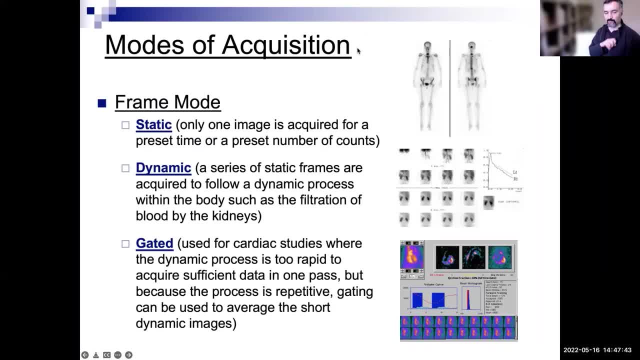 different phases of it and you put them different phases of it, and you put them together together, together, all right. so, as as mentioned before you, all right. so, as as mentioned before you, all right. so, as as mentioned before, you, know, know, know, most commonly we have static imaging. 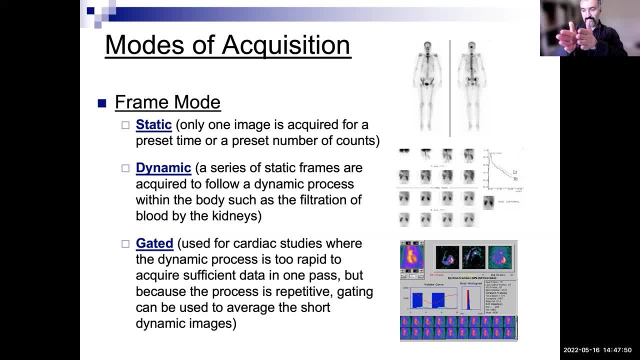 most commonly we have static imaging. most commonly we have static imaging and it's not truly static. i mean you do and it's not truly static. i mean you do and it's not truly static. i mean you do have a, have a, have a acquisition time, but you end up with a. 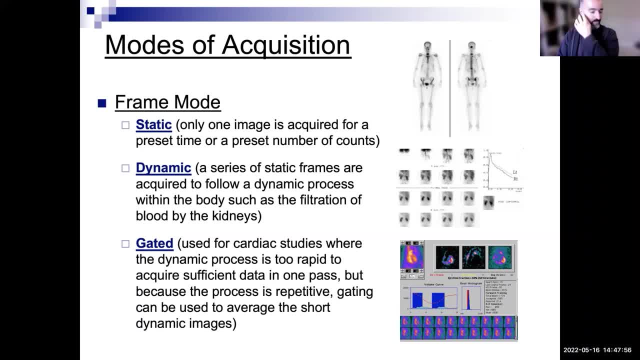 acquisition time, but you end up with a acquisition time, but you end up with a single image, single image, single image which is acquired over. let's say a few which is acquired over. let's say a few which is acquired over, let's say a few minutes, minutes. 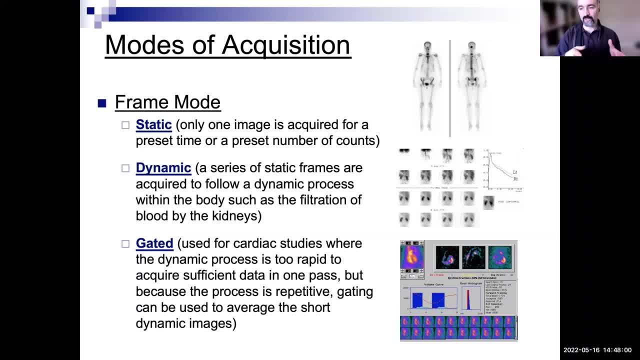 minutes. but if you do multiple snapshots of the but if you do multiple snapshots of the but if you do multiple snapshots of the body, body, body like one frame, another frame, another like one frame, another frame, another like one frame, another frame, another frame, another frame frame, another frame, another frame. so you're going to get multiple. 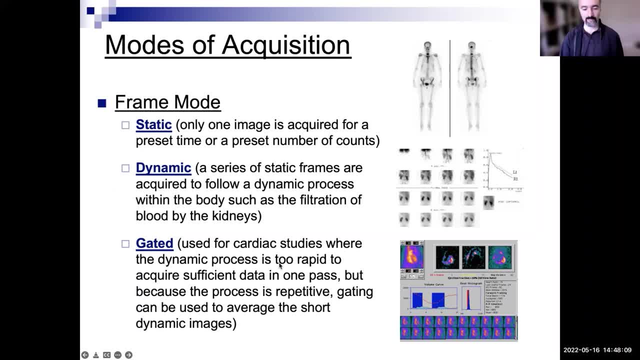 so you're going to get multiple, so you're going to get multiple images, uh. so therefore dynamic images, images, uh. so therefore dynamic images, images. uh. so therefore dynamic images, and finally we have gating, and finally we have gating, and finally we have gating. so so let's talk about that a little bit. 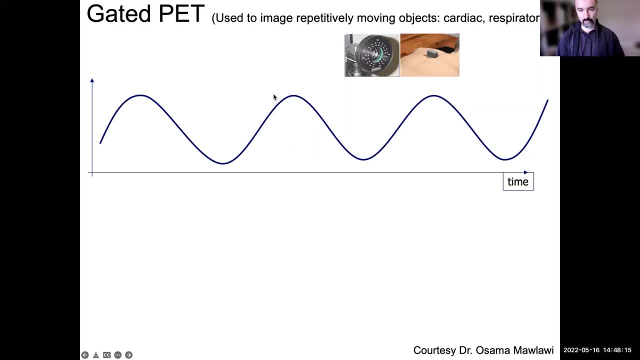 so so, let's talk about that a little bit. so so, let's talk about that a little bit. example of gating. example of gating. example of gating uh, which is used to image uh, which is used to image uh, which is used to image repetitively moving organs. 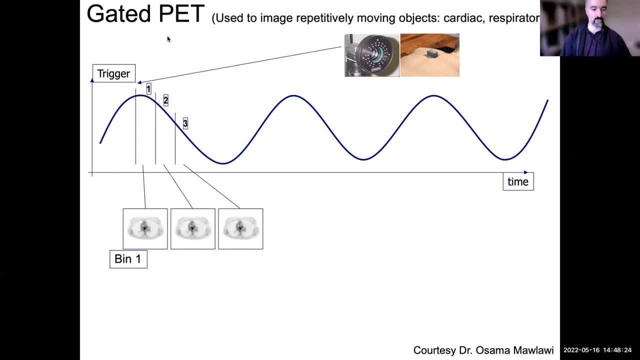 repetitively moving organs. repetitively moving organs, so cardiac and also respiratory. so cardiac and also respiratory, so cardiac and also respiratory movements, movements, movements. so you would be subdividing a cardiac, so you would be subdividing a cardiac, so you would be subdividing a cardiac cycle. 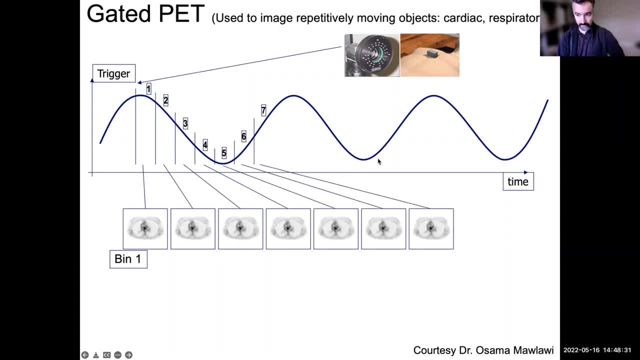 cycle cycle, or a respiratory cycle, or a respiratory cycle, or a respiratory cycle into multiple beams, into multiple beams, into multiple beams. in this case, in this case, in this case, this is respiration. you could put a block: this is respiration. you could put a block: this is respiration. you could put a block over the body, or maybe even do like. 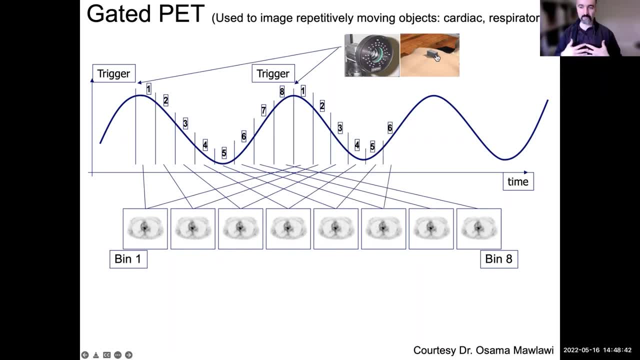 over the body, or maybe even do like over the body, or maybe even do like blockless imaging, where you somehow blockless imaging, where you somehow blockless imaging, where you somehow measure how somebody's measure, how somebody's measure, how somebody's breathing. you know, people have used 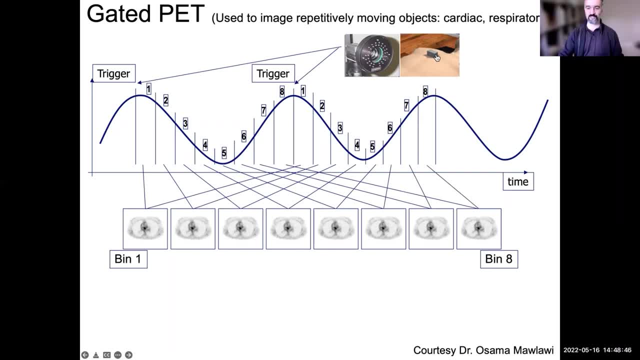 breathing. you know people have used breathing. you know people have used microsoft. connect you know to to microsoft. connect you know to to microsoft. connect you know to to image: how the volume is, for example, image how the volume is, for example. image how the volume is, for example, different innovative waves. but the 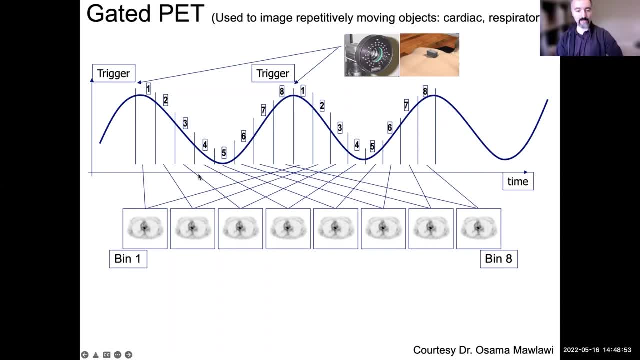 different innovative waves, but the different innovative waves, but the breathing cycle. we can measure breathing cycle. we can measure breathing cycle. we can measure subdivided into- let's say, five frames subdivided into, let's say five frames. subdivided into, let's say, five frames, and you always bring signal from. 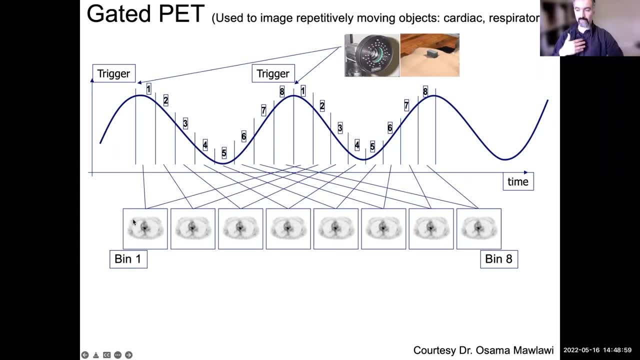 and you always bring signal from, and you always bring signal from that fifth, that fifth, that fifth, that is corresponding to that kind of a, that is corresponding to that kind of a, that is corresponding to that kind of a breathing phase, breathing phase, breathing phase and, um, or it could be eight, right or? 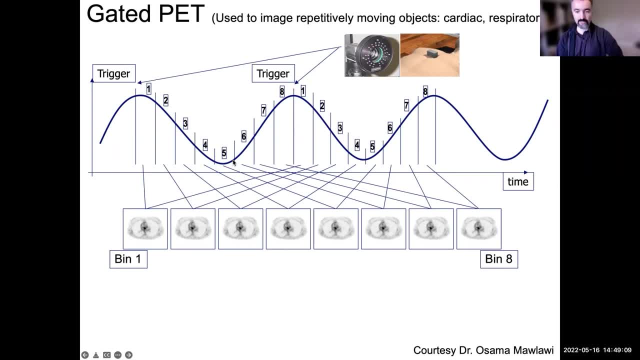 and um, or it could be eight right, or and um, or it could be eight right, or in this case it's actually eight, not in this case it's actually eight, not in this case it's actually eight, not five, five, five. so eight, um, and so you get eight phases. 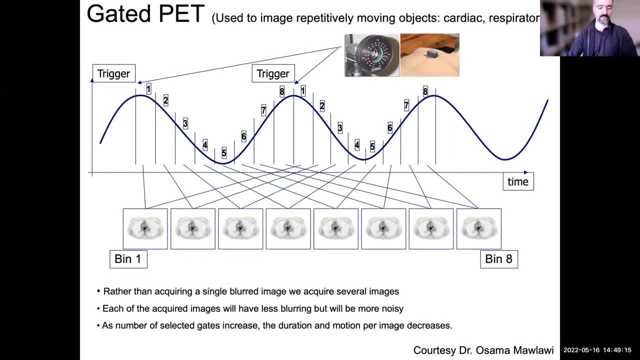 so eight um, and so you get eight phases. so eight um, and so you get eight phases, eight gates, eight respiratory things, eight gates, eight respiratory things, eight gates, eight respiratory things, and that the advantage is, and that the advantage is and that the advantage is okay. what is that? why, why, why should we? 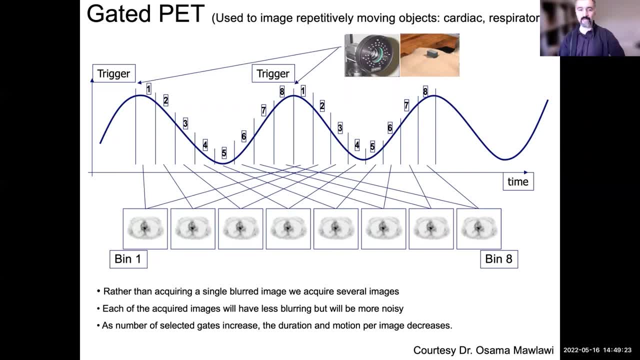 okay. what is that why? why? why should we? okay, what is that why? why, why should we? or why would anybody ever do? or why would anybody ever do? or why would anybody ever do? um gaining, um gaining, um gaining. what's it, what's the advantage? what's it, what's the advantage? 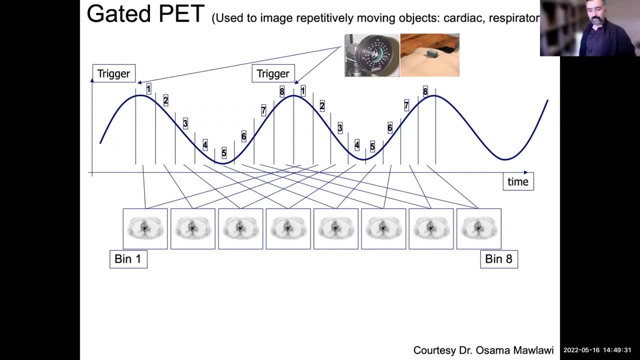 what's it? what's the advantage? any guesses, any guesses, any guesses. instead of just one big breathing cycle, instead of just one big breathing cycle, instead of just one big breathing cycle, just putting all of these together. any guesses- there you avoid the artifact. any guesses: there, you avoid the artifact. 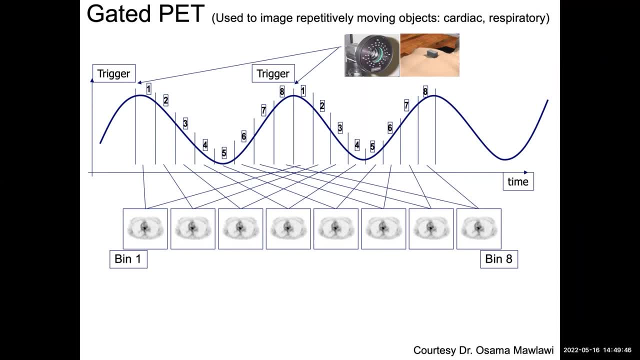 any guesses. there you avoid the artifact of having the organ in a bunch of, of having the organ in a bunch of, of having the organ in a bunch of different, different, different shapes. i guess, yeah, yeah, exactly so shapes. i guess, yeah, yeah, exactly so shapes. i guess, yeah, yeah, exactly so. it's like breathing. 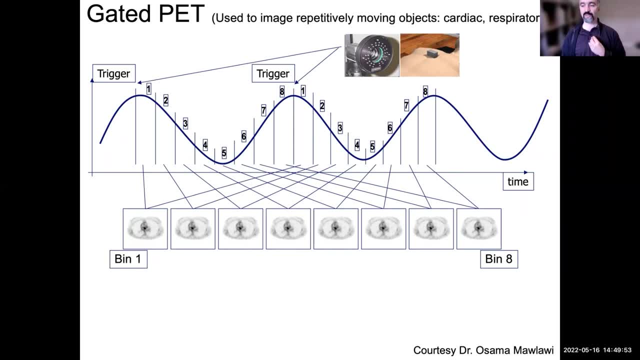 it's like breathing. it's like breathing like. imagine looking at a tumor for like. imagine looking at a tumor for like. imagine looking at a tumor, for example, example, example, as you're breathing, the tumor is as you're breathing. the tumor is as you're breathing, the tumor is moving up and down. so when you image it, 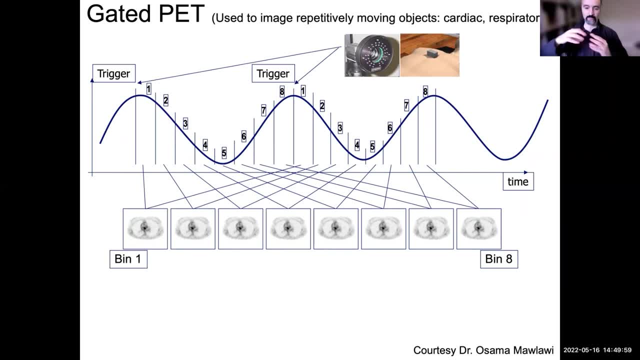 moving up and down. so when you image it moving up and down, so when you image it, if you're not, if you're not, if you're not doing gating, you get a blurred tumor. doing gating, you get a blurred tumor doing gating, you get a blurred tumor. now that you may even miss the tumor. 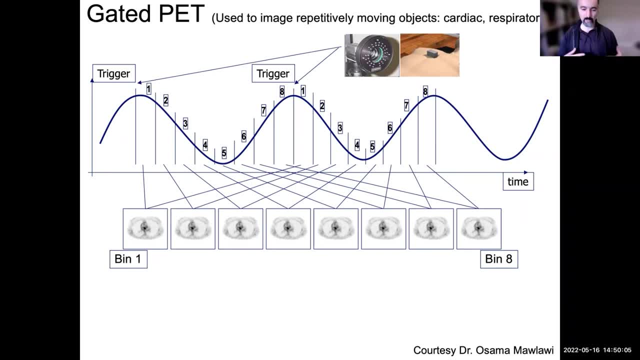 now that you may even miss the tumor. now that you may even miss the tumor, because if it's a really small uptake, because if it's a really small uptake, because if it's a really small uptake thing you may blur up, so that's one thing you may blur up, so that's one. 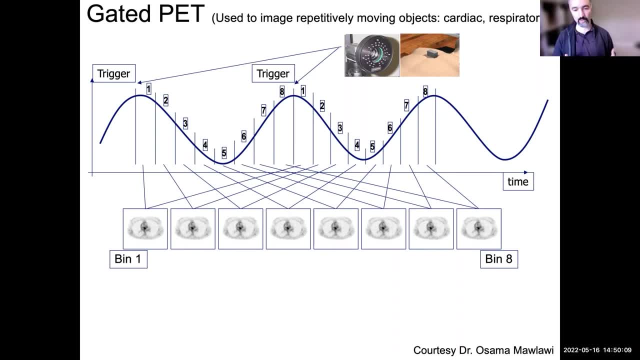 thing you may blur up. so that's one right. so you're trying to do more right. so you're trying to do more right. so you're trying to do more. essentially it's motion correction, or essentially it's motion correction, or essentially it's motion correction, or removing motion degradation. 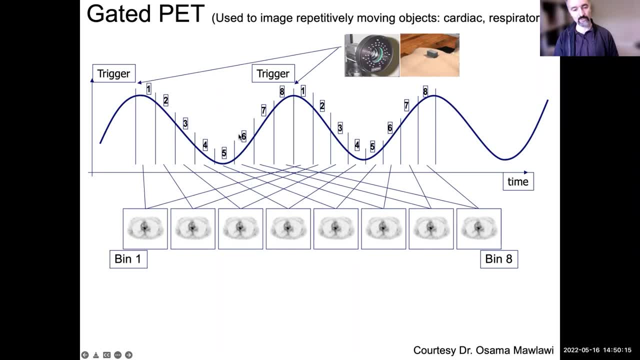 removing motion degradation. removing motion degradation, but the problem is when you're doing. but the problem is when you're doing, but the problem is when you're doing this and subdividing this into eight, this, and subdividing this into eight, this and subdividing this into eight parts, each of these images is going to. 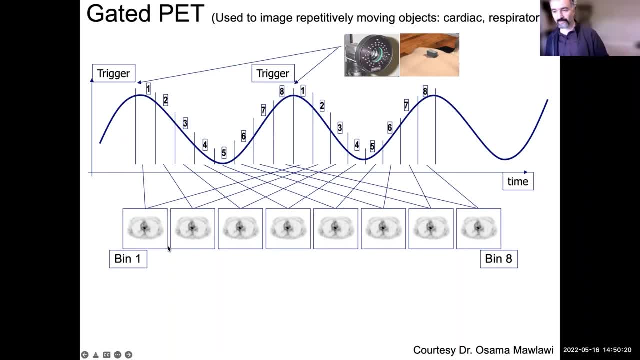 parts. each of these images is going to parts. each of these images is going to have, let's say, one eighth of the signal. have, let's say one eighth of the signal. have, let's say one eighth of the signal. so you're going to get what if you have? 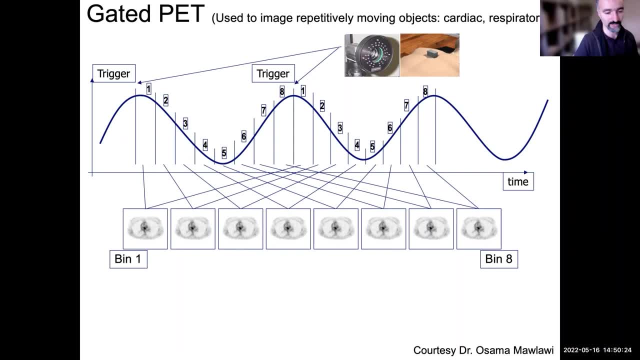 so you're going to get what if you have. so you're going to get what if you have one eighth of the signal. what is what is one eighth of the signal? what is what is one eighth of the signal? what is? what is that going to do to the quality of the? 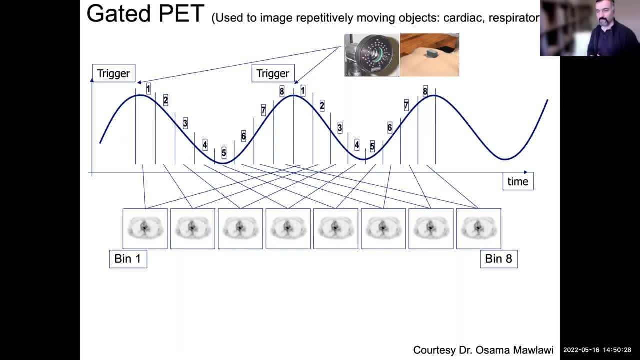 that going to do to the quality of the? that going to do to the quality of the image? what is it going to change? gives you better resolution? less motion gives you better resolution. less motion gives you better resolution, less motion, but what does it? degrade sensitivity. what's that? 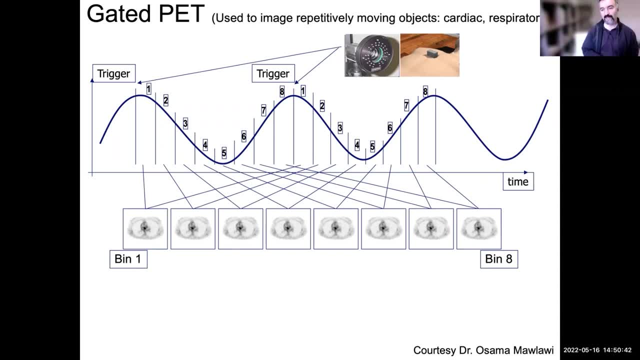 did you say sensitivity? yeah, yeah, so. did you say sensitivity? yeah, yeah, so. did you say sensitivity? yeah, yeah, so, yeah, exactly so you're getting less. yeah, exactly so you're getting less. yeah, exactly so you're getting less. less signal per image which gives you less signal per image which gives you 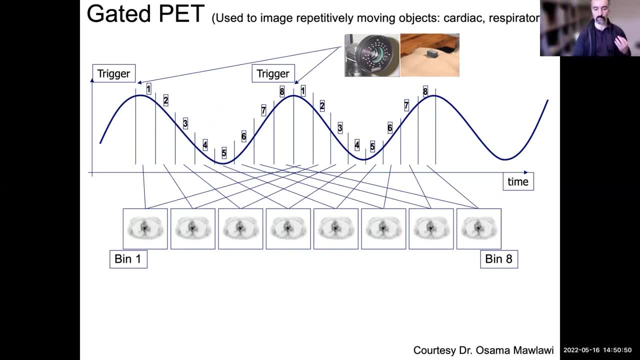 less signal per image, which gives you more noise, less sensitivity or less. more noise, less sensitivity or less. more noise, less sensitivity or less. signal per image. gives you more signal per image. gives you more signal per image. gives you more noise. so the images become noisier and 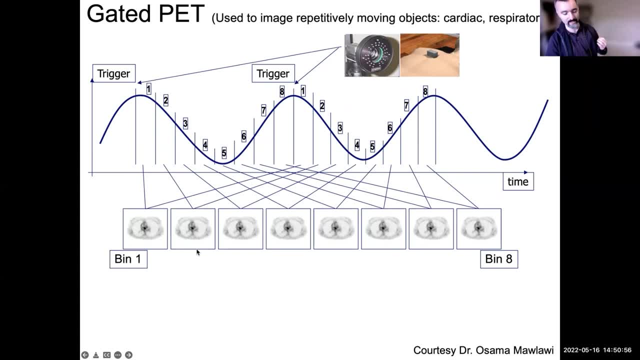 noise so the images become noisier, and noise so the images become noisier. and this is one reason where this is one reason where this is one reason where, right now, in existing right now, in existing right now, in existing uh uh uh practice, let's say in: 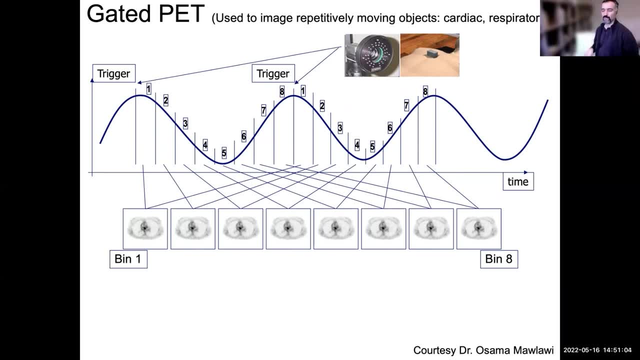 practice. let's say in practice, let's say in pet imaging, pet imaging, pet imaging, this is really not being routinely used. this is really not being routinely used. this is really not being routinely used because at the end of the clinicians, because at the end of the clinicians, 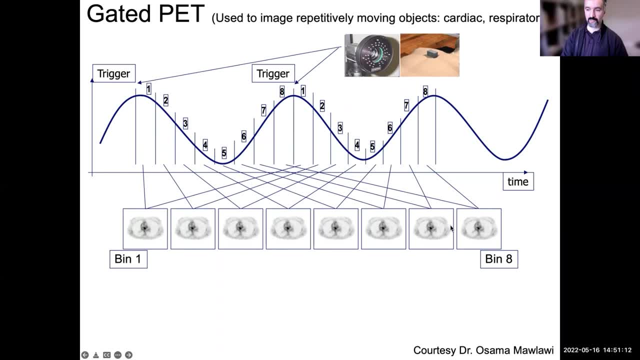 because, at the end of the clinicians didn't like the fact that having like didn't like the fact that having like didn't like the fact that having like, the fact that the images are noisy, the fact that the images are noisy, the fact that the images are noisy. however, if you have a fun, a way and 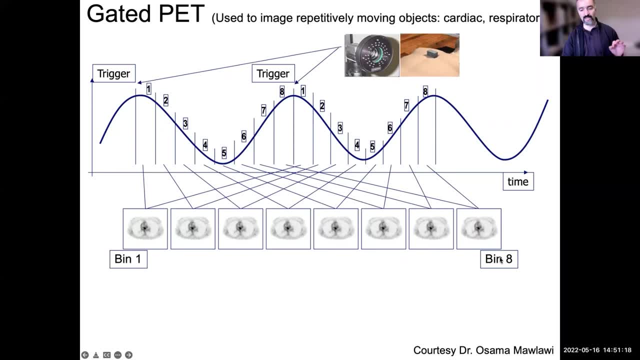 however, if you have a fun a way- and, however, if you have a fun a way and there's active research in this area- there's active research in this area. there's active research in this area- you have a way to get these eight images. you have a way to get these eight images. 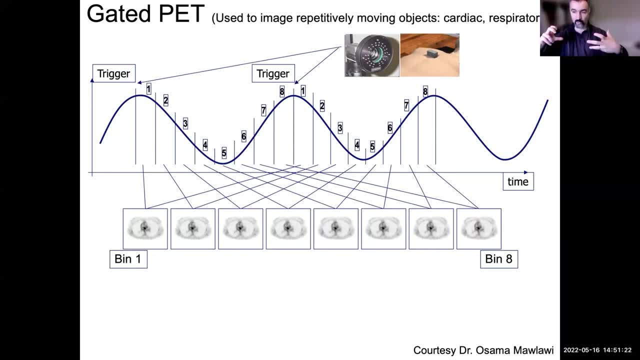 you have a way to get these eight images and register them like non-rigid and register them like non-rigid and register them like non-rigid registration. so you're going to get the registration. so you're going to get the registration. so you're going to get the original quality of signal, because 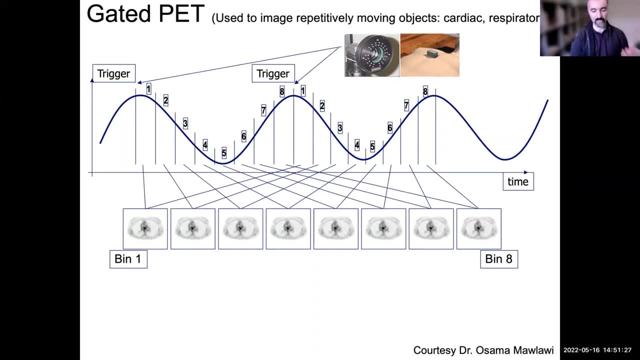 original quality of signal. because original quality of signal? because you're adding them together. but you're adding them together, but you're adding them together but registering and adding and you're registering and adding, and you're registering and adding and you're getting sharper images. so there's active. 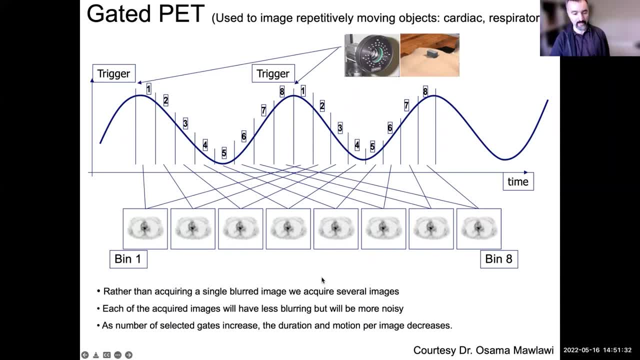 getting sharper images. so there's active getting sharper images. so there's active, very active research in this area, very active research in this area, very active research in this area. um, um, um, yeah, yeah, yeah, so, and as the number of selected, so and as the number of selected. 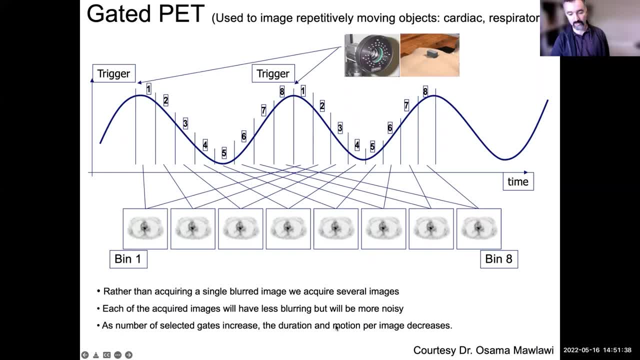 so, and as the number of selected case increases, you get case increases. you get case increases. you get less duration and less motion. so that's less duration and less motion. so that's less duration and less motion. so that's good. but you also get more noise. good, but you also get more noise. 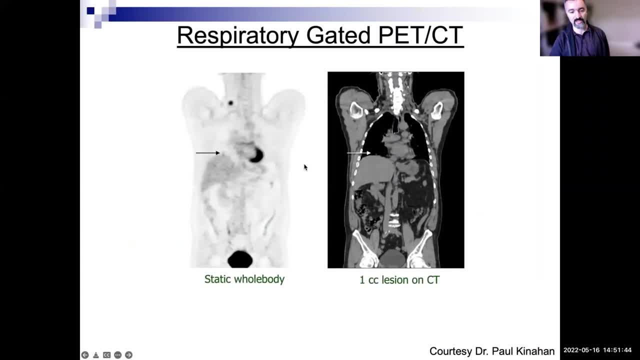 good, but you also get more noise per image. you got to find a way to deal per image. you got to find a way to deal per image. you got to find a way to deal with that. here's an example with that. here's an example with that. here's an example. uh, you've got a one cent one, uh. 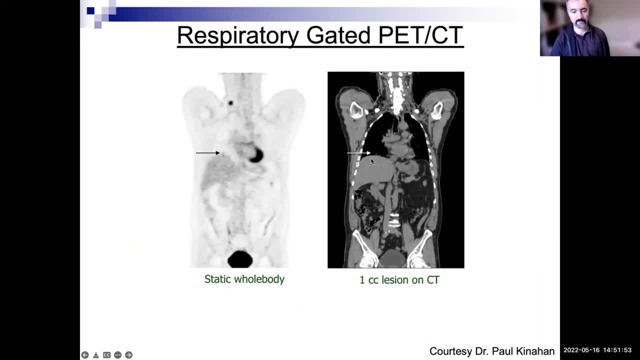 uh, you've got a one cent one. uh, uh, you've got a one cent one. uh, cc, one milliliter, cc, one milliliter, cc, one milliliter. lesion lesion: lesion on ct. this is with respiratory with on ct. this is with respiratory with on ct. this is with respiratory, with respiration happening. it's very hard to. 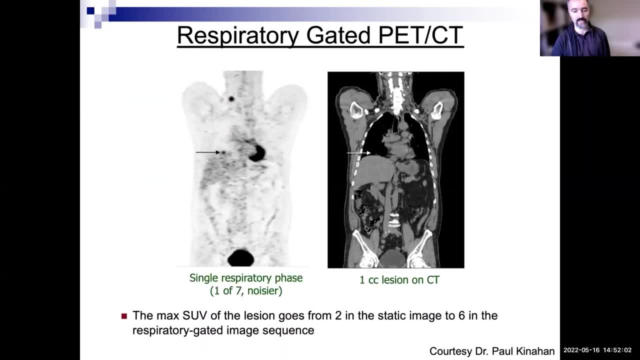 respiration happening. it's very hard to respiration happening. it's very hard to see right. but once you do respiratory, see right. but once you do respiratory, see right. but once you do respiratory, gating, you start seeing it much better. gating, you start seeing it much better. 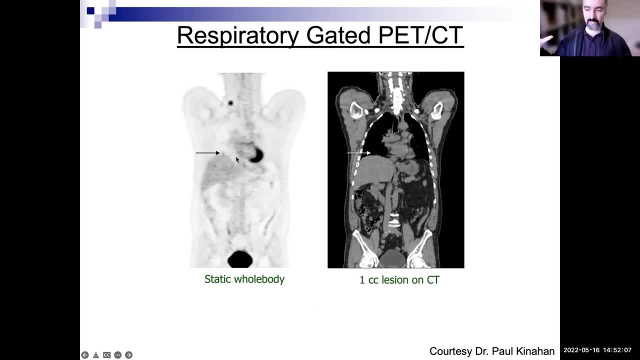 gating, you start seeing it much better. of course they show best examples here. of course they show best examples here. of course they show best examples here. right, this has been blared out, whereas right this has been blared out. whereas right, this has been blared out, whereas here it has not. but notice how the 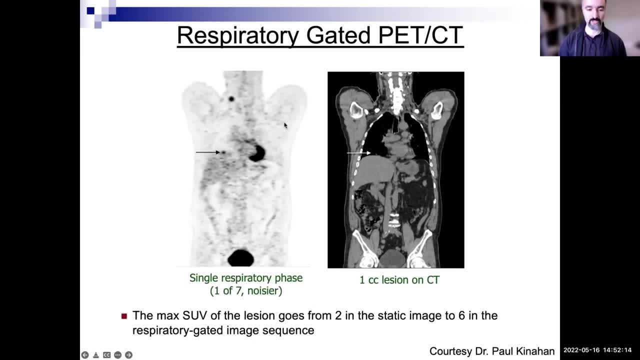 here it has not. but notice how the here it has not. but notice how the image is less noisy here than here. here image is less noisy here than here. here image is less noisy here. here the image is noisier, so you could be. the image is noisier, so you could be. 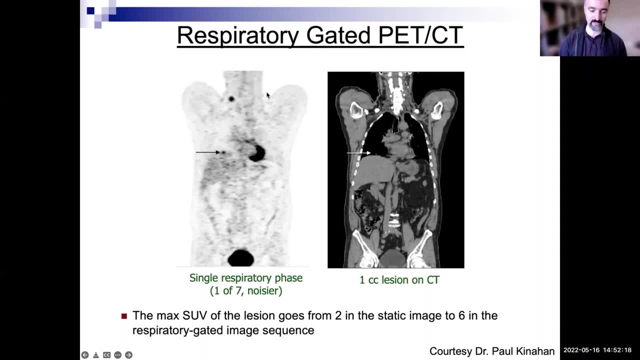 the image is noisier, so you could be thinking of this as a tumor by mistake, thinking of this as a tumor by mistake, thinking of this as a tumor by mistake because you're getting signal that, so because you're getting signal that, so because you're getting signal that, so that makes it, you get. 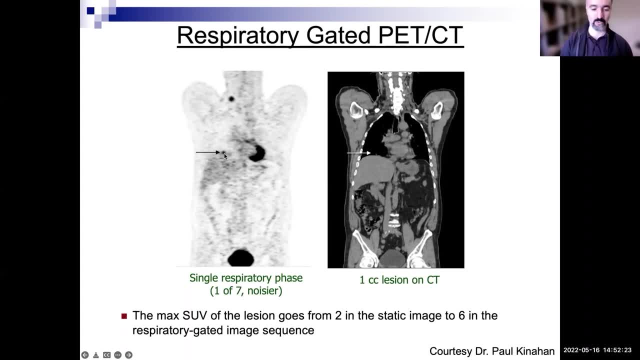 that makes it, you get, that makes it, you get, sure you, you may, you may get more true, sure you, you may. you may get more true, sure you, you may, you may get more true you may detect more stuff you may become. you may detect more stuff you may become. 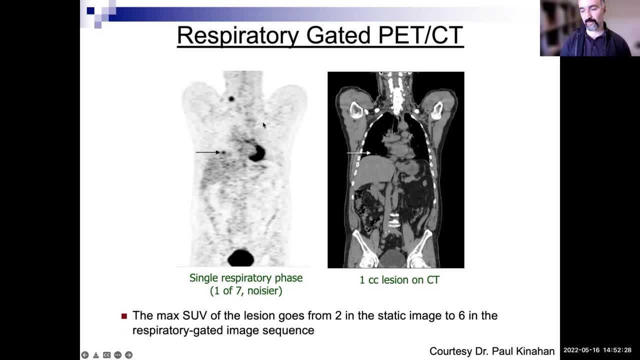 you may detect more stuff. you may become more sensitive, but more sensitive, but more sensitive, but also your specificity may go down, like also your specificity may go down, like also your specificity may go down, like you may start detecting false positives, you may start detecting false positives. so there's a trade-off. 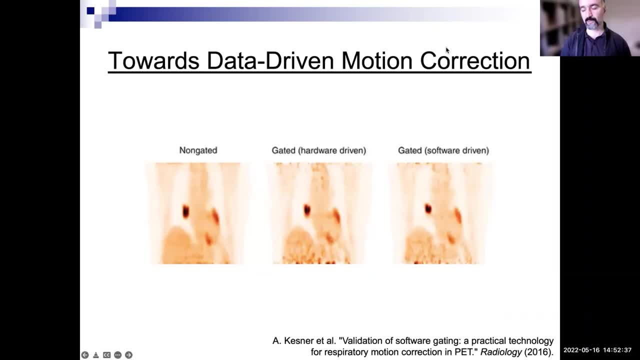 so there's a trade-off. so there's a trade-off, but there's a lot of movement towards, but there's a lot of movement towards, but there's a lot of movement towards data-driven methods. where you don't data-driven methods, where you don't data-driven methods, where you don't, where you use the original signal itself. 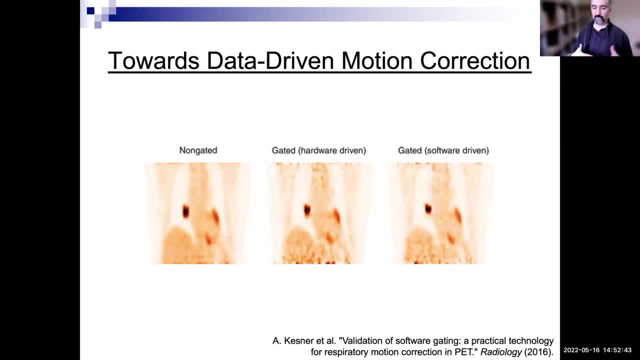 where you use the original signal itself, where you use the original signal itself, used. you don't even use a block on the used. you don't even use a block on the used. you don't even use a block on the chest. you don't use external chest, you don't use external. 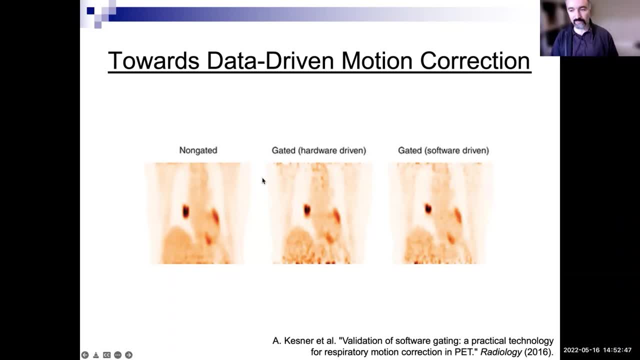 chest. you don't use external tracking devices but use the signal of tracking devices. but use the signal of tracking devices, but use the signal of itself that you're acquiring to get a itself that you're acquiring, to get a itself that you're acquiring, to get a sense about how the body is moving. 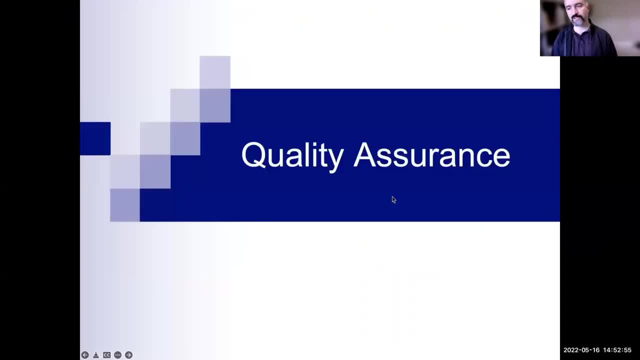 sense about how the body is moving, sense about how the body is moving and somehow doing stuff so it's work in, and somehow doing stuff, so it's work in and somehow doing stuff so it's work in progress, progress, progress, um, it's a very active field of research. 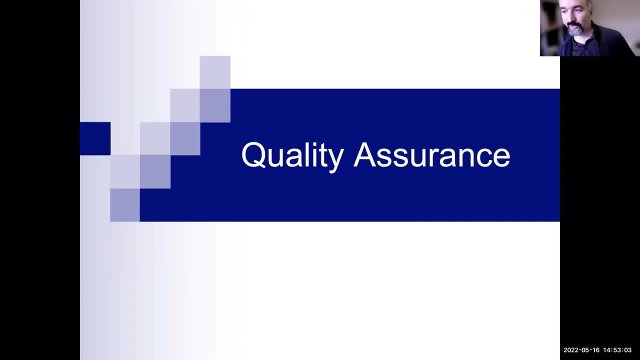 um, it's a very active field of research. um, it's a very active field of research and it has been for a long time. we had, and it has been for a long time. we had, and it has been for a long time. we had hoped this problem would be solved, but i 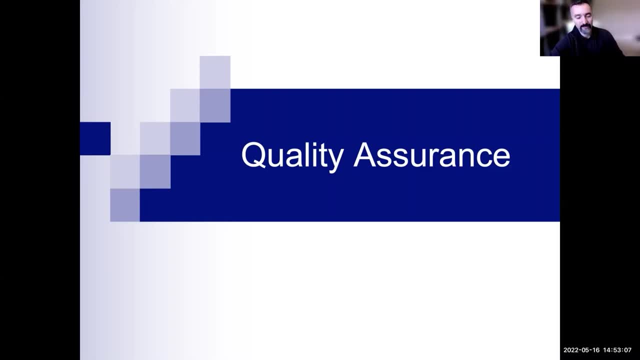 hoped this problem would be solved. but i hoped this problem would be solved. but i think from think, from think, from you know. sometimes you know how you know. sometimes you know how you know. sometimes you know how physicists don't talk to clinicians too. physicists don't talk to clinicians too. 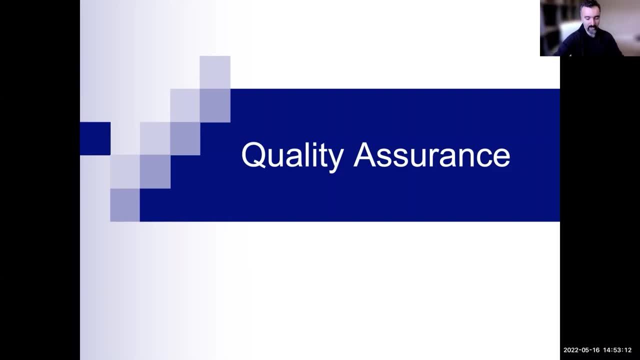 physicists don't talk to clinicians too much and much and much and vice versa. if, if people have been vice versa, if if people have been vice versa, if if people have been really talking and collaborating a lot really talking and collaborating a lot, really talking and collaborating a lot more on different topics, things would 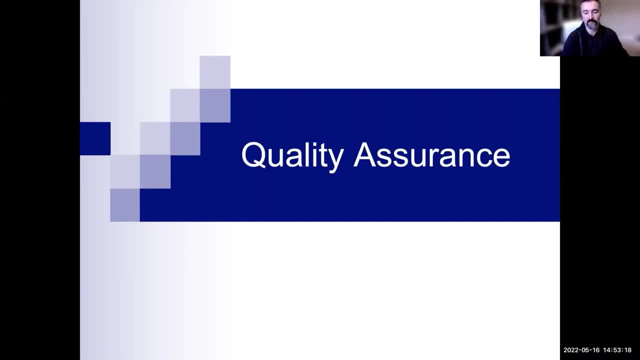 more on different topics. things would more on different topics, things would have come very probably soon, have come very probably soon, have come very probably soon. um. so we need to bridge those gaps um, um. so we need to bridge those gaps um, um. so we need to bridge those gaps um. and this is why i'm very appreciative. and this is why i'm very appreciative and this is why i'm very appreciative that you're you're taking these, that you're you're taking these, that you're you're taking these lectures and you're trying to understand lectures and you're trying to understand. 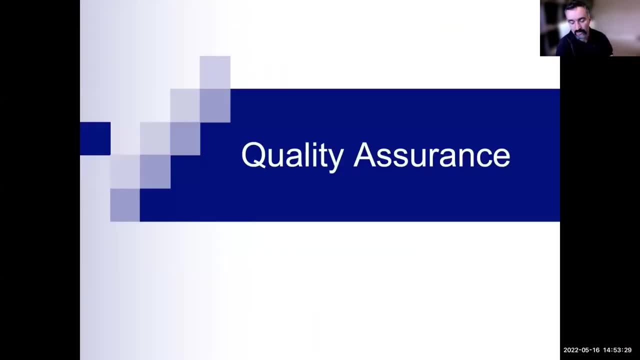 lectures and you're trying to understand the physics more. some of the smartest the physics more. some of the smartest the physics more, some of the smartest people. when i was at, i was people when i was at. i was people when i was at. i was at johns hopkins university. right, uh, the. 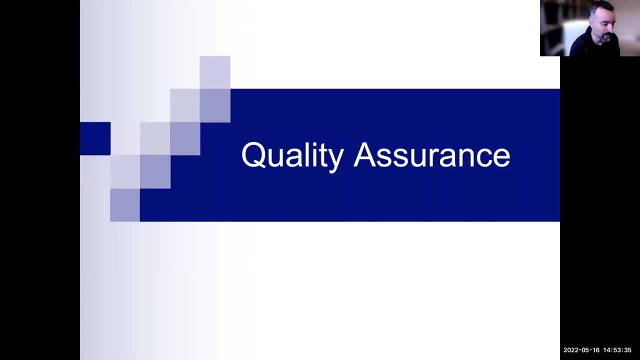 johns hopkins university- right uh, the johns hopkins university, right uh. the radiology department for about 13 years. radiology department for about 13 years. radiology department for about 13 years. some of the smartest people i know. some of the smartest people i know. 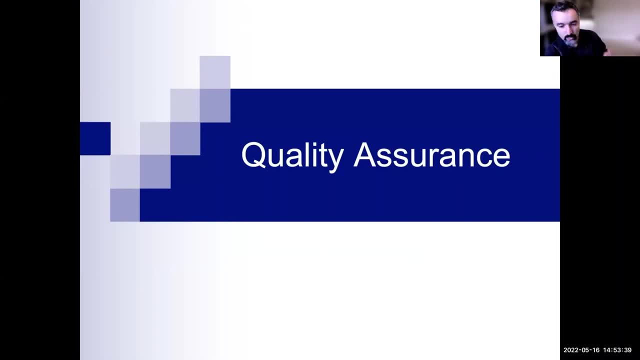 some of the smartest people i know, md scientists and physicians. they md scientists and physicians. they md scientists and physicians. they understood, understood, understood. they understood the physics, they understood the physics. they understood the physics behind what was going on, they would. behind what was going on, they would. 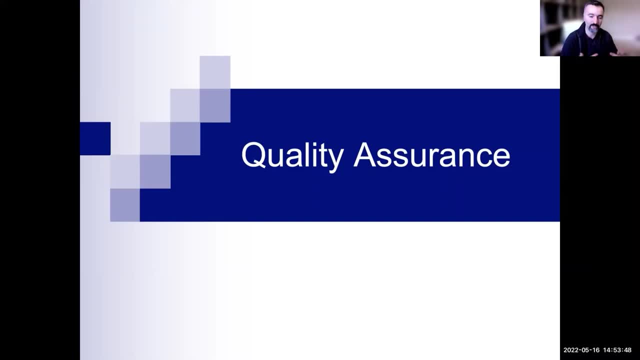 behind what was going on. they would give us brilliant suggestions. we would give us brilliant suggestions. we would give us brilliant suggestions. we would. it shouldn't be both sides of the eye, or it shouldn't be both sides of the eye, or it shouldn't be both sides of the eye, or we should be all together and 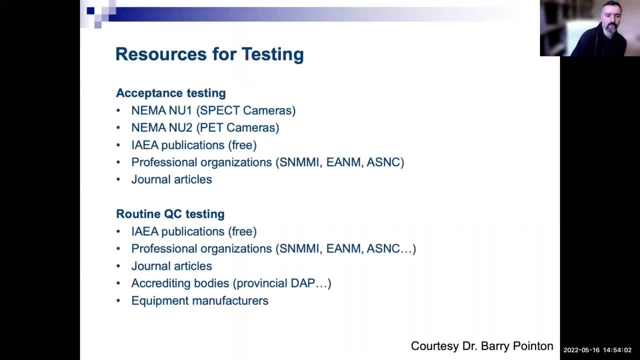 we should be all together and we should be all together and integrated and things happen at least in integrated, and things happen at least in integrated, and things happen at least in some places, some places, some places. so, um, so, um, so um. what are some of the aspects of quality? 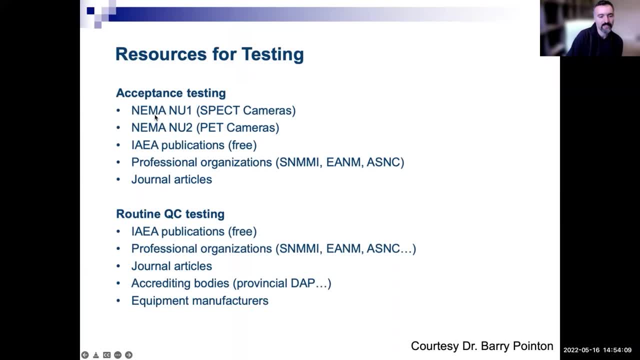 what are some of the aspects of quality? what are some of the aspects of quality assurance or quality check, assurance or quality check, assurance or quality check? there are all kinds of acceptance testing. there are all kinds of acceptance testing. there are all kinds of acceptance testing. how do you accept a scanner that is? 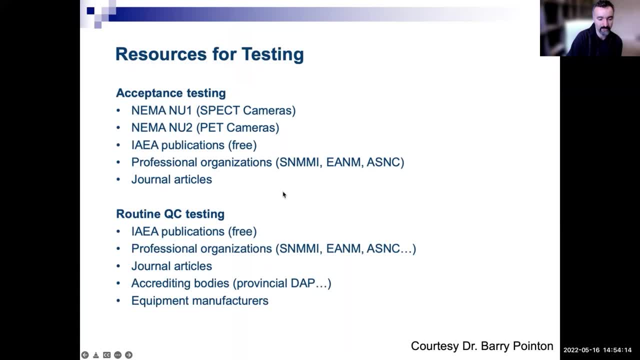 how do you accept a scanner, that is, how do you accept a scanner that is performing well? this is a part of our performing well. this is a part of our performing well. this is a part of our job right as physicists, that we do job right as physicists, that we do. 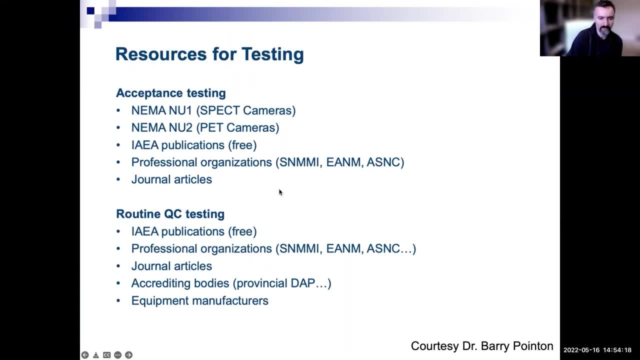 job right as physicists that we do: acceptance testing, acceptance testing. acceptance testing um with different kind of fandoms, with um with different kind of fandoms, with um with different kind of fandoms, with different uh, with different kind of different uh, with different kind of different uh, with different kind of uh. required specifications: 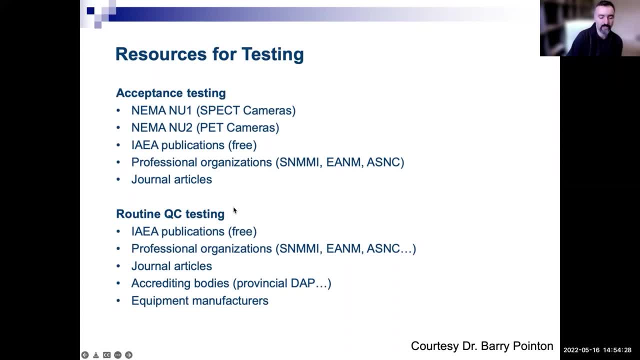 uh required specifications. uh required specifications. and after you accept the scanner, you and after you accept the scanner, you and after you accept the scanner, you also have to make sure it continues to also have to make sure it continues to also have to make sure it continues to work well. so you do routine qa or routine. 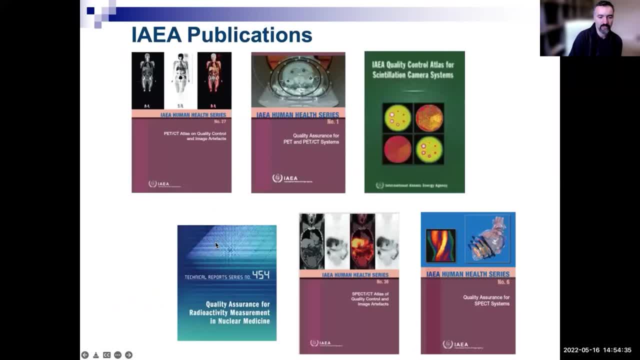 work well, so you do routine qa or routine work well, so you do routine qa or routine qc, qc, qc. and there are different organizations that and there are different organizations that and there are different organizations that talk about this. so a whole bunch of talk about this. so a whole bunch of. 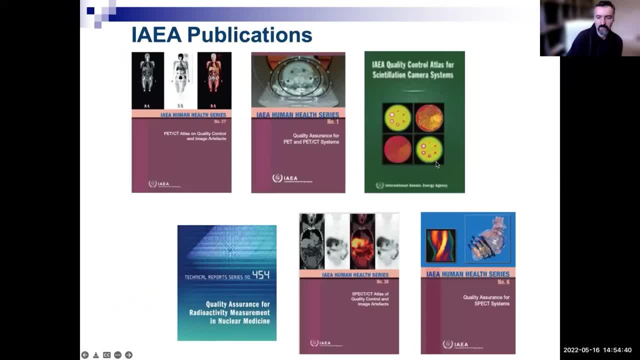 talk about this. so a whole bunch of publications. i won't go through through publications. i won't go through through publications. i won't go through through it, it, it. this one is pretty good. i would say the this one is pretty good. i would say the this one is pretty good. i would say the iaea. 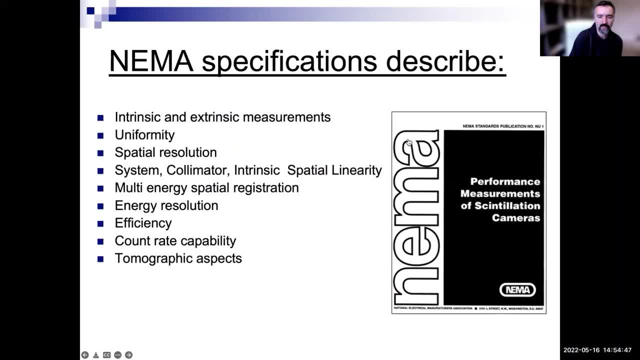 iaea. iaea of the atomic agency is pretty good. uh of the atomic agency is pretty good. uh of the atomic agency is pretty good. uh nima nima. is this organization that nima nima? is this organization that nima nima is this organization that creates very specific specifications. 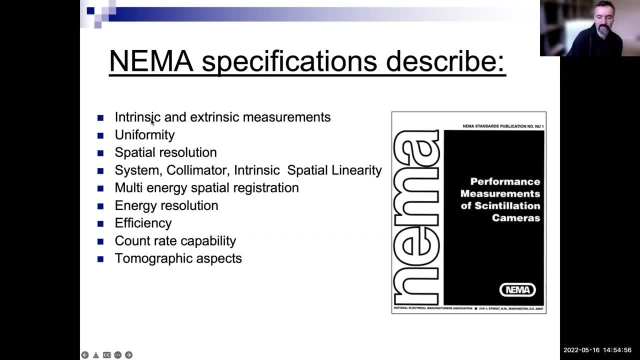 creates very specific specifications. creates very specific specifications: um on, um on, um on. you know what are some of the things that you know. what are some of the things that you know, what are some of the things that are important in acceptance testing, are important in acceptance testing. 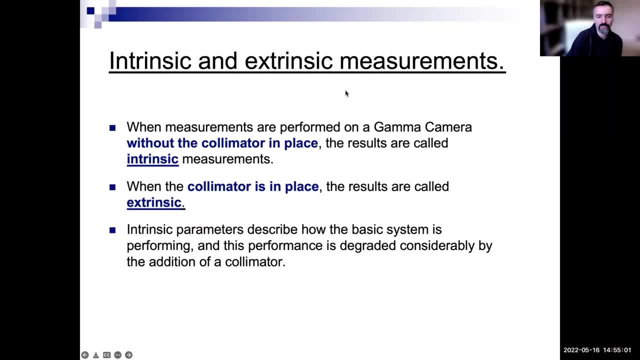 are important in acceptance testing, for example, for example, for example. so we do intrinsic and extrinsic. so we do intrinsic and extrinsic, so we do intrinsic and extrinsic measurements. what does that mean measurements? what does that mean measurements? what does that mean if you do some kind of quality assurance? 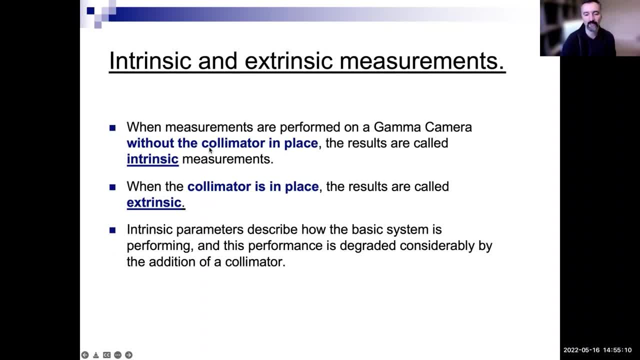 if you do some kind of quality assurance, if you do some kind of quality assurance on a gamma camera without the? on a gamma camera without the? on a gamma camera without the collimator on it, collimator on it, collimator on it. we call that intrinsic measurements. if 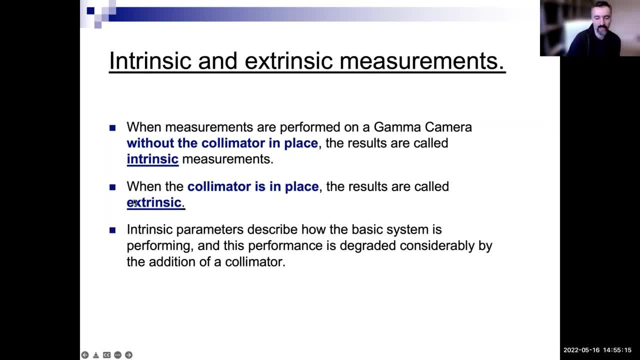 we call that intrinsic measurements. if we call that intrinsic measurements, if it's with the collimator also, it's with the collimator also, it's with the collimator also, it's extreme extrinsic. it's extreme extrinsic, it's extreme extrinsic, and both are important and of course, you. 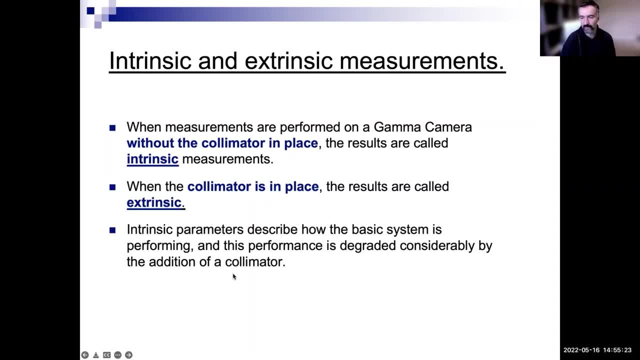 and both are important. and of course you, and both are important. and of course you can imagine the performance is degraded. can imagine the performance is degraded. can imagine the performance is degraded by adding a collimator collimator by adding a collimator collimator, by adding a collimator collimator is there to kill signal. 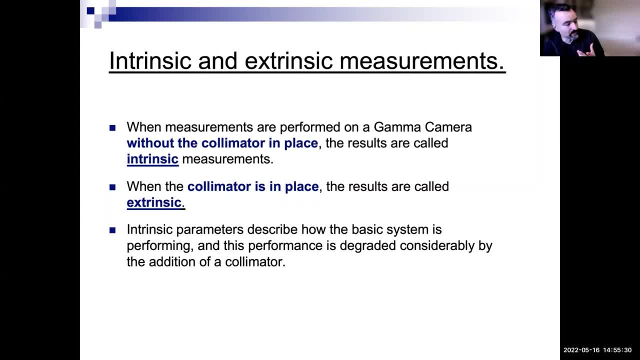 is there to kill signal? is there to kill signal? right, um, right, um, right, um, and does stuff, but we have to use a and does stuff, but we have to use a and does stuff, but we have to use a collimator, collimator, collimator. uh, but anyway, the extrinsic and 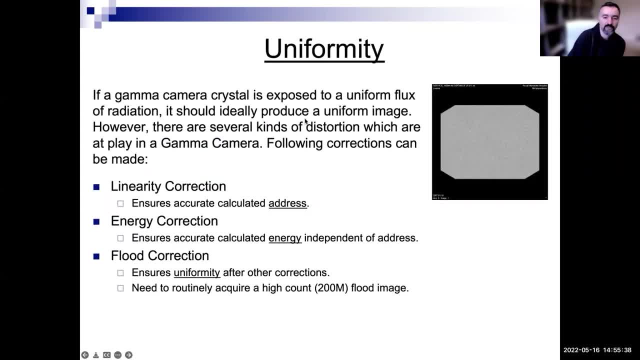 uh, but anyway the extrinsic and, uh, but anyway, the extrinsic and intrinsic performances are different. intrinsic performances are different, intrinsic performances are different. so uniformity you obviously want, so uniformity you obviously want. so uniformity, you obviously want something that is uniform otherwise, something that is uniform otherwise. 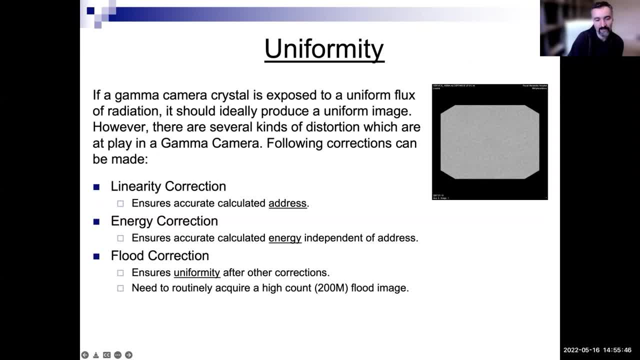 something that is uniform. otherwise you may see stuff that don't really. you may see stuff that don't really. you may see stuff that don't really exist in in in reality. so so what are exist in in in reality? so so, what are exist in in in reality? so so, what are some of those? 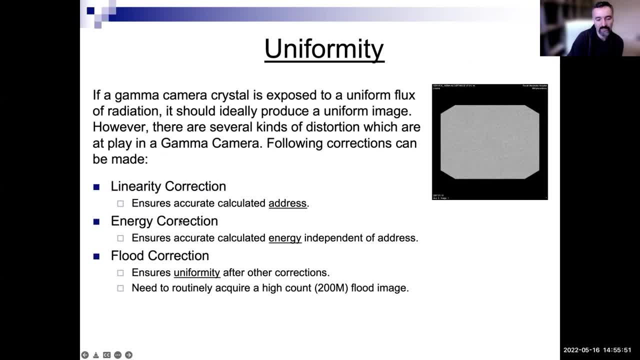 some of those, some of those uniformities, linearity, we'll talk about uniformities. linearity: we'll talk about uniformities. linearity, we'll talk about this, this, this, energy and flood. so so, energy and flood. so so, energy and flood. so so, if a gamma camera is opposed to uniform, 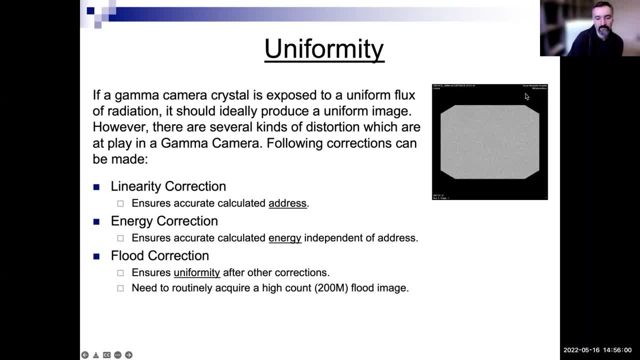 if a gamma camera is opposed to uniform. if a gamma camera is opposed to uniform flux of radiation, it really should look flux of radiation. it really should look flux of radiation. it really should look uniform, uniform. but there are some distortions and once. but there are some distortions and once. 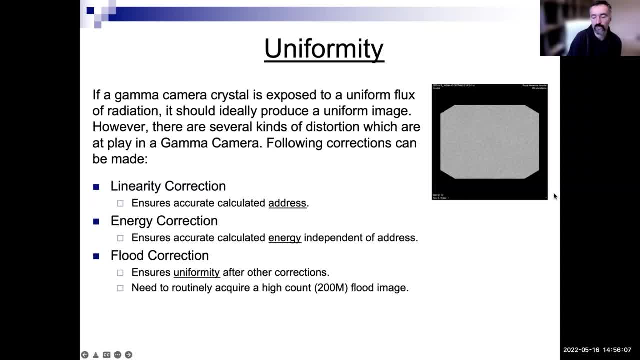 but there are some distortions and once you correct for those distortions, using you correct for those distortions, using you correct for those distortions, using these three corrections, hopefully you're these three corrections, hopefully you're these three corrections, hopefully you're going to get a nice. 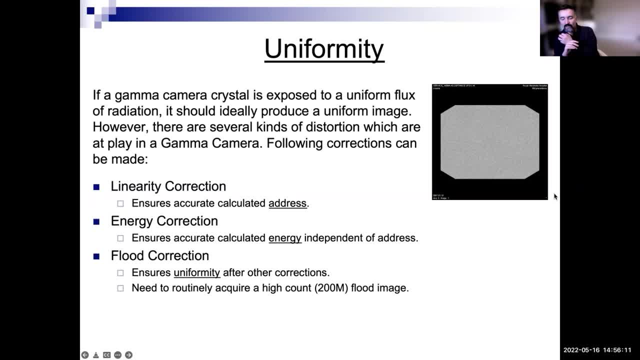 going to get a nice, going to get a nice uniform flood image if you don't get a uniform flood image, if you don't get a uniform flood image, if you don't get a daily uniform flood image. something is daily uniform flood image. something is daily uniform flood image. something is wrong. 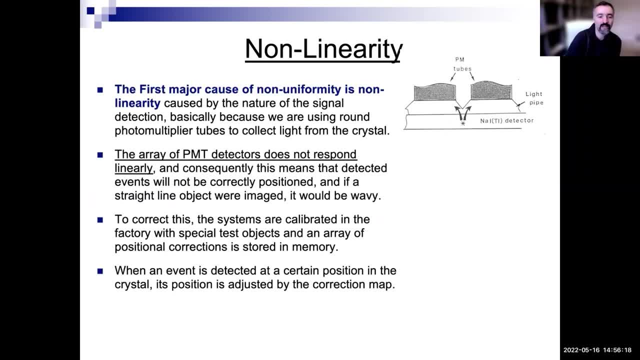 wrong, wrong, you have to fix it. so non-linearity is a you have to fix it. so non-linearity is a you have to fix it. so non-linearity is a first major cause of non-uniformity, first major cause of non-uniformity. 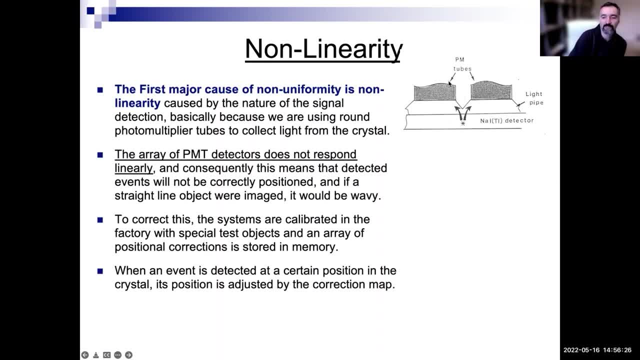 first major cause of non-uniformity: um, and the point is that a pmt, i've um, and the point is that a pmt i've um. and the point is that a pmt- i've mentioned pmt's a couple times, mentioned pmt's a couple times. 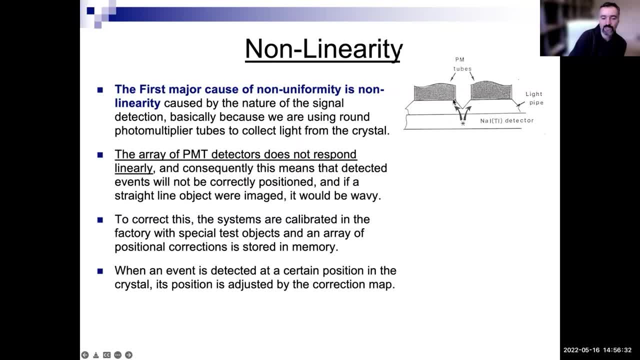 mentioned pmt's a couple times. the edge of a tmt responds to signal. the edge of a tmt responds to signal. the edge of a tmt responds to signal differently than the center of a pmt. differently than the center of a pmt, differently than the center of a pmt. just an observation. so if you're here, 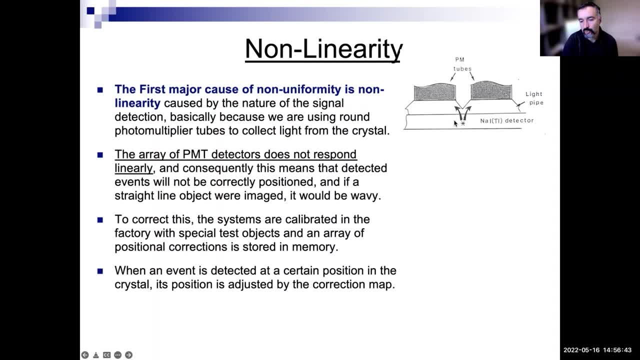 just an observation. so if you're here, just an observation. so if you're here, you're going to be the sensitivity to a you're going to be the sensitivity to a you're going to be. the sensitivity to a point here is going to be different than 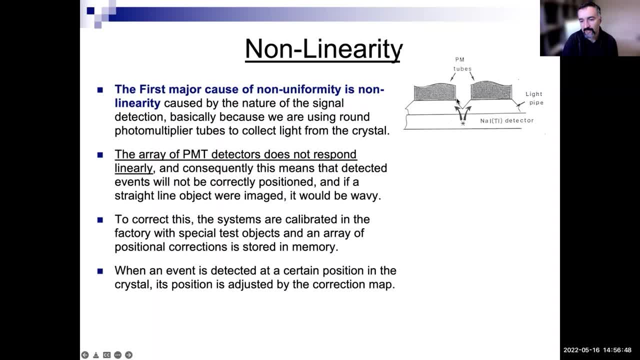 point here is going to be different than point here, is going to be different than a sensitivity to a point here. a sensitivity to a point here, a sensitivity to a point here, okay and so, okay and so, okay and so, and remember the position the angular, and remember the position the angular. 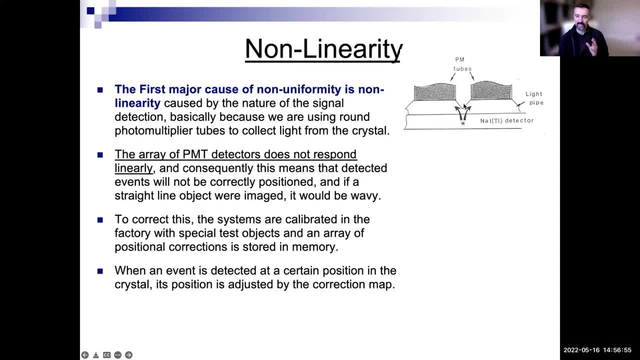 and remember the position the angular logic was based on how much signal you logic was based on how much signal you logic was based on how much signal you get in different places, get in different places, get in different places. if you're not taking that point into, if you're not taking that point into, 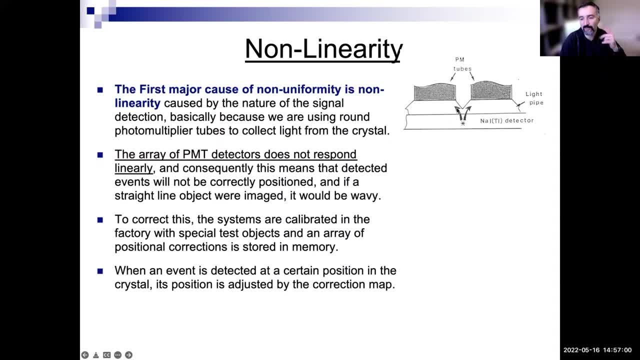 if you're not taking that point into account, you might be thinking: oh, i got account. you might be thinking: oh, i got account. you might be thinking: oh, i got less signal here. therefore, less stuff is less signal here. therefore, less stuff is less signal here. therefore, less stuff is here. but no, that's simply because the 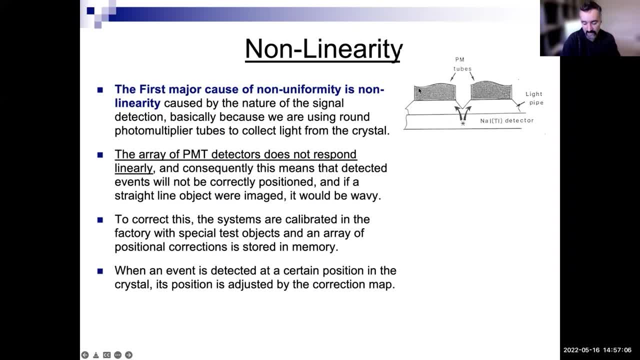 here. but no, that's simply because the here, but no, that's simply because the edge of a pmt detects stuff less than the edge of a pmt. detects stuff less than the edge of a pmt. detects stuff less than the center of the pmt. 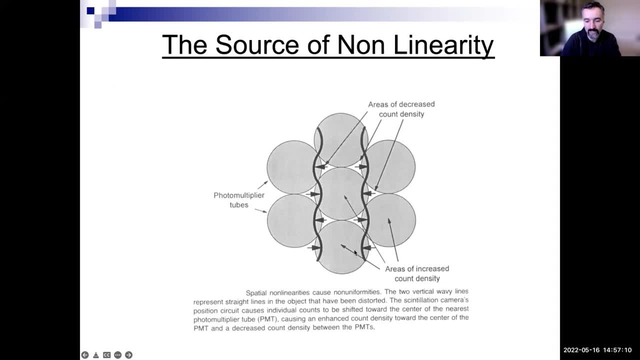 center of the pmt, center of the pmt. so if you don't correct for that, you're so. if you don't correct for that, you're so. if you don't correct for that, you're gonna get these strange and weird. gonna get these strange and weird. 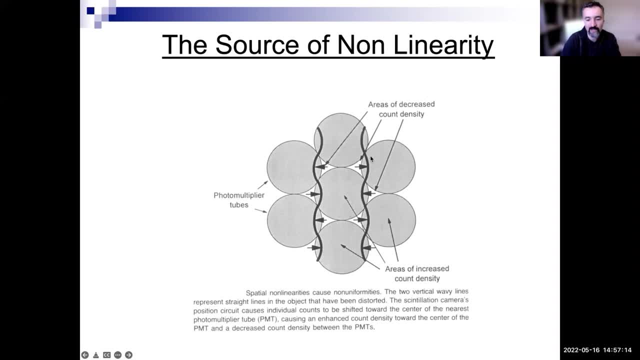 gonna get these strange and weird shapes, okay, shapes okay, shapes okay, but that's, we already know this. and so if, but that's, we already know this. and so if, but that's, we already know this. and so, if you just make like, if you just um, you just make like, if you just um, 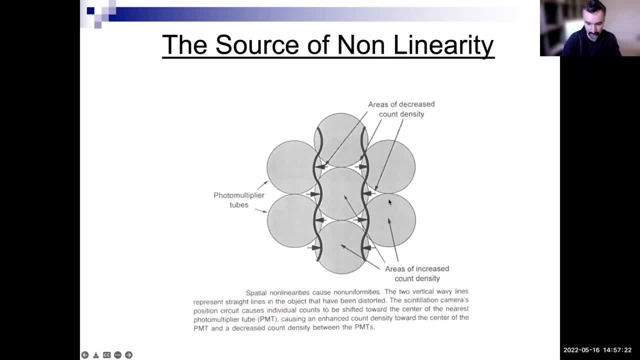 you just make like, if you just um, if you just image like line sources and if you just image like line sources and if you just image like line sources and you get this, you can correct for them, you get this, you can correct for them, you get this, you can correct for them. and you basically say: hey, if i detect. 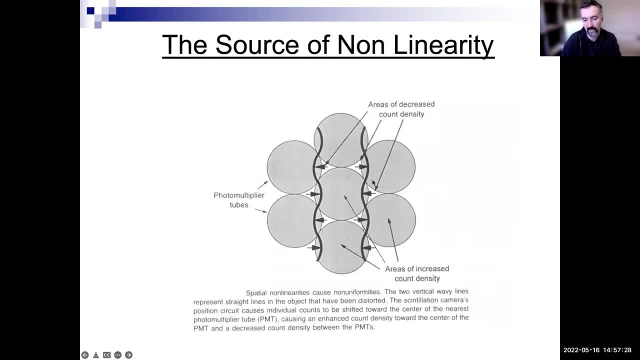 and you basically say, hey, if i detect. and you basically say, hey, if i detect something at this position, i'm going to something at this position. i'm going to something at this position. i'm going to add an extra x, add an extra x, add an extra x, i'm gonna. if i see something here, i'm. i'm gonna. if i see something here, i'm i'm gonna. if i see something here, i'm gonna move it by this much, if i gonna move it by this much, if i gonna move it by this much, if i something here, i'm gonna move it, it's. 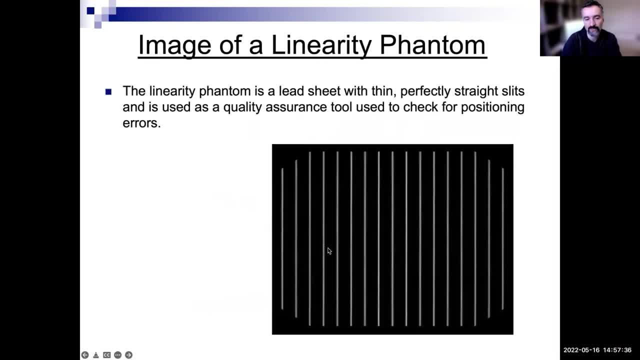 something here, i'm gonna move it. it's something here, i'm gonna move it. it's almost like a lookup table. almost like a lookup table. almost like a lookup table. it's very easy to do so. you have linearity. it's very easy to do so. you have linearity. 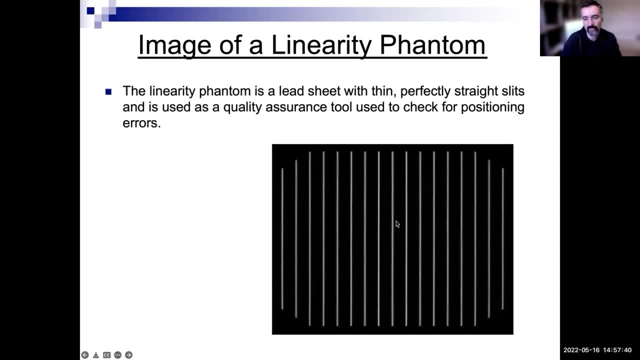 it's very easy to do so. you have linearity phantom. these are like phantom. these are like phantom. these are like lead shields with thin lead shields, with thin lead shields with thin slits. um so they're gonna give you slits. um so they're gonna give you. 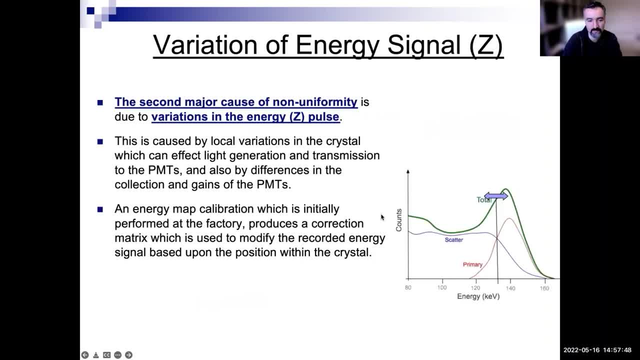 slits, um. so they're gonna give you these weird non-linearities, but then these weird non-linearities, but then these weird non-linearities, but then you look it up and you fix it. you look it up and you fix it. you look it up and you fix it. the second one is variations in the 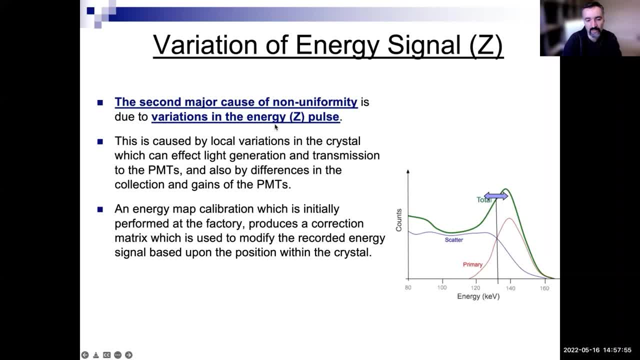 the second one is variations in the. the second one is variations in the energy, energy, energy. okay, so, okay, so, okay. so this is also caused by variations in. this is also caused by variations in the. this is also caused by variations in the in the crystal, in the crystal. 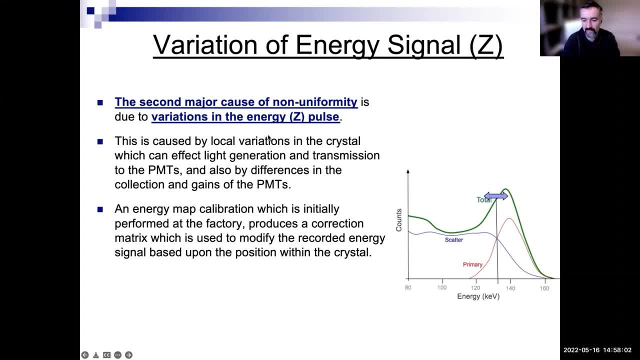 in the crystal, um, um, um. so so the crystal itself, so so the crystal itself, so so the crystal itself, uh, if, if, if, you, uh, if, if, if, you, uh, if, if, if you image stuff in a crystal, the sensitivity image stuff in a crystal, the sensitivity image stuff in a crystal, the sensitivity is very 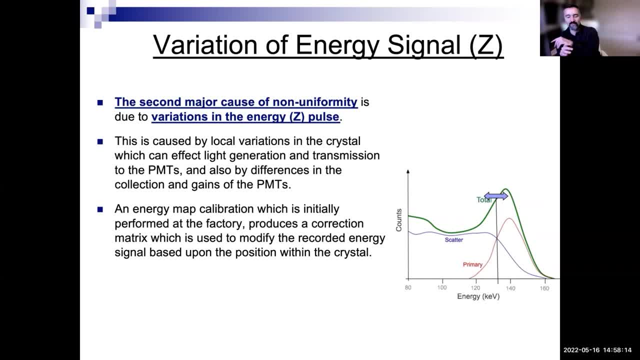 is very, is very in a crystal, so at some place in a crystal. so at some place in a crystal, so at some place. you may be thinking i'm, oh, i'm detecting. you may be thinking i'm, oh, i'm detecting. you may be thinking i'm, oh, i'm detecting, uh. 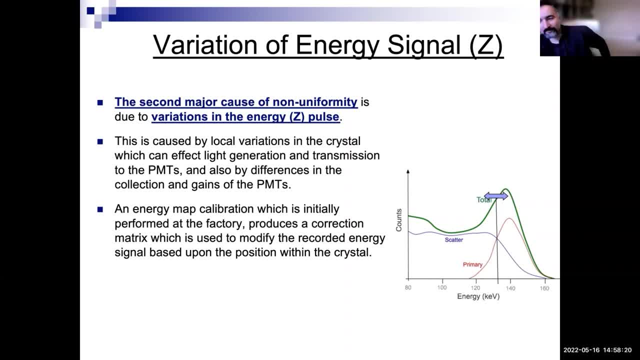 uh, uh, you know 140, you know 140. you know 140, um, um, um, kv. but it's really kv, but it's really kv, but it's really because the sensitivity of the crystal is because the sensitivity of the crystal is because the sensitivity of the crystal is different. you're getting more signal. 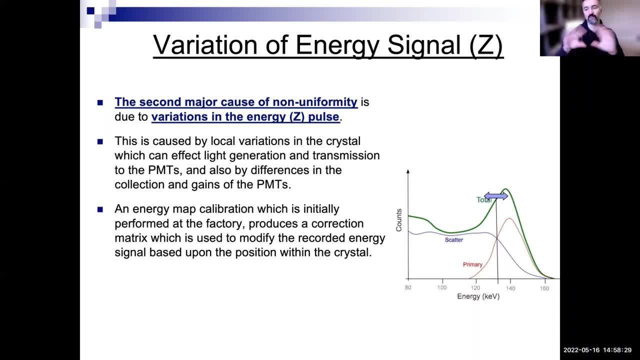 different, you're getting more signal. different, you're getting more signal. you think, oh, that means the original ray. you think, oh, that means the original ray. you think, oh, that means the original ray must have had more energy, but no, this is. must have had more energy, but no, this is. 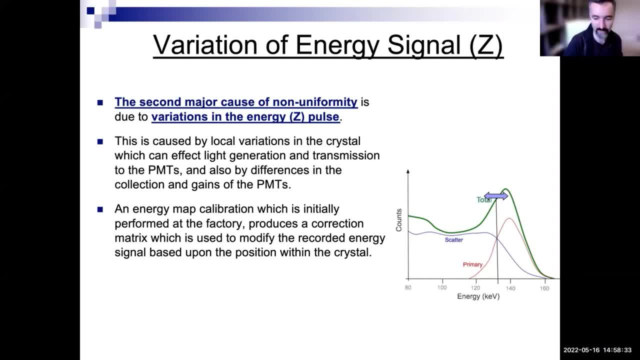 must have had more energy. but no, this is just because, just because, just because the crystal is not uniform, so again you, the crystal is not uniform. so again you, the crystal is not uniform. so again you can correct for this because you know, can correct for this, because you know. 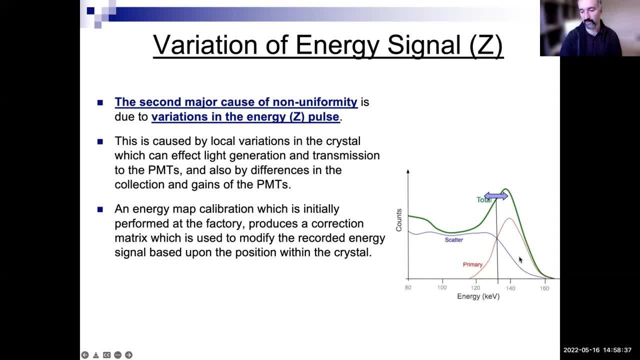 can correct for this, because you know the truth. the truth is supposed to be 140, the truth, the truth is supposed to be 140. the truth, the truth is supposed to be 140 kv, kv, kv. so if i get a signal that is centered at, so, if i get a signal that is centered at: 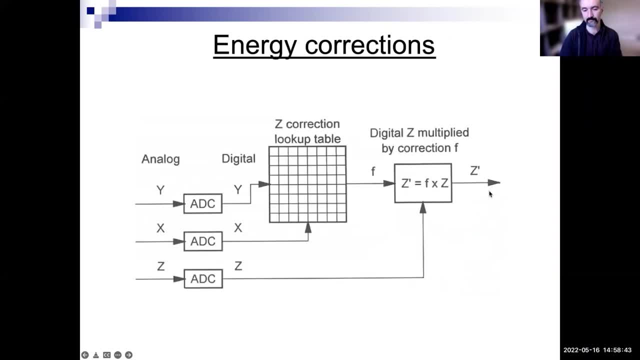 so if i get a signal that is centered at the wrong place, i'm just going to shift the wrong place. i'm just going to shift the wrong place, i'm just going to shift it and fix it, it and fix it, it and fix it. so you fix the z signal, the energy. 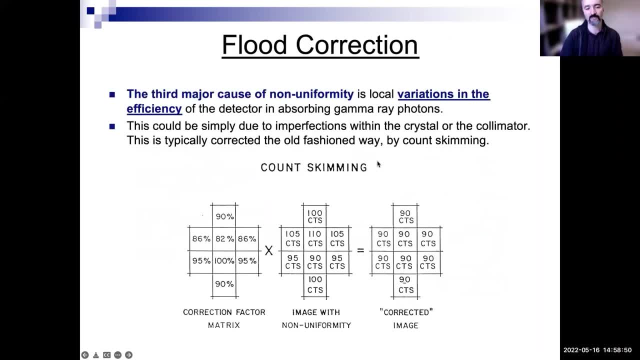 so you fix the z signal, the energy. so you fix the z signal, the energy signal, signal, signal, and so, and then the third part is: and so, and then the third part is: and so, and then the third part is: is, is is efficiency of the detector. so so after 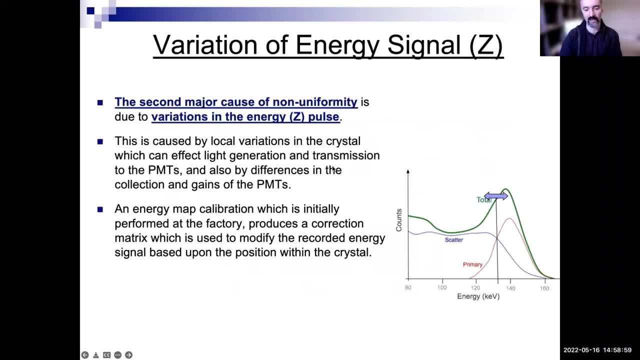 efficiency of the detector. so so, after efficiency of the detector. so so, after you do these two things, you do these two things, you do these two things, right, uh, after you do these two, two, right uh, after you do these two, two, right uh, after you do these two, two things, you take care of the. 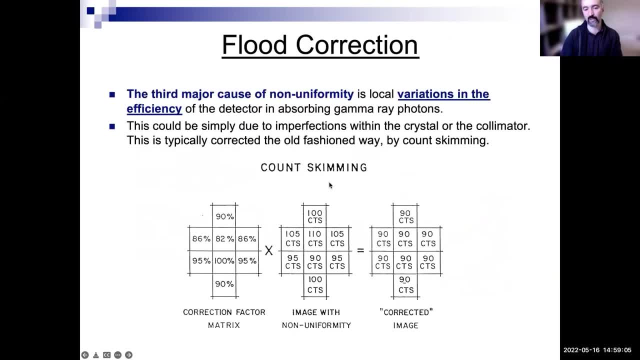 things you take care of, the things you take care of: the shifts in the energy and the position: shifts in the energy and the position shifts in the energy and the position. you still may get some non-uniformities. you still may get some non-uniformities. 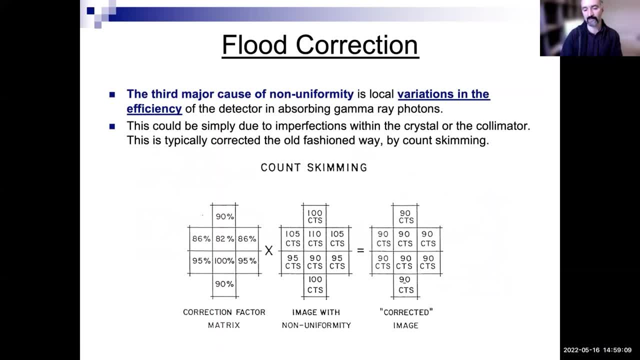 you still may get some non-uniformities. okay, okay, okay, um, um, um, and then you can do count skimming, or and then you can do count skimming, or and then you can do count skimming, or whatever. just say okay, whatever. just say okay, whatever. just say okay, after i did everything, i still get on. 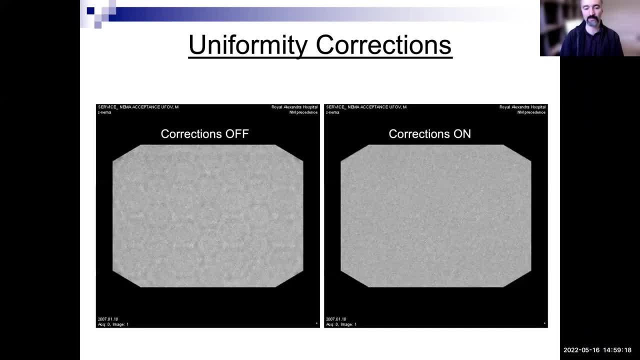 after i did everything, i still get on. after i did everything, i still get on uniformities, uniformities, uniformities, and then you can still have a lookup, and then you can still have a lookup, and then you can still have a lookup table and fix that. so if you don't do, 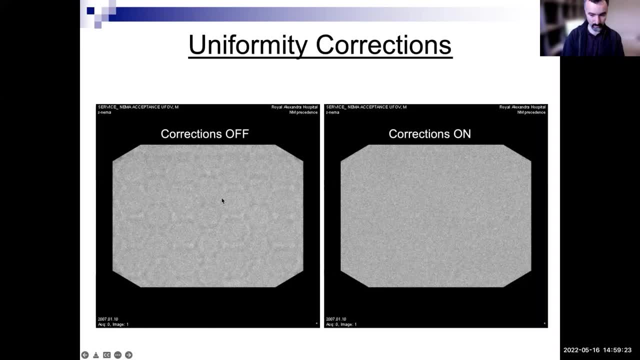 table and fix that. so if you don't do table and fix that, so if you don't do these corrections, you may get something. these corrections, you may get something, these corrections. you may get something like this which looks awful, i mean sort. like this which looks awful, i mean sort. 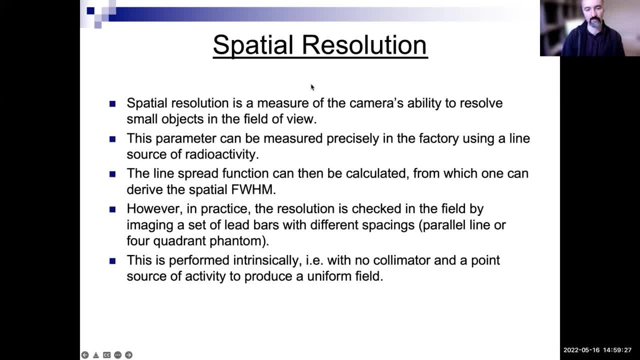 like this which looks awful- i mean sort of right. this looks much better of right. this looks much better of right, this looks much better. so spatial resolution is another. so spatial resolution is another. so spatial resolution is another measurement that that we make. it's a measurement that that we make, it's a. 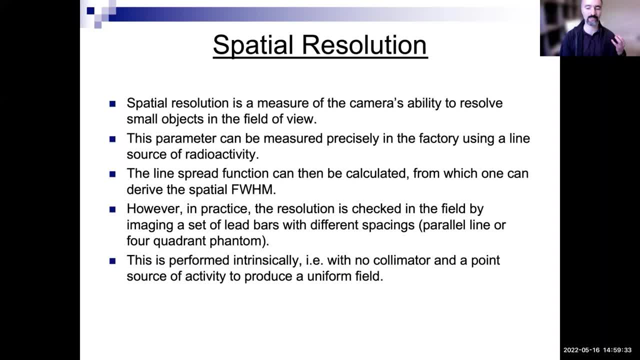 measurement that that we make. it's a very like. if some of those are special, very like. if some of those are special, very like, if some of those are special resolution, you should probably know what resolution, you should probably know what resolution, you should probably know what that really means. and it's basically the. 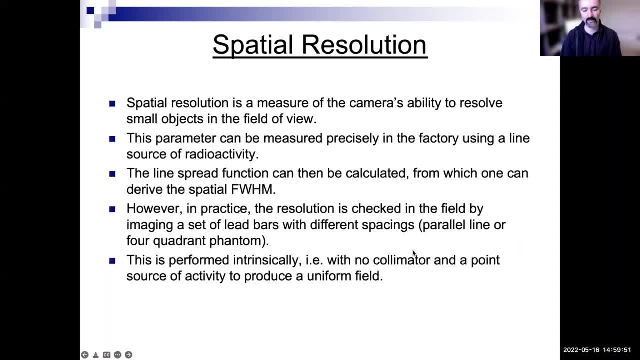 that really means, and it's basically the. that really means and it's basically the. and this is performed intrinsically with and this is performed intrinsically with and this is performed intrinsically with no column meter, no column meter, no column meter and a point source. 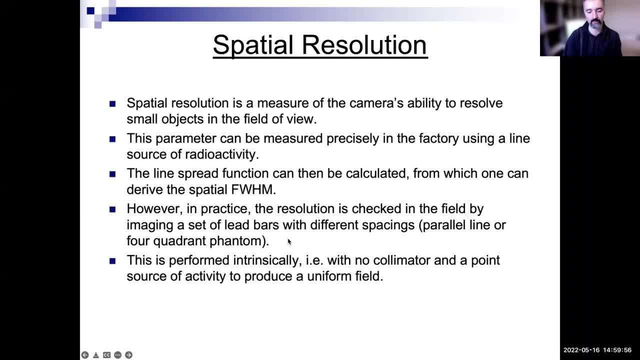 and a point source and a point source, or you could be putting line sources, or you could be putting line sources, or you could be putting line sources, so we could be putting a single point. so we could be putting a single point, so we could be putting a single point source and measuring that. 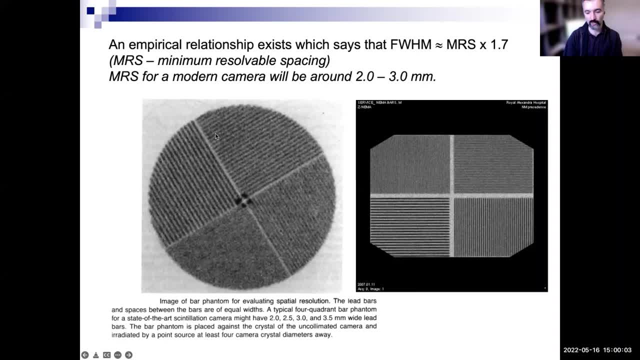 source and measuring that source, and measuring that, uh, uh, uh, and then we could be putting uh line, and then we could be putting uh line, and then we could be putting uh line. sources, sources, sources, to see how able we are to resolve these. to see how able we are to resolve these. 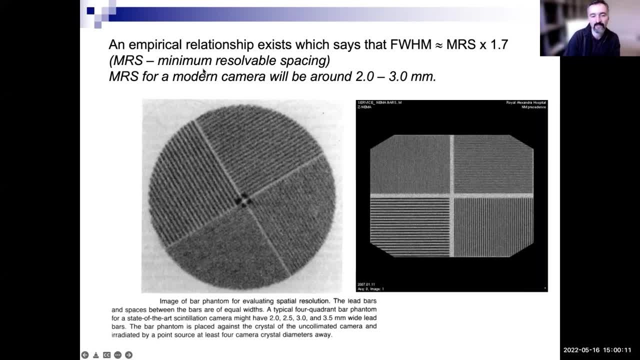 to see how able we are to resolve these separations between these line sources. separations between these line sources, separations between these line sources. and that turns out to relate to the. and that turns out to relate to the. and that turns out to relate to the resolution of a single point source. 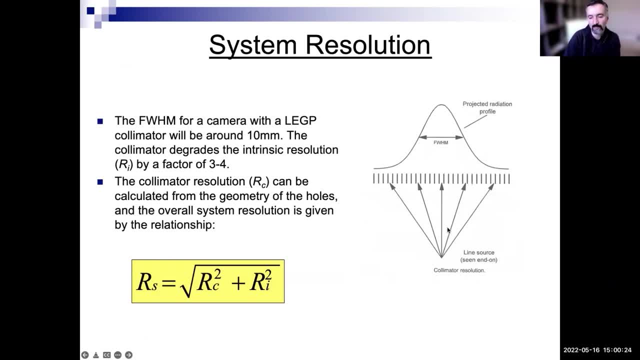 resolution of a single point source. resolution of a single point source. there's some math behind that. there's some math behind that. there's some math behind that. so we kind of talked about this, so we kind of talked about this. so we kind of talked about this um. 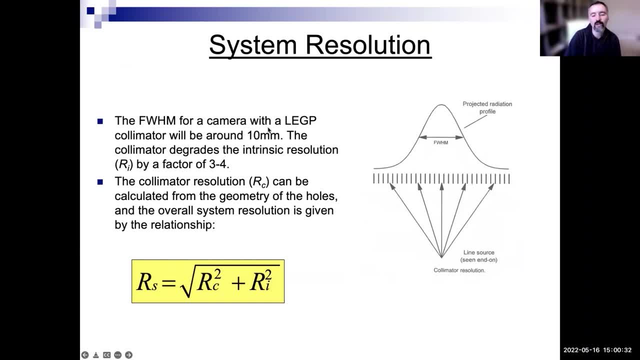 you have um the you have um the you have um the resolution of a typical resolution, of a typical resolution, of a typical leap or low energy general purpose, or leap or low energy general purpose, or leap or low energy general purpose or all-purpose. columnator is around one. 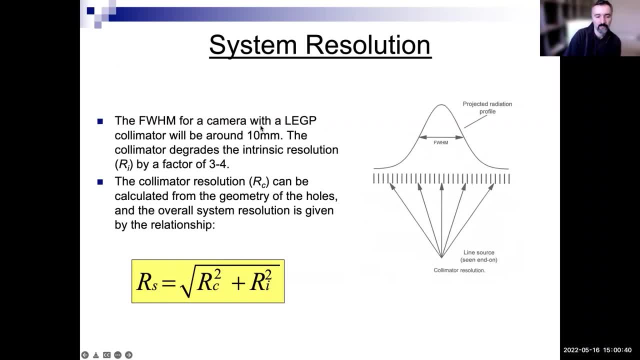 all-purpose columnator is around one. all-purpose columnator is around one centimeter. centimeter, centimeter, um, um, um and the column area degrades the. and the column area degrades the. and the column area degrades the. would have been better, but once you added. 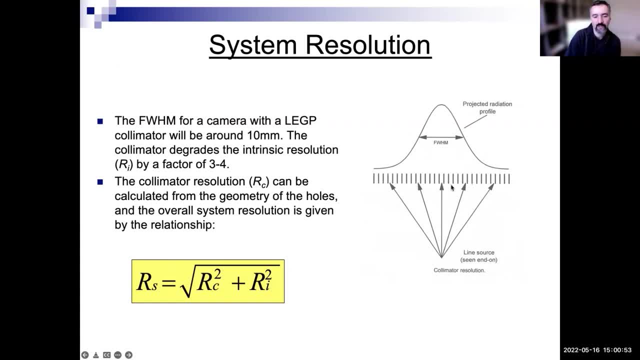 would have been better. but once you added, would have been better. but once you added these, these, these, uh stuff happened, uh, stuff happened, uh, stuff happened okay. so in other words, if, if, if, if i okay. so in other words, if, if, if, if i okay. so in other words, if, if, if, if i attach a point. source: 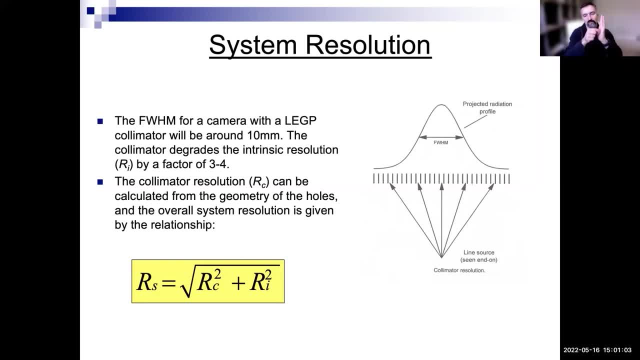 attach a point source. attach a point source to a crystal. if i attach it, you will be to a crystal. if i attach it, you will be to a crystal. if i attach it, you will be able to see it very well, able to see it very well, able to see it very well. but once you start putting in a columnator, 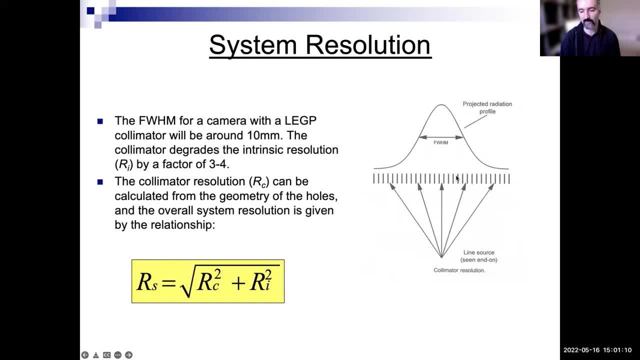 but once you start putting in a columnator, but once you start putting in a columnator, um, um, um, and also, depending on the distance that, and also depending on the distance that you have to to this, you have to to this, you have to to this, you're going to be, uh, degrading things. 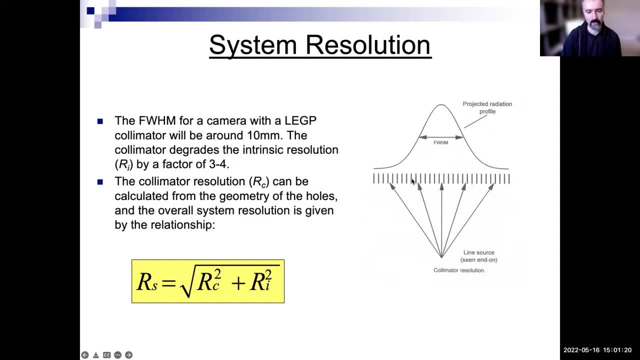 you're going to be, uh, degrading things. you're going to be, uh, degrading things, so, so, so, so, and it depends on the geometry of the so, and it depends on the geometry of the so and it depends on the geometry of the holes. overall resolution. so you've got. 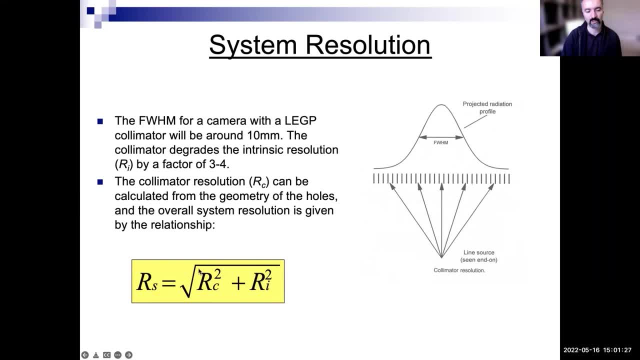 holes: overall resolution. so you've got holes. overall resolution. so you've got intrinsic resolution, intrinsic resolution, intrinsic resolution. you've got collimator resolution. so you've got collimator resolution. so you've got collimator resolution. so notice this: right now, if something enters here, i don't know if- 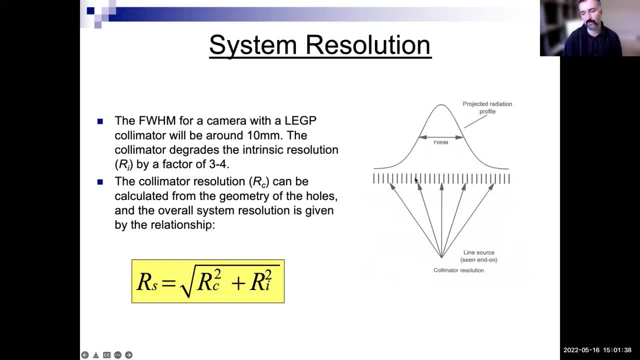 if something enters here, i don't know if. if something enters here, i don't know if it entered here or here or here, or it entered here or here or here, or it entered here or here, or here or here. so that defines, uh, that almost defines here. so that defines, uh, that almost defines. 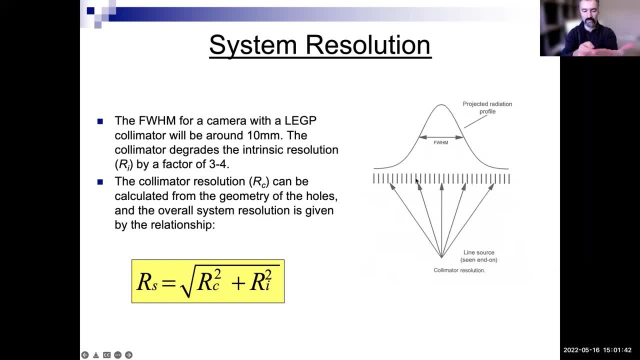 here. so that defines- uh, that almost defines, the resolution. whereas if i had the resolution, whereas if i had the resolution, whereas if i had attached this to the crystal, you would attached this to the crystal, you would attached this to the crystal. you would know, literally well, know, literally well. 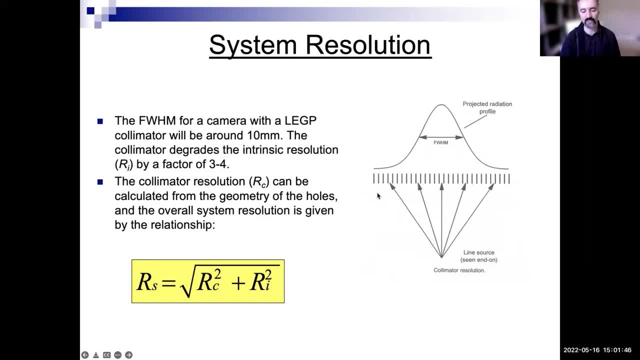 know literally. well, it's here, um, so i won't go through it's here, um so i won't go through it's here, um so i won't go through those details. but the point is that those details. but the point is that those details. but the point is that, um, the point is that the overall 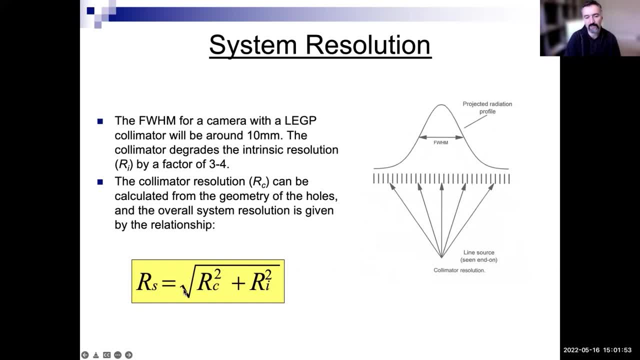 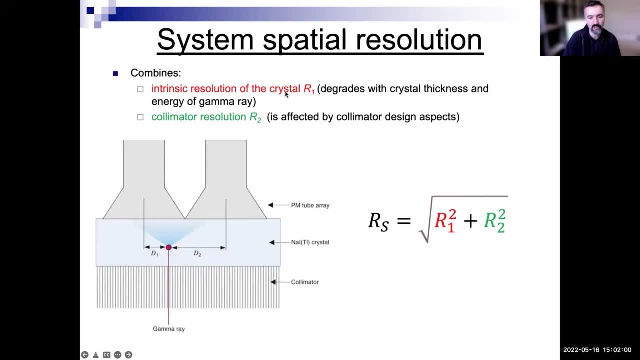 um, the point is that the overall um. the point is that the overall resolution, resolution, resolution is worse than the intrinsic resolution. so um, and there's multiple things going, so um, and there's multiple things going, so um, and there's multiple things going on. there is the contribution of the 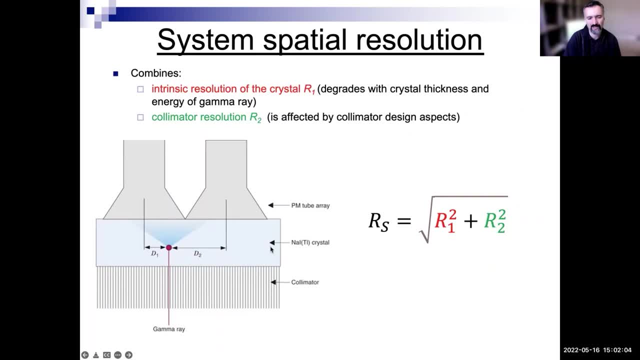 on. there is the contribution of the on. there is the contribution of the intrinsic resolution of the crystal. which intrinsic resolution of the crystal, which intrinsic resolution of the crystal, which depends on things, depends on things, depends on things like the crystal thickness, etc. the energy, like the crystal thickness, etc. the energy. 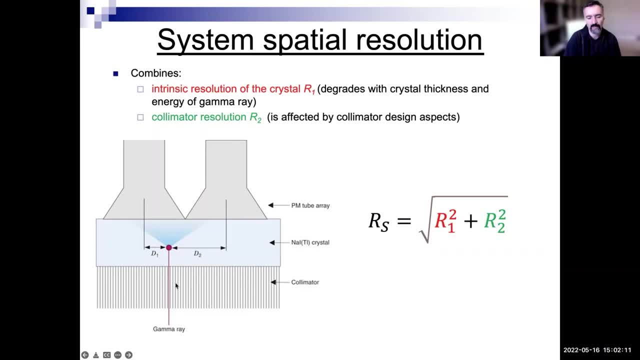 like the crystal thickness, etc. the energy of the gamma ray, of the gamma ray, of the gamma ray, but also the collimator design itself, but also the collimator design itself, but also the collimator design itself gives you a certain resolution, and these gives you a certain resolution, and these 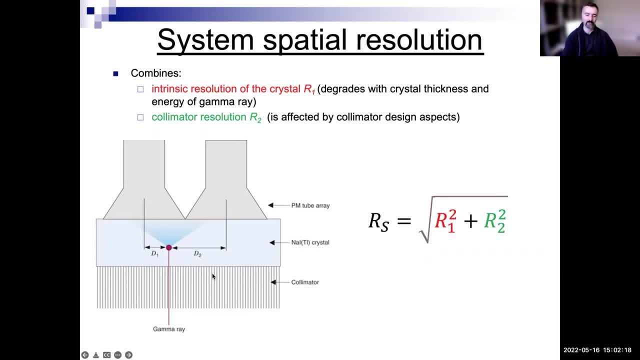 gives you a certain resolution and these two things compound together, two things compound together, two things compound together um to give you the overall resolution, um to give you the overall resolution, um to give you the overall resolution because, again, if you put a point source, because again, if you put a point source, 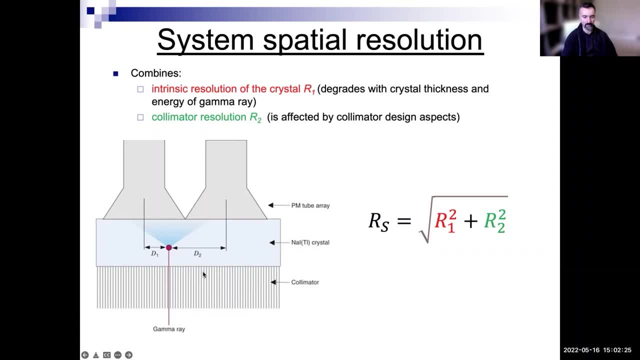 because, again, if you put a point source right here, that would give you the right here, that would give you the right here, that would give you the intrinsic resolution, intrinsic resolution, intrinsic resolution. but once you add a collimator, your. but once you add a collimator, your. 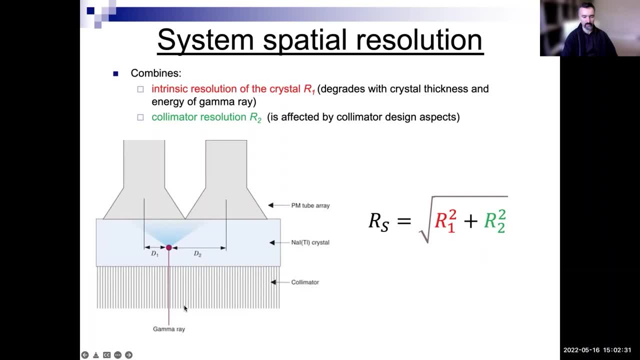 but once you add a collimator, your resolution starts to become here, resolution starts to become here. resolution starts to become here, right, so you wouldn't know if you want right, so you wouldn't know if you want right. so you wouldn't know if you want to know where within this? 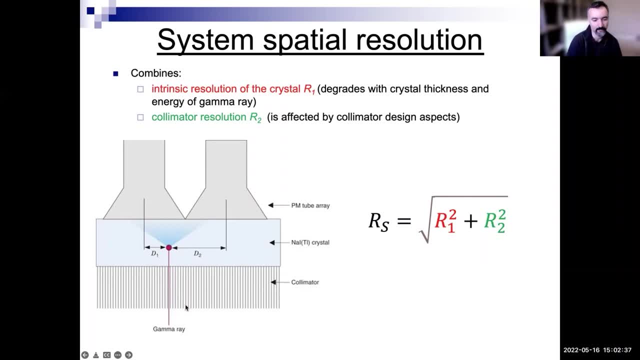 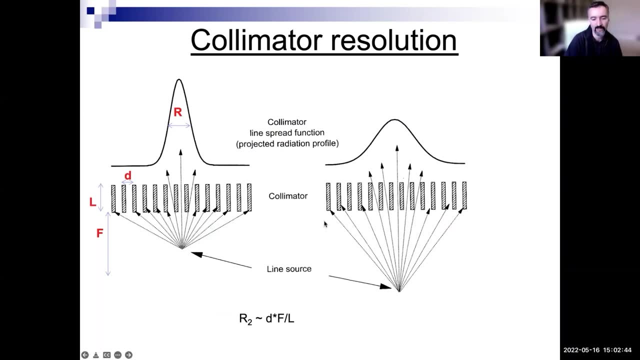 to know where within this, to know where within this point, sources. okay, so, and as you mentioned before, as you get, and as you mentioned before, as you get, and as you mentioned before, as you get, farther away, farther away, farther away, as your distance increases, your, as your distance increases, your. 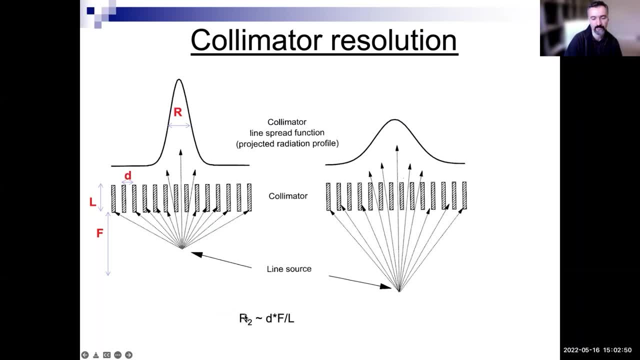 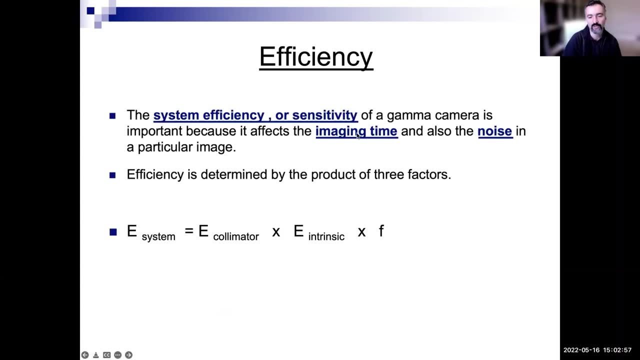 as your distance increases, your resolution gets bigger, which means it resolution gets bigger, which means it resolution gets bigger, which means it gets worse, gets worse, gets worse, okay, so, okay, so, okay. so you know, we talked about that, you know we talked about that, you know we talked about that: the efficiency or the sensitivity of a 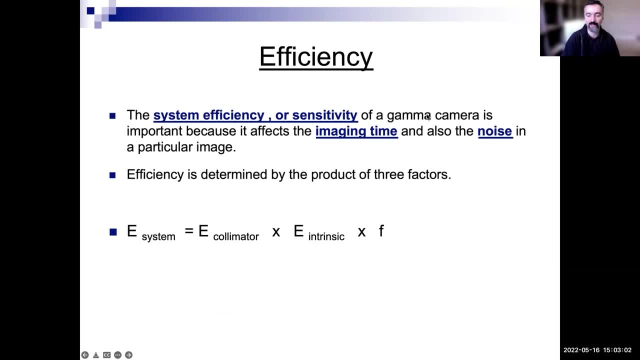 the efficiency or the sensitivity of a. the efficiency or the sensitivity of a gamma camera is important because it gamma camera is important, because it gamma camera is important, because it affects the imaging time. remember how i affects the imaging time. remember how i affects the imaging time. remember how i said: 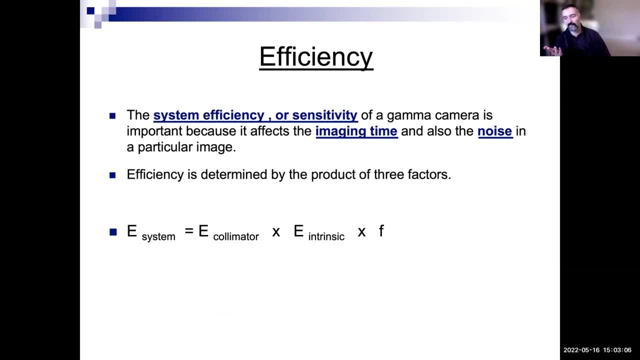 said, said: if we could image forever, we wouldn't. if we could image forever, we wouldn't. if we could image forever, we wouldn't. this wouldn't really have it. have a this wouldn't really have it. have a this wouldn't really have it. have a problem- this wouldn't be a problem. but we. 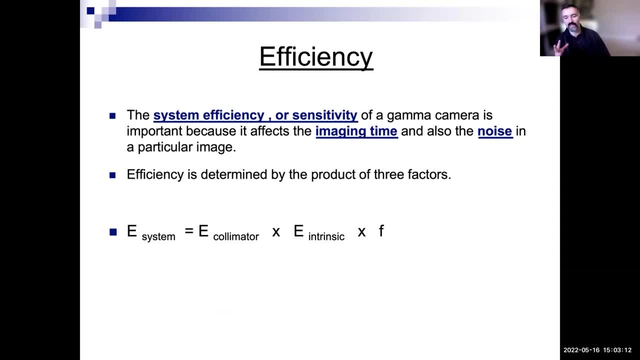 problem. this wouldn't be a problem, but we problem. this wouldn't be a problem, but we cannot image forever. therefore, we cannot image forever. therefore, we cannot image forever. therefore, we cannot have a really poor resolution, cannot have a really poor resolution, cannot have a really poor resolution camera. 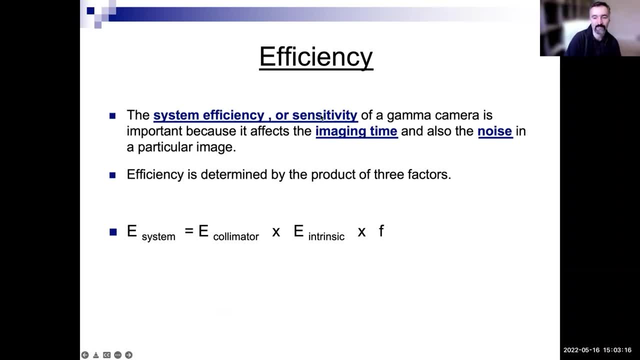 camera, camera, um. so it's really going to define the um. so it's really going to define the um. so it's really going to define the noise in the image and the. you know noise in the image and the. you know noise in the image and the. you know minimum imaging time that you need to. 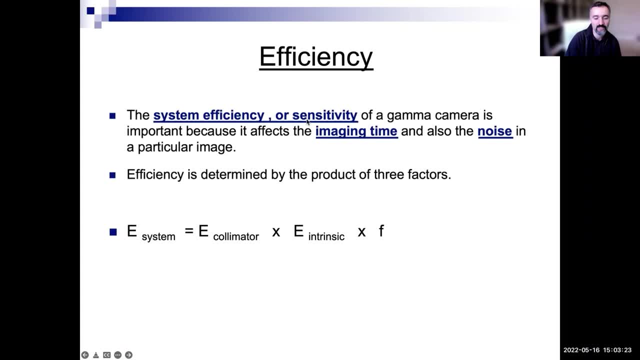 minimum imaging time that you need to minimum imaging time that you need to get a decent image. so the efficiency is: get a decent image. so the efficiency is get a decent image. so the efficiency is important. what is the efficiency of the important? what is the efficiency of the? 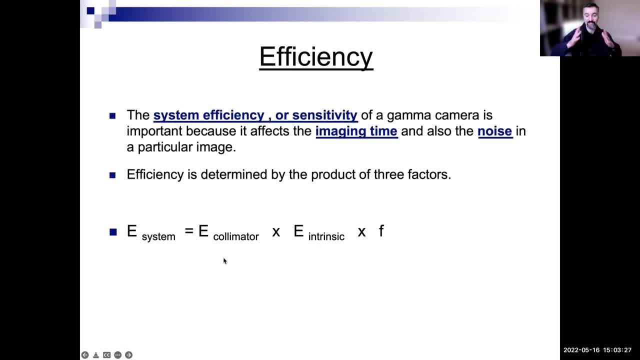 important. what is the efficiency of the detector? what is the efficiency of the detector? what is the efficiency of the detector? what is the efficiency of the collimators? because collimators kill collimators, because collimators kill collimators, because collimators kill signal. if you make collimators really 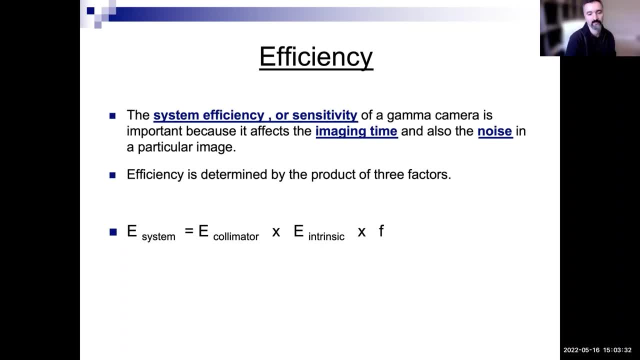 signal. if you make collimators really signal. if you make collimators really long or tall, they're going to kill more. long or tall, they're going to kill more. long or tall, they're going to kill more and more signal and more signal and more signal. okay, so so these are very important so. okay, so, so, these are very important. so, okay, so, so, these are very important. so the efficiency, this is a mind-blowing. the efficiency, this is a mind-blowing the efficiency, this is a mind-blowing number. it's almost depressing the number. it's almost depressing the 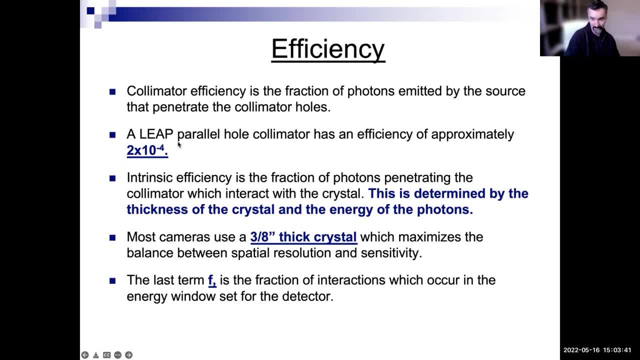 number. it's almost depressing. the efficiency of a common purpose, efficiency of a common purpose. efficiency of a common purpose, let detect, let let um, let, let let um, let, let, let let um. collimator. parallel hole collimator is collimator. parallel hole collimator is collimator. parallel hole collimator is about this much, which means out of every. 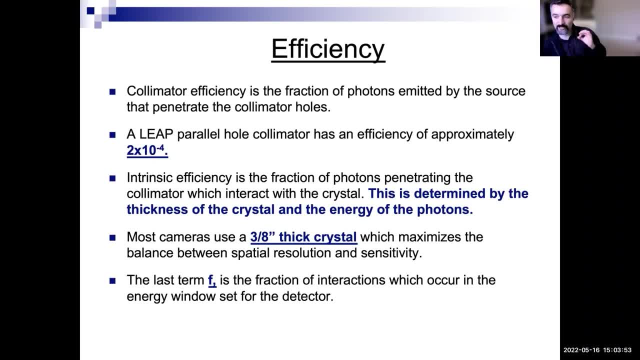 about this much which means out of every, about this much which means out of every thousand, thousand, thousand. sorry. out of every 10 000 photons, sorry out of every 10 000 photons, sorry out of every 10 000 photons emitted from the body, emitted from the body. 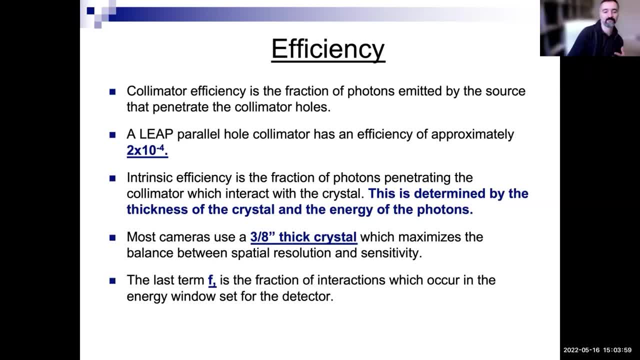 emitted from the body. only like, only like, only like. two of them get detected. two of them get detected. two of them get detected now with pinhole cameras. this number is now with pinhole cameras. this number is now with pinhole cameras. this number is increasing, increasing. 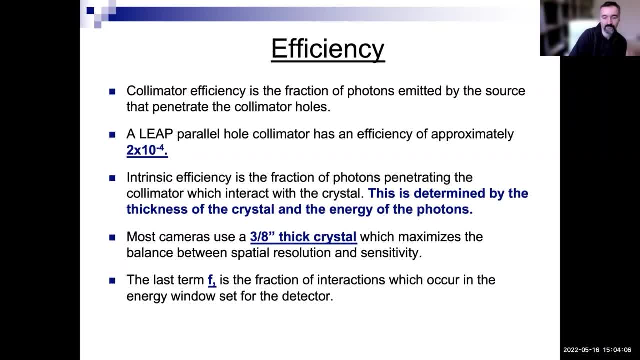 increasing, but we're looking at definitely less. but we're looking at definitely less, but we're looking at definitely less than a percent than a percent, but we're looking at definitely less than a percent. more than 99 percent of more than 99 percent of more than 99 percent of signals being killed. 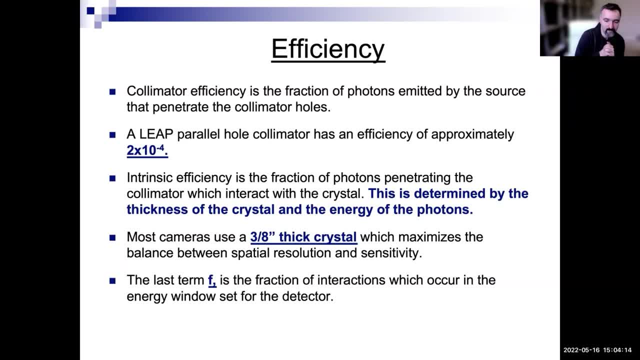 signals being killed. signals being killed: okay, so, okay, so okay, so, um, um, um. so that's why it's important to to build, so that's why it's important to to build, so that's why it's important to to build bigger cameras that are covering larger. 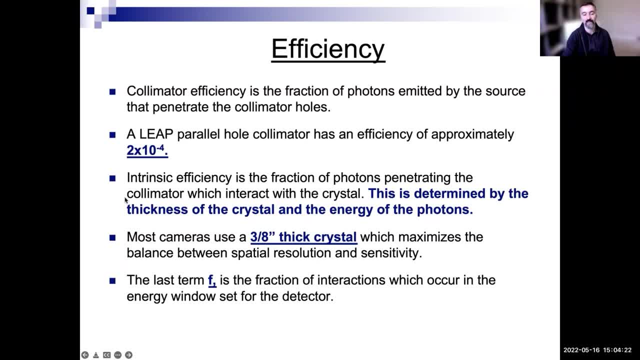 bigger cameras that are covering larger, bigger cameras that are covering larger parts of the body. to come close to the parts of the body. to come close to the parts of the body, to come close to the patient as much as we possibly can and patient as much as we possibly can. and 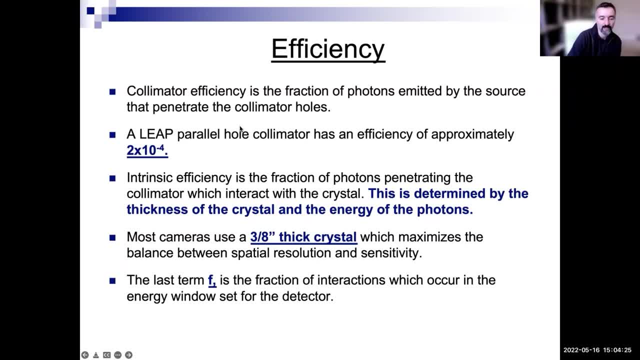 patient as much as we possibly can, and to build more innovative to make more, to build more innovative, to make more, to build more innovative, to make more innovative, innovative innovative, uh scanners, uh scanners, uh scanners, okay, so, um, okay, so, um, okay, so, um, that last term f that we had. 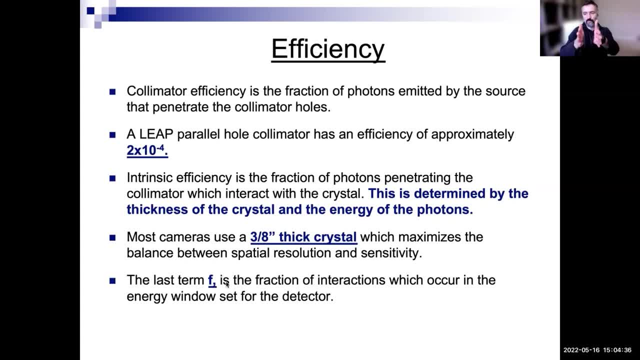 that last term f, that we had that last term f that we had uh uh, uh has to do with the energy resolution of. has to do with the energy resolution of. has to do with the energy resolution. of course you could make the energy, course you could make the energy. 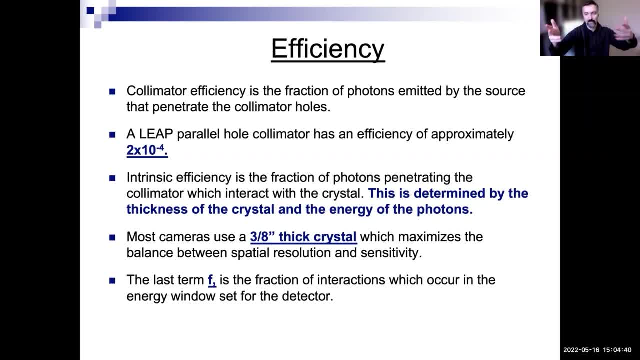 course you could make the energy resolution, uh, or the energy window bigger resolution, uh, or the energy window bigger resolution, uh, or the energy window bigger. but then that way, sure you're getting, but then that way, sure you're getting, but then that way, sure you're getting more sensitivity, but you're also. 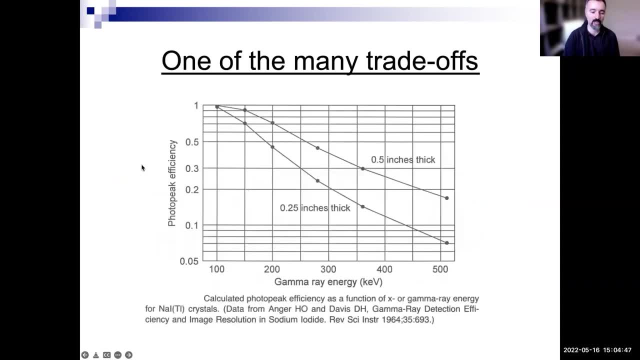 more sensitivity, but you're also more sensitivity, but you're also bringing in more non-wanted events, bringing in more non-wanted events, bringing in more non-wanted events. so here's a plot of so, here's a plot of so. here's a plot of the efficiency as a function of the 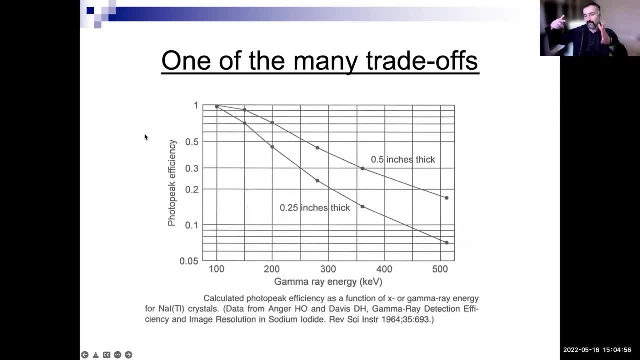 the efficiency as a function of the, the efficiency as a function of the energies. the higher the energy your energies, the higher the energy your energies, the higher the energy your efficiency goes lower because the efficiency goes lower, because the efficiency goes lower because the gamma rays are going to be so penetrating. 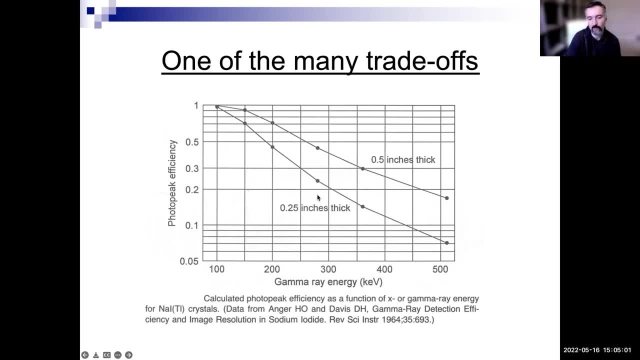 gamma rays are going to be so penetrating. gamma rays are going to be so penetrating they could even pass through your. they could even pass through your, they could even pass through your crystal, crystal, crystal. so so the width or the thickness of. so so the width or the thickness of 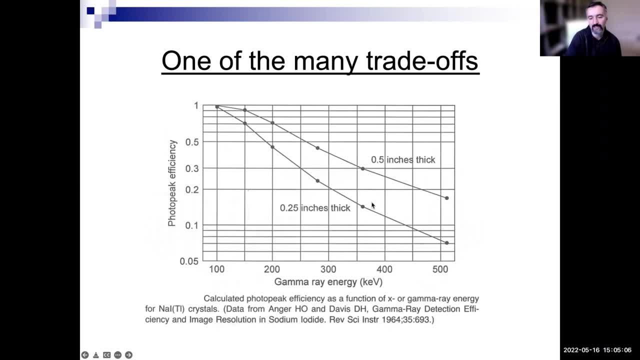 so. so the width or the thickness of the crystal, the intrinsic sensitivity of the crystal, the intrinsic sensitivity of the crystal, the intrinsic sensitivity of the crystal, the crystal, the crystal increases as the width becomes bigger, increases as the width becomes bigger, increases as the width becomes bigger. that makes sense. 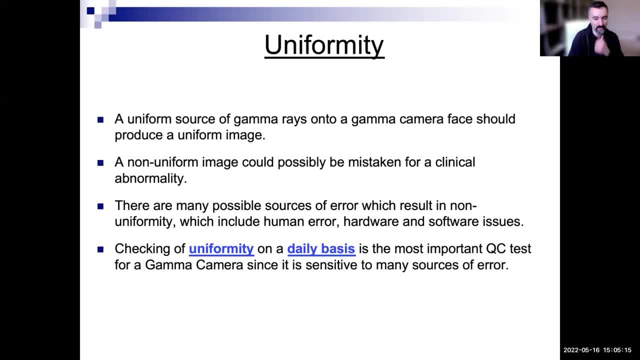 that makes sense. that makes sense. um so some artifacts that you might get. um so some artifacts that you might get. um so some artifacts that you might get. you might get uniformity, you might get uniformity, you might get uniformity. artifacts um a non-uniform image could. 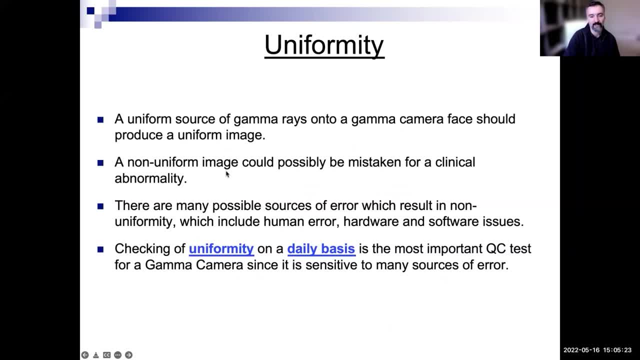 artifacts um a non-uniform image could artifacts um a non-uniform image? could be mistaken for a clinical abnormality, be mistaken for a clinical abnormality, be mistaken for a clinical abnormality, and that's really bad right. so, uh, and that's really bad right, so uh. 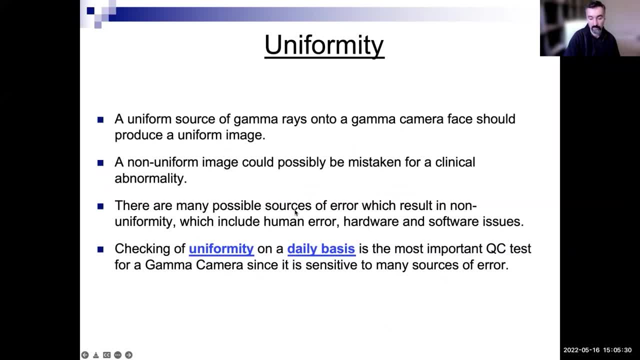 and that's really bad right. so, uh, that can uh result. uh, there are many that can uh result. uh, there are many that can uh result. uh, there are many possible sources of error which results possible sources of error which results possible sources of error which results in non-uniformity. 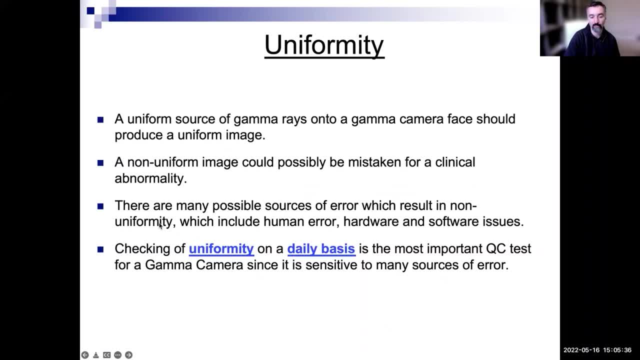 in non-uniformity, in non-uniformity, um. so what are some of the reasons that? um so? what are some of the reasons that? um? so what are some of the reasons that the most important qc test that is done, the most important qc test that is done? 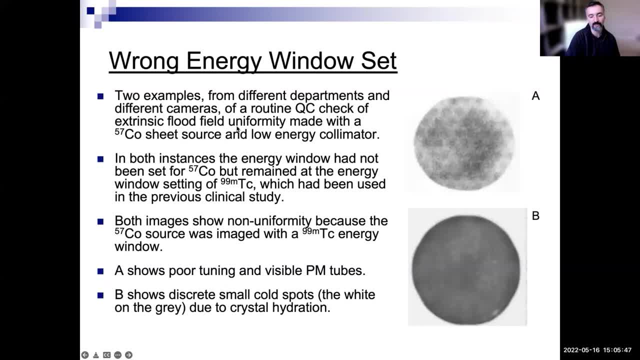 the most important qc test that is done on a daily basis, on a daily basis, on a daily basis um now this could be caused by human um. now this could be caused by human um. now this could be caused by human errors, like the errors, like the errors, like the. the human operator, the technologist sets. 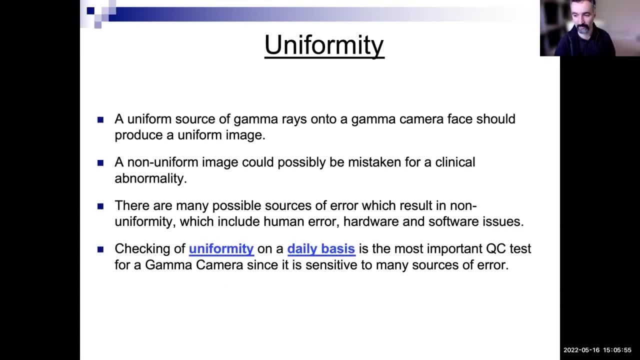 the human operator. the technologist sets the human operator, the technologist sets the wrong energy window, the wrong energy window. the wrong energy window because it's the like it's 140 kb, but because it's the like it's 140 kb, but because it's the like it's 140 kb, but they set it to be 300 and so 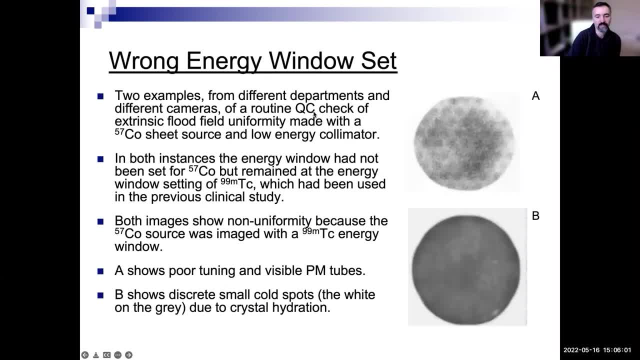 they set it to be 300, and so they set it to be 300, and so everything's all messed up. everything's all messed up. everything's all messed up. that's one example. that's one example. that's one example. um, um, um. this is a routine qc check of an. 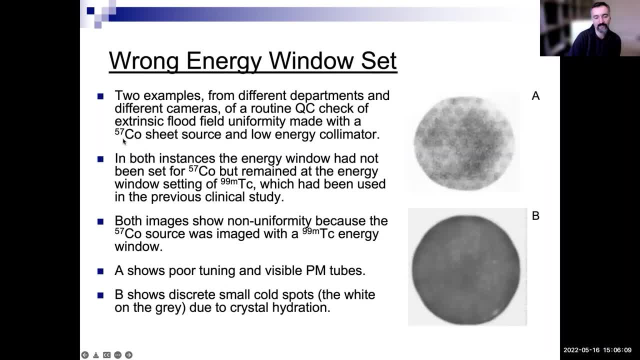 this is a routine qc check of an. this is a routine qc check of an extrinsic source that is used like daily extrinsic source. that is used like daily extrinsic source. that is used like daily, like a daily scan, but they use the like a daily scan but they use the. 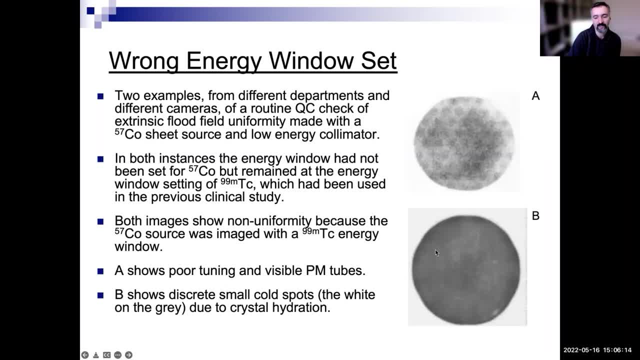 like a daily scan, but they use the wrong low energy collimator. wrong low energy collimator. wrong low energy collimator. okay versus not, okay versus not, okay versus not okay. so so using the wrong energy, you're okay. so so using the wrong energy, you're okay. so so using the wrong energy, you're going to get really different signals. 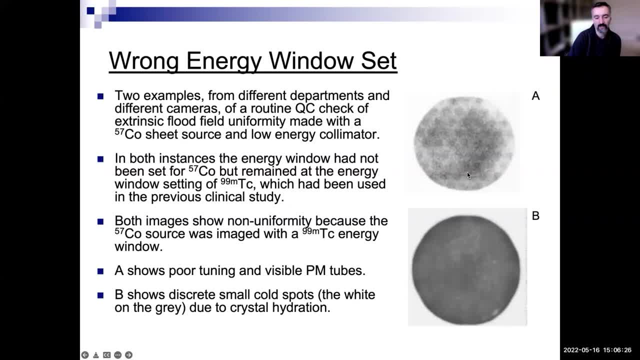 going to get really different signals. going to get really different signals. both images show some non-uniformity. both images show some non-uniformity. both images show some non-uniformity. uh, uh, uh. because the source was imaged with. because the source was imaged with. 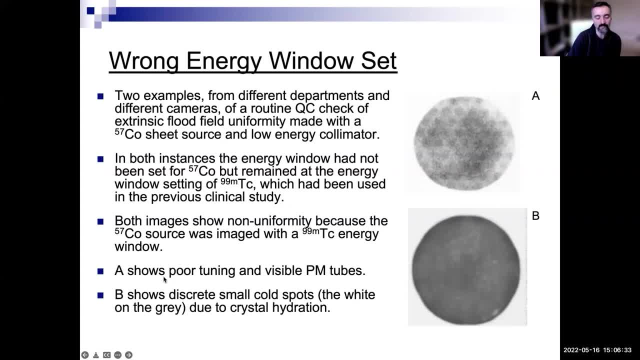 because the source was imaged with technetium energy, technetium energy, technetium energy. okay, okay, okay, so, so, so, this one, this one, this one is because of uh poor toning too is because of uh, poor toning too is because of uh poor toning too, okay. 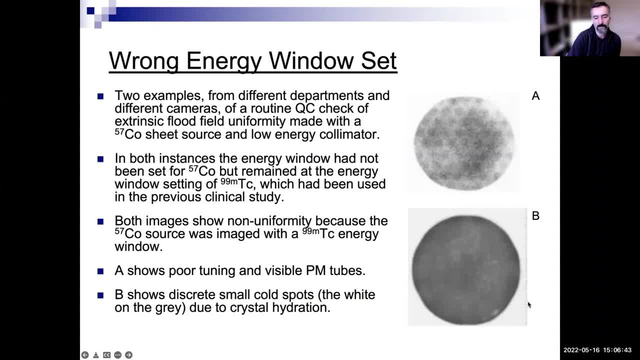 okay. okay, this one has crystal hydration issues, okay, but there's a whole bunch of things okay, but there's a whole bunch of things okay, but there's a whole bunch of things going, so there's something going, so there's something going, so there's something actually wrong with these. 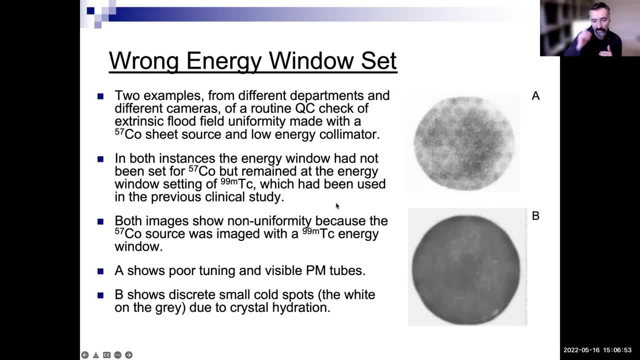 actually wrong with these, actually wrong with these. but on top of that, the energy window. but on top of that, the energy window. but on top of that, the energy window. being off creates issues. being off creates issues. being off creates issues. okay, okay, okay, so, uh, so, uh. 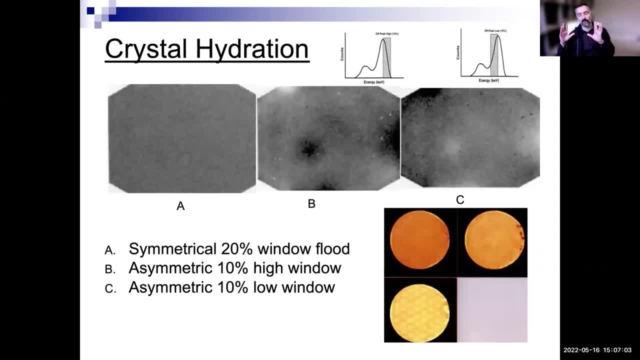 so, uh, so then how do we do it's almost like so, then how do we do it's almost like so? then how do we do? it's almost like too many things, too many things, too many things are gone wrong. there's something wrong. are gone wrong. there's something wrong. 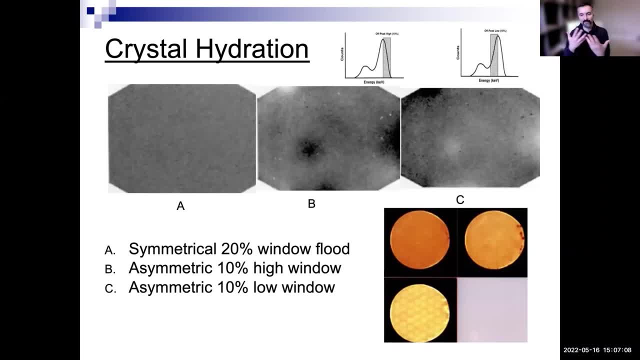 are gone wrong. there's something wrong and our setting is wrong, but sometimes a and our setting is wrong, but sometimes a and our setting is wrong, but sometimes a wrong setting done in different wrong wrong setting done in different wrong wrong setting done in different wrong ways can actually tell you what's going. 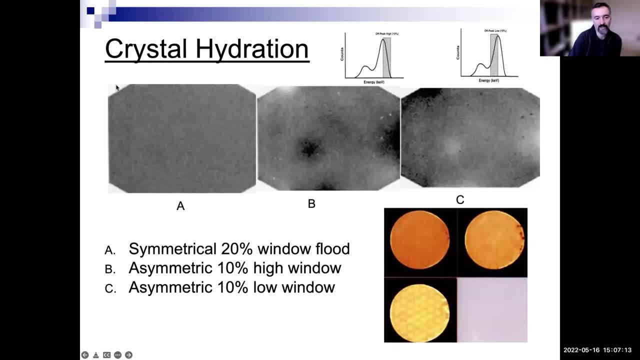 ways can actually tell you what's going. ways can actually tell you what's going on, on on. so if you put a uh, if you have crystal, so if you put a uh, if you have crystal. so if you put a uh, if you have crystal hydration, if you put a symmetric energy, 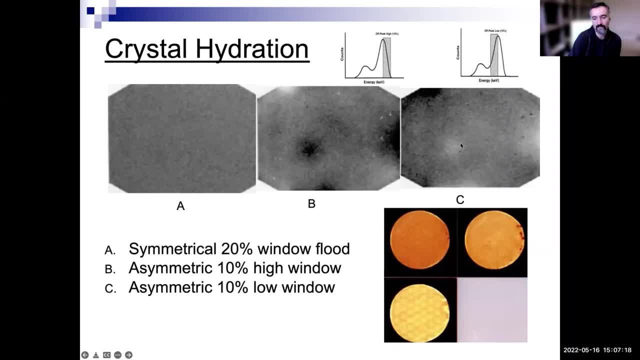 hydration. if you put a symmetric energy hydration, if you put a symmetric energy window, you get this window. you get this window, you get this, but if you put the wrong window, you. but if you put the wrong window, you. but if you put the wrong window, you start to see these kinds of artifacts. 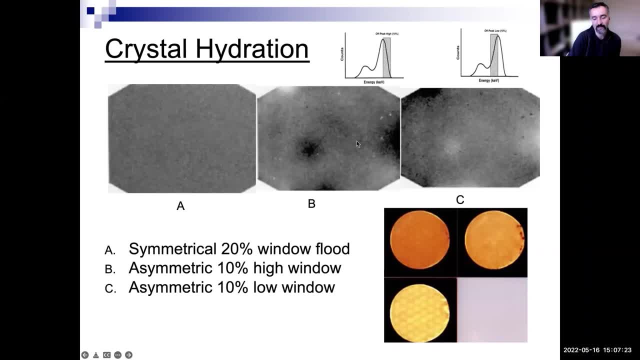 start to see these kinds of artifacts. start to see these kinds of artifacts so that, actually, in a funny way, this was so, that, actually in a funny way, this was so, that, actually in a funny way, this was hidden here, hidden here, hidden here. once you put the, 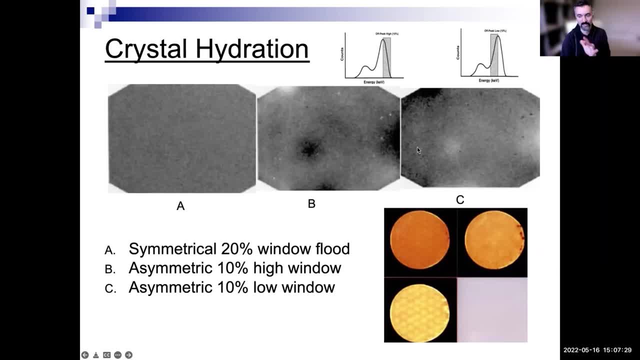 once you put the, once you put the wrong artifact, you start to see wrong, wrong artifact. you start to see wrong, wrong artifact. you start to see wrong energy window. you start to see wrong energy window. you start to see wrong. things in there too. things in there too. 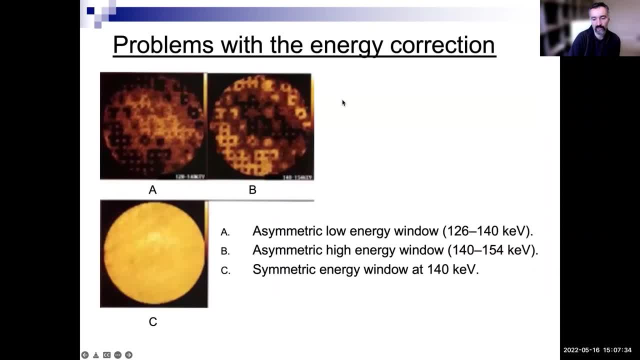 things in there too. right um so energy correction. if not right, um so energy correction. if not right, um so energy correction. if not done right, done right, done right. uh can result in things, for example, if uh can result in things, for example, if uh can result in things. for example, if you put an, 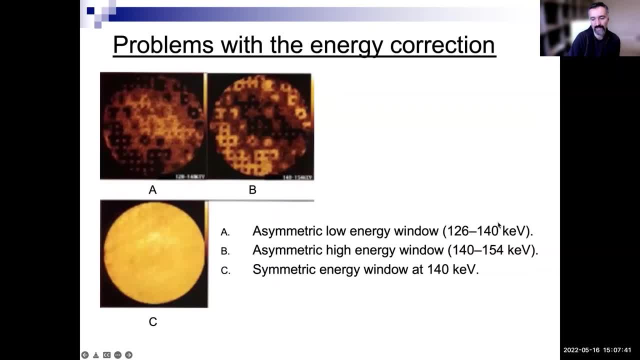 you put an, you put an asymmetric low energy window. that is asymmetric low energy window. that is asymmetric low energy window. that is barely covering the main energy, that we barely covering the main energy, that we barely covering the main energy that we care about, care about, care about we get something like this or a high. 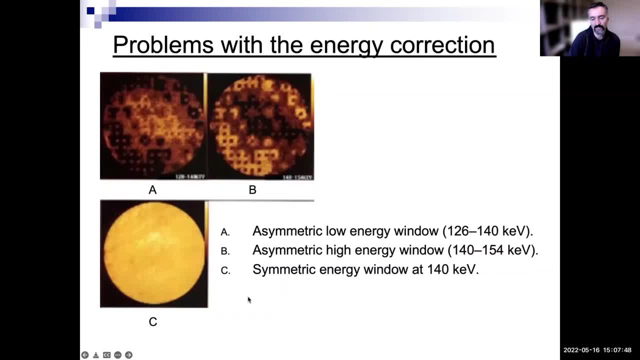 we get something like this or a high. we get something like this or a high energy window. that again energy window. that again energy window. that again doesn't show the things we care about. doesn't show the things we care about. you get this, but once you put in a 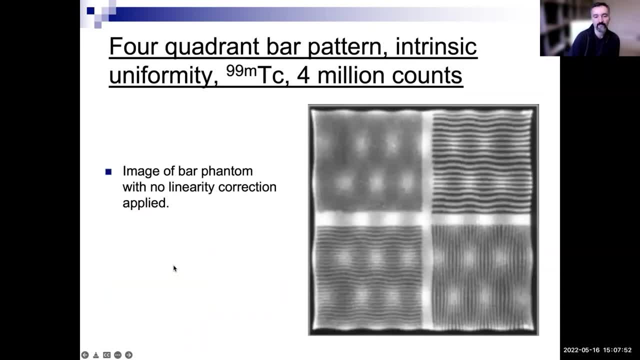 you get this. but once you put in a, you get this. but once you put in a symmetric energy window, you get the thing: symmetric energy window. you get the thing symmetric energy window. you get the thing that we want, that we want, that we want. here's an example of non-linearity: 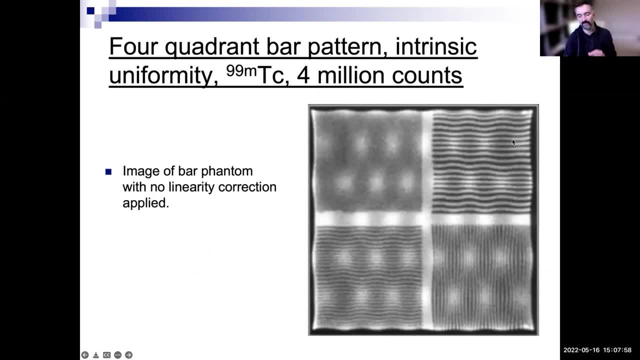 here's an example of non-linearity. here's an example of non-linearity: correction. remember those things where correction. remember those things where correction. remember those things where the edges of the pmts are different in the edges of the pmts, are different in the edges of the pmts are different in the center of the pmt. if you don't do, 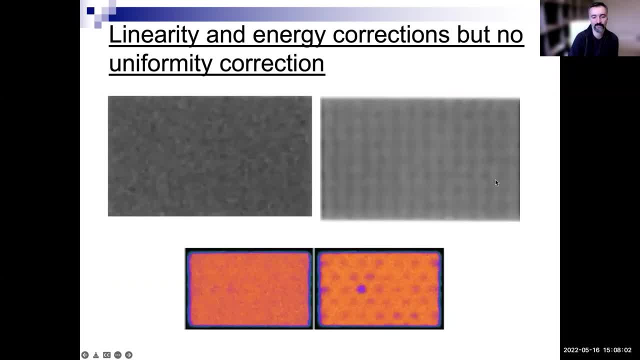 the center of the pmt. if you don't do the center of the pmt, if you don't do energy, energy, energy, linearity correction, you're going to get linearity correction. you're going to get linearity correction. you're going to get cracked crystals. you're going to see. cracked crystals. you're going to see cracked crystals, you're going to see. you sure you want to fix this? otherwise, you sure you want to fix this. otherwise, you sure you want to fix this. otherwise, you're going to start thinking of this. you're going to start thinking of this. 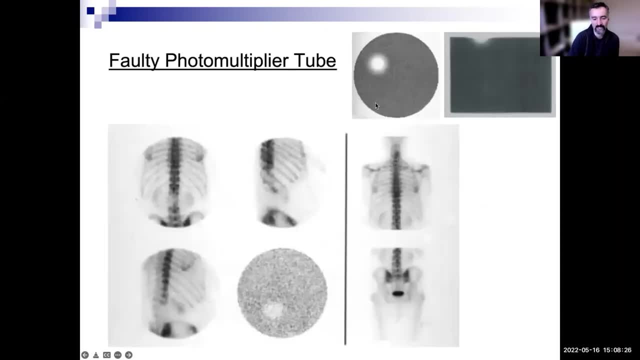 you're going to start thinking of this as defects in the human body, as defects in the human body, as defects in the human body, such as in this scan. this was a faulty, such as in this scan. this was a faulty, such as in this scan. this was a faulty pmt. 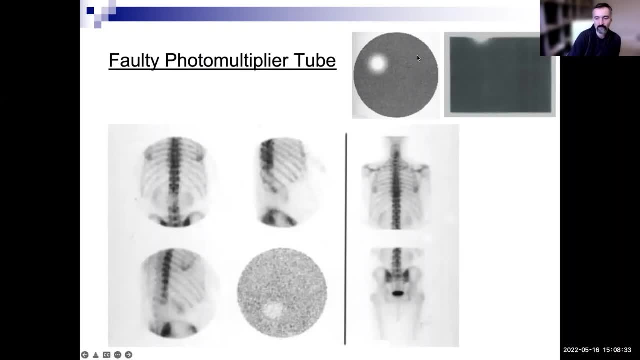 pmt, pmt. the technologies had not caught it, so the technologies had not caught it, so the technologies had not caught it. so they would find this only later, probably they would find this only later, probably they would find this only later, probably. and then you've got a patient that is. 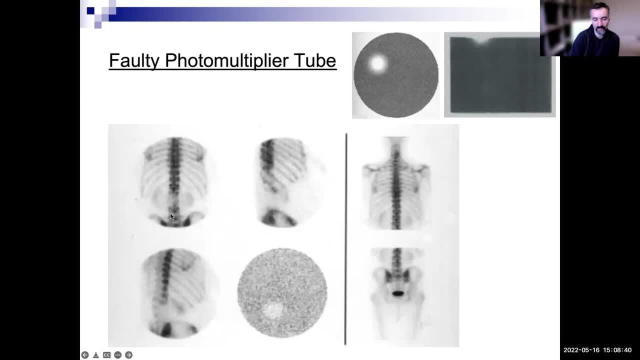 and then you've got a patient that is, and then you've got a patient that is being scanned and you're seeing some being scanned and you're seeing some being scanned and you're seeing some artifacts here and you know that could- artifacts here- and you know that could. 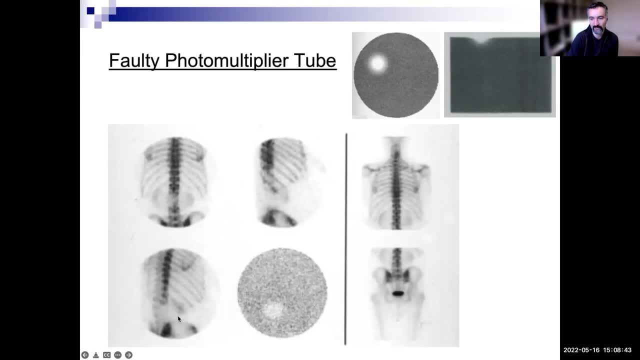 artifacts here and you know that could be totally confusing the diagnosis. be totally confusing the diagnosis. be totally confusing the diagnosis. whereas it was really had nothing to do. whereas it was really had nothing to do, whereas it was really had nothing to do with the patient, had everything to do. 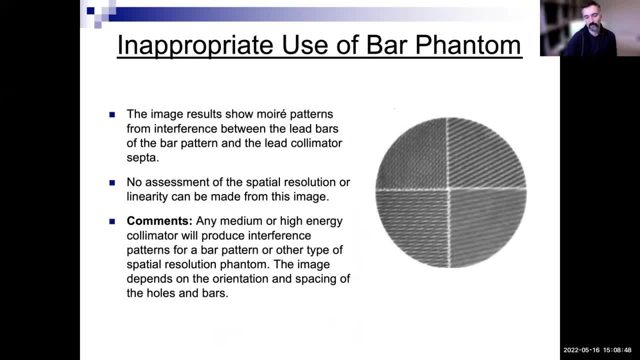 with the patient, had everything to do with the patient, had everything to do with the scanner, with the scanner, with the scanner. the bar phantom. if you don't place it, the bar phantom. if you don't place it, the bar phantom if you don't place it exactly parallel and perpendicular in 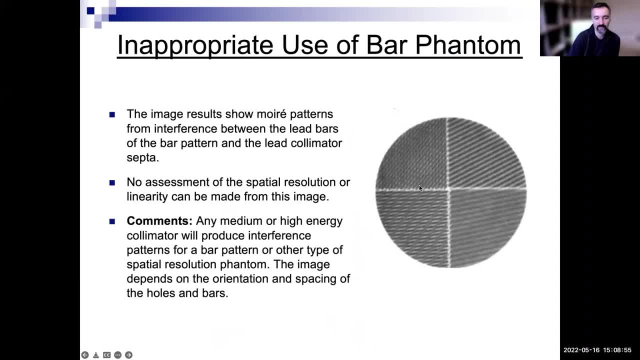 exactly parallel and perpendicular. in exactly parallel and perpendicular in the right way. you're going to get the right way. you're going to get the right way, you're going to get aliasing, uh, sort of artifacts, okay. and also in tomography because: okay, and also in tomography because. 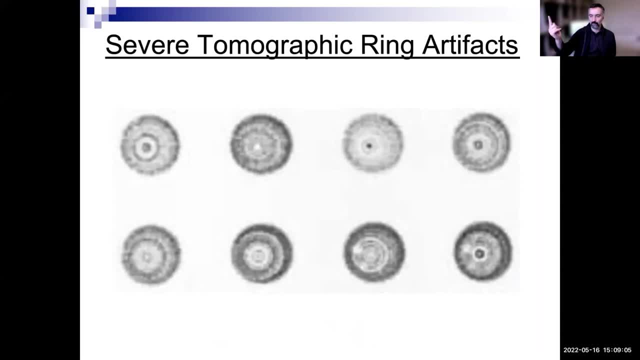 okay, and also in tomography, because you're rotating the camera, you're rotating the camera, you're rotating the camera if the camera is not properly rotating, if the camera is not properly rotating, if the camera is not properly rotating and it's not centered at the center of 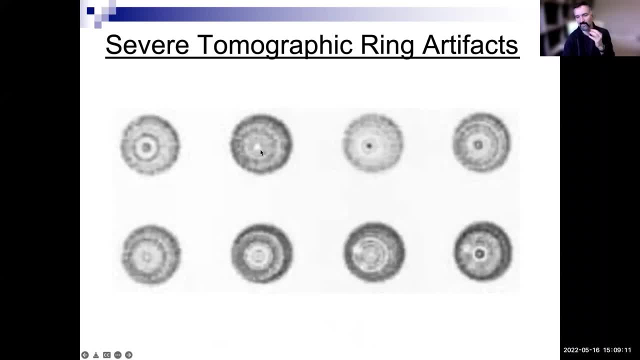 and it's not centered at the center of and it's not centered at the center of the image, the image, the image. the reconstruction is going to get all the reconstruction is going to get all the reconstruction is going to get all messed up on it, because the center of 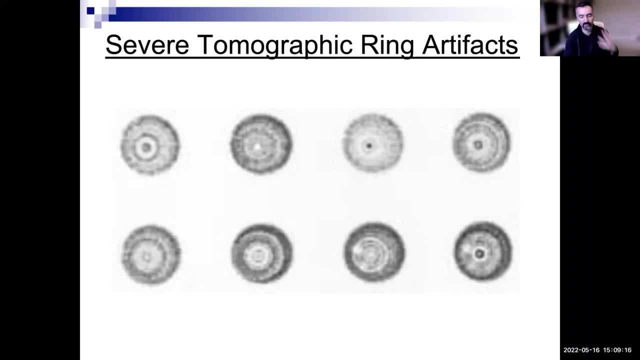 messed up on it because the center of messed up on it because the center of your rotation is not the center of the. your rotation is not the center of the, your rotation is not the center of the image, and things are being confused here. image and things are being confused here. 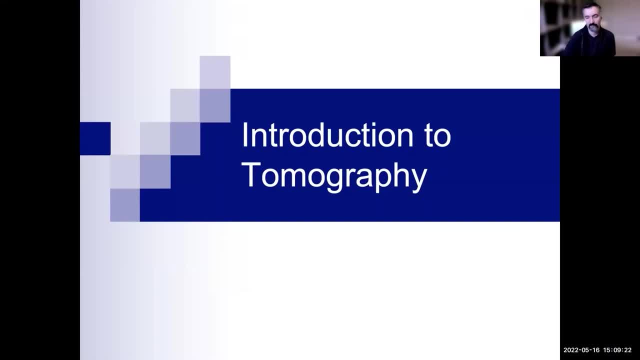 image and things are being confused here. any questions so far? no, no, no. okay, so let's talk about tomography time. okay, so let's talk about tomography time. okay, so let's talk about tomography time is very exciting, honestly, it's, it's um is very exciting, honestly, it's, it's um. 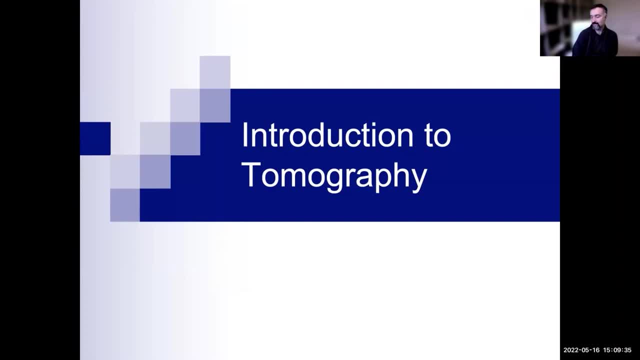 is very exciting. honestly, it's, it's um. it's just mind-blowing how tomography. it's just mind-blowing how tomography. it's just mind-blowing how tomography actually works- like today's actually works, like today's actually works, like today's. you know, medical imaging works based on. 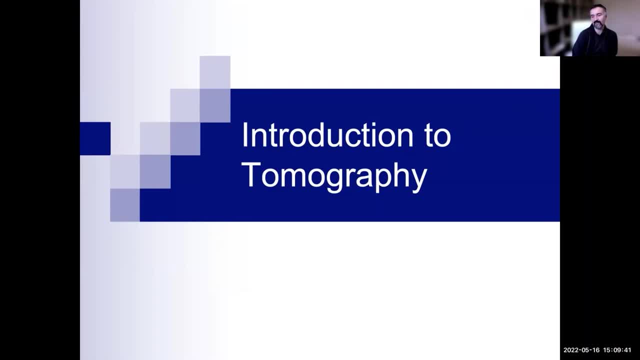 you know, medical imaging works based on. you know, medical imaging works based on tomography. the idea is tomography, the idea is tomography. the idea is: you're going to penetrate into the patient, you're going to penetrate into the patient, you're going to penetrate into the patient, right so? so tomography comes from the. 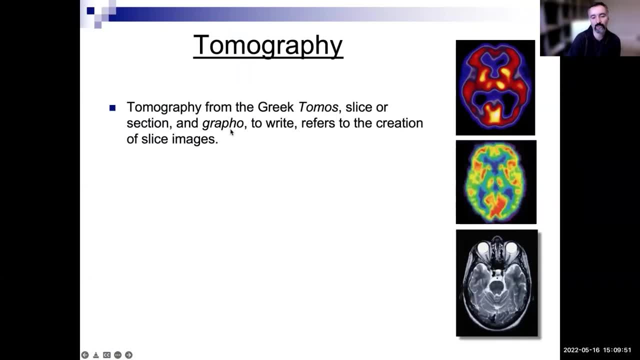 right. so so tomography comes from the right. so so tomography comes from. the greek tomos means to slice or section. greek tomos means to slice or section. greek tomos means to slice or section, and grapple, which is to write, and grapple, which is to write. 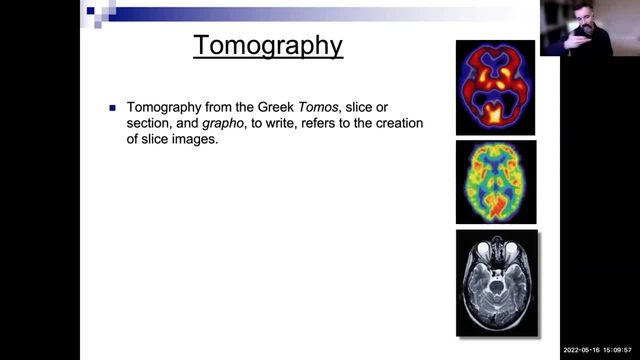 and grapple, which is to write, so you're writing, or you're creating, so you're writing, or you're creating. so you're writing, or you're creating slices, slices, slices of images, of images, of images through your patient, without actually through your patient, without actually through your patient, without actually slicing your patient. 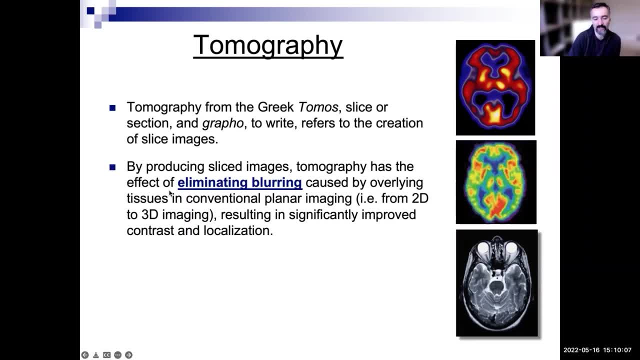 slicing your patient. slicing your patient by producing sliced images, tomography. by producing sliced images, tomography. by producing sliced images, tomography effect. uh has the effect of eliminating effect. uh has the effect of eliminating effect. uh has the effect of eliminating blaring, otherwise you're getting a projection, and so all. 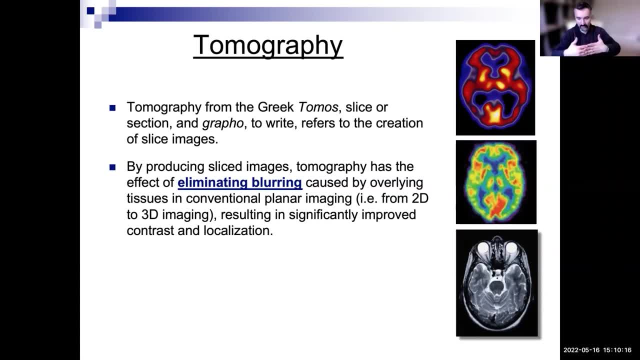 you're getting a projection, and so all you're getting a projection, and so all the layers of your body are adding. the layers of your body are adding. the layers of your body are adding together to give you a signal so you get together to give you a signal, so you get. 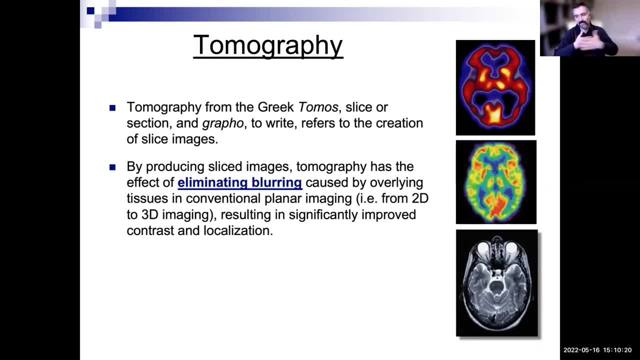 together to give you a signal. so you get a 2d planar projection, but that's a 2d planar projection, but that's a 2d planar projection, but that's doesn't that has significant blaring, doesn't that has significant blaring? 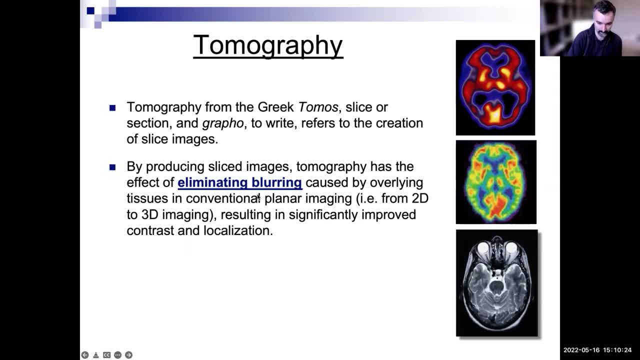 doesn't? that has significant blaring, because you're not resolving the, because you're not resolving the, because you're not resolving the different planes, different planes, different planes- and that's of course going to give you, and that's of course going to give you, and that's of course going to give you better contrast and localization. you. 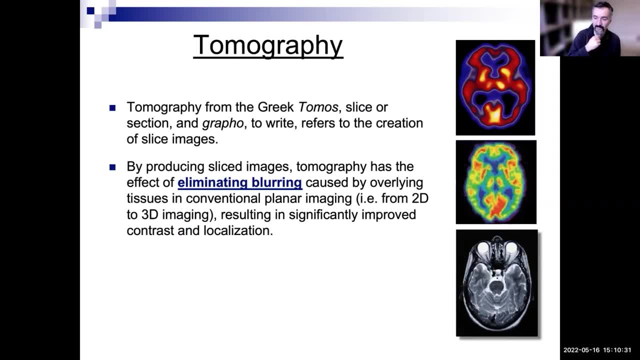 better contrast and localization. you better contrast and localization. you know where the tumor is. you know where. know where the tumor is. you know where. know where the tumor is. you know where the, the, the myocardial. you know defect is myocardial. you know defect is myocardial. you know defect is perfusion, defect is, etc. 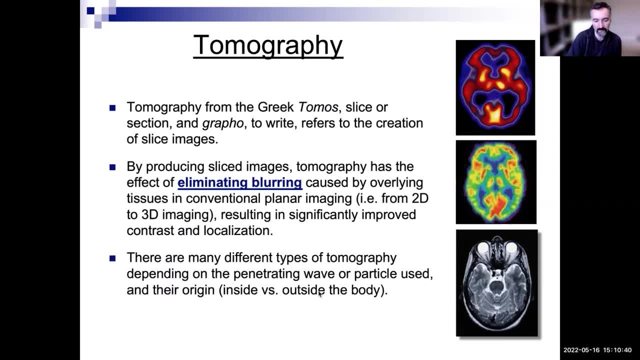 perfusion defect is, etc. perfusion defect is, etc. there are many different types of. there are many different types of. there are many different types of tomography, depending on tomography, depending on tomography, depending on what is used- is it waves? what is used, is it waves? 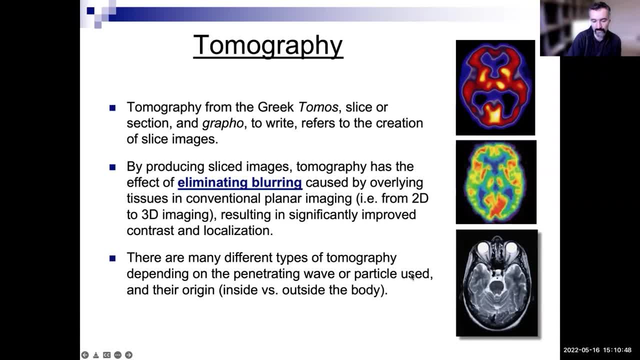 what is used? is it waves that are being used to image or that are being used to image or that are being used to image, or particles that are being used to image, particles that are being used to image, particles that are being used to image, and also their origin? whether? 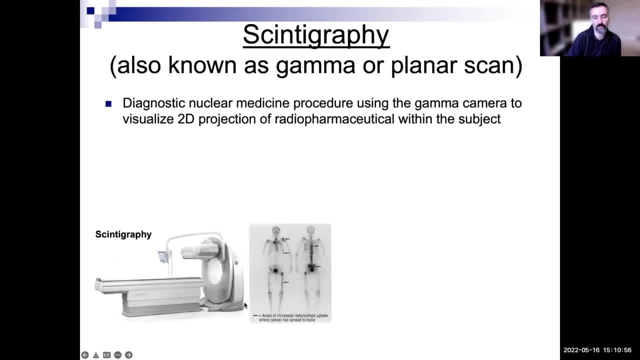 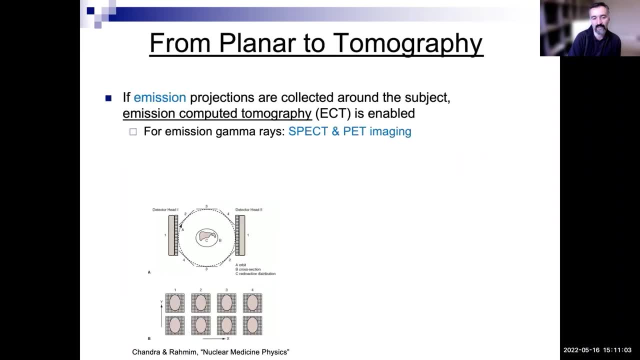 and also their origin, whether you know, for example, the waves, the signals coming from inside the body or outside the body, which we've alluded to before. so we already mentioned these before. we mentioned scintigraphy is analogous to x-ray radiography and when you go to planar- we showed this before- and you're rotating around. 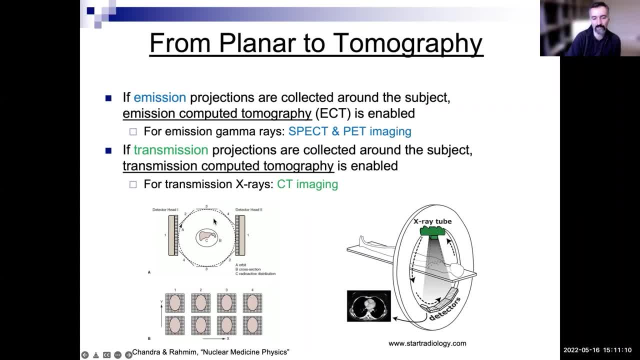 the sorry when you go from planar to tomography, when you're rotating around the subject you're. if the source is x-ray, transmission x-ray- we call that ct. if the source is emissions coming from inside the body, gamma rays, then we call that spec and pet image. now people often think that ct. 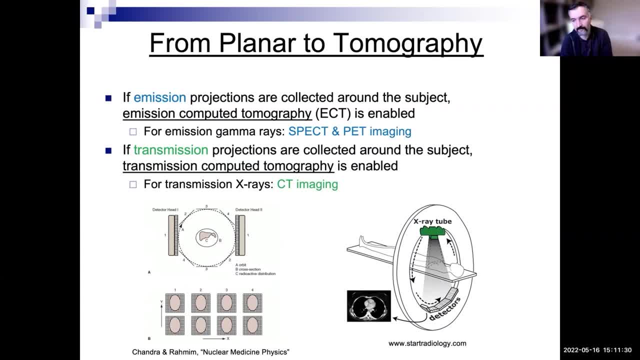 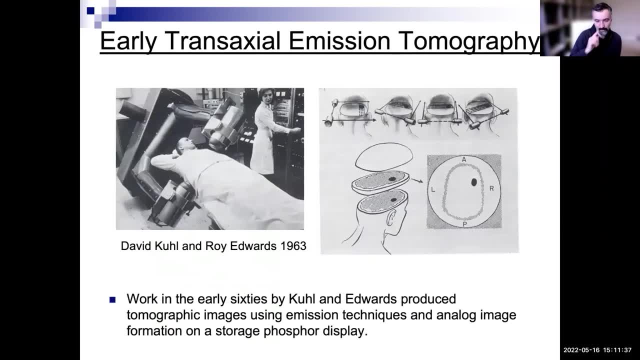 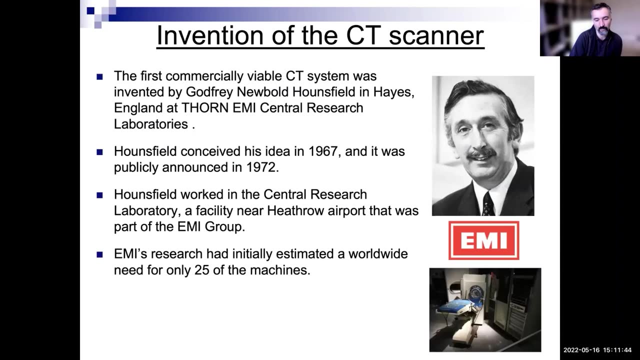 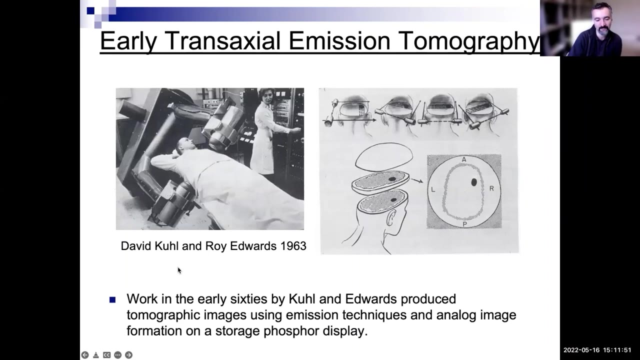 came ct. you know x-ray tomography came before nuclear medicine tomography. but that's actually not true it's. it's quite impressive that in 1963, well over a decade before uh, or nine years before the first uh ct scanner was publicly announced. 1972 in 1963, uh, david cole and roy edwards, they invented tomography in emission tomography. so 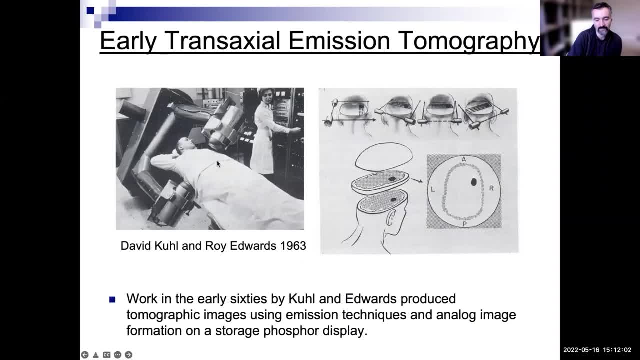 this is a patient who's been injected with radioactivity, i suppose. uh, so this is early 60s here. and they said: well, we got detectors, let's rotate the detectors around the patient now, back then they didn't know how best to reconstruct, so they did the simplest. 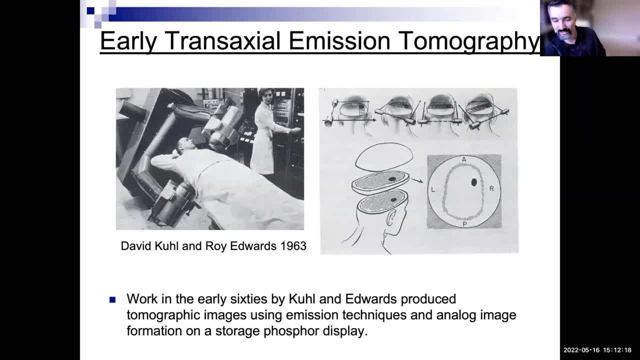 imaginable reconstruction, which is back projection. it's not the best. it's going to be quite blurred, it's not as good as filter back projection, but it's backward. it works to some extent. uh, so they did it. they, they invented this, but i don't think people took much. 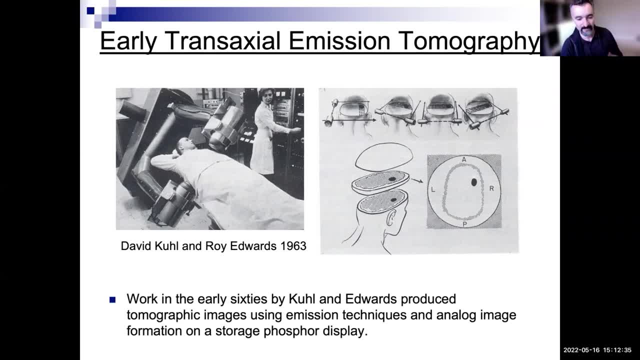 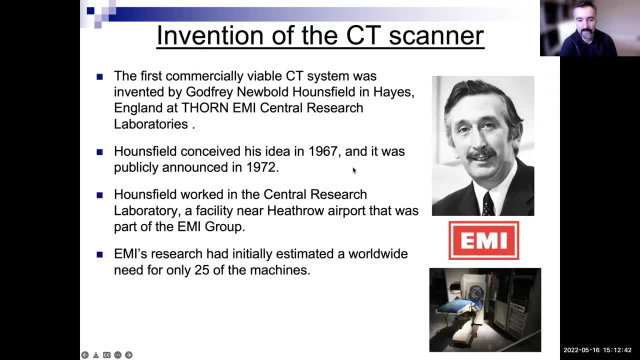 notice. so actually emission tomography, nuclear medicine tomography, showed up before ct did, but ct really ended up having more popularity early on. um, you know, uh, sarah godfrey- godfrey hounsfield of course- invented this. he was sort of in this research arm of the emi. emi was the company. 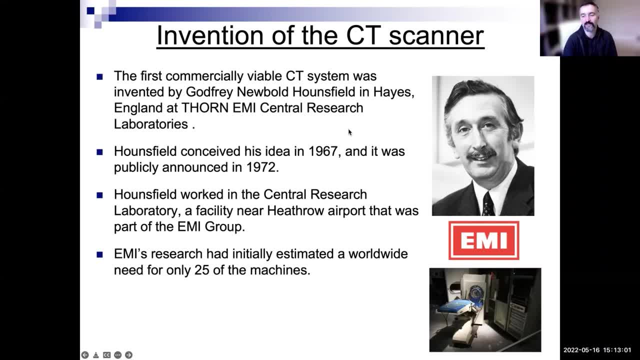 associated with the beatles, for example, amongst many other records, and they had some funds, as you know, allocated for research. so he kind of he thought of this idea in 1967, took him five years to publicly announce it. um initial estimate was that the entire world may need maybe about 25 of 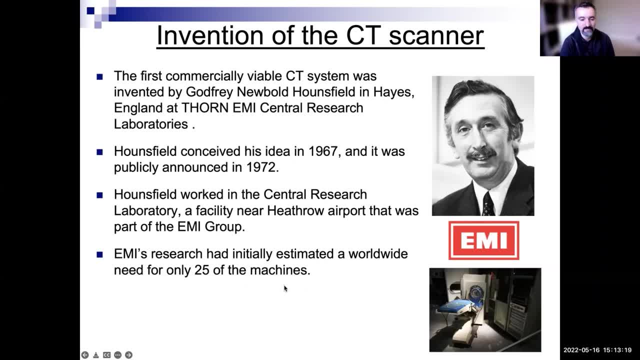 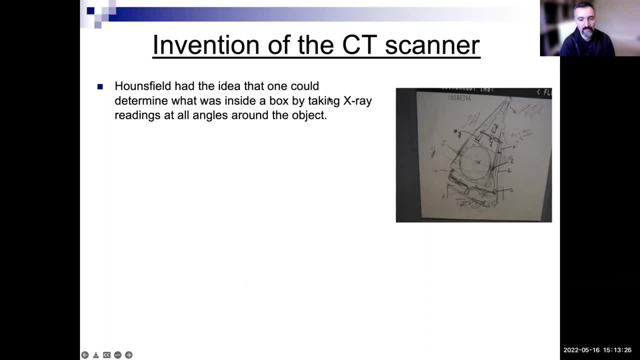 these machines and of course, that's. that's um. that has changed. so he had this idea that you could determine what's inside a box by taking x-rays at all angles around it, which is tomography. you shine x-rays through it. you don't know where in the box the attenuation is occurring if you just look at one direction. 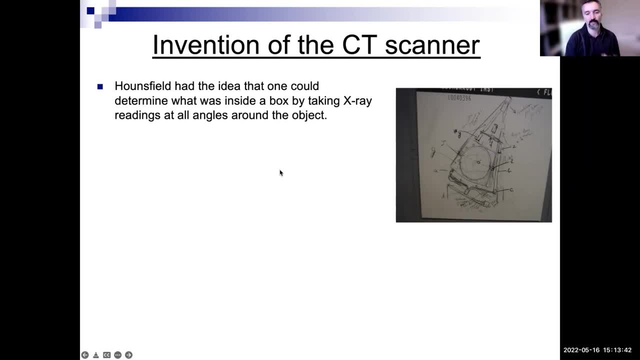 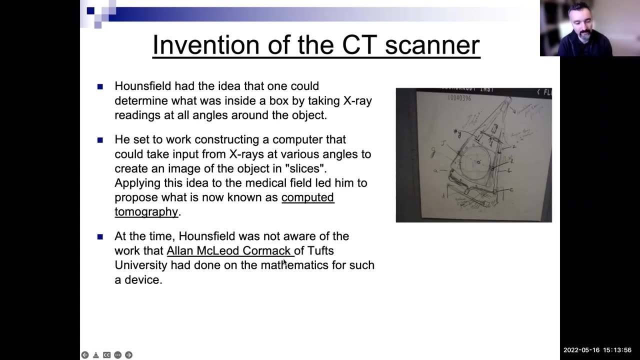 but once you go around all directions you're going to be able to resolve it using a, you know, tomographic reconstruction, for example. so he called this computer tomography right and turns out there was this other guy, alan cormack. he sort of had similar ideas and he wrote, i think, a couple of papers sort of saying this: 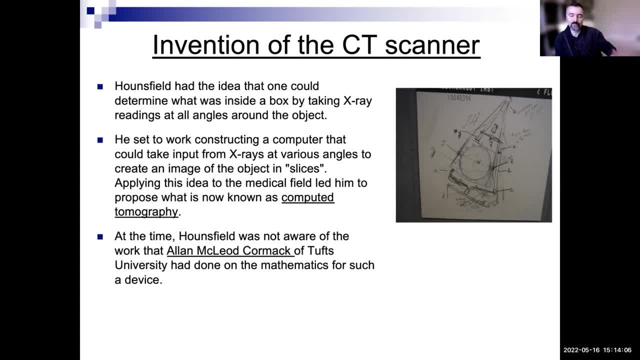 but nobody really noticed, took notice of it. he kind of developed the idea, moved on to other things and um, and turns out, decades earlier this guy called radon had also conceived of these ideas anyhow. so so so poundsfield develops this and then people realize, oh, cormac is also saying the. 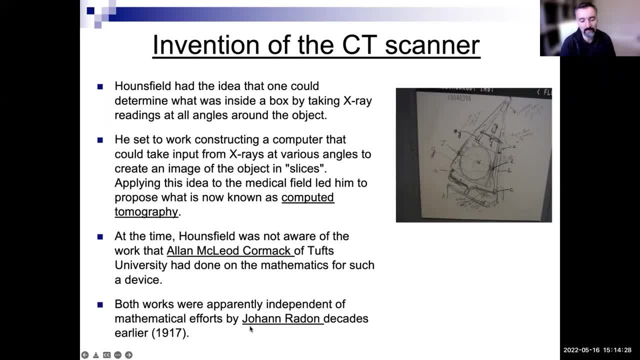 same thing along the same time, but then again radon, and had had also thought of these decades earlier. therefore, we call the projection operation the radon transform, when you take an image and sum it all along rays to see what the x-ray image or the gamma ray image, uh, looks like. but these 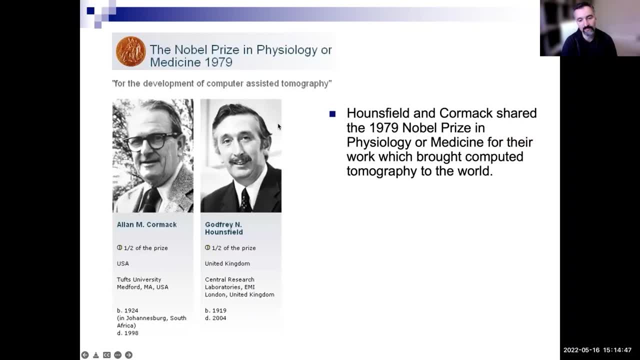 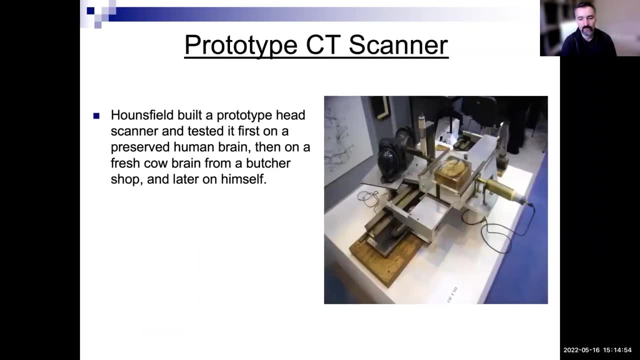 two individuals. um won the nobel prize in 1979.. um, and yeah, so, um. so there's some prototype where you know studies on preserved human brain, then a fresh cow brain from a butcher shop, and later he also imaged himself, and these are the. 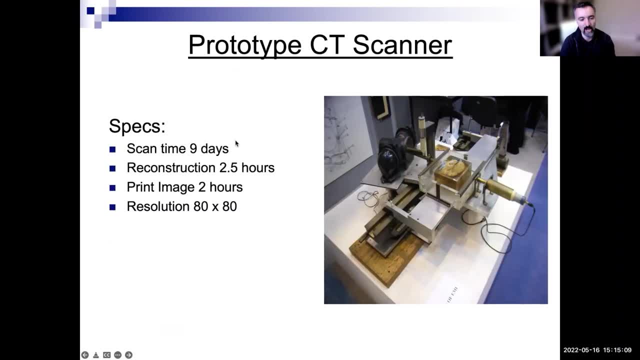 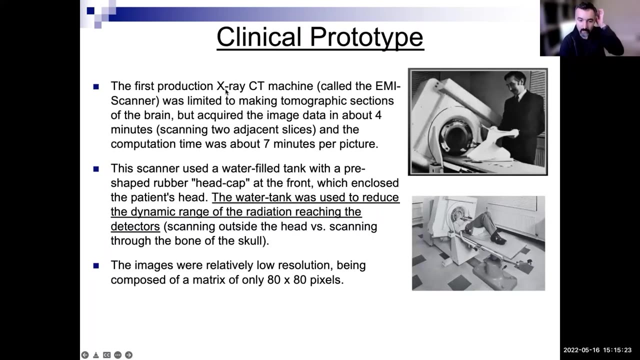 kind of images they were originally getting. scanning time was nine days on some of these samples. reconstruction was many, many hours, or at least a couple hours here. uh, there were printing images. resolutions were not so grand, but it's great. but you know, and then, um, you know, uh, when this was constructed it took about four. 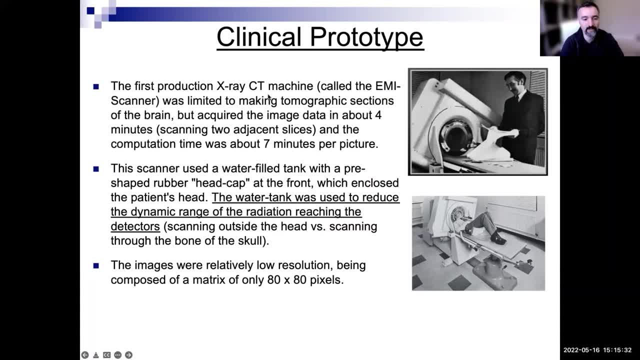 minutes, ultimately, uh, at about seven minutes per picture. when you, when they built the actual clinical prototype, i think in 1972 or soon after he announced and they had to do stuff in there, like they had to have a water tank because, um, they had a big dynamic range, like from parts of 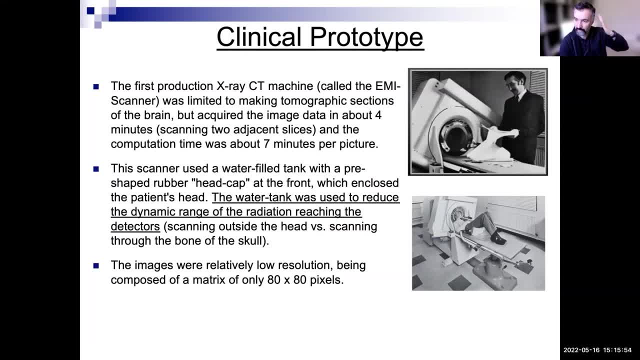 the brain, because the there's smaller intersection with the brain, you would get much less attenuation, whereas here you get much more attenuation. so the range of numbers they would get on detectors were very different. so they, the the detectors, couldn't handle so much difference, so much dynamic range, so they actually use a water tank to kind of make everything almost equally. 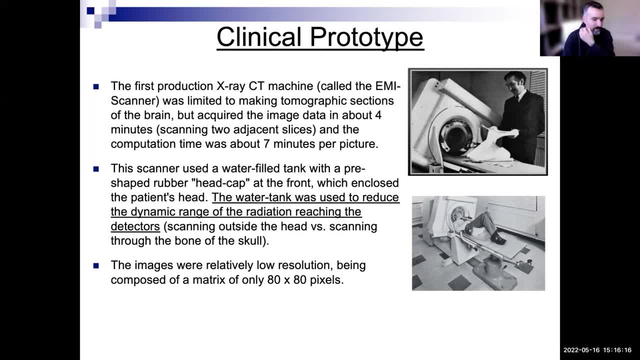 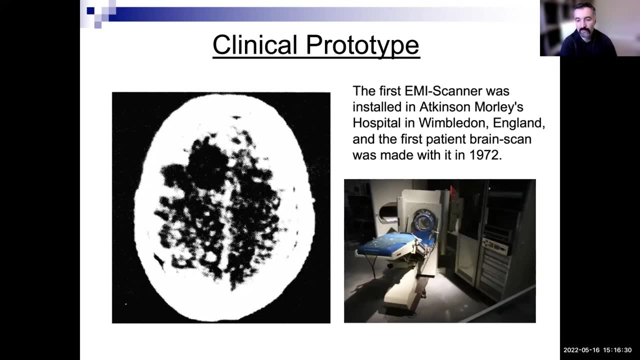 in terms of equal in terms of amount of transmission. we don't do this, of course. now these detectors are much better, they can handle these differences in the range of numbers that we get much better, okay, so so the first uh patient brain scan was was made in 1972 and, of course, to commemorate him, 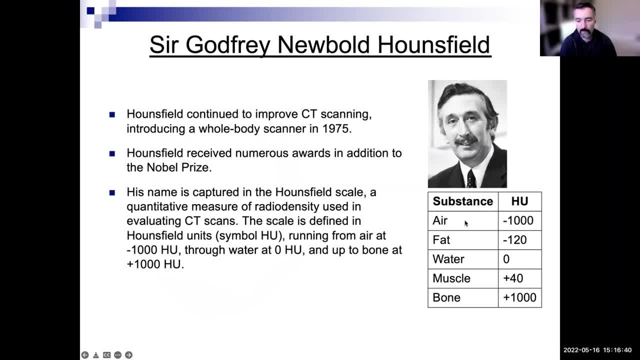 uh, and, by the way, whole body scan in 1975 to commemorate him, the hansfield units are used and i know, you know it was like the water, the number is zero. hansfield units, that air bone, etc. etc. um, so back to back to, and i don't want to say forward. 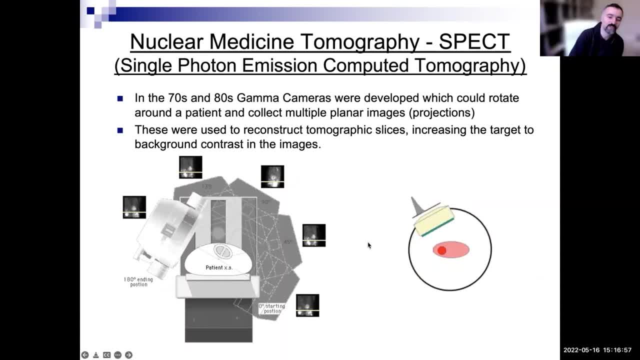 to put back to, because emission tomography was actually constructed in 1963, as we saw. but then later this was revisited in the 70s and 80s, probably energized by the role of ct, because there's always interactions between the scientific disciplines, right? so people started taking this. 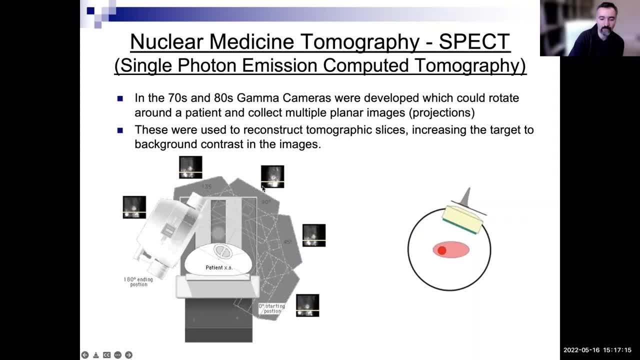 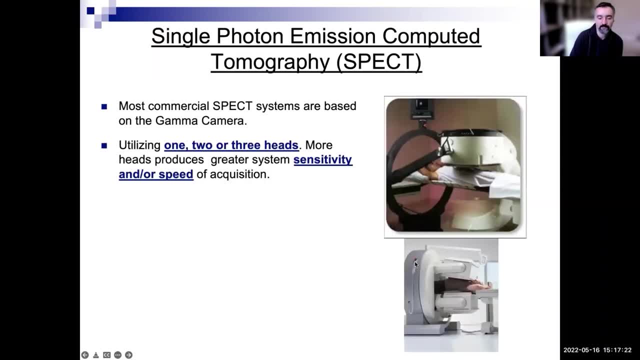 quite more seriously, rotating the gamma camera around the patient, as you can sort of see here, and using image reconstruction, so you could have a single head rotating around the patient or dual heads working on the patient, or even have triple heads like one, two, three rotating on the patient. so the 2d planar images. 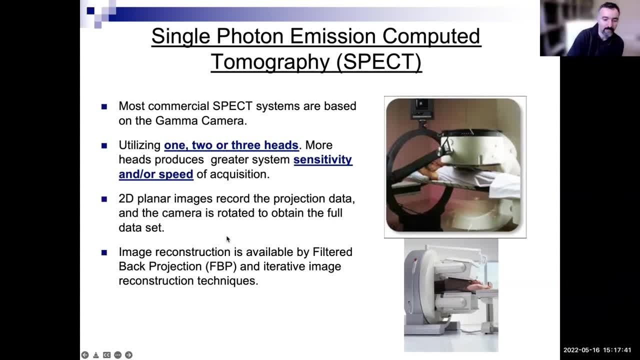 get the projection data and the camera is rotated and image reconstruction can be done either using so-called filter back projection, which is a pretty good uh technique, or iterative image reconstruction, which is even better, and nowadays people are talking about artificial intelligence based recons that assist these. 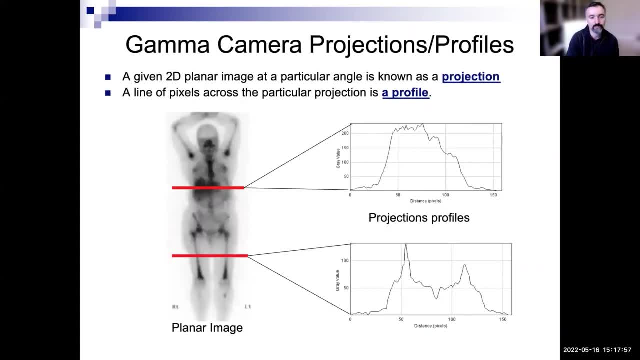 methods. um, so yeah, so this is a projection of the patient. we call this a 2d planar image at a particular angle. so therefore a projection and then a line of pixels along this particular projection. we call that a profile, so there's a profile through the. 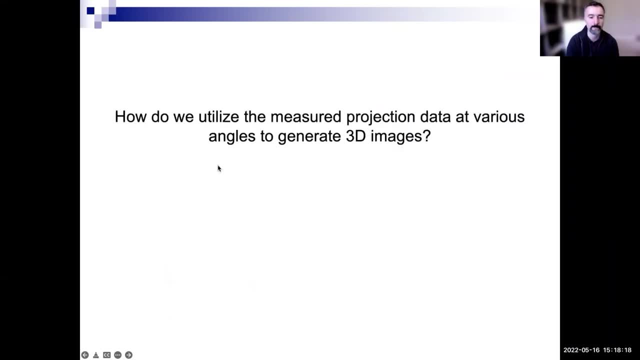 patient. remember we rotate. we're going to be rotating around this patient. so how do we utilize the measure projection data at various angles to generate 3d images? that's the question. i got a whole bunch of his intuition and their intuition was: if you rotate around the patient, you know. 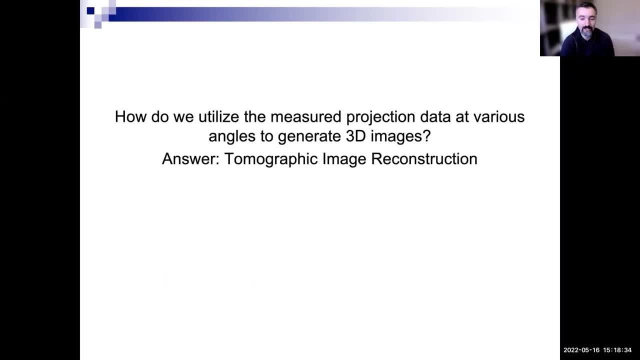 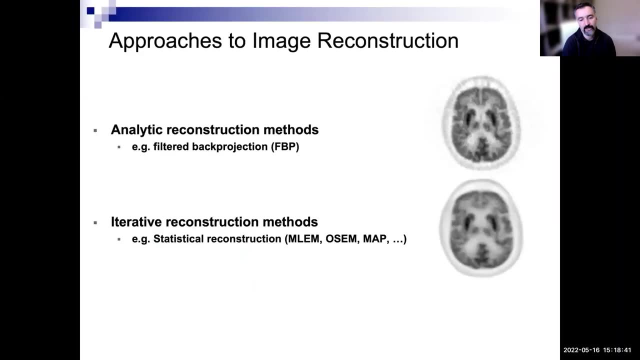 what's going on inside the box. well, how do you actually do it? and that is a beautiful feel of tonographic image reconstruction. okay, so there are a number of approaches to image recon. there are analytic techniques. you might have you heard these in in the world of ct. 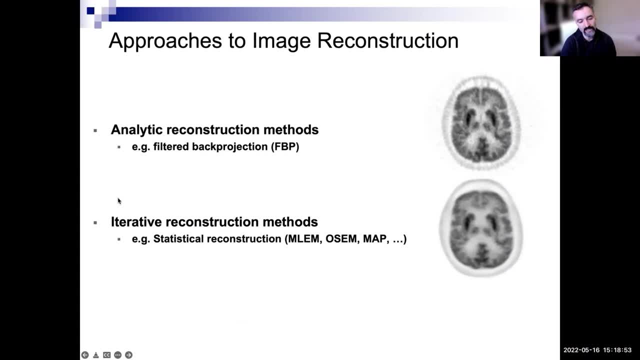 also, and there's iterative techniques. so the world of ct is only in recent years really coming to iterative techniques, that it used to really be focused almost purely on filterback projection in clinical routine. but in our world, the world of nuclear medicine imaging, we switched quite a. 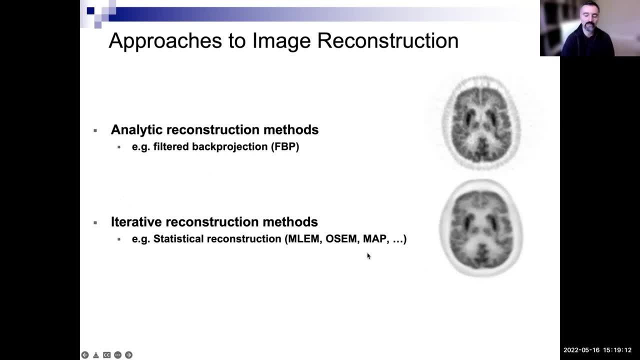 while ago, long time ago actually, to iterative methods. one reason was because because the signal in in nuclear medicine imaging is coming from inside the body, we cannot be injecting too much into our patients and therefore there's the images can be noisier, unlike ct where you suddenly give a. 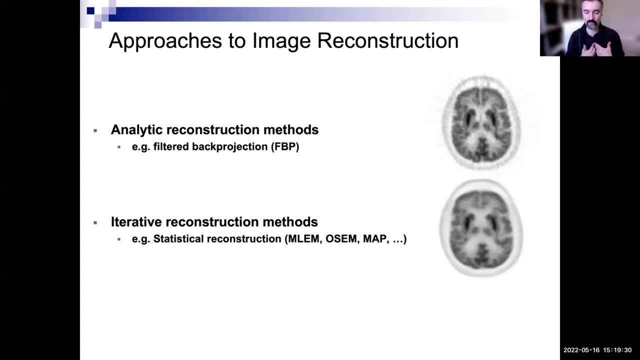 massive dose or relatively large dose, and then you stop. you cannot do that in our field. it's already inside your body. you can't stop that radiation, so you gotta give it a limited amount. so we we have been dealing in nuclear medicine with uh noisy images and we just know that we have to switch. 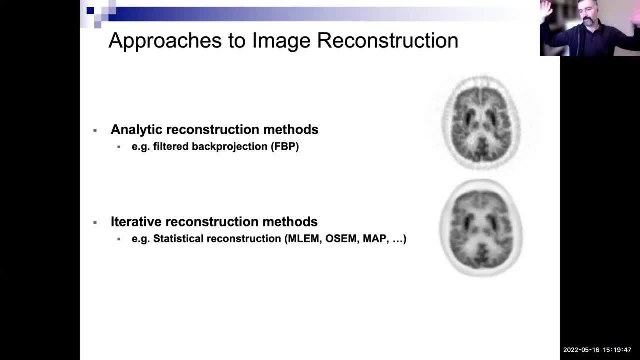 to iterative methods, then the world of ct. initially they were like: well, this is already good enough. but now they're thinking: well, why, why are we? why? why can't we just inject our patients? or sorry, in the world of ct, why can't we just giving you much, much less doses? because the public's mind has been activated. 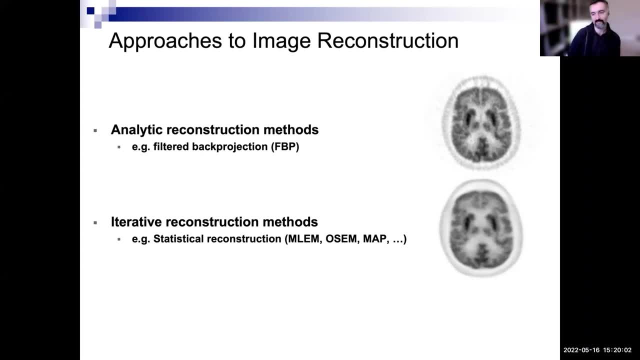 they're like: why are you dozing us too much, can you not dose us less, etc. etc. the answer is yeah. if you do iterative recon, you could actually achieve um very good images, and nowadays people talk about ai, driven ai based artificial intelligence based recon that you could get. 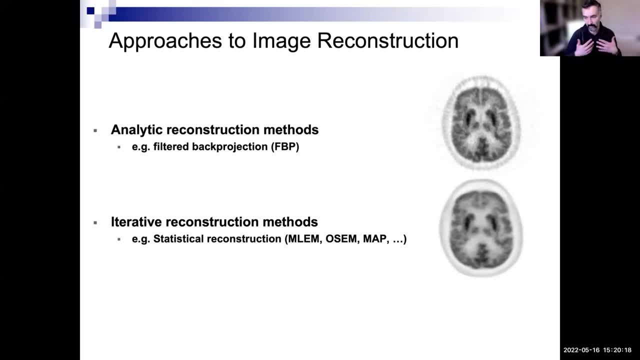 significantly less injected radioactive- radioactivity in our field- and also inject, you know, beam doses to patients in ct and get very high quality images. um, so we got again. you got analytic methods and we got iterative methods. iterative methods- a big part of that is statistical methods. i just want to mention, though, that not all. 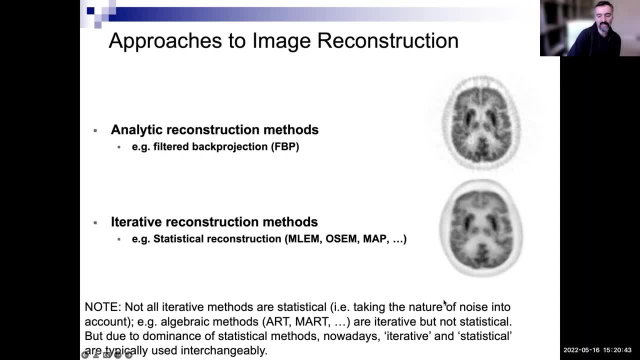 iterative methods are statistical. statistical means that you understand the noise pattern and the structure. you take that into account. there are some other methods, like algebraic methods, that are iterative. they go in a loop but they're not smart enough to think in terms of the nature of 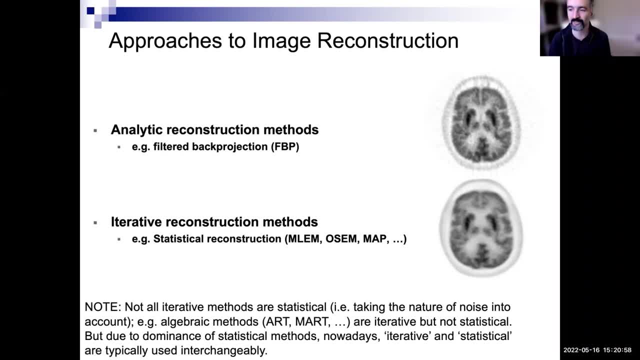 noise. they're like: i'm just going to solve this, i don't want to think about this. is gaussian noise, poisson noise? i don't care, i'm just going to solve this. so that's why i think iterative statistical recall methods are are in in what we're presenting here, have demonstrated added. 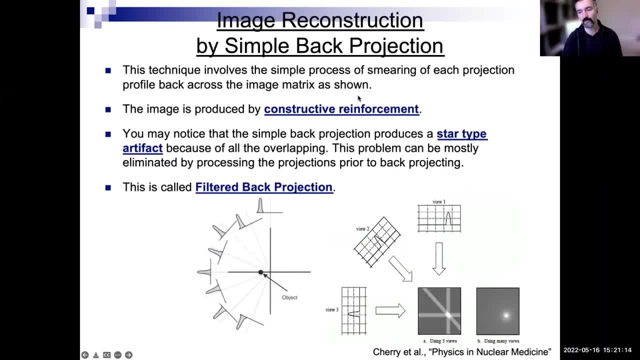 value. um so simple back projection. remember that original uh device i was built in emission tomography- simple back projection. so how does it work? all you do is, as you're rotating around your patient, imagine you got a point source. this point source is going to show in this: 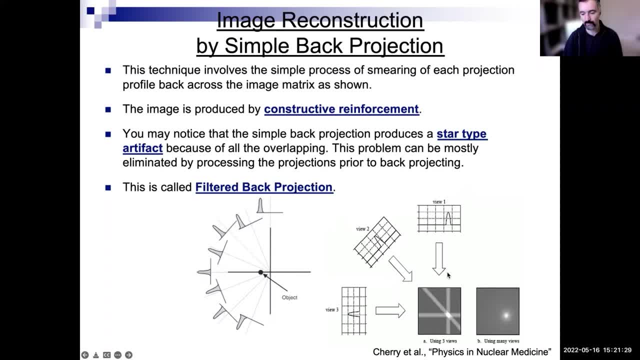 projection here, in this one, here, here, here. all you do is you back project all these from all these angles. when you back project, you're going to get this. this is a reconstructed point source- notice how it's blared, because you're, you're really um, there's a lot of uncertainty. 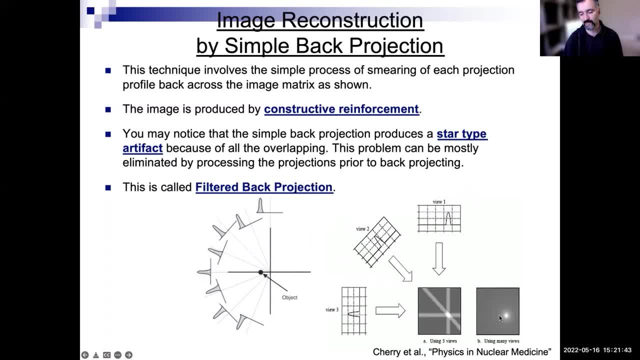 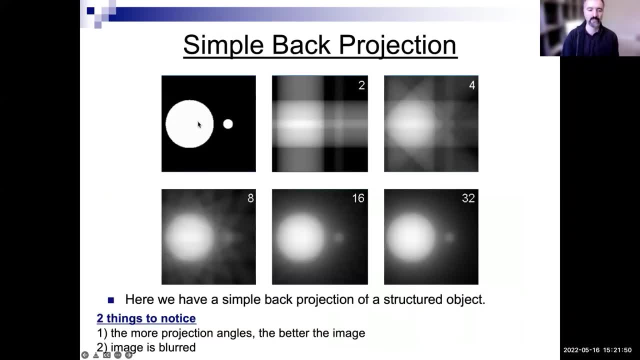 your back projection is going to show. in this projection here, in this one here, here, here, back projecting. there's a lot of signal here that is in the wrong place. you're not doing any filtering, so you end up with something that is like blared. here's an example: um, this is the 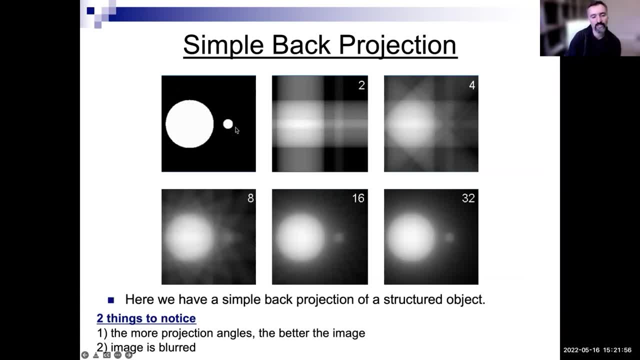 original image. if you do only two projections, let's say along this direction and along this direction you back project them. this is the image you're going to get. terrible. if you do along four angles, this is the image you get: eight, sixteen, thirty two. so this may look good to you, but it's. 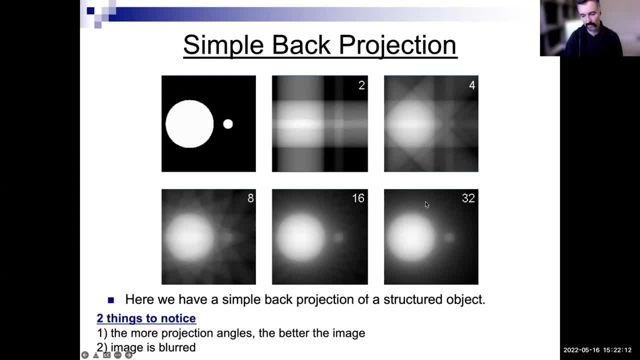 really not that good. when you think about it, the contrast between the two is going to be really not that good. when you think about it, the contrast between the two is going to be not great. you have all this kind of spill spill out, if you want to call it. of course, the more 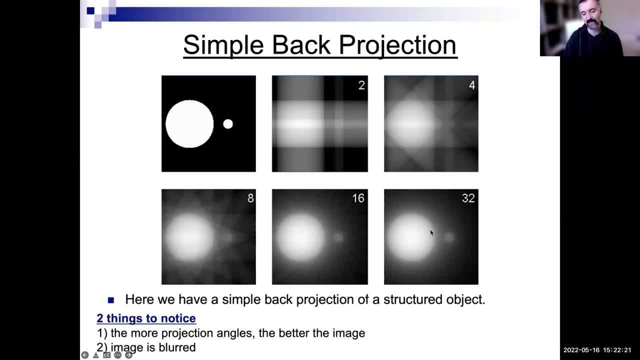 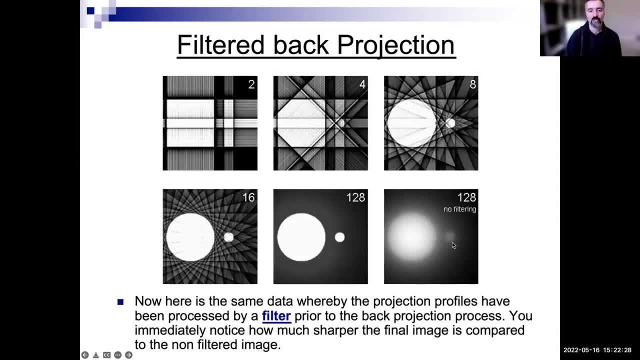 projection angles are better in the image, but the image still, even at this angle, at this so many angles- 32, 64, 120- it's going to be blurred. so filter back projection and let's not talk about filtering what it means yet, but just stuck to it, which is informed, which is very intelligent. 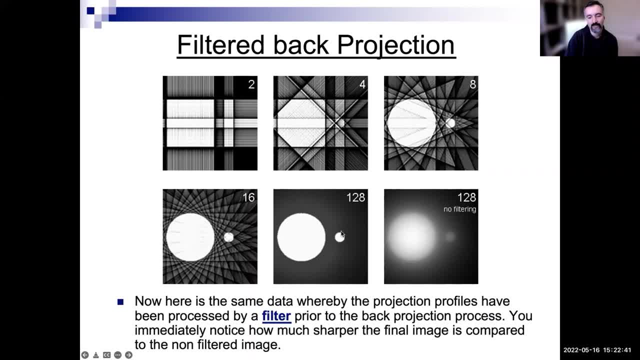 and you actually end up with this. look how filter back projection is much better than non-filtered back projection, just simple back projection. see how blurred it is, as we were showing before. before we were showing for 32, but even 128 angles does not look great, whereas with filter back projection, sure you see a little. 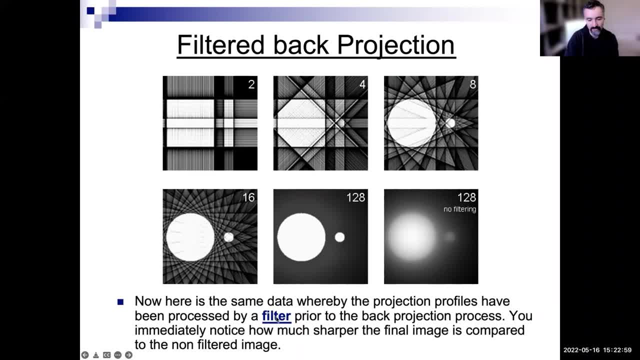 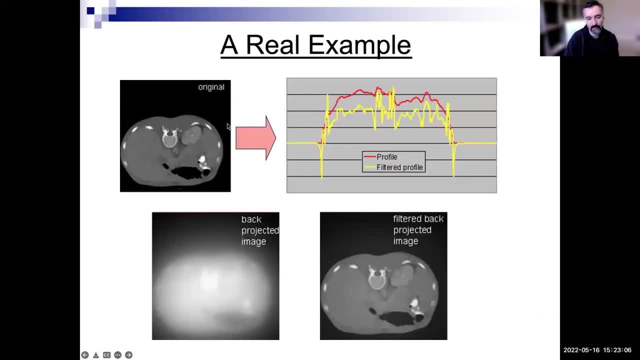 bit of artifacts here and there, but it's much, much better than this. there is this magic filter that gives you much better images. here's another example of a you know an example of a patient and you can see that the back projection image looks awful. filter back projection looks quite better. 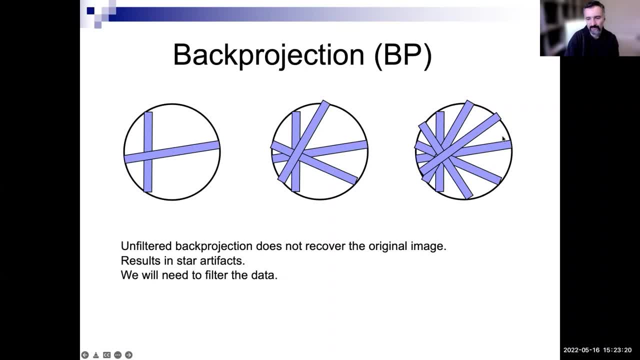 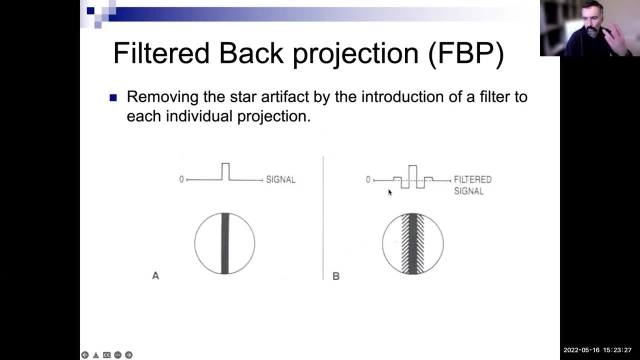 so, yeah, back projection, you just back project everything, but again the signal is not filtered. it's messy filter by projection says no, no, i'm not going to back project this. i'm first going to do some weird filtering which is, in form, intelligent. there's a lot of beautiful math behind this. 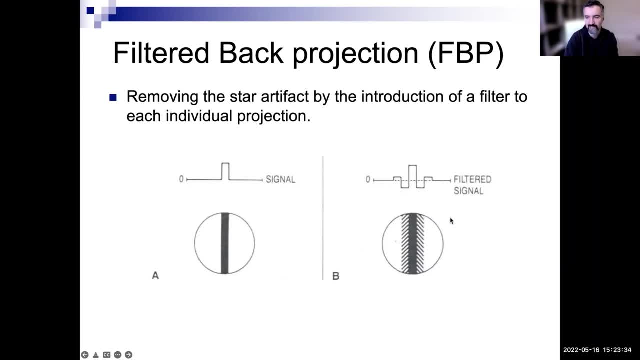 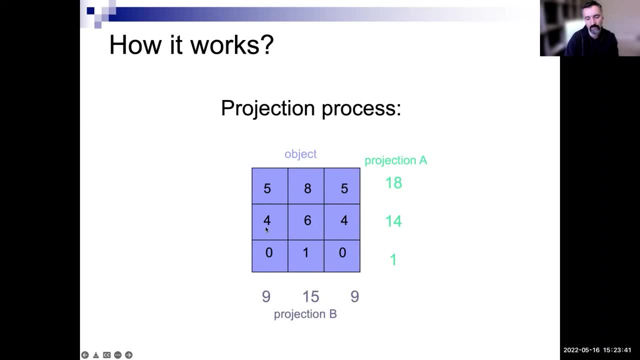 and then i'm going to back. but you know this looks weird, like why would you ever do that? but it turns out it's a good idea. so just to give you an example, you've got a box of numbers. imagine this is your patient and three by three, grid you forward, project this patient, you get the. 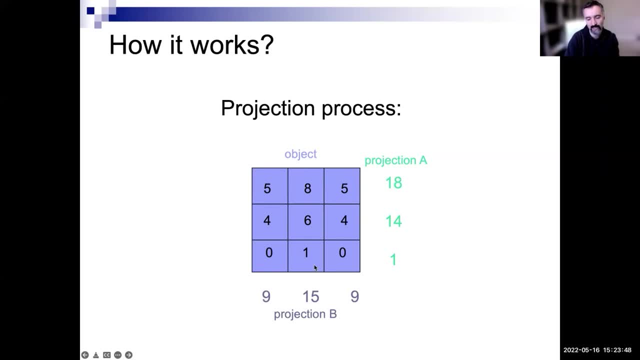 total of 18 counts here forward. project 14 counts for project one. four, project nine, fifteen, nine, from these two sets of numbers, imagine like two angles of projection, x-rays, for example. you wanna, or you know, emission scans, camera scans. you want to reconstruct this if you back project the. 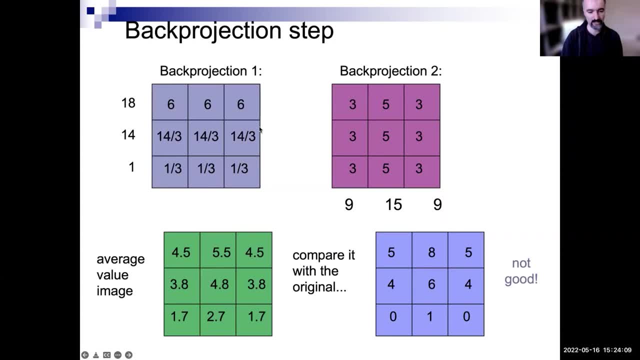 numbers: the 18 gets equally split between these. 14 gets equally split. one equally split. same with these three. you add them up. these are the images you get. so sorry, uh, what was that? yeah, this is the original image. this is the new image you get by adding all these. doesn't look that great, this. 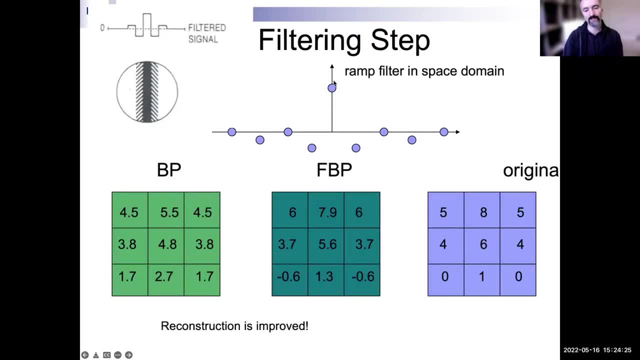 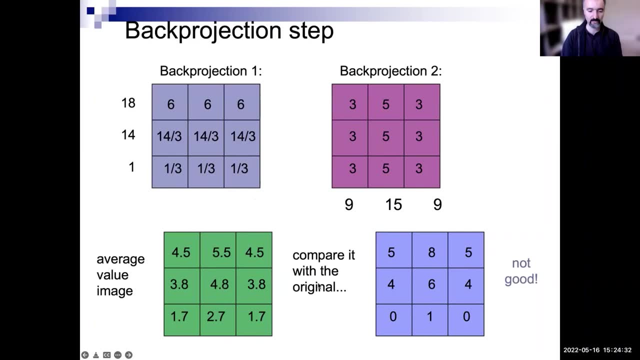 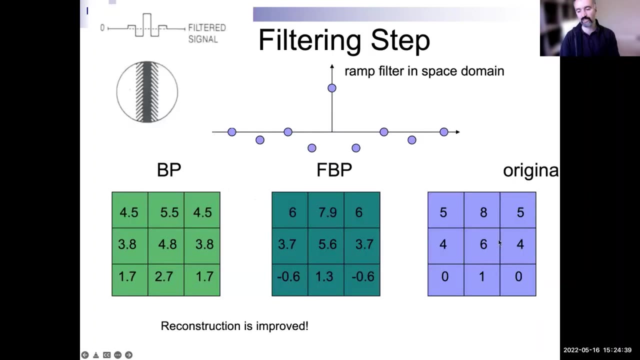 six has become 4.8. but if we do this filtering step first, then back project, filtering sec, then then back project, these are numbers we're going to get. look how the center which did correct value, true value being six, in back projection it became 4.8, but here in back projection is 5.6, which is 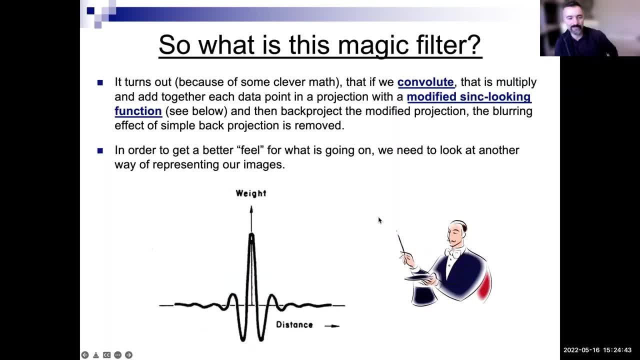 quite closer to six, so it's better. so what is this magic filter? turns out because of some clever math that, if you convolute right, uh, that is simply add and multiply together each data point in a projection with this sync looking function, which looks like this: we first convolute these profiles. 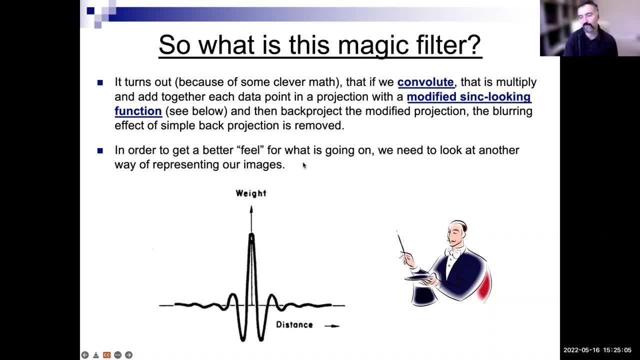 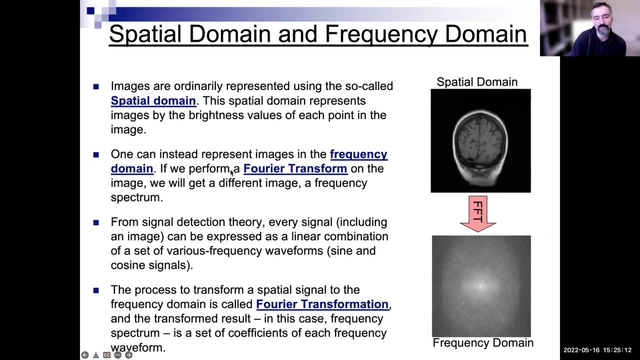 and then back project them. it turns out mathematically you can show that in a perfect scenario you're going to get the original image back, okay, so, um, there's a bit of uh. what does this thing even mean? what is this sync filter that you have to do? this takes us to the domain of frequency domain, a strange, bizarre domain, lovely. 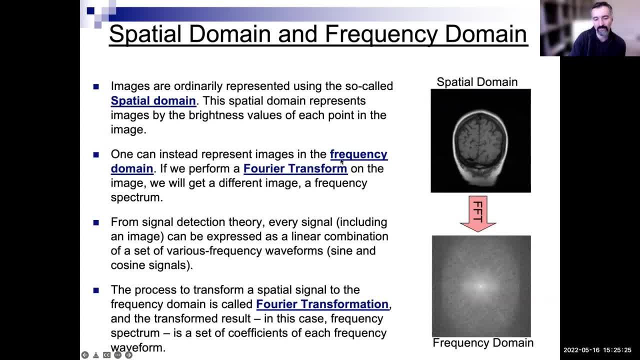 domain you know fourier transforms. you might have heard of mr fourier initially when he said these people couldn't believe what he was talking about. but basically you can represent any signal, any image in 1d, 2d, 3d in a frequency transform domain. the center of this represents zero frequencies. 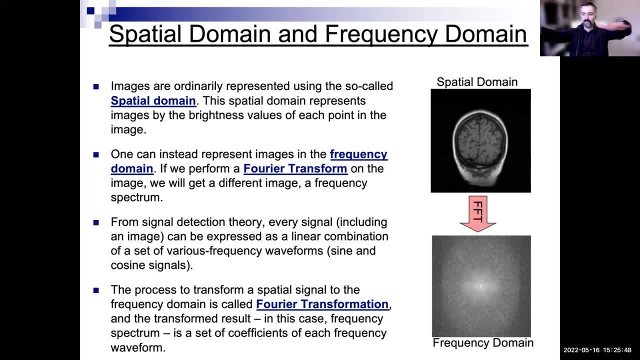 zero frequency means you've got like a dc offset, like a constant, and as you get away from the center this represents how much sinusoidal behavior of increasing frequencies you have. so you've got an image that has a lot of edges and a lot of you know quick movements in it, like sharp. 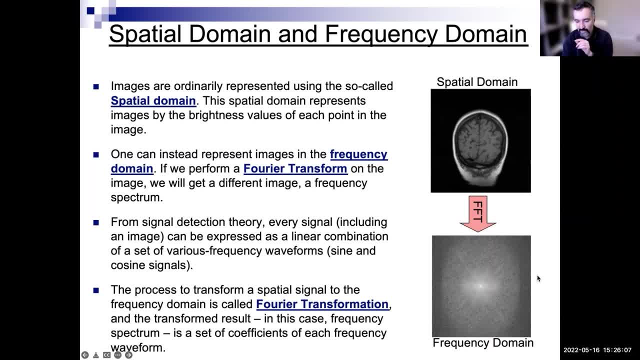 changes. you're going to get higher and higher frequency content as you move outside from this ring. but if you get a really constant image, a boring image with not much massive changes, you're gonna get a lot of concentration in the center and not much going on at the edges. so the process 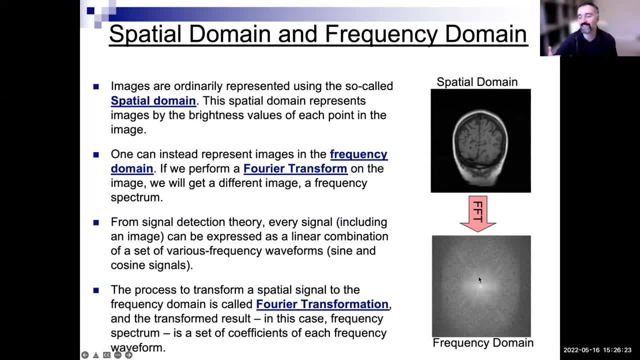 to transform an image into its equivalent sinusoidal frequency content is called a fourier transform. so it turns out, any image can be represented by a summation of a whole bunch of sinusoidal curves. which was a strange discovery about a four-year. okay, then it turns out just. 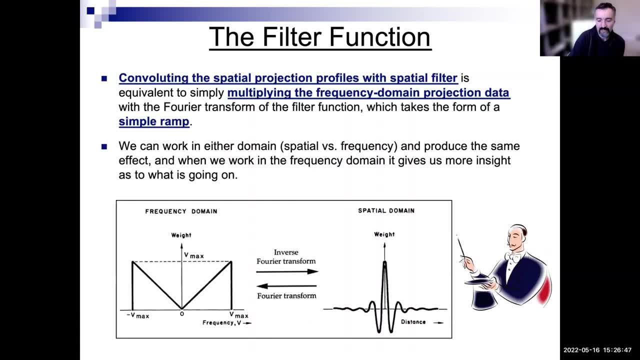 hanging there. this is probably the most difficult part of what i'm saying today. if you've got this thing, this sync function that mathematically you can show, you have to convolute your image with before you back project turns out in the frequency domain. it looks like this: 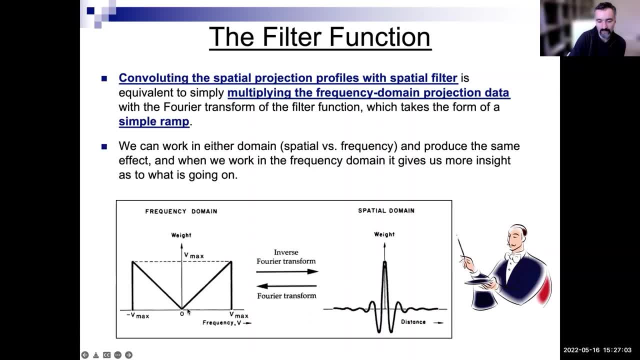 so this signal, the frequency domain, has no content at zero, but has a lot of content at a certain frequency. okay, so we call this is okay. so this is like a ramp filter- you might have heard of the term ramp- so the ideal uh filter in its frequency domain. 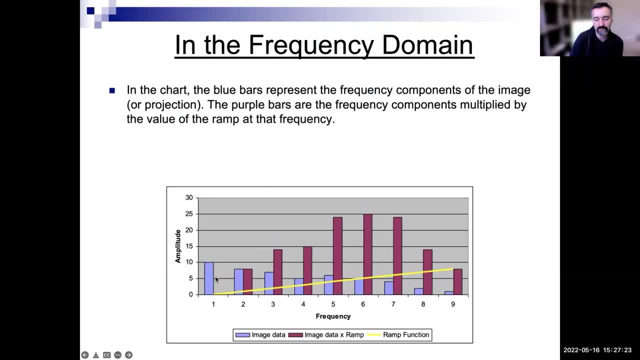 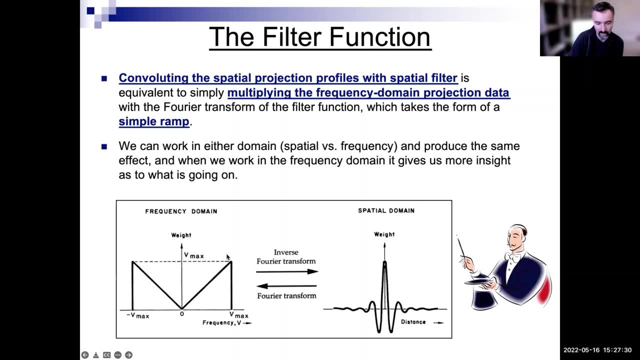 looks like a ramp. okay, now this ramp has a number of roles. look how it's basically saying- i'm going to really emphasize: add, aggregate to the higher frequency content and the lower frequency. it has an intuition. it says: in the projection operation, your device has been receiving these projections and killing high frequency content, like lowering. 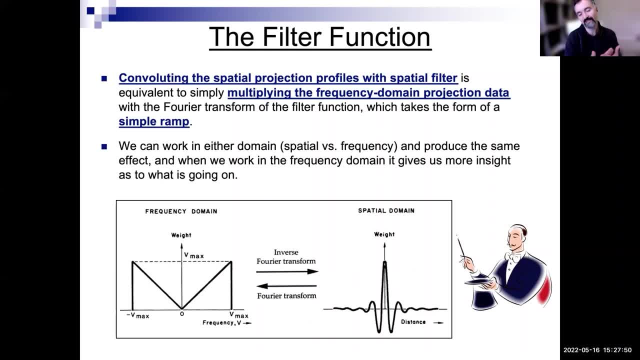 their impact because you're projecting. it's like saying: hey, you're projecting, you're killing me here, let me help you, let me amplify, let me undo some of the harm that this projection has done and bring up some of the frequency content. so you try to bring up, uh, some of the 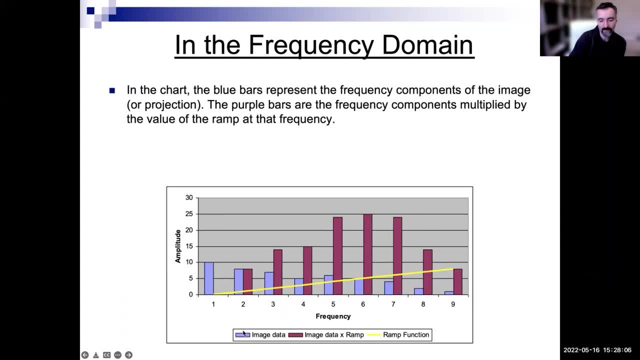 frequency content. so okay, so imagine this is your imaging data, but this isn't the frequency. like how much frequency content does your imaging data have? imagine that the um, this is, this is what you've actually measured in the projection operation. but the ramp filter says no, no, take your signal and actually 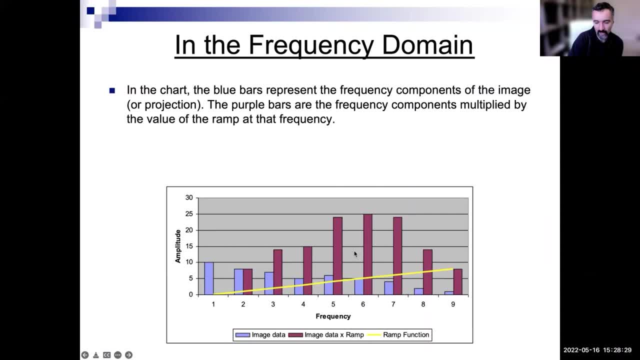 multiply it by me so i give you higher content in these frequencies. these are the mid-range frequency. the really high range frequencies tend to correspond to like things like noise, but the mid-range frequencies are real content. this is how the body looks. it has mid-range frequencies. 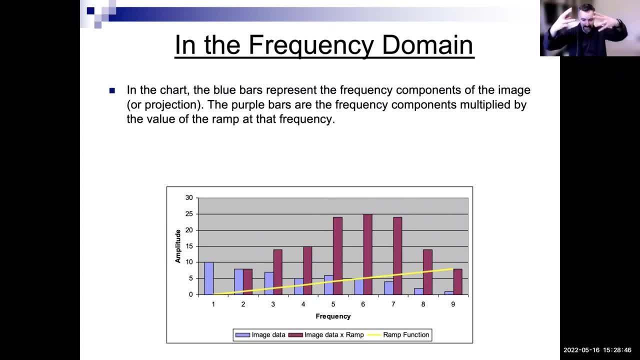 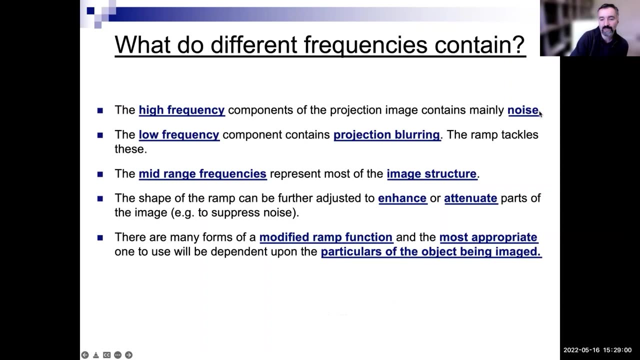 it's not just some boring flat structure. the body, the body has, has some frequency content and when you multiply your signal by this ramp filter, it brings out the best, it brings out the truth in it. okay, so the high frequency component, the really high frequent component, can contain mainly noise. 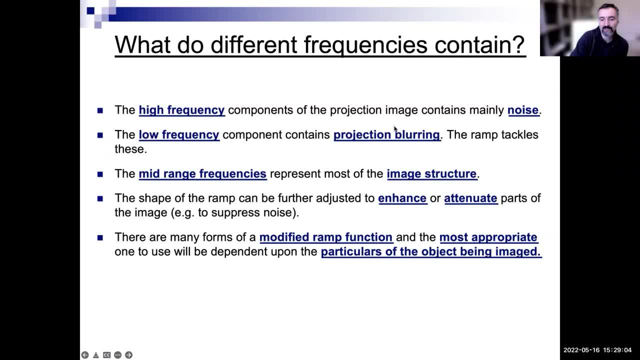 the low frequency content is the blaring noise content. the low frequency content is the blaring due to the projections. What we really want to emphasize and amplify is the mid frequency, mid range frequencies- okay, And the shape of the filter itself can be changed. 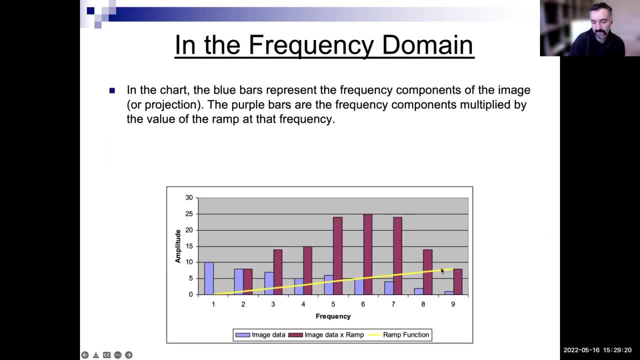 There's an ideal filter, but the truth is that this filter does suggest that as you get more and more signal here, I'm gonna amplify it more and more. but you don't really want that, because this stuff here is noise, So you may wanna even cut this part of the ramp. 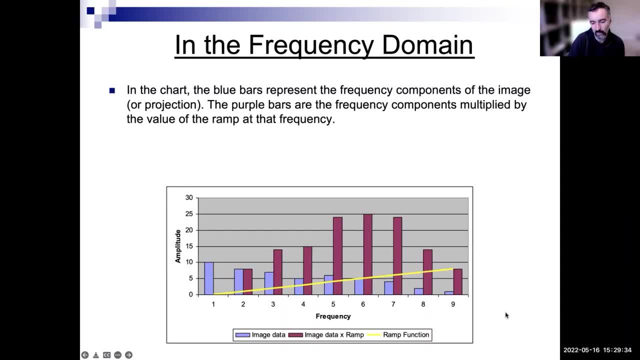 and say: you know what. You're going out of your way too much. My image is noisy. You're kind of clueless about the fact that my image is noisy. Don't amplify this part too much. Amplify this much more. 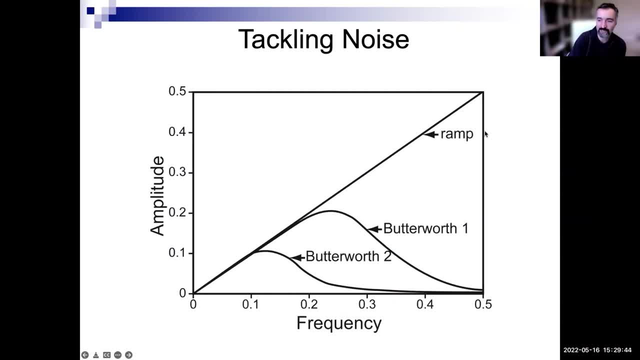 So that's why people switch from a ramp filter, which is great Theoretically. it's best if you have a noise free image, but we do have noisy images to begin with And therefore it can really amplify high frequency noise to modified versions of the ramp right. 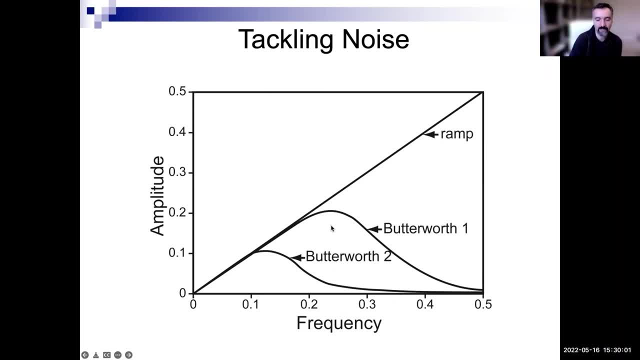 Since, like other kinds of filters that kind of amplify the mid range, So ramp looks like this. but we can end up with other things like this. We were just showing the Butterworth, different kinds of Butterworth hamming hand pars and different kinds of filters. 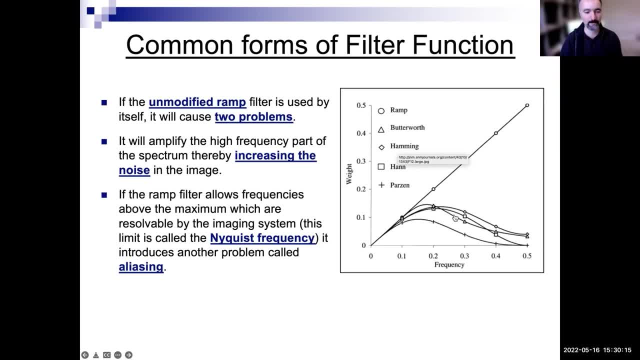 that kind of amplify the mid range frequencies, Cause we don't wanna amplify the noise, Okay, and if the ramp filter allows frequencies above the maximum which are resolvable in imaging system, it could even get aliasing stuff. So you really don't want filters. 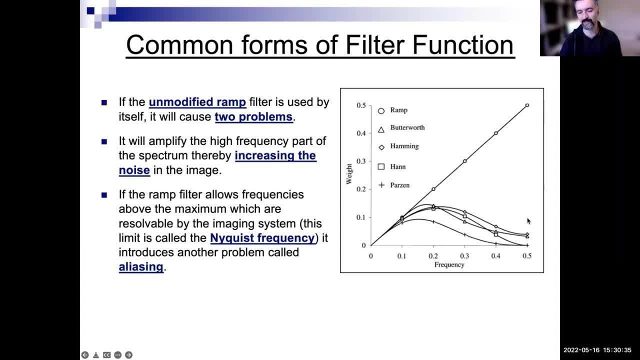 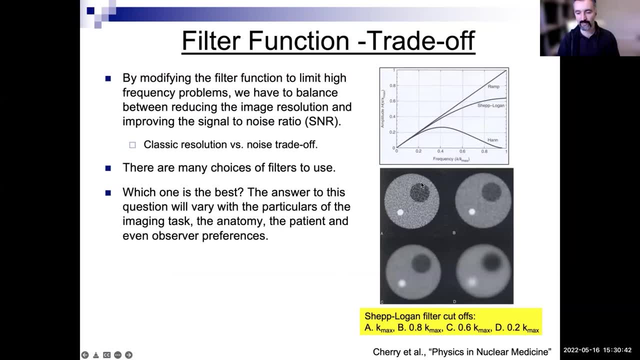 that really allow too high frequency content, because they're gonna create these aliasing artifacts. So here are some examples of reconstructions. This is reconstruction using a ramp filter. This is Shep Logan. Yeah, so exactly. So as you increase the 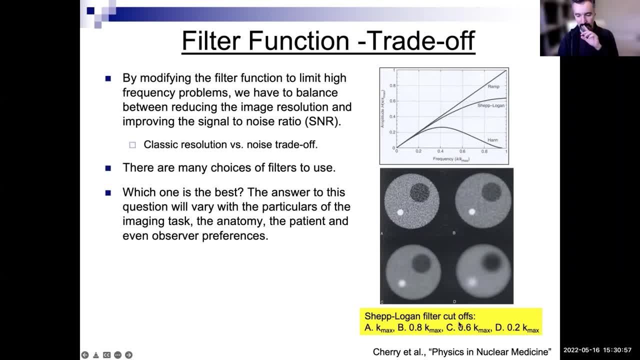 as you bring down the Shep- Logan in a sense- or you have a cutoff frequency, you start to not amplify high frequency signal. Therefore you're gonna get less noise images, but because you're kind of limiting frequencies, which you're amplifying. 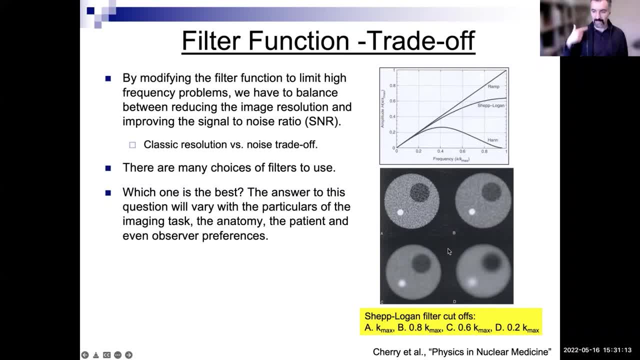 you also do get limited resolution. Remember how, today, we were talking about resolution versus sensitivity trade-off. You cannot win on both. sometimes, when you're just playing with the parameter Here, you're changing the filter. The filter is giving you less and less noise. 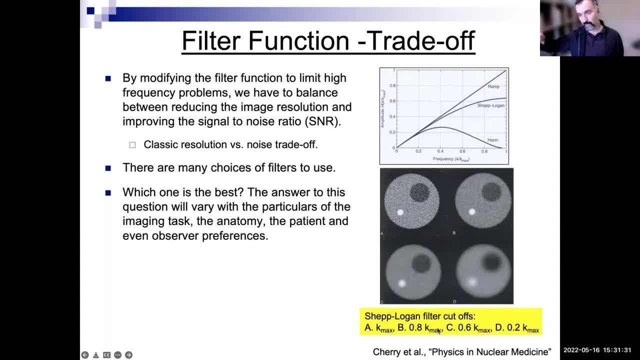 because it's having a high cutoff. it's removing the high frequency amplification, But it does give you more and more blurred images too. So it really depends on the application, which one you prefer. There's a classic resolution versus noise trade-off. 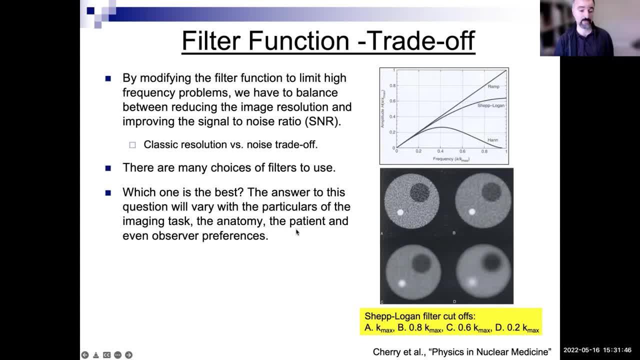 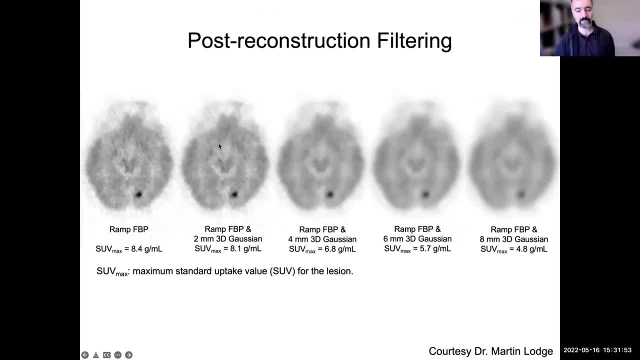 Which one's the best. Depends on the anatomy. depends on the patient. depends on what your observer preference is. Depends on the task. really depends on the task. Same thing with when you post, filter the image. Let's say you already reconstructed an image. 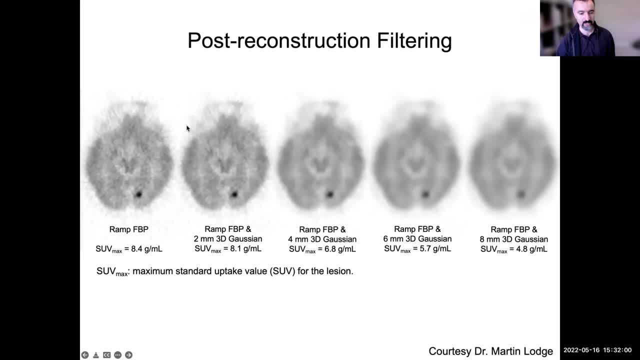 You could still filter it with like a Gaussian filter. So these are all ramp reconstructions. but So these are all ramp reconstructions. but So these are all ramp reconstructions. but you could be post filtering the images. Notice how, as you increase the 3D, Gaussian 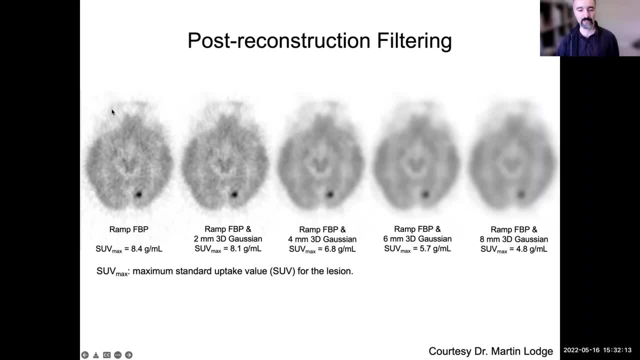 with from two millimeter to four millimeter, six millimeter, eight millimeter. This is actually something I'm doing right now as a physicist. We're having a very interesting study: brain imaging study, multiple centers, study of the effect of vascular disease. 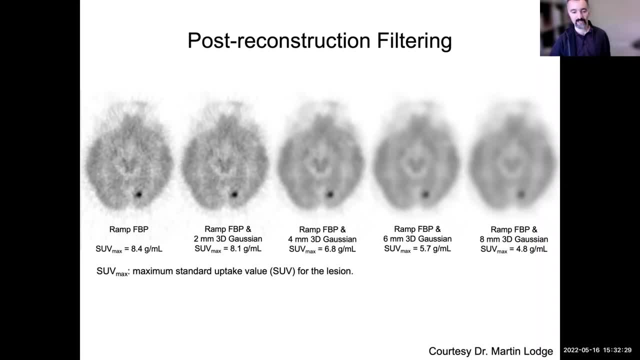 actually on brain function, which is quite interesting and fascinating, And we're having multiple sites, so we're gonna talk more about this in a bit And we're gonna have a little more time- toamos, I guess- but I'll just keep the rest of this in the chat. 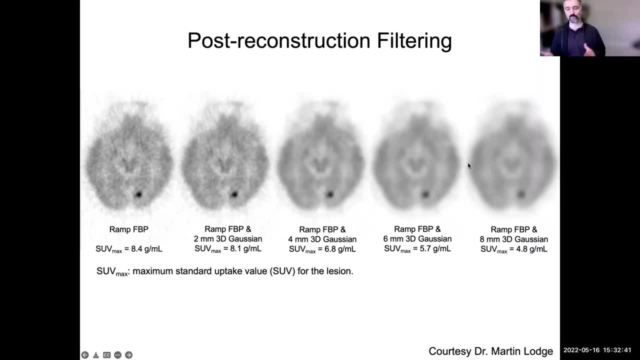 So anyway. so I'm here today with these post filtering numbers. So when I increase these numbers, I get images that are blurry but they have less noise. So which one do I pick? So I'm playing with this and I'm trying to make it more consistent. 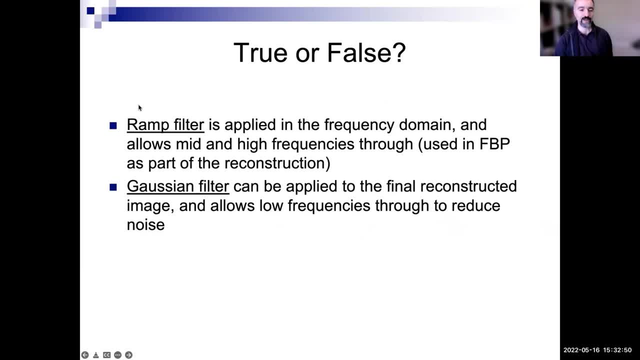 between the different sites. So, true or false? help me out here. RAM filter is applied in the frequency domain and allows mid and high frequencies through, whereas Gaussian filter can be applied to the final reconstructed image and allows low frequencies through in order to reduce the noise. 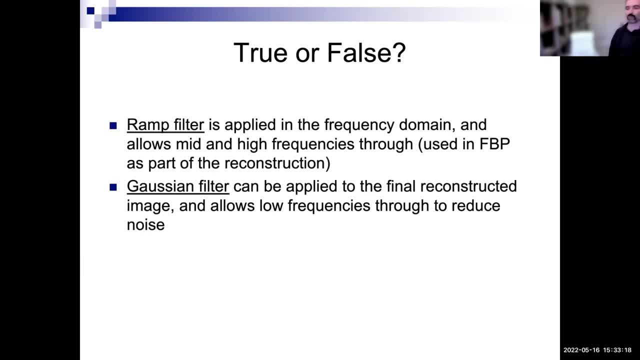 Is this collective statement true or false? So that gram filter is something you do during reconstruction, whereas Gaussian filtering is something you do after reconstruction? Any thoughts, Any thoughts, Any, anybody. In the words of Lion King's son: somebody, anybody. 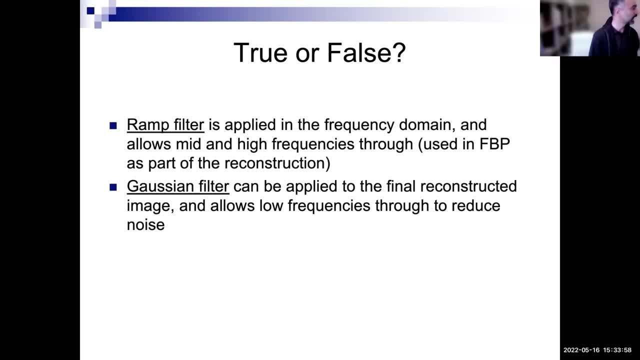 Is it true? It's true, Thank you for that. Yeah, so it's true. So ram filter happens during reconstruction, Gaussian is after it and gram filter is there to amplify mid and high frequencies. But if you don't really cut it off at high frequencies, 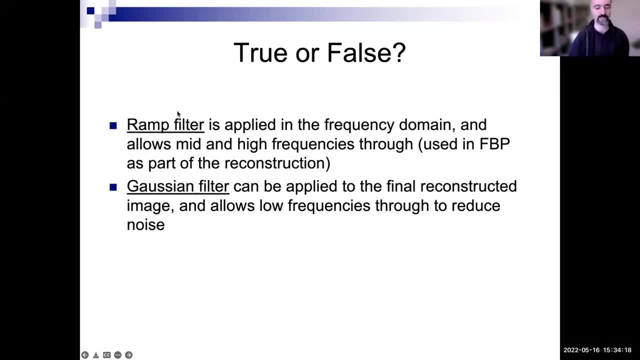 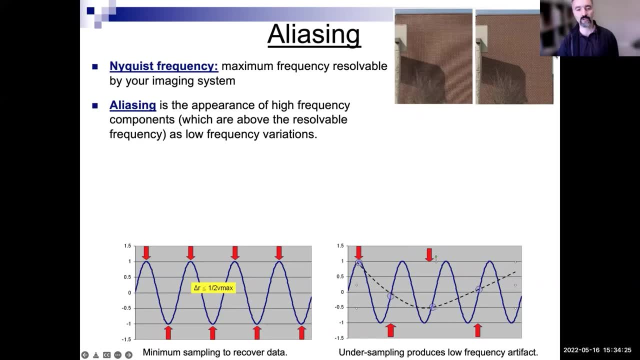 it does amplify noise, so you could post filter or you could change the filter itself, So you could do a combination of these, basically Aliasing. is this weird phenomena sometimes hard to explain? that of course this is the same building, it's just that the camera being used. 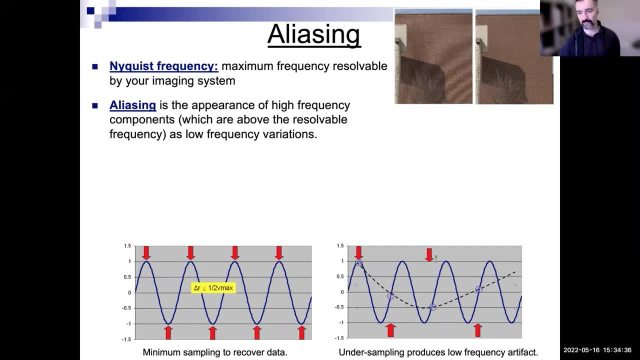 you know old TV systems, you would see aliasing in them a lot. This is the same building. it's just that the camera that is being used, its resolution, interferes with these really high, high frequency content of the image and might create weird patterns, as you can see here. 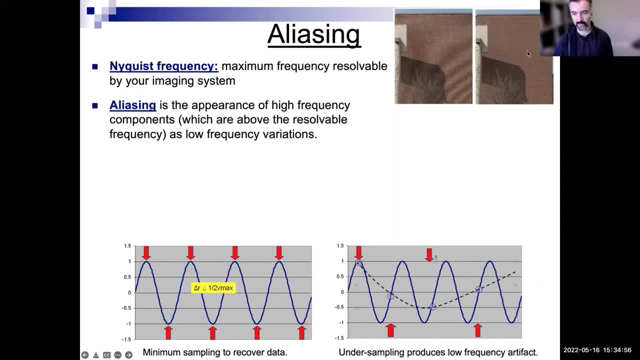 Imagine you've got this. these are the bricks. Think of this as the bricks that you're in this object. This is a frequency content And if you have a resolution, that is better than this and the size of the bricks, meaning smaller, meaning finer. 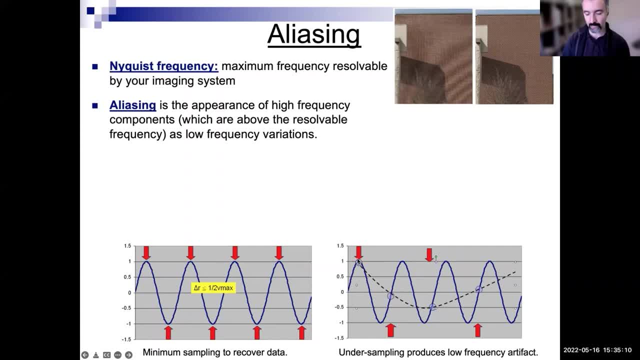 you're gonna be able to resolve them. But imagine that you are only able to resolve resolutions from here to here, to here to here, which is not as fine, as I should really say half the brick size. Imagine, this is the brick size. 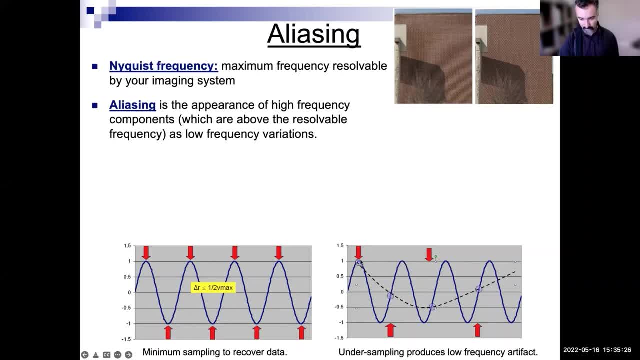 from here to here is the size of a brick. If your resolution is not better than half, you're gonna sample this one here. this one's gonna sample it here. this one's gonna sample it here. You're gonna think and imagine that you have a signal like this: 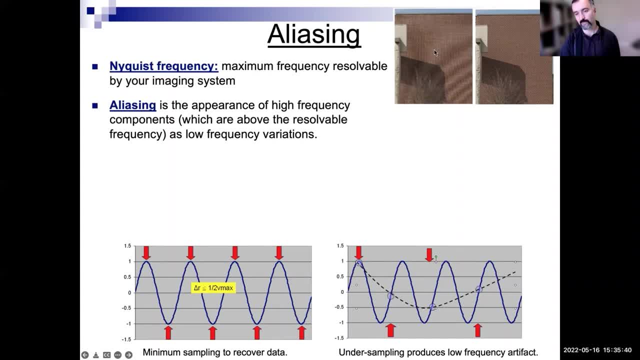 a high wavelength, low frequency. You see these weird things here happening. They look much, much longer in wavelength compared to the size of the bricks, And this is this weird impression that the human eye forms. So aliasing is the appearance of high frequency components. 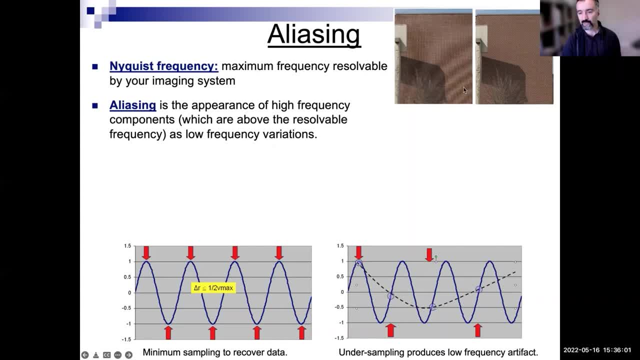 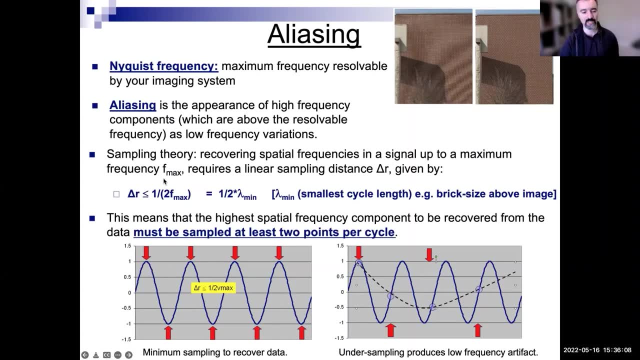 as low frequency variations. You have high frequency stuff but you start seeing these low frequency variations. The theory says, the sampling theory says if you sample your frequency content at better than half of its length, you're good. So if you get the smallest cycle length, 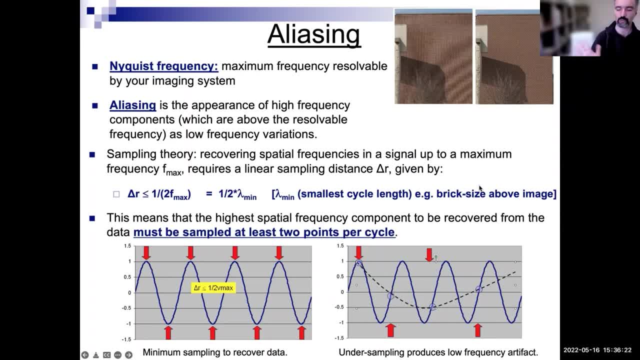 it has to be the or the brick size. if you sample at half the brick size, you're good, half or better. But if you sample at worse than half the brick size, half the wavelength, you're gonna get these weird low frequency variations. 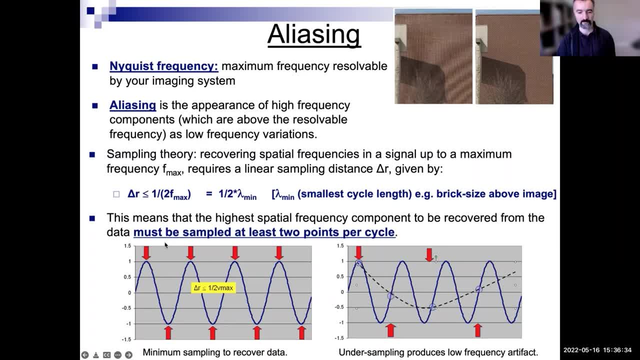 These are the variations that are purely artifacts, So you need to be sampling, at least at two points per cycle, the highest frequency content that you have. Now there's a practical rule of thumb Here we thought about full width at half maximum. 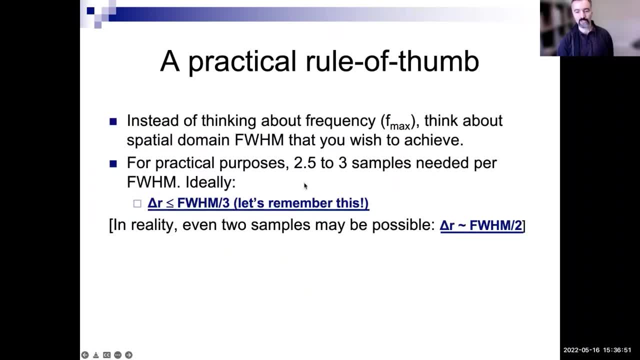 the repetition patterns. But we also like to think of the full width, at half maximum resolution of a scanner, Like if I have a point source, how big is the point going to look Typically? you know, inspect, we've seen, you know. 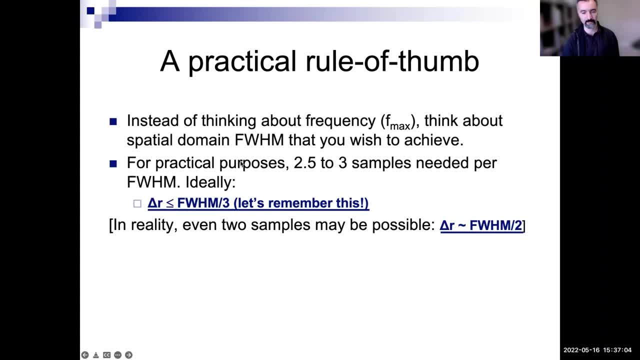 we've seen that one centimeter in PET. we've seen like half a centimeter. For practical purposes, this rule translates to the fact that you need to be sampling at around a third of your resolution. I'm taking up: even half is okay. 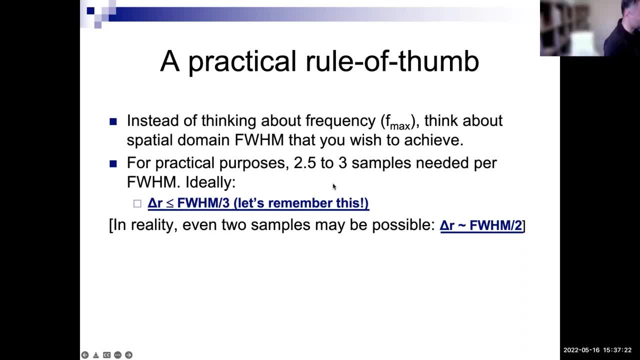 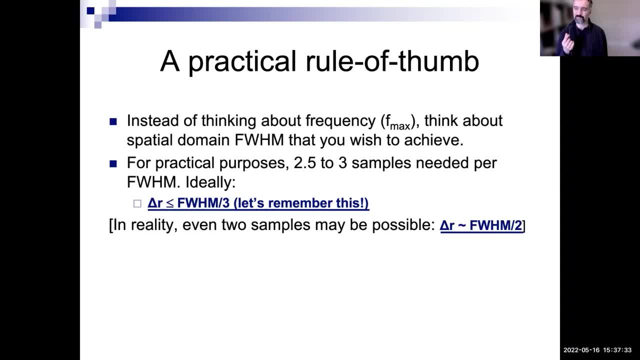 if you have an object that you want to resolve down to. if you have an object that you want to resolve down to six millimeters, your detectors in PET, for example, six millimeters, your detectors in PET, for example, should be about a third of that to two millimeters. 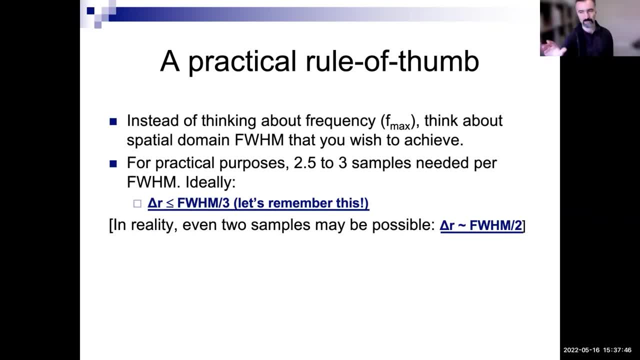 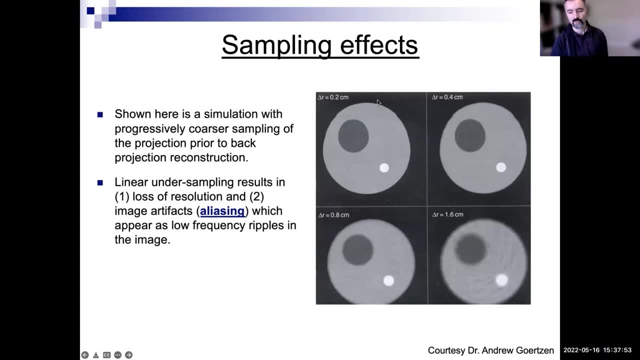 So if you have about two millimeters, you're going to be able to resolve six, maybe four, Like it depends whether you take this rule of thumb to be a third or a half give or take, And if you don't, you're going to get aliasing artifacts. 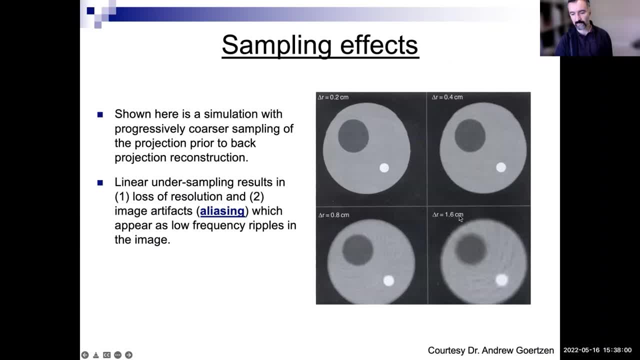 All right. so, for example, here's a sampling that is happening. that is really really. here's a sampling that is happening. that is really really. that is really poor: 1.6 centimeters. You're going to start seeing aliasing. 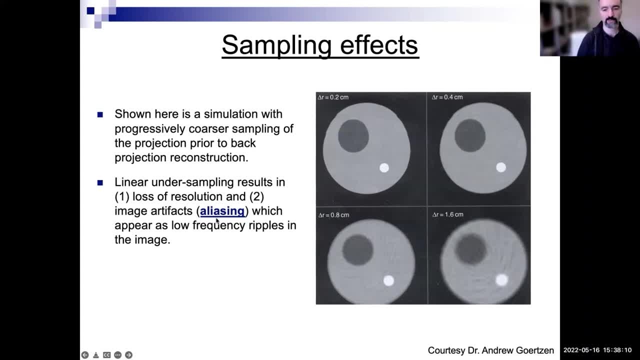 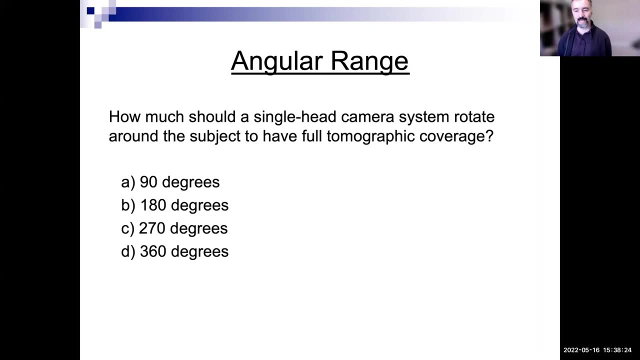 You get loss of resolution and aliasing, So you want to be careful about it. It depends on the resolution of the object that you want to resolve anyways. So here's a question for you: How much should a single head camera system rotate around the object or the subject? 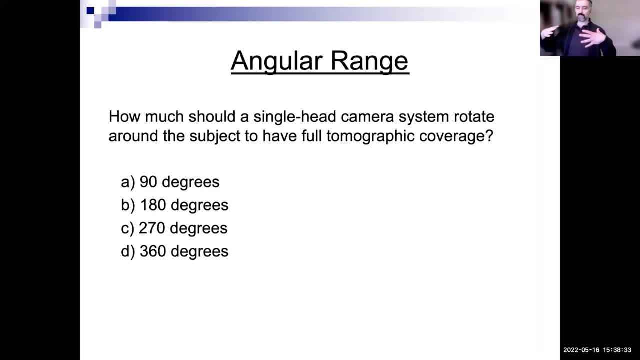 to have full tomographic coverage. If I'm a patient and you want to go around me to do tomography, how much are you supposed to rotate around me in order to allow full tomographic coverage and therefore resolving my body? What do you think it is? 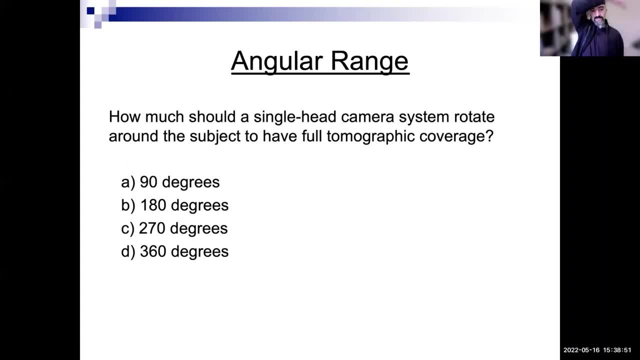 90 degrees, 180,, 270, or all the way 360?? What's your guess? I would have thought 360.. Right, and that's what I would have thought too. But it turns out, Ali, that is actually half of that here. 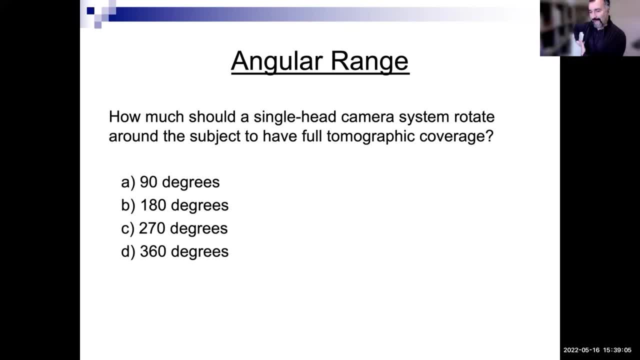 Why? Because the same signal that is going to the back of you, the same signal can be coming to the front of you, Meaning so the answer is actually 180.. The reason is because you're having a projection. whether this projection 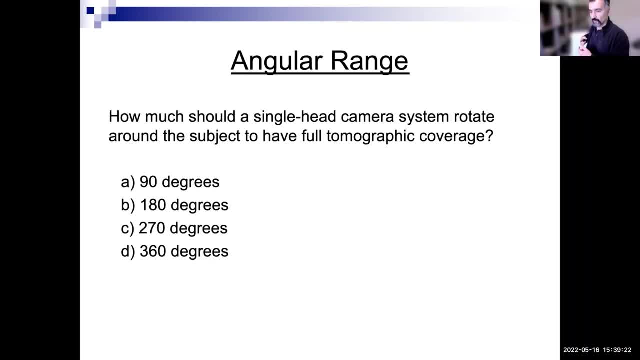 whether you're summing this way or you're summing that way, the sum is the same. So you know what I mean. Now, of course, attenuation changes, But put that aside for a moment. Imagine there's no attenuation. 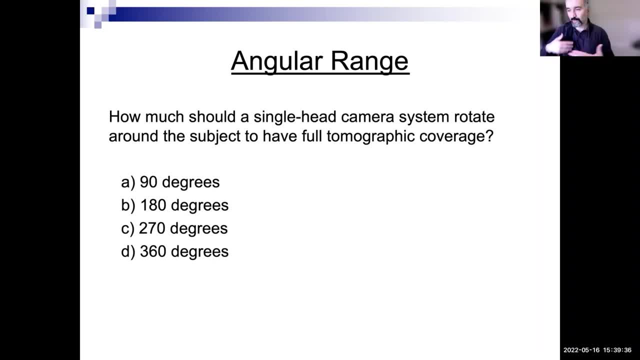 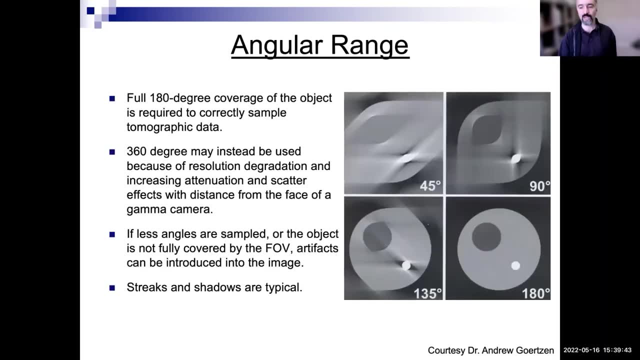 Imagine you're just summing counts. Whether you're here or at the back of me, you're looking at the same thing. You're looking at just these lines that are passing through me. So it turns out to be 180 degrees, And look if you do less than 180 degrees. 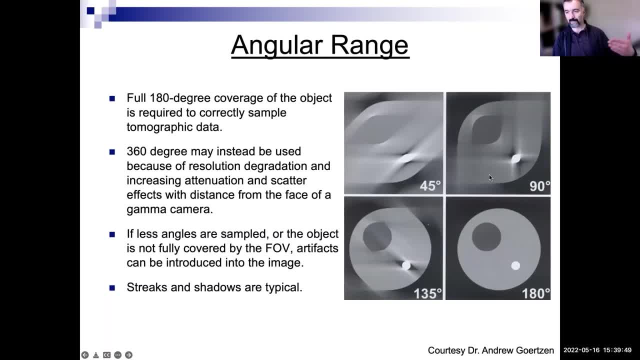 you're going to get terrible images right. As you increase the amount of coverage of the body that you have, you're going to get better and better and better images. Now, of course, you could do 362, because of a number of other reasons. 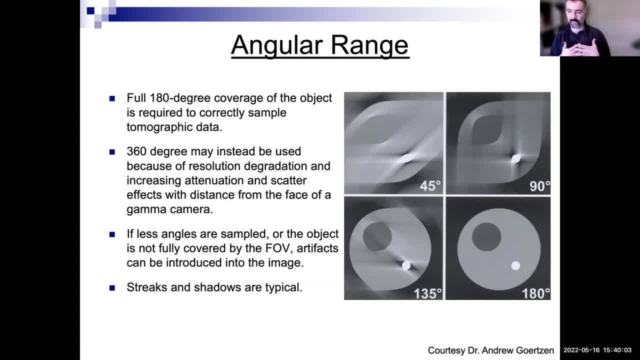 Remember how I said: the closer that you are to the detector, the better. Well, that's when these things enter the picture. If I really care about the front of my body more than the back of my body for imaging, sure, then stay here. 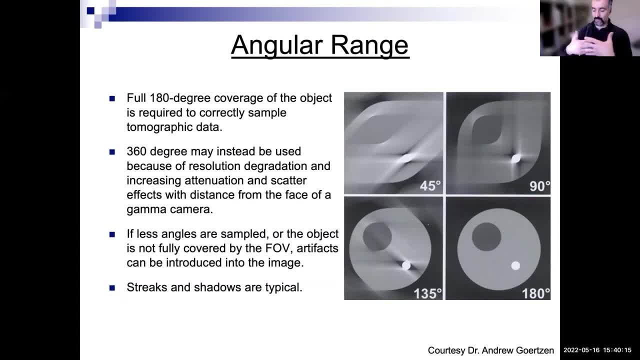 But if you want to resolve the whole body front and back, and you only do imaging at the front, you're going to get poor resolution at the back of my body because it's too far away from my collimators. So in that case, 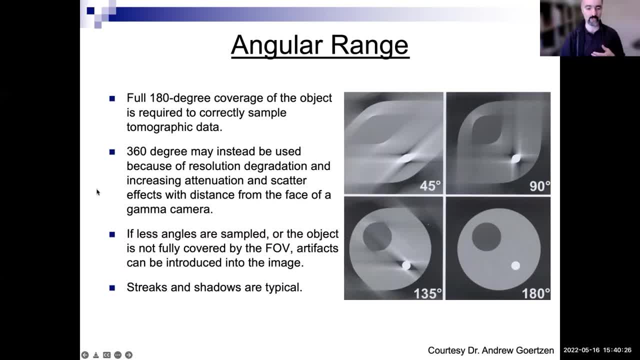 it's actually better for you to do a whole 360 coverage so you don't have this resolution degradation. Same thing for attenuation. If you're close to here, you're going to be seeing less attenuation from stuff here where you're going to see more attenuation. 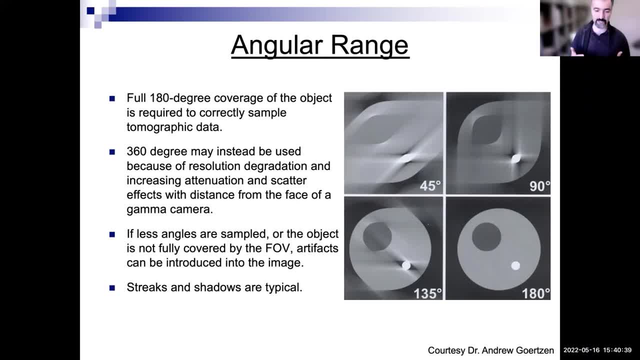 from the stuff at the back. Therefore, you're going to have a significant loss of signal possibly. So again, you don't have to cover 360 degrees, but if you care about full coverage, you can. But if you're looking at the heart, for example, 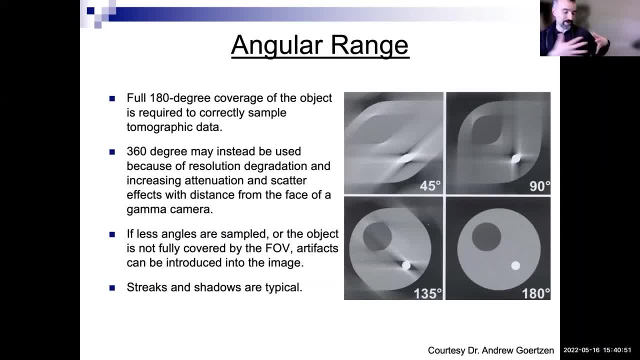 if you really want to focus on the heart, then you can just stay around here. You don't have to go from the back because you're closer to the heart this way. So it depends on the application And if less angles are sampled, for example. 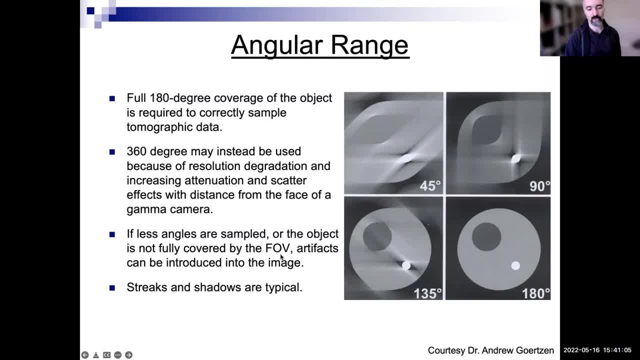 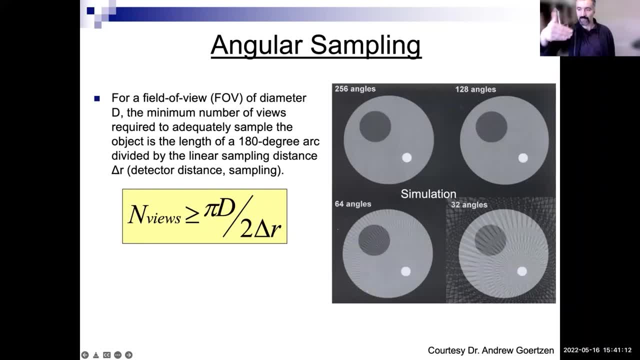 or the object's not fully covered. you're going to see all kinds of artifacts, Angler sampling, how many angles? like sure I've got to go around 180 degrees, but how many angles? There's a formula for it that people use. 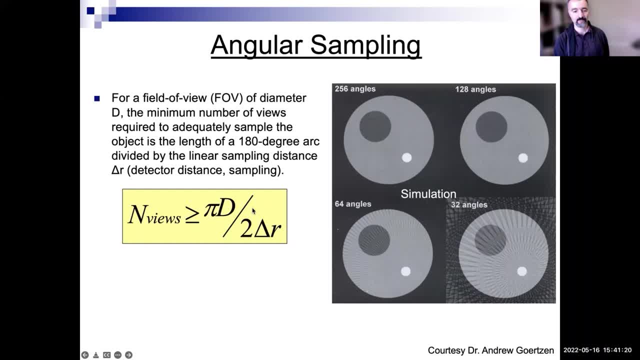 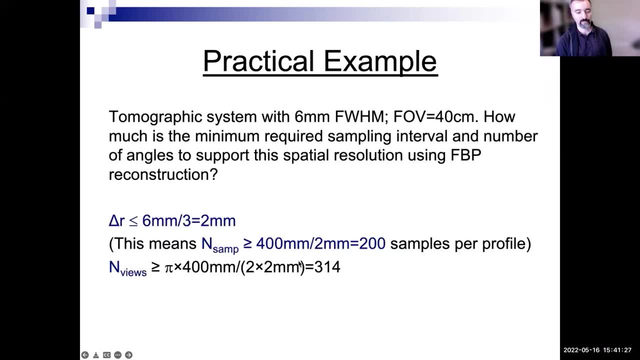 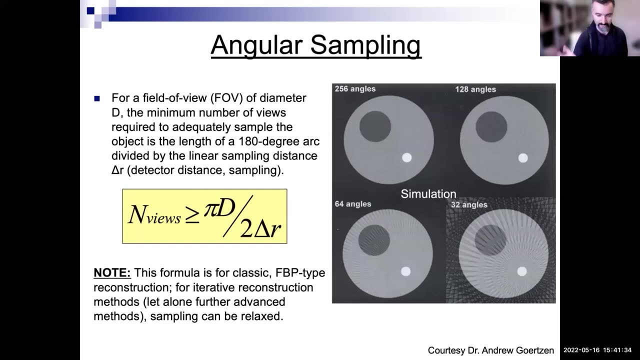 We won't go through that, but you know there's a formula, And so this formula is, however, for filter back type sort of reconstruction, for iterative recon, And also nowadays, with artificial intelligence driven, all these things are starting to change because you know, 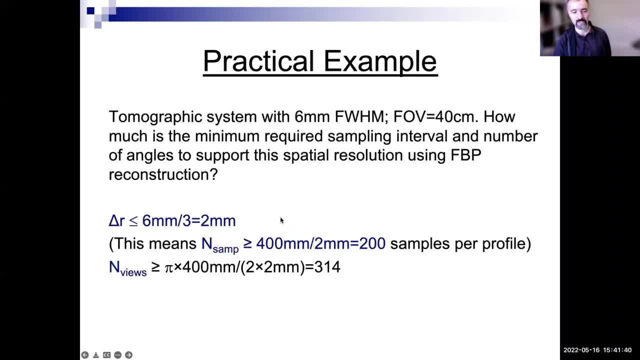 some of these proofs don't work that way or, you know, the concepts are different. So, just as a practical example, I want you to feel this, make it more tangible. Imagine you have a tomographic PET or SPECT system that has a full width, half maximum. 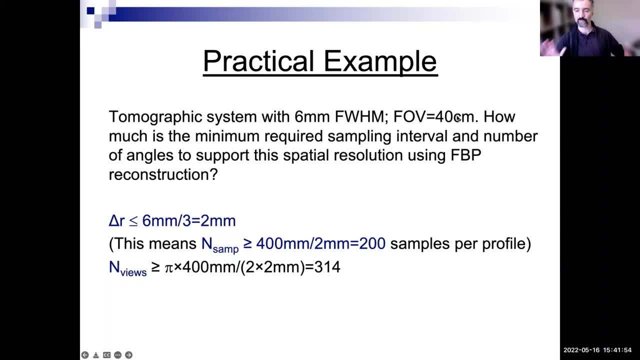 of six millimeter resolution. Imagine the field of view. How much is the field of view that it images Like? just think 2D coverage is about. you know, the diameter of the field of view is 40 centimeters. How much is a minimum required sampling interval? 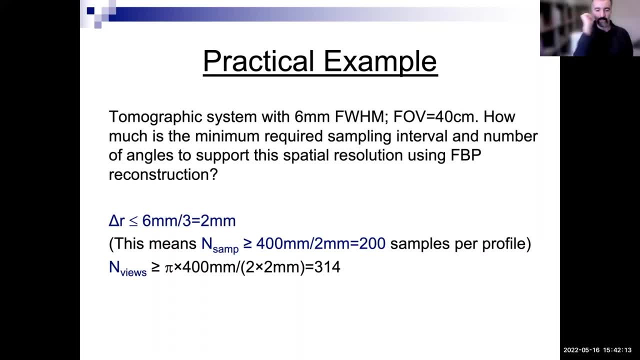 Like how many, what should be the detector size And how much? how many times should you? or how many angles should be going around the patient? Okay, so the rule of thumb said the sampling should be about a third of the resolution. 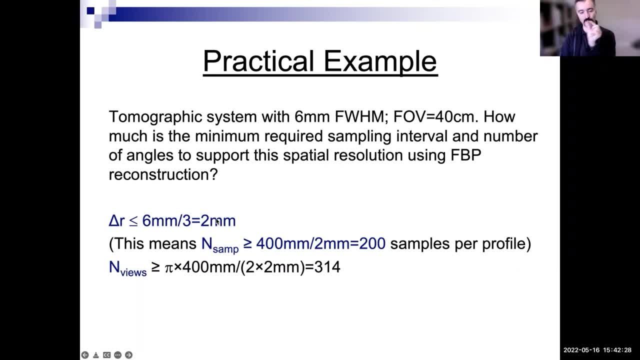 So that gives me two millimeters. So the detector size should be two millimeters. And then this means, if the field of view is 400 millimeters, you're going to have 200 samples. So you're supposed to be having 200 detectors, for example. 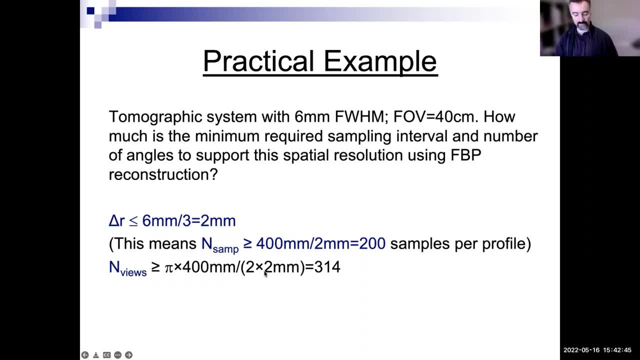 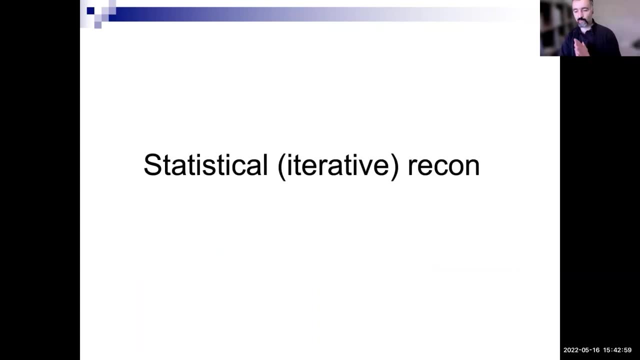 to cover 40 centimeters And if you put it inside this formula for the number of angles that you need, turns out to give you about 300. So you need to be rotating 300 times ideally to achieve such a that you're going to get the data. 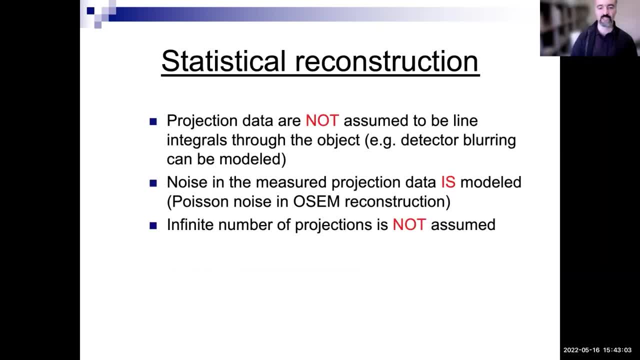 Now let's move on to statistical iterative reconstruction. Statistical iterative reconstruction has three really great things about it. You don't have to assume that what passes through your body is a perfect line, Because in fact, when you enter crystals and detectors, there could be some layering. that happens. 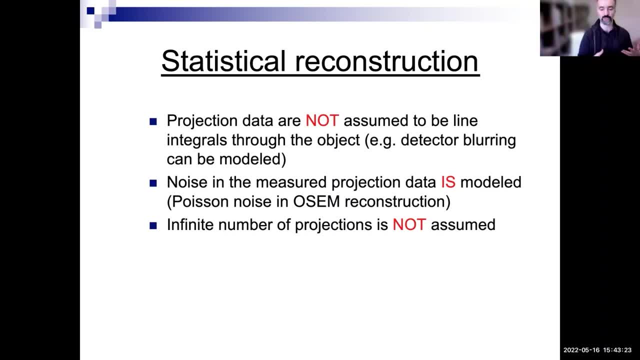 gathering inside the crystal. Nothing is perfect. Good model loads, Good model blaring happening in the detection process. Also, filter back projection really doesn't assume any noise model or a very simplistic Gaussian noise model, whereas noise is Poisson. actually There's this noise that detectors measure. 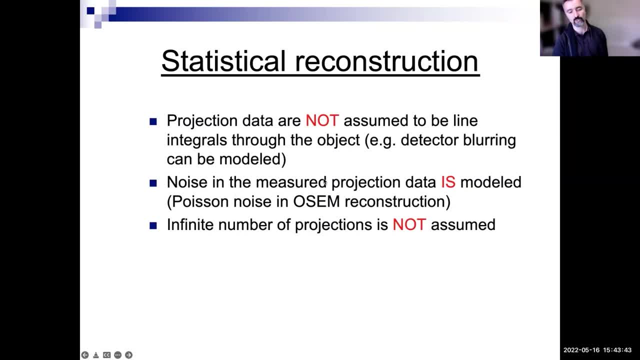 It's called Poisson noise, It's not Gaussian noise, And so we can actually model that in image reconstruction. Finally, filter back: projection type algorithms assume you have an infinite number of angles around the patients and you have a lot of them, but you don't have to have a lot of them. 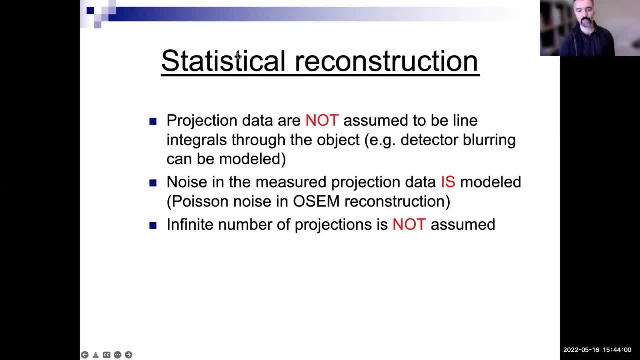 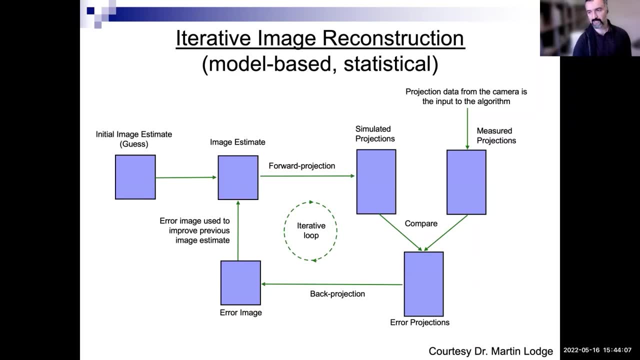 And sometimes you don't have a lot of them and none of these need to be assumed to be able to do this. So I won't go through the details, but basically iterative recon in also in the world of CT. recon similarly works like this: You start with an initial image. 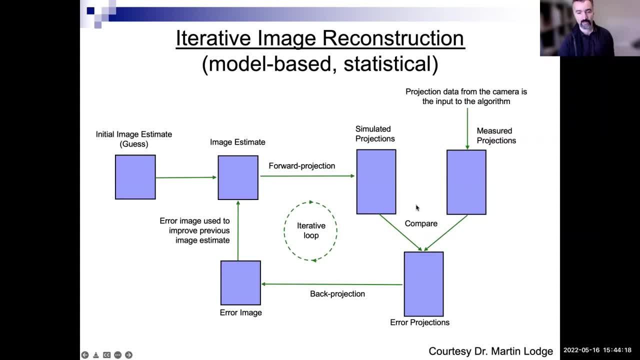 You say: if this is the truth, what do I expect to get in the projections? What kind of detection do I expect to measure? So you have to have a forward model, like radon transforms. It says: if this is a truth, this is how much signal you're gonna get in your detectors. 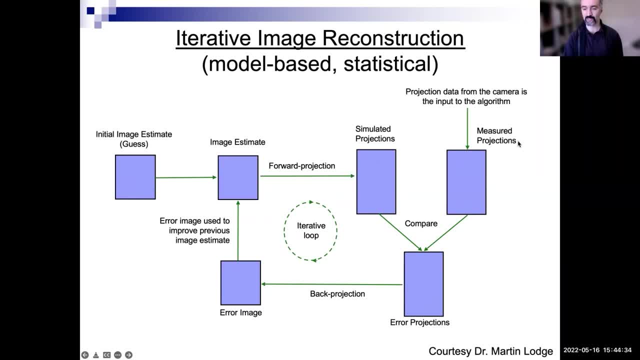 Then you compare that with the actual measure projection, actual measured detector values. You compare them and calculate some kind of a ratio or a difference, for example, between them as a measure of error. Then you back project it. You come back to the image space. 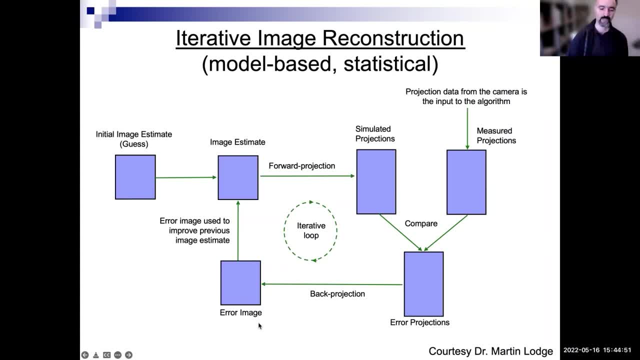 and you've calculated some kind of a correction image that says: look, these two are not that close to each other. I'm not impressed. I'm providing you with a correction. Now, correct your initial guess, Give me a better guess, And then you, so you improve your guess. 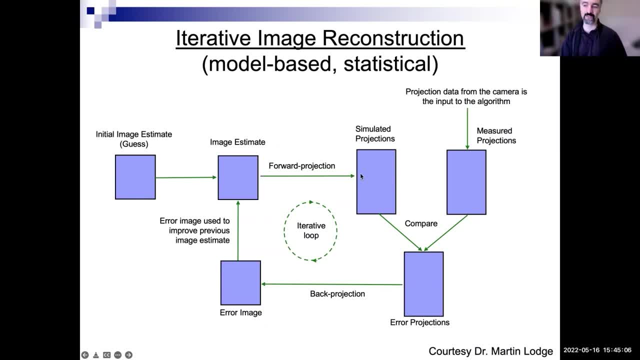 Then you again keep doing this and say, okay, this is my new guess, And you're gonna say: fine, I'm gonna give you another chance, another iteration. What would this image look like in the projection space, in the detection space? How does it compare with what I actually measure? 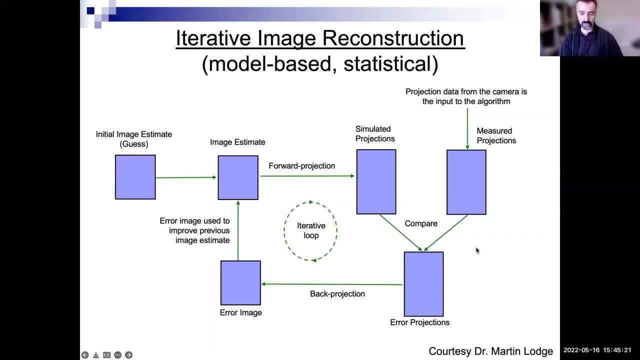 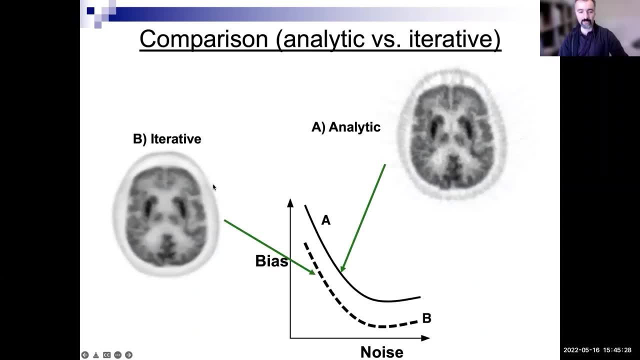 Oh, it's still not there yet, Let's do a correction, So on and so forth. And so with more and more iterations you get better and better images, And iterative reconstruction, I would say, tends to do better than analytic recon. I would say, if you were plotting bias versus noise, 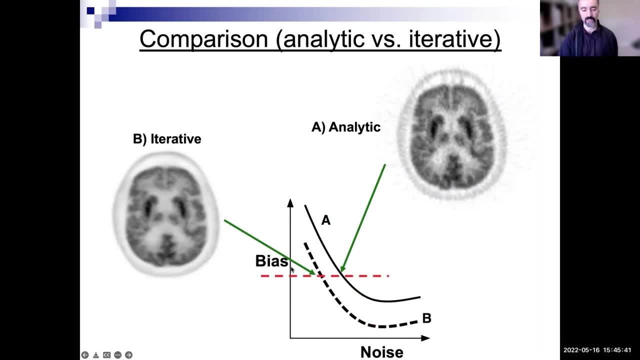 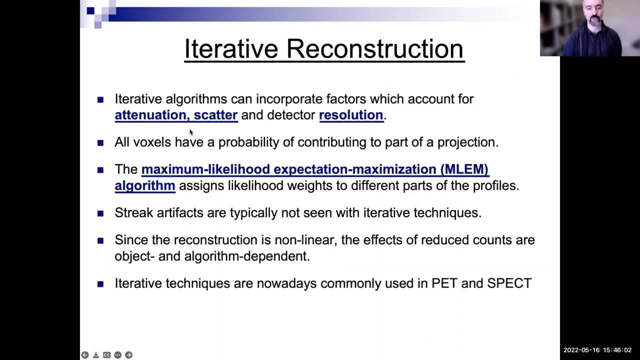 for the same bias and deviation from the truth. you would get less noise in iterative methods. So gradually in our field and increasingly in other fields, people are switching to analytic- sorry, to iterative, statistical methods. So as a summary, they can incorporate things like attenuation and scatter and resolution. 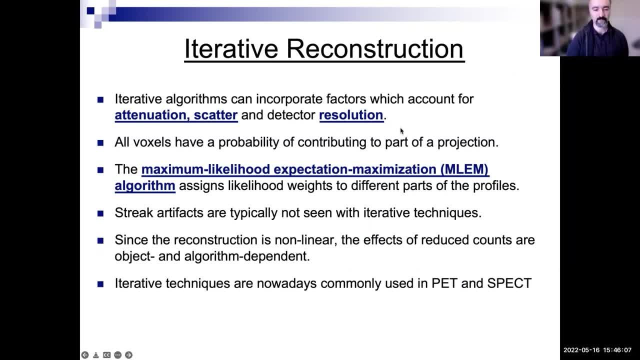 in the detectors quite better. The MLM algorithm is very well known. does very well models of Poisson noise. It's called the maximum likelihood expectation Maximization was introduced in 1982. And it's really used very routinely nowadays. You may get streak artifacts in filterback projection but 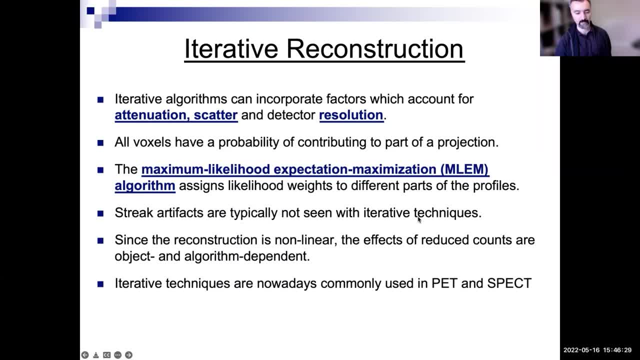 they're not seen with iterative techniques. There is some non-linearities with OSCM because, unlike filterback projection, which is kind of linear, this one is not. but for you know, just just just, I don't want to oversimplify, but I might. 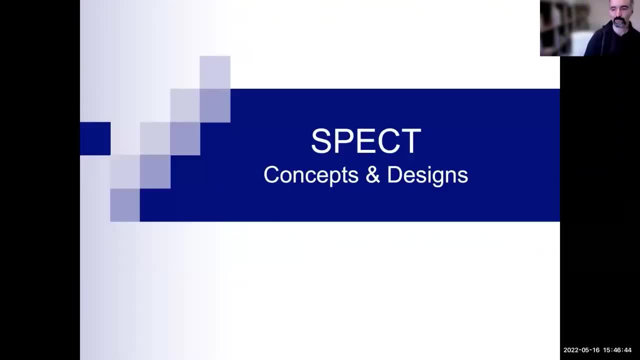 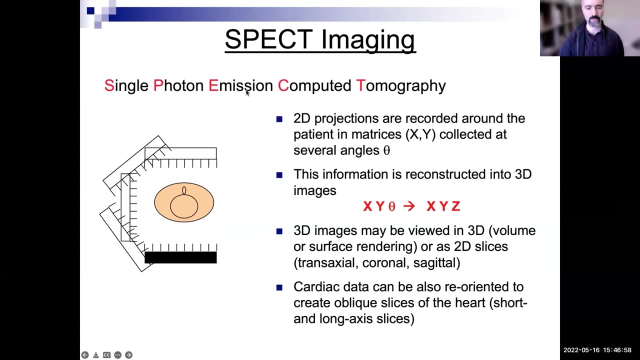 I mean, they tend to be better. Of course you have to know some of the artifacts that they may produce, like iterative recons, but they're pretty good. Last part of my talk today is focusing on SPECT concepts and designs. So again in SPECT you have single photon emission. 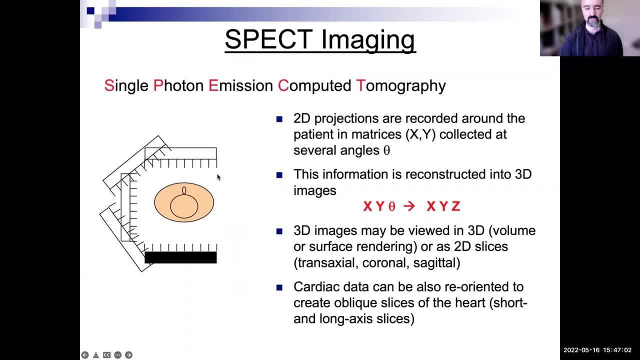 computer tomography. you rotate it around the patient So you have an X and Y coordinates inside the detector, Sorry, so imagine you've got this detector, it's got, it's got an X and Y goes inside X and Y and you rotate it at different angles, right? 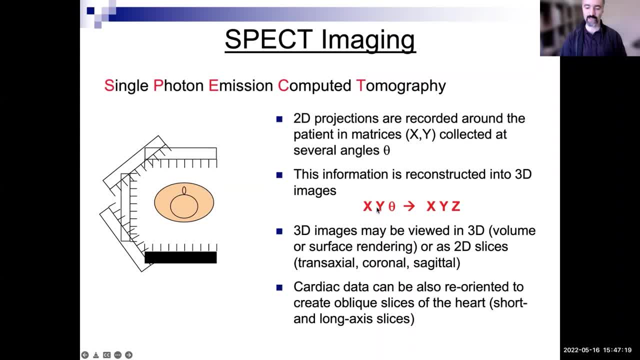 And then you change, you get those data- the X and Y coordinate values- at different angles, and somehow, using image reconstruction, you convert that to reconstructed 3D images of the patients. Of course, cardiac data can be reoriented, et cetera, et cetera. 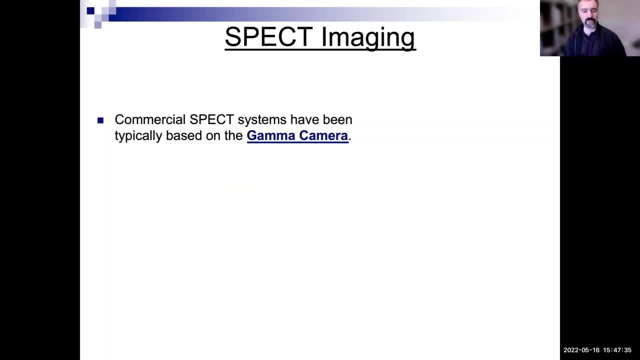 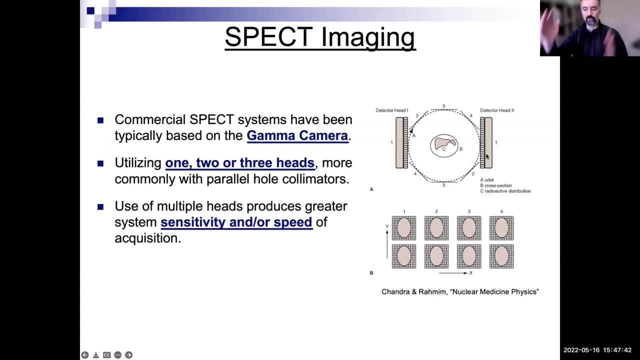 We won't go through those details, but commercial SPECT systems have been typically based on the gamma camera, again using one or two or three heads. Here's an example of two heads and you would be rotating around the patient. This is an oversimplified example. 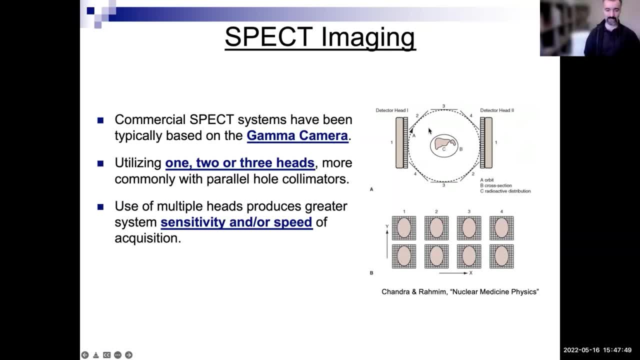 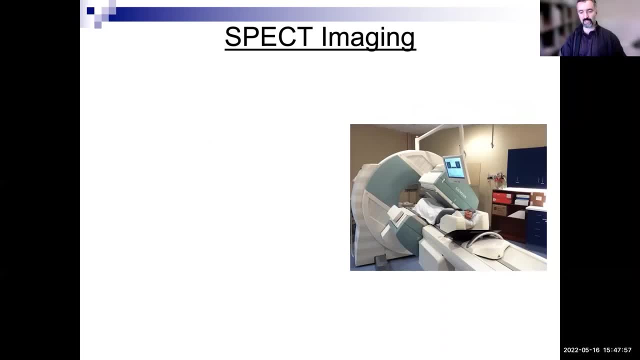 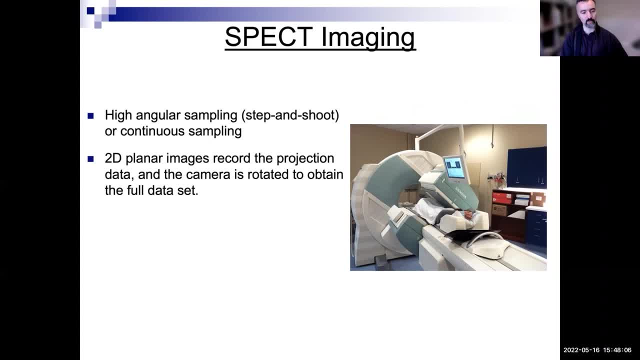 or you could do continuous, but step and shoot is more popular. more common 2D planar images are created. Again, this is the X and Y coordinates. You create these 2D planar images, but you rotate them. 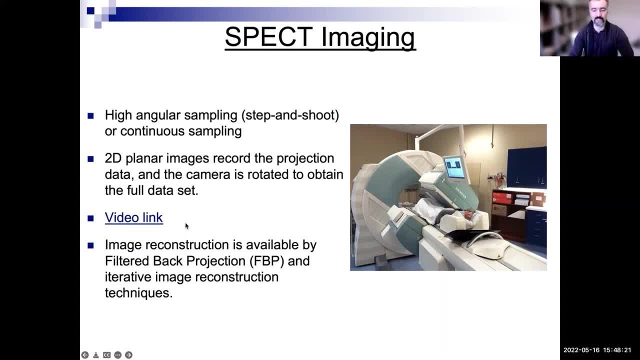 I won't go through the. I'll send you the notes. You can look at some examples- Somebody giving a tour, I think, of facilities et cetera, And in our YouTube videos we go through these in a lot more detail. 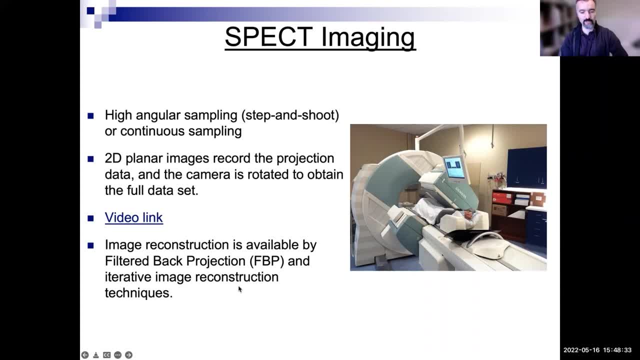 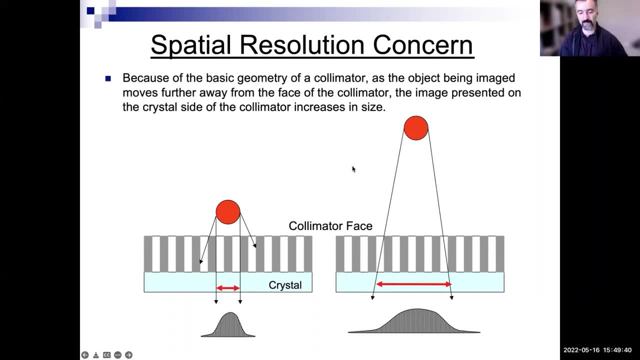 Image reconstruction is available by filter-back projection or iterative recon. We already talked about that. The spatial resolution has a concern, as we've mentioned multiple times: As you get farther away from the collimator, you get poorer resolution. Okay, So this? what are the implication of that? 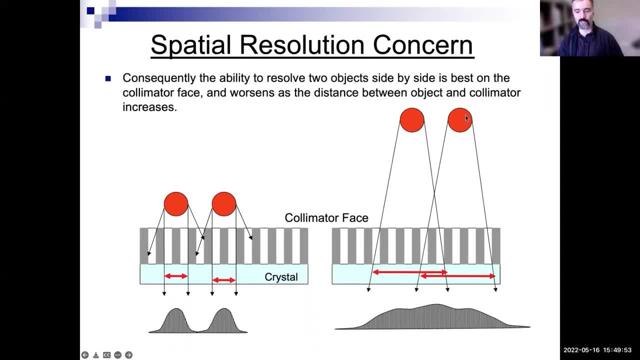 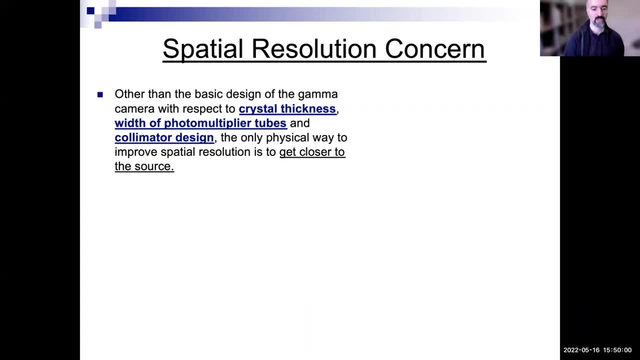 Implication is that obviously the resolution is worse. So you cannot resolve these two points Whereas you can. So to do that, we have to play with certain things, And this all depends on a whole bunch of designs. But at the end of the day, 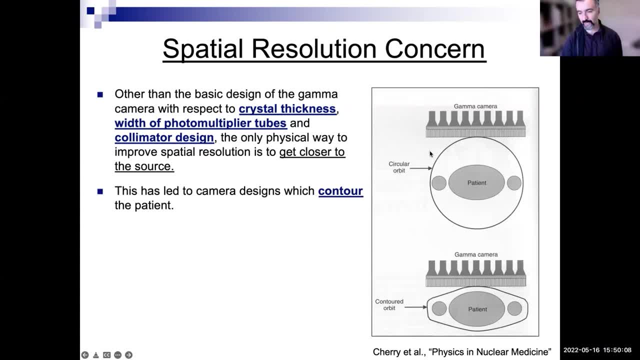 given the system that you already have, you could try to rotate this around the patient in a contoured orbit, not a circular orbit, So you can bring it closer to the patient. So right, So contouring the patient in this way. 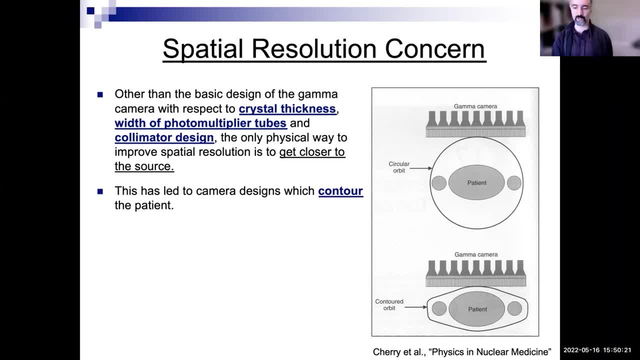 So you get closer to the chest, for example, as opposed to having a circular distance pathway. And also there's a question of you know what kind of reconstruction based improvements can we do, Because again, there's attenuation happening in the body. 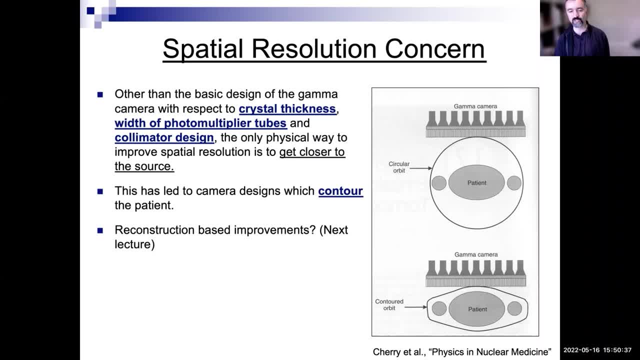 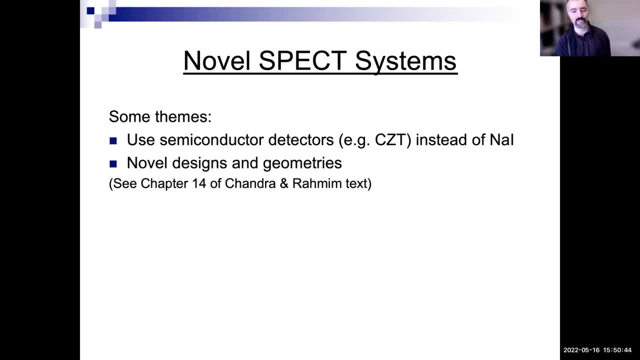 scattering happening in the body, blaring happening in the crystals. Why can't we do the correct for these? So these are something we're gonna talk about next time in the next lecture. There are a number of novel spec systems, some that move beyond sodium iodide scintillators. 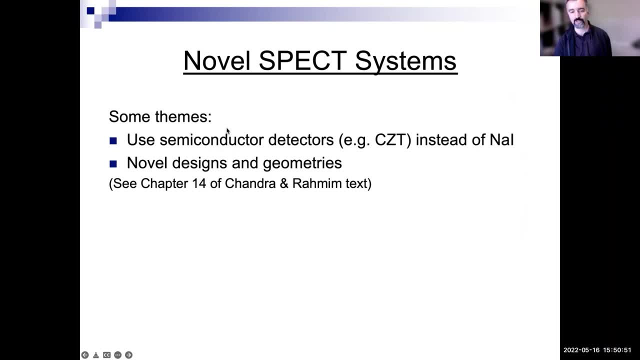 to more expensive but better detectors, so-called semiconductor detectors, CZT or synovial TZT or CZT, And so let's quickly talk about that And some novel designs and geometries which chapter four of our text talks about. So basically, when you switch to semiconductor or 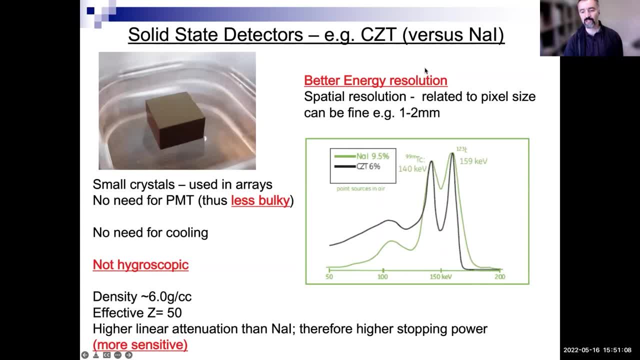 solid state detectors, you end up with better energy resolution. Okay, So the resolution can actually improve significantly, right? I mean, here's one example, but it can improve even more. Also, you can actually get less bulky material. They're more expensive, but they're less bulky. 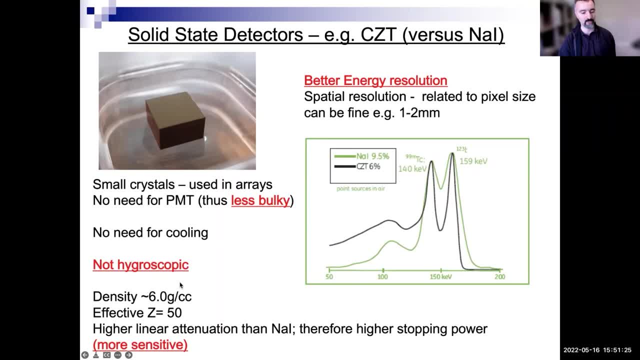 and they're not sensitive to humidity. right, And at the end of the day, you can have higher attenuation, therefore higher stopping power, so more sensitivity. Okay, So you get better resolution and better sensitivity. This is an example where it's a win-win. There's no. 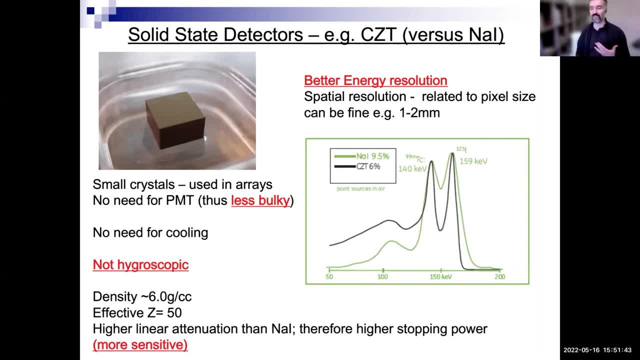 trade-off between resolution and sensitivity, because you're changing your material. You're changing your material, which has better resolution and sensitivity, But again it's more expensive. So historically, uh, it's taken a while to transition towards this, but increasingly this has been happening. 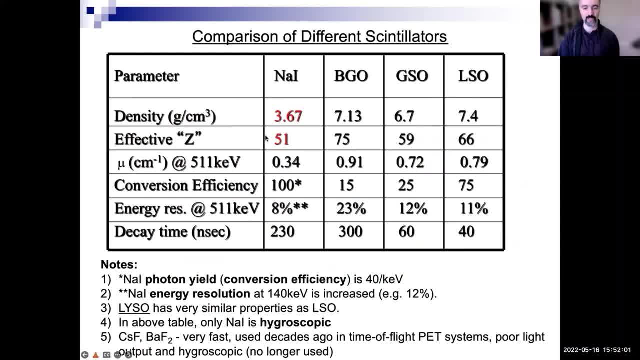 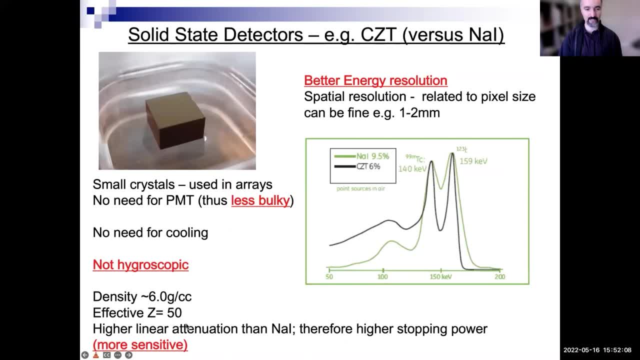 Um so, again looking at the numbers, look at sodium iodide. the effective Z is 51. Okay, That part is the same as let's say in this example of a CZT or CZT, but the density here is less than. 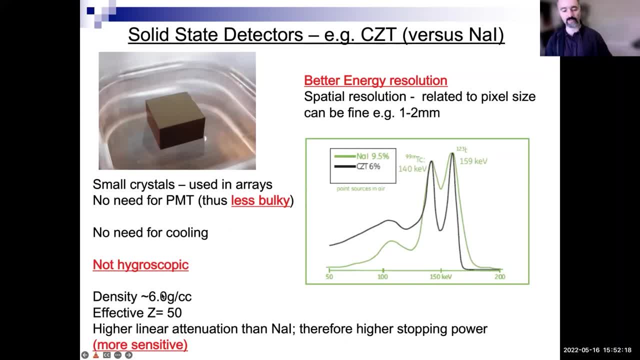 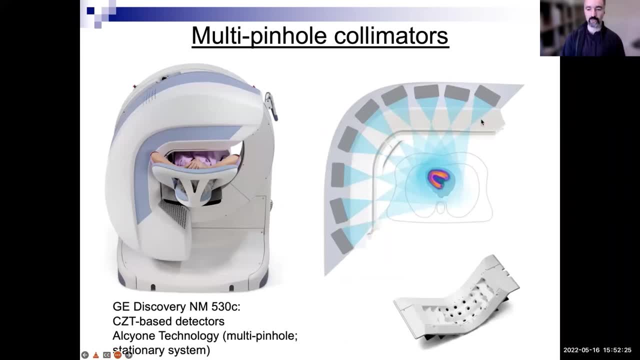 the density we're having. Because of the higher density, you're going to get better sensitivity for solid state detectors. Just to show you an example: Multi pinhole- I already showed this before, where you could be using pinholes to get really 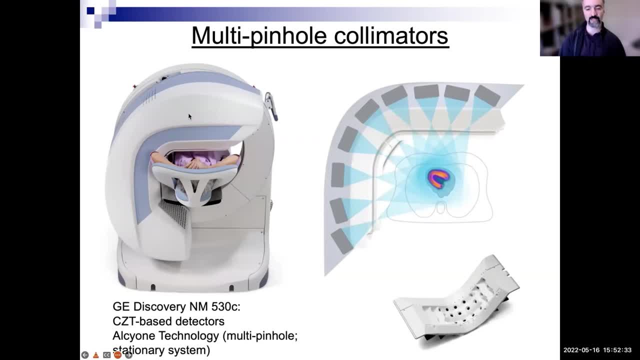 Now this system, you no longer need to rotate the entire camera. It's just that these pinhole collimators do rotate, so you don't physically see it, but it's inside the camera. it will rotate, So it allows less mechanical movement. 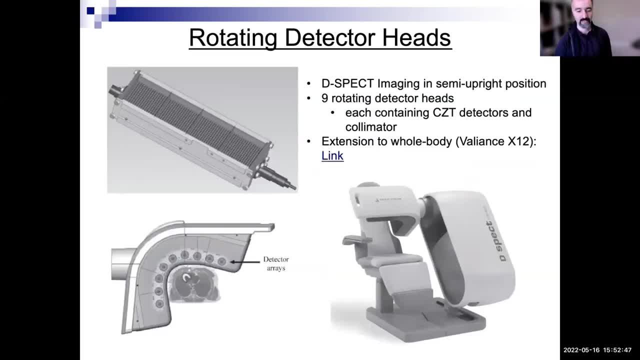 It's a very innovative way of looking at it. Um, uh, actually I take that back. These ones don't rotate, It's not a big problem, You just rotate it. The number of times you rotate it, the" Z. 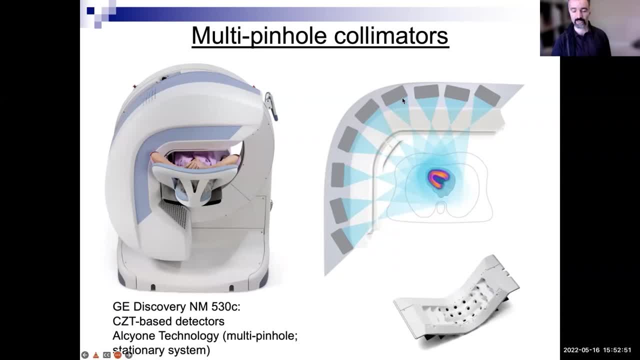 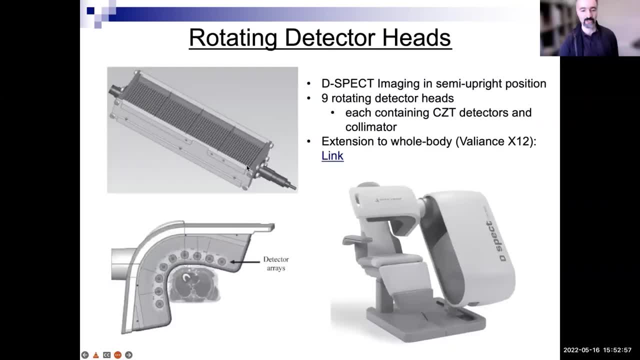 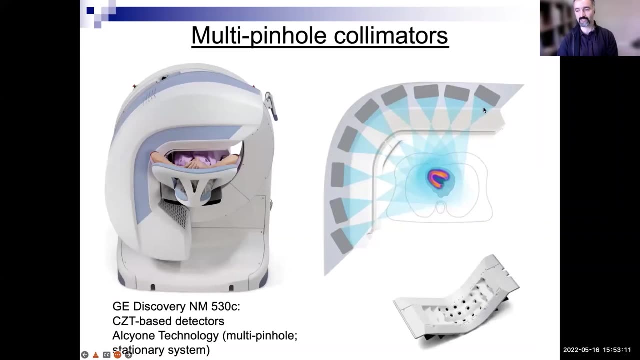 result, which is even more amazing. but in this design you're having these things. uh, where you've got these upright positions? these ones are rotating, these ones are. so, again, the system is not rotating, but what's inside the system is rotating, whereas here, because you're having pinholes, it turns out. 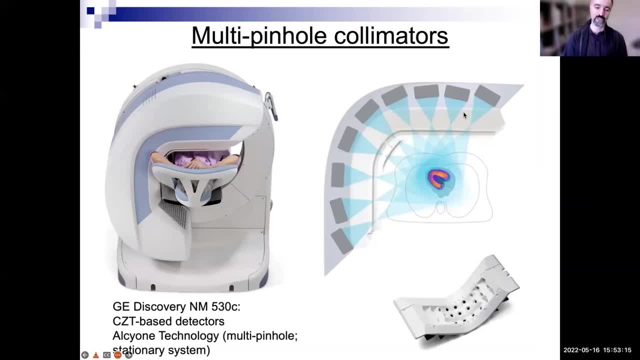 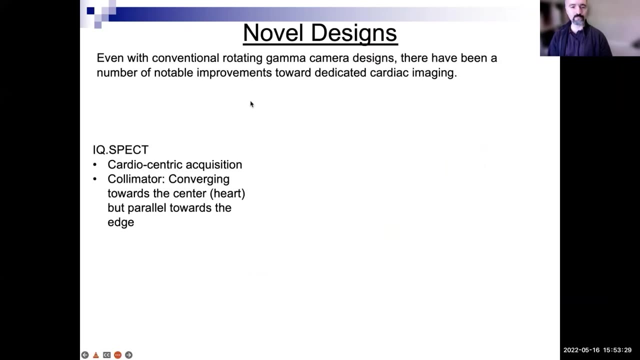 you're sampling at so many angles you don't even need to be rotating this. so it's a stationary, very impressive stationary camera um, which is kind of like what the pet world does, naturally, but for a spec world to be able to build a stationary camera, it's been a very impressive um there's. 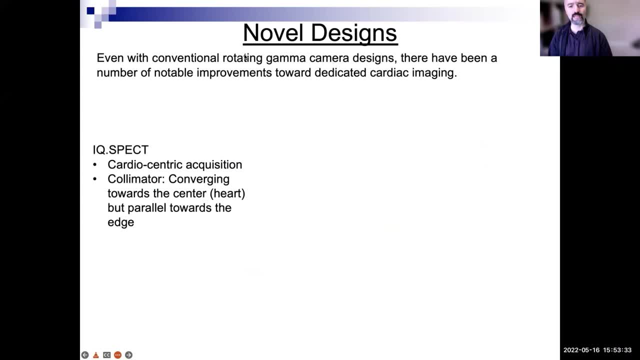 also um. you have things that are conventional rotating gamma camera designs but the um because they're dedicated cardiac imaging. they kind of change certain things about the collimators so they move instead of a parallel whole. collimators more to converging, but it's not converging everywhere, it's only converging towards the heart. 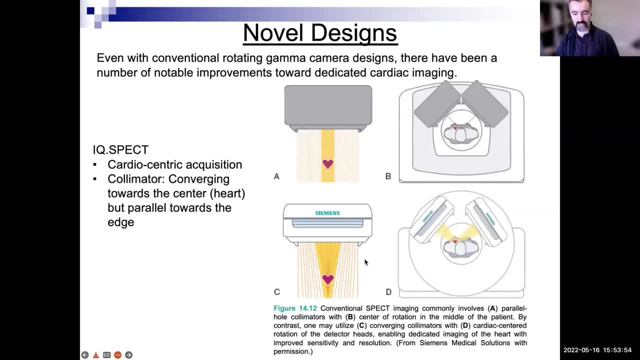 but parallel elsewhere. so it's a very strange design in a good way. notice how it's parallel here, but as you get closer to the heart it becomes converging. so i can't really call this a converging collimator, but parts of it are converging. okay, so parts of it are converging. 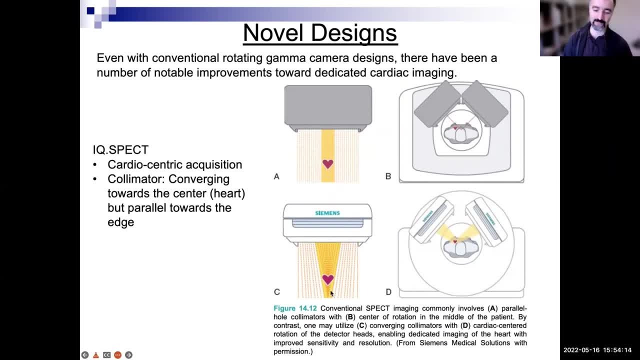 and in a funny way these ones are diverging. so collectively it's covering the same field of view, but it puts more emphasis on the sampling at the center than at the away from the. or, you know, if the heart is centered it puts more emphasis on the heart sampling and else outside. this is it's a. 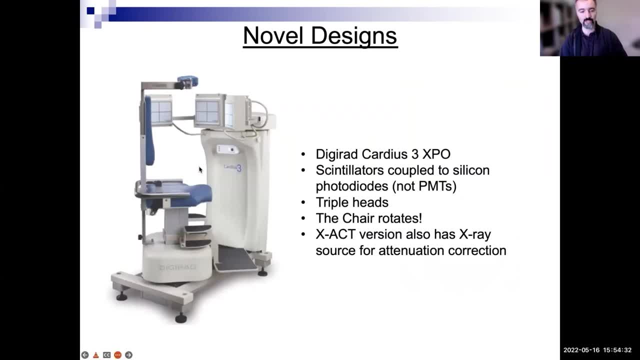 mix of things. so it's kind of an innovative design or you could have the patient sit on um sit on a chair you can see here and you could be rotating right. so if you have a chair- and i said this many years ago i was visiting a center- 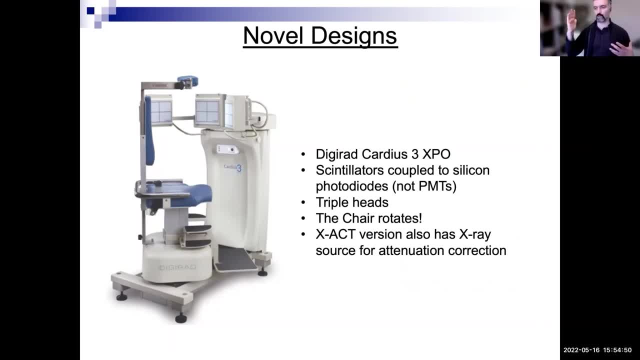 they had a very conventional planar camera and he said: well, okay, i cannot rotate this around my patient. well, why don't i rotate the patient? so there's all these designs. so this is kind of actually doing it's a, it's a triple head. instead of the system rotating, um, you could have the chair. 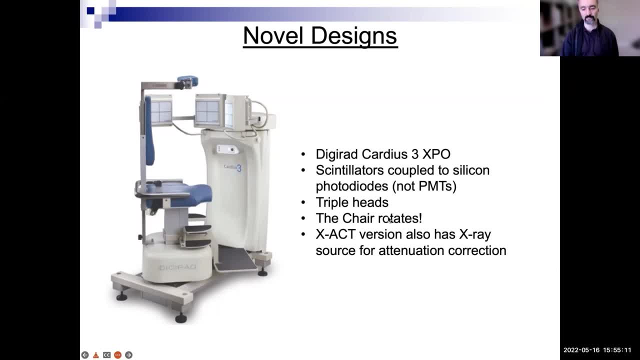 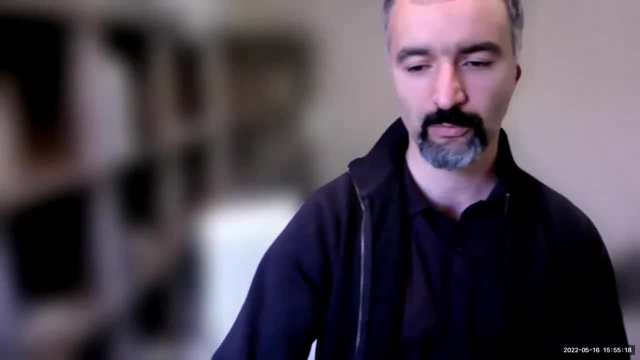 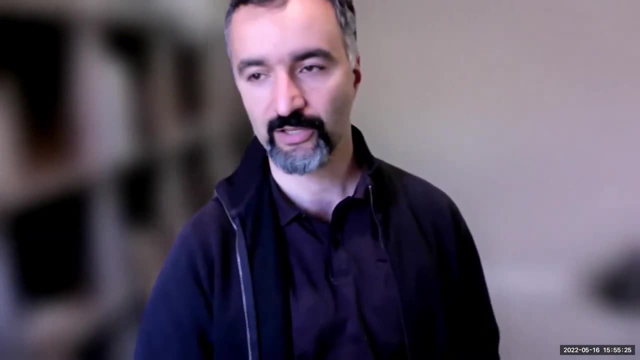 for example, rotating- okay, and you could have x-ray sources for attenuation, correction, etc. which we'll talk about more next time. okay, so i'll stop here, because next time we'll talk more about quantitative aspects, how to generate quantitative uh spec images. also, let's talk a lot more about pet imaging and also let's talk a lot more about 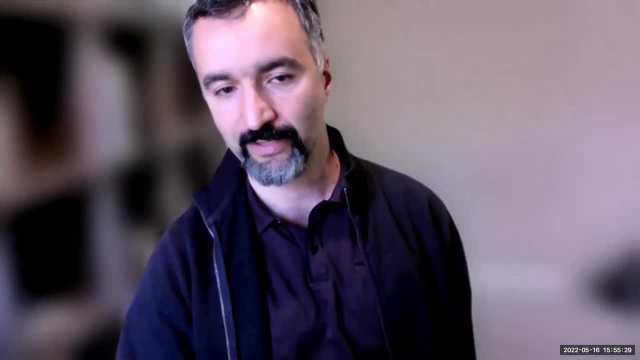 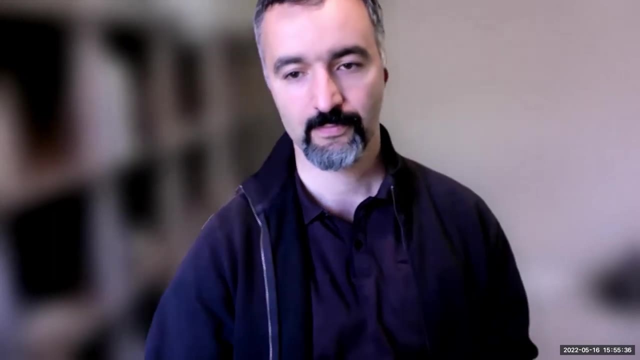 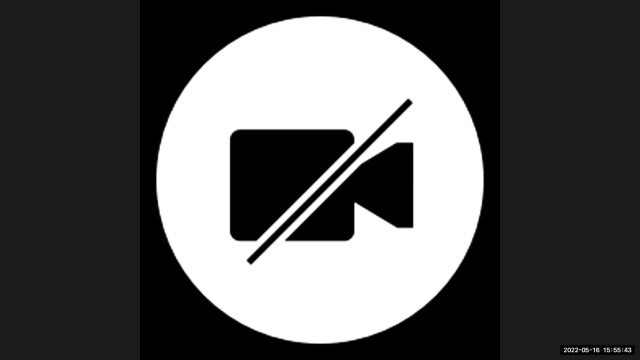 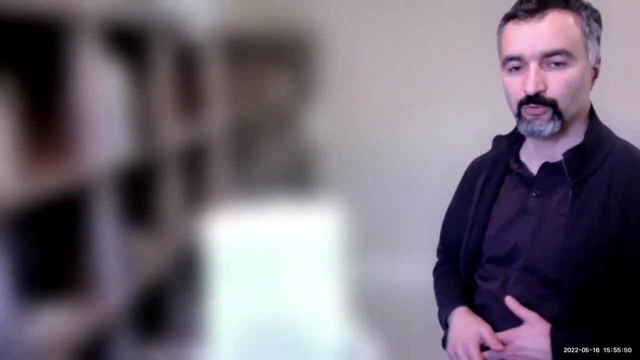 a radiopharmaceutical therapy, which is very, very exciting. okay, i'll stop here any, any questions? okay, thanks so much, thank you. thank you very much, and um, and if you have any questions, let me know and i can send you. i'll send to ali, to the other alley, i'll send her um, the um, the. 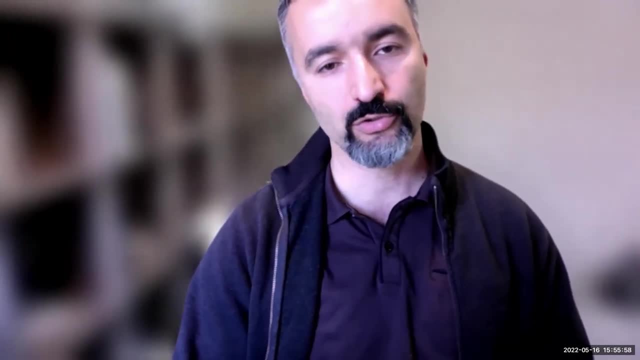 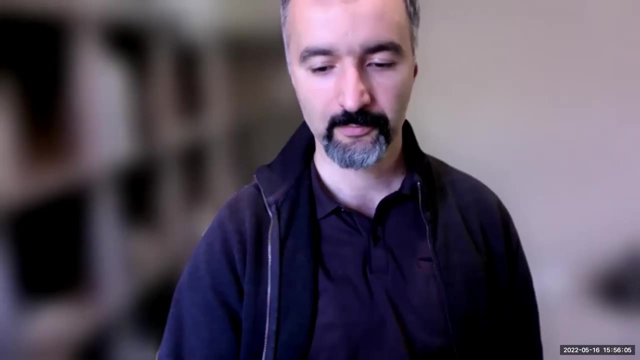 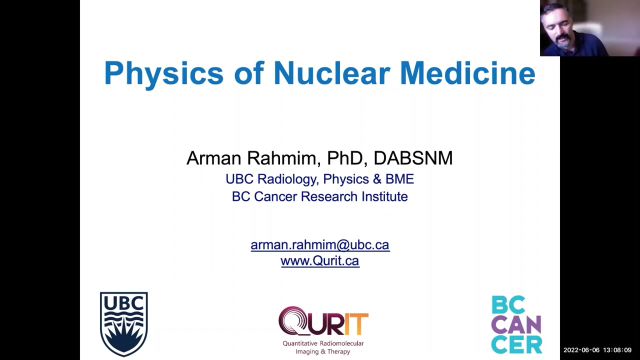 powerpoint uh, or the pdf for the powerpoint, so so you, you would be able to all look at. okay, that's great, thank you. yeah, thank you, thank you, have a great day. bye, so welcome to this uh session. uh, continuing our discussion on the physics of the. 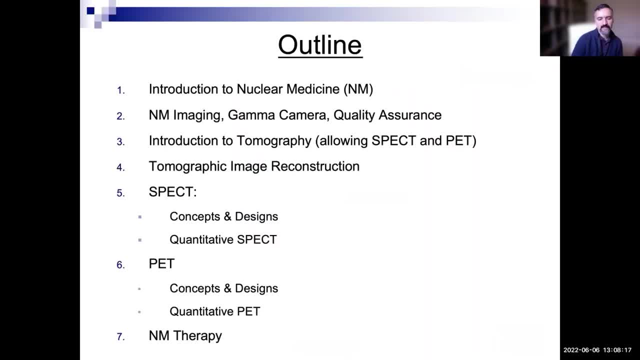 world of nuclear medicine. um, we sort of covered up to. we covered the introduction introductory aspects, uh to nuclear medicine into tomography, to, to, to how uh imaging is done, quality assurance and inspect. we looked at concepts and designs but we want to wrap that up with quantitative. 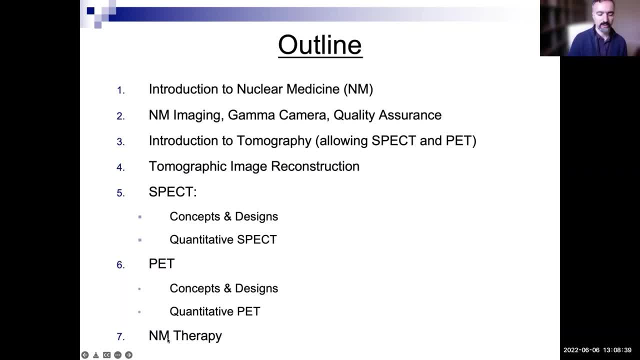 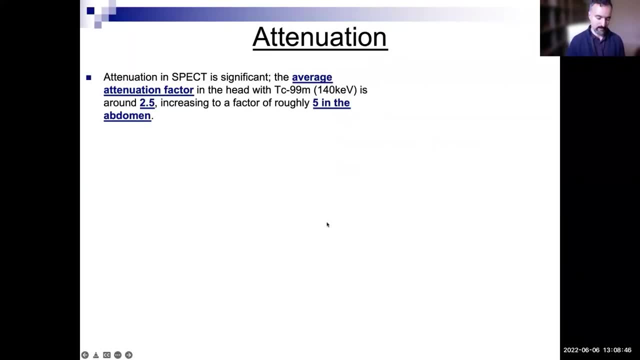 spec and how that's done, and then move on to pet and finally to nuclear medicine, uh, therapy. so, um so, SPECT has been thought for years not to be quantitative, which is not true, okay, So let's clarify that misunderstanding. It's no longer true. 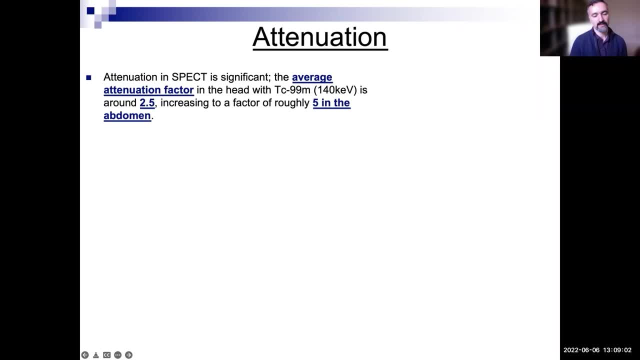 But let me explain why people thought for a long time that SPECT is not quantitative and why, in fact, it was not quantitative until people managed to fix it. So one key issue was attenuation in SPECT, For example, in the head, human head, with technetium 99M around, you know. 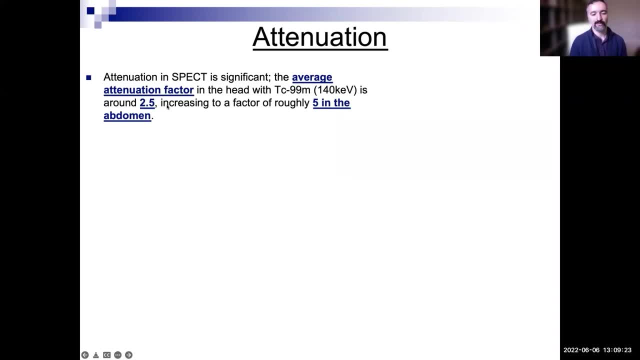 the attenuation. the average attenuation factor is 2.5, increasing to a factor of roughly 5, meaning you know when it's 5, one in five events only survive. okay. So it's a factor of 5 attenuation that's happening. 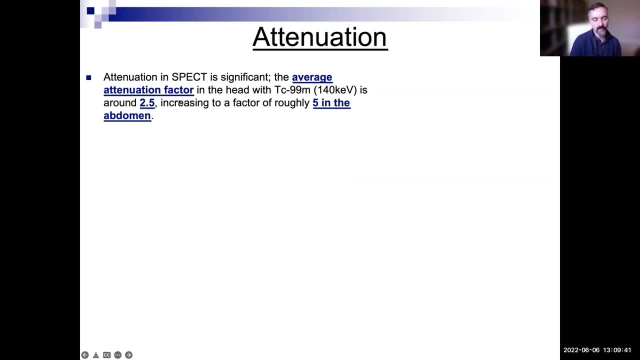 You're losing a lot of events, or in this case You know you're losing, you're only one out of two and a half events sort of survives, So something like that. So the point is that when you do filter-back, projection attenuation, correction was not done. 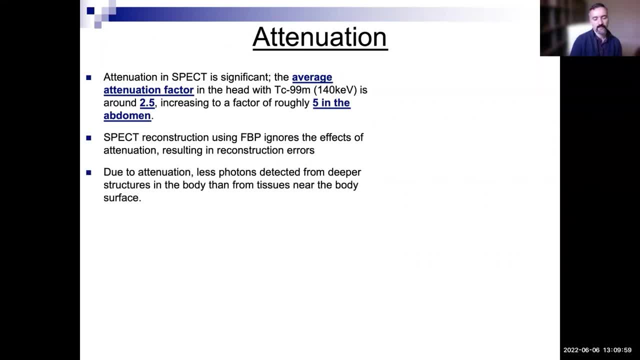 and resulting reconstruction errors. And then when you have attenuation in the body, so, for example, the radiation is attenuated, let's say through the photoelectric effect, and it's absorbed and it never makes it to the detectors. Okay, Then if it's especially deeper in your body, that's more likely to happen. 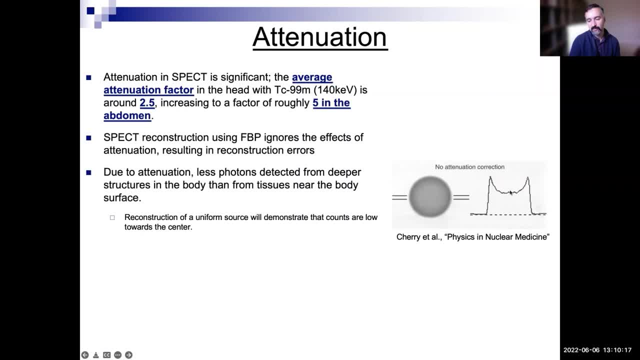 So if you actually look at some object deeper, when you do reconstruction deep within the object or the subject, you're going to see underestimations, right. So these are things that in fact, even physicians had adapted themselves to. 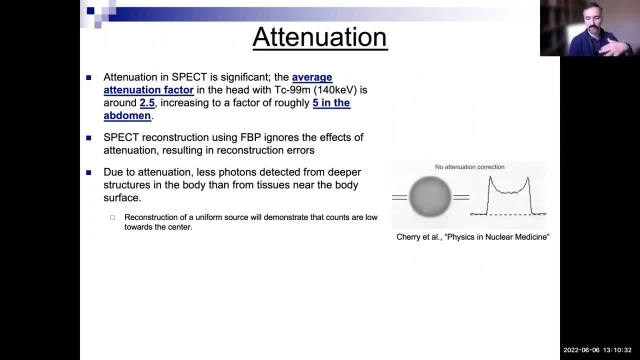 When reading an image, they're like: oh, this thing is because of attenuation, not because of an actual defect, for example. And so and the issue is that in the body we don't have uniform attenuation, So it's not straightforward. 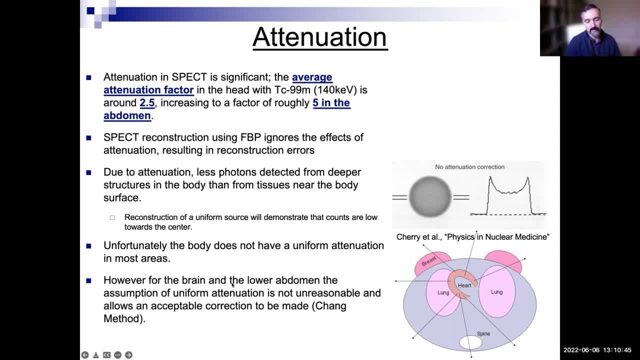 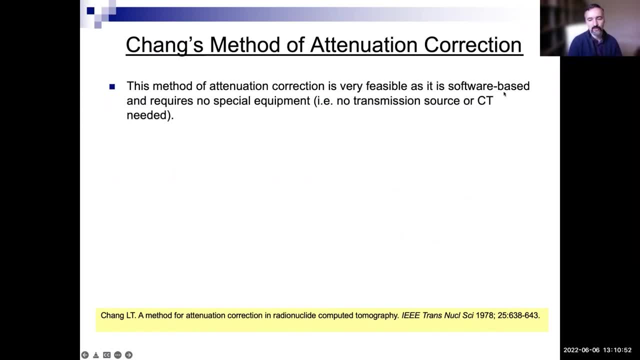 But in brain or lower abdomen, you know, you could sort of assume, people sort of used to assume, that you had uniform attenuation. So there's this thing called the Chang method that people used to use. It's a software-based method. No special equipment, like no CT or no transmission source was there to calculate the attenuation. 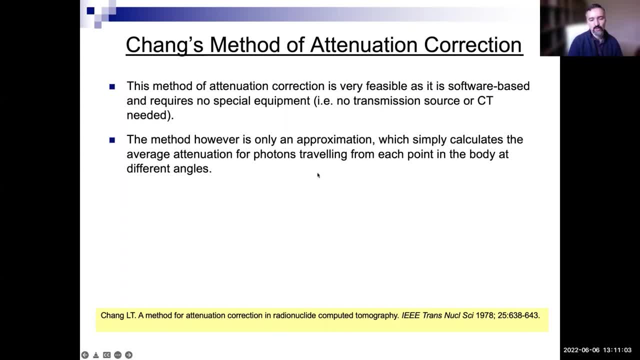 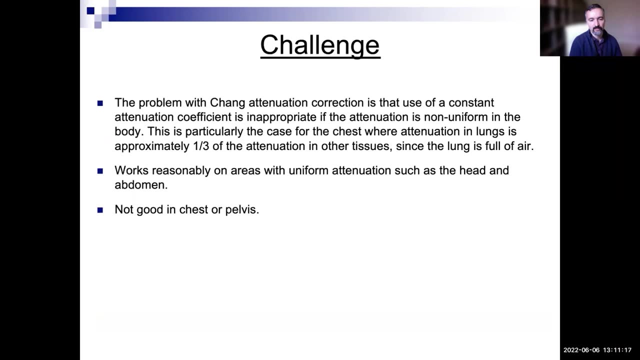 But it's still. it's an approximation which sort of assumes uniform attenuation in the body, almost like assuming the body's like all soft Tissue, for example. And so they did some kind of multiplication right. But the problem is that that's inappropriate in non-uniform body. 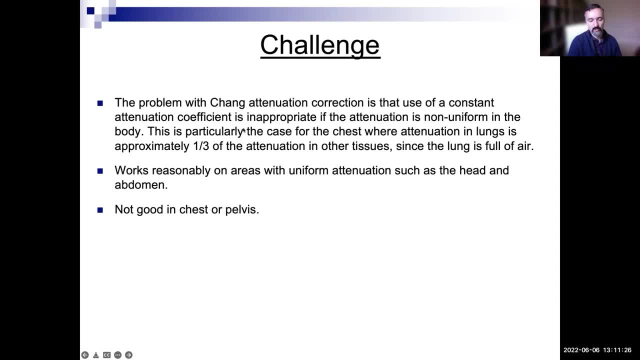 I just keep saying the same thing. you know, for chest, imaging, the lung, we've got a serious issue where attenuation is quite less than in other tissue. And so again, with head and abdomen, lower abdomen, it sort of works. 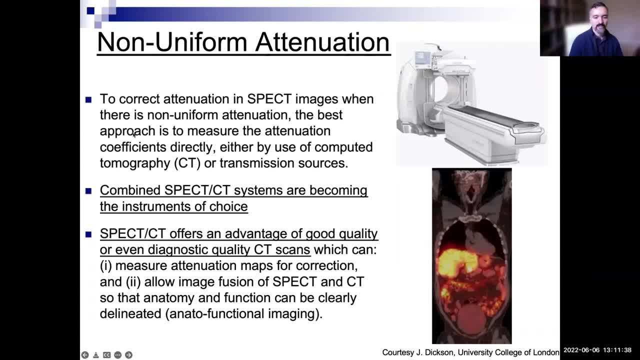 But then we, when we have non-uniform attenuation. there's a way to correct it. There's two ways to work for it. One is use CT, like in a spec-CT camera, which are increasingly utilized, Or using some kind of a transmission source, almost like a low-cost version of CT. 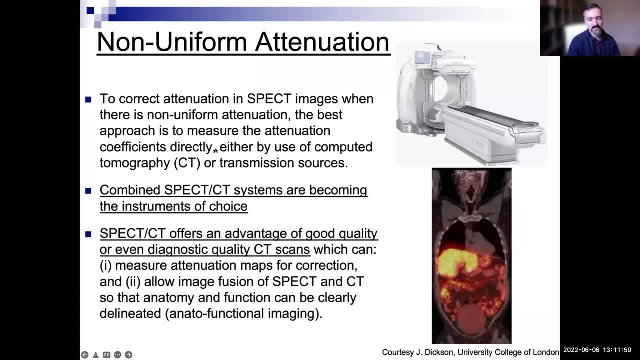 where you have something sort of going around, kind of the same concept as CT, which is what used to be used before CT and spec were kind of merged together. But again, spec-CT is becoming the instrumentation of choice for quantitative imaging because you could do the CT at a very fast time. 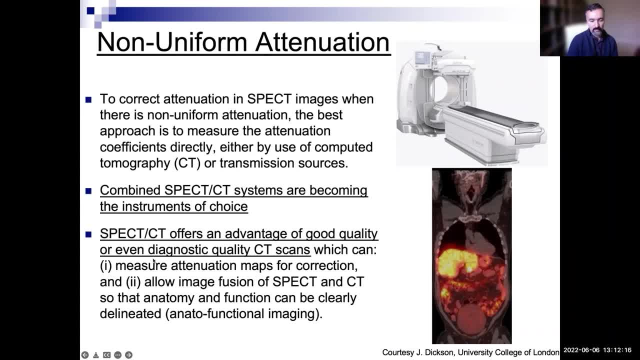 and you get very reliable numbers, And so you measure the attenuation maps and then you allow, so you use those attenuation maps to correct for attenuation in the reconstruction of SPECT. Same thing is, by the way, true for PET. We'll get to that later. 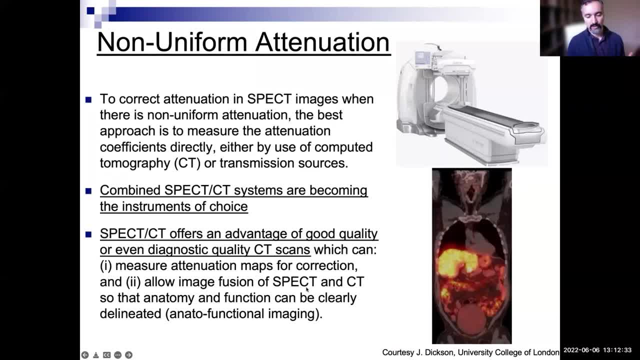 Also, when you have SPECT and CT, that allows you to do fusion of imaging like, let's say, anatometabolic imaging or anatofunctional imaging- you know, depending on what function SPECT is imaging and anatomies being measured by CT. 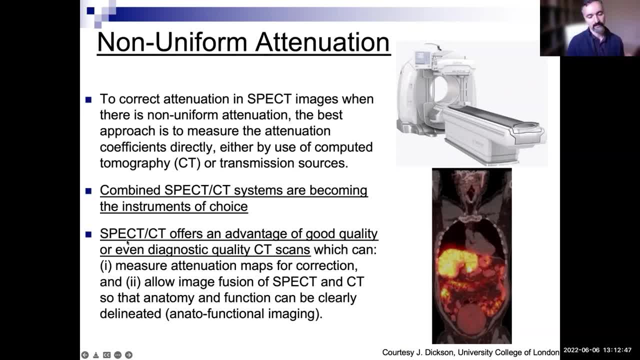 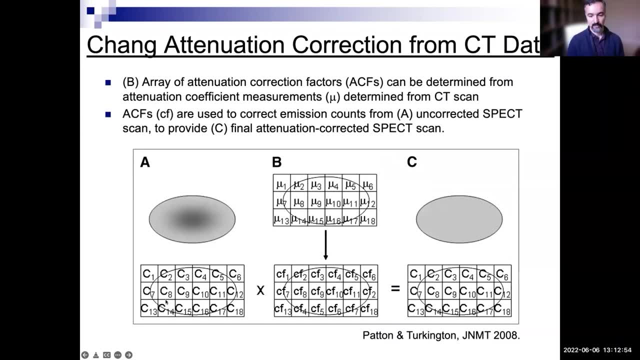 So merging has two advantages: You get more quantitative SPECT and also, just from a clinician's perspective, having fused images is valuable. So again, Chang correction method- you sort of assumed- oh well, I already talked about that- using uniform data. 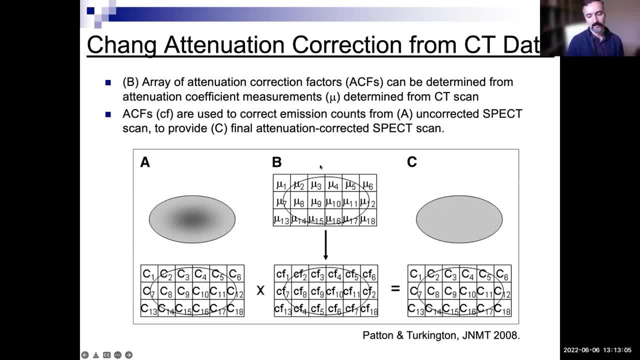 but you could also, you know, take the measure attenuation coefficients from CT, for example, and you could also, you know, take the measure attenuation coefficients from CT, for example, and you could also, you know, take the measure attenuation coefficients from CT, for example. 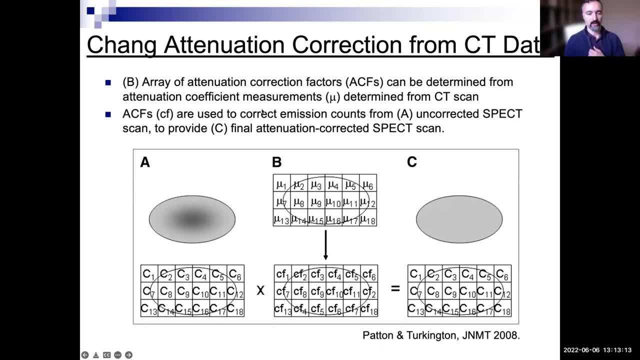 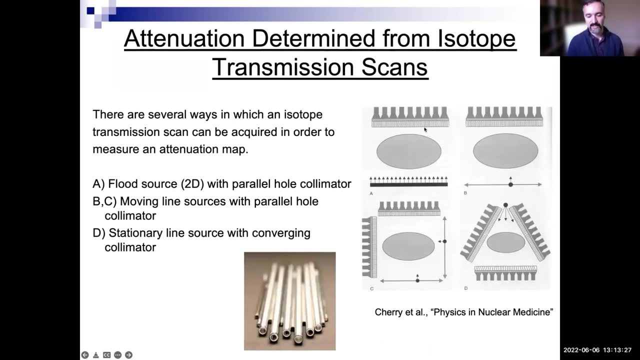 and you could also, you know, and then you could calculate the attenuation correction factors. So this is kind of like a Chang method, but benefiting from the CT data, and you could get quantitative numbers. So instead of CT you could also use transmission scans. 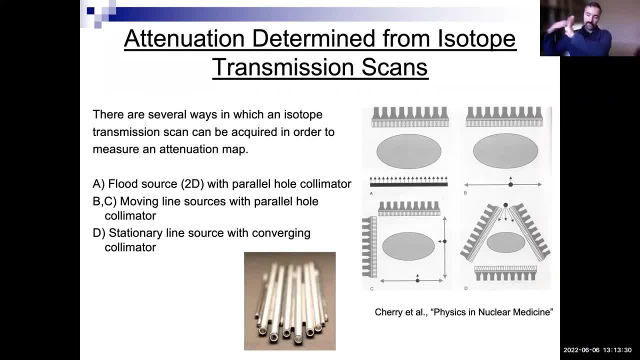 This is what used to be done. So either there was nothing being done or there was transmission sources, but then increasingly there's use of CT. So when you have a transmission source, you're basically having this hot rod, for example, like it could be a moving line source, right? 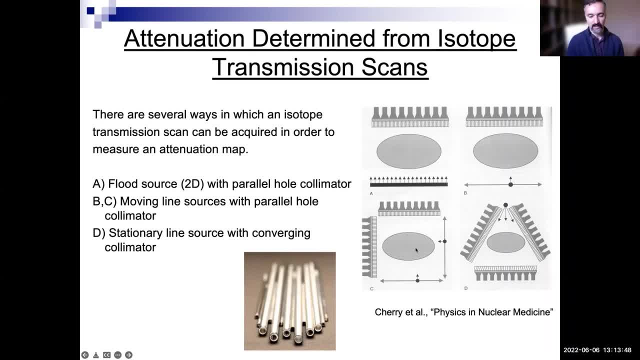 Or a stationary line source with converging collimator, as we were sort of having here. This is actually a line if you look at it this way, But again, so you could be. essentially, the point is to expose your object with transmission coming from outside. 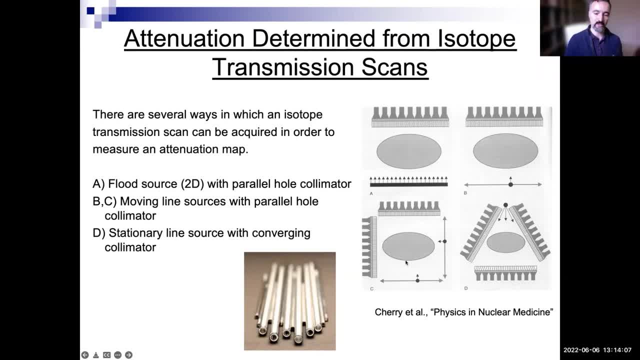 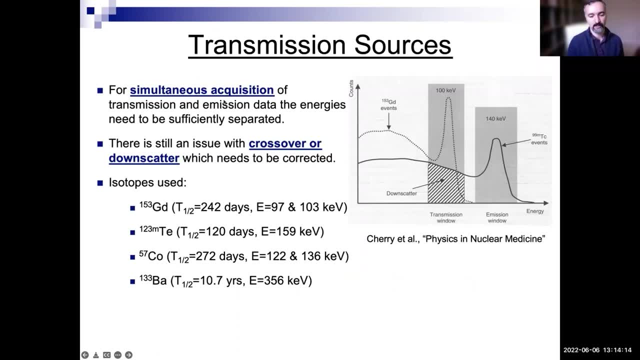 the same concept as CT and that allows you to measure how much attenuation is happening. So you could also in the past- especially people again when transmission was more and more popular- you could do simultaneous acquisition of transmission emission. You still do. 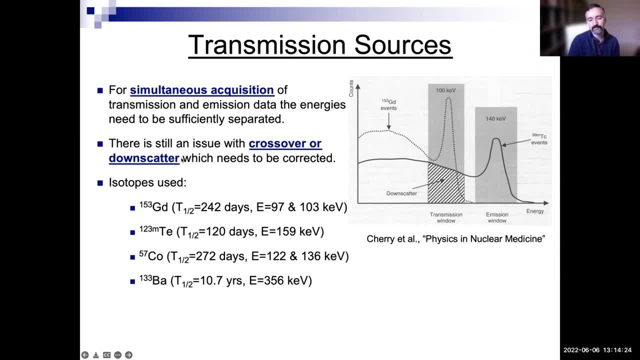 You can, But there's gonna be a bit of crossover because if this is your transmission window, let's say you've got something that, for example, you've got gadolinium-153 at 97,, around 100,, for example. 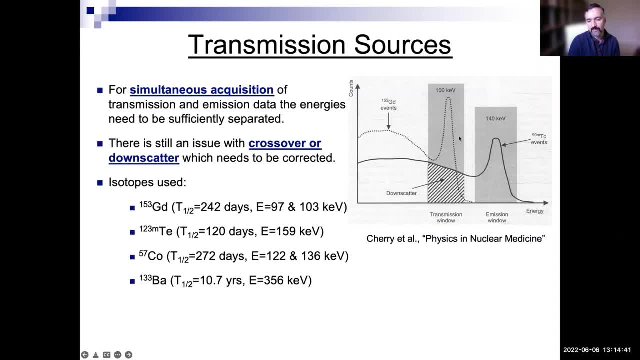 If you've got, you put this energy over that for transmission measurements and this energy over the technician 140 kV for emission. But there could be crossover, Like if an event is coming here but it's scattering in the body, lowering its energy. 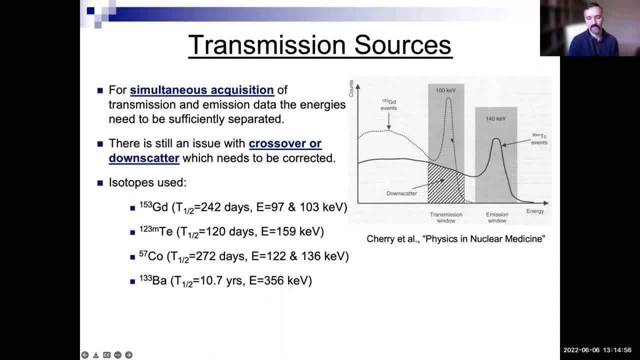 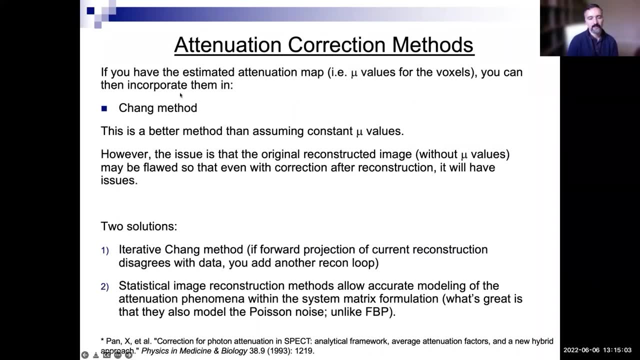 by the time it arrives at the detector it might be in this window and it might confuse things. So there's a lot of work, research, on how to deal with these things. So if you have an estimated attenuation map again from CT or whatever, you could use. 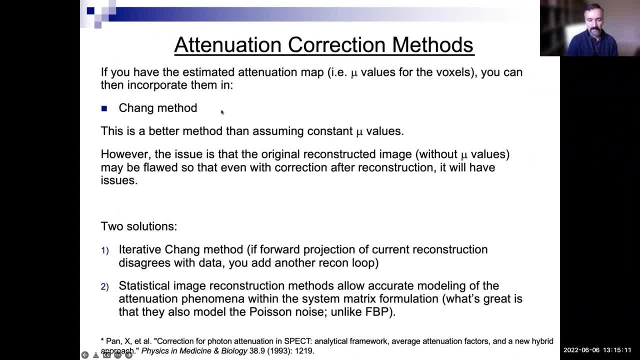 the Chang method. The issue here we're having with the Chang method is that it is being based on the. you reconstruct an image and then you correct it, But that reconstructed image, the original one itself, is wrong. So you could do iterative Chang. 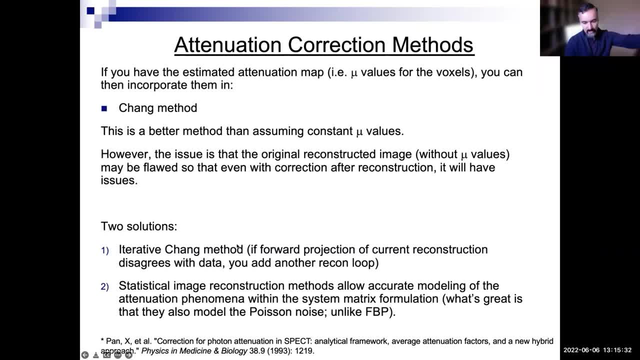 but honestly, people are moving away from this And Chang is not in the picture too much anymore. People are really converging towards statistical iterative image reconstruction where you can really model the attenuation factors within the reconstruction. So, if you wanna remember, one thing is the fact: 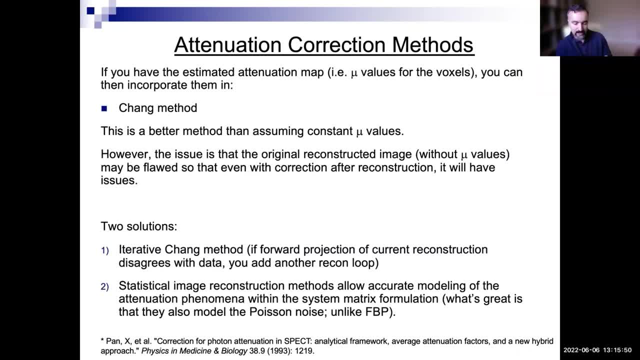 that field of nuclear medicine, ahead of the CT world, really started to converge on using iterative statistical imagery reconstruction, giving you truly quantitative reconstructions in both SPECT and PET. So SPECT is now quantitative if you're doing CT or transmission to measure attenuation. 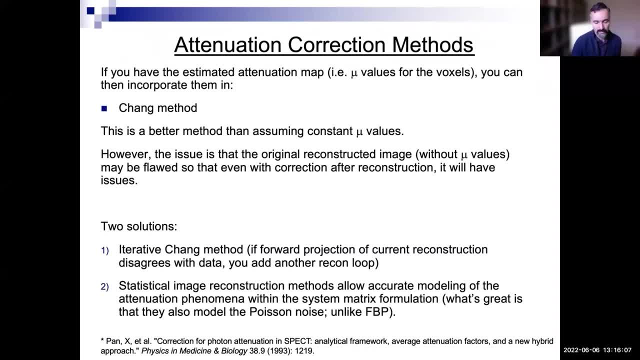 and then the CT world, of course, has arrived in the C-23, it's doing increasing or iterative reconstruction. The nuclear medicine was ahead of the city world in doing this And partly, as I mentioned last time, this was because we were limited in count. 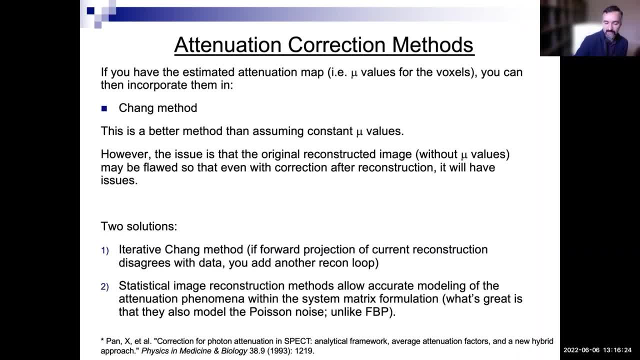 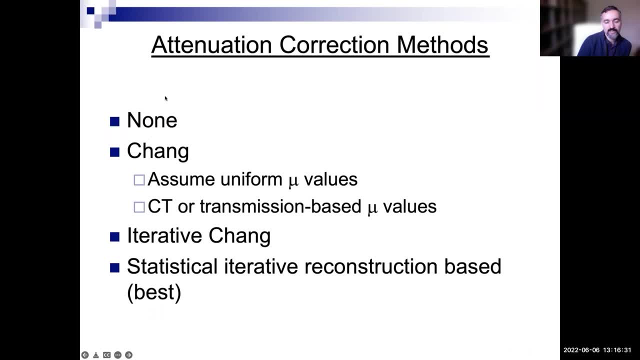 and therefore you're getting noisy images and you felt the urgency to use image reconstruction, that in an iterative, statistical way, and results were great. So, again, people used to do nothing. You know some doctors to this day just are used to looking at non-attenuation corrected images. 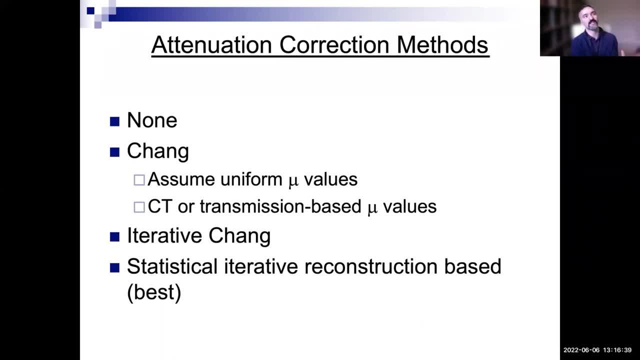 and just sort of figuring out if this is an artifact of the recon or if this is a real defect, let's say myocardial perfusion defect. But then Chang came in and then iterative Chang. but really the best approach is statistical iterative reconstruction. 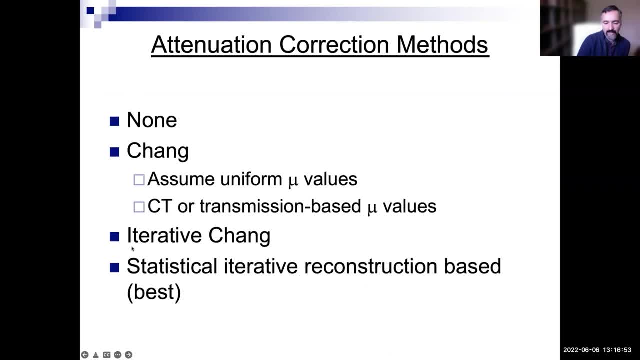 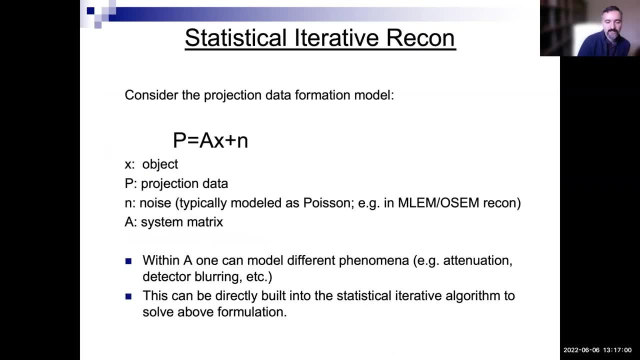 Of course, nowadays people are also looking at incorporating AI-based methods, artificial intelligence-based methods, as the next generation of techniques. So, statistical iterative reconstruction. the concept is that you have some image, let's assume you know the truth. If you know the truth using the so-called system matrix, 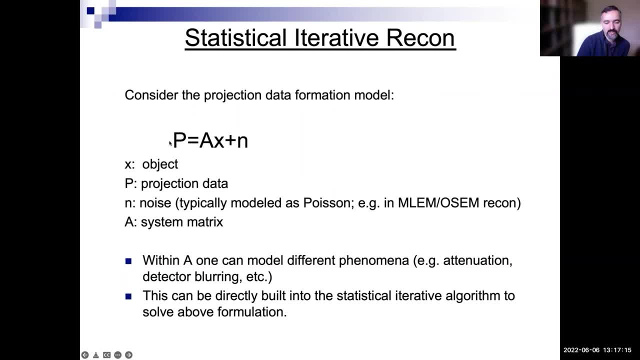 which models the relationship between the image space and the projection space. you can calculate what the projection space is And then you can sort of model the fact that there is noise being added to it, like Poisson noise. So if you have such a system, 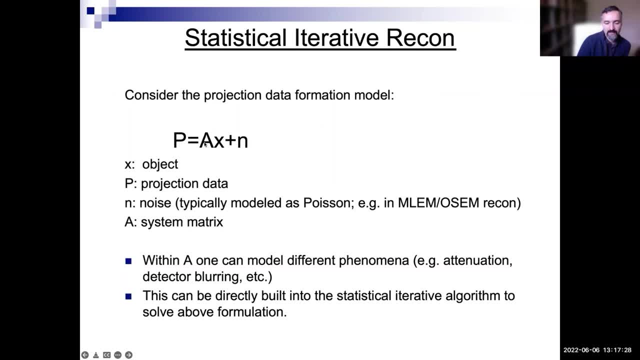 you can actually within A, within the system matrix, model how much attenuation is happening, because your CT gives you how much attenuation is happening. So you could actually build this and then when you do reconstruction based on this formalism, you could model that. 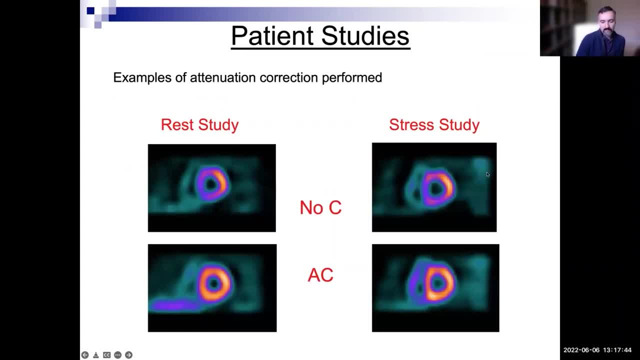 So here are examples of rest and stress, myocardial perfusion studies, And with no correction. you get these kinds of things For a normal patient. you see clearly, you see some kind of artifacts, but this is not a real artifact. This is not a real defect. 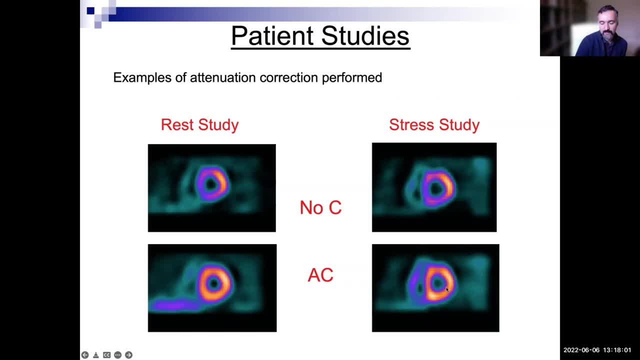 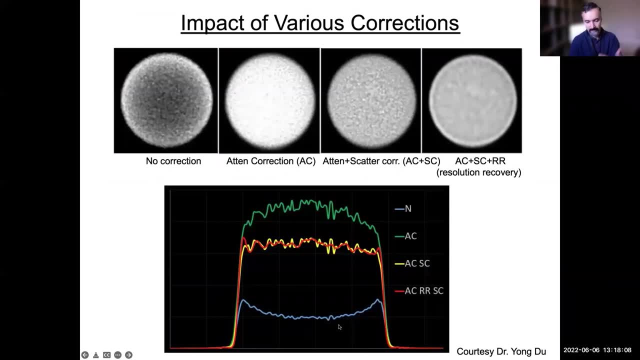 This is an artifact, Whereas once you do attenuation correction you get these images. So we talked about again no correction. You see this sort of drop dip in the middle. After you do attenuation correction, something funny or bizarre happens. 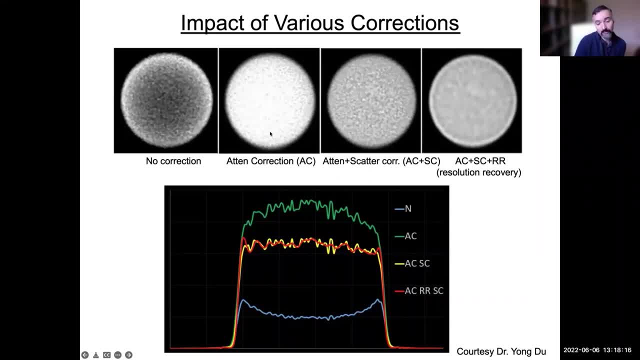 People initially were like, look, we told you not to do attenuation correction, because once you do attenuation correction instead of a dip you almost have a like you kind of have a awkward trend, okay. So they're like, oh, something's wrong here. 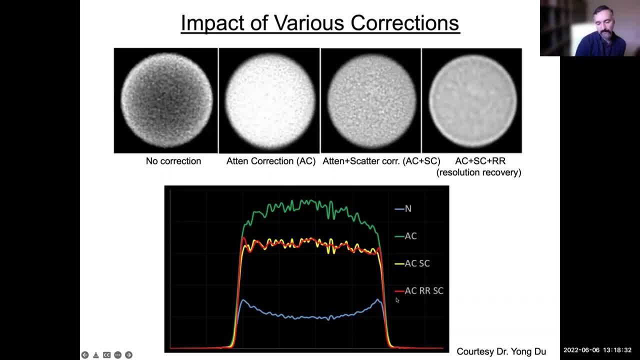 Why isn't this flat? Well, guess what? Sometimes, when you correct for a big issue, the smaller issues start to show up. This is now another issue. You have taken care of attenuation, but another issue shows up, and that's the issue of scattering. 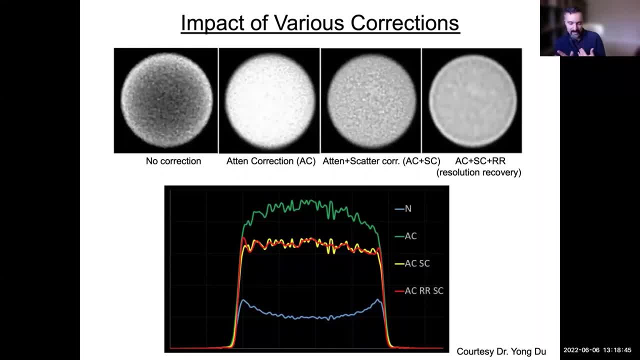 Attenuation is when you lose events and the event that was intended to be detected at a detector was never detected, But if, in the meanwhile, you also have scattering and the event is being scattered but being detected in the wrong place. Now some of the detectors are detecting more things. 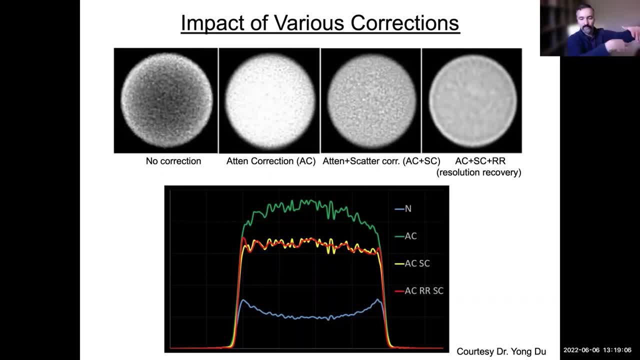 than they would have, because, again, just scattering is moving in that direction. So you need to then correct for a scatter And once you do that you get this nice flat distribution. There's other things like resolution recovery. that makes images sometimes look smoother and even sharper. 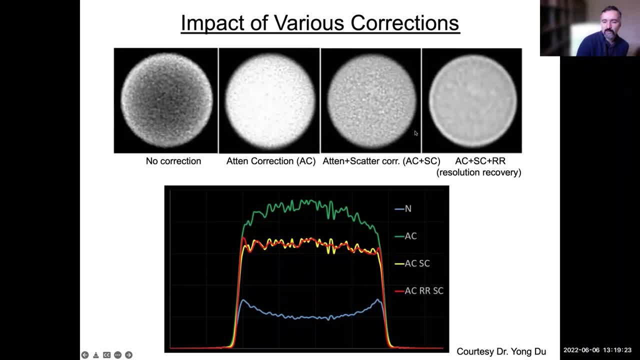 but then they might give you some edge artifacts, But essentially there's all these corrections people work on, And so we've gone from having an image like this, which doesn't look good at all, to images like this and that, which look quite better. 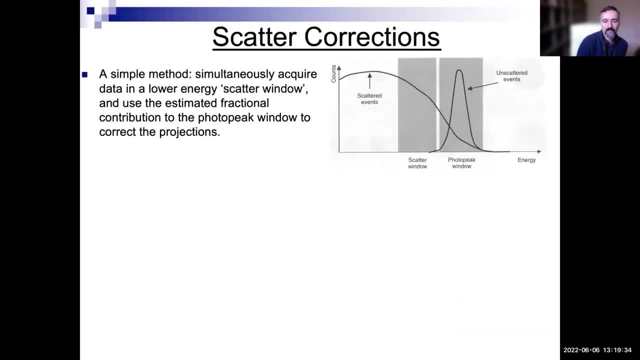 So scatter correction. there is a simple method to do scatter correction And that is by putting a lower energy window to actually measure how much scattering is happening, because those are the lower energy events that are coming here. And when you measure how much scattering is happening here, 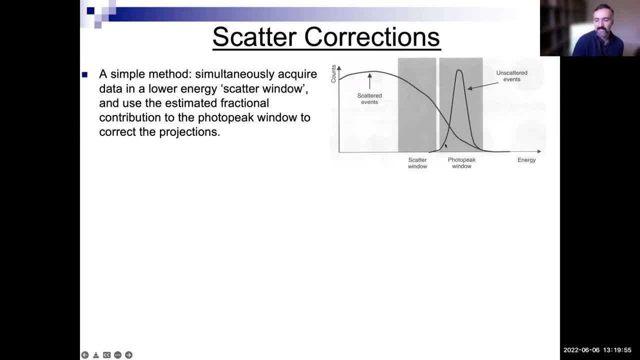 you can sort of extrapolate about how much scattering, because here you don't know, Here you're receiving a bunch of events. Some of them are real events, some are scattered events. Which one is, which we don't know. But if you put an energy window here, 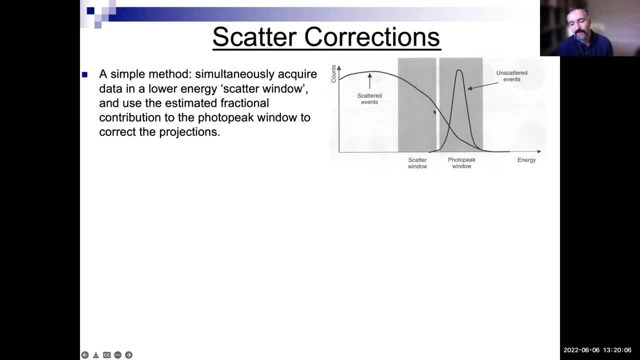 you kind of have an estimate of how much stuff is here. You kind of using mathematics or interpolation or extrapolation, you kind of calculate how much of this would be here, And then you would subtract this amount from that to get the true images. 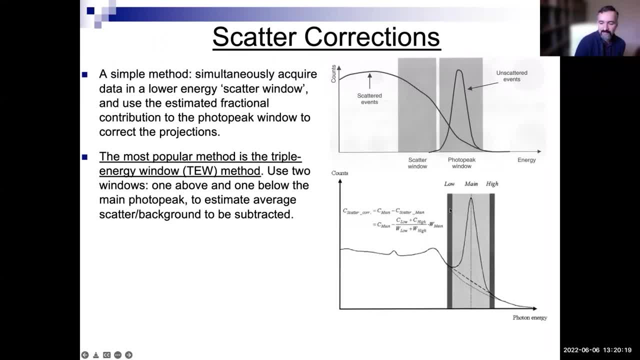 Or you could use triple energy method, When you put an energy window below your photo peak window and above it, and then you do average in between what you measure here and here to estimate how much scattering is happening there, and then you subtract, And then there's other advanced methods. 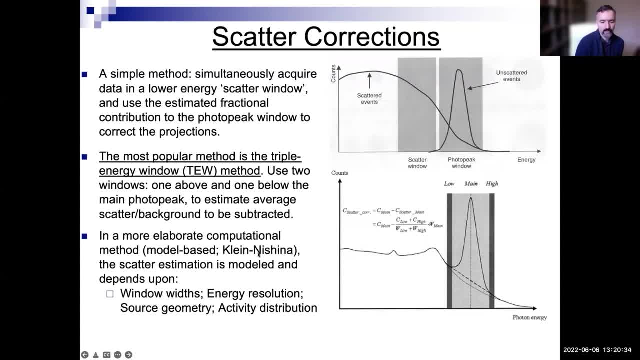 like advanced modeling using Klein-Nishino forms, et cetera, et cetera. So there are other methods And you start with an initial image estimate, You estimate the scatter based on that, Then you correct for it, et cetera, et cetera. 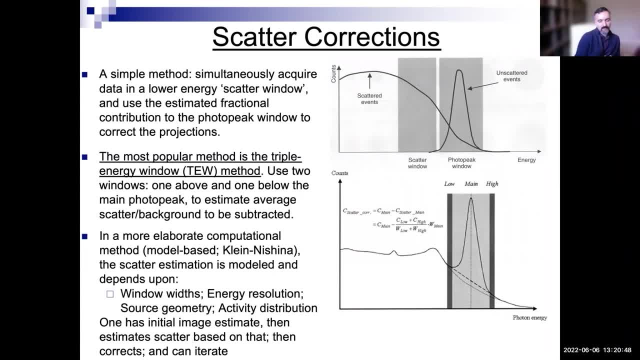 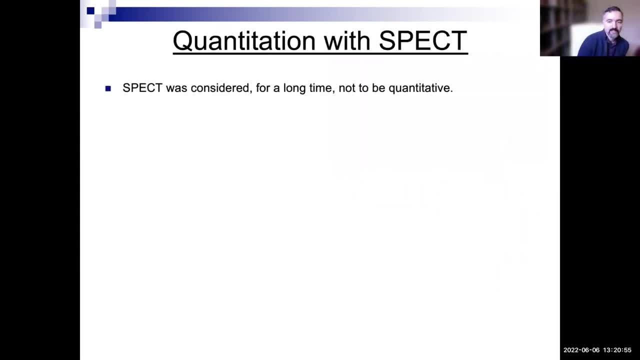 It's kind of analogous to iterative chunk: You start with something, Based on that you get a new image, update And based on that you keep updating yourself. So I again want to emphasize: SPECT was considered for a long. 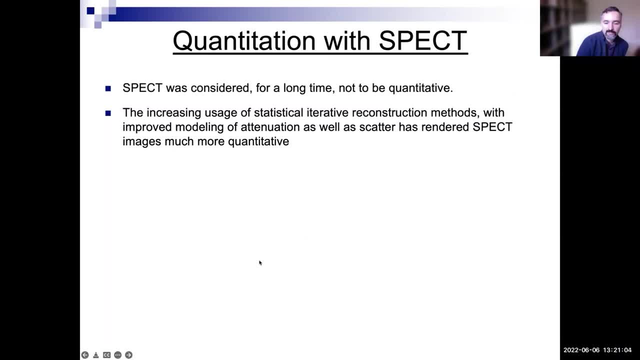 time not to be quantitative, But increasing use of statistical iterative recon with improved modeling of attenuation as well as scatter, has really made it much more quantitative. There are other things you could model, like collimator detector blaring, Like the collimator scattering or entering the detector. 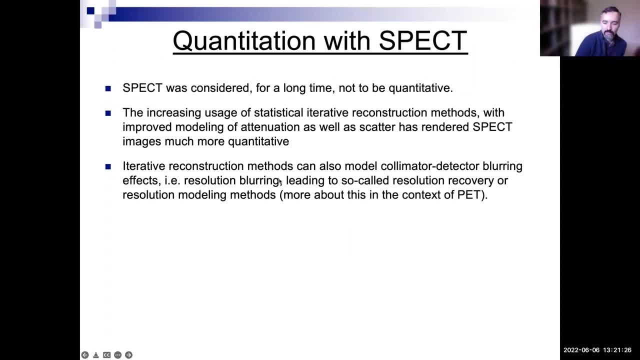 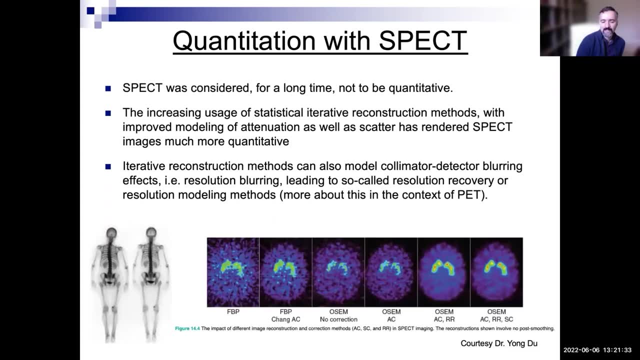 but then scattering to the nearby detector. You can actually model these things, the resolution recovery or resolution blaring That ends up giving you a typically sharp looking images which can be advantageous for certain applications. So again, example of just good old filterback projection. 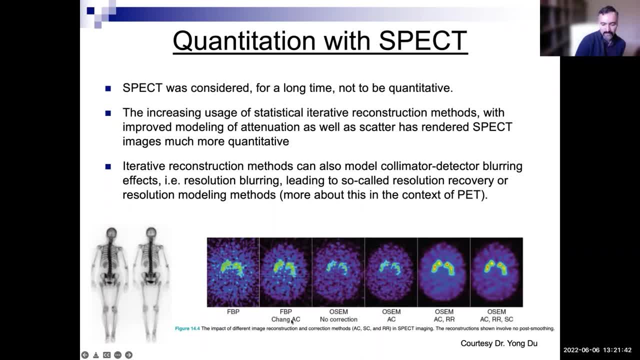 with no correction: Filterback, projection with Chang, attenuation correction, And then you switch to iterative statistical methods, the so-called order, subset, expectation maximization method And the images you see, And then you add attenuation correction, And then you add resolution recovery. 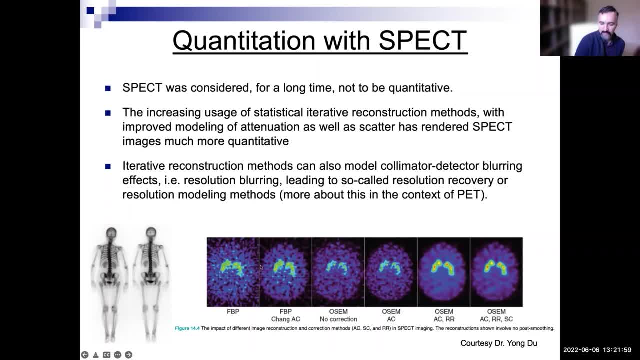 And then finally you add scatter correction. You see, gradually The images have gotten better and better. They tend to be sharper and less blurry. Just overall, there's been tremendous improvements in the quality and quantitative accuracy of SPECT and PET images. 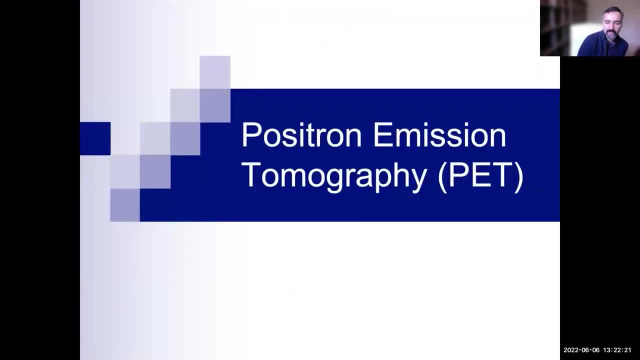 So images have become more quantitative, So you could assume SPECT is quantitative if you're doing proper corrections. OK, So let's move on. Let's move on to PET. Please stop me. if you have any questions, Let's move on to PET. 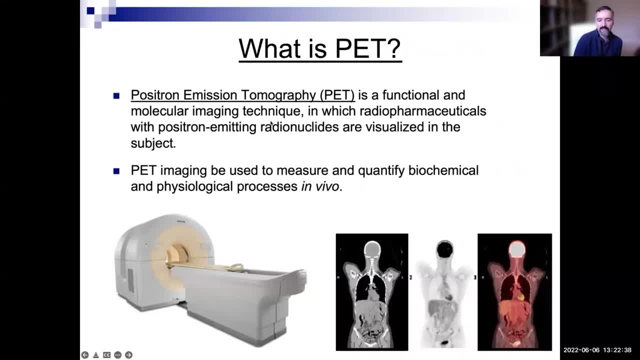 So what is? PET Stands for positron emission tomography. It's a functional and molecular imaging technique in which radiopharmaceuticals that emit positrons are visualized all right, And it allows you to quantify them too. It's not just about looking at pretty pictures. 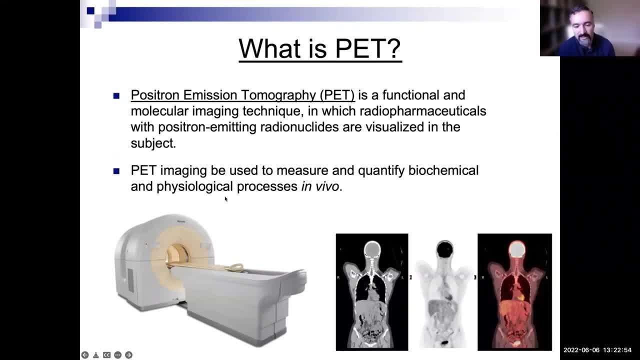 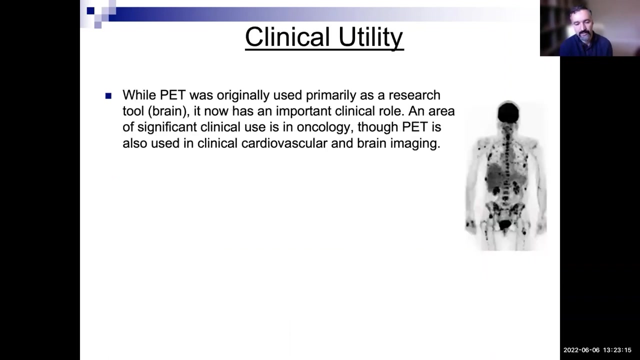 You can get numbers So you can actually quantify these biochemical and physiological processes in vivo. It's extremely powerful. It can quantify physiological, biochemical, molecular phenomena with exquisite sensitivity, like peak comolar sensitivity, for example. Originally, PET was used as a research tool in the brain. 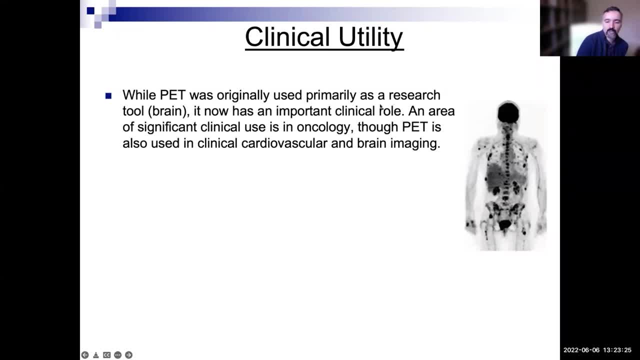 But then it took a very important clinical role. There was significant clinical, subsequent clinical use in oncology. But PET is of course used in other frameworks too, for cardiovascular imaging and brain imaging, The most widely used. so just to comment here: 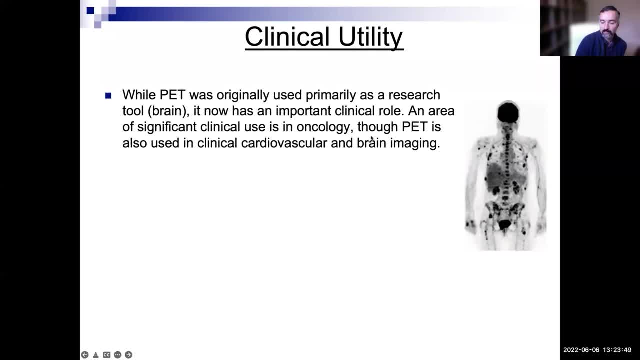 originally it was brain research, But now it has clinical brain applications too. right So for, let's say, for amyloid imaging in Alzheimer's disease, But the most widely used radiopharmaceutical or a radiotracer. the reason we say radiotracer is because 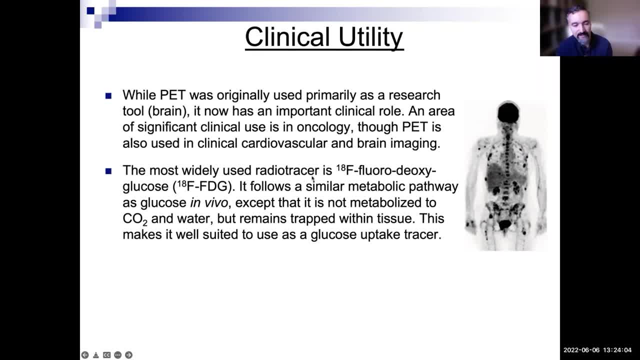 you use small amounts of it for imaging When you're doing therapy, as we'll see later. then the word radiotracer is not appropriate. It's radiopharmaceutical. So I myself tend to increasingly just say radiopharmaceutical. 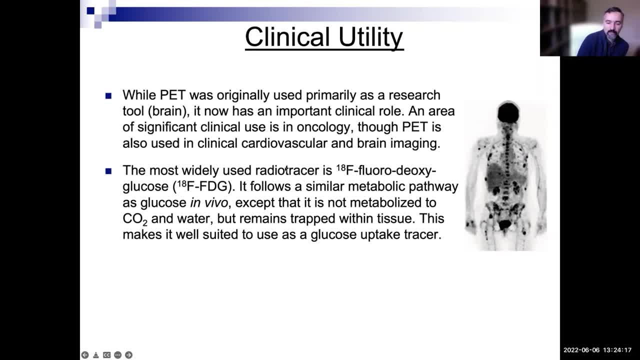 The most widely used radiopharmaceutical is, or radiotracer is, fluorodeoxyglucose, labeled with fluorine 18.. Has similar metabolic pathway as glucose in vivo, but it's not metabolized further down the chain. We'll see this in a second. 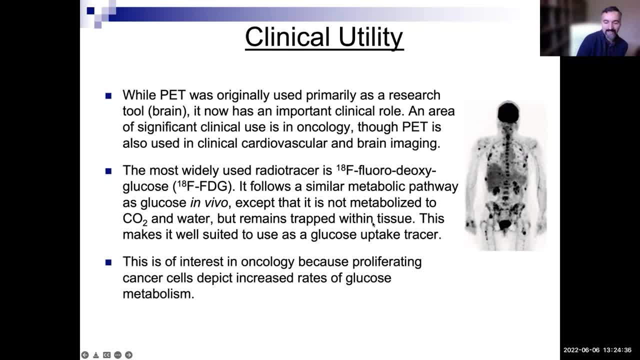 And it but is trapped within tissue and it accumulates. That's why you can see tumor and increase metabolism, increase metabolic activity that is created by tumors. So this is, and this phenomenon, this phenomenon is of interest to oncology, but also well, because proliferating cancer cells 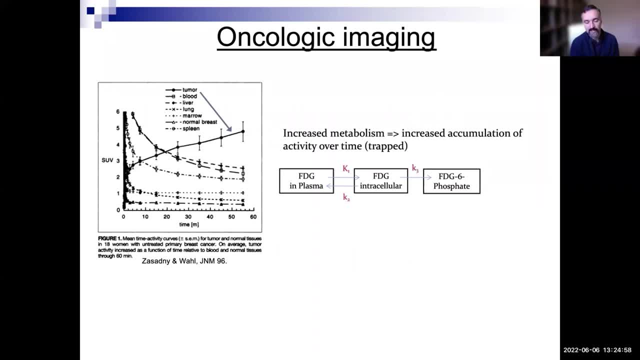 they pick increased rates of glucose metabolism, as you know. but there's other applications to it. But here's an example. You're having a subject injected. You wait for, let's say, 60 minutes typically in the clinic. then you do imaging. 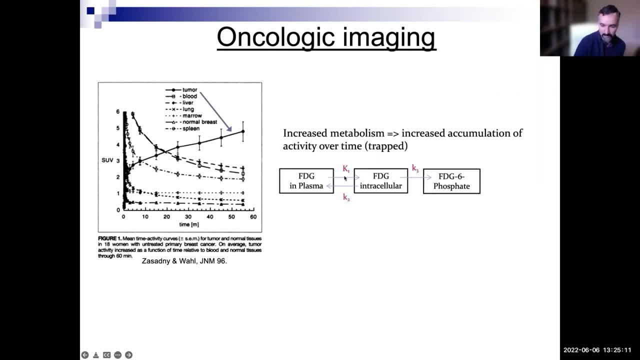 You can sort of see that because of this trapping mechanism. So this is fluorodeoxyglucose in like. sometimes I call it radiolabeled sugar, which is not precise, but it just gives you a picture of things. Fluorodeoxyglucose in plasma enters the intracellular space. 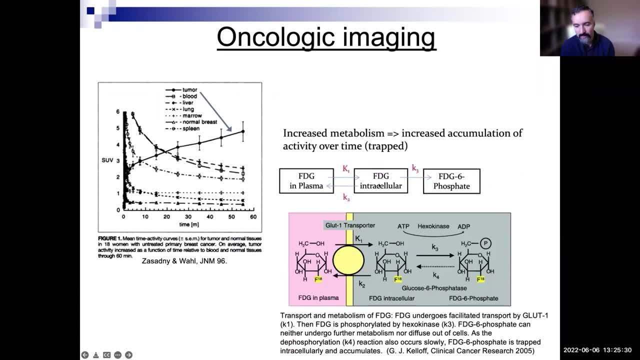 This is an oversimplification. There's more compartments, but you can sort of think of it as intracellular space. And then finally there is through. there's a phosphorylation that happens by hexokinase, And when phosphorylation happens, 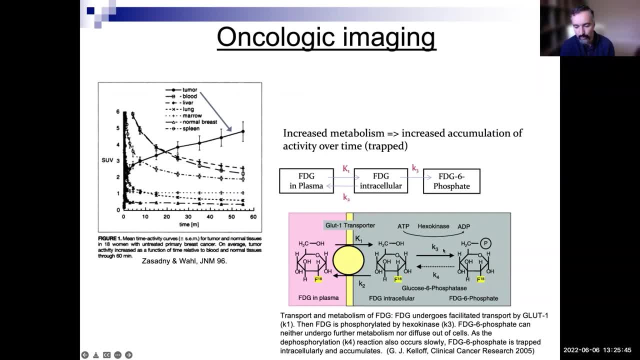 then you have fluorodeoxyglucose 6-phosphate, and it gets trapped here. It can no longer undergo metabolism or diffuse out of cell. It gets trapped here And that's kind of nice actually, because it accumulates, for example, in tumors. 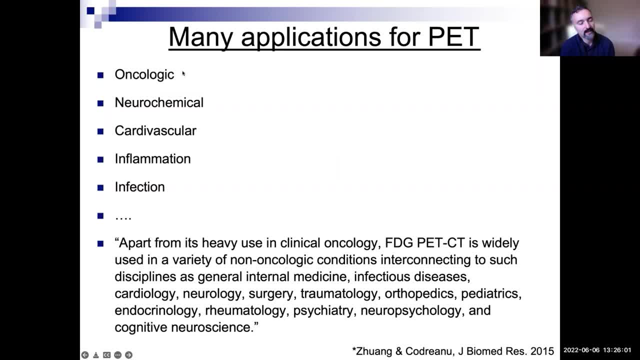 and you can sort of visualize. But again, the only application of FTG is not oncology, though it is. the work force of PET is in this space, but there's so many other things happening: inflammation, infection, et cetera. 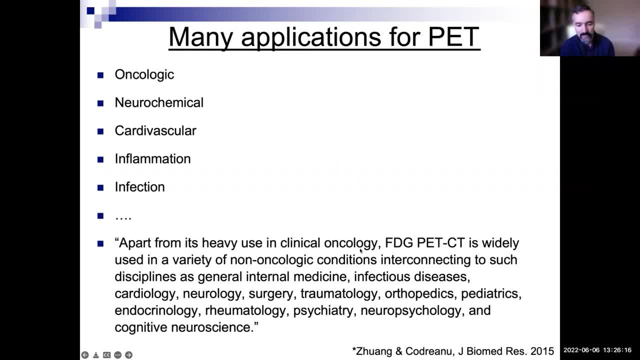 Apart from just a quotation here, apart from it's heavy use, FTG PET-CT is widely used in a variety of non-oncologic conditions interconnecting to such disciplines that generate intra-medicine infectious diseases. we sort of said that. 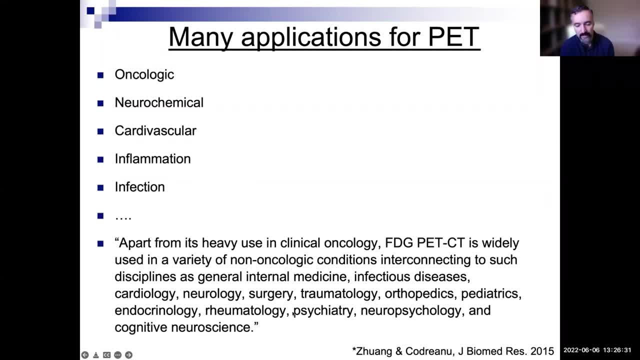 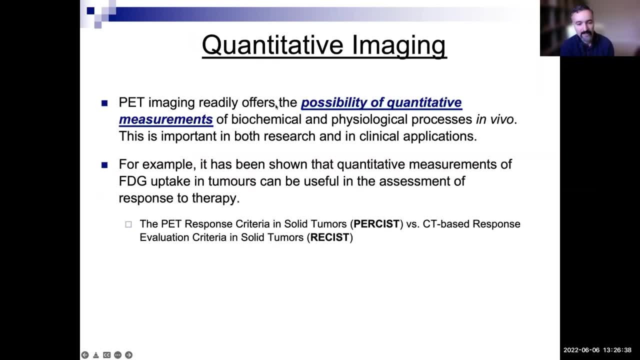 Here: cardiology, neurology surgery, dermatology, et cetera, Many, many, many, many, many many frontiers. And again, PET allows you to quantify phenomenon processes. For example you could consider looking at: 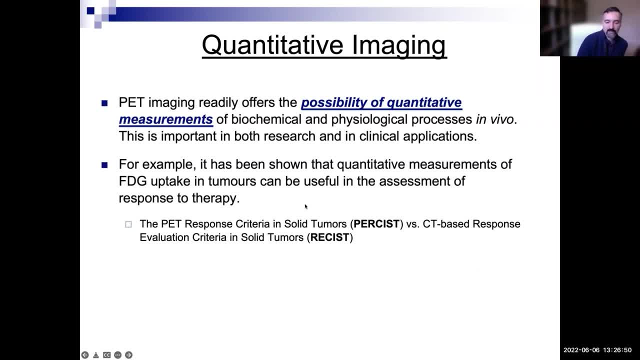 assessment of response to therapy, even subtle changes. Right, so you've heard of resist criteria in using CT-based response evaluation in cell tumors. Well, there's the PET version of that. the so-called PET response criteria in cell tumors persist, which can be very powerful. 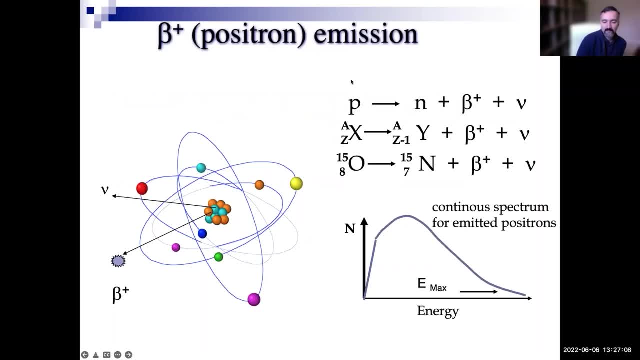 So how does this happen? Basically, in this phenomena, what you have is a proton giving rise to a neutron plus a positron. Now, this is a neutrino and it doesn't really matter for all practical purposes, but these two matter. 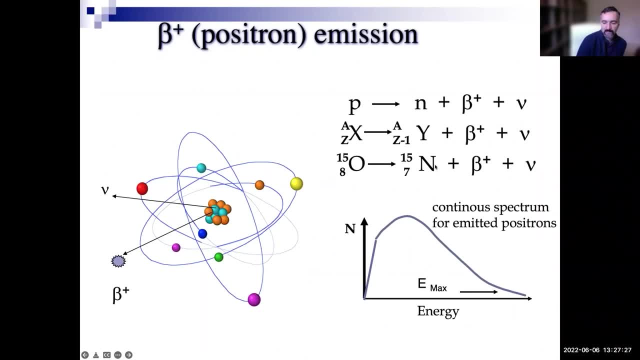 And so, for example, if you have oxygen-15, that gives rise to nitrogen-15, with a positron, And that positron is emitted with a range of energies, And then, after that positron is emitted, it might travel a little bit, 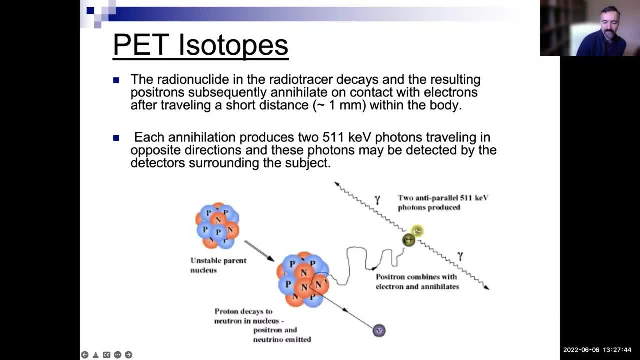 So here's an example Again you've got an unstable parent gives rise to a daughter and in that phenomena releases a positron. A positron is a positive electron, same weight. It's an anti-electron- same weight, just positive. 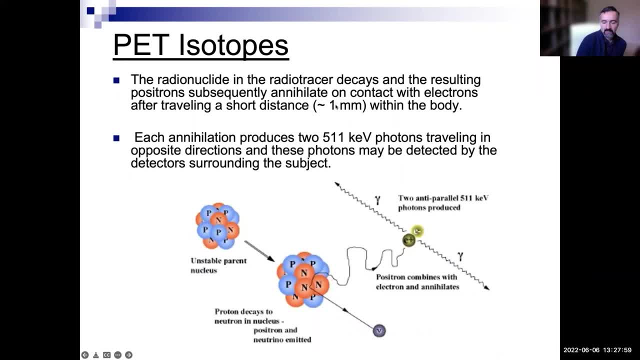 And then it travels a little bit. often less than one millimeter depends on the rate of pharmaceuticals. Some radiopharmaceuticals give you more energetic positrons and some give you less energetic positrons. So, for example, in F18,. 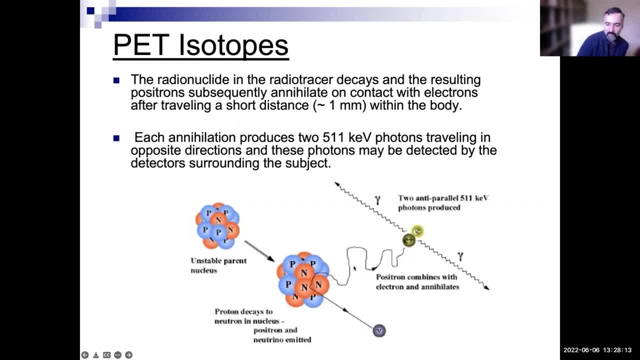 this number is actually less than one millimeter, So after traveling a little bit. then it combines with an electron. the two of them annihilate and give rise to two photons. This is a classic example of E equals MC squared the original. 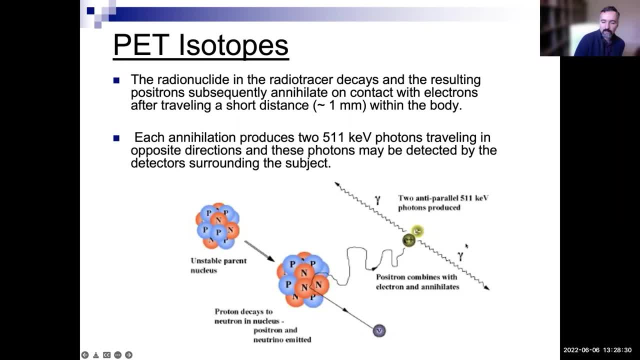 rest mass of the electron positron is obliterated and you only get photons left and these two anti-parallel 500 keV photons are generated. notice the energy is quite high. it's not like 140 keV for spec. so we got an issue: PET. this is why PET is so expensive, because these are highly energetic. 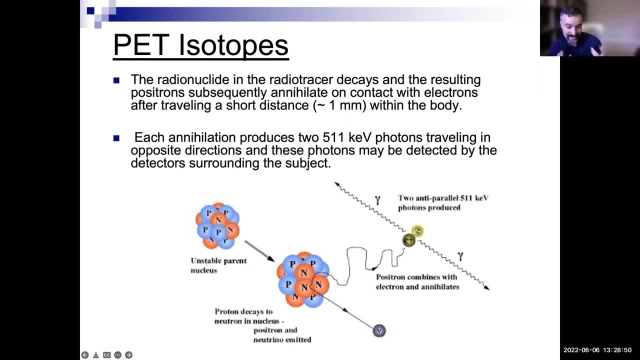 photons. so you got to build the machinery to detect such high energy photons. so that's what makes PET expensive. but it's extremely powerful because you get two photons, not one. that doesn't mean just that the sensitivity is just times two. no, it means sensitivity is like times a hundred. 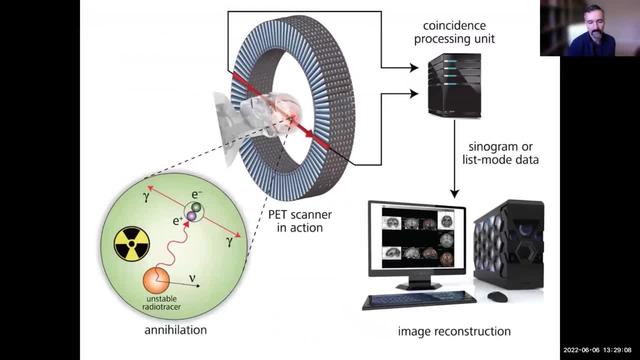 you may say: why on earth is that? so hold on, I'll tell you why in a second um, hold on to that thought. so so, uh, so, again just showing the same thing. you've got positron annihilating and you get two anti-parallel photon. now, if you have a coincidence, 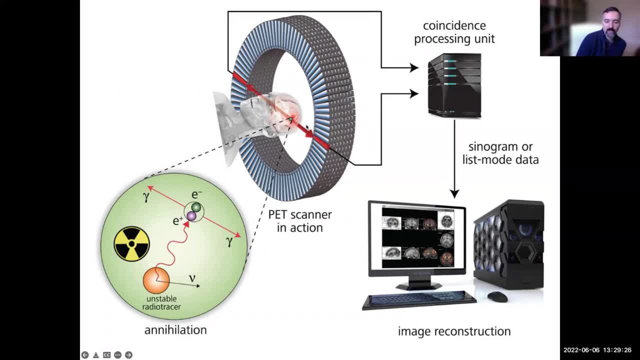 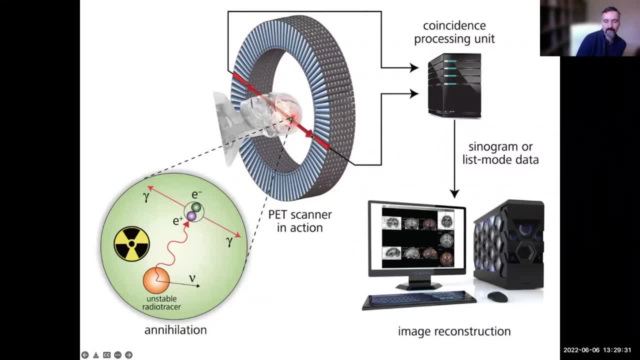 the same time. sure, this one is a little bit closer to here, so this one gets here a little bit faster than that one, but you know roughly they're arriving at similar times. if I have a coincidence, detection system says, hey, I got something here. I got something here. I'm going to draw a line. 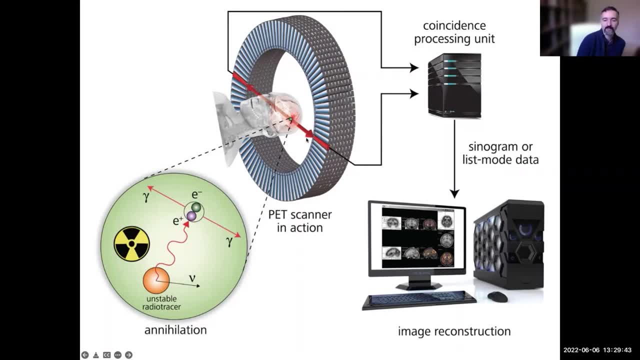 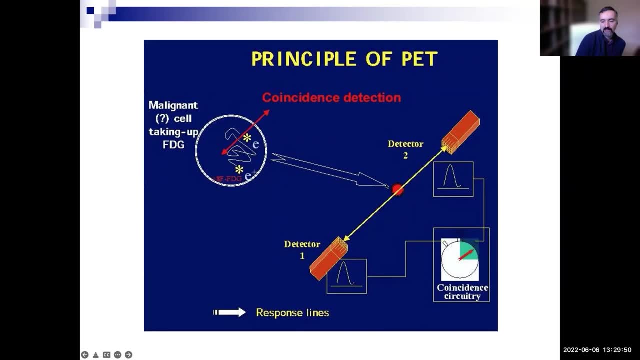 of response. it must have come from somewhere along this line, okay, um, showing the exact same thing again. you've got, let's say, accumulation in a malignant cell. you've got, uh two, two detectors that are detecting the two photons coming from it at almost the same time. 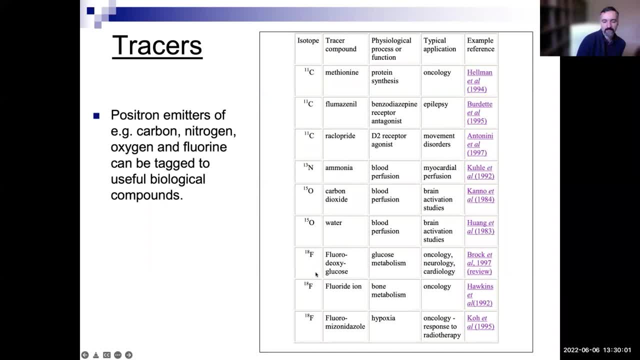 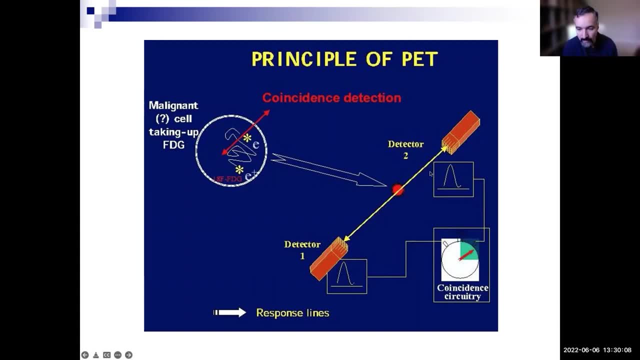 through a coincidence circuitry. you know that you draw a line of response- okay- and then from that you can end up reconstructing. you don't know where along the line of response it came from, but that's okay, because you're going to be collecting data from all angles and in tomographic 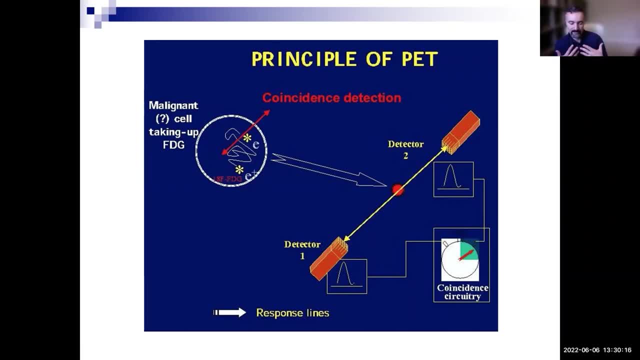 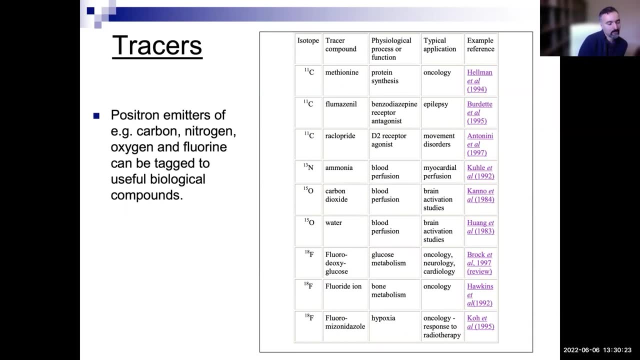 imaging. if you're collecting from all angles, it turns out mathematically you can invert the problem and get the original distribution, but still hold on to the thought. why is it that PET can be almost like even 100 times more sensitive than SPECT? why is that? hold on to that. 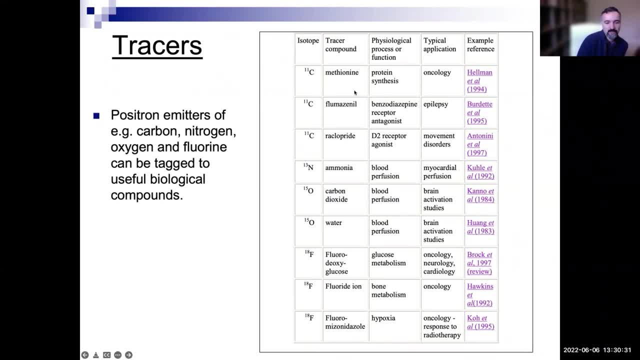 so here are examples of radio tracers or radio pharmaceuticals used in CT. again, you could label with C11, for example. nitrogen 13, oxygen 15, fluorine 18. there are some popular examples, but binomial is limited to these. fluorodeoxy glucose we already talked about in many different 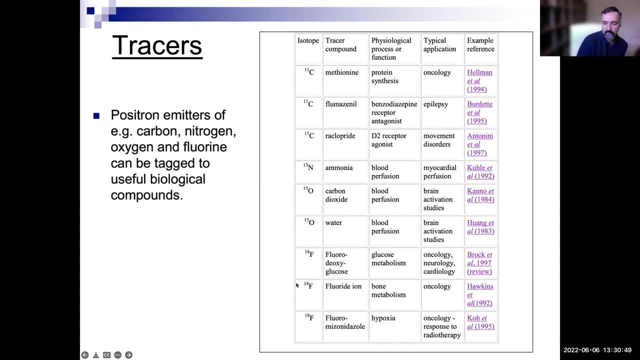 applications, but there's other ones too, right? so so you could be studying um, sky's the limit, because you have, there's different, multiple, different isotopes you can use and then you you could tag many different molecules with these and therefore you're looking at many different physiological processes that you could be looking at. examples of six radionuclides: 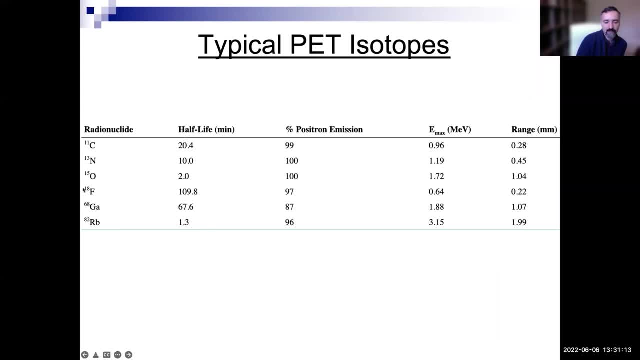 used in PET, uh with their half-life. so so again, f18 is is very popular under two hour um. gallium 68 is popular, also um, and here you'll have the sort of positron range. you see that the positron ranges typically are, uh, less than a millimeter. a couple of examples where it's: 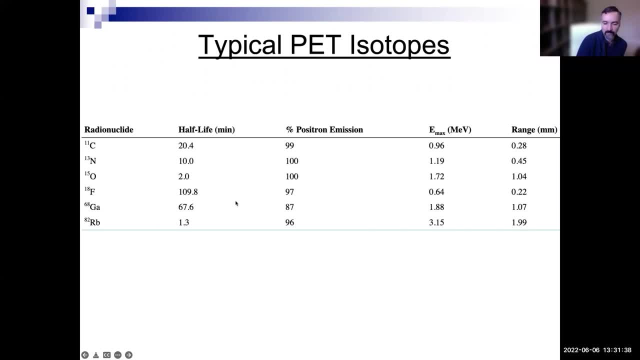 like quite more than actually. one example is quite more than one millimeter, because rubidium is highly energy, gives rise to highly energetic, uh, positive, so so the image might be somewhat more degraded. um, but again. fluorine 18: we're looking at sub millimeter positron range. 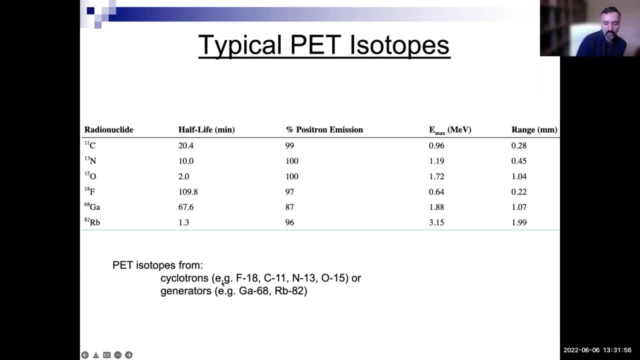 um, and the pet isotopes can be produced based on cyclotrons or or generators, and there's a there's the different economic models. for example, there's a debate about you know what works in each country and continent based on their business and economic models, right, so so, uh, you know. fluorine 18. 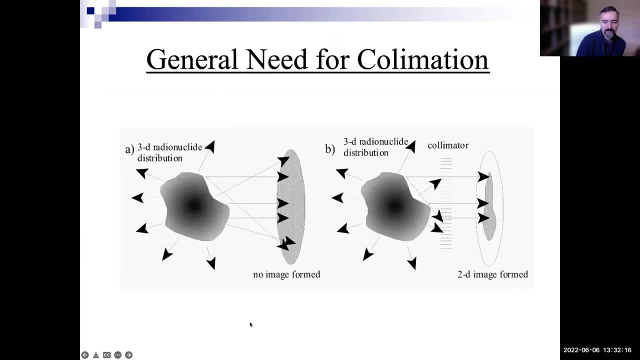 versus gallium 68. you know there's different ways to produce these. uh, we're now at a point where we can try to understand why sensitivity of PET is so, so great and so fantastic. so we said this before: if you have, if you're doing single photon imaging and 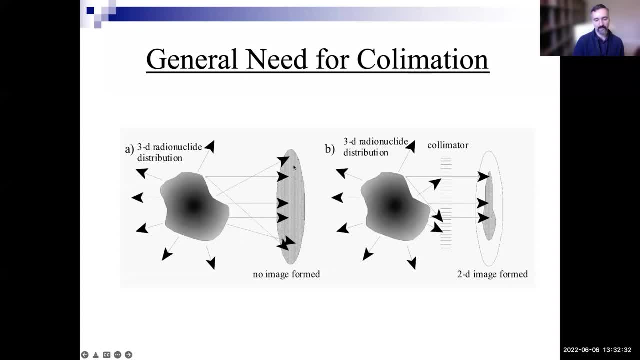 you don't use any columnators, you don't know where these humans came from, so you cannot visualize. that's why we inserted physical collimators, which we talked about last time, in in gamma imaging, to to restrain events that are coming in, so that they're only coming at this angle, otherwise we 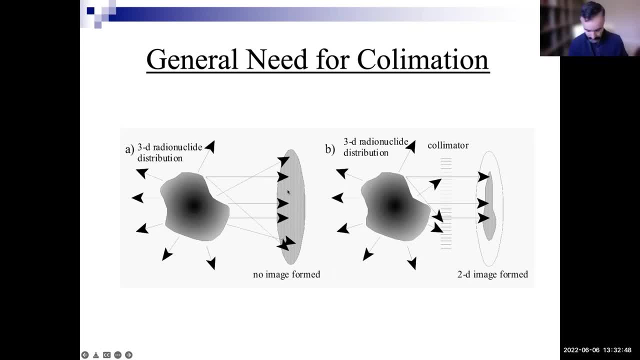 don't know where they come from, which line of response they come from, so we're more interested in from, and the pre-construction becomes near impossible. But when you insert a collimator, guess what you're doing? You're killing a lot of events. 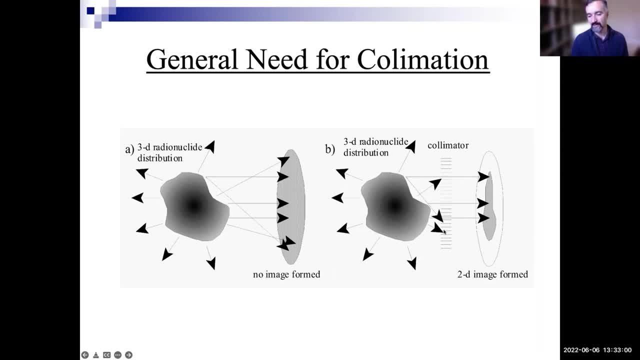 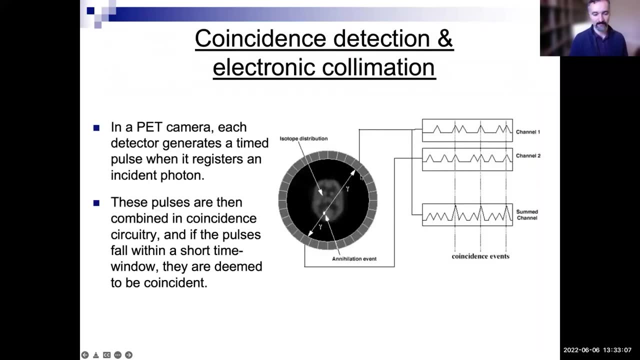 You wanna understand which direction they came from and in the process you kill. a lot of events Turns out in PET you don't have to insert physical collimators. why? Because you have digital collimation If you've got two photons that are being generated. 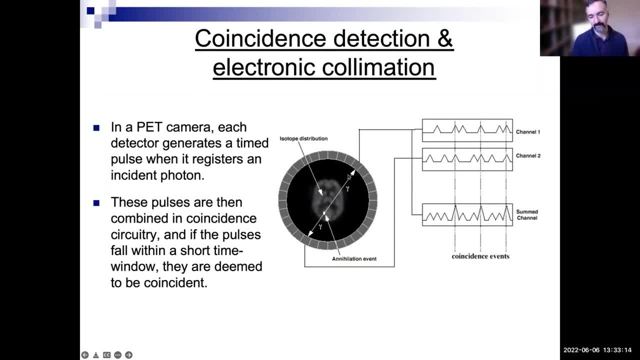 you don't need a collimator to be inserted here to kill events that are not coming at a certain angle. You have coincidence and the system says, hey, I just got something. This one says, hey, I just got something, but at the same time, almost the same time. 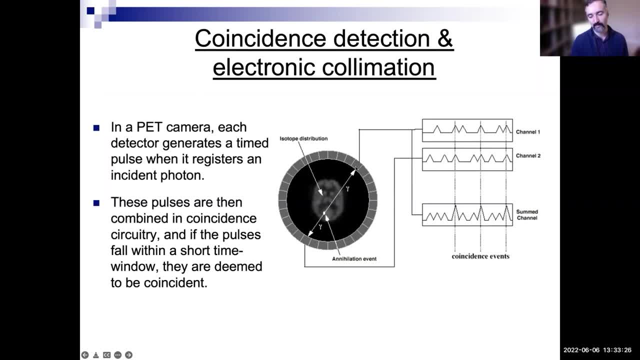 So let's draw a line of response here. So this one: you don't need a collimator to restrict what comes to it. You could have an event come to it at this angle or this angle, As long as there's a pair on the other side that says: 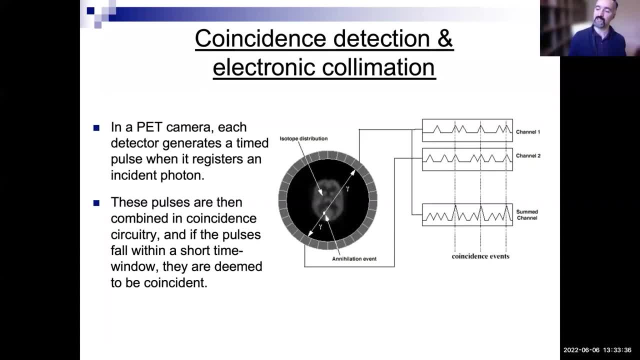 hey, I just got something with you and you can draw that line of response. you can measure that, So you're killing much less events. That's why the sensitivity can be something like two, even three orders of magnitude better. So what a coincidence, right. 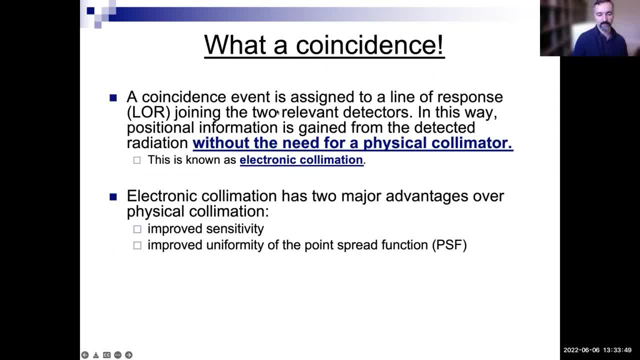 So yeah, So a coincidence event is assigned to a line of response, drawing a line joining the two relevant detectors, And so there is no need for a physical collimation. This is electronic collimation, And that has two major advantages. 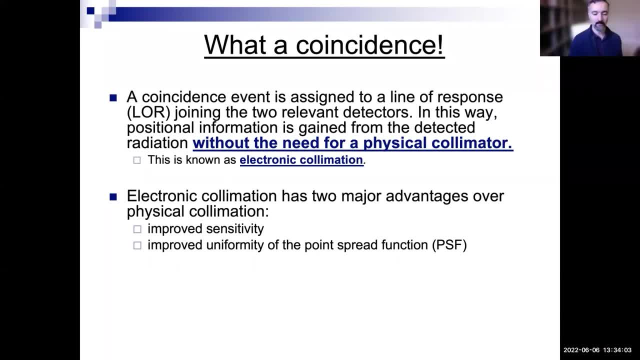 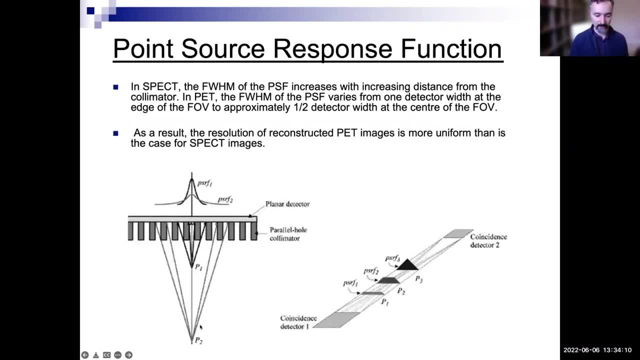 Improved sensitivity, which I just told you, but it also allows you to get a more uniformity along the point spread function. You might recall that we mentioned last time that as you get closer to the collimators in a gamma camera, as you get closer. 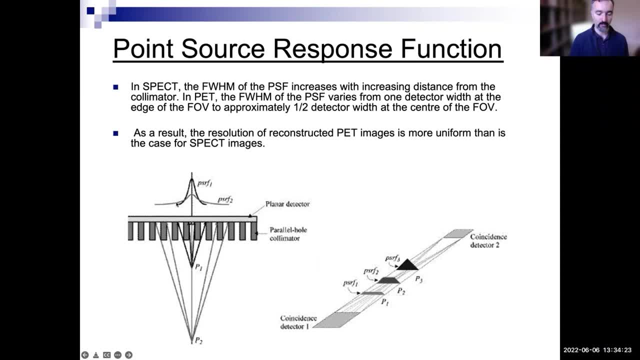 the resolution gets better, And as you're farther away, the resolution is worse. That's why, when we image patients, we like to. we don't like to go in circular orbits, We like to bring them into, you know, orbits that are closer, for example. 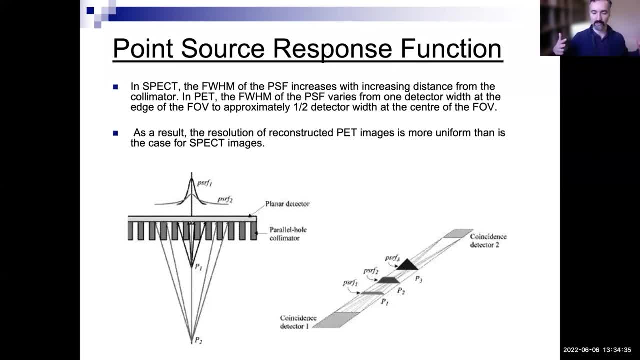 to the chest of the patient. So so the orbits may be non-circular, because we want to get as close as possible, But in PET, because you've got a detector here and a detector here, it's not just one one-sided. 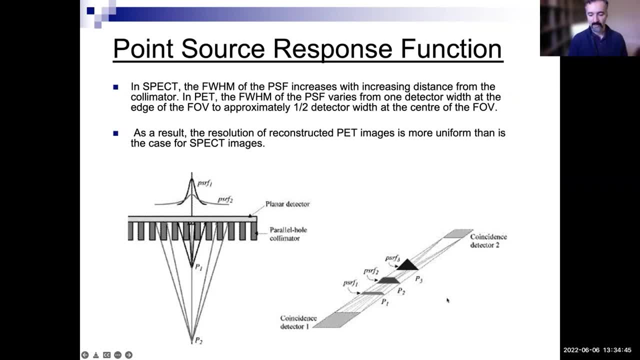 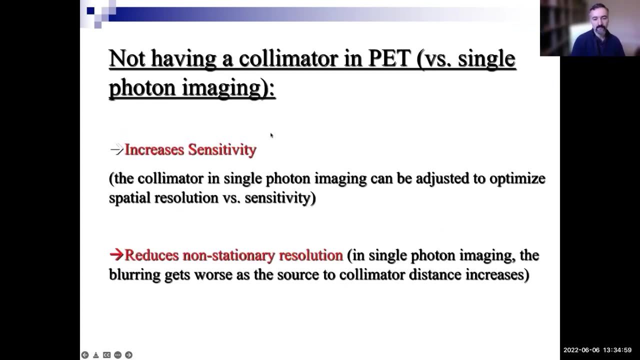 it's two-sided, one here and one here. It turns out that whether you're here or here, or here or here, the resolution doesn't change much, Because again you've got detectors on both sides, not just on one side. So increased sensitivity, right. 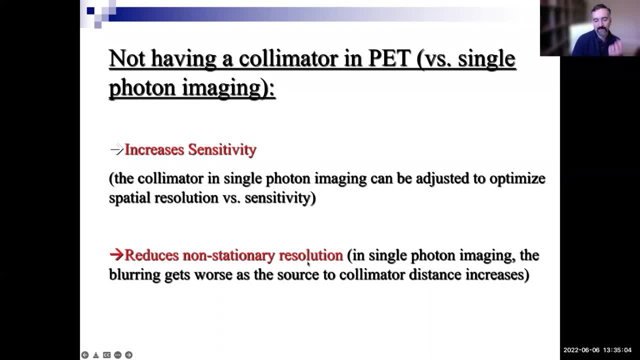 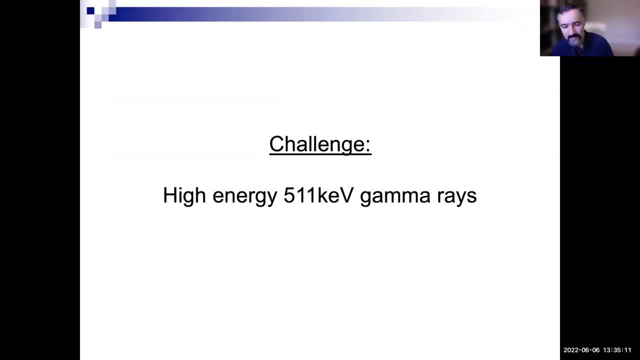 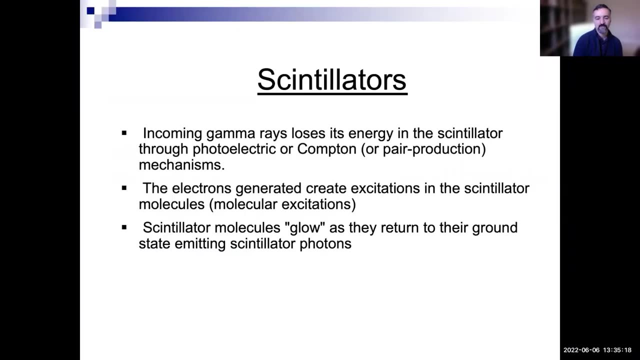 And reduces this dependence of resolution on distance. Okay So, but the challenge- and this is why PET is expensive- is the high energy 5-link 511kV gamma rays. So how do we, how do we deal with that? 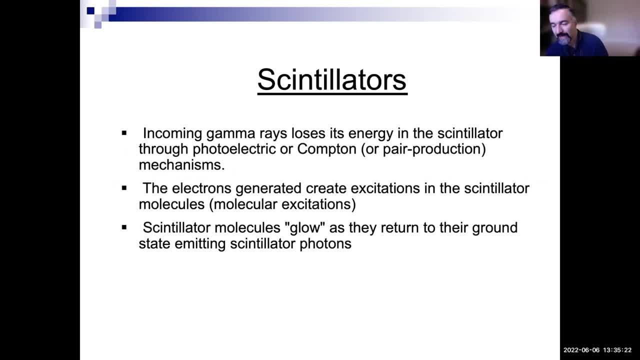 So we need scintillators. We are. we are obviously using scintillators for gamma too, but you need you need different kinds of scintillators for PET than for than for SPECT. So we talked about scintillators before and 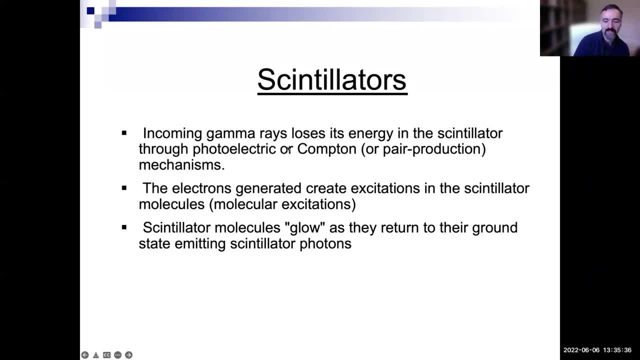 or at least we referred to it. But but the concept is that when you have an incoming gamma ray, it loses its energy in the scintillator. So gamma ray comes in scintillator loses energy, actually creates some kind of motion. 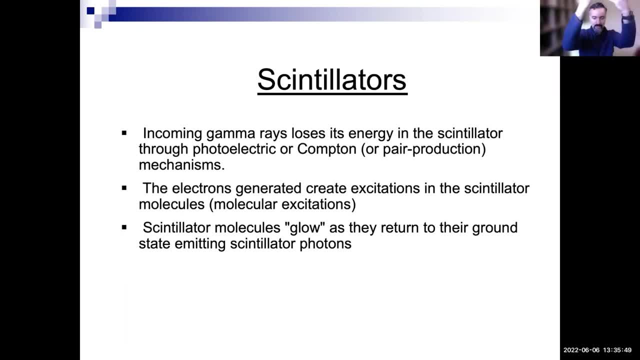 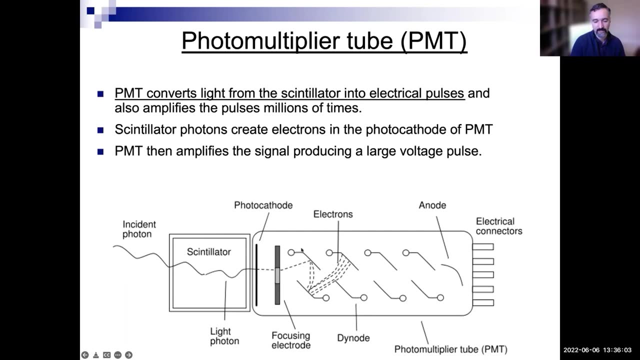 molecular excitation. and then when the scintillator, which is excited, comes back to its normal state, it glows and produces, like uh, actually visible light. and this visible light enters the, the photo multiplying tube, and then it amplifies it to give an electric signal. so again, high energy, gamma ray. 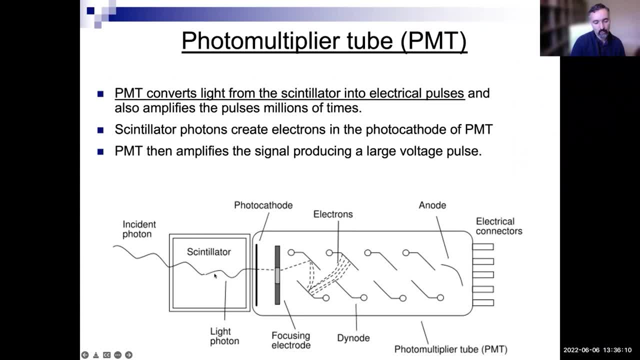 coming in, the scintillator absorbs them itself, gets excited and then comes back to its own normal state, emits some visible light. much, much lower energies than here, but lots and lots of them. they enter here and then, through this pmt multiplication phenomenon which we talked about before, you, end up getting, um, a strong current that you can measure. i'm telling you. 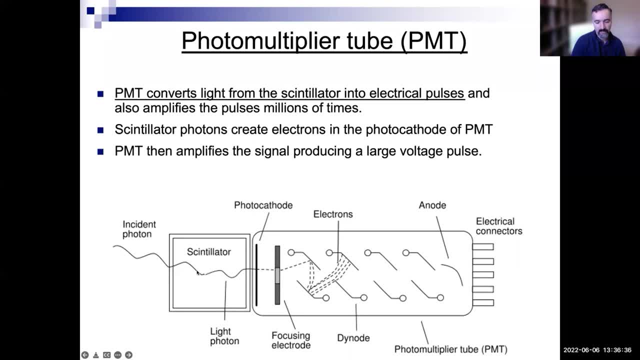 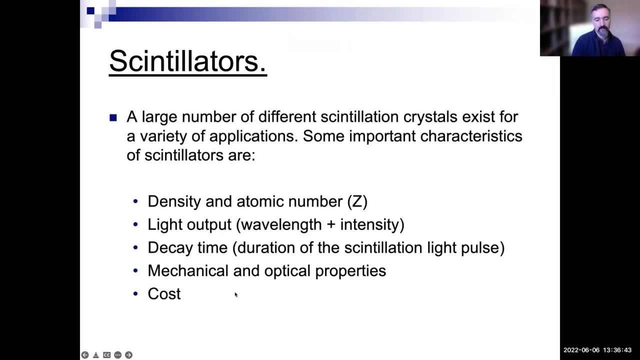 what was the original uh energy that you detected here? because the more energetic that this is, the more scintillation light you get. um, so you um. a large number of different scintillation crystals exist and they have a number of properties. again, we talked about this: density, atomic number, light output, decay time, certain. 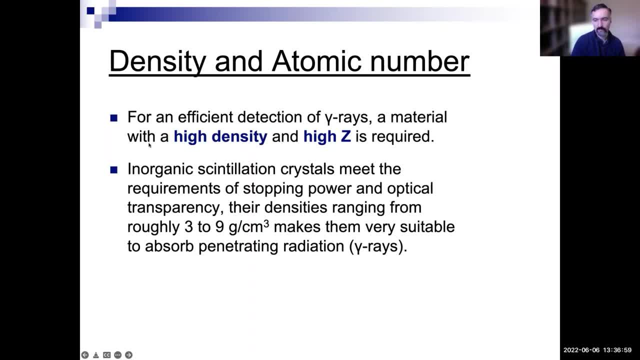 properties. but at the end of the day, if you want to absorb, if you want to stop highly energetic gamma rays, you're going to have high density and high z or high z to stop it. but you don't want to just stop it. you also want to have a good scintillator. right, i could design something. 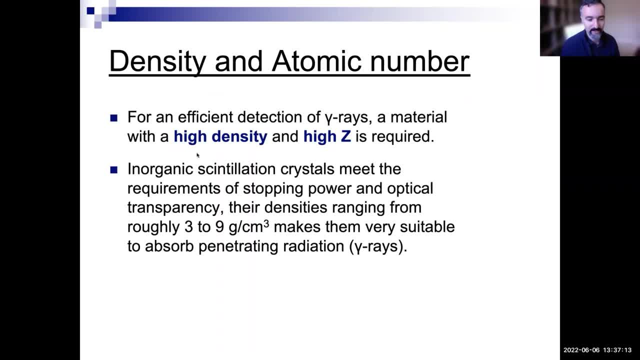 that is extremely dense and stops like. but you've got to also sense it has to be a good scintillator. um, and you have Soyuz right scintillation samples that can02. but inorganic scintillation crystals meet this requirement, having high stopping power, high. 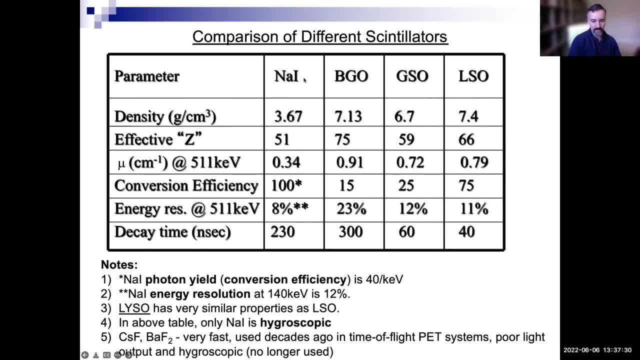 densities allowing to do that. so here's a table right and sodium iodine, as is used in in gamma imaging, meaning single photon imaging, may for example planar imaging and speck. you see it's 511KV instead of the 140, or you know, lower energies. 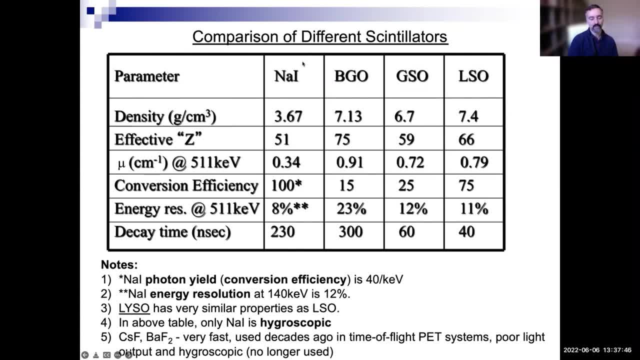 People are trying to use sodium iodide for PET, but it was not doing a good job, So people designed denser, denser materials. Okay so BGO, GSO, LSO, BGO and LSO. you keep hearing. 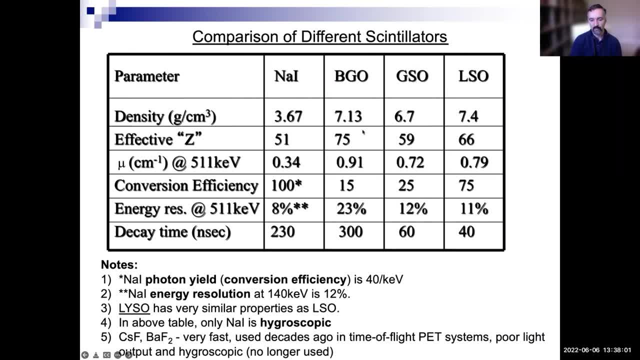 and they have very good properties. You know the stopping power is quite better than sodium iodide. Conversion efficiency is very good for LSO compared to sodium. Sodium iodide is great for conversion even though it doesn't stop as well, but once it stops it yields very good light. 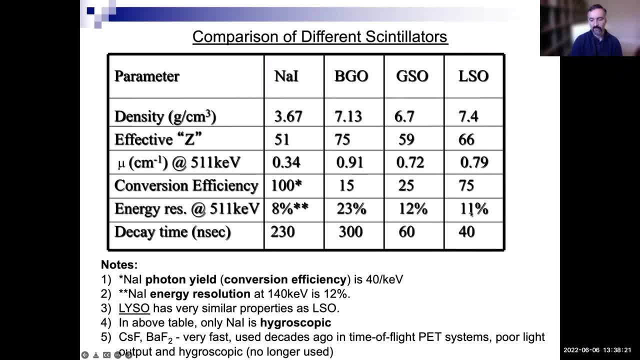 LSO comes close And resolution again for LSO because it emits a lot of light. their resolution- also energy resolution- comes close And one of the cool things, or important things, is that the decay time with LSO is also small. It means that the scintillator 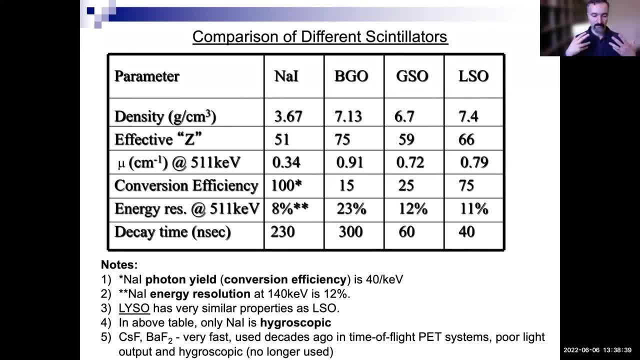 almost has smaller dead time, Like it doesn't get saturated as easily because at the processing time every event that it processes takes less time than the other one. So energy has really increased the usage of LSO or LYSO, which is similar to it. 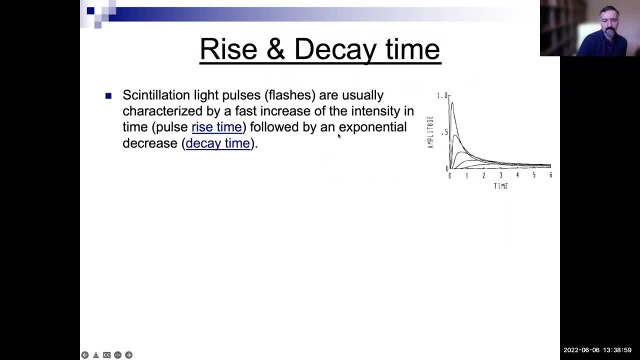 or BGO, is still being used as well. So again, when something comes in, you get a pulse, rise time and you get an exponential. This is almost like a processing time Scintillator: something hits it, it gets excited, It starts to emit things excited. 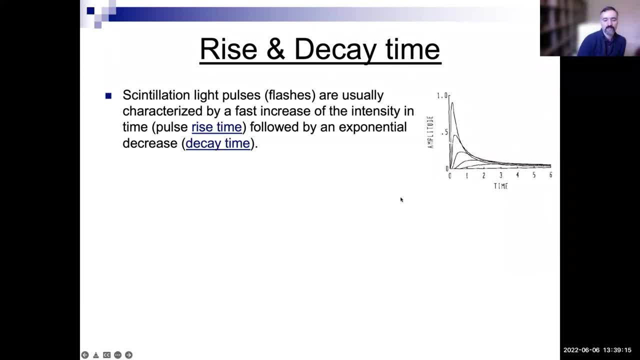 and then all this processing is happening and then it starts to have an exponential decay time. So this is a rise time, decay time, And so you wanna have a fat and these two are sort of correlated. So the faster that this is, the faster that is. 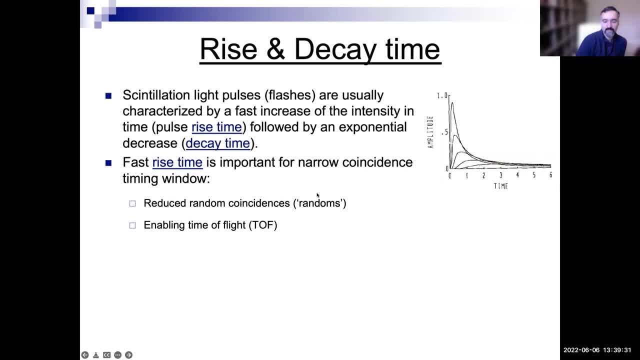 So if you have fast rise time, that means you can really reduce the so-called random coincidences. We'll talk about that later. This allows you to also enable time of flight later. Just hold on to that thought that these two words are important. 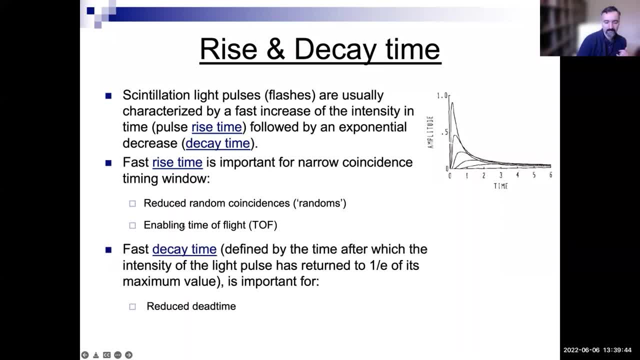 random coincidences and time of flight. We'll come back to that later. Faster decay time, as I just told you, gives you less dead time because there's less saturation. You're quickly getting over this processing time, So if a new event comes in here, you're able to process it. 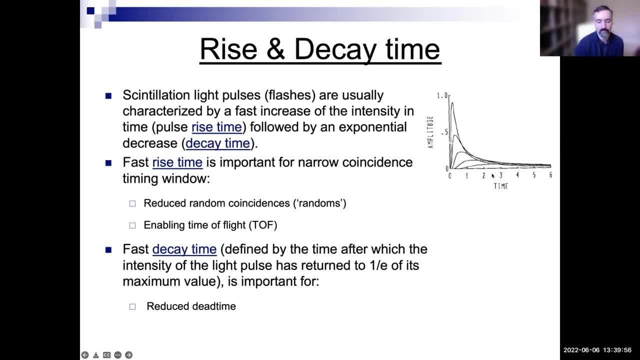 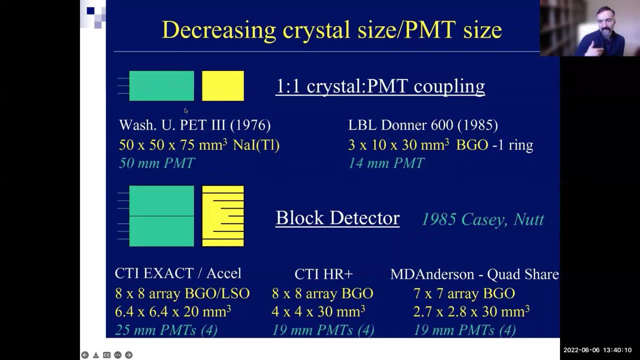 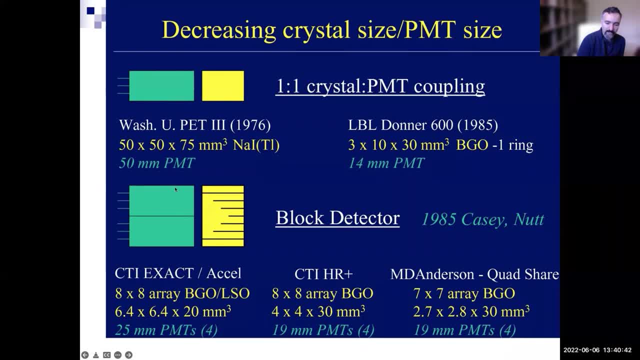 this one here is gonna deposit almost all of its scintillation light here, Whereas if this guy's here, most of it goes here, but some of it goes here, and this guy's here, half of it goes here and half of it goes here. 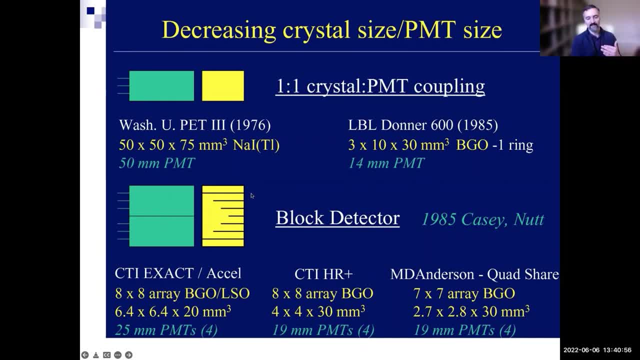 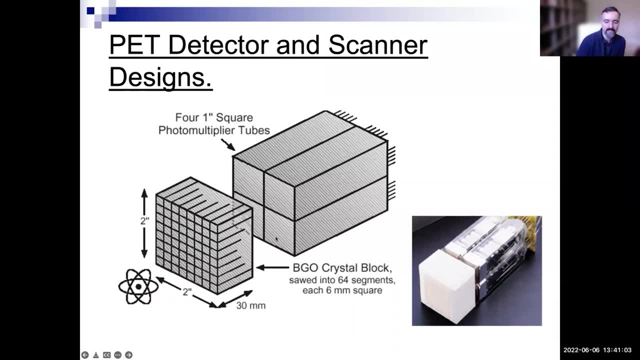 By averaging between how much signal this is getting versus that is getting, you can actually calculate where along this you're detecting, And that's X, and then you could do it similarly for Y. This is how visually it looks, And again, visually is how it looks. 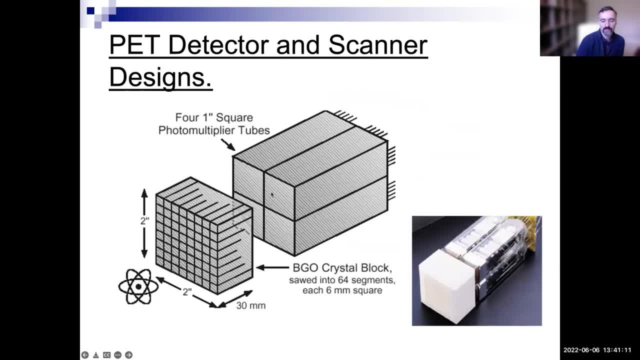 let's say an eight by eight coupled to a two by two set of PMTs, And again, depending on where you are on the X and the Y, the amount of signal you deposit in these four will be proportionally or somewhat changed, and then you can figure it out through angular logic. 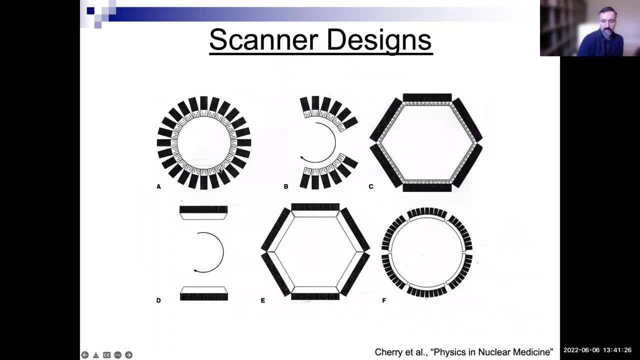 Different scanner designs have been considered. This is a very popular one, just a circular design, but you've also had these ones right, And you've also had partial ring designs right, But these are the most popular ones. They're fully covering the field of view. 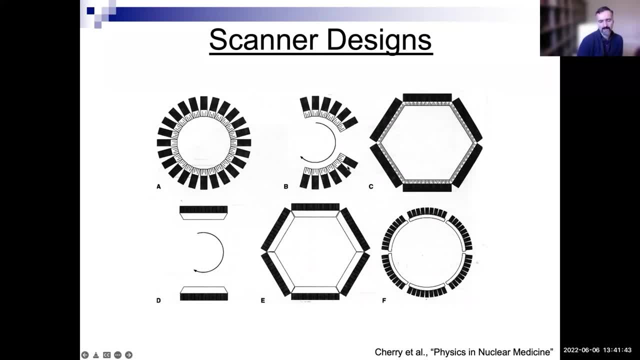 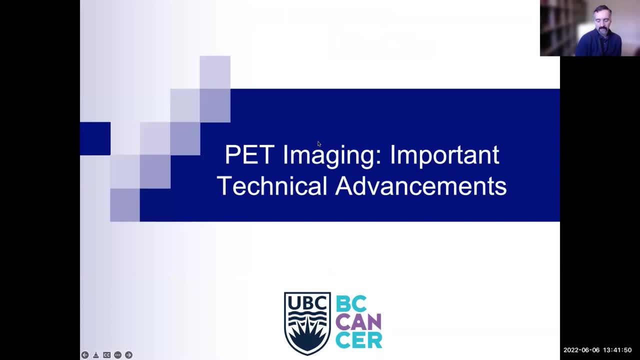 but people are exploring the idea of partial ring PET scanners, especially with artificial intelligence. You know you can probably do better reconstruction, fill in the gaps, et cetera. Okay, so what are some of the important technical advancements besides what we just mentioned? 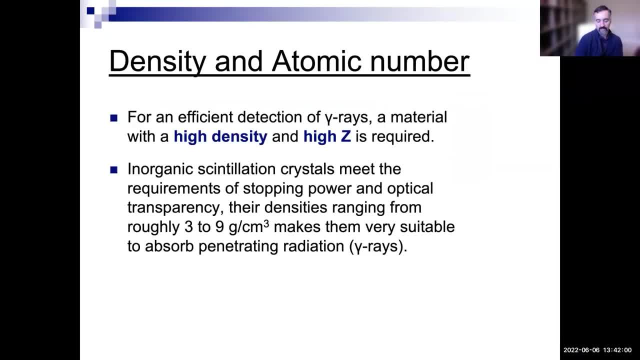 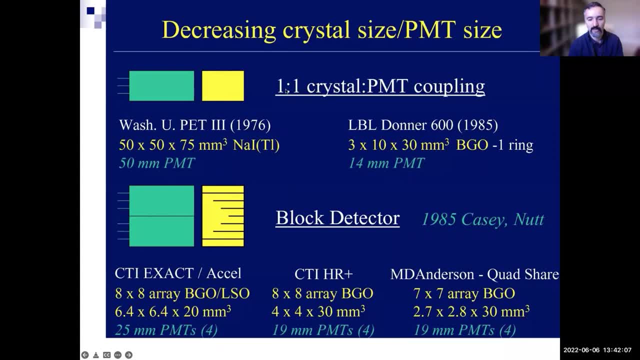 What did we just mention? We talked about the idea of using good and better scintillators. We talked about the idea of doing moving beyond one-to-one coupling and, instead of one crystal being mapped to one PMT- This would make PET scans super expensive. 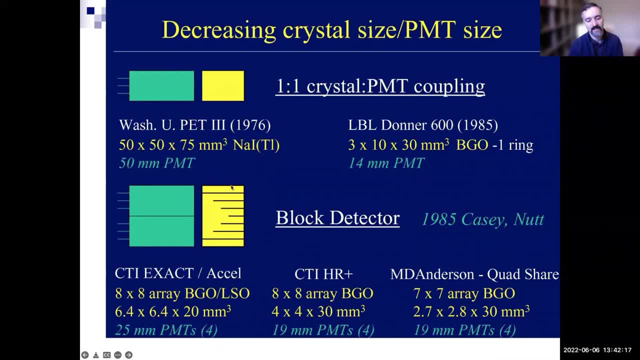 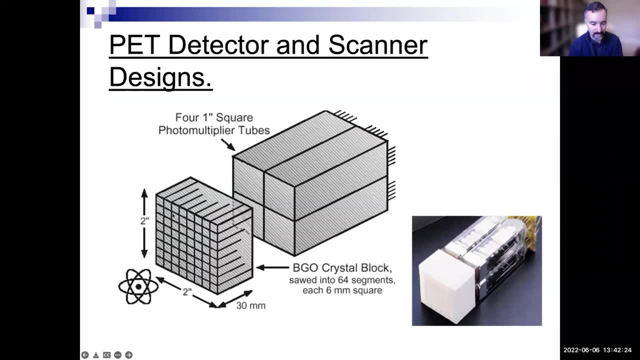 because for every crystal you're gonna need one PMT, Whereas here for every 64, you need four of them For every 64. in this design you need only four PMTs, So you could actually create very good high resolution PET with only fewer PMTs. 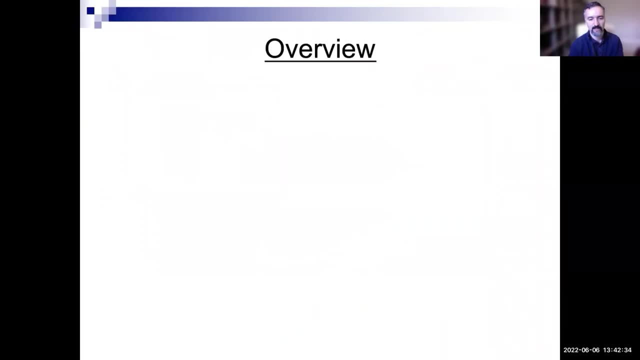 So making the- you know- high resolution PET with only fewer PMTs. So making the- you know- high resolution PET with only fewer PMTs. So making the- you know it not so expensive. But besides that, what else has happened? 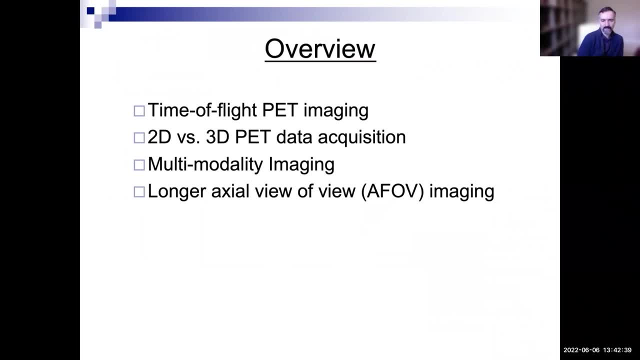 in some of the developments. So I'm gonna talk about some of the key developments in the world of PET, Time of flight, PET. I promise you I'll talk about it. So about 2D versus 3D PET data acquisition: 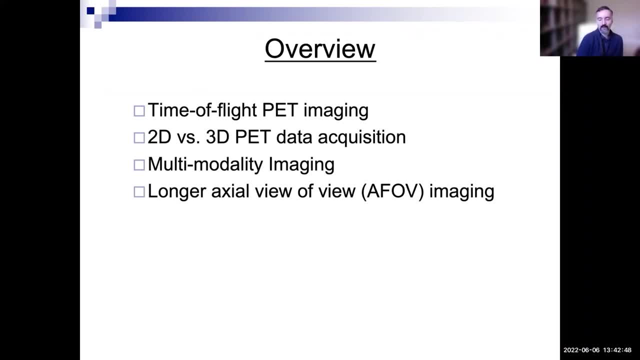 not image acquisition. Images are always 3D. If you're doing tomography, your images are 3D. No, but acquisition itself Multi-modality, meaning PET-CT or PET-MR and longer axial field of view image. 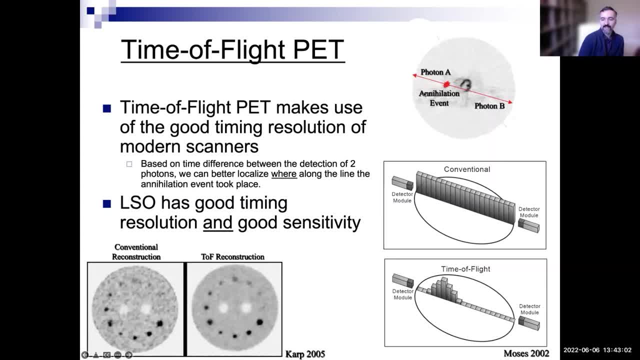 So what is time of flight? PET? Remember how I kept telling you if you got an event, if you got an event here, this one technically gets here a little bit faster than that one. Well, can we measure that? Can we measure how much faster this one gets here than that? 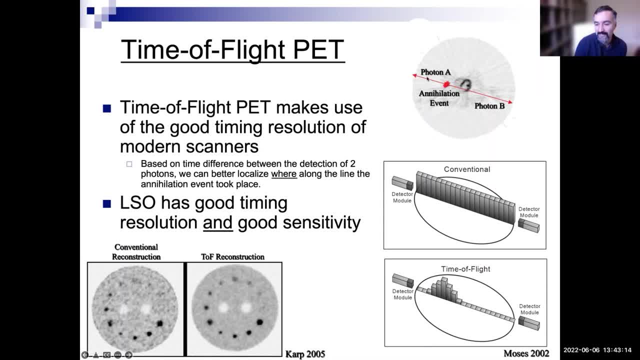 Because if you can measure how much faster this gets here than that, we can actually know where, along the line of response, the event came from, Because nowadays- normally not nowadays, like in the original non-time of flight- this is what we have. 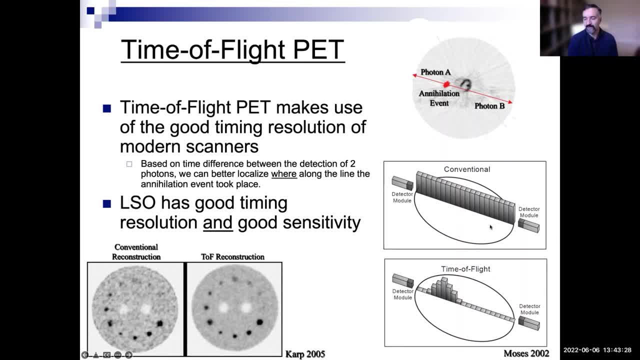 We don't know where it came from, And so we would back project the entire thing. But because you're doing image reconstruction and you're collecting from all angles, you can figure it out. But what if you didn't have to back project this entire thing? 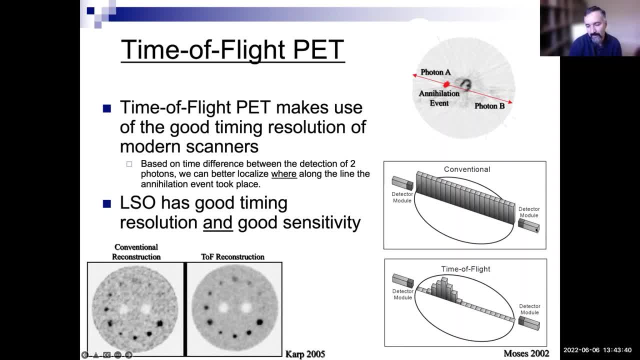 Remember you're having noise in your detectors. What if I don't back project this entire noise And if I sort of have a feeling that it must be somewhere here, because I got a signal here a little bit faster than a signal here, then that actually ends up reducing noise. 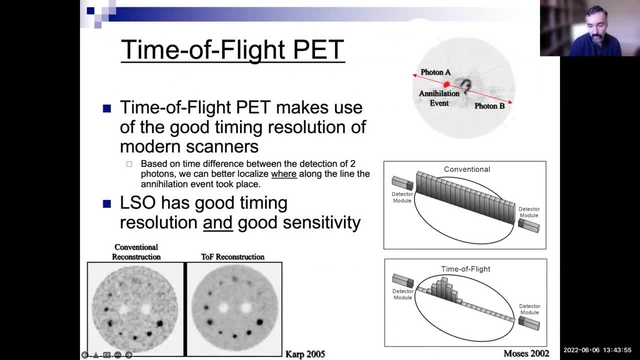 as you can sort of see here Now, if you had really really really good timing, you don't even have to do image reconstruction anymore. You just know exactly where this event came from Here. But we don't have that kind of a good timing right now. 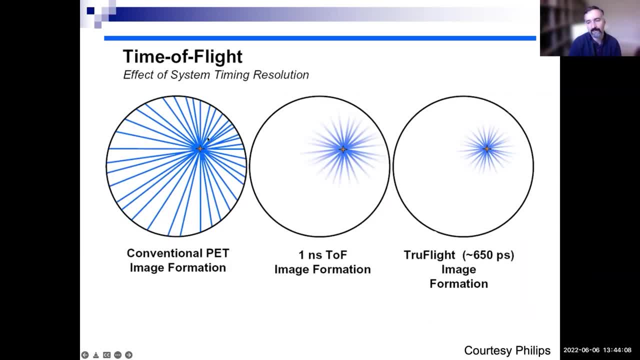 So this is a conventional PET. You don't know where it came from. You would back project everything. do field training, do whatever iterative recon, You'll get it right. But at least this is how you back project it. But if your time of flight or the timing resolution 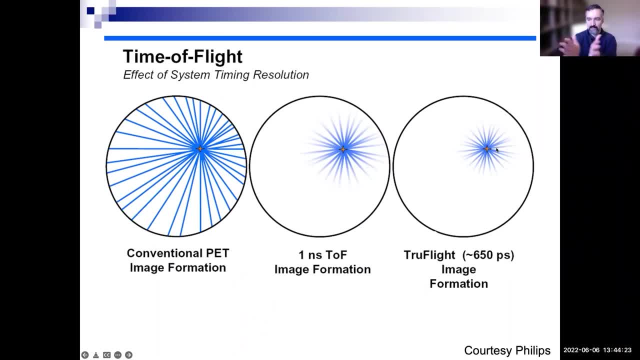 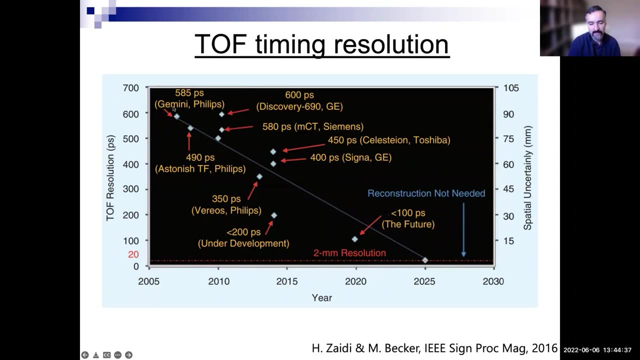 in your coincidence becomes better and better, you're back projecting smaller and smaller segments. So it turns out, because you're back projecting less noise across smaller segments, you're gonna get less noisy images. But if in the future- I mean this is a projection of the past, 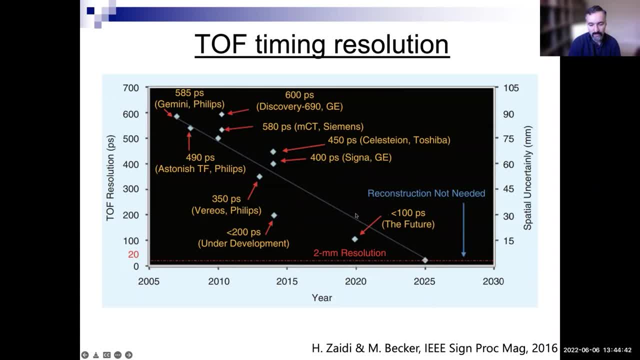 And right now you know we're talking. you know, some clinical scanners that we're having are actually around 200 picoseconds actually. So this was a good prediction back then. that was made in 2016.. But if this trend continues, perhaps in the future- 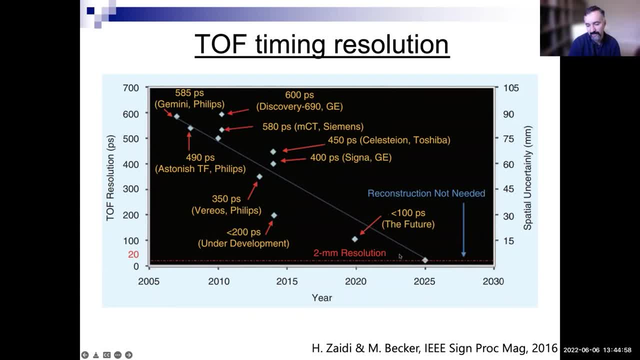 we might even reach this place or maybe not. This may curve off like that, But if we go below a certain resolution, we might reach two millimeter resolution, which means we don't even have to do image reconstruction. We'll know within two millimeters. 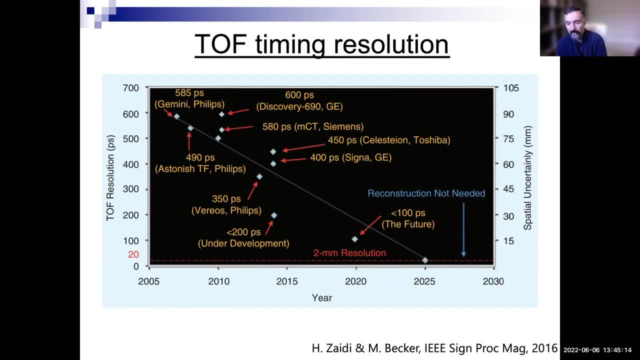 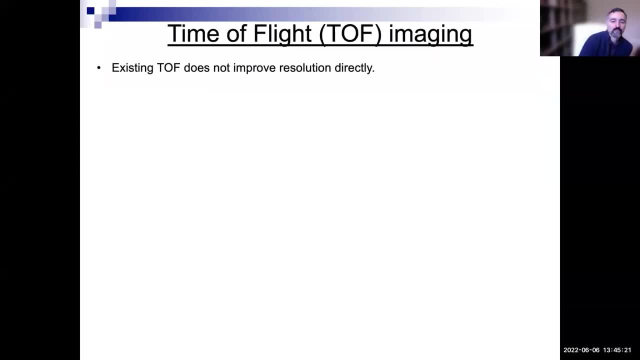 if, where the event came from. But we're not there yet. So we still have to do reconstruction, We still have to do back projections and stuff, but at least we're getting less and less noise. So existing time of flight does not improve resolution directly. 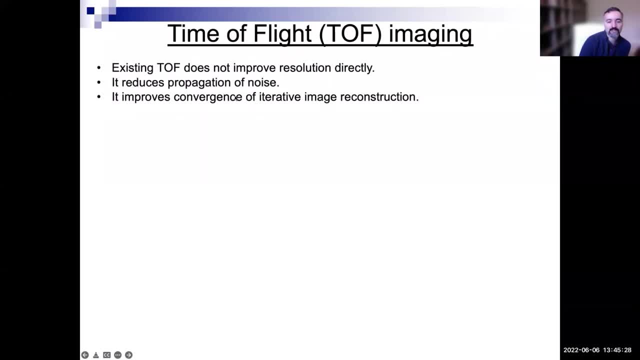 but it reduces propagation of noise. Therefore you get less noisy images and allows your iterative recon algorithm actually to converge faster. So for a similar number of iterations one arrives at a higher contrast image because it's converging faster without noise amplification. 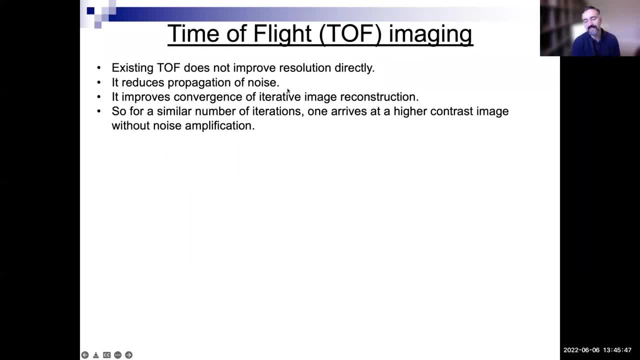 because it's reducing propagation of noise. So time of flight is great, So the scanners nowadays have it. This is an example of a non-time of flight image. This is the time of flight. If you look carefully, you'll see that contrast might be improved in some places. 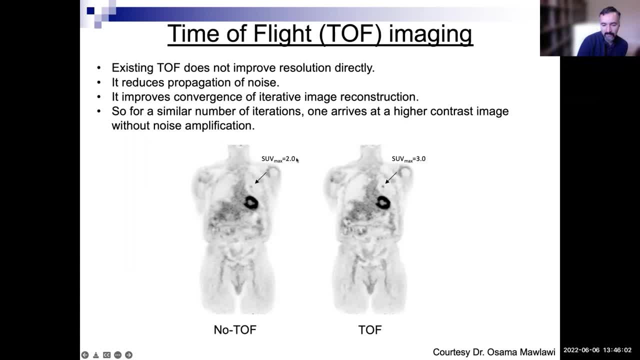 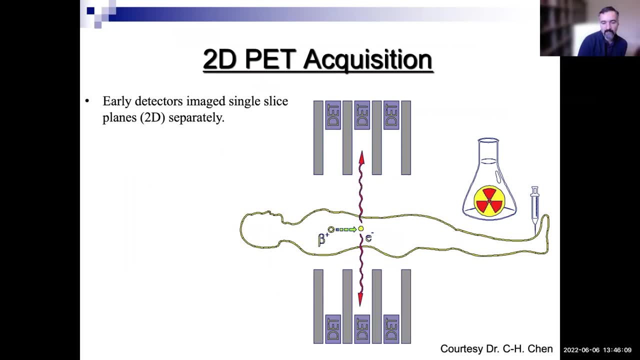 but look at this particularly, The contrast: here is around two whereas here is three. You start to think: something's at least more clear. What's the other technology Originally in PET? you know the saying: you can't handle the truth. 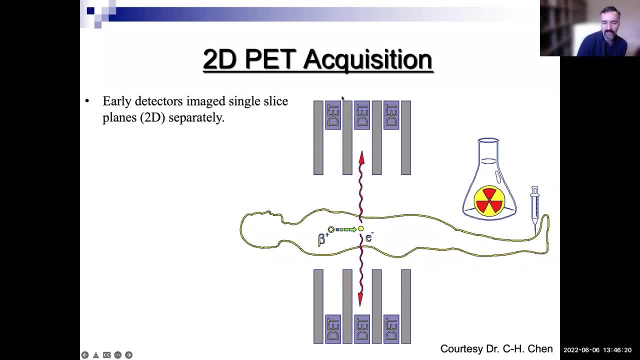 It's almost like the signal was just too much to handle. So people would insert some kind of step top kind of like only between the axial rings, not between the, not in a within a plane, but only between the rings. 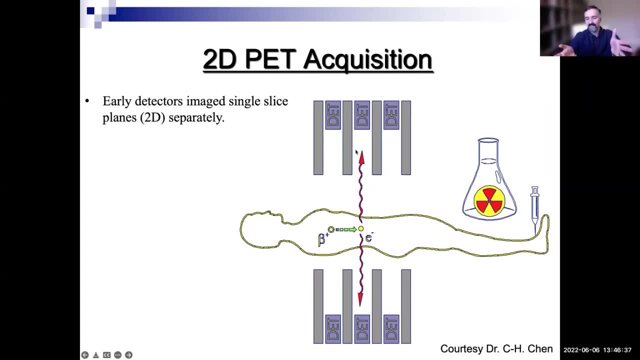 Actually they would insert SEPTA, So they would just process it, So they wouldn't have to process so much signal coming at oblique angles. So this is what people used to do: 2D PET acquisition by inserting SEPTA. 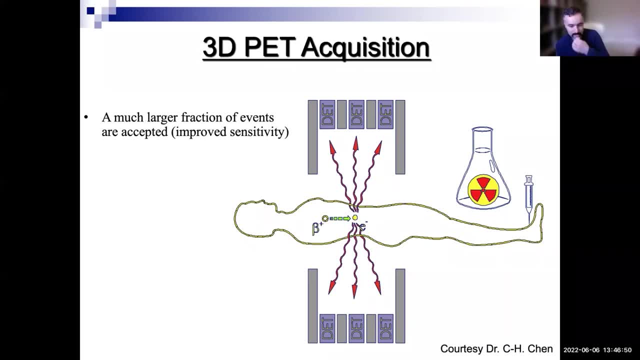 But then people thought, well, why not get rid of it? So what I mean? okay, we get more signal. Sure, more signal might mean that you're going to need greater storage and computational demand, but we'll deal with it. 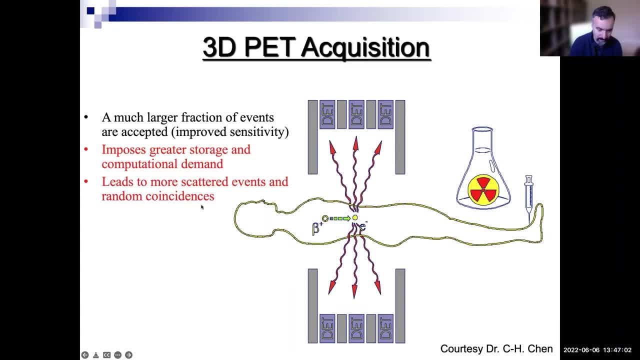 You might get more scattering, more randomness. You might get more scattering, more random coincidences. I still have to tell you what random coincidences are. Well, okay, we'll handle it, but we do get much, much improved sensitivity because we're not killing these events. 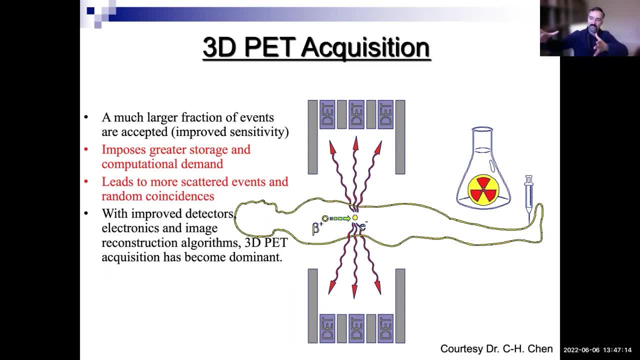 So, in the same spirit that, going from SPECT to PET, there is an increase in sensitivity. Same thing: Let's remove the SEPTA and we go from 2D PET acquisition to 3D PET acquisition And with improved- you know- image reconstruction. 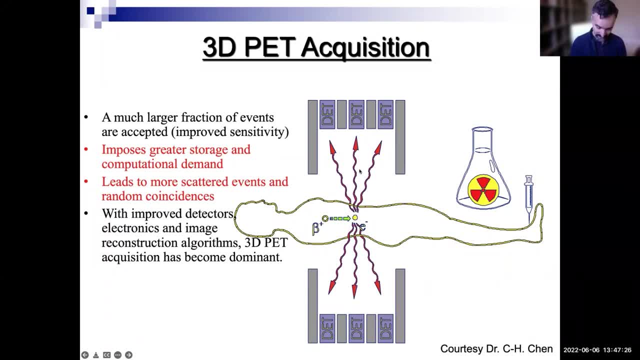 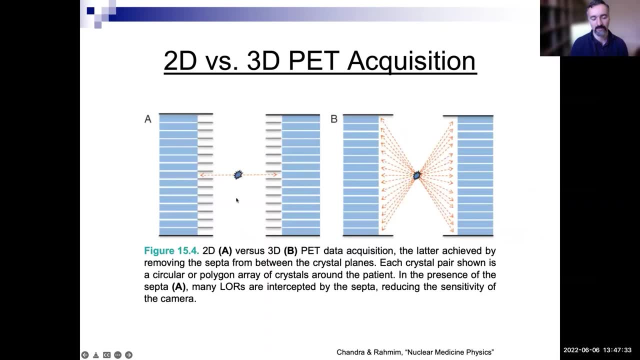 improved electronics to handle this, this, this increase signal that's coming, that's that switch was made. So again, going from 2D PET acquisition with SEPTA between the axial planes- the patient would be lying like this- to something like this improved sensitivity. 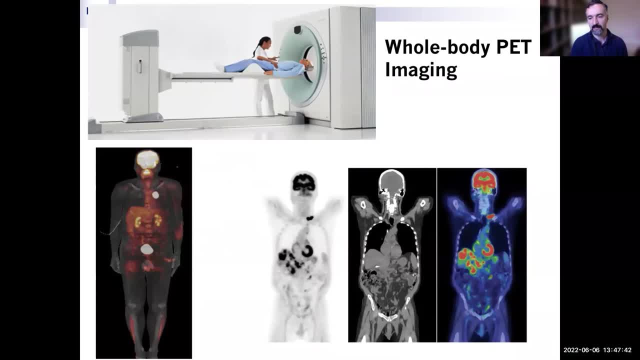 So again, images got better. Another thing is that people do whole body PET imaging right, So this is very popular and commonly used and prevalently used in PET imaging You can do, because the sensitivity is so good- you can do a whole body imaging. 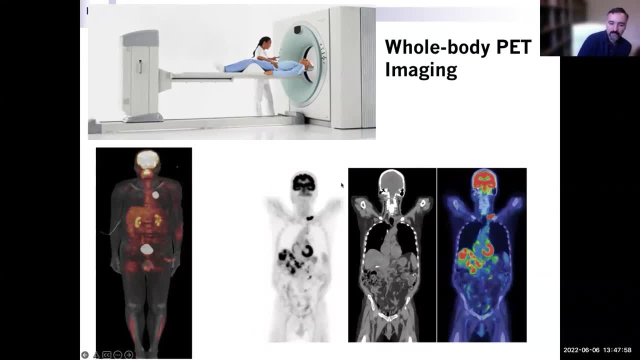 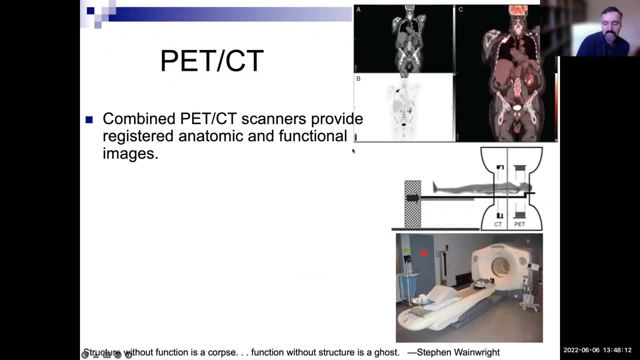 Now, sometimes whole body means true whole body, but sometimes it just means, you know, from here to here, for example. okay, So it depends on the protocol, but it means multiple PETs, And the other thing is that we do multi-modal imaging. 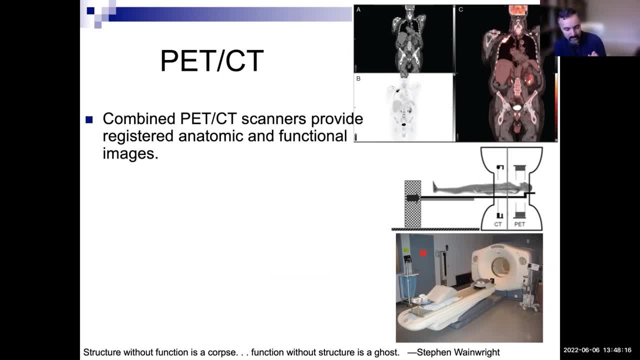 As I mentioned to you, adding CT to SPECT or to PET allows you to measure how much attenuation is happening, but it also allows you, the clinicians and the physicians, to look at the images in fused mode. So, again, CT can be used for better visualization. 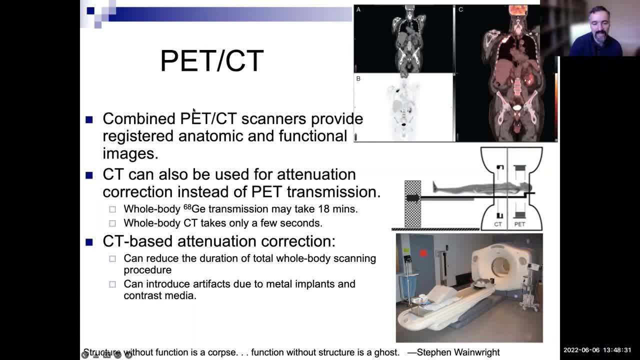 And when you're doing a single scanner, combined PET-CT, there's less shift and drift in the body. If you have some PET scanner here, some CT scanner here while the organs move et cetera, But it's on the same bed, you're just translating the bed. 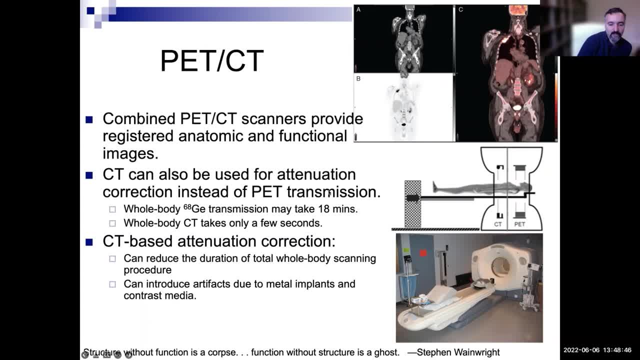 So you get better registration. Again, CT being used for attenuation correction. People used to use transmission sources, but that would add like an extra something like 20 minutes, But with CT that's only a few seconds. So that's why, when this concept was introduced, 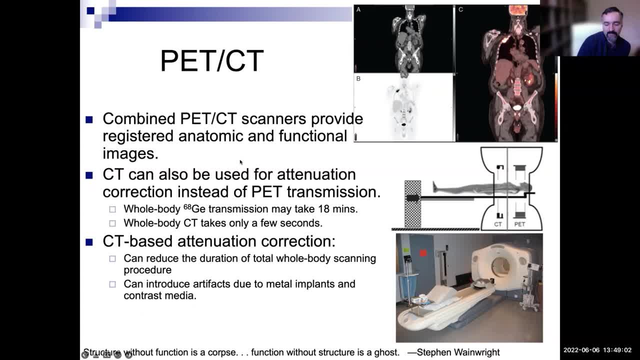 in the late 90s, people implemented in year 2000, the first clinical scanners that went from PET-only to PET-CT. in the span of only three years, The market share of PET-CT went from 0% to almost 100%. 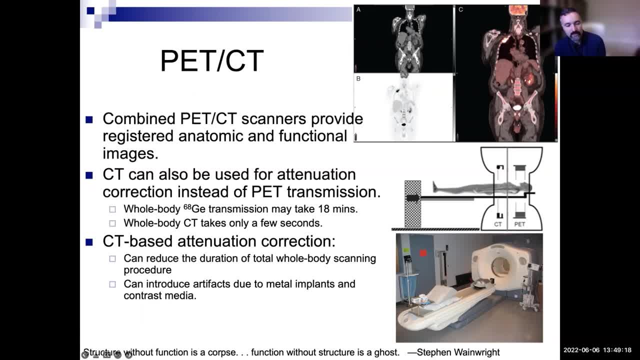 It was revolutionary thing: PET-only pretty much became PET-CT And so PET-CT based attenuation correction can reduce this duration. It can reduce the duration from 18 minutes of these slow movements of transmission sources to only a few seconds, but it can induce certain artifacts. 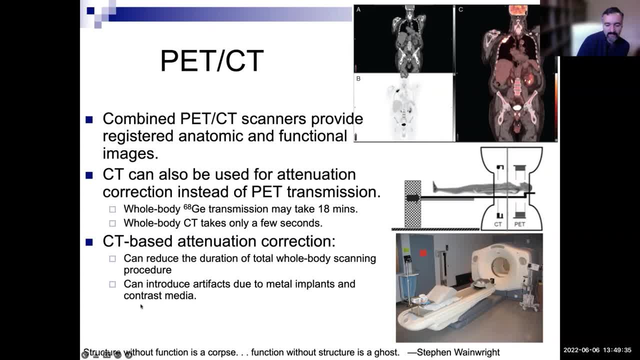 For example, CT might be sensitive to metal implants, contrast media, but then there are solutions, workarounds around it. So I like to saying structure without function is a corpse and function without structure is a ghost. So PET-CT allows you to do both. 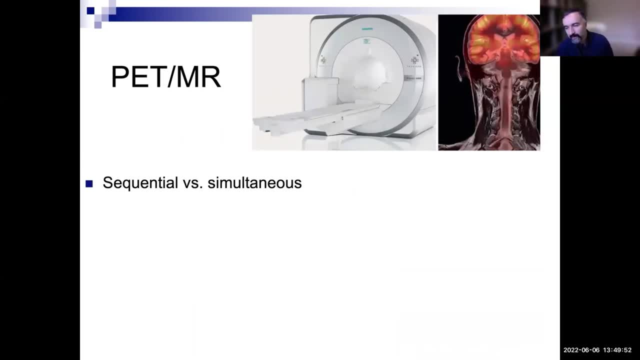 PET-MR is also a has been a, you know, definitely a trend. There's a lot of excitement around it When it started to show up. you could do sequential PET-MR, kind of like PET-CT, or you could even do simultaneous PET-MR. 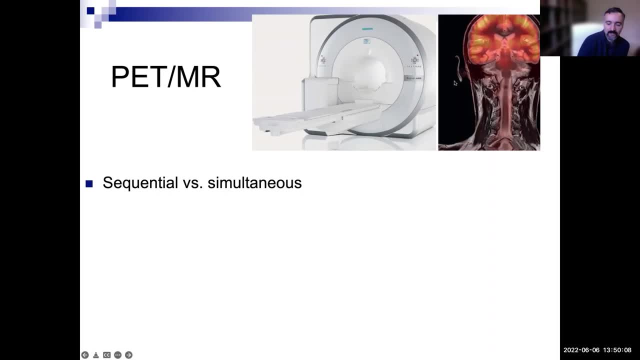 They had to redesign the scanners because the PMTs- when you have photo-multiple tubes, you have a lot of magnetic field. It just messes things up. So they move towards a solid state. you know solutions, semiconductor solutions. So yeah, this is what I just told you. 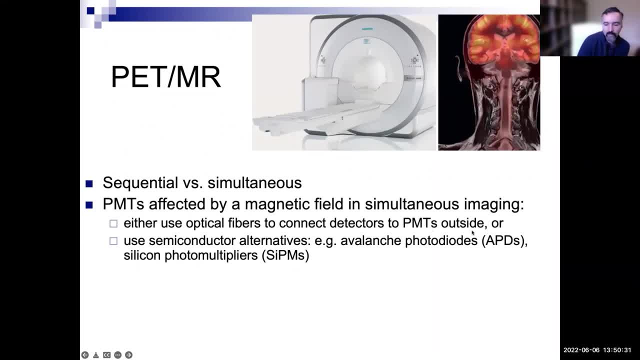 So people consider semiconductor alternatives like avalanche photodiodes, APDs or silicon fotomultipliers, And this thing is so good because they're more compact that even though people wanted them for PET-MR, so they're not sensitive to magnetic fields. 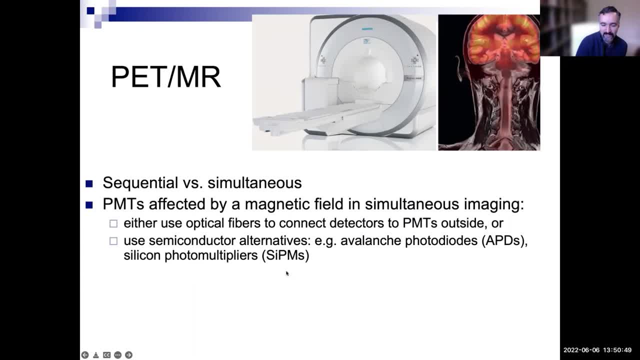 but they're so good that people are not even switching PET-CT scanners to these kinds of alternative semiconductor alternatives. And we sort of talked about last time, about last time, some advantages of semiconductor approaches to detection. but uh, attenuation correction in mr is complicated because mr signal is governed by proton density and relaxation. 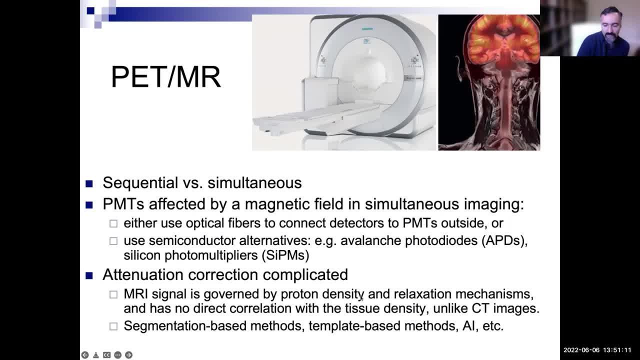 mechanisms, as you know, and it doesn't directly correlate with tissue density, unlike ct. ct, it's, it's about, it's about, uh, tissue density, it's about electrons, okay, so, so, so, so, uh, there's a bit of a mismatch between attenuation for pet anymore, and therefore, therefore, what's happening here is that people have used other techniques, like 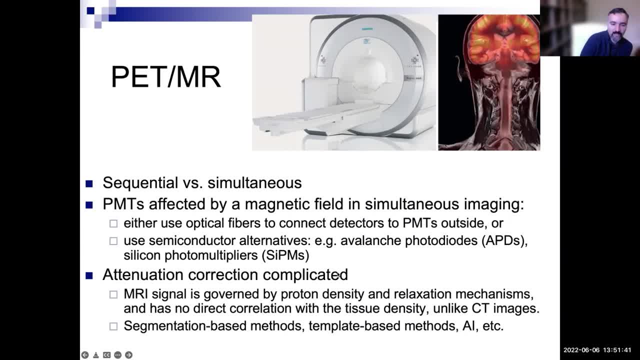 segmentation based method, ai- or template based methods- ai- to do this. but you know it's moving forward. the question really is: is petamar worth it? because it's. it's very. it's much more expensive than pet city. it's an amazing tool for research. clinically. people have been looking for some. 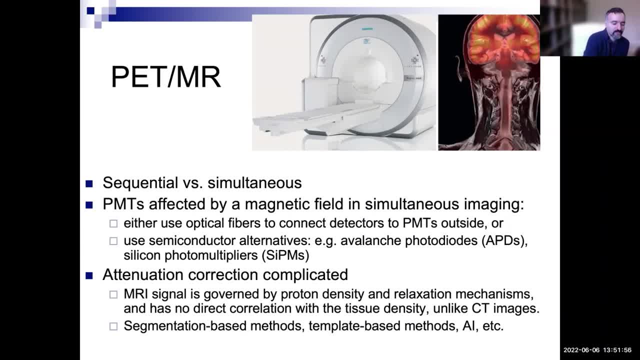 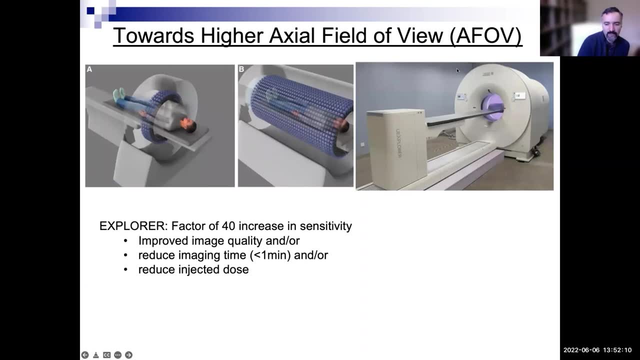 applications for it. um, so it's, it's continues to be, uh, an area of exploration and interest. but, you know, majority of scanners in the field nowadays are our pet ct, not perma. and this is a new, uh exciting development in the field where the actual field of view of a pet scanner, which used to be only like 10, 15, 20 centimeters, because it's already 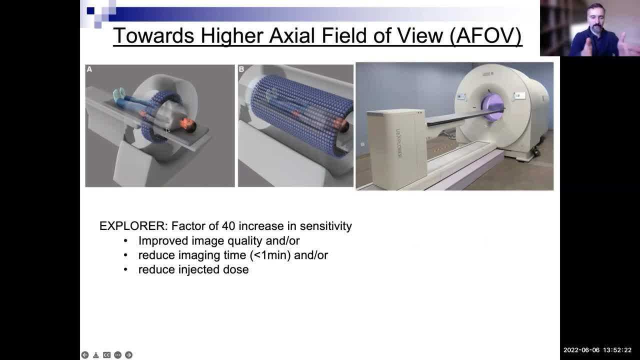 so expensive, and then you would have to shift the beds, multiple bed positions, to do dynamic, to do a whole body imaging there's. you know, some explorations came initiated by fantastic colleagues at uc davis and then uc pen and in europe, etc. where they were like: well, why not? 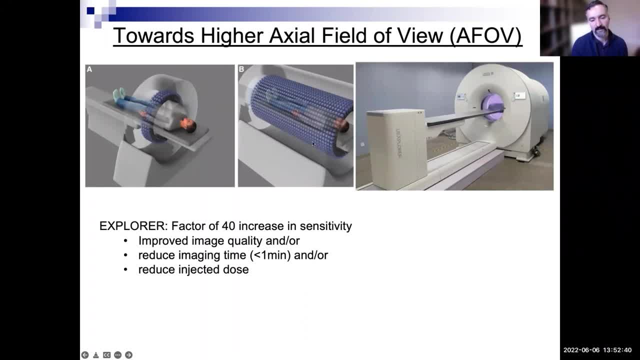 just build a much bigger scanner. uh, now you can imagine this is this is going to be a lot bigger, um. and then you can imagine this is going to be a lot bigger um, and then you can imagine this is going to be monumentally expensive compared to that. right, but they took a risk and they, they activated the. 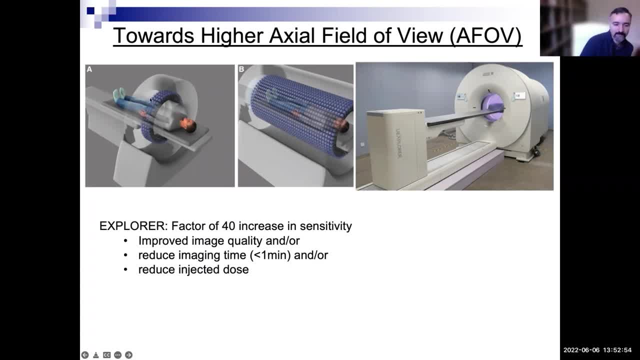 imagination of the community. for example, in this design where they went from, let's say, a field of view of 15 to like two meters, you could get a factor of almost 40 increase in sensitivity. so you could get much, much improved image quality. or think of it this way: you could reduce the um. 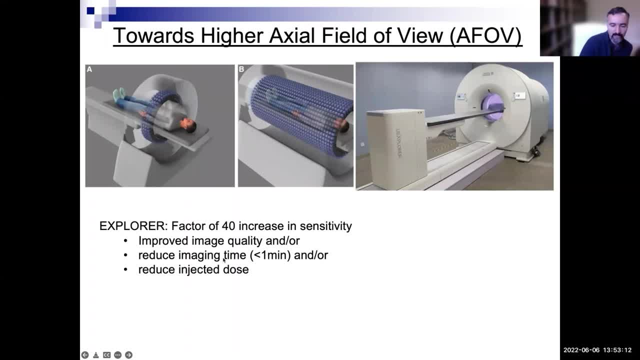 if, if the sensitivity is 40 times more, you could reduce the imaging times to even less than one minute per patient, you could even think about doing breath hold pet- it's like hold your breath done- well, not that fast, but you know- or you could significantly reduce injected doses to patients. 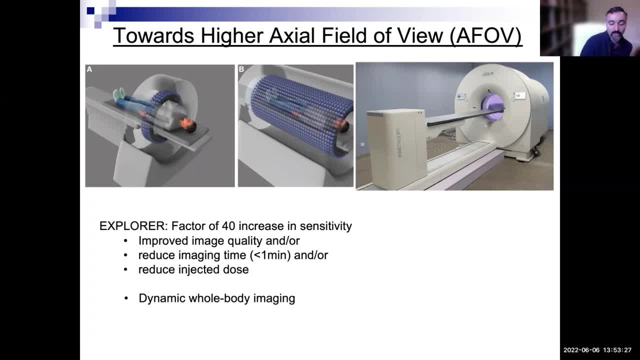 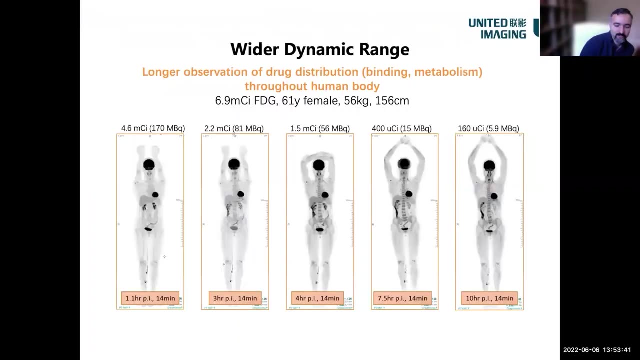 pediatric, or you could even scan. you could do dynamic whole body because you could, you could. this patient is being covered across his or her body and then what you're having is that you could. you could observe the dynamics of the radio pharmaceuticals. so a lot of exciting possibilities. 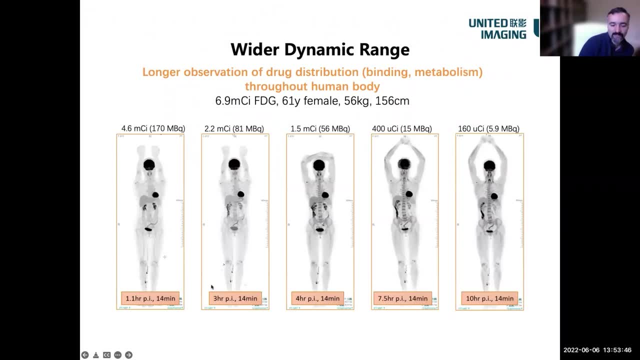 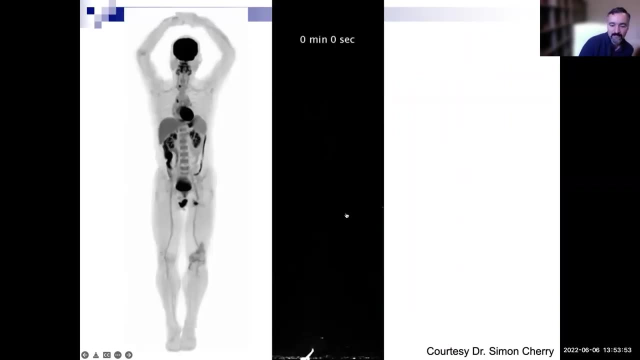 or you could even image the patients many hours after injection. like this is an example of a patient being imaged 10 hours after injection and yet you're getting cool images just so. it's pretty outstanding results. here's an example of the kind of things we couldn't even imagine doing dynamic. 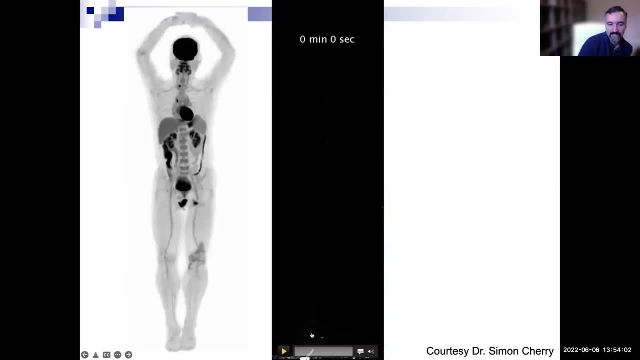 whole body imaging. look, look at these times. each reconstruction at the beginning is after every second. one second of acquisition gives you enough data to do image reconstruction. watch, see that something's been injected- radio pharmaceuticals being taken up. the heart is distributing it across the body. now the image. 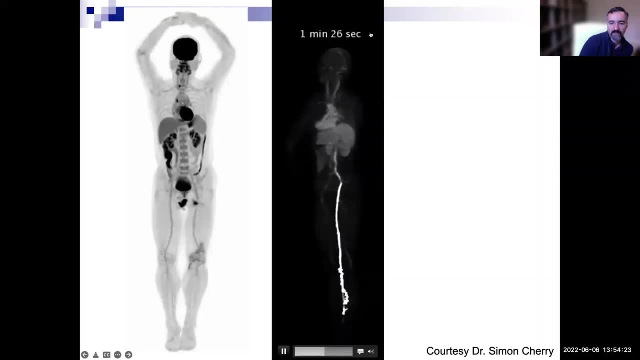 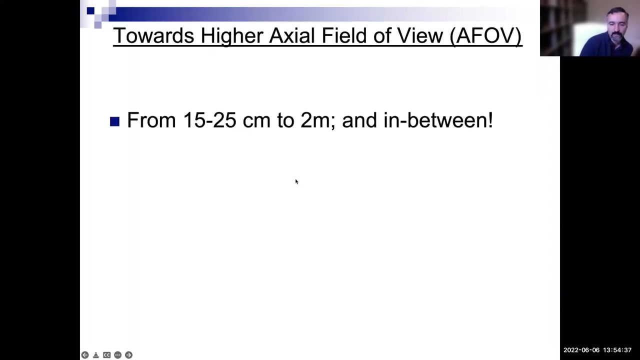 intervals are starting to become a little bit larger, maybe every few seconds, then it's going to switch to every 10 seconds, maybe every minute. you sort of see these images, so providing just amazing images. so we're going from maybe here, which is what used to be, to here and things in. 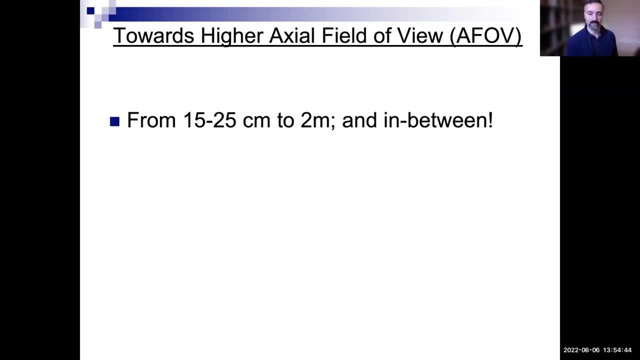 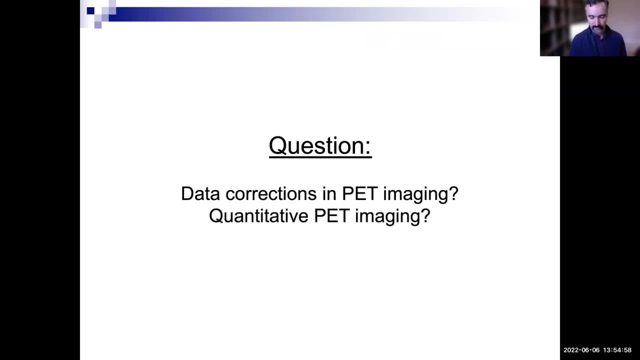 between right. so, for example, you could have a long actual field of view pet scan that's one meter long right. so what are some of the data corrections that we can do in in pet image? um, and can we achieve quantitative pet imaging? so yeah, the answers: of course we can, but how do we do? 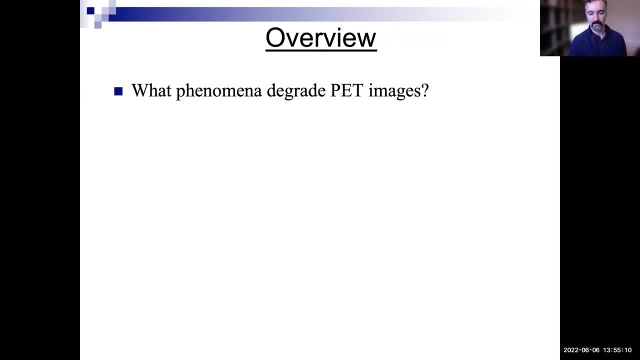 first of all, what are some of the things that degrade that? the quality and the quantitative accuracy of pets would be known. so we could, you could 2D and quantitatively get quantitative accuracy of pets. so we know, so we. So then I tell you how we tackle them. 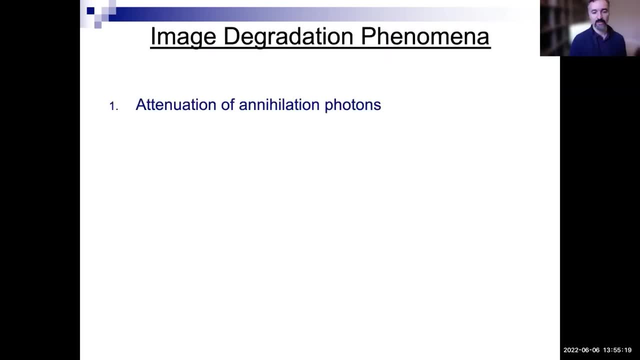 So what are those key things and how can we compensate for them? So I think I mentioned something like eight different things here. So attenuation is a big thing in both PET and SPECT. A signal originally intended to be detected in some detector may not be detected. 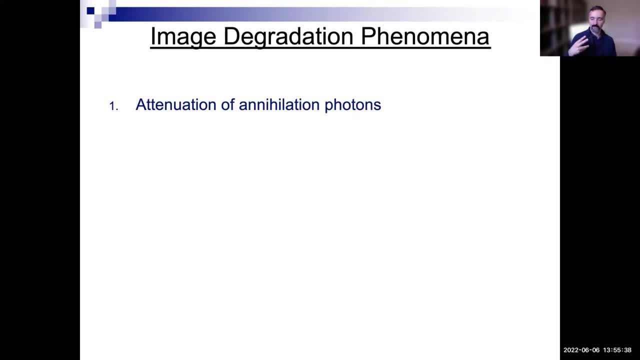 either because it got absorbed, like in the photoelectric effect, or- which is not really common in PET, because the energies are so much higher, or it could be scattered away. When something's scattered away, it means it's not detected where it was meant to be detected. 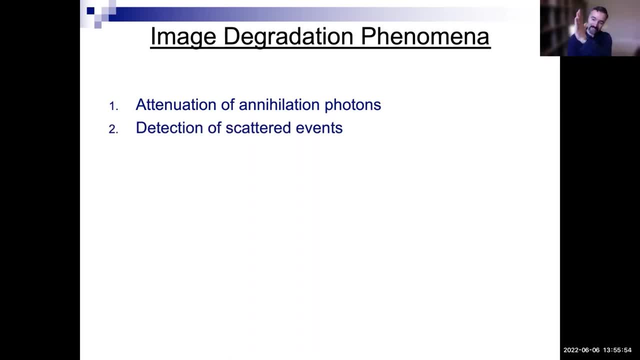 So for that original line of response, it's an attenuation. But then if it gets scattered away and gets detected somewhere else, that new place is receiving more stuff than it meant to. at least for that particular point It was not intended to be there but it ended up being there. 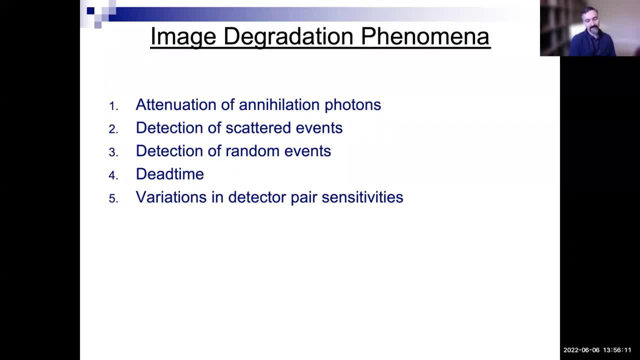 Random events. we'll talk about that. Dead time is sort of alluded to it. Variations in sensitivity of the or pair sensitivities, decay resolution, degradation issues, like you enter a crystal but then you're detecting a mirror by a crystal. 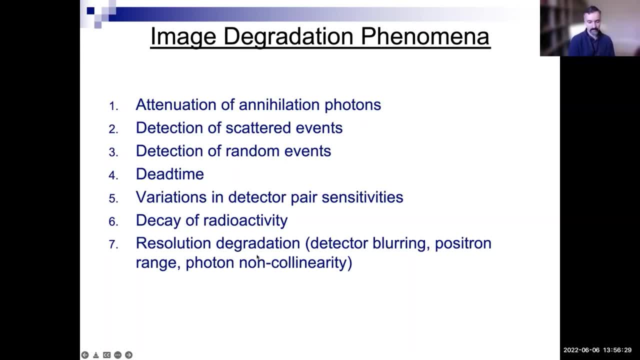 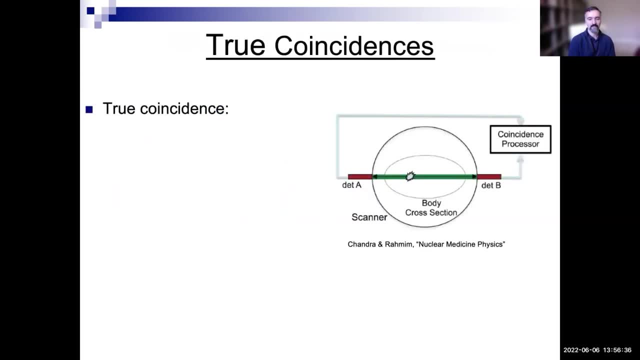 Things like positron range- we sort of talked about that Photonaut community. I'll talk to you about it. Depression movements- So these are some things that degrade quality and quantitative accuracy of PET images. How do we tackle them? So let's talk about what a true coincidence actually is. 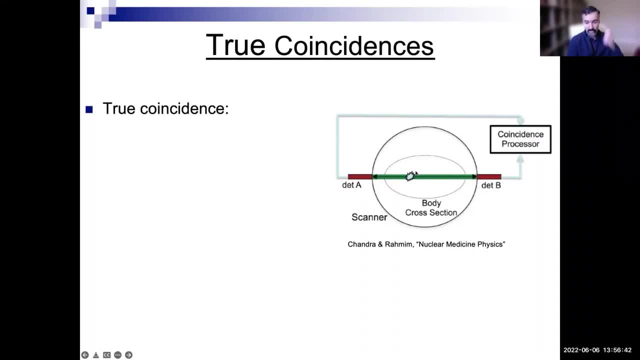 A true coincidence is a cleanup event, Right? So it's basically when the two anti-parallel gamma rays are detected, they're just being good, Okay, nothing's happening to them, You're just receiving them, That's it. you draw a line of response. 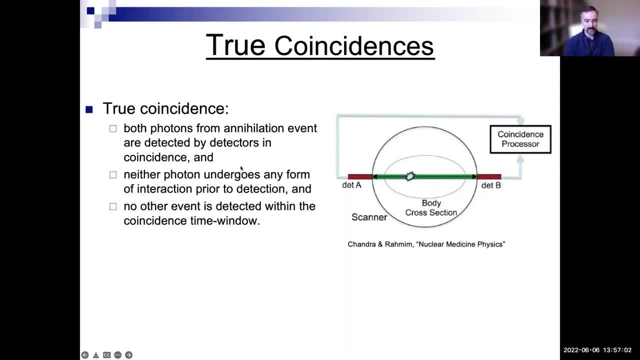 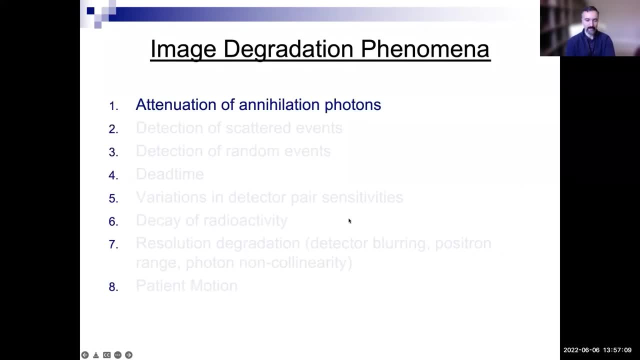 Yeah, and neither has undergone any interactions prior to being detected, and nothing else is being this, is it? these are the only two things that are being detected right now. Simple and easy. So let's talk about these eight things. So, attenuation, what is attenuation? 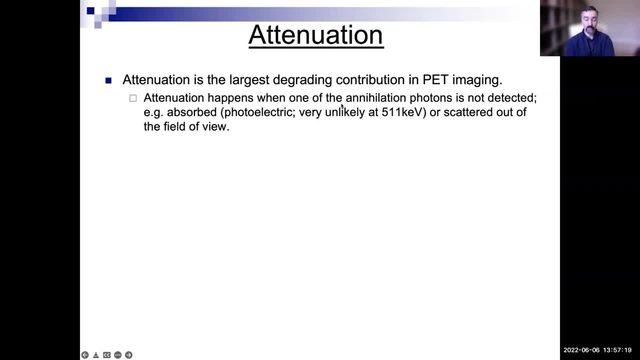 Attenuation is the largest degrading contribution in PET. The good news is it's easy to actually correct for it in PET. Just hold on a sec. It happens when one of the annihilation photons is not detected. For example, it could be absorbed. 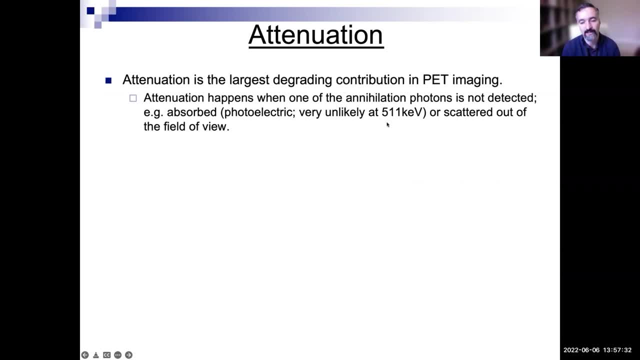 like photoelectric effect, but that's not likely at all in 511 kV. It's more likely at 140 kV, for example for technician imaging, But or it could be scattered out of the field of view, The two photons, along a single line of response. 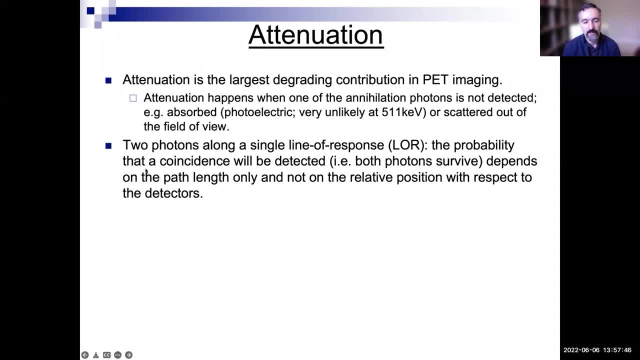 consider them. The probability that a coincidence will be detected, meaning both will survive, depends on the path length only, and not the relative position. Look at this here. You got an event here. it gives you two gamma rays. The probability that neither of these two is attenuated. 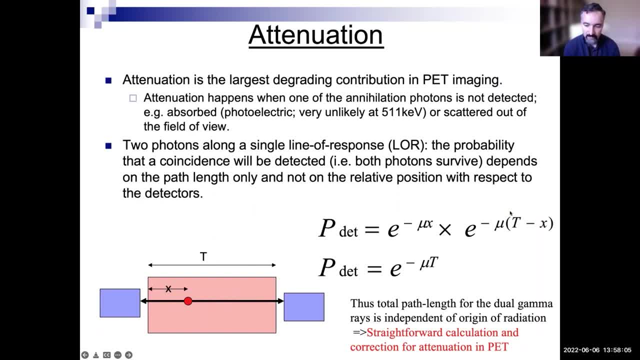 therefore, both of them make it turns out to be. you can look at some math, but it doesn't matter where the source is. It only depends on the line of response, the length of this. This length Doesn't matter if this point is here or here, or here or here. 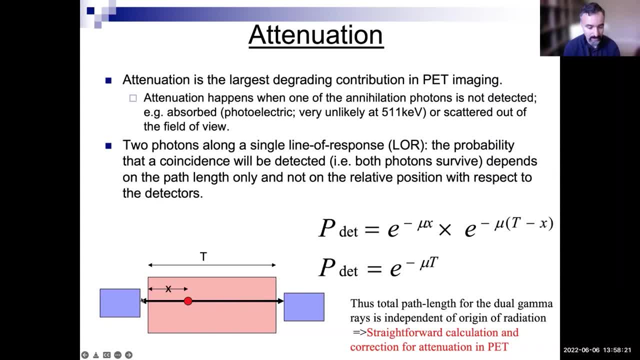 That's unlike SPECT. In SPECT, if you're here, because you're only giving one gamma ray, not the other second one, whether you're here, you're attenuated less than if you were here, Because if you were here, 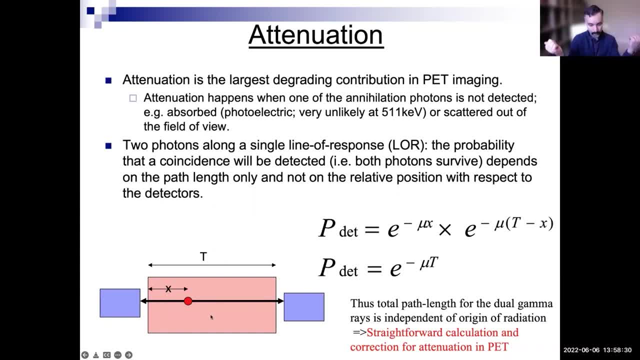 you would have to go through a longer distance. But here, because you got two photons, both of them have to make it, So it doesn't matter where the original source is in this line of response. So this actually allows you to do a straightforward calculation. 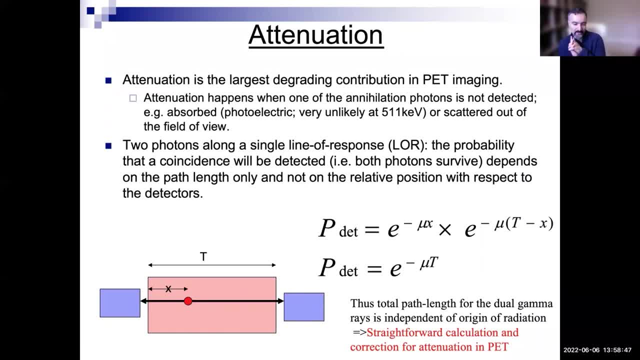 And this is why people used to think PET is quantitative but SPECT is not, because they didn't know how to deal with this in SPECT. But it turns out in SPECT too. you can do it. It's more complicated than PET, but it can be done. 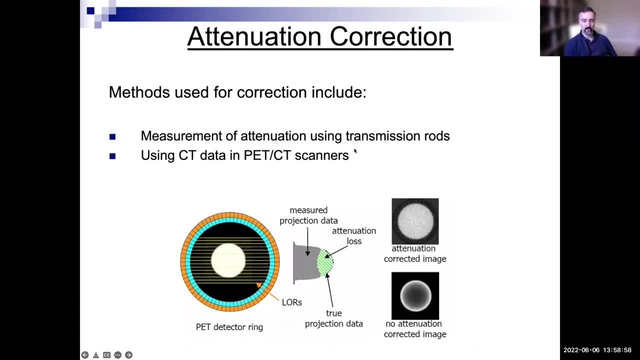 So attenuation correction, you could again use transmission rods or you could use CT to measure how much signal is being attenuated And once you measure that, you can apply that to the reconstruction using different ways like pre-correction of data. 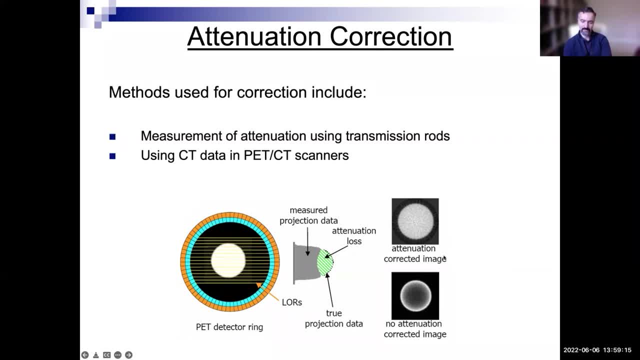 or in the reconstruction phenomenon, step itself and go from an image like this that has this dip in the middle, because so much is being attenuated, to something like this. What about scattering? Scattering- is this When you've got an event like this? 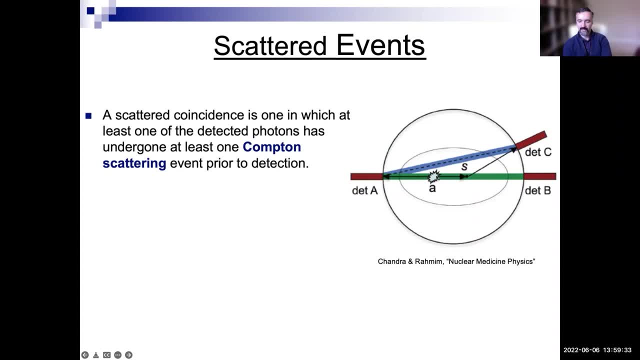 one of them make it fine. but the second event: before it gets to detector B, it gets scattered and unfortunately is detected here. So you think now these two photons received it. You don't think they did receive it. You think that the original line of response you draw. 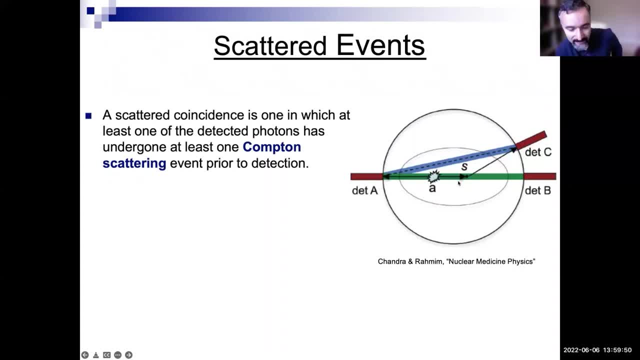 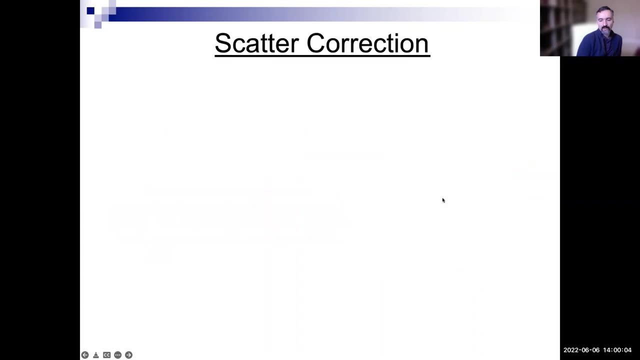 is this and you think it must have come from somewhere along here. So you've been led by the scattering, misled by the compound scattering And again, because the direction is changed, you're gonna be assigned to the wrong line of response. 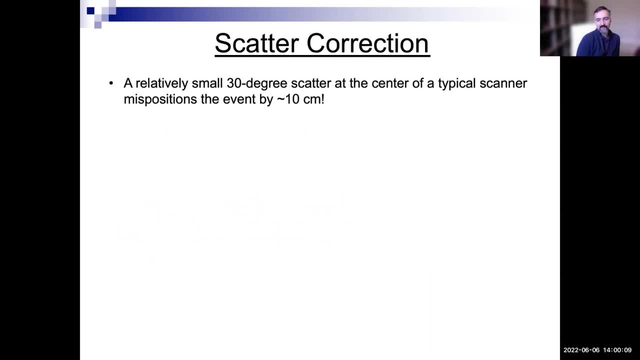 And even a small 30 degree scatter at the center of a typical scanner can misposition the event by 10 centimeters. So it's really messed up actually, And in 2D mode, scattering used to be only 15% of the events. 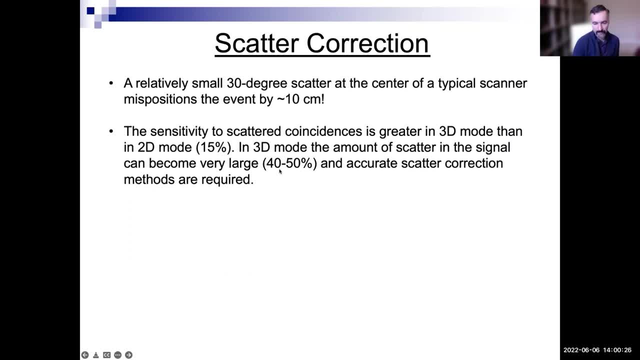 In 3D data acquisition mode it's like 40 to 50% of events are scattered. It's massive. So people used to say scatter is the enemy. So you gotta deal with scattering. But there are very good techniques. 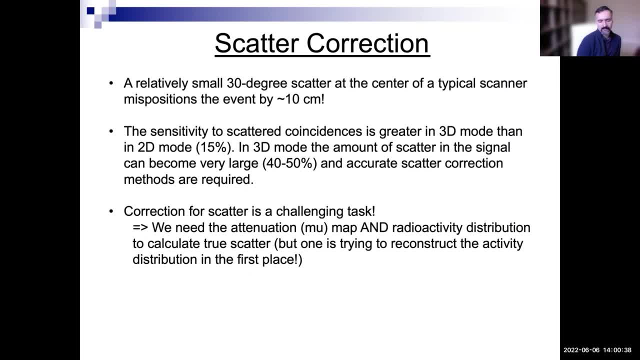 It's challenging but it's been tackled. It's challenging because to estimate scatter you need to know the reconstruction, but to do the reconstruction you need to know the scatters. But then you can do iterative methods, for example. 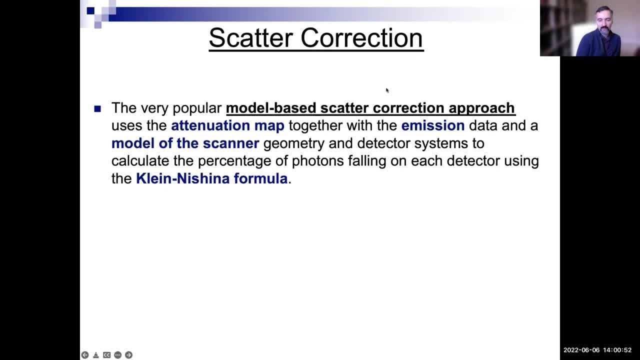 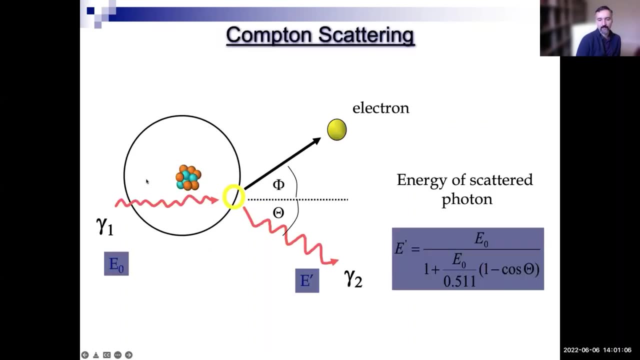 or other techniques. There's a very popular model-based scatter correction approach that uses the attenuation map. They measure using CT along with the emission data model of the scanner and modeling of the phenomenon of scattering- so-called Klein-Meschina formula to figure it out. 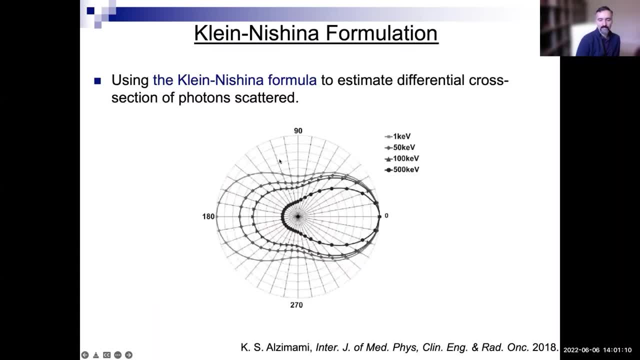 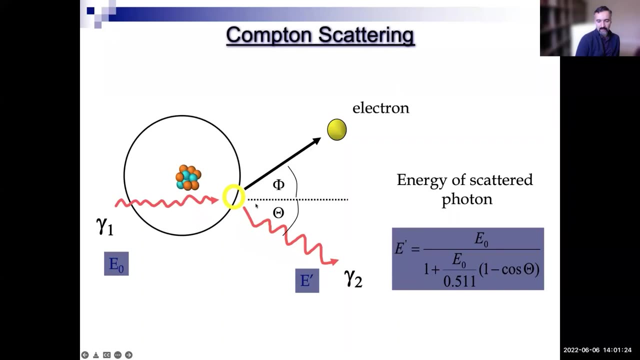 So again you've got content scattering happening. There are formulas about. The Klein-Nishina formula sort of gives you estimates of different cross sections of photons. For example, if you're coming along this direction right and you've got a deviation here this angle, what is the chance of getting this deviation versus that deviation versus that deviation? 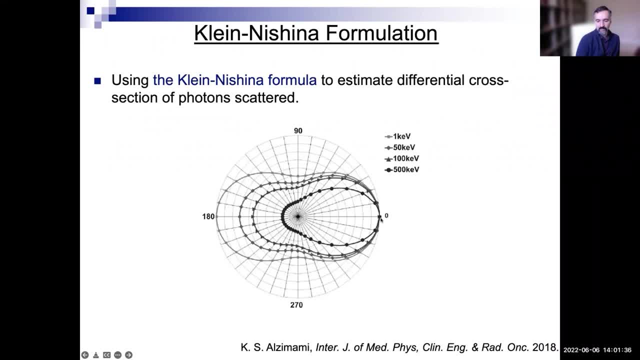 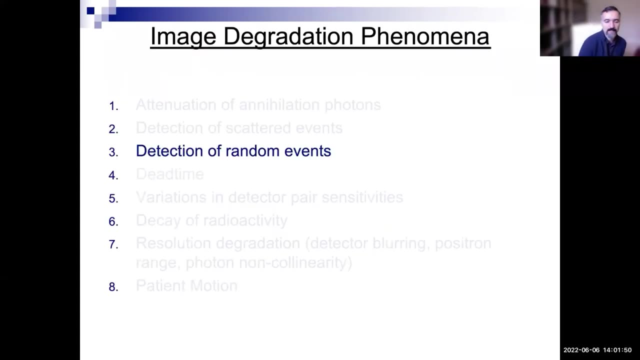 So, for example, for different energies, zero degree deviation. you know this is a likelihood, relative likelihood. You can sort of see zero is here, 180 is here and things in between are like that. But you can calculate those and build those in your scattering calculations. 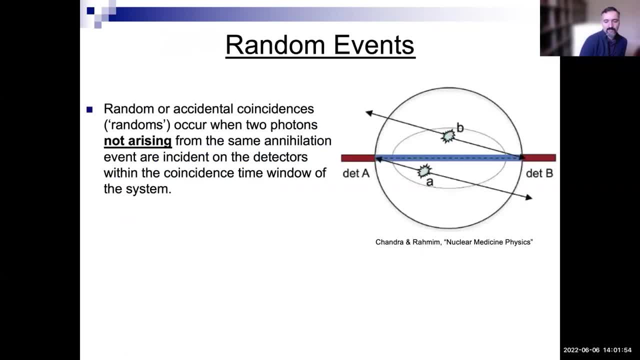 Detection of random events. So what are random events? So look at these two. just hang in there with me. Look at these two events. These are two separate events. These two events have nothing to do with each other, but by bad luck they took place at the same time, almost the same time, And by another bad luck, one of their events was lost, let's say, due to attenuation. 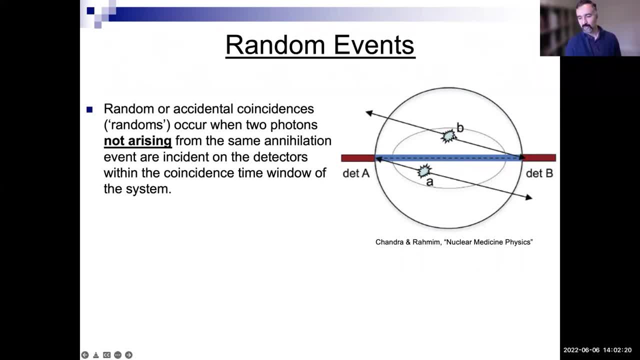 It never made it to the detector, but the other one did So. one event from this, one gamma ray from this event and one gamma ray from this event made it. These two others were lost And by bad luck they were at the same time and suddenly the PET scan is confused. 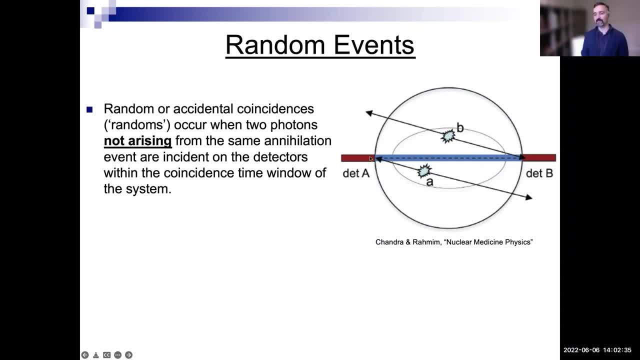 It's like, what's going on? It's like what's going on. It's like, oh, I just got something here, I just got something here. It's all at the same time. It must be from the same event. So I'm going to draw a line of response here. 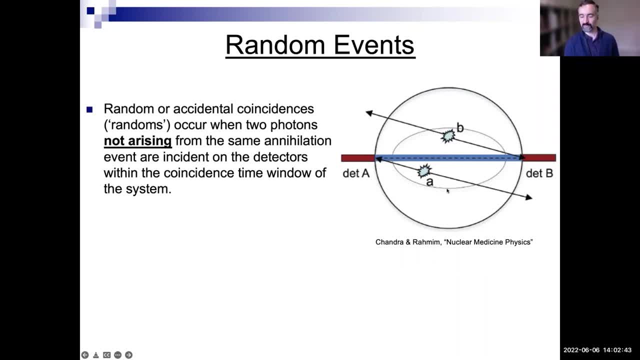 It must have come from here some event, but it was actually two events at two different places, So this is called a random event, random coincidence when two photons not arising from the same annihilation are incident and detector within the coincidence timing window. 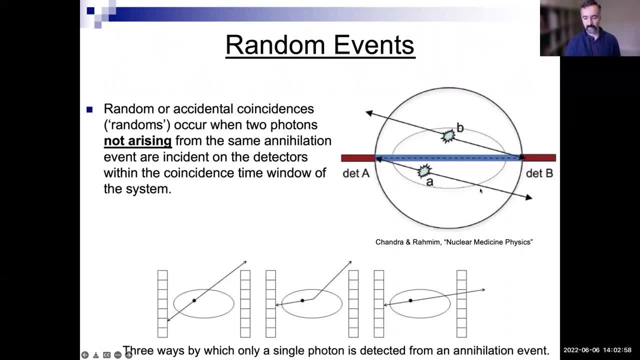 And why is this other event lost? It could be due to attenuation, for example, that this event is lost, Okay. so, for example, it got scattered away, so it got lost, But it might have also not ever even been meant for detection, Like, if you've got an event like this, this one will only give you that, whereas this one was never even meant to be detected. 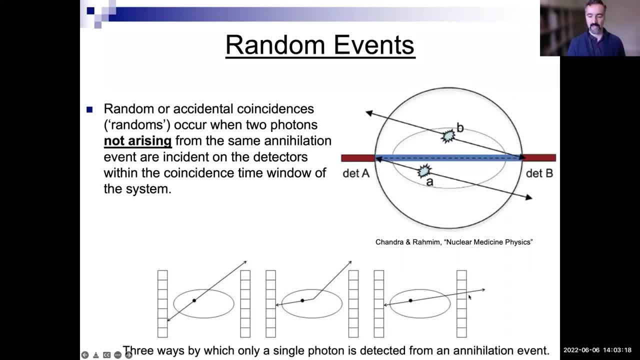 So you've got a single event here, a single, And you could also, just by bad luck, again go through the detector not being detected. So you're going to get these single events single hit, single hit. These two single hits are at the same time. I'm going to be confused in my system. 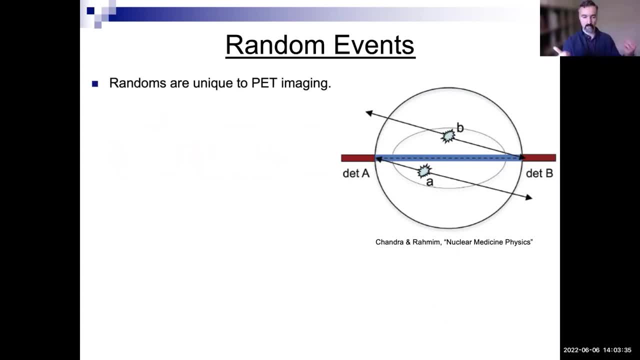 And randoms happen in PET because you've got two photons, we've got a coincidence detection system, And so there are formulas- I won't go through this, but there are formulas- to calculate, based on some measurements that we make, what is the likelihood of measuring randoms, And you can actually build those. 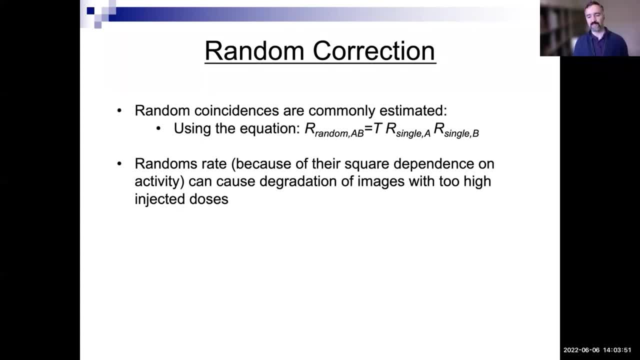 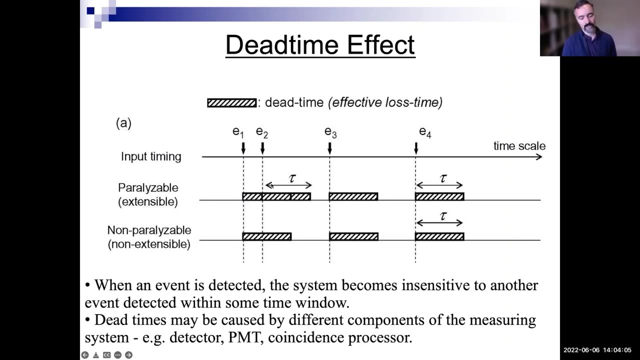 into the reconstruction. There are ways to correct for randoms. It seems like a very complicated phenomenon but actually it's relatively easy to correct for It's almost like a background correction, I think. Dead time- we talked about dead time a little bit. You can you have. you can have two kinds of different. 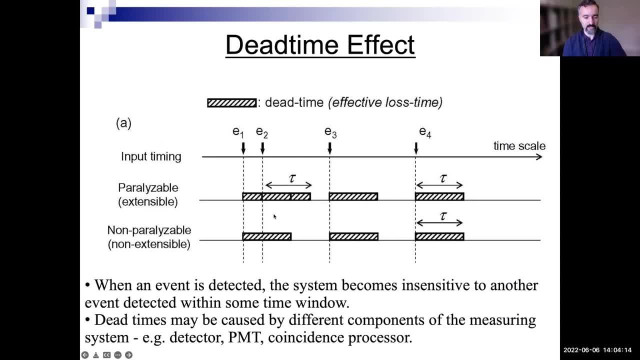 types of dead time. one is paralyzable, one is not paralyzable. Paralizable sort of says event 1 came in. I need some time to process it. let's say this much If you come in in the middle of my processing time: 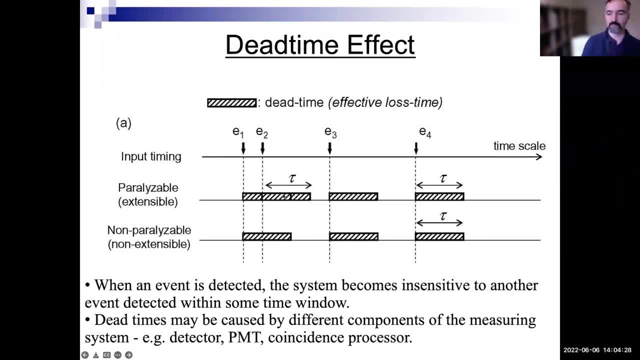 you've disrupted me, you've paralyzed me and I'm going to penalize you because I don't know what to do next. Non-paralyzable. which is better. it says: okay, fine, You come in, I'm going to ignore you, but at least you won't paralyze me. 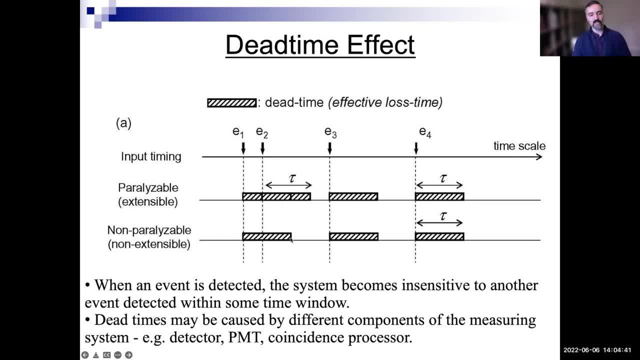 I'll be done for the first event by this time. So some phenomena and dead time happens along the chain of imaging. You've got scintillators, right. You've got PMTs. You've got the electronics. You've got the coincidence detection system. 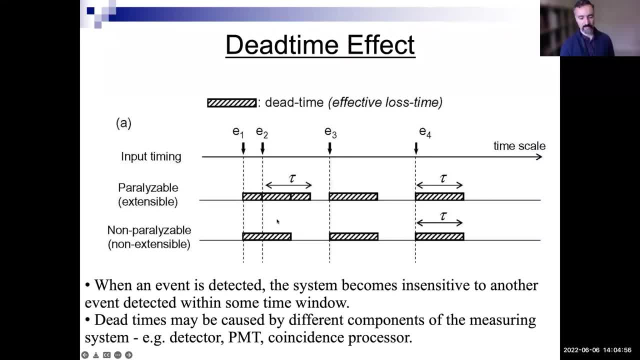 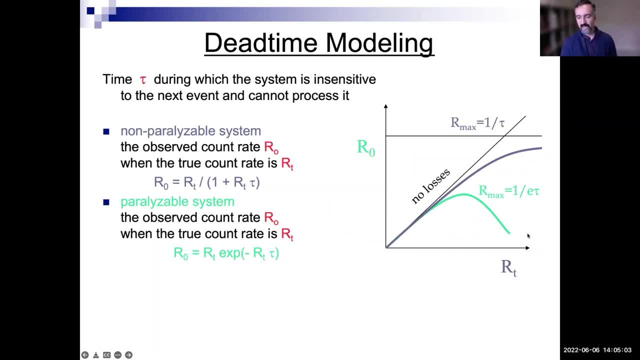 Some are paralyzable, Some are non-paralyzable, But the point is that dead time is there. okay, So dead time is there. And again, this is the incoming rate of events. As the number of events increases, the actual number of events you measure does not increase. 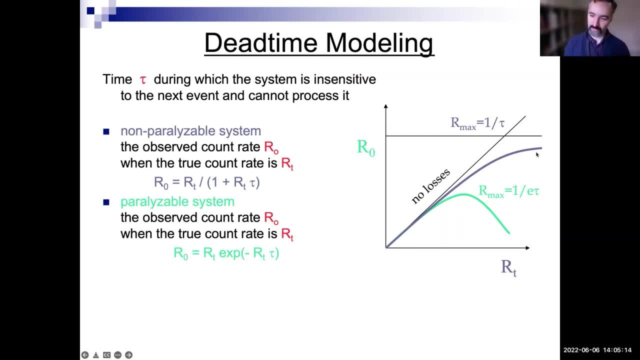 linearly because you cannot handle the truth. okay, So there's more dead time. But if it's paralyzable, not only does it not go up linearly, at some point it starts to be truly paralyzed If there's so much signal coming that I cannot process anything. 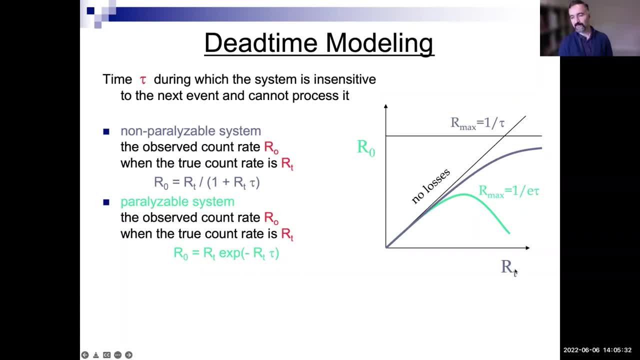 I don't have time to process anything, I will not process anything. So in an extreme case, when you move here down here, you might actually end up measuring nothing, because I'm totally paralyzed. You're overwhelming me, I cannot even process a few events here. 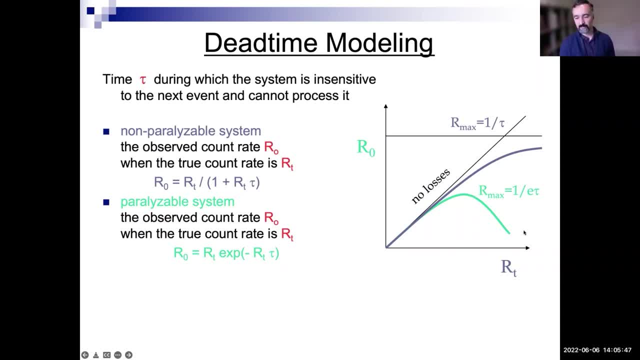 There's some formulas for it, but that's the essence of it. Paralyzable is worse than non-paralyzed And again, in nuclear medicine we have a combination of paralyzable, like scintillation detectors, and non-paralyzable, like some electronics contributions. 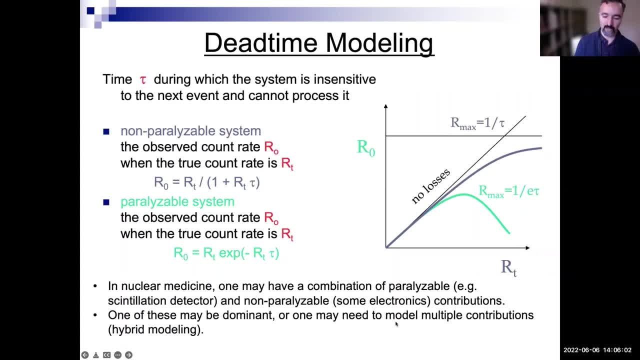 It depends which one is dominant, right, Or when we need to model multiple contributions, like hybrid modeling, which one is you know. So, for example, I used to work on a scanner. In that scanner, the key paralyzation was sorry, the key dead time effect was because 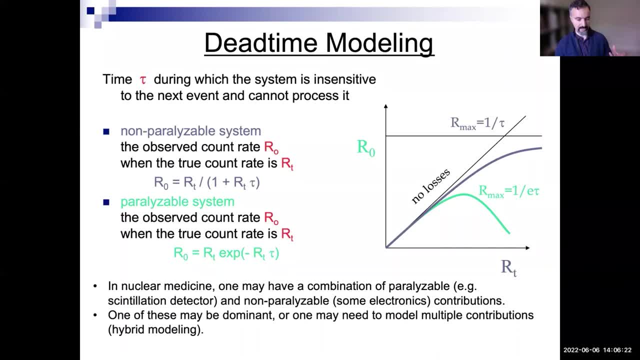 of the coincidence circuit. It just couldn't handle events And detectors were not. It can't handle it. So this was the bottleneck. If you reach a certain amount of counts, let's say 30 million, you know singles per second. 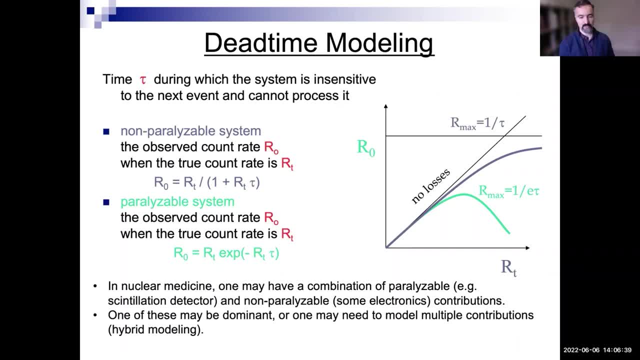 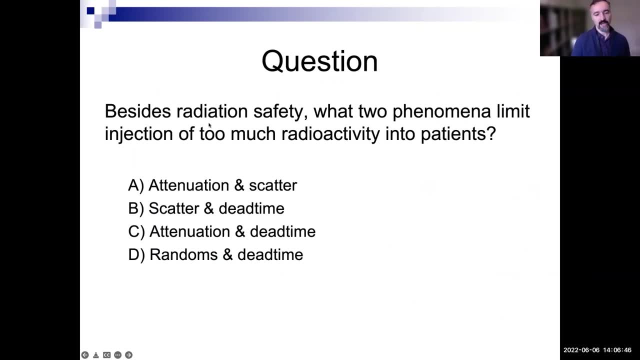 the coincidence. detection just would give you artifacts. So it depends. So let me ask you all a question: Besides radiation safety, what two phenomena limit injection of too much radioactivity to patients? In other words, let's say radiation safety was not an issue. 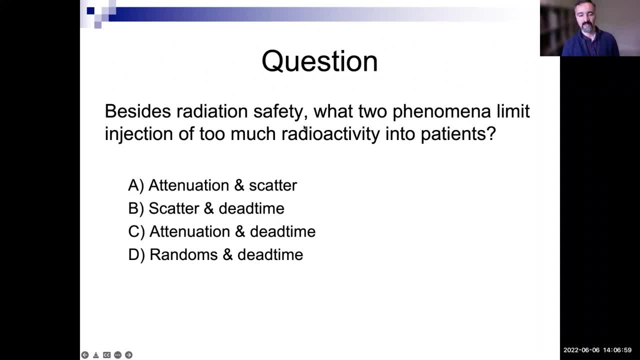 We could inject our patients however we wanted. Besides this, ethical and radiation safety issues, what are two things down here that tell you? you know what? No, no, no, You really should not be injecting too much. Attenuation and scatter scan at that time. attenuation at that time, randoms at that. 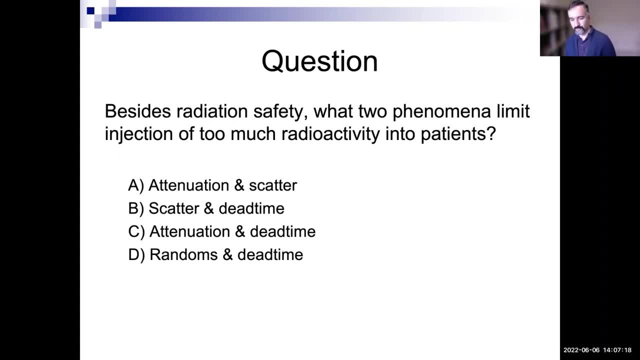 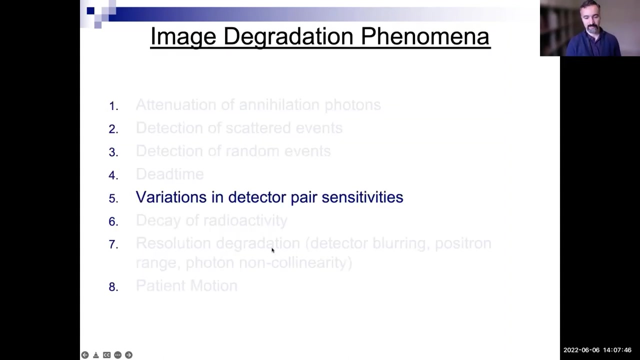 time. What does everybody think? Any suggestions? Can you help me narrow it down Anybody? So dead time is one of them, because I just said it. If, for example, oh, we got somebody saying something, Okay, Somebody saying not sure. 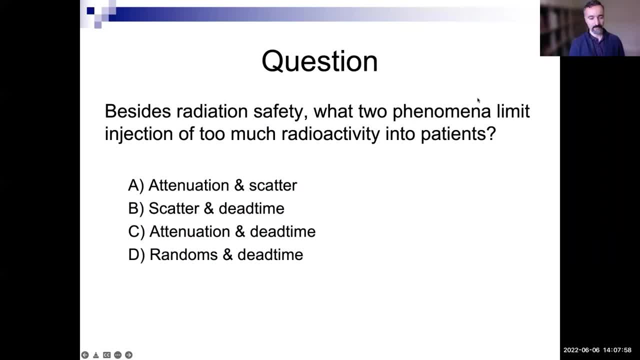 That's good, That's good to hear from you. So, yeah, Dead time is one because, again, if you inject too much, especially if you have a paralyzable system right- And we always have paralyzable somewhere- 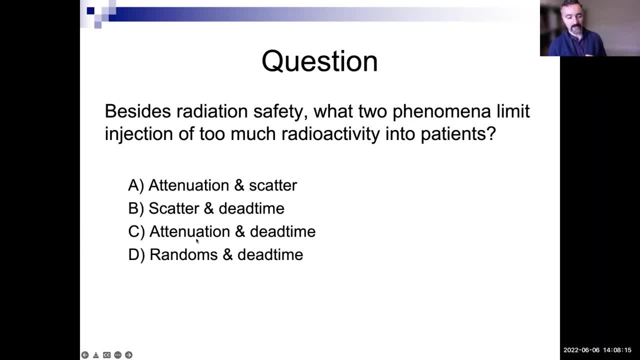 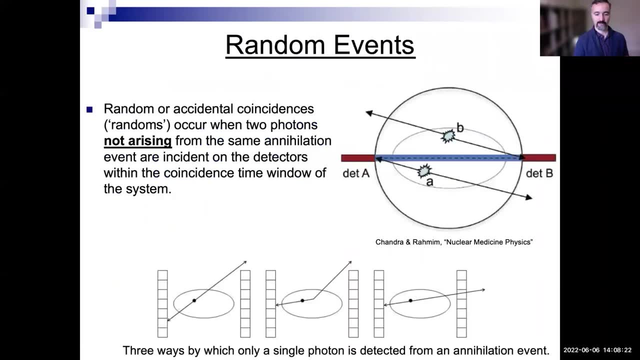 Then it paralyzes, gets paralyzed. So dead time is one, The other one is randoms. Why? Because, remember, randoms depends on two events being sort of arriving here, You have two events, One here and one here. And if 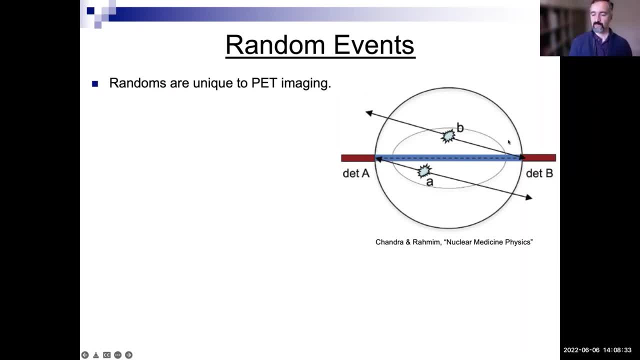 You're doubling or tripling the injected dose, you're going to get double or triple the number of singles. but then the number of randoms depends on singles here and singles there. So it's almost quadratic. It depends quadratically. The rate of randoms increases roughly with the square of the activity. 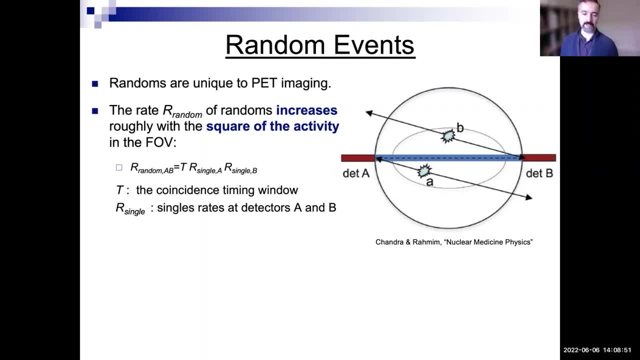 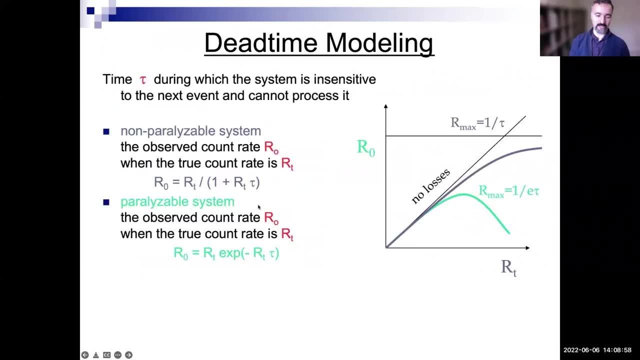 So if you double the injector radioactivity, you might get four times randoms. So at some point it starts to become terrible. So, so, so we cannot inject too much. Besides radiation safety and ethical issues, we can inject too much because of we're going to 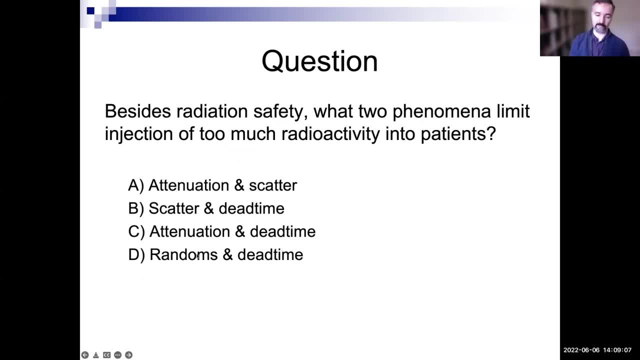 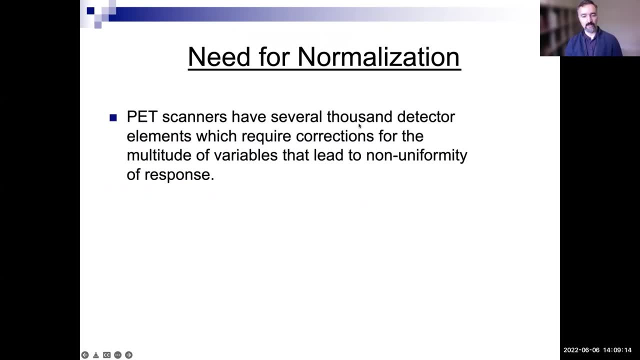 saturate the system with through that time And we're going to get a lot of brands. Okay, Variations in detector pair sensitivities is the fifth topic to talk about. You have several thousand detectors in pet, each requiring you know each of these pairs. 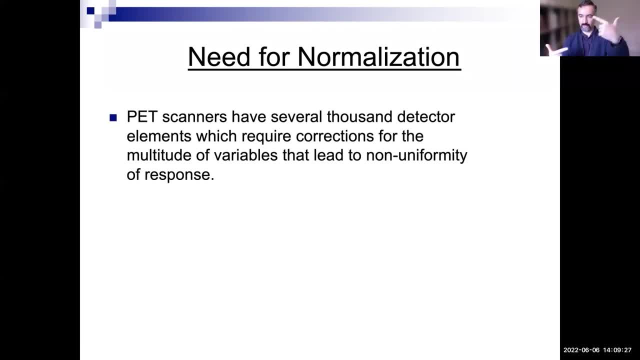 And sorry, I mean they're individually, they have their own issues and then they're impaired together and, like the geometric Sensitivity, sensitivity between different pairs And since the photon can enter, detected from different angles, there's angle dependent sensitivity is something we don't have inspect, but we have it because, again, we don't have physical collimators. 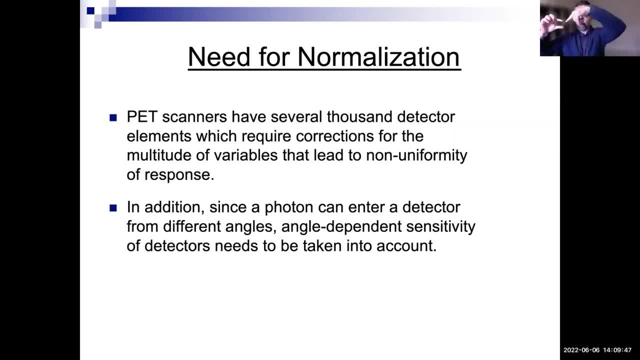 At detector, events can come at it at different angles, So it would have different geometric sensitivities. If I come this angle, it might be less sensitive to me than if I come this angle. So you've got a model for all of those and the the the the process to compensate for this phenomenon. 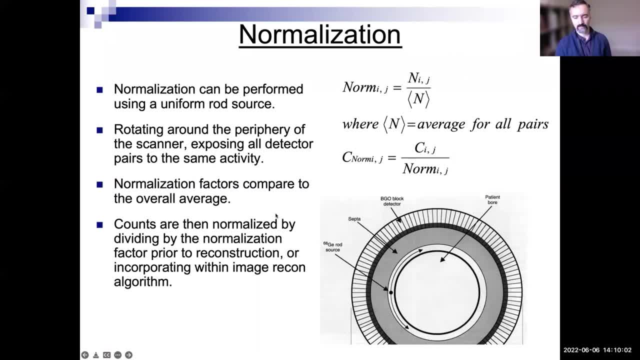 It's called Normalization. I won't go through details at all, but essentially you could have a rotating rod source, for example, that you put in there, You measure, you know how things are being detected, you know in in a simple, you know, original way you would measure all possible, collect all possible detective pair measurements and you just normalize. 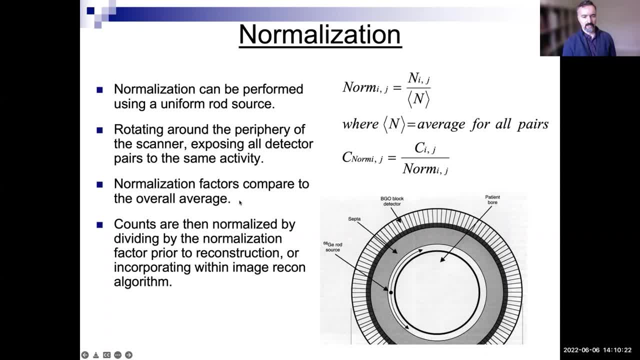 There are other ways to do um, uh, to do this in a in a more rapid way. But the point is that, yeah, I can measure you, but at the end of the day, you can measure this pair How? 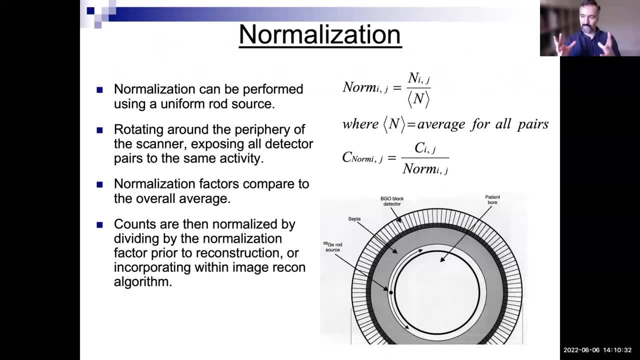 Sensitive is it, this pair? How sensitive is it? So if I have uniform activity, I should be getting measuring the same thing, or I have. if I have uniform activity in this rotating rod, whether I go this way or that way, or this space should give me the same activity. but it won't. 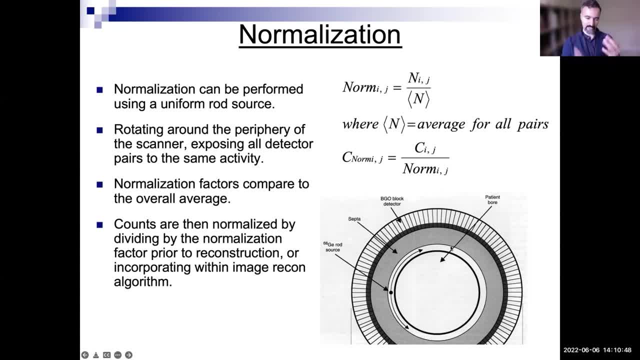 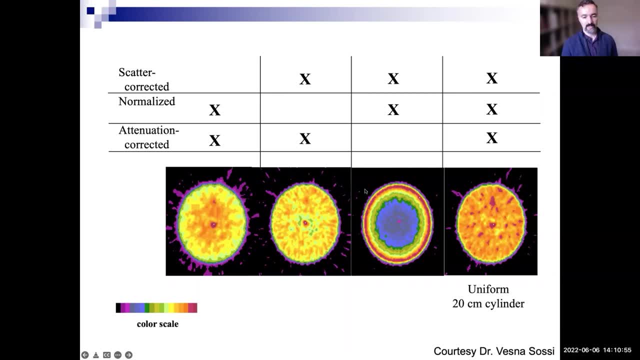 And, because of these, detect different pair sensitivities So you can correct for it. So examples where here's an image that has: uh, actually, let's look at this image. This is an image that has not been Corrected for attenuation. 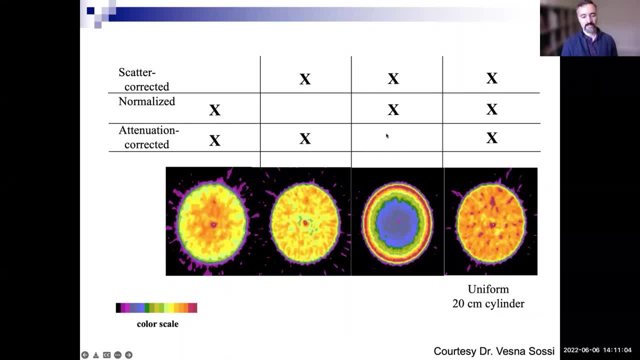 See, see this deep in the middle. If you correct for attenuation but don't worry for scattering, you get the opposite effect, which we sort of saw. for respect, If you don't go in for normalization, you get something like this, which is a little bit patchy: 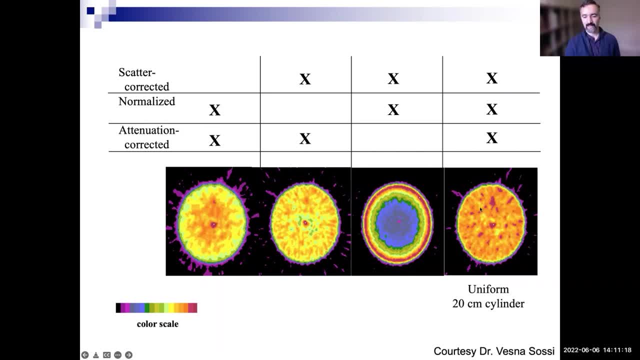 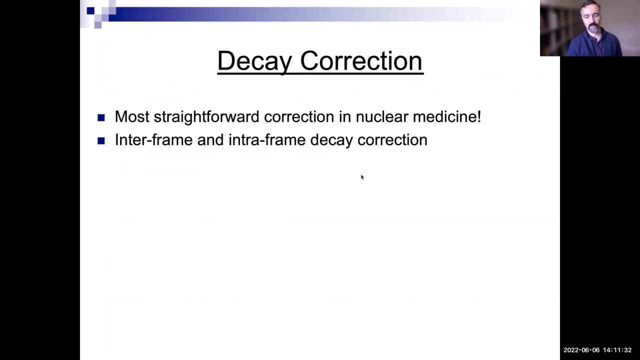 I suppose it's not as smooth as you can get it. And then if you do all of them, you get something like this, um which which turns out: I mean, I'm not, but to be smoother, just Better, uh uh. DK is the easiest one to correct, for it's the most straightforward correction: nuclear medicine: 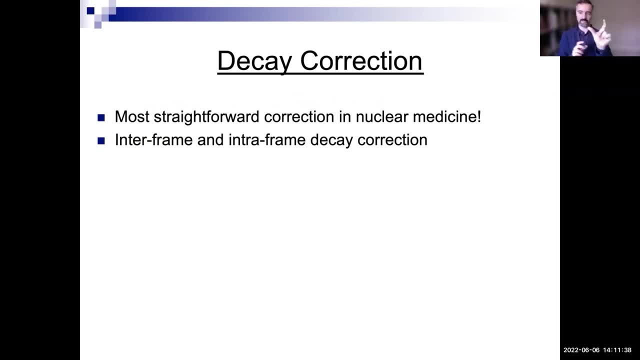 You can calculate how much within each frame- let's say you got five minutes acquisition- You know how much within that frame the activity decays. It's just a law of nature, You know it. And how much between frames, if you're doing dynamic imaging, or since the time I injected, how much has the radioactivity decay? 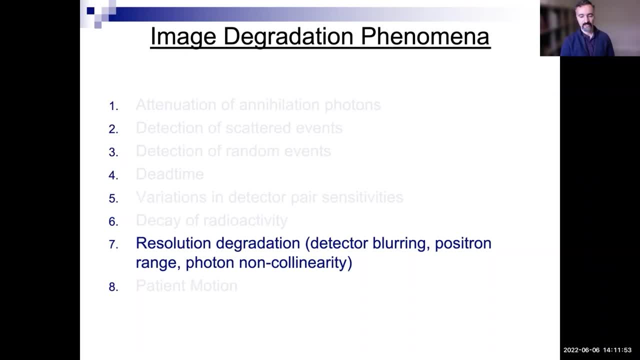 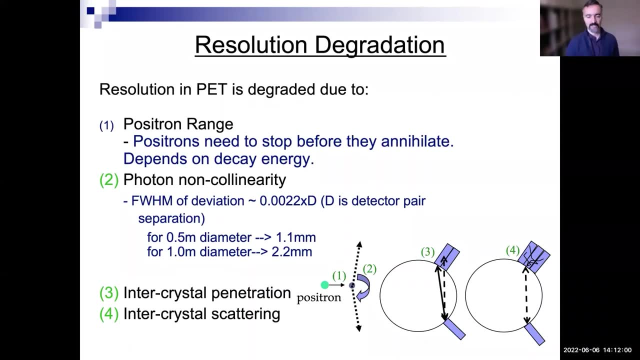 It's very easy, very, very easy, to do resolution degradation. You know all these different things that degrade the resolution of pet. you could actually model, but let's try to understand. And then first, before we take a break, um, the resolution degradation can happen due to a number of reasons in pet. one is positron range. 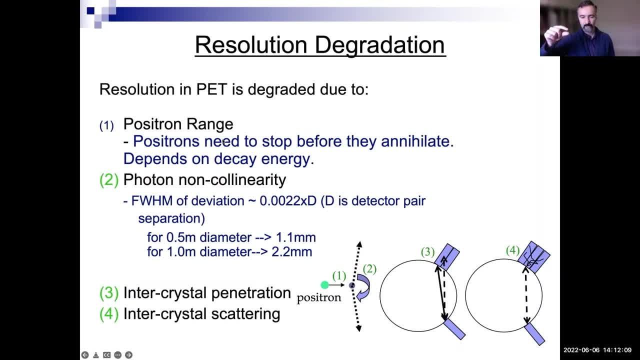 We already talked about that. The positrons need to travel a little bit before they get stopped and they combine with an electron to give you those anti-parallel gamma rays. Um, there's also photon non-collinearity. This may actually shock you, but uh, this thing happens technically. 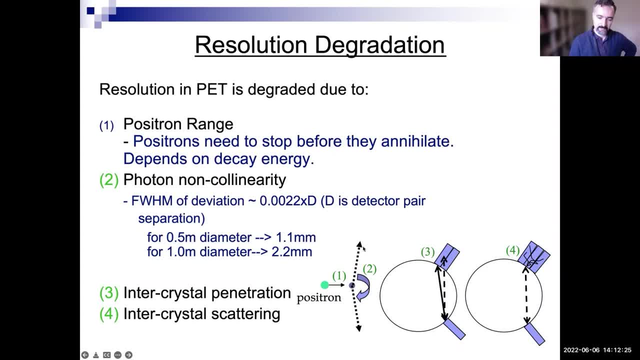 These two things may not be at exactly 180 degrees, It turns out, because the positive, for example, may have a more Momentum when it combines with an electron, there might be a little bit of a forward bent. Now, this is not a huge band. 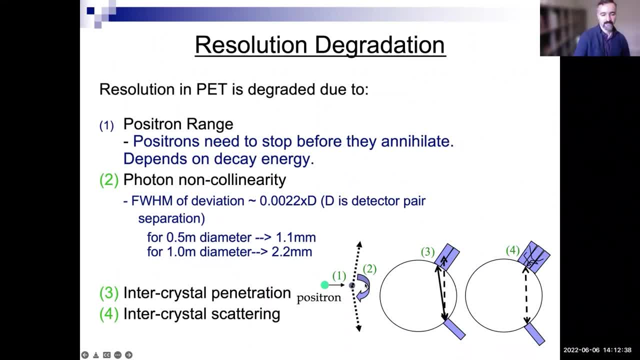 This is an exaggerated drawing. We're looking at like a less than half a degree deviation, but this less than half a degree deviation in the large distance of a like a one meter diameter scanner can give drives to something like two millimeters. one to two millimeter resolution degradation. 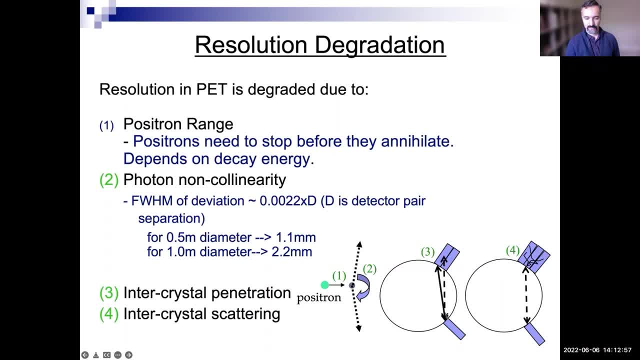 There's also crystal blaring issues. If, If I'm entering a Crystal at an angle before you're successful in stopping me, I may have penetrated to the nearby uh crystal And so I may be detected here- not here, because I penetrated sideways and it thinks I entered the crystal here. 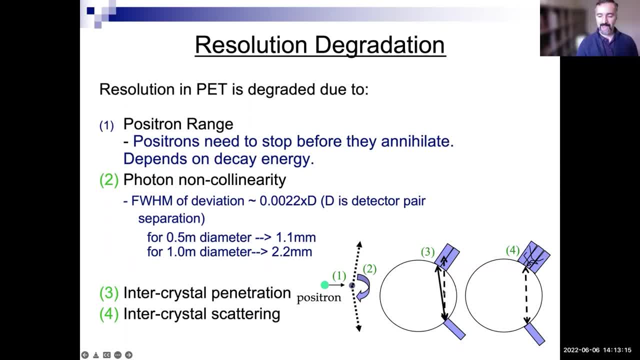 Whereas I didn't. this gives rise to the so-called parallax effect. As you move away from the center of the field of view, because you're going at the detectors at an angle um uh, you get the resolution degradation more here than in the center. 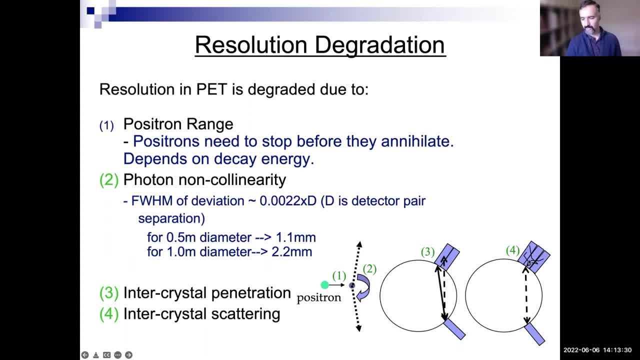 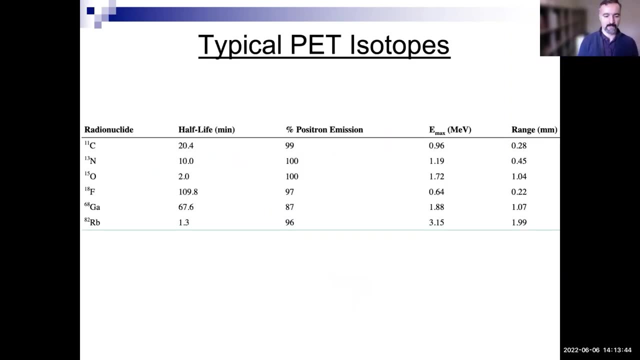 But even if you're going at it at, At at the straight angle or at the side angle, you may enter this detector, not penetrate, but you may actually be partially absorbed but then scattered to nearby crystals and just get degraded. So, um, uh. so I'm showing this because of the positron range that I showed you before. 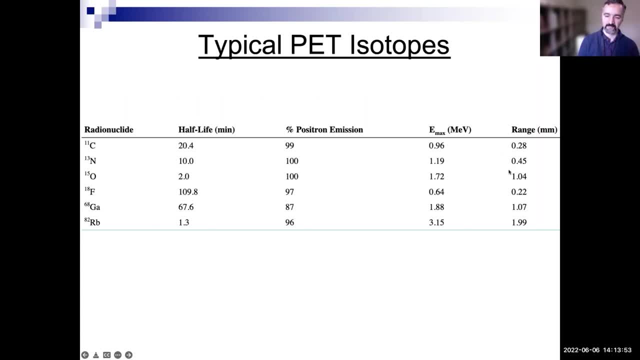 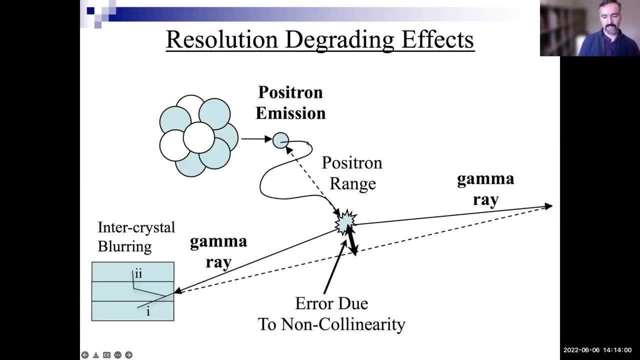 Again, the amount of positron range depends on the radionuclide. again, fluorine 18,, which is very popular, has very small positron range, which is good. Uh, another way of showing the exact same thing: uh, you've got original positron. travels a little bit. typically less than a millimeter, gets, um, uh, obliterated with an electron towards uh or annihilated uh, giving you the two gamma rays, but the gamma rays might be slightly bent, less than half a degree actually. 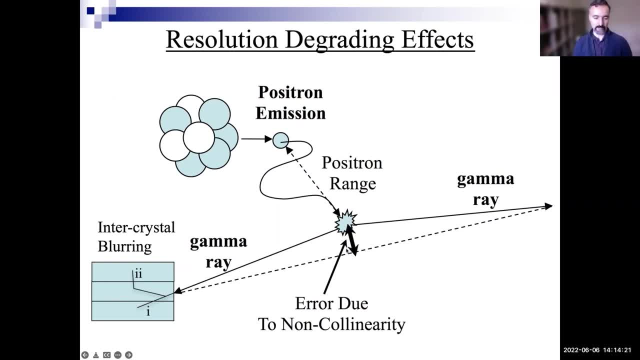 Uh, but this deviation might be about one to two millimeters. and then it enters a crystal. It may penetrate through. that's one kind of problem. or make, make it crisp, You make it scatter in the crystal. Anyhow, you're going to get crystal blaring. 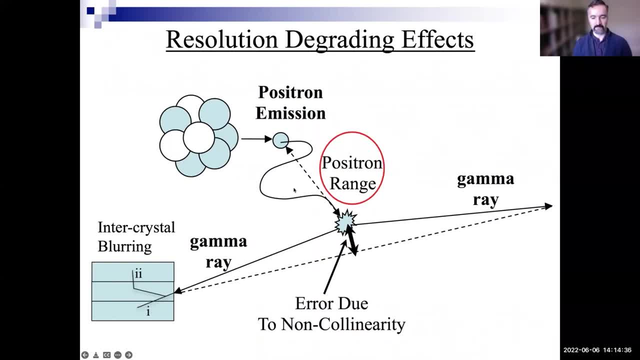 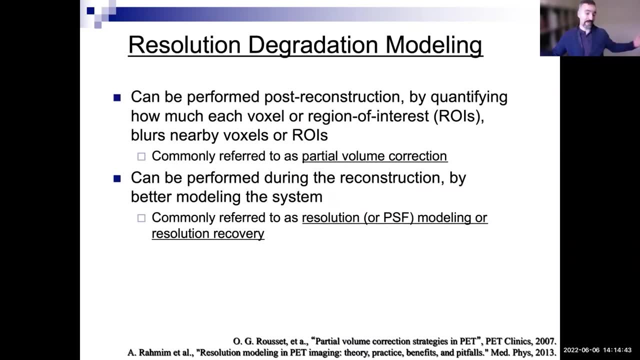 You enter this crystal, but you may end up being detected here or here. Yeah, So we just talked about this. Um, so you can actually. in the past, people used to say, well, that's just the way it is. 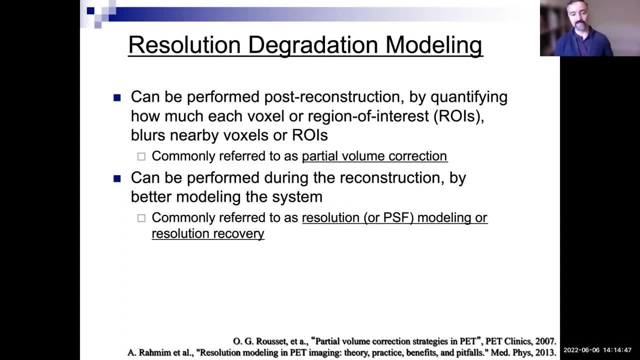 Images are degraded because they are, but no, you can actually try to tackle these issues. Um, so if you tackle these issues after reconstruction- people typically call that the partial volume effect- You model these phenomena, You try to sort of correct for them or account for them. 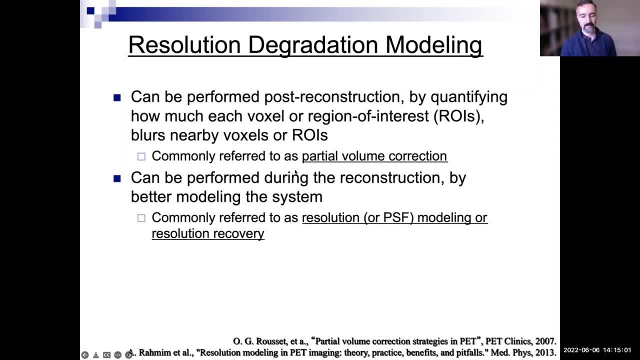 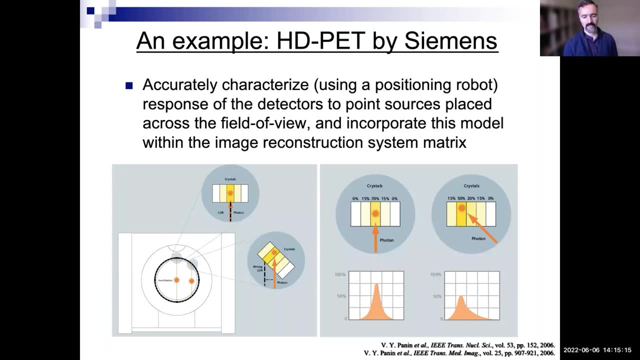 Model these effect events within the image reconstruction. We typically call it resolution modeling- in the spec world, more commonly, resolution recovery or PSF model, which the vendors are providing. Now it's giving you sharper images. Again, different vendors do it differently. 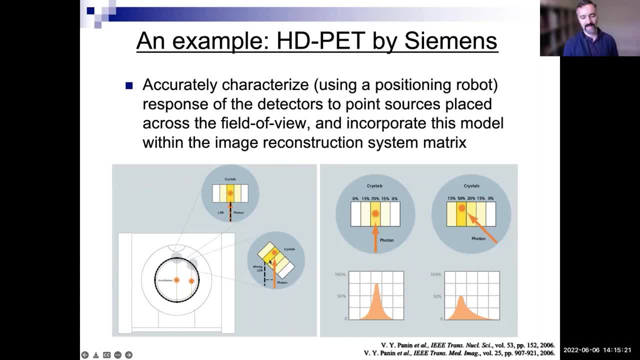 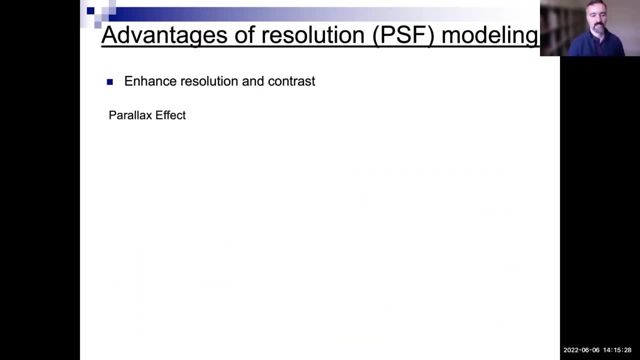 You can model, for example, what's the likelihood, if I enter a crystal at an angle, how I will blare, and you could model these blarings into your reconstruction, getting sharper images. So again, uh, here's an, here's a typical acquisition, uh, where you see the parallax effect as you move away from the center of the field of view, because you can't handle those uh events entering crystals at an angle. 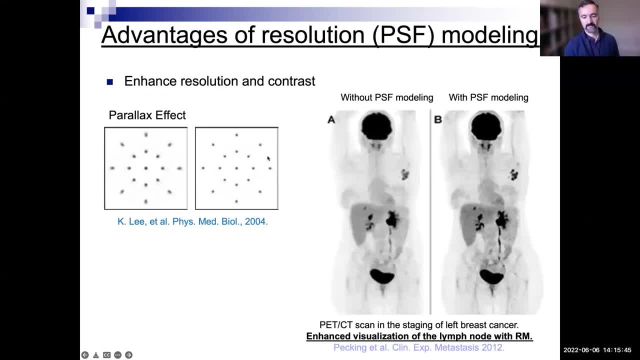 But once you do resolution modeling, you get less parallax effect. Here's an example of a of a reconstruction without PSF modeling and with PSF model. It looks sharp, It looks better at this, It looks better quantitatively. 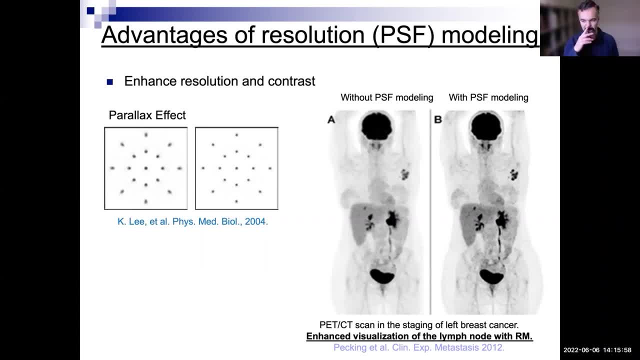 It can be better. detection wise, It can be better. It's not. It's not as obvious as time of flight. time of flight, no question. doing it is always better than not doing it. PSF modeling: it can improve performance, but, but you have to be cautious about it. 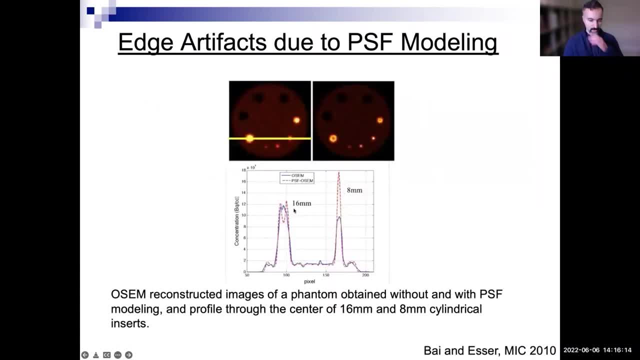 In fact, sometimes you may get um edge artifacts or overshoots. So here's an example where, at the edges, you may get these edge artifacts when you do resolution modeling or edge overshoots. So so, examples of images without 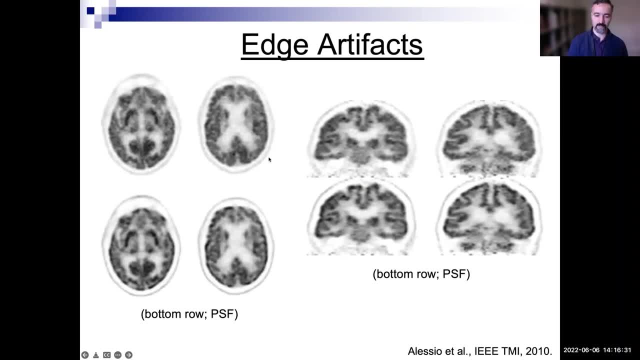 Uh, without resolution modeling. but when you do resolution or PSF modeling you may get these edge artifacts which are not real, so you gotta be careful about it. So for so some brain imaging applications. I remember when I was at Hopkins we would turn this off in the clinic. 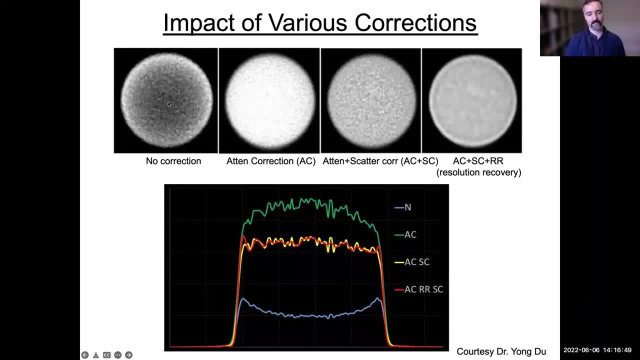 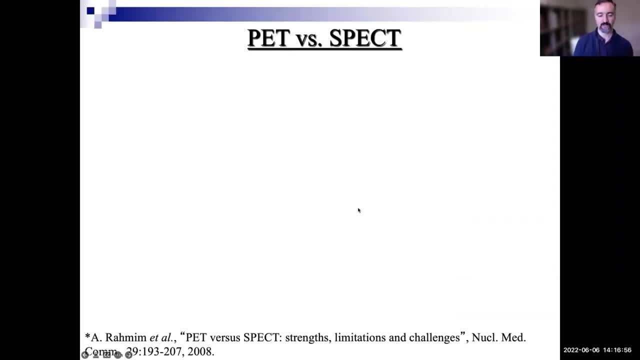 So again, I showed this before for for SPECT: when you do no correction, then then when you do attenuation, then you do a scatter and then maybe resolution modeling, the images change and tend to get better. So I have this. 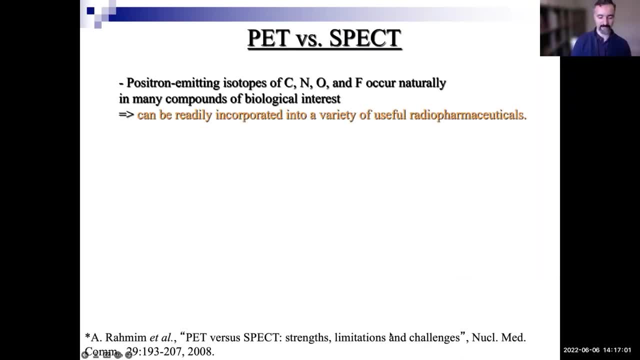 Um review article. you may want to check it out. It's called PET versus SPECT. To my great surprise, it's been accepted by the community with lots and lots and lots of citations. It's um, I don't know what. why? it's probably because there's a nice comparison between the two modalities, where it's almost like it's a face-off between PET and SPECT. and that comparison. 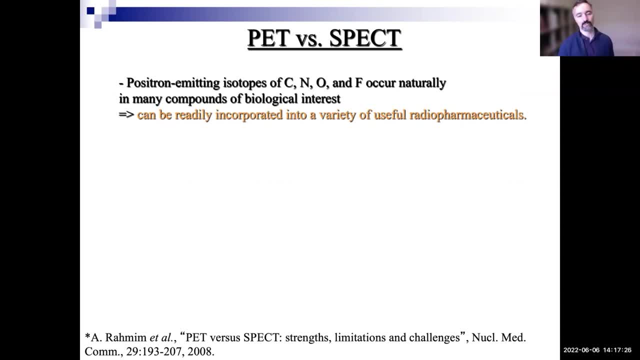 The reason I wrote it that way was because by comparison, sometimes you learn about each modality better. So when you compare the two, You, you, you learn more about each of them. So some of the key points in this article were that, um, you know, some positron-emitting isotopes can naturally occur, uh, whereas um, and therefore it can be readily incorporated in useful radiopharmaceuticals. 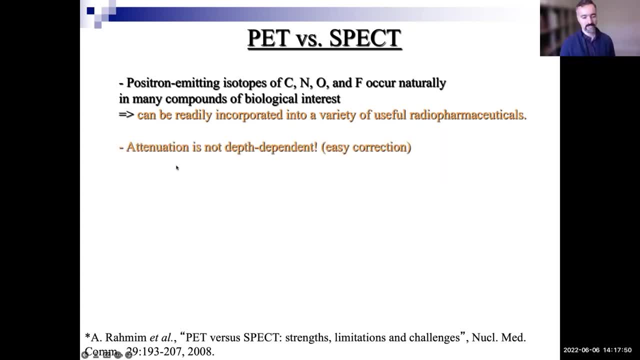 That's not really physics, that's chemistry. but moving on to the physics which is the core part of this article, attenuation in PET is not depth dependent and it's easy to correct. for We don't. We don't need a collimator, a physical collimator, in PET. 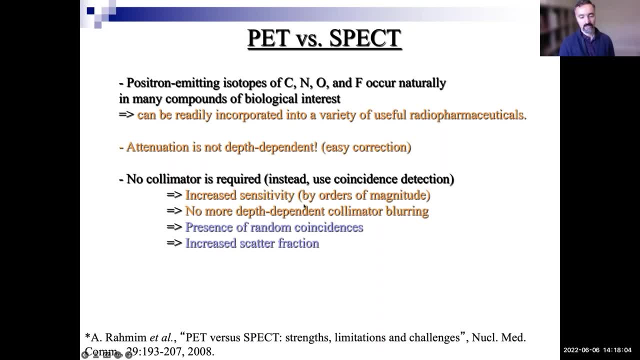 That's why we get a much better sensitivity. but orders of magnitude uh. the blaring is no longer dependent on your distance to the, to the detection system. But we do get random coincidences in PET which we do not get in SPECT, which is one reason you cannot inject too much. 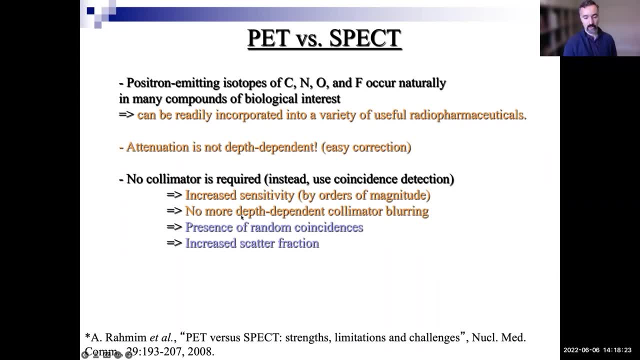 We do get increased scatter fractions. So these are more complications where the reconstructions tend to handle them well. Um, and There are some limitations where, for example, in PET we have positron range and non-collinearity. We don't even have that in SPECT right. 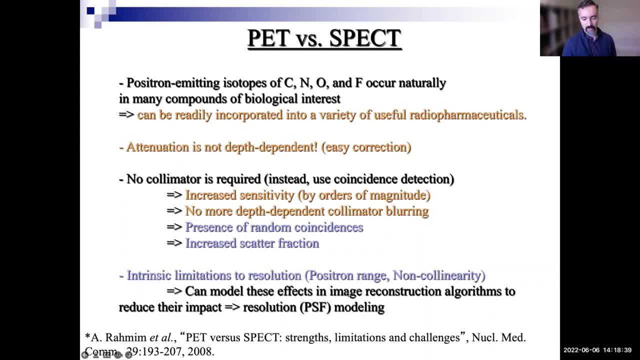 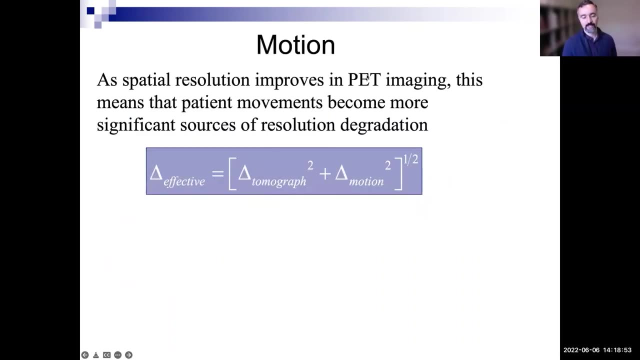 Um. but again, you can model these in image reconstruction algorithms, for example uh, as an example to the resolution model Um. so it's good to know all of these. Finally, patient motion- uh. and spatial resolution improves in PET imaging. you know, having gone from, you know order of centimeter to half a centimeter. 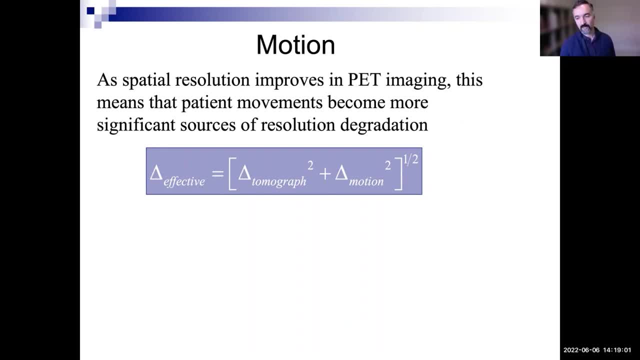 Now trying to get below half a centimeter on some PET scanners or small animal PET scanners we're looking at one or two millimeter, three millimeter resolutions. um uh, patient movements, you know, become more more significant because it's not just a resolution of the uh camera that matters but a resolution of the movement of the patient. 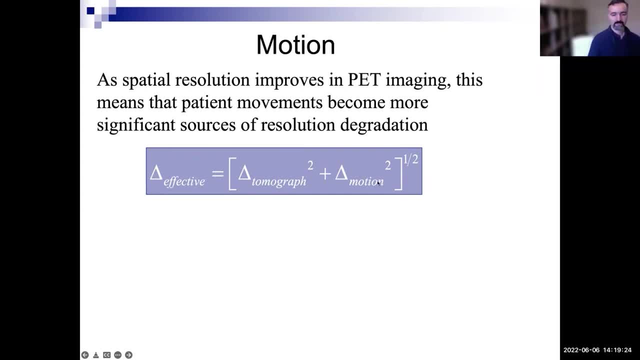 Like think of motion as almost like a blaring operation. So as you build these, you know great scanners understand, Unless you deal with motion somehow, then you start being, as you make this number smaller and smaller. if this number doesn't get better, you're not going to have a good, effective resolution. 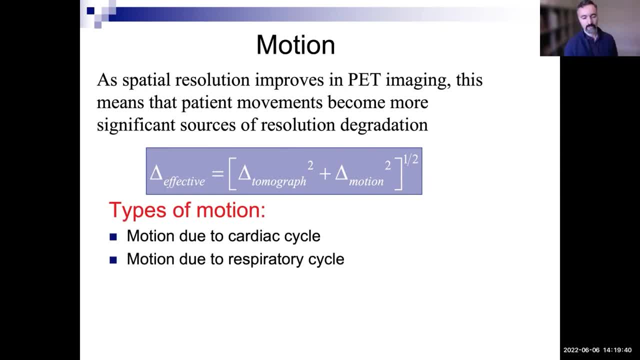 So there's different types of motion due to cardiac cycle, due to respiratory cycle, and other kinds of motion due to coughing, drifting, leg crossing et cetera, right, So, um, we sort of talked about gating methods before. uh, sort of right. 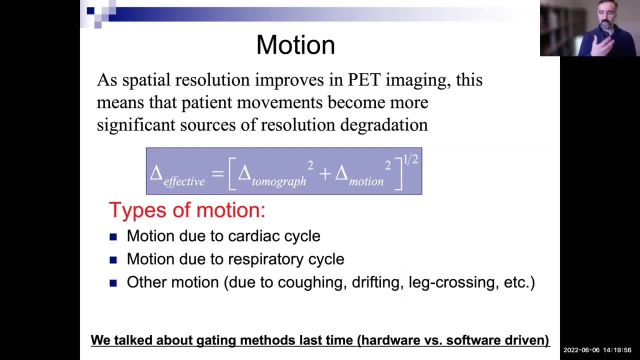 So the idea that you could do respiratory- uh, you can Measure the respiratory cycle and do gating and separate the signal into separate case. You could use an actual hardware to look at the human breathing cycle or you could do software data driven approaches. but this is an active area of research. 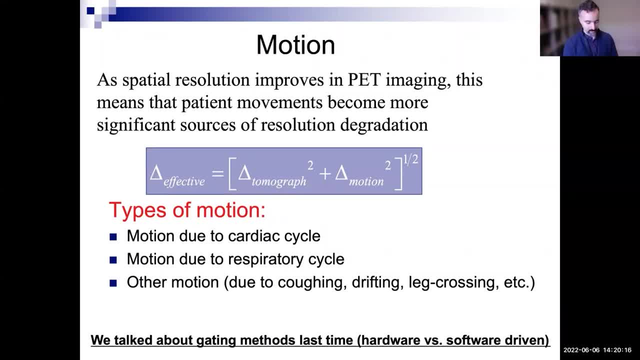 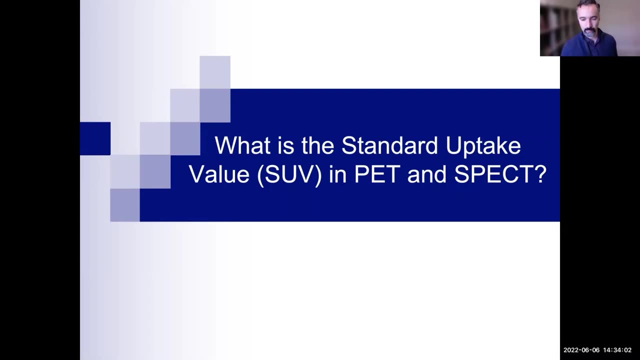 Um so. so those are eight confounding issues in pet, and there's a solution to every one of them And that's why pet images have become increasingly better. So the standard optic value SUV is is a term You'll keep hearing in the nuclear medicine world, especially in the pet world, but it's also increasingly using the spec world. 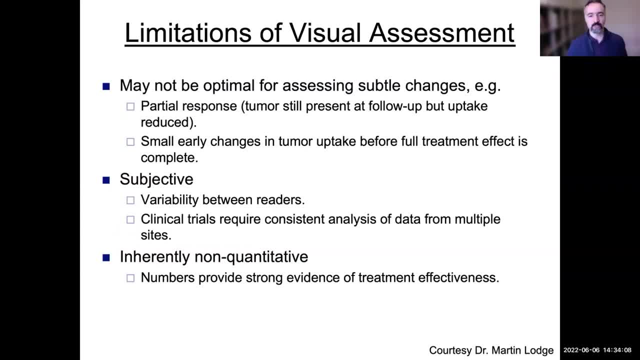 Um. so. so there are limitations to visual assessment. Um, it may not be optimal for looking at subtle changes like impartial response or small early changes before full treatment effect is complete. Um, it's a bit subjective. um, and some clinical trials. 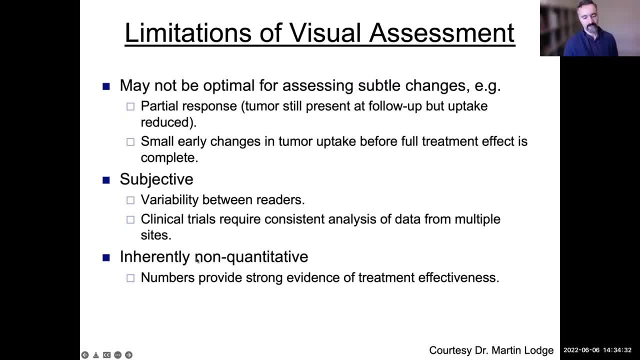 I think consistent analysis is is important and inherently it's non quantitative. That is not to to that, that is not to think that this should replace visual assessment. I think it's more about sort of providing value and added value to the human uh decision maker. 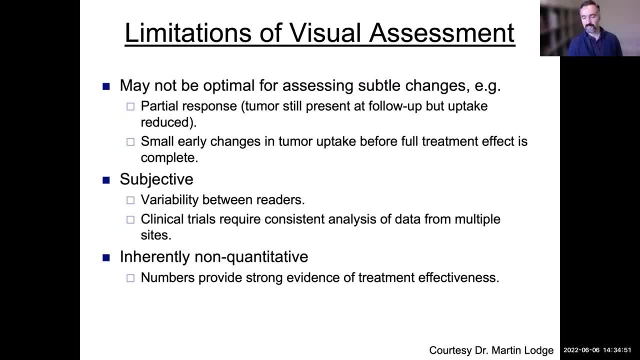 Uh. so, um, you know, the the human is central in this whole thing, and AI and quantitation all should be at the service of what, what, what, what we decide It needs to be done. Um, so quantification, uh, uh, is is important. 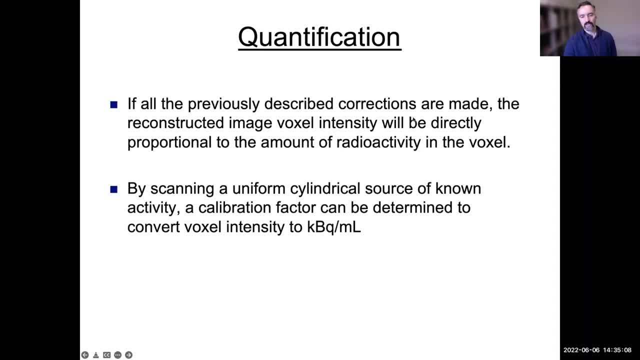 It can add value And if all the previously described corrections are made, the reconstructed image of oxygen intensity will be directly proportional to the radioactivity. So you know how much is there. It's kind of powerful actually. um, by scanning a uniform cylindrical source of known activity, then it can use a calibration factor. 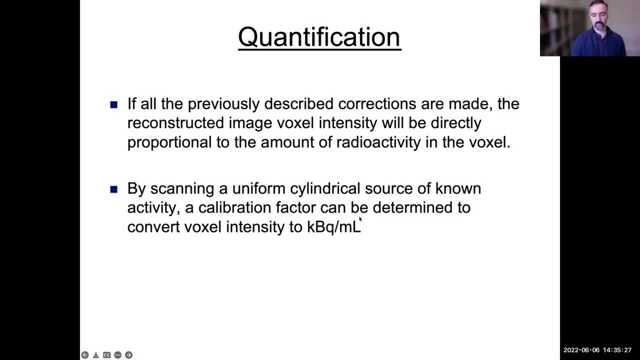 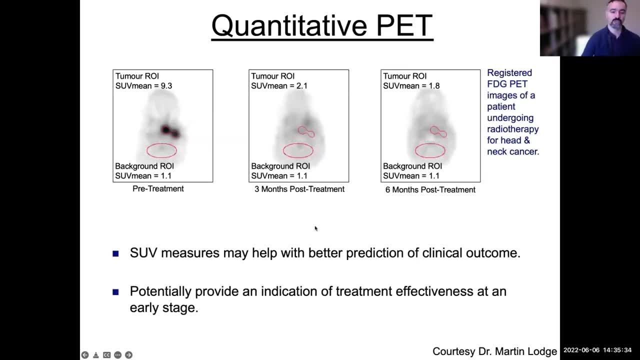 Um to to change. you know voxel intensities to. you know the radioactivity, Like uh, kilobyte corals per ml, whatever the units of concentration use. So here's an example of of a patient over time background radioactivity: SUV mean relative distributions. 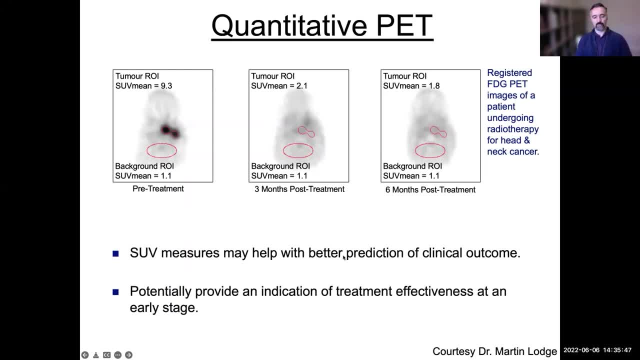 Um so so SUV can give you certain numbers. that allows you to track things. SUV is not concentration, It's like a normalized concentration with respect to, for example, some Of background. you'll see it in a second Uh, but it's, it's uh. it can be powerful in in looking at treatment effectiveness. 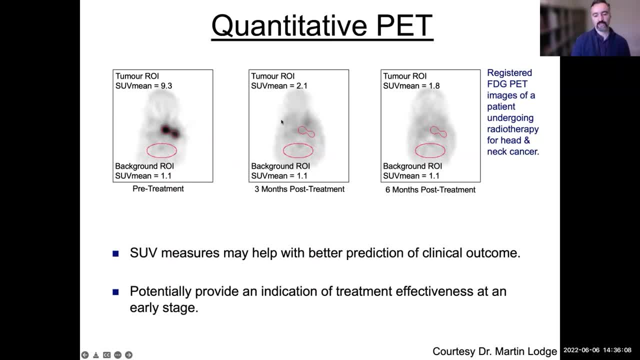 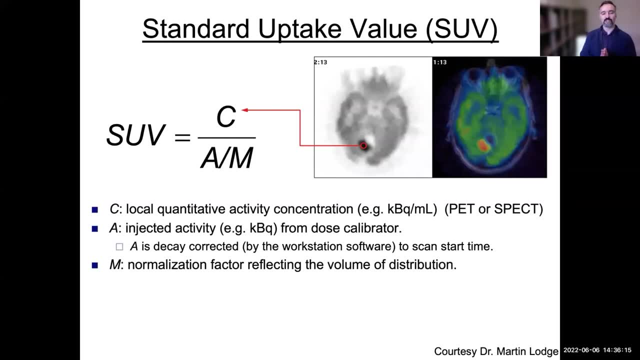 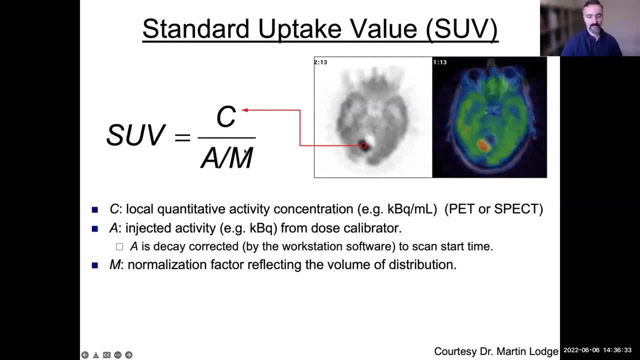 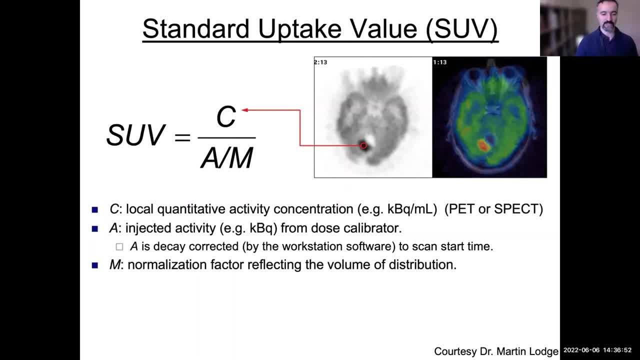 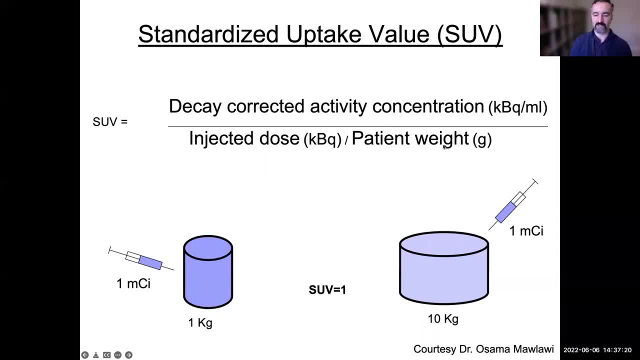 activity concentration divided by 18K T to 30K T injected dose divided by, let's say, patient weight, um, so you can sort of see that, um, you know, if you think of one ml as having one gram, like for water, soft tissue, roughly speaking an suv of one. 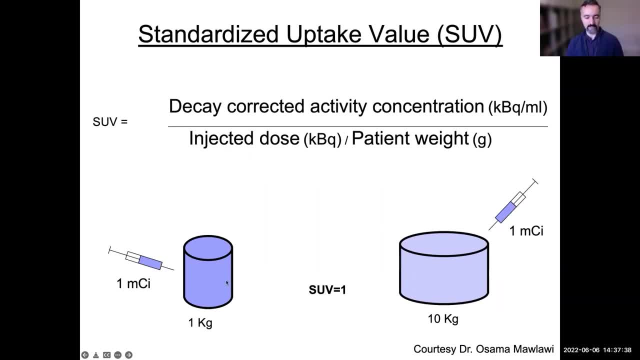 you know whether you're injecting one milli here into this or one milli here into this. sure, this is going to give you more concentration because this is smaller. but once you normalize by the injected dose and the patient, let's say weight or size or volume, it's going to normalize out. 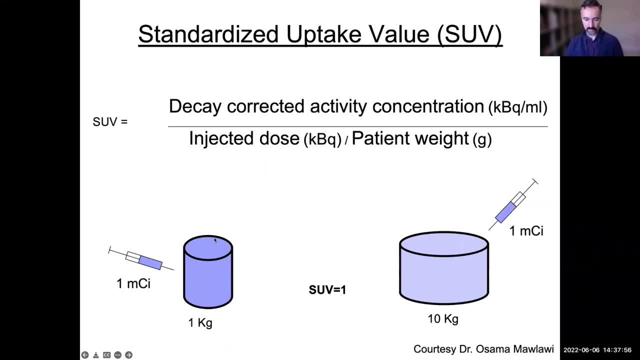 and you're going to get an suv of one in both of these images, even though this is more concentrated because you're normalizing by this- you're going to get an suv of one. suv of one means like average of background uptake if, if you, for example- uh, here make the volume smaller and make the 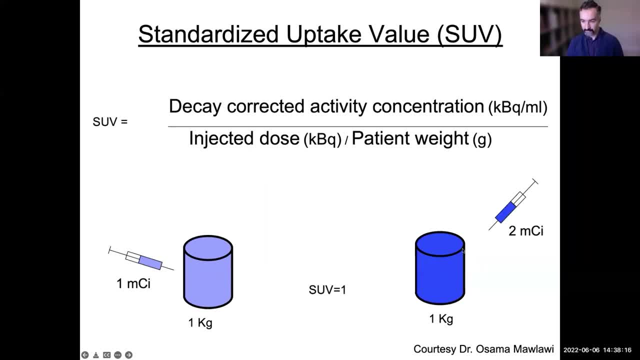 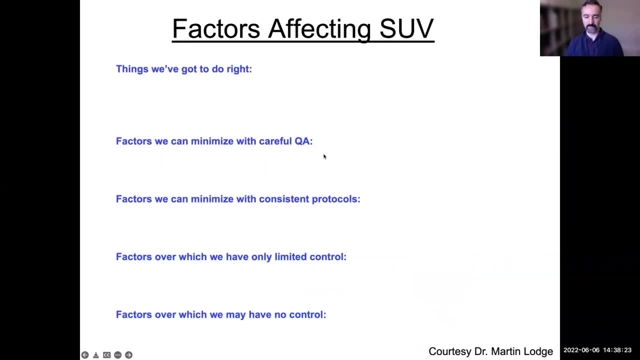 injected rate even higher again. this is going to be very dense, very concentrated, but again, suv is still going to be one because this is going to normalize at the bottom, because you're going to divide it by a higher number. so there are a number of factors that affect suv. are things we've got to do right? 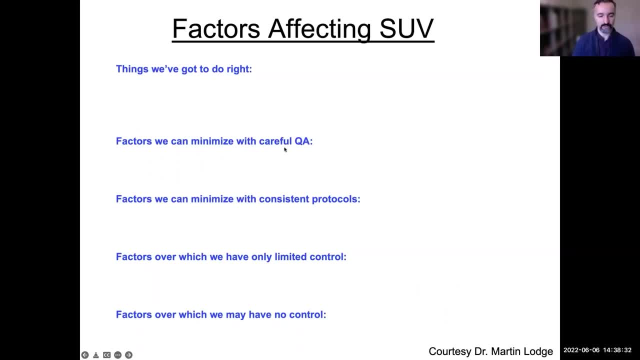 certain things that we can minimize with careful quality assurance or with consistent protocols, some over which we have some limited control, some over which we have no control. so things like clock synchronization. we've got to know what is the exact time between when i measure my radioactivity and when i measure my radioactivity. and when i measure my radioactivity. 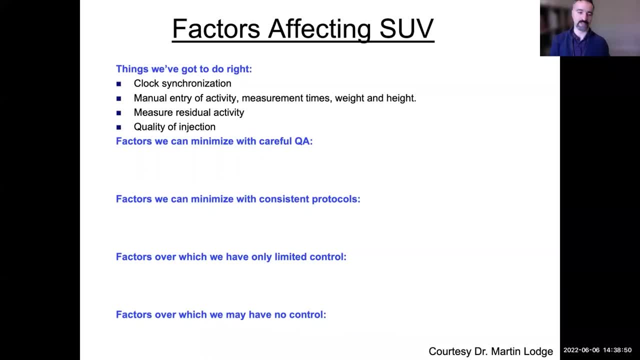 and when i inject it into the patient, something like that. right, you got to enter the correct weight and height of the patients. you gotta, you gotta. quality of the injection has to be good. you gotta make sure the entire injection enters uh, uh, enters the bloodstream, etc. etc. okay, so um. 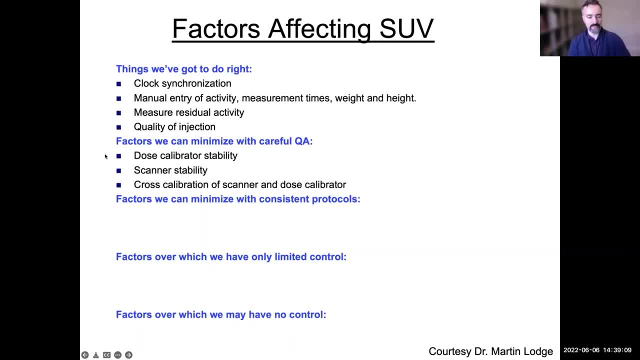 certain things we can minimize, like proper stability of the dose measure calibrator to measure the injected dose, the scanner itself being stable, doing good qc, qa, which we sort of talked about last time. um, things we can minimize with consistent protocols like patient preparation: right if a patient is not fasting, that might really complicate things. 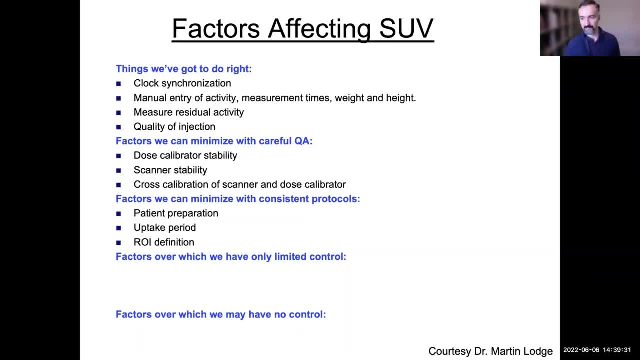 because the body might show certain metabolisms. that's because the patient is not fasting, not because there's elevated um activity due to disease. uh, definition of the regions of interest, consistent definitions, something to have some control over patients, patient motion, um playing and using consistent protocols and parameters can make a difference. 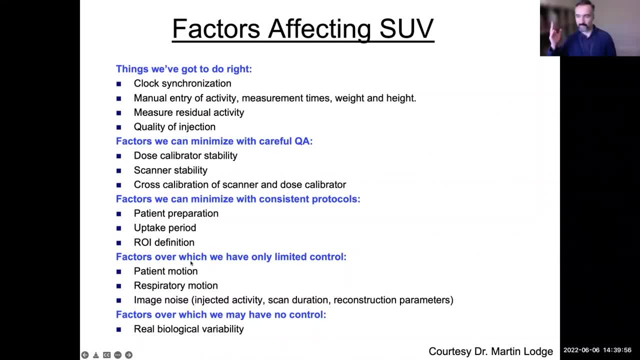 on the image, noise, and there are certain things we just cannot control. even if you have the same patient, everything else being perfect, but it's the same human showing up today versus tomorrow, there may be biological variability and there's just nothing you can really do about that, even after. 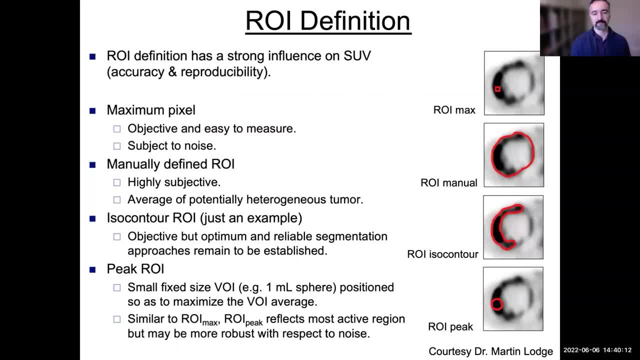 controlling fat, proper fasting, everything. so how you define the roi matters. are you going to measure the maximum amount of roi? you're going to measure the maximum amount of roi? you're going to measure the maximum pixel maximum uptake? how are you going to draw the regions of interest, or are you going 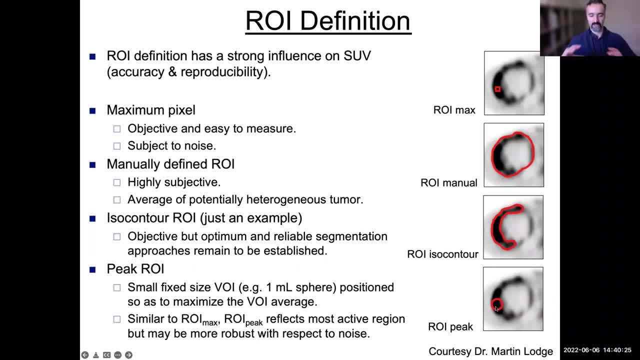 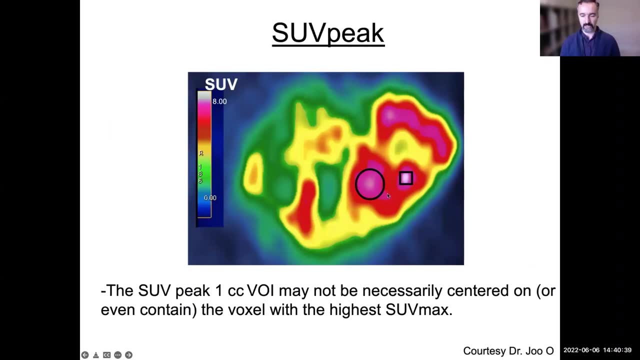 to take this thing called roi peak, where you make a sphere that's one cc, move it around the tumor to see where you get maximum uptake. different ways to calculate suv, for example, suv max- yeah, it's the hottest pixel of voxel. but if you do suv peak, where you take a 1cc volume, move it around until. 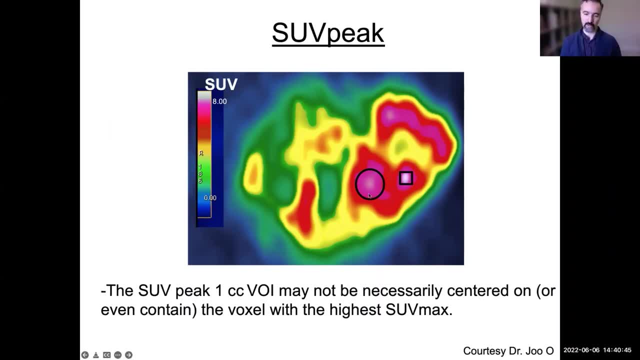 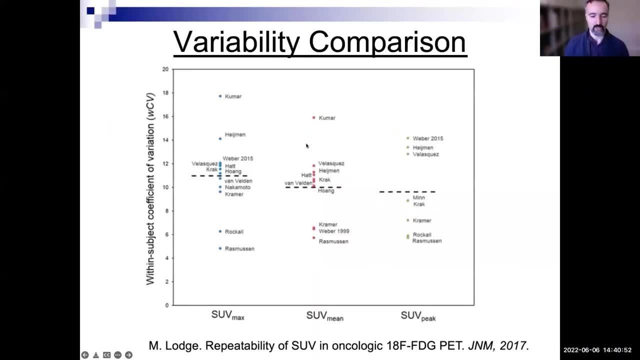 it's maximized, um, it may show another part of the tumor. it may get maximized and it may show the size of the tumor. it may give you different values and there's some variability associated with with how safe is it so if um? so, uh, same subject being scanned today versus tomorrow- some kind of a test? 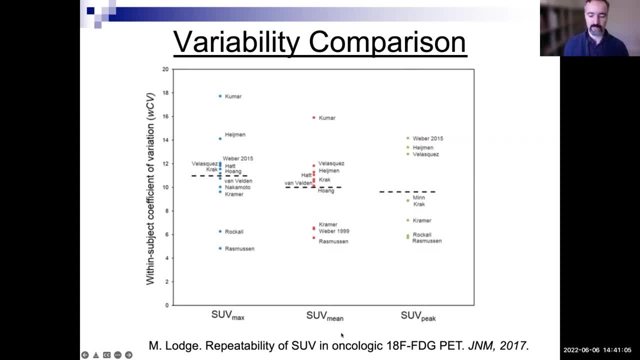 free test. there's variability in the measurements: suv max, whether you calculate suv peak or average tumor uptake, there's variability in there. it's not going to be perfect. there's day-to-day variability: noise due to the scanner. everything else, part of it is due to biological variability. 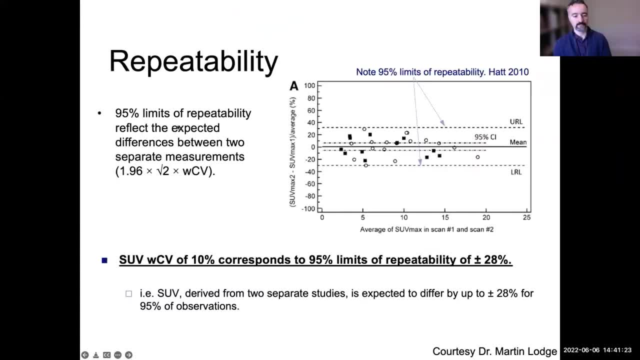 um, you do some math, etc, etc. you can show and prove, given the studies that have been out there. look at this number: 20, almost 30. the 95 limits have. repeatability is almost 30. what does that mean? it means that if i image you today and you come back tomorrow and i image you again, test. 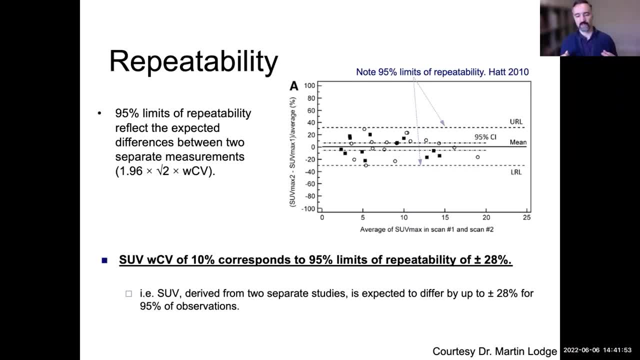 retest, there's a 95 confidence interval that these two are within 30 of each other. so if if the change is more than 30, is highly likely that this is not due to biological and noise variability. this is due to real change in the patient, which means that treatment, for example, 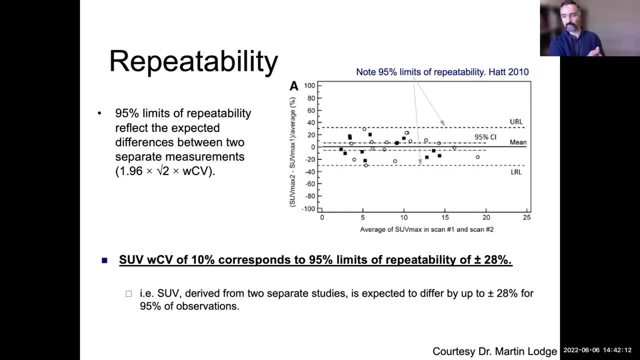 is working or not working. if you scan me today before you and sometime after treatment and that changes more than 30, that's very likely it's a real change. it's not due to biological day-to-day variations in the patient. it's a real, real change. 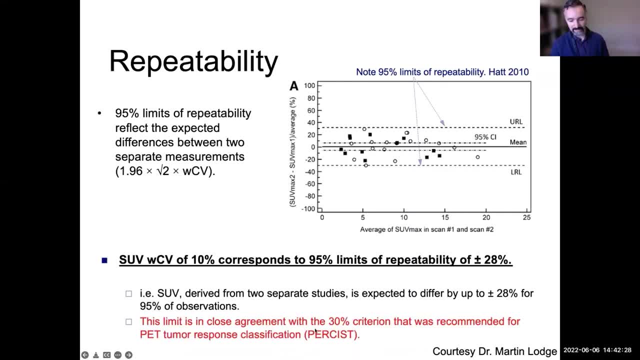 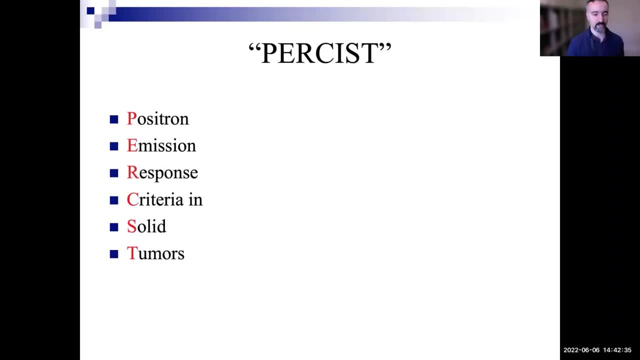 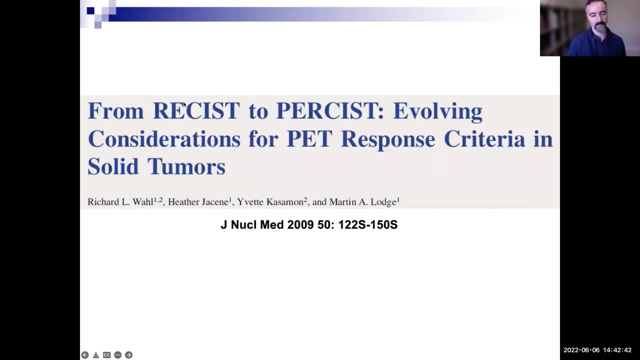 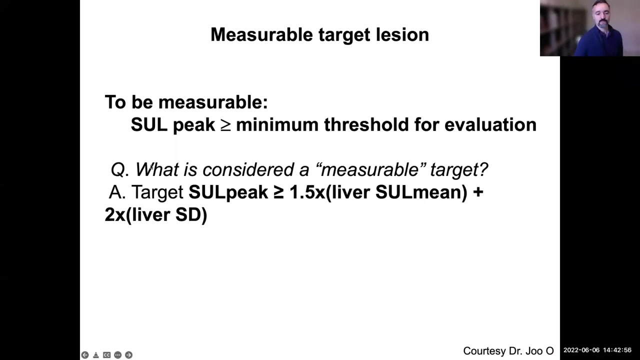 so, so, so in fact the persist criteria use this number 30. so they say: if the change is, so, stop what. persist stands for positron emission response criteria and solid tumors. my colleagues at hopkins, when i was there, did this amazing work and, uh, the that mean plus some kind of variability in it. 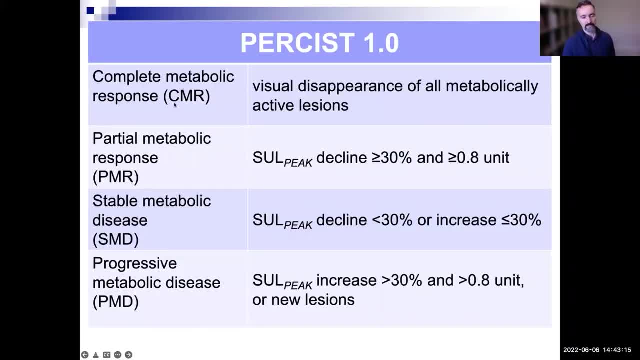 and then there's four criteria: complete metabolic response in therapy, partial response, stable disease and progressive disease. and you see this number, 30 percent, keeps showing up. so, for example, if you decline by more than 30 percent, or, right meaning, if you uh, uh, yeah, or or if the other way, 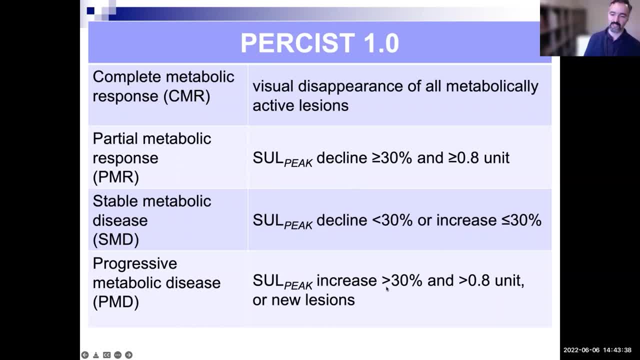 around if that's actually starts to increase by more than 30 percent. so there is this number. that's arrived at by some mathematics and some statistical considerations. if it's more than 30 percent change, it's very likely it's a real change. there's other techniques beyond suv. there's 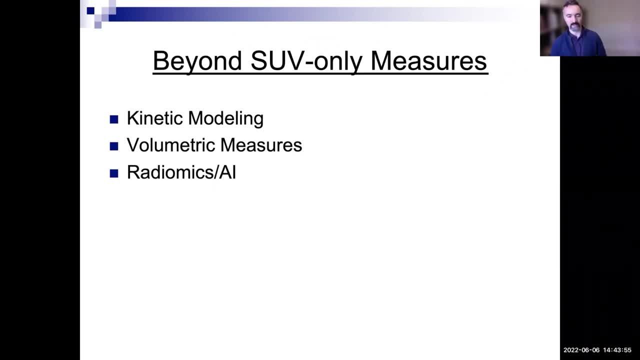 field of kinetic modeling which really tries to look at more, better quantitation of physical phenomena like the, for example, uh rate of metabolism. suv is not the rate of metabolism. suv almost semi-quantitative. it's a measure of how much you're going to be able to do in the future. so it's a measure of how much you're going to be able to. 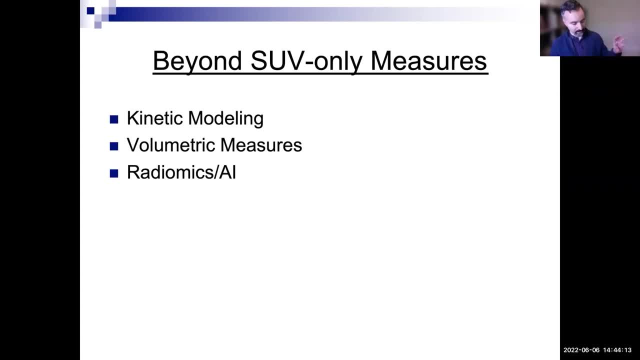 it's a measure of how much you're going to be able to do in the future. so it's a measure of how much radioactivity, in a sense, is here. but, um, how can we quantify the rate of metabolism? there are techniques to do that, but often they require dynamic imaging. there's a lot of interest and 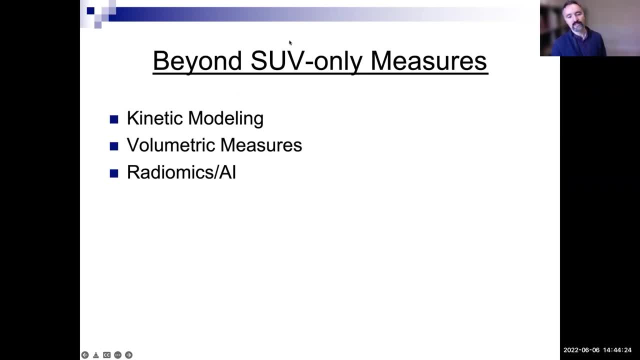 activity in this area, moving beyond just measuring intensity, because suv is a matter of intensity, but looking at volume of tumors, there's study after study showing that the volume of the tumor for certain cancers can be even more telling than the intensity of the tumor right. so that's important. 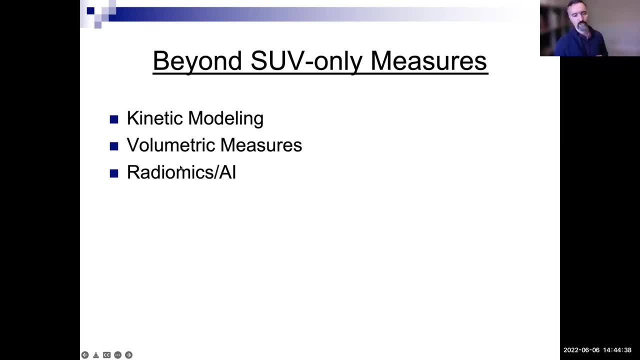 and also doing uh ai, artificial intelligence and radiomics, where you don't just look at, and also doing uh ai, artificial intelligence and radiomics, where you don't just look at uptake or volume, look at texture heterogeneity, which might indicate things like hypoxia, proliferation, you know, etc. etc. so there's a lot of area. there's a lot of interest in this. 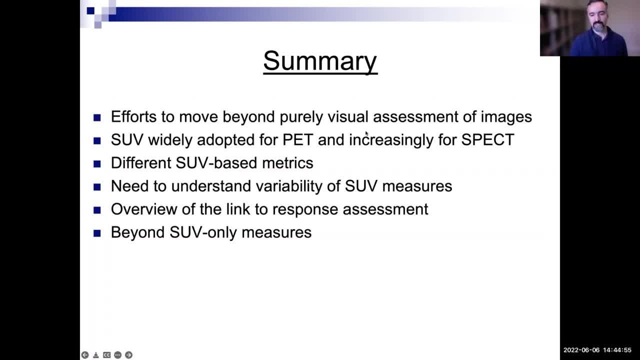 area. so, in summary, efforts to move beyond purely visual assessments that are happening. uh, suv has been widely adopted for pet and increasingly for respect for different kinds of suv measures. suv max average is to be peak suv. we need to understand variability of suv and how to link it to response assessment and look at other metrics beyond suv only. 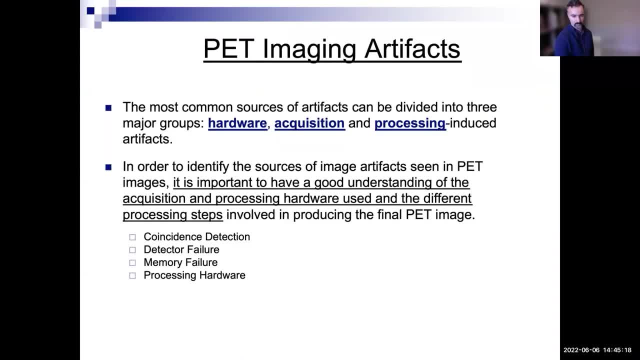 intensity only measures. so there are some artifacts in the world of pet that we have to be aware of. there's three. their sources could be coming from the hardware, the acquisition and the processing. it's important to have a good understanding of the acquisition, processing hardware used and the different processing steps involved. so, for example, there is something arising from the 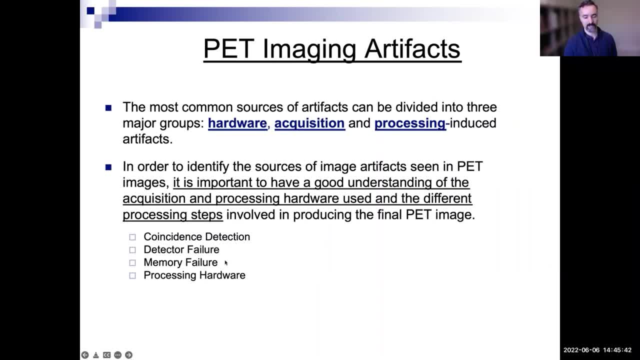 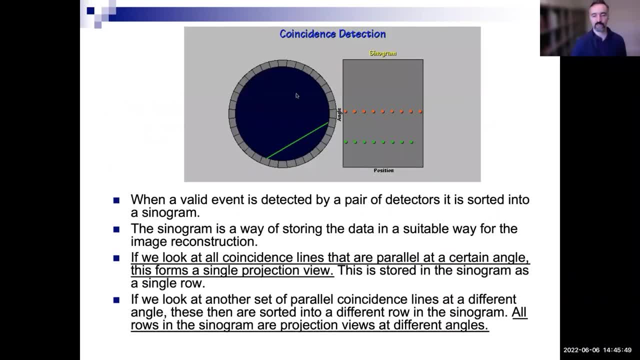 detection being faulty or the detector specifically failing, or the memory failing or some kind of a processing hardware failing right. So here's a coincidence: detection: You've got a ring around the patient. Remember, in PET we've got a stationary system. 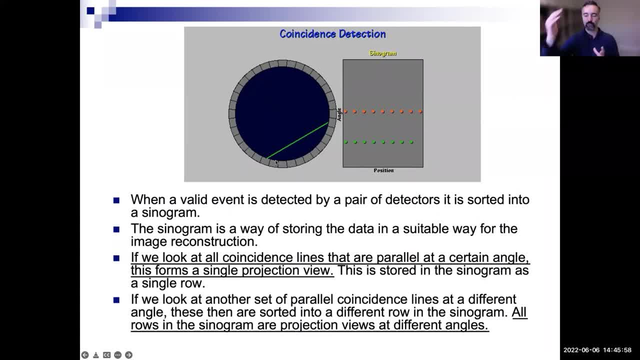 Because, again, the beauty is, you could collect from all angles, You don't have to rotate something around the patient with collimators, The stable system, And when an event is detected like a pair of events, this is a line of response. 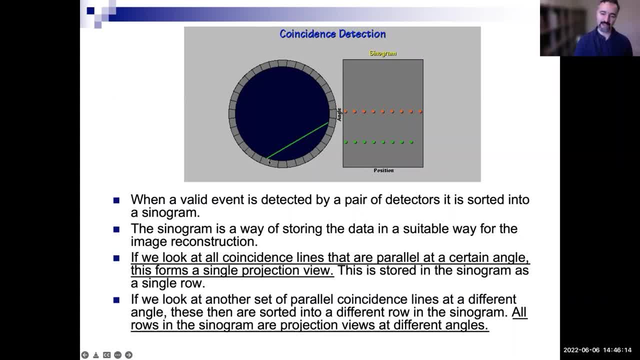 You could use a so-called sinogram. In a sinogram you say: what is the angle of this event? Let's say: the angle is this number here, Whatever that number is, let's say 30 degrees or whatever- And as you move up and down, 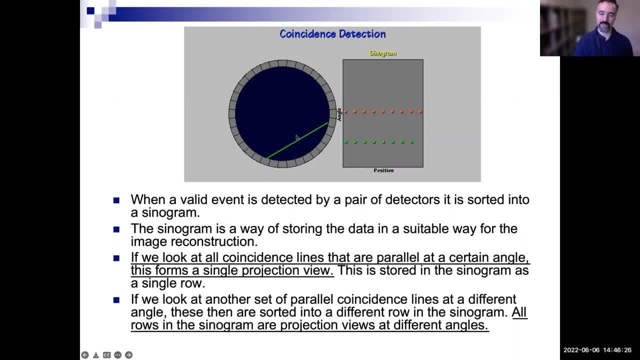 the position of this changes with respect to the center, like a particular distance. So this line would be here, but then more lines. If I change in this direction, it would be here, So. so this is like. this is what we get. 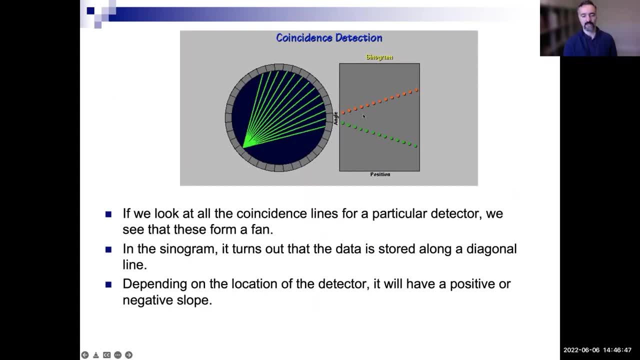 And then if you think of just one detector, how it pairs and combines with all of these, turns out in the sinogram domain. if you plot it, you're gonna get this line, Because both the angle keeps changing. These are different angles. 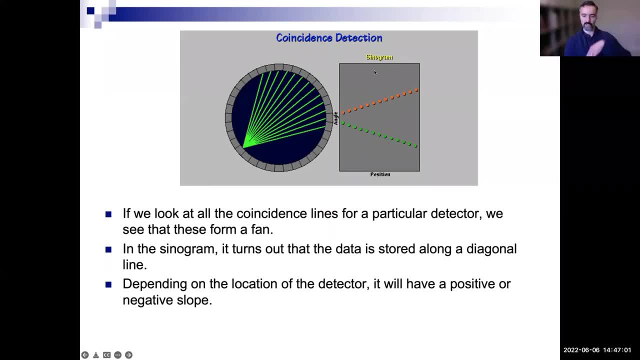 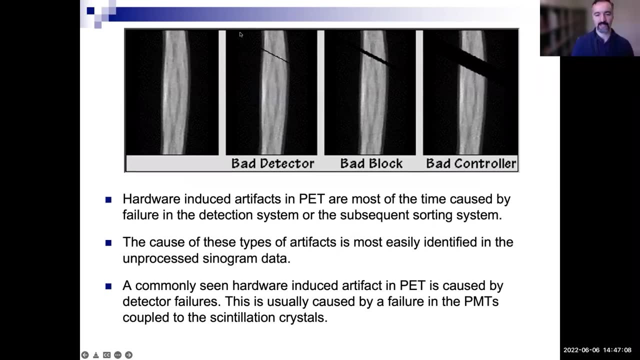 And the distance from the center keeps changing. But you get a line in the so-called sinogram domain. So if you suddenly see in your sinogram data, in your projection data, in your data measure data, a line like that, it probably means there's a bad detector. 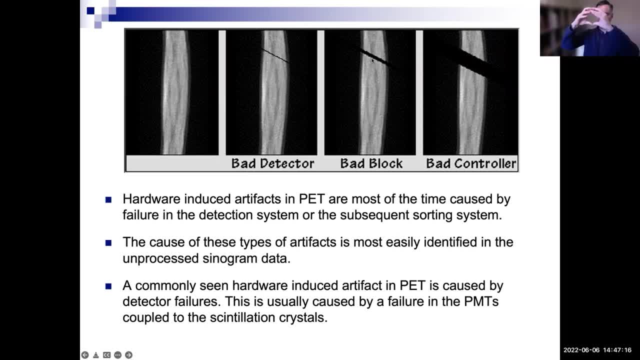 If it's thicker, it might mean that it's not just a detector but the entire block containing, let's say, an eight by eight set of detectors. that's out. Or if it's even wide, there might be the whole controller controlling multiple blocks. that is out. 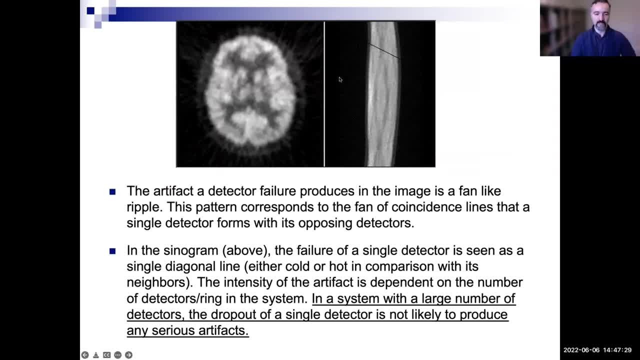 So those are some of the things you can identify, And if you have a few of these, sometimes a single one of these doesn't really show up in the image, but then, as more add, you see: oh, oh, oh, oh oh. 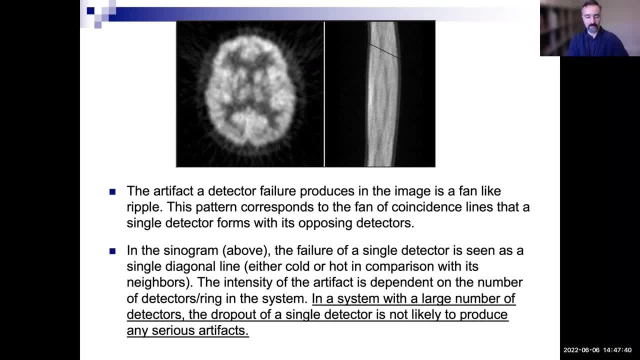 And if you have more add, you sort of get ripples. So this is a diagonal line here. And if you have a lot of detectors with dropping, so in a system with a large number of detectors, drop out of a single detector is not gonna show up really. 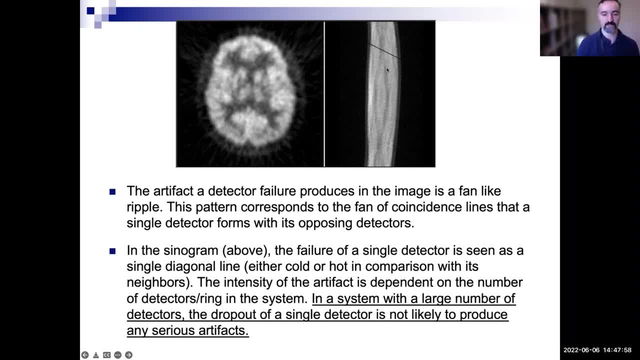 But if you have multiple detectors missing a whole block, you're gonna start seeing it. But- and there are ways to deal with this. So there are ways to say: okay, I lost some data. Well, obviously I gotta fix my scanner. 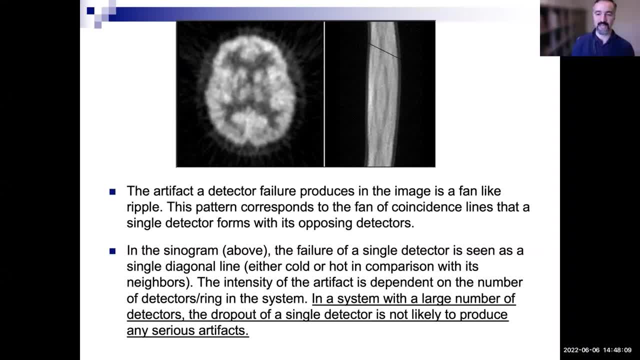 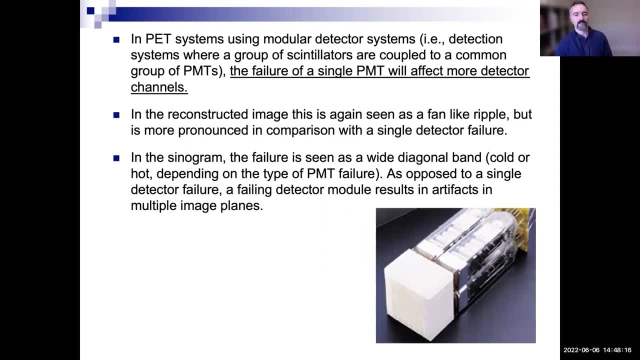 but also maybe I can go and fix it. I can go back and process my data somehow to fill in these gaps or to ignore those gaps. Ignore them intelligent, not neglectfully. And if a PMT fails, multiple detector channels are messed up. 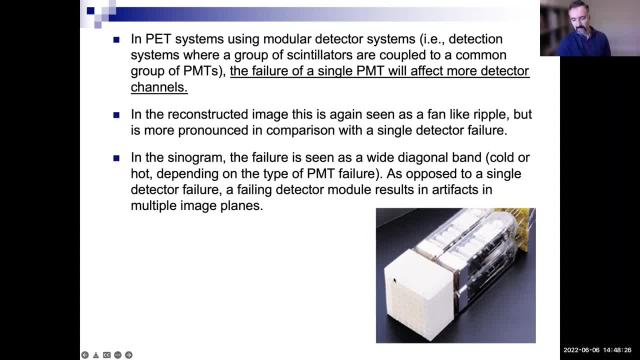 because remember a PMT. so here's a four- sorry- eight by eight block, a block of eight by eight crystals with four PMTs. If one of these PMTs fails, it's servicing a whole bunch of detectors. it's servicing a whole bunch of detectors. 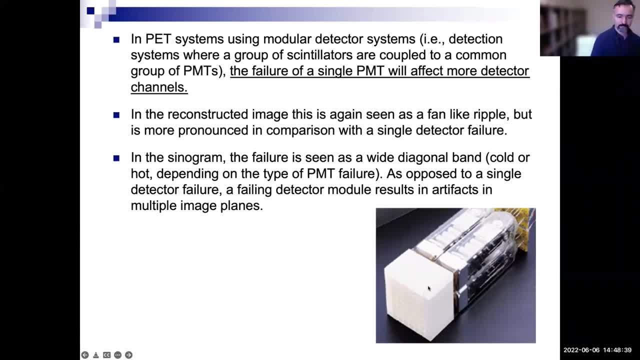 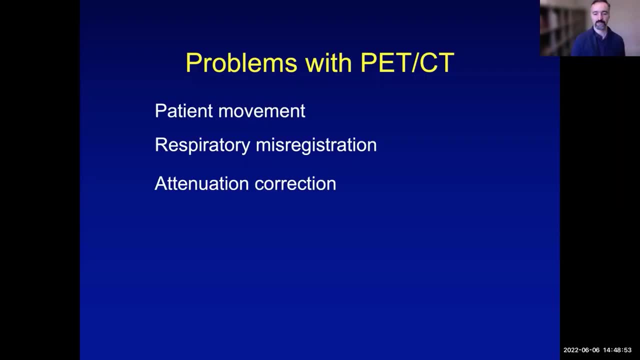 it's servicing a whole bunch of detectors. that's gonna confuse things, okay. So again you could say fan-like ripples, but it's gonna be more pronounced than a single detector failure And you get a wider diagonal band if a PMT fails. 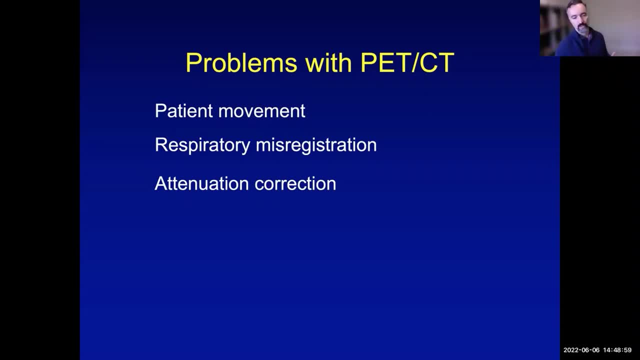 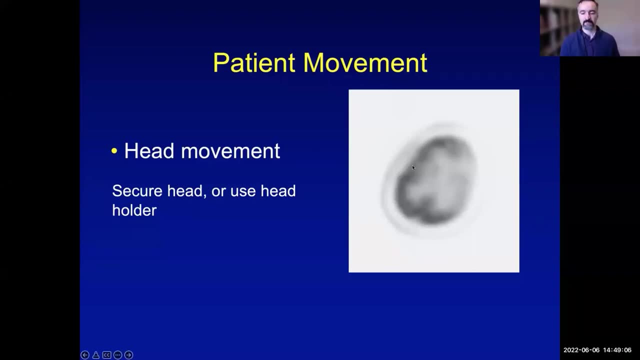 There's other issues that can appear in images: patient moves. there is misregistration between PET and CT that messes up the attenuation. So here's an example where the patient has moved And when you're doing attenuation correction, let's say you're using the CT. 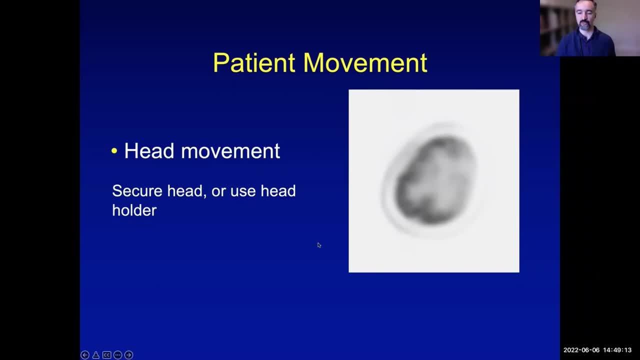 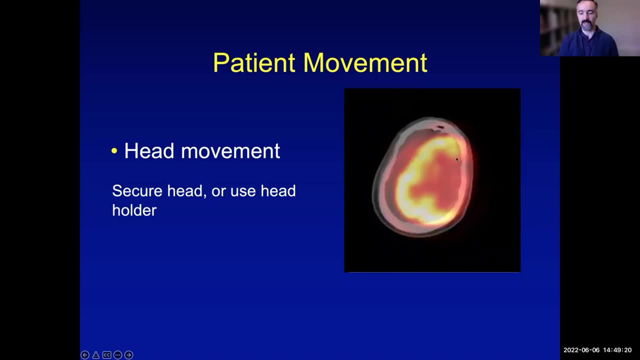 but then you're doing your PET reconstruction, they're misaligned so the corrections you're doing might be totally off. So when you then plug the CT on top of the PET you say, wow, what a big misregistration that contributed to the attenuation correction. 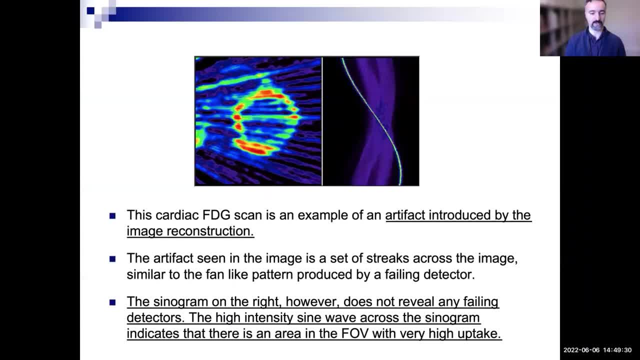 So you have to go back, align them better and then do the reconstruction. Sometimes you may get some artifacts like this and you may look at this. you're like, oh, oh, oh, oh, you would be like water on earth. is this um right? so you set up streaks um and then you inspect it. 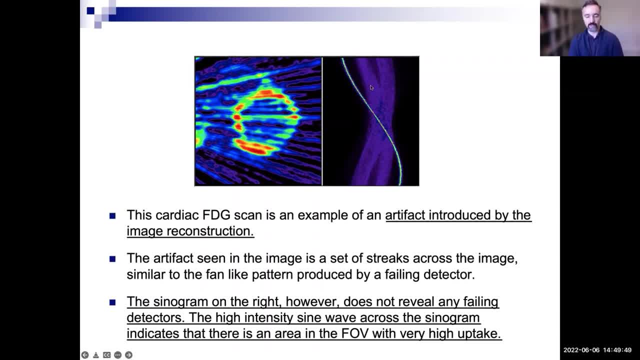 and nothing seems to have to have failed. but then you look at the image domain. you see this high intensity sine waves across the cypress. sine around it shows that there is an area in the field of view. this means that there is a point in the field of view that is going to be very 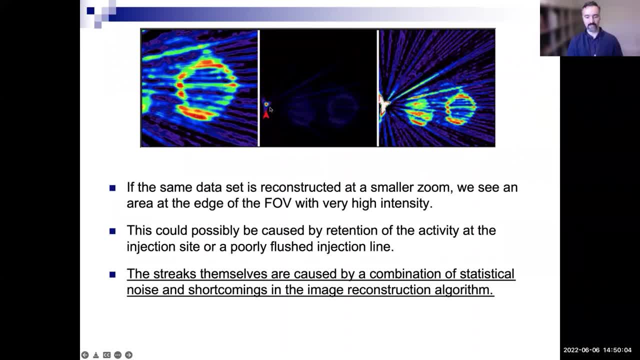 high uptake and guess what, when you zoom out of this image and you go out there, there is a point right here. okay, so this could have been the retention of activity at the site of injection. poorly flushed injection line. okay, um, and so how do you deal? okay, so we just identified. how do we? 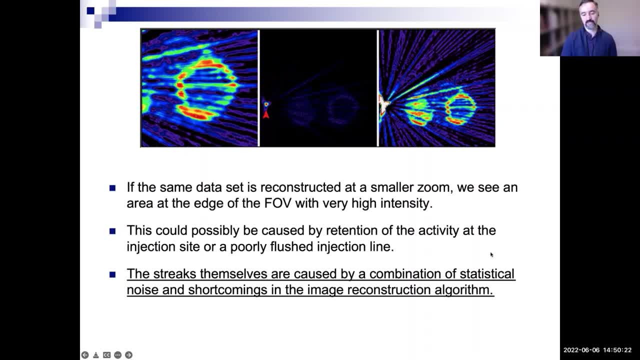 actually is: how do we deal with this? well, if you use techniques that sort of models noise, statistical noise- better, um, you might be able to tackle it, because some reconstruction algorithms, if you have very high uptake somewhere, um they they may get messed up, but increasingly image reconstruction algorithms are able to handle. 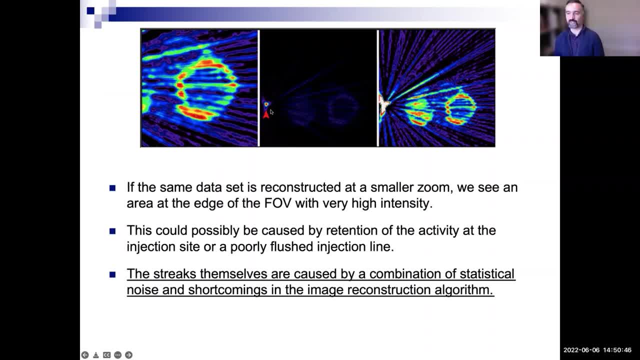 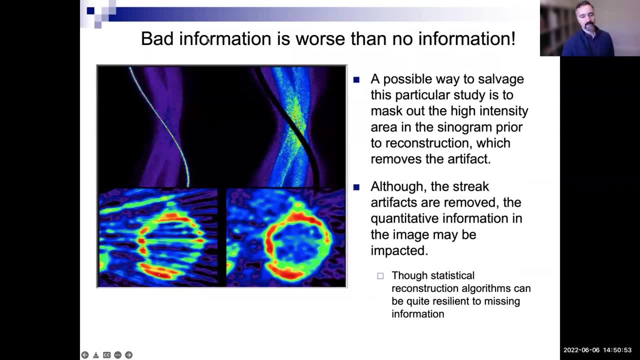 this kind of an issue because, at the end of the day, it's not really an artifact. it's just that there's super high radioactivity here and a reconstruction is supposed to deal with that, and bad information is worse than no information, and so so when you have this very issue here, 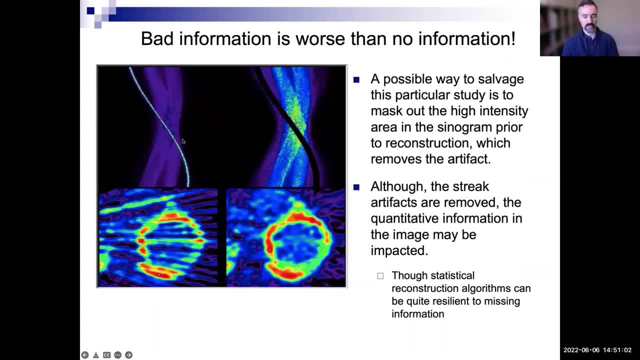 that we talked about. well, sure, you could do reconstruction. there are again some reconstructions that might be able to handle this, but some won't. and if you cannot handle it well, then at least you can block it out. so you could put, put something here, block it. 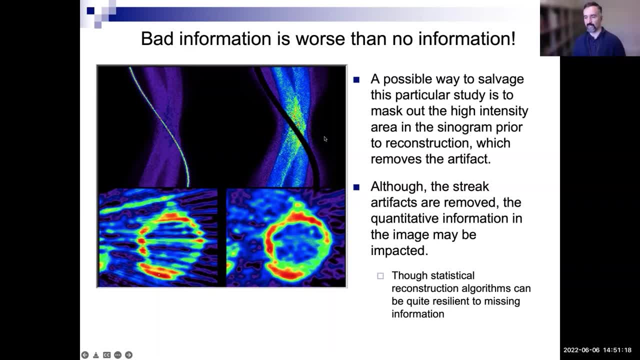 out and in a way assume as though that's there's a gap in the scanner, as though you have no data acquired there, not that nothing was measured, no, you modeled the reconstruction, saying there's a gap in my scanner here. i'm not going to model that space, you know. so you sort of remove that. 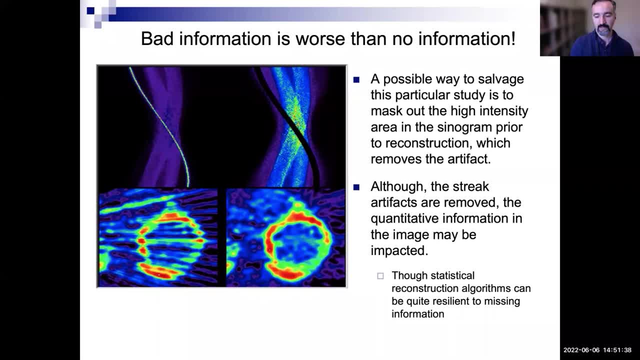 data, um, something like that i mean. essentially, what you're really saying is that any detector, any lines of response passing through that super high area. i'm going to assume i have gaps in my scanner. this is not to be taken as a rule of thumb. these are just examples of how we would play with. 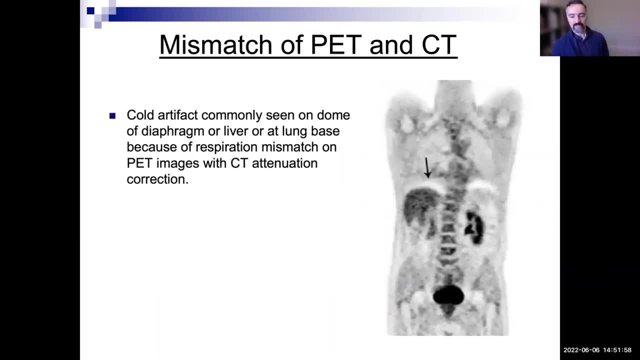 data and to fix issues if there is breathing mismatch. remember we showed the brain. now there's a breathing mismatch. uh, for example, if there's a breathing mismatch, there's a breathing mismatch there. there's a breathing Braud. Цologia there works in out cœc. 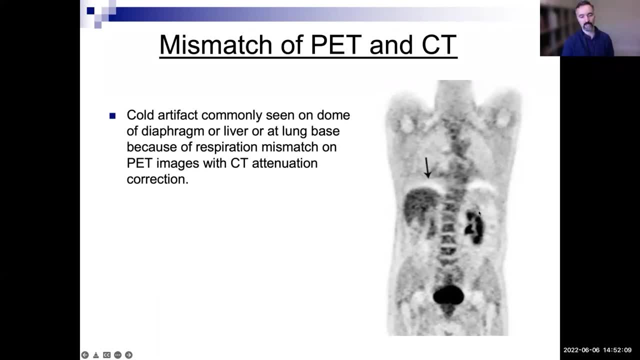 you have to look at that here you would see about a lot of little bits. you wouldn't see those too many here. next thing can i say is that when you look at the right side, that was another movement. here's another movement, for example, on the dome of the diaphragm or 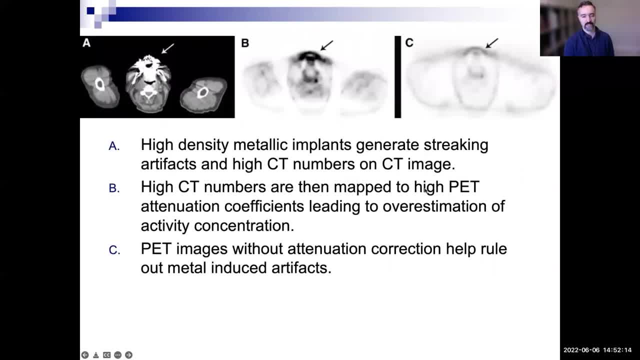 with that at around the lung base. you'll probably be able to see them, for example, at the dome of the diaphragm or liver. you would be able to see them, be able to see that. you see that some respiration mismatches and so lever, or at the lung face and so sometime this is because of breathing right. so the ct was. 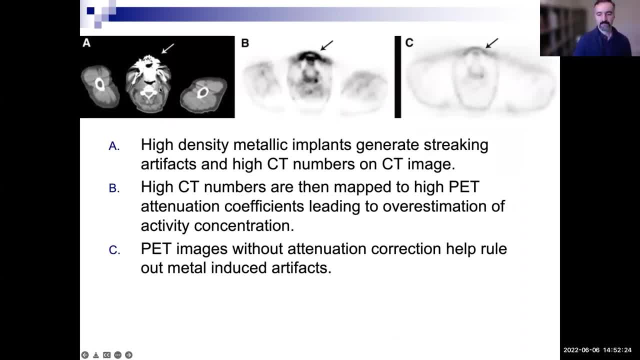 because of breathing right. so the ct was at a different phase than the PET. for example, uh high density metallic implants can generate streaking artifacts on ct and i mean you're doing intensity for pet simply because it thought there's so much attenuation here that i'm going 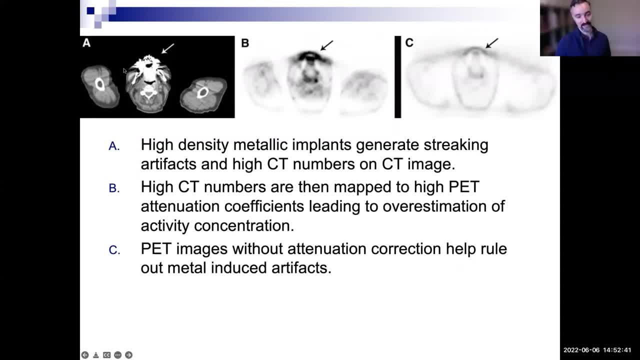 to have to over compensate for it, whereas this was really not an issue at all for the pet world. it's just that it's a metallic artifact that really messes up the ct image, but it's actually okay. the pet image would have handled it fine if this ct was not suggesting super high numbers. 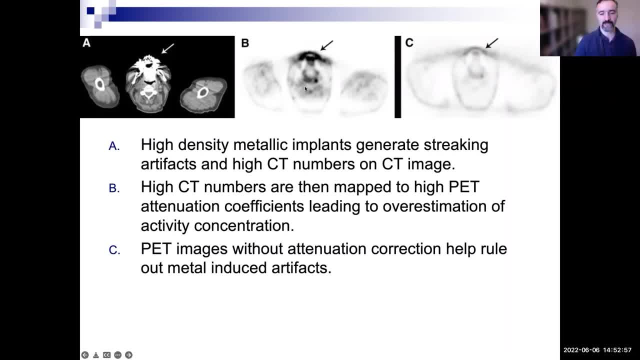 um, and so sometimes if you do, if you don't turn off attenuation correction, you see that might go away and you're like, oh, that's the problem. now how do you actually deal with metallic artifacts? on ct, that's a whole different debate, but there's- or different uh topic, but you know typically these: 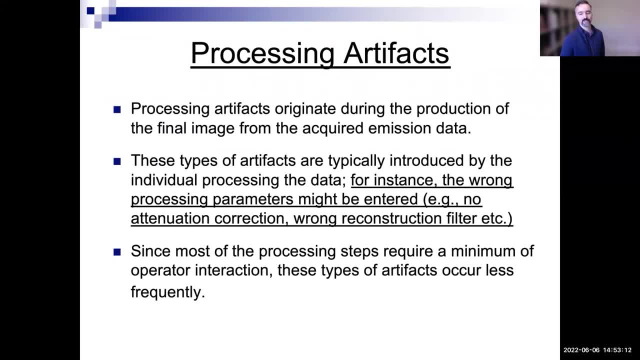 have been dealt with pretty well. processing artifacts- um. you might have just entered the wrong processing parameters. you might have told it it's it's f18, whereas it was c11. i might have told it. oh, you might have forgotten to turn attenuation correction on, um. you might have. 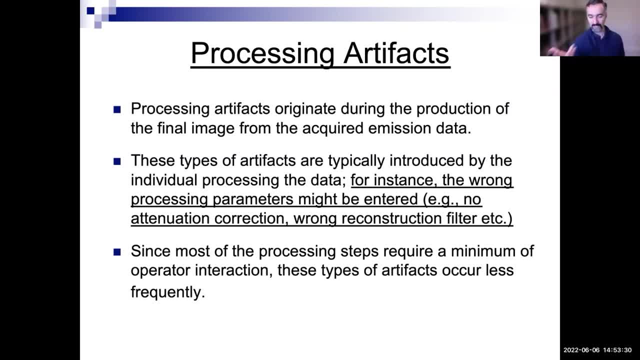 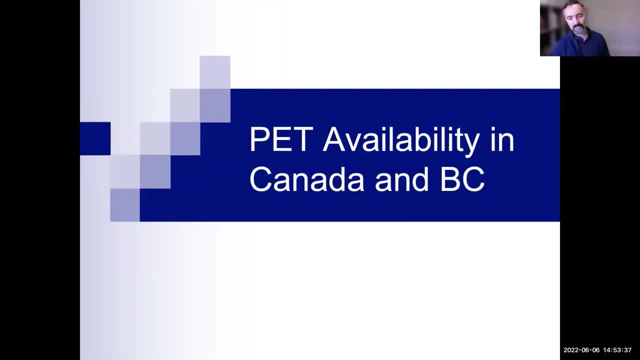 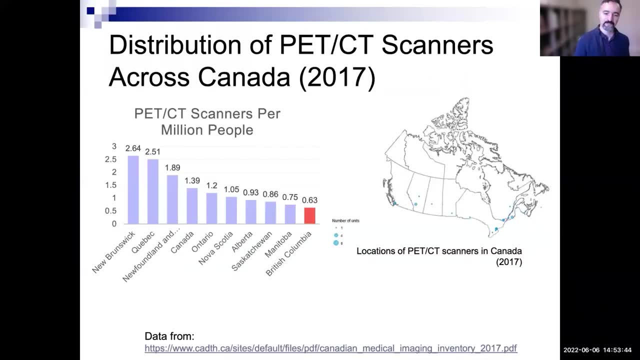 used the wrong reconstruction filter, so you're going to get the wrong image simply because you, as an operator, entered in the wrong number. so all these things can be- uh, hopefully tackled better. i just want to share a few slides about a sense of urgency that we need to have more pet scanners in canada and in our province. this is a plot from 2017. 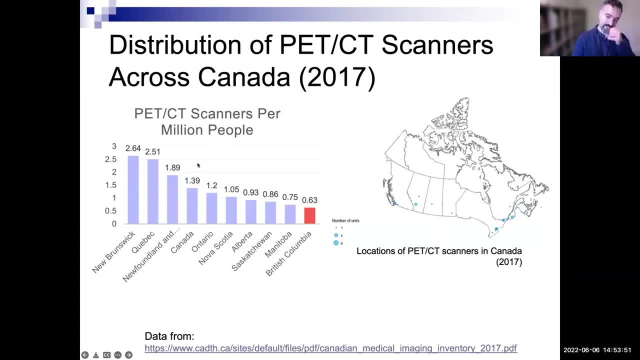 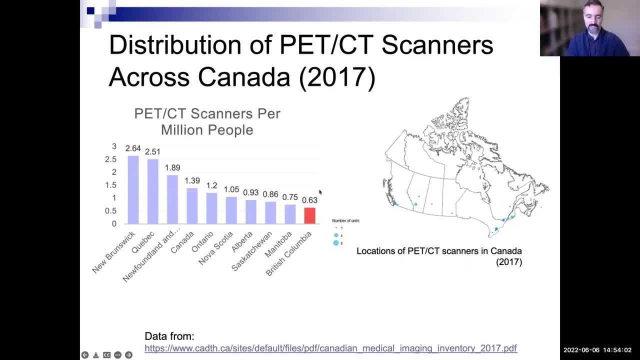 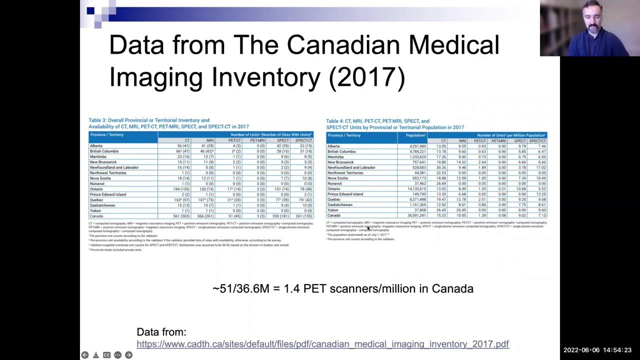 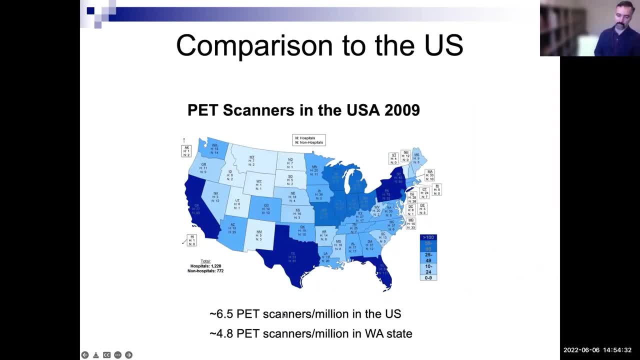 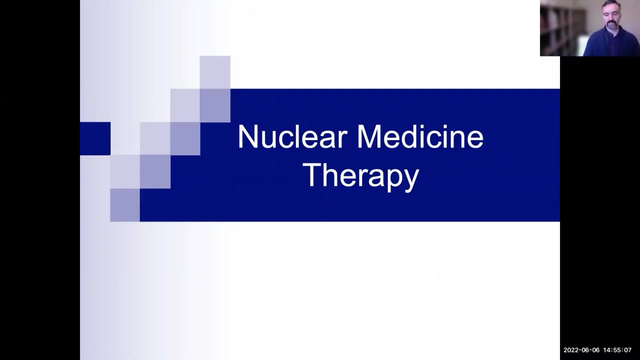 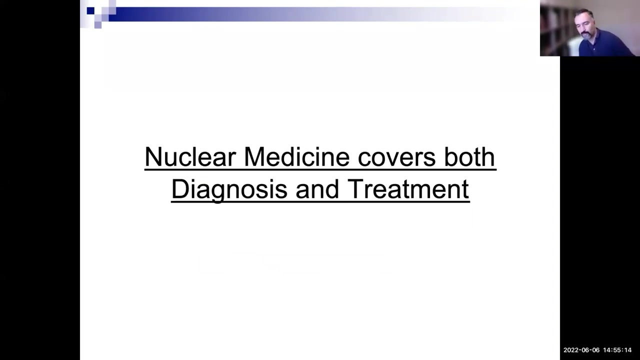 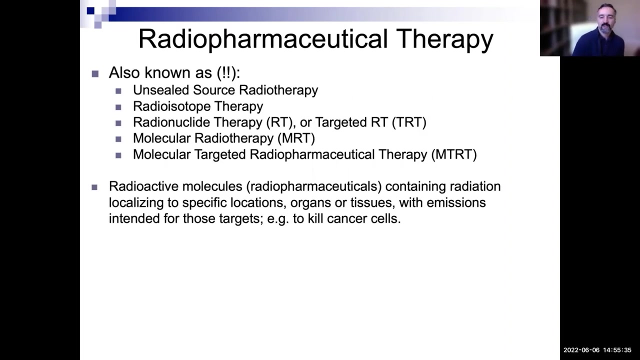 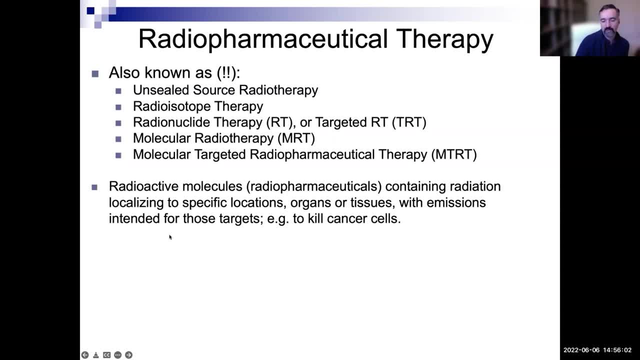 localizes to a location, sits there, emits particles to kill its target, But a tumor, for example, expressing creating a certain protein. if you have a molecule that targets that protein and it is tagged by and labeled by a radioisotope. 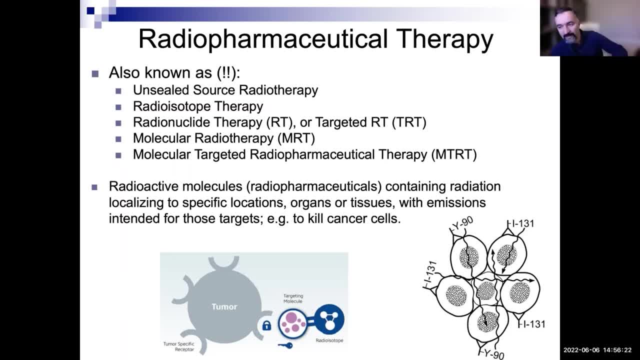 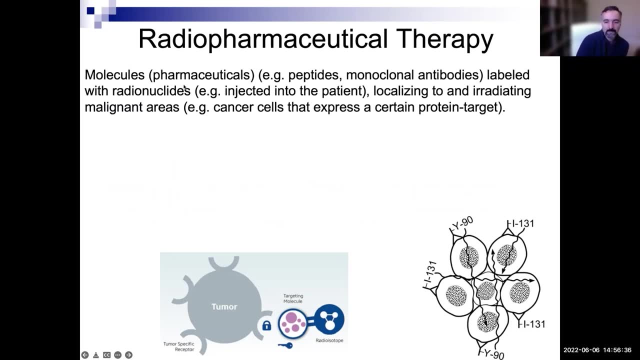 that emits particles. So emitting gamma rays is for imaging. emitting particles is for therapy. If it emits particles like electrons, for example, it can kill tumors, for example. So molecules, radiopharmaceuticals that are labeled with radionuclides. 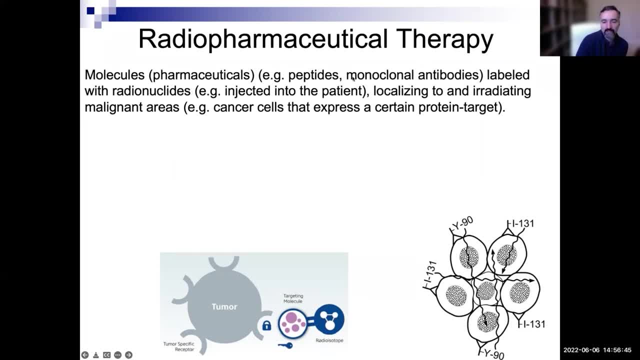 So people have antibodies, these larger molecules, but increasingly people are also excited about small molecules, peptides, and then you would radiolabel them with radionuclides. Again, they localize and they irradiate the malignant area. So some special examples of radiopharmaceutical therapy. 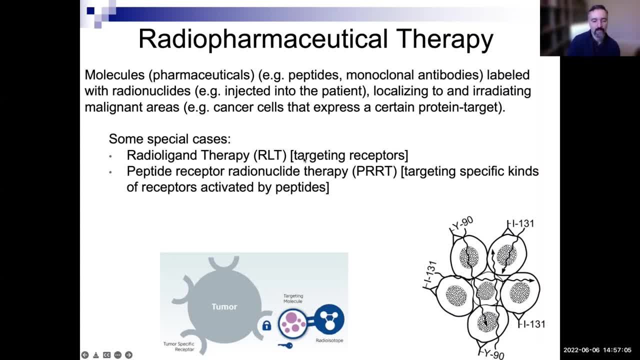 radioligand therapy is when you're targeting receptors as your target, So-called peptide receptor radionuclide therapy, targeting specific kinds of receptors activated by peptides, and radioimmunotherapy when using antibodies- monoclonal antibodies, Okay- Whereas here, typically, we're looking at peptides. 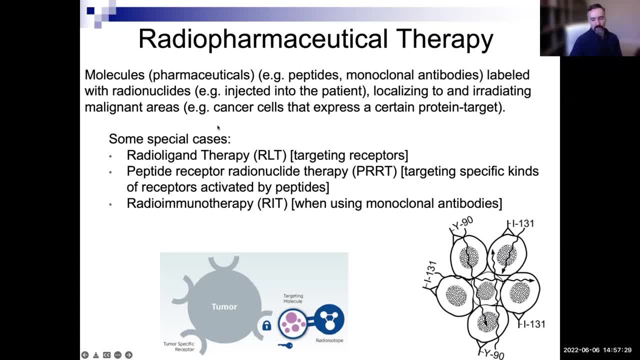 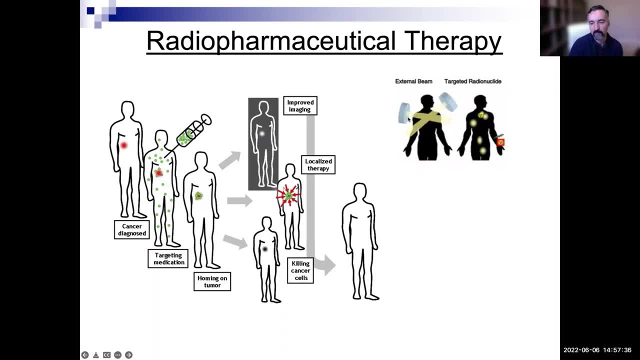 for example. So you know, external beam radiotherapy is the paradigm you're all very familiar with, but the molecular radiotherapy is different. You're injecting into the patient. it is going the body, is distributing it to targets throughout the body. 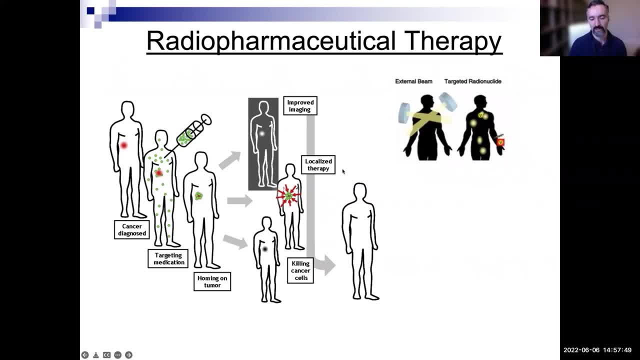 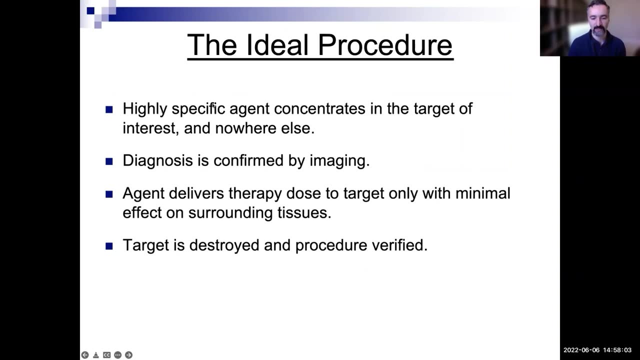 that are expressing a certain protein, a certain target, a certain receptor, and it sits there for tens of hours, for days, and bombarding it with particles. So the ideal procedure for radiopharmaceutical therapy is when you have highly specific agents. 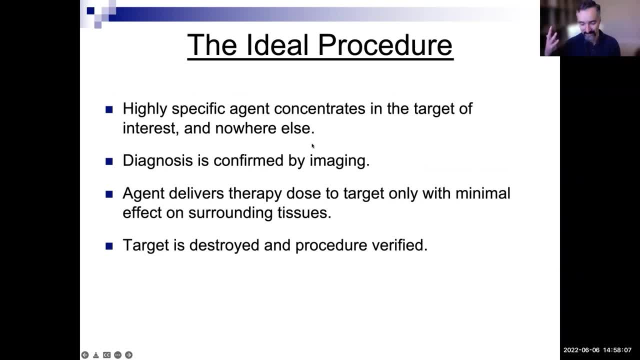 that concentrate in the target and nowhere else. no organs at risk. that's the ideal scenario. That's never the case. Diagnosis is confirmed by some kind of imaging, So you're not just treating, but you're seeing what you're treating. 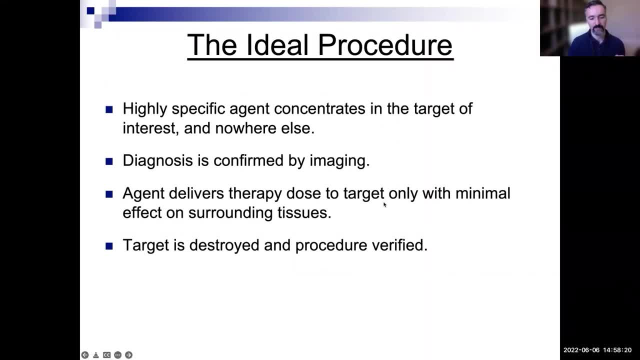 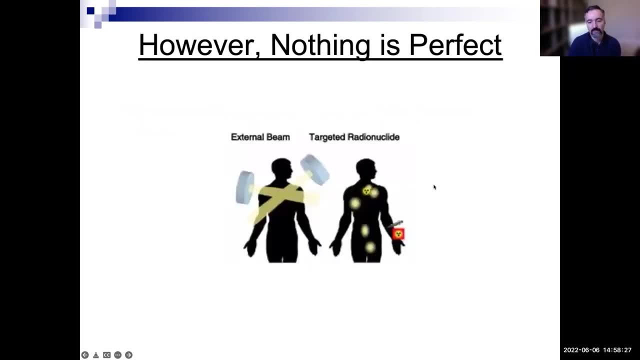 That's theranostics. we can do that, we'll get there. Agent delivers therapy dose to target only with minimal effect on surrounding tissues and target is destroyed and procedure verified. So again, we're looking at radionuclide, radiopharmaceutical therapy. 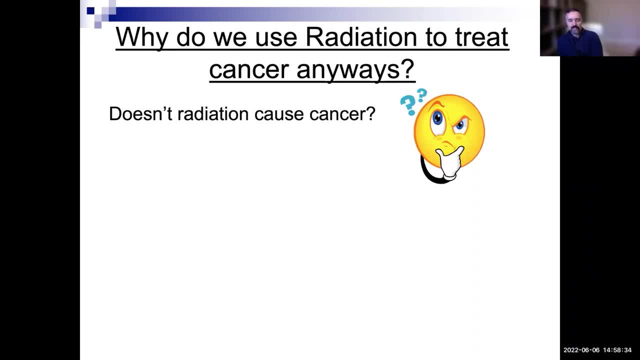 The question is: why do we even use radiation to treat cancer? Doesn't radiation cause cancer? Of course you're gonna have lectures on radiation, biophysics et cetera, and you're gonna learn about all these things. There's really two types of damage. 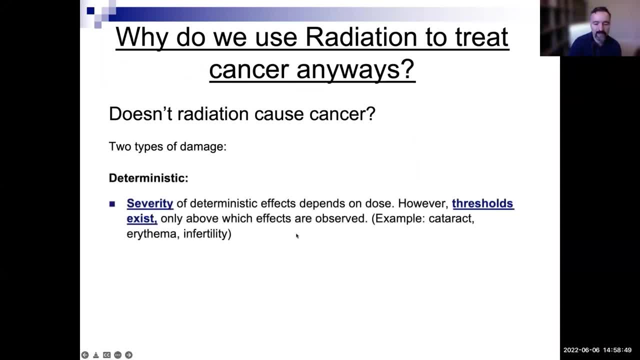 There's deterministic damage where severity of the effects depends on the dose and there are thresholds. So above a certain threshold it is deterministic that you're going to get increasing severity due to the dose of cataracts et cetera. But stochastic is when there's a probability, not severity. 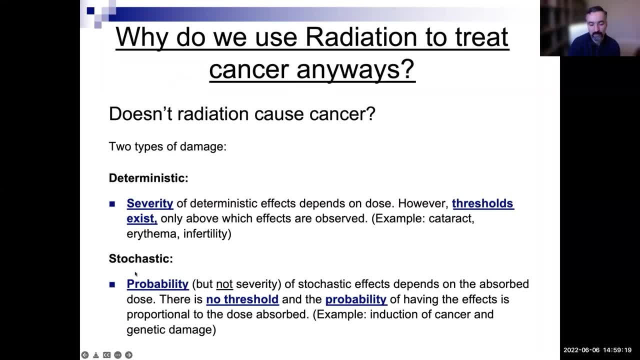 More doesn't mean worse, but more means more likely than you. for example, you're gonna get cancer. So the probability of the effect is more likely than less. probability of these effects depends on the absorbed dose, So the higher the absorbed dose. 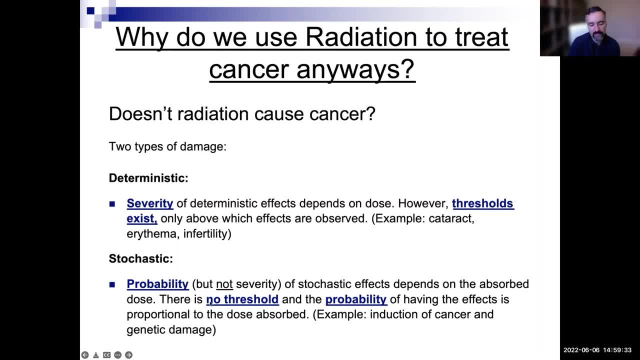 the more likely that you're going to develop, for example, cancer. There's no threshold, it seems. I mean there's a bit of a debate about this, right, You know, is there a threshold, But no known threshold, I should say, And the probability of having the effect is proportional to the dose. 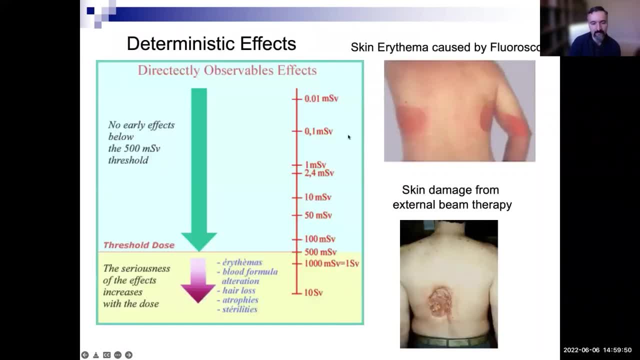 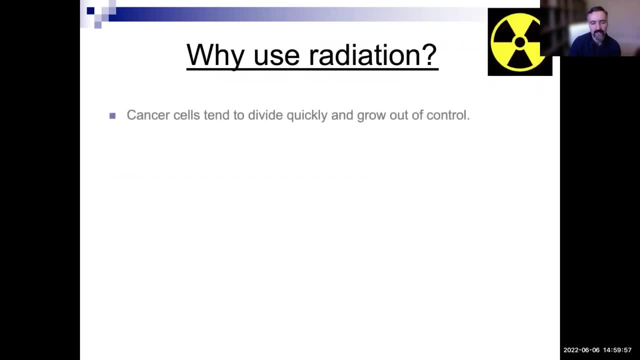 absorbed, So induction of cancer. So again, you have deterministic effects And this lecture is not to deal with these. So why are we using radiation? Cancer cells tend to divide quickly and grow out of control. Radiation therapy kills cancer cells that are dividing, but it also affects 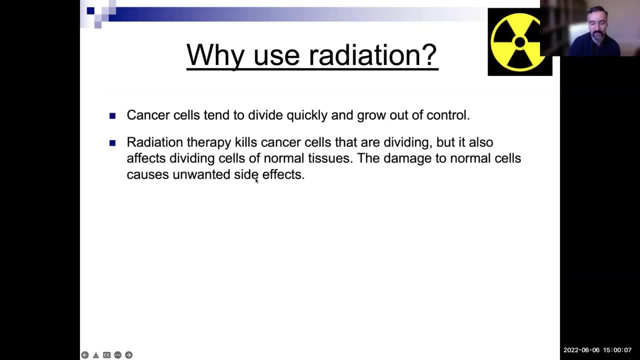 dividing cells of normal tissues. So the danger to normal tissues, the organs at risk, is important to consider to minimize side effects. So it's always about a balance between destroying the cancer cells and minimizing damage to the normal cells And the risk of producing a secondary. 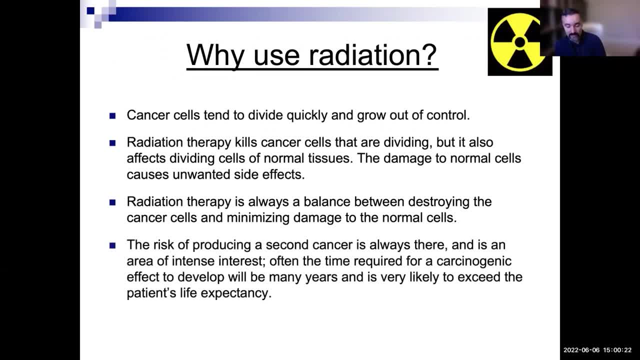 cancer is always there and is an area of intense interest, But the time you know and the time required for a carcinogenic effect to develop over many years is very likely to exceed the patient's life expectancy. Of course, this is a very sort of 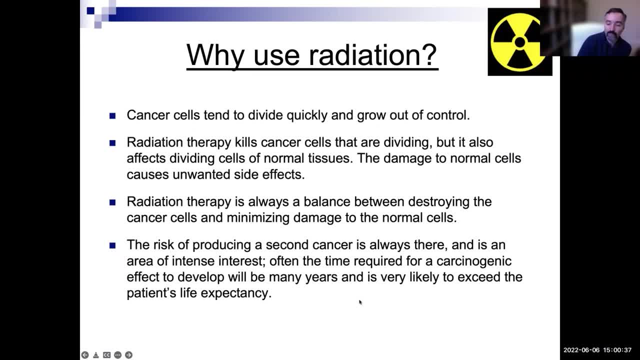 almost oversimplified- actually, not almost definitely an oversimplified- statement. It's an area of active interest. Depends who you're dealing with. You know, with children their bodies are more sensitive to radiation, They have a longer life ahead of them, They're smaller, So 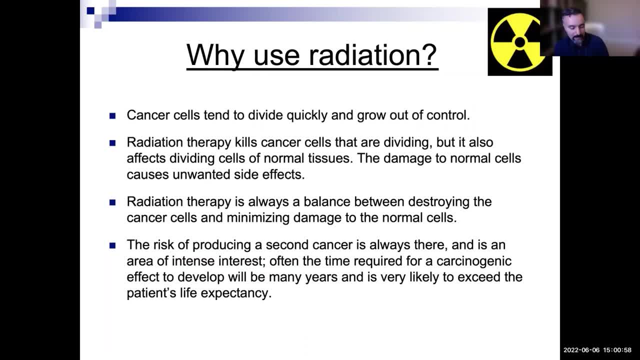 you have to be super careful with in pediatric context. Therefore, the image gently can't paint So, but the point is that you can have the right, you can try to look for the right balance right, And the public sometimes does get overly worried about this, Whereas, of course, 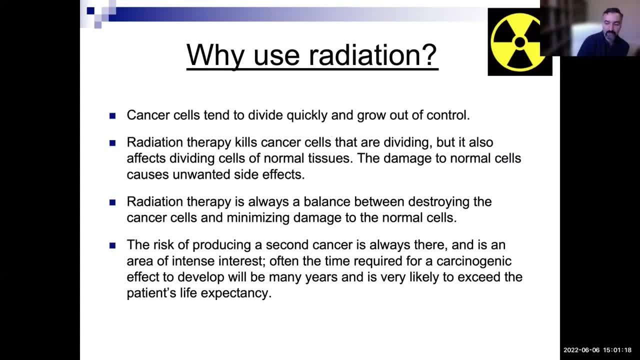 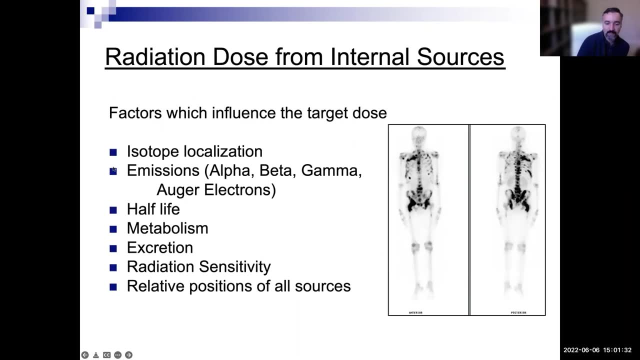 these therapies, as I'll show you some results, can really can be used, as great you know, tools and weapons against, against cancer. So you have an isotope that localizes, It might emit a bunch of things: Alphas, which are nuclei of the helium, Betas, which are beta. minus is an electron. 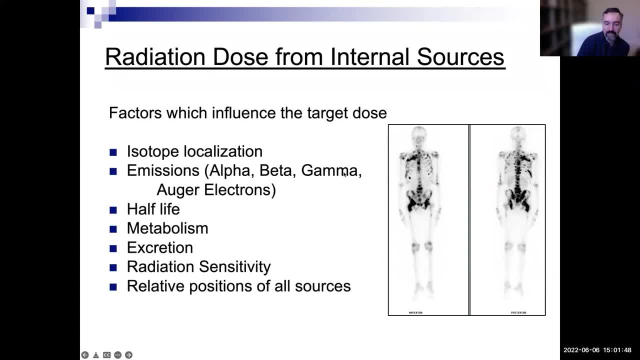 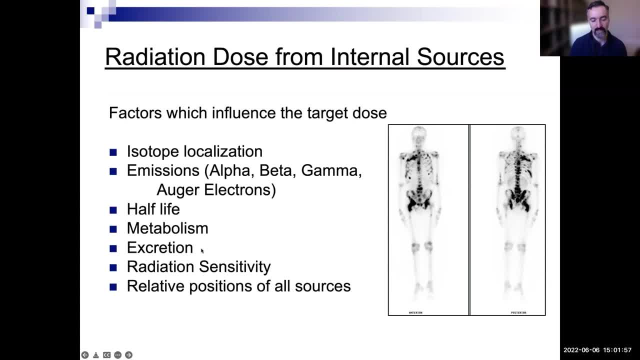 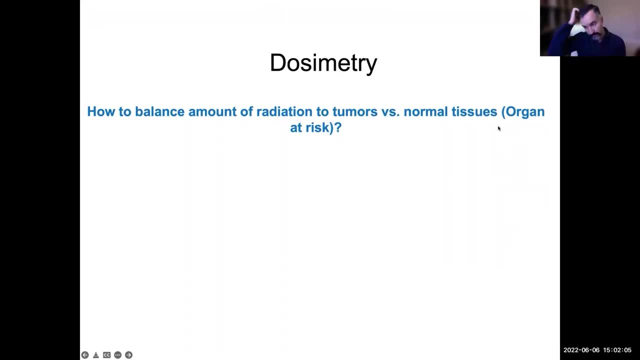 amount of radiation to tumors versus normal tissues. right And, for example, external radiation therapy. that's normal In our field, radiopharmaceutical therapy. we're pushing for the community to perform dosimetry Because some people say, well, let's just inject. 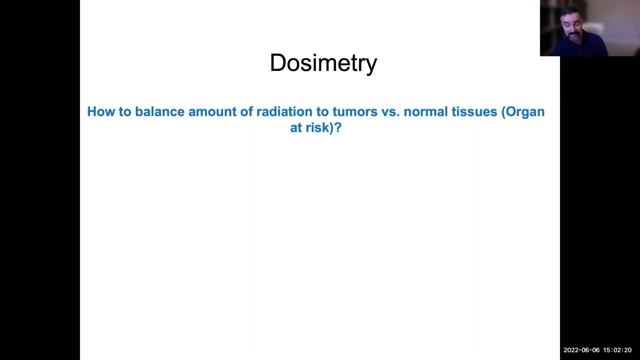 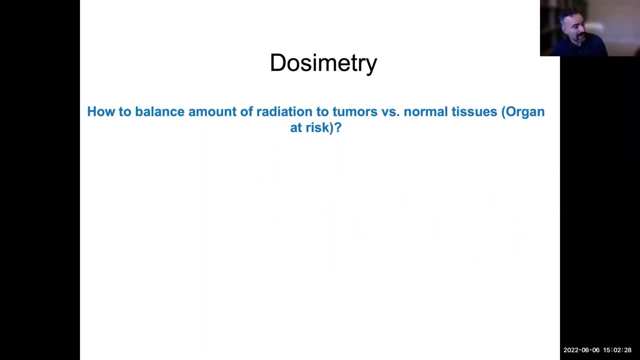 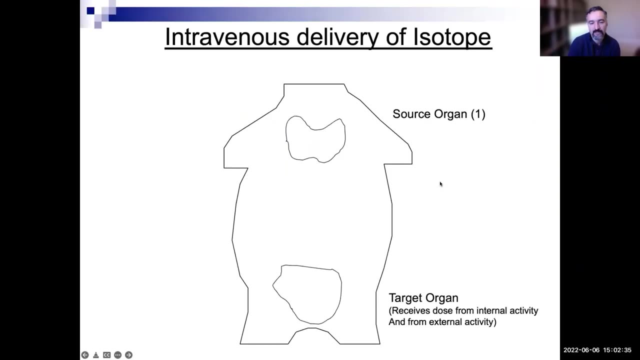 the ethical way to go ahead, to measure how much actually is being delivered to the tumors and to balance the treatment efficacy with normal organ toxicity. So you've got a delivery of an isotope intravenously, for example. let's say You've got a target organ, Okay, And you've got. 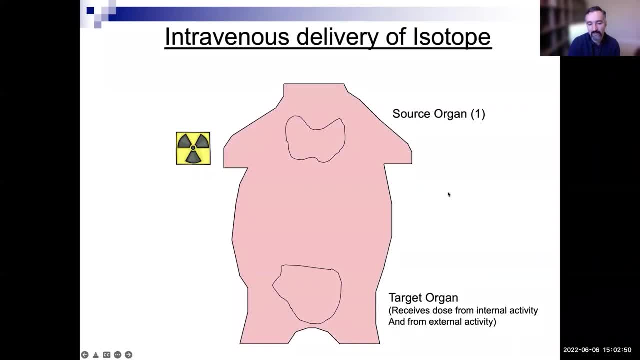 a source organ. So this is just a measurement thing. So, for example, a second you inject, okay, there is accumulation in these two different things And you ask a question. Let's say you ask a question: How much radiation is this organ? 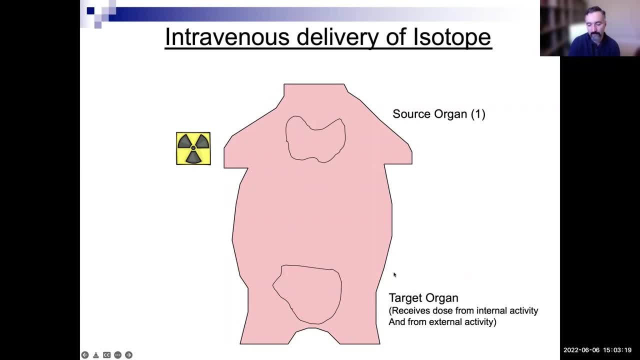 getting from this organ. So that's the source target. Okay, So how much? I want to know how much radiation is getting from this organ. So that's the source target. Okay, So how much? So how much dose I'm getting here from what I injected, which is how much it accumulates? 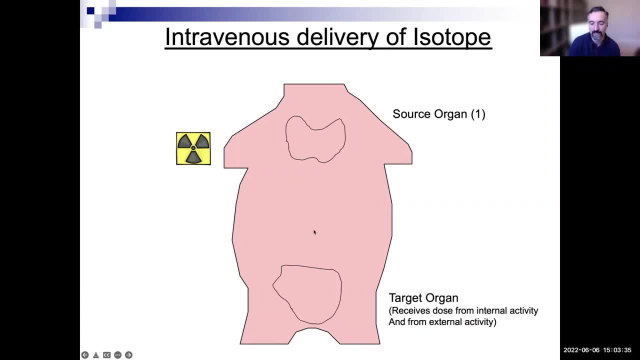 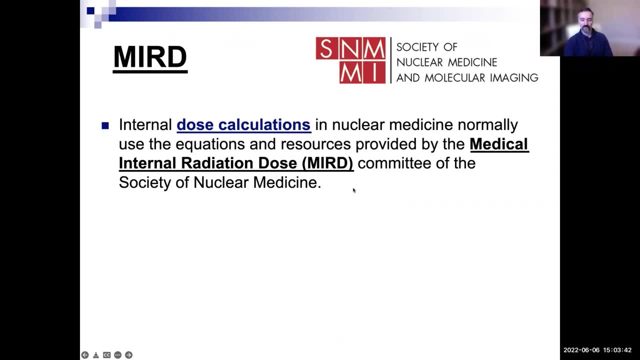 but also from nearby organs, when they emit light, for example. that passes through me as it comes through. So, in turn, those calculations are normally using certain equations and resources by the merit committee And standards. models have been developed in the past and there's 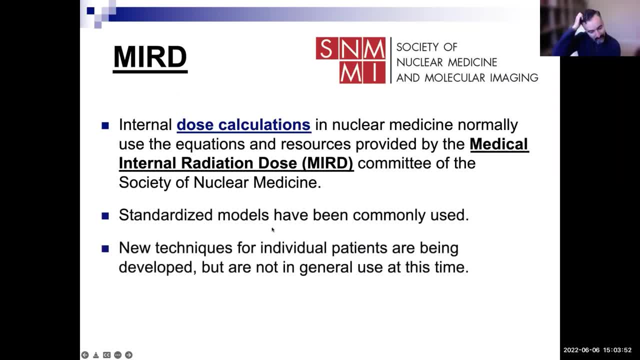 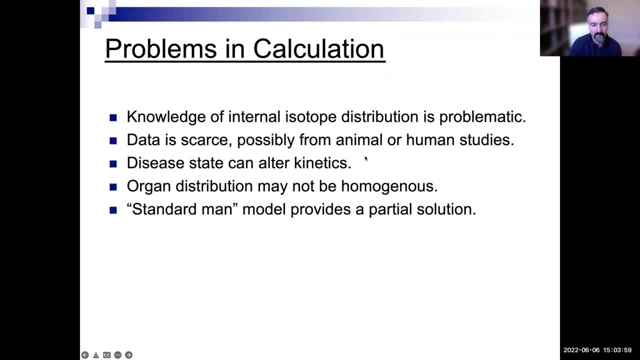 increasing movement towards personalization Instead of a, you know, standard man. you know it's towards personalization. You need knowledge of the internal isotope distribution. So you've got to image the patient after you injected radiotherapy to see how much and where, Or even 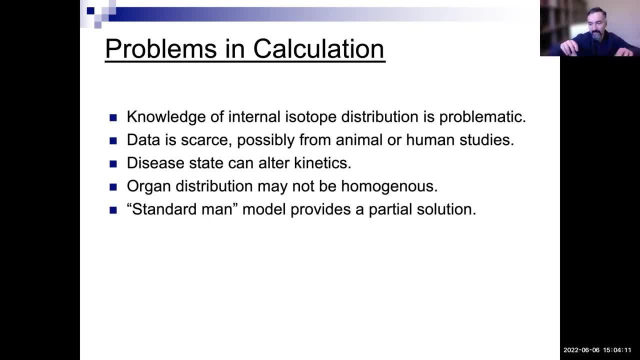 once you inject, if that thing you've injected itself emits gamma rays, you could actually use a SPECT scanner, for example, to measure what's there, And there's a number of problems in calculations. Data is scarce. You may not have a lot of information. 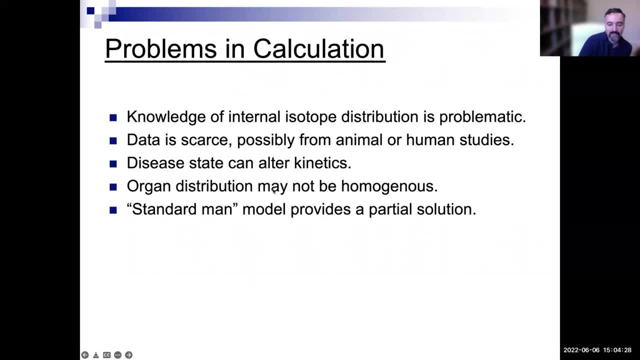 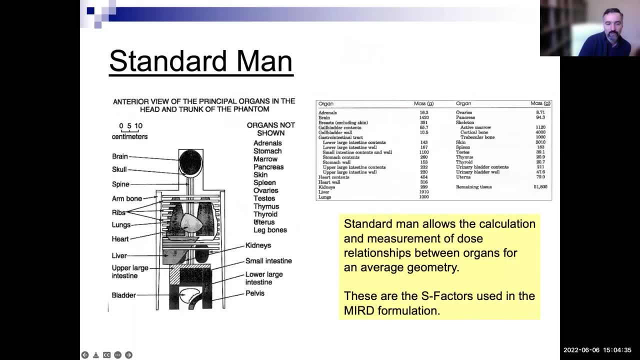 The kinetics might have changed, Organ distributions may not be homogeneous And the standard man is only a partial solution. You know, here's a standard man, But there's a need to understand more Like. here's a question: If there's an accumulation, deliver. how much dose is going? 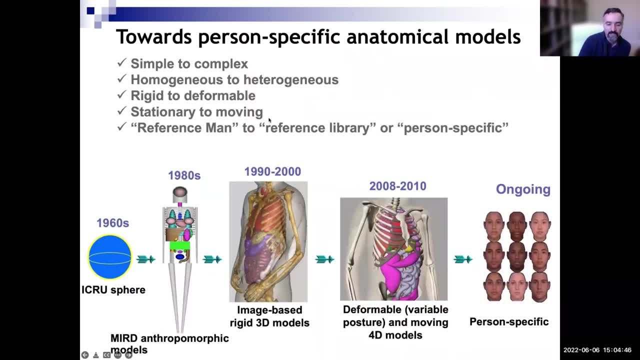 to go to the kidney for the standard man. But you've got a whole range of people. So there's been movement towards personalization of models So they could do dose calculations not just on the standard man but but on men and women of different ages, for example, right, and different body types, right. 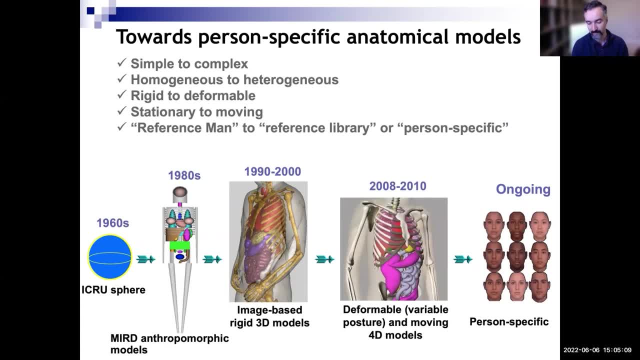 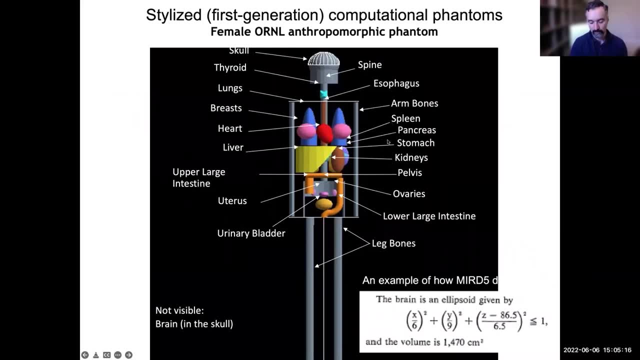 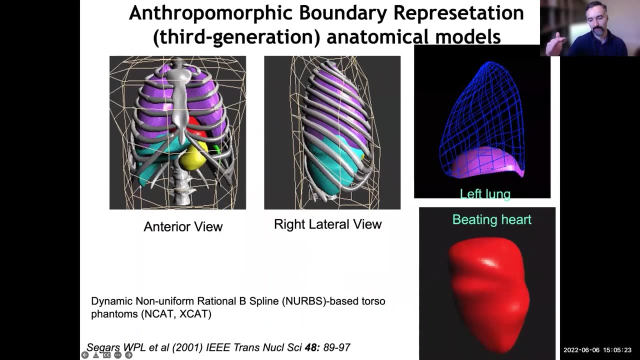 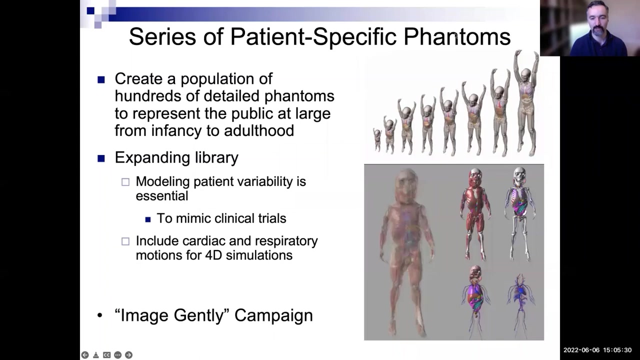 different phenotypes. So again, moving beyond really conventional geometrically defined phantoms to voxel-based definitions, to fitting smooth surfaces to the body. So you know there's a lot of movement in this space. This is an area of active research I'm just sharing with you. 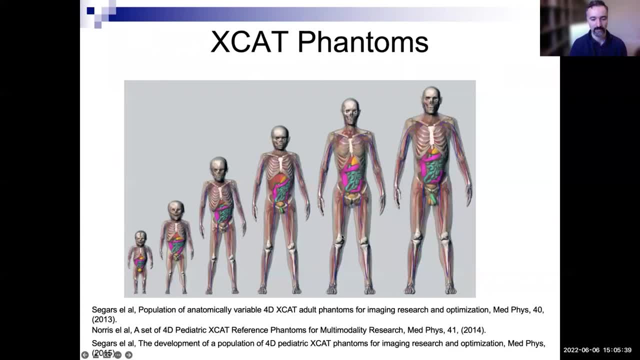 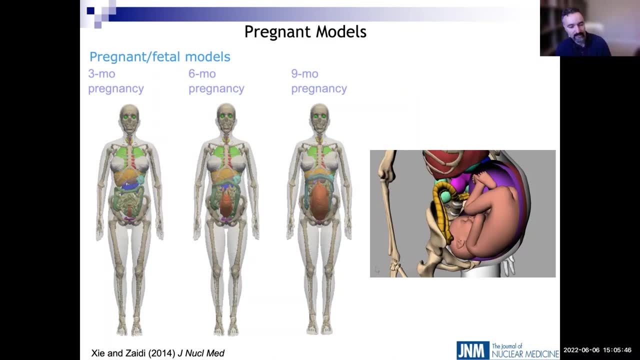 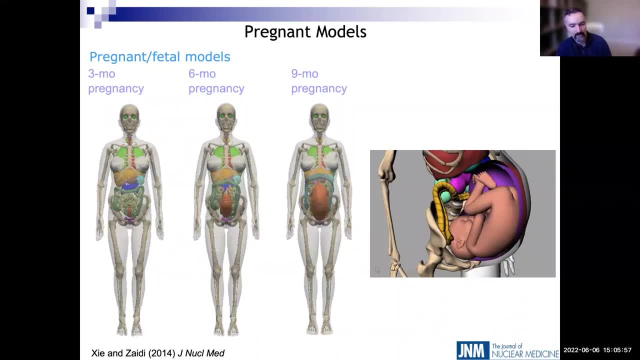 it's very complex. Again, you do the derivativex analysis because of course, as things change anyways, you can do the calculations because of pregnancy and how much is being delivered. So again, to a fetus you can have radioactivity delivered directly right, but also indirectly. 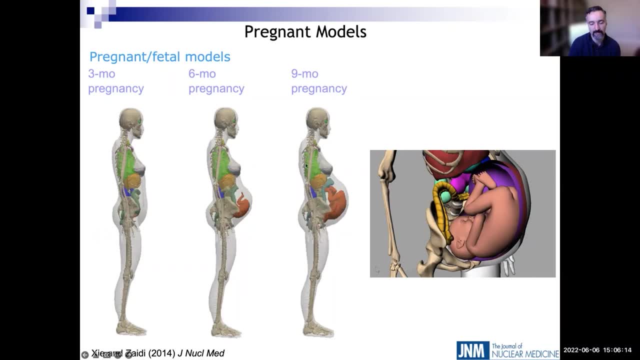 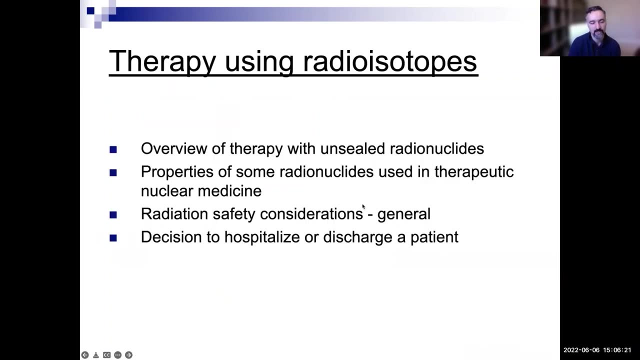 through the bo-, through the rest of the body of the mother, right, Whether the activity ends up in the fetus or ends up elsewhere, but then, through radiation, enters and impacts in the fetus. So So, yeah, so therapy using radioisotopes. 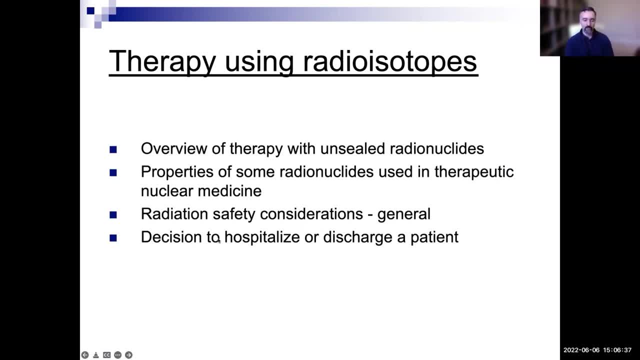 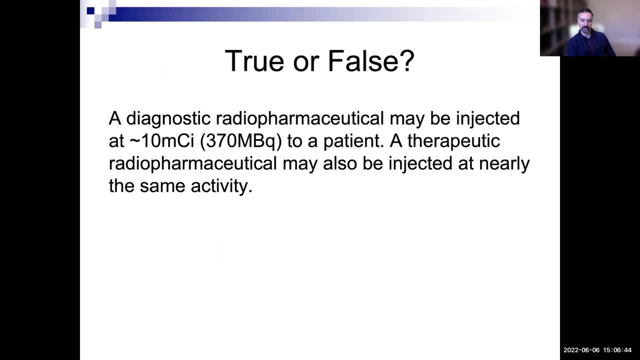 Let's talk about that. It's a question of: okay, when you, for example, when you discharge a patient, what are some radiation, occupational hazard issues right for the technologist, for example? I want to ask you a question here. 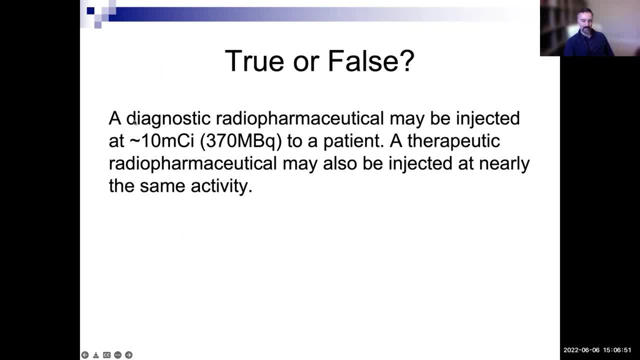 A diagnostic radiopharmaceutical may be injected at a certain radioactivity, let's say 10 millicuries, A therapeutic pharmaceutical may also be injected at nearly the same activity. Is this true? So, for example, when we do FDG PET, this is how much we might inject. 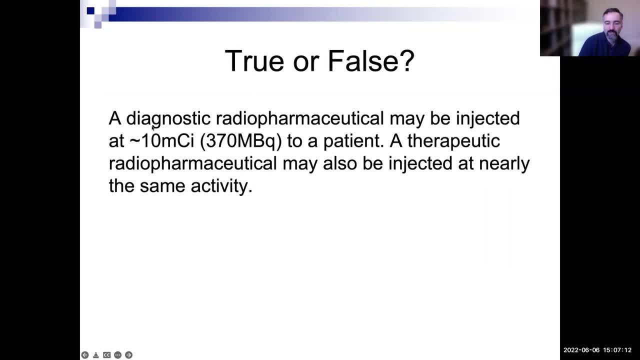 Is it true that a therapeutic radiopharmaceutical may also be possibly injected at the same radiopharmaceutical dose, Or does it at the same injected radioactivity, Or does it have to be Higher than this? Anybody any thoughts on this? 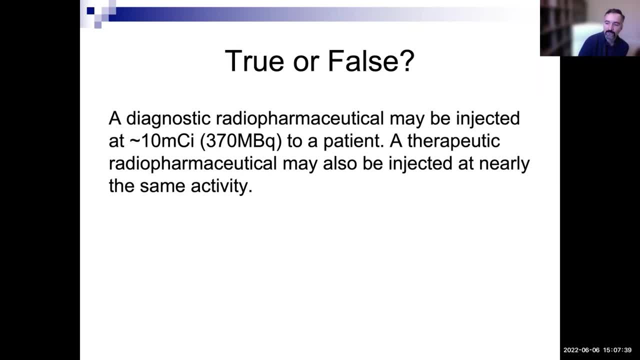 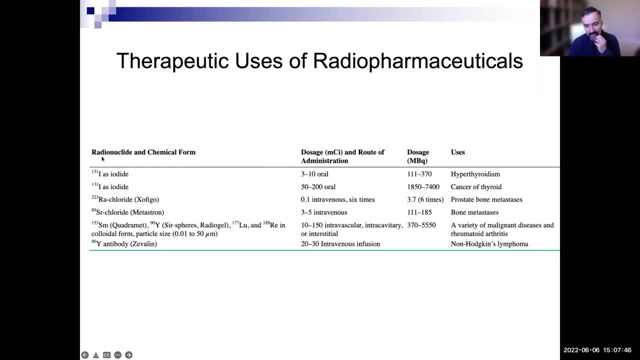 I think usually the typical response is no, it has to be much higher. But the answer is no, it doesn't, because it depends on the half-life. For example, if you've got something that is having, For example, if you've got something that has a long half-life, which 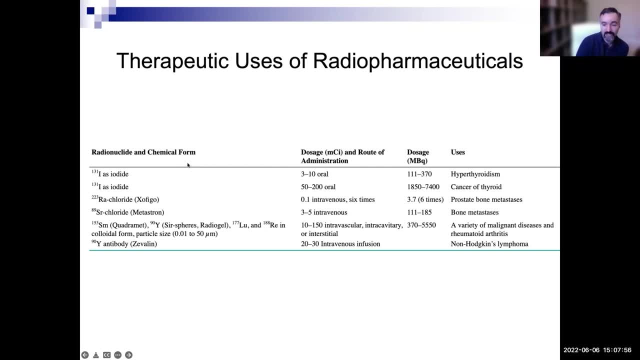 Which, Which, Which, Which therapeutic isotopes do? even though you're injecting the same, let's say, 370 megabecquerels, it's there in the body for a long time because there's a large half-life. It's not like F18. 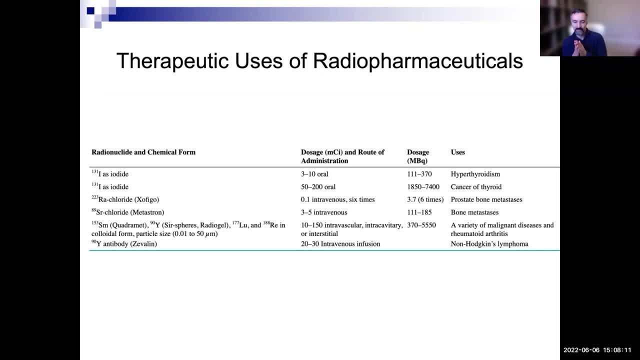 where the half-life is only two hours, The physical half-life. here the physical half-life might be days. It's actually okay to inject the same radioactivity, but that radioactivity is there to stay for a long time, So the total accumulated dose will be much higher, which is 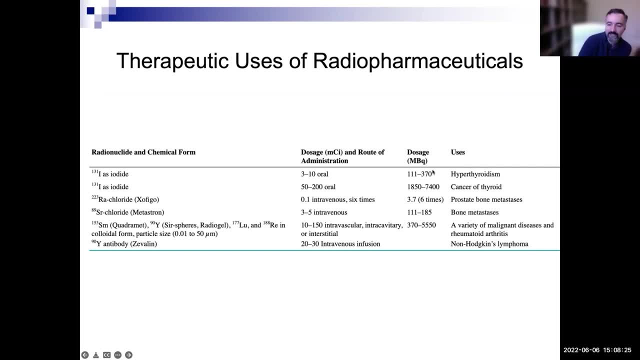 what we need. So, yes, it's possible that the injected radioactivity is only 370 megabecquerels, which is 10 millicuries, but because it's there for a long time, it can be therapeutics. These are different examples of how some of these things are injected or taken up orally, for example. 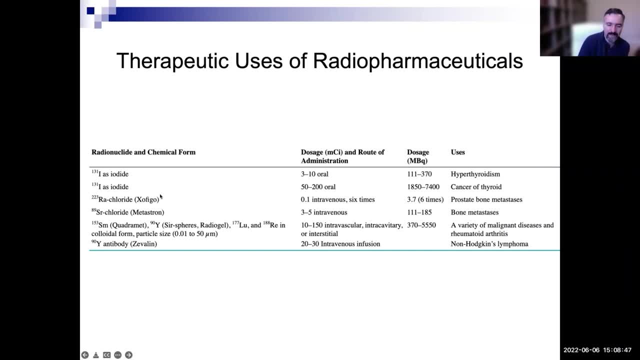 And so different uses, indications. just some examples: Lutetium and Yttrium-90 are, for example, two very sort of important applications that are being used increasingly. So Yttrium-90 is here. I didn't mean the antibody. 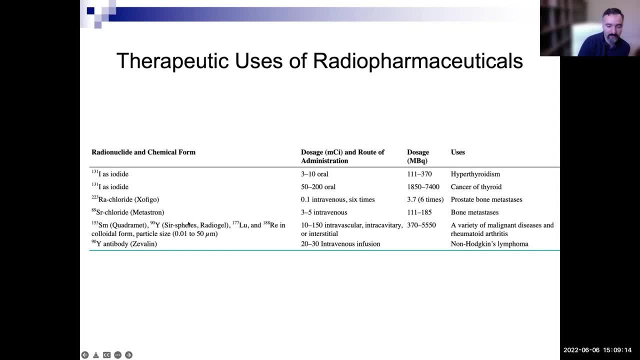 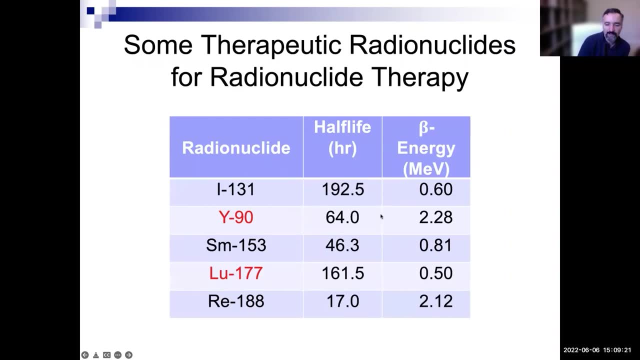 I meant just using Yttrium-90 in different, actually here for spheres. So I would say these two are very hot topics and we can talk about them here. So you see the half-life, half-life of the order of days, right, And they're emitting beta-negative, which means 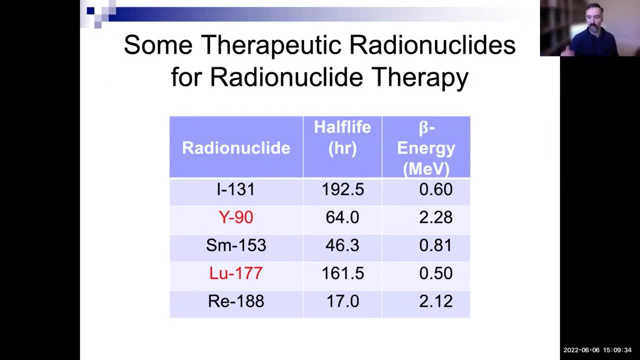 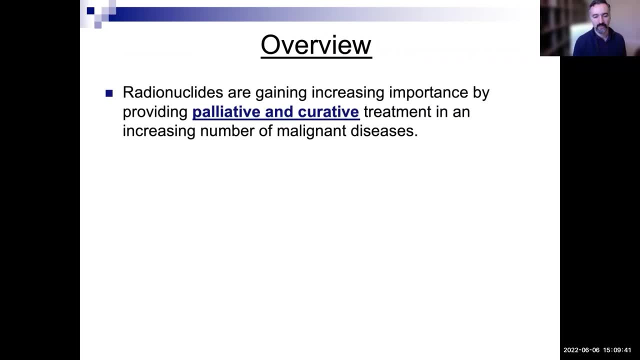 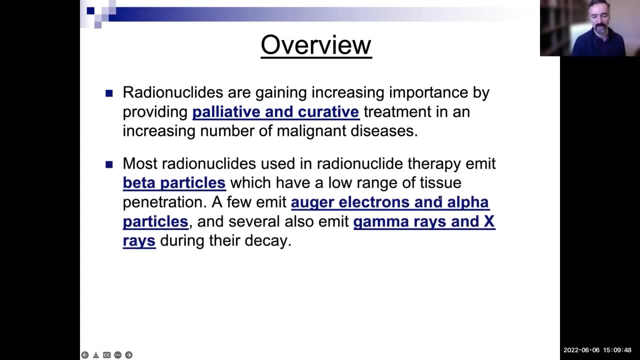 electrons. So that's how what the killing mechanism is, or the particle has been released, And so there's a lot of interest in palliative and curative treatment phenomena. You could have be emitting beta particles, OJ electrons or alpha particles. Now some of these also emit. 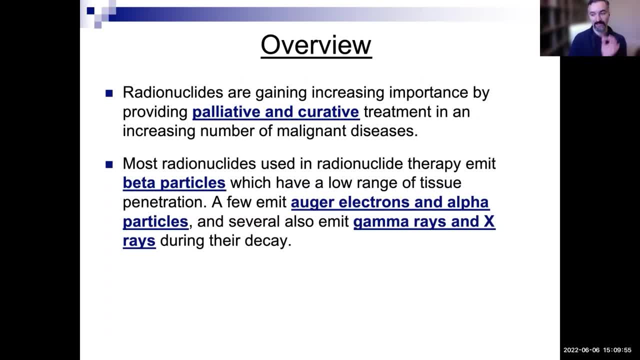 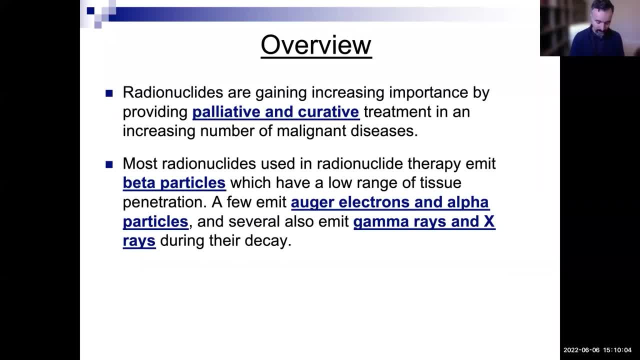 but if if you have a radiopharmaceutical or a radionuclide that emits both particles for therapy and some light for imaging, then the same radionuclide is theranostic in itself. So so again, iodine is something that's been used for decades. Okay, 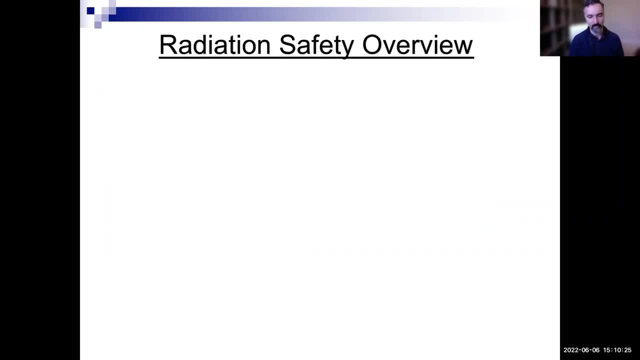 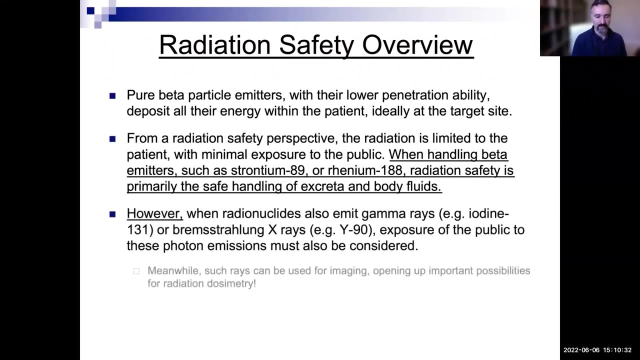 Uh, but there are new ones that are taking people away with a lot of excitement. So I'm going to skip over some of these uh radiation safety issues or just go with them. go over them very quickly. Uh, from a radiation safety perspective. 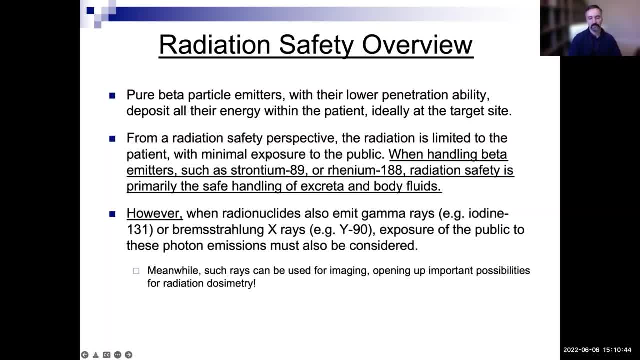 uh, there's typically not much exposure to the public. Okay, Uh, one aspect with some radionuclides is the safe handling of excreted body fluids. With a number of other ones, there is some gamma rays or some so-called bremsstrahlung X-rays coming. 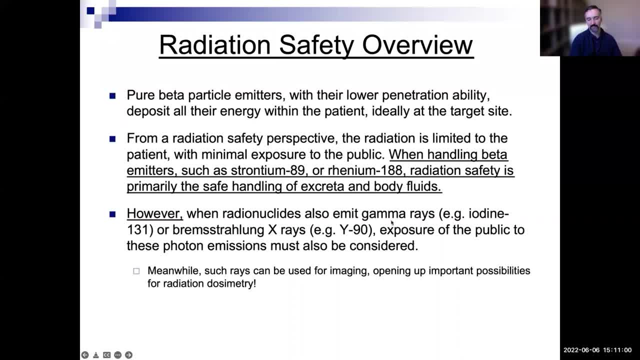 out of the body of the patients. It was important to understand exposure of the public to these. So, even though they're being treated by particles coming up, but there's some light, some gamma rays or X-rays coming out too, Um, we have to understand how much that is. 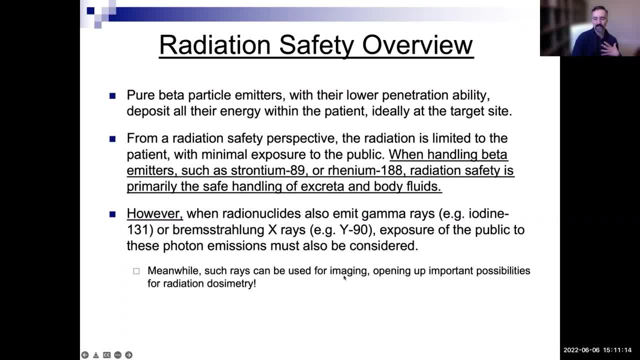 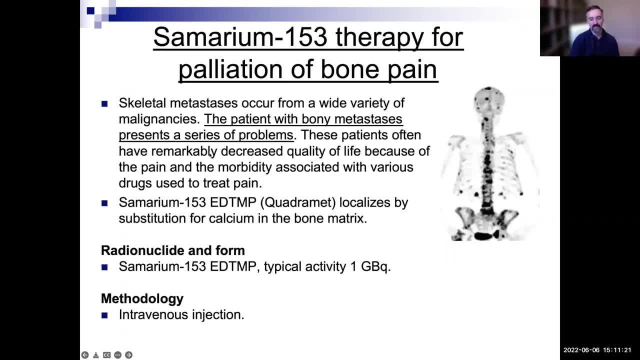 how safe it is to be around those patients. But the beauty of these things that you can also use them for imaging, so that allows you to do radiation dosimetry while the patient is being treated. Okay, So again, I'm not gonna go over these in detail. 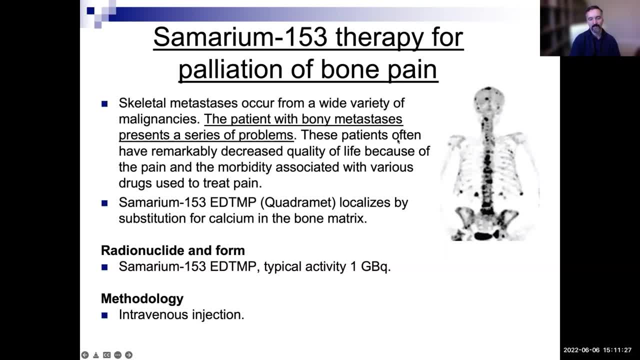 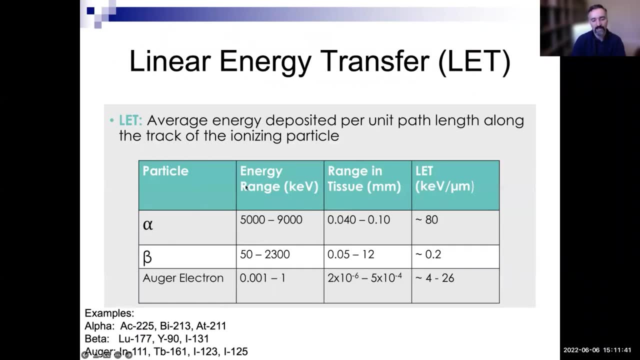 So here's an example of using samarium for palliative care of bone pain with bone metastases. And again, the particles could be alpha, beta or Auger electrons. They have different ranges, different tissues, So beta particles have longer tissue range. 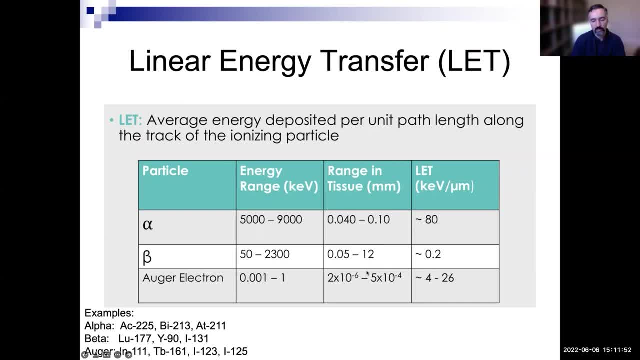 whereas alpha is more localized and Auger is even more localized. An example of alpha, beta and Auger right. So again, lutetium is popular, Atrium-9 is popular, but people are really looking at things like actinium for alpha therapy, et cetera. 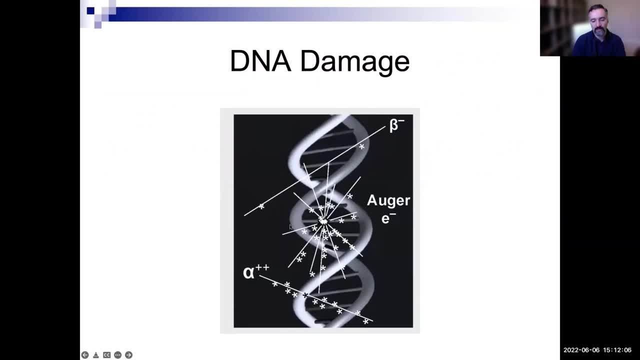 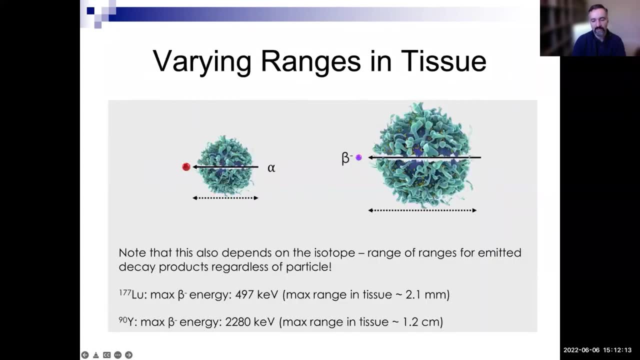 So again, beta can go a larger distance, Alpha can be more localized, even do double DNA break, and Auger is even more local. So again, also the beta itself depends, Like you could have two different betas like lutetium or Atrium-9, they have different beta. 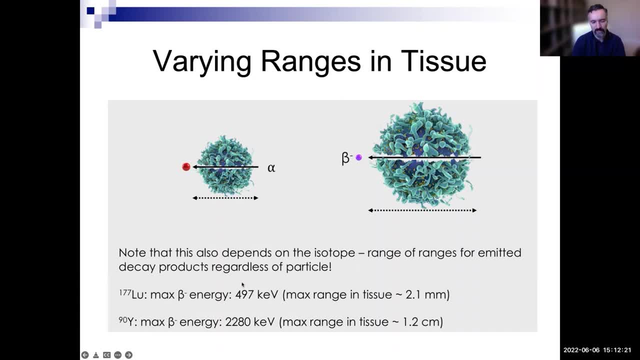 maximum beta minus. Beta minus means electronic. So you have two different electron energy ranges. When the electron comes from in a nuclear phenomenon, we call that beta, because it's not coming from the shells, It's coming from the generated because of a nuclear phenomenon. 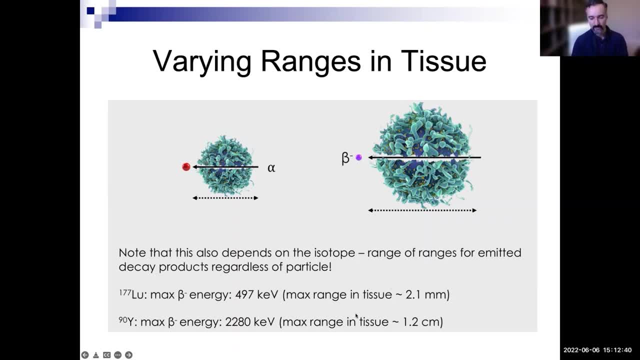 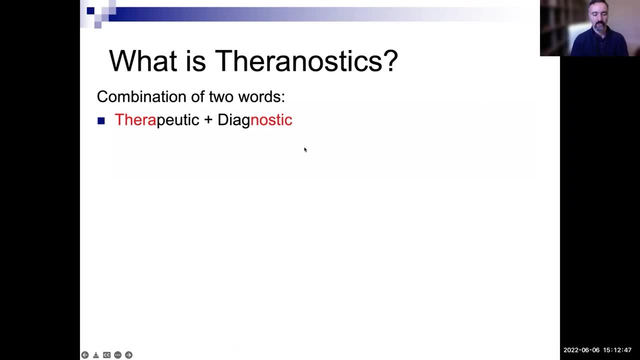 But anyhow, effectively it's the same thing. The source is different, but you see the range in tissue of lutetium on average, or the maximum, is higher than the Atrium-9.. So what is theranostics? Combination of two words: therapeutic and diagnostic. 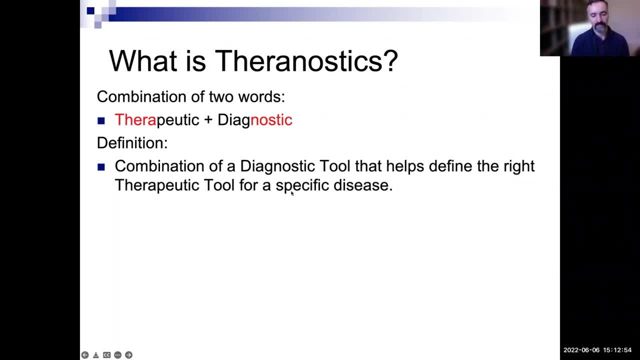 It's a very important board and field of research. It's a combination of diagnostic tool that helps define the right therapeutic tool for a specific disease. So it's extremely natural in nuclear medicine Why? Because you can use a radionuclide label agent. 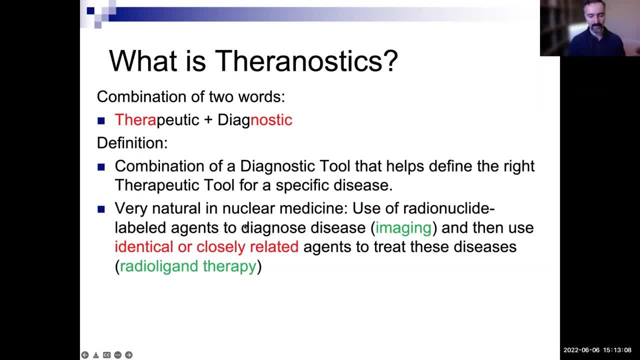 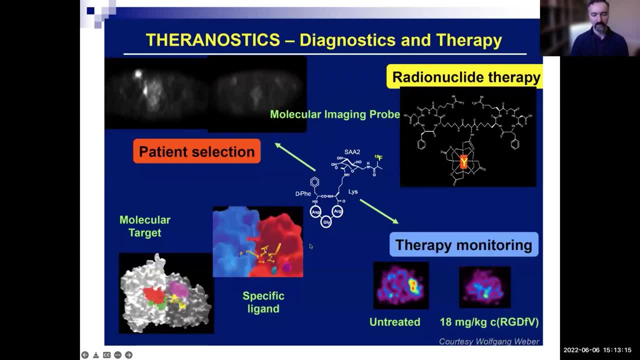 to diagnose disease for imaging and then use the same thing or closely related agent to treat those diseases, like radiopharmaceutical or radioligant therapy. So here's an example where you've got a molecule that is radiolabeled with something that emits gamma rays. 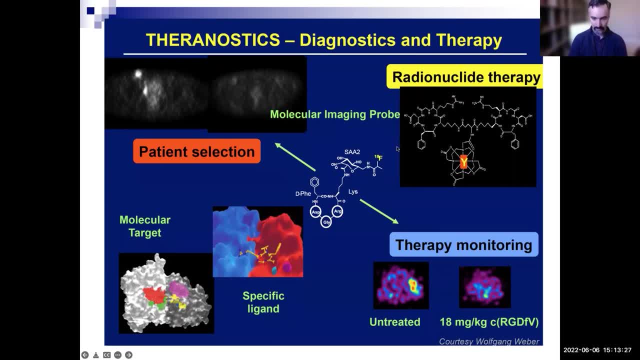 This molecule: if it's radiolabeled with something that emits gamma rays, then you can do imaging. If it's radiolabeled with something else that emits particles, you can do therapy. So the idea that you can treat what you see and then see what you treat. 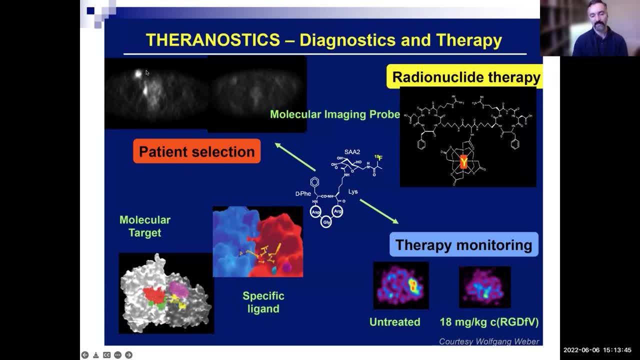 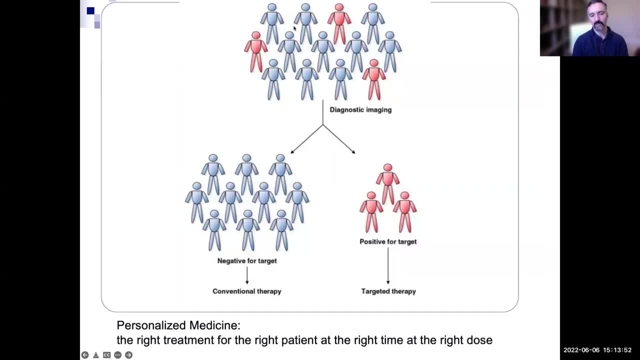 So first see it, make sure it's there, then treat it and then see followup during the therapy or after therapy, what you actually did to it So you could take a number of patients, pre-select using imaging. which one of these express those proteins. 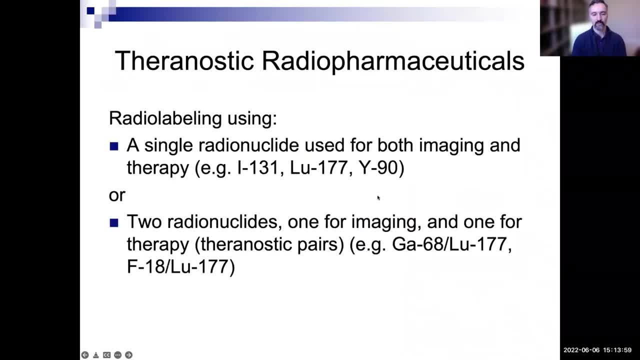 put them on therapy and then follow what happens to them. So theranostic radiopharmaceuticals could be a single radionuclide that has both imaging and therapy. like idon-1, therion-1 gives you both particles. 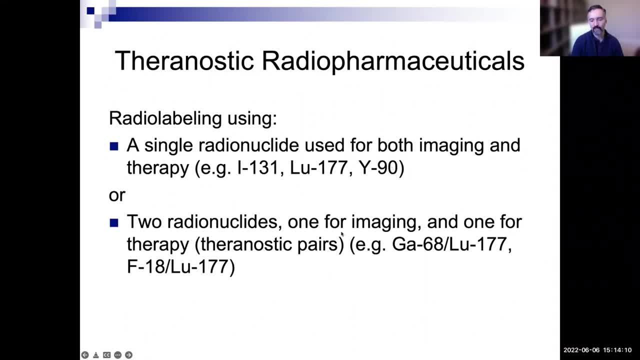 and gamma rays, lutetium-190,. or two different radionuclides: One is for imaging, let's say gallium-68 for PEH, and one is for therapy, lutetium-177,. okay, You could do that too. 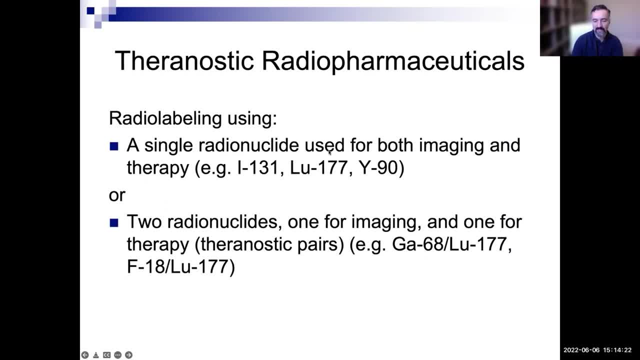 Don't notice. lutetium-177 also gives you light, so you could. even in itself it's theranostic. but you could also use it as a pair where this is only for therapy. You don't really measure the gamma rays coming off of it. 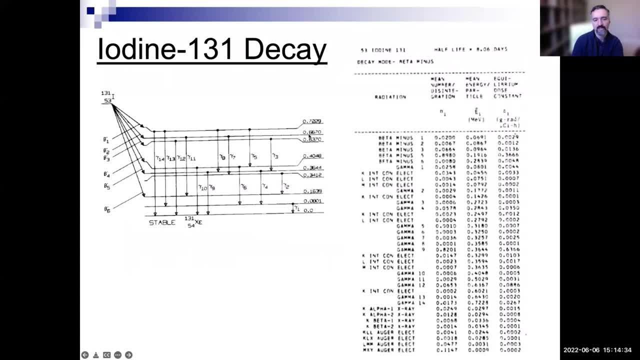 but you pair it with a pre-therapy PET, for example. So idon-1-31, there is beta minus, there's- you know that is being emitted. There's also gamma rays being emitted. So you can visualize what you're doing. 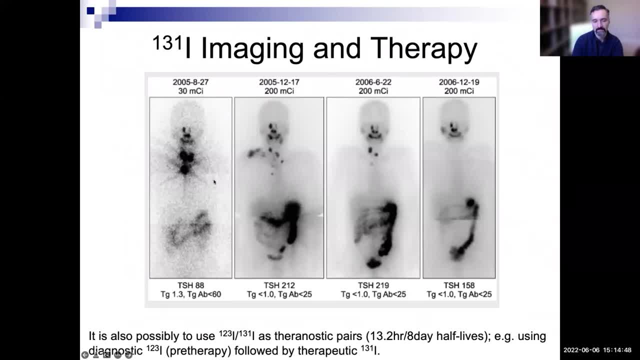 So this is a patient: 30 millicuries. you're seeing what you're doing. You're seeing that accumulation, You're seeing what you're doing. Okay, And then you could also use pairs like idon-1-31 for therapy. 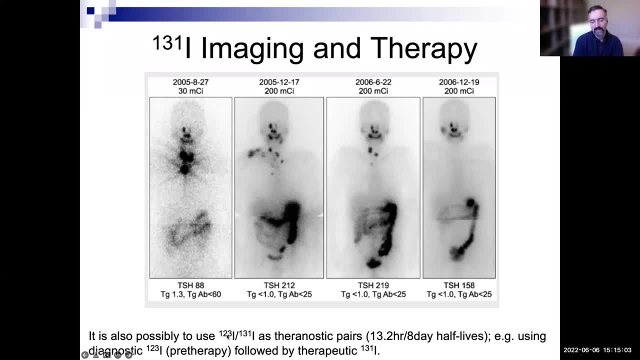 but then you do idon-1-123 as a theranostic pair because it has a much smaller half-life. Instead of eight days it's only 13 hours. So you could use this for pre-therapy diagnostics and then you could do the therapy. 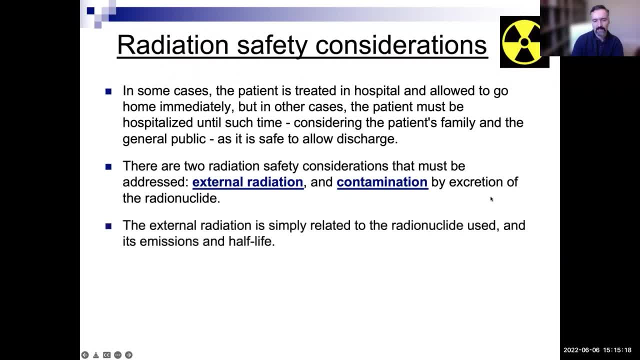 So radiation safety issues- again issues of external radiation and contamination by excretion, that you have to be, you know, careful about. So the excretion aspect, contamination of patient's environment, These are things that one has to be. there are protocols about it. 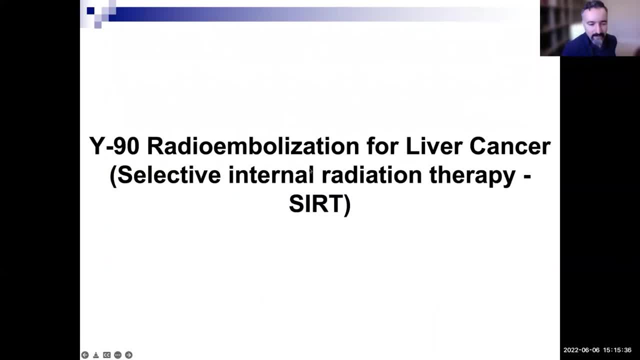 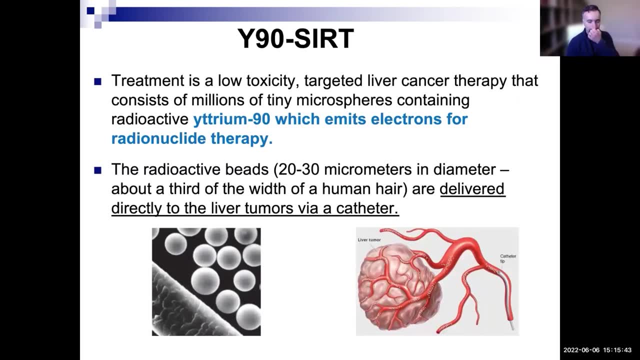 and I'm not gonna go through that, those details. Another example which is quite interesting is Yttrium-90 radioembolization for liver cancer. This is kind of a cool area. It's kind of like brachytherapy to microbrachytherapy. 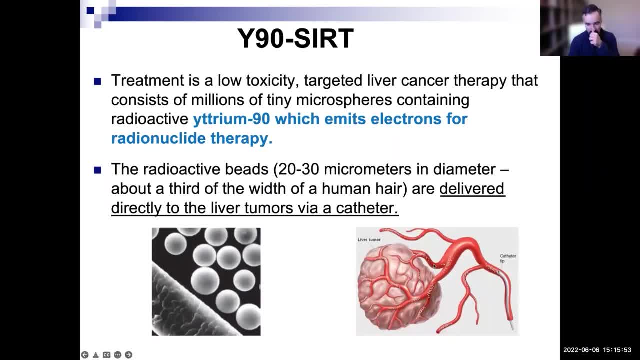 because, in a sense, what you deliver gets lodged in the vessels. It's actually a kind of a mix between radiopharmaceutical therapy and brachytherapy. It's this hybrid entity which is not easy to categorize. It's a category of its own. 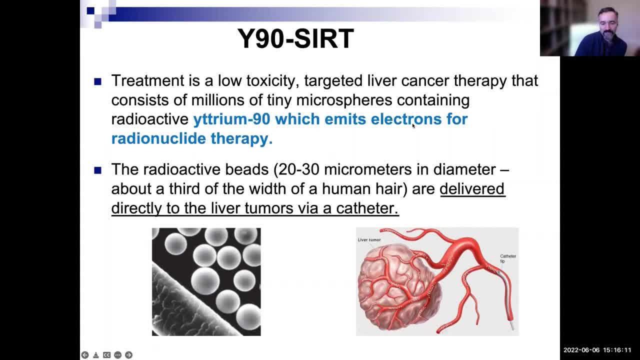 Basically, what you do is you have Yttrium-90,, which emits electrons, and then you put them in radioactive beads and you deliver them directly to liver tumors via catheter. And then so it goes and the catheter tip here. 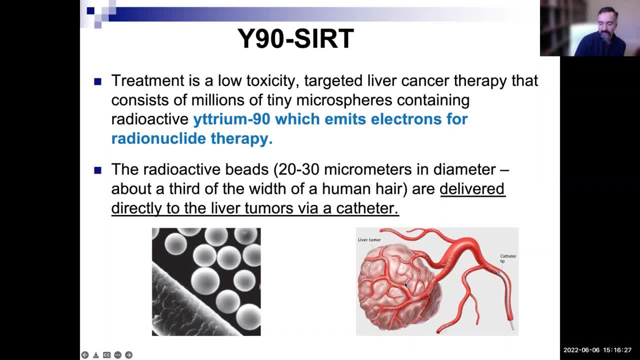 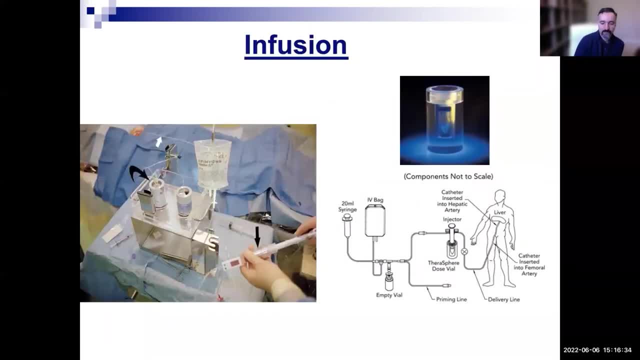 and then they get lodged here in the vessels, They sit there for a long time and they bombard the heck out of the tumors, right? So here's an example of the infusion and different kinds of spheres or beads that can be used. 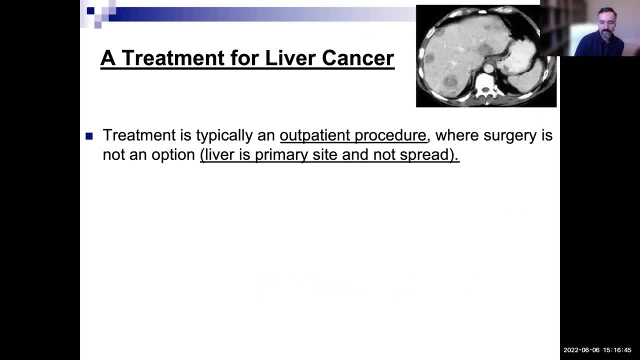 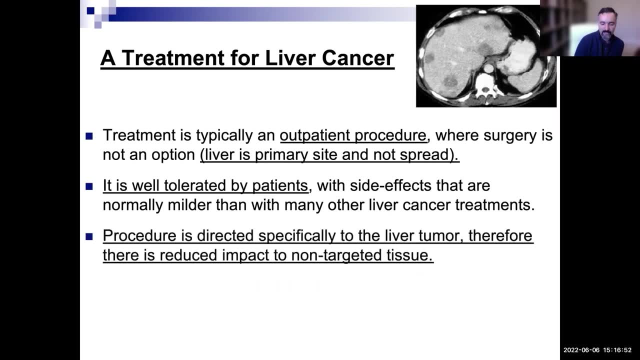 Okay, Typically it's an outpatient procedure. Liver is a primary site, well-tolerated. focusing on liver tumor, I'm minimizing impact to non-targeted issue And patients can be further treated because you don't block the vessels of the liver. 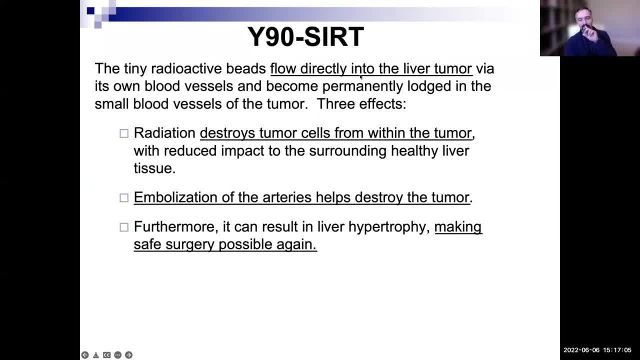 So the beads, the radioactive beads, flow directly into the liver tumor and three things happen. One, you're destroying tumor cells from within the tumor. right, because they're there radiating. Secondly, it's a radioembolization or embolization. 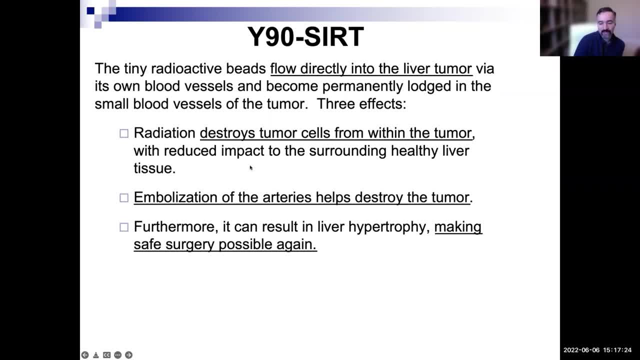 So you're embolizing the arteries right And so you're suffocating it, suffocating the tumor in a sense, and you're helping destroy it. And third, which is kind of interesting thing, it can actually result in liver hypertrophy. 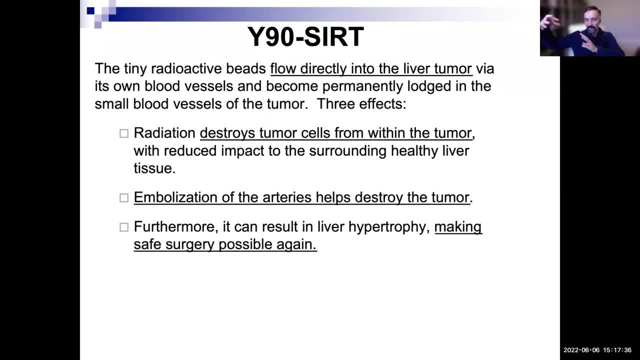 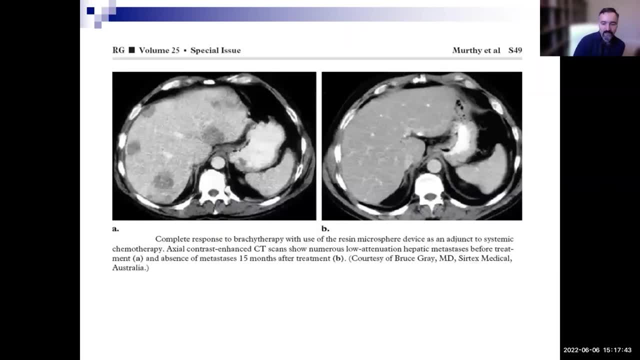 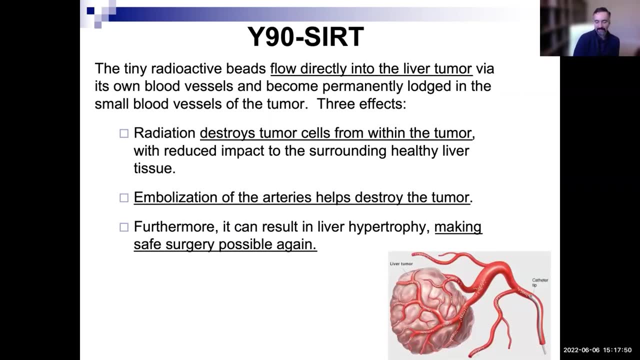 In normal tissue it actually can result in growth. So diffraction, once you're done, you may have had a case where you may have had a kind of a liver that was non-resectable, but after therapy the tumor has shrunk. 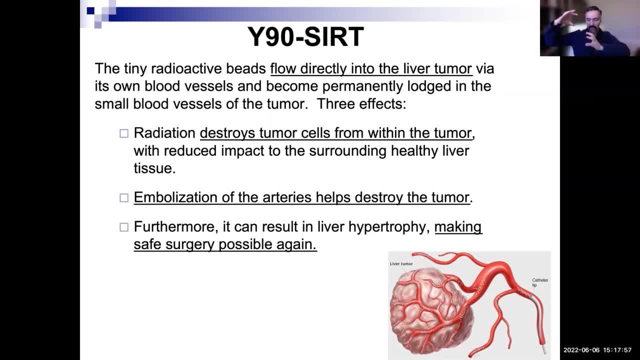 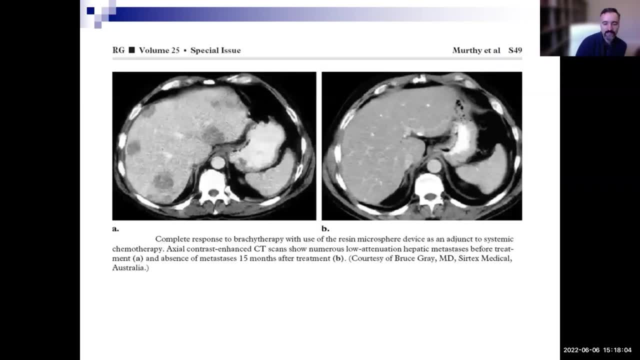 and the normal tissue has actually sort of undergone hypertrophy and the ratio has become just right so that it is now resectable. So some images of CT, for example before treatment, here and after treatment, And it reminds you how can you image it well? 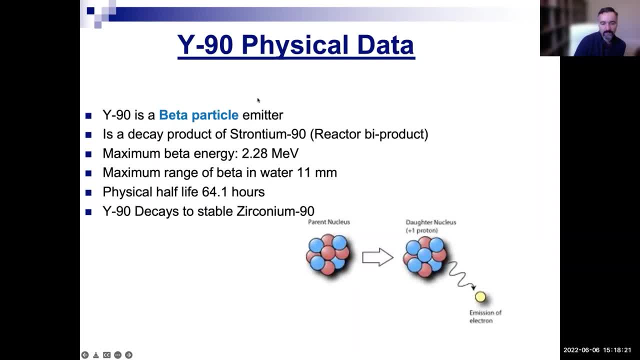 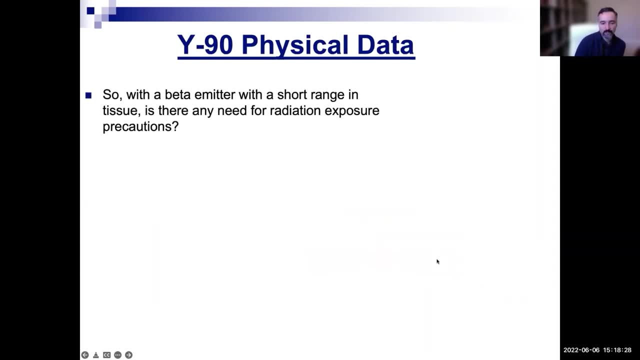 it's a beta particle emitter. that's a particle for therapy, but it also- it can also- result in so-called bremish drawdown phenomena. So, first of all, from a radiation safety, if it's emitting beta, do you have to worry about radiation exposure? 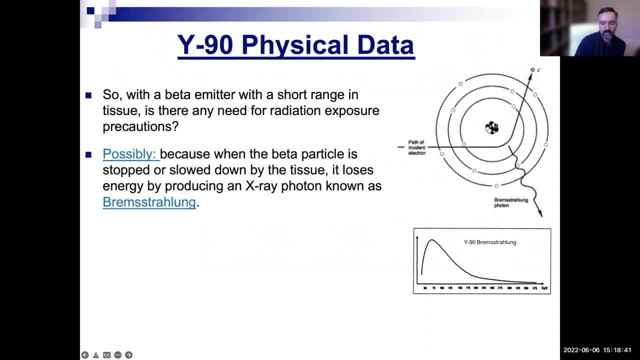 The answer is yes, because when you've got beta particles that are slowed down by the tissue- some of their- they lose some of their energy through the so-called bremish drawdown phenomena As it's curving through here, as the beta rays are being produced here. 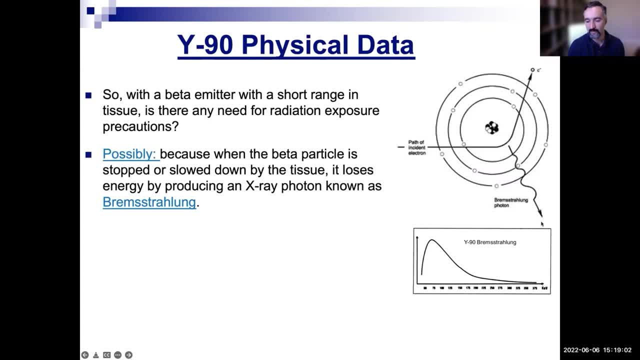 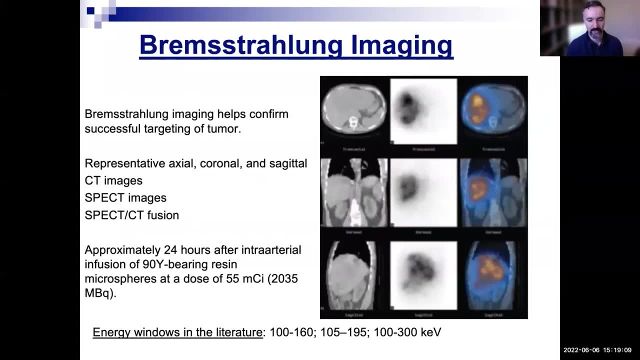 in this curving here, it creates bremish drawdown photons And this sort of can come out of the body. So that's the issue. So there's a radiation thing associated with that. But you can actually use those bremish drawdown x-rays. 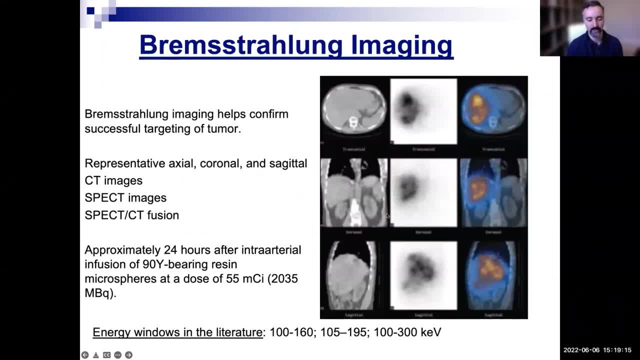 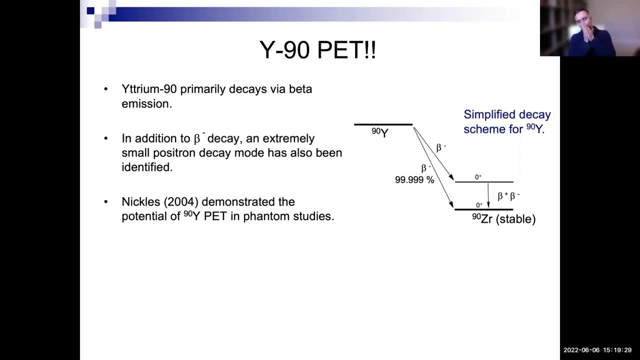 to do imaging actually, So you could actually use SPECT imaging to visualize those x-rays coming out, And so you could do SPECT imaging and visualize what's going on there using the right energy windows, et cetera. There was also discovery that there's a very minute amount. 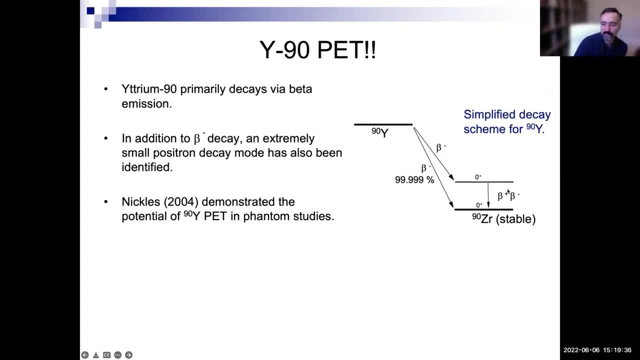 of PET signal, many positrons. very, very small amount of positrons. It's not even shown here because it's so small compared to the 99.9999%. It's a very, very, very small amount that people discovered. you know the fraction. 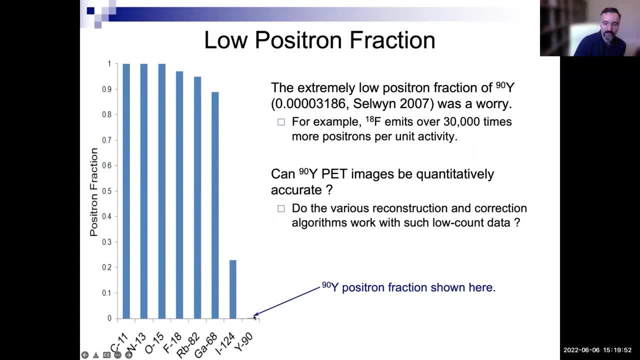 the fraction of positrons is so small it's even hard to see it here, okay. So, for example, fronar 18 emits, relatively speaking, 30,000 times more positrons. So at some point people thought, well, so what? 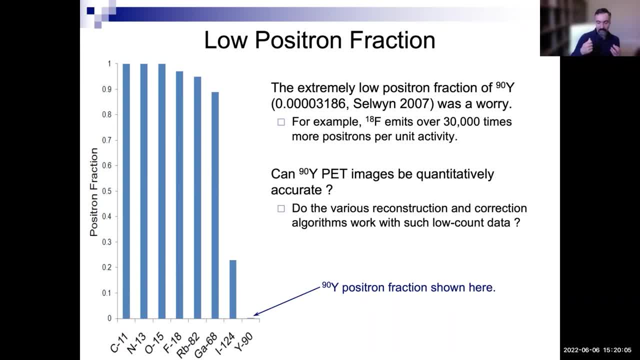 But then because, again remember, PET is more sensitive than SPECT, much more sensitive than SPECT because of the coincidence detection, the fact that you don't have physical collimators. People ended up showing that because you're injecting high doses here. 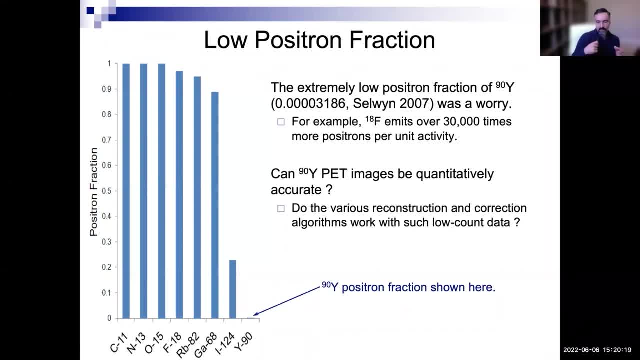 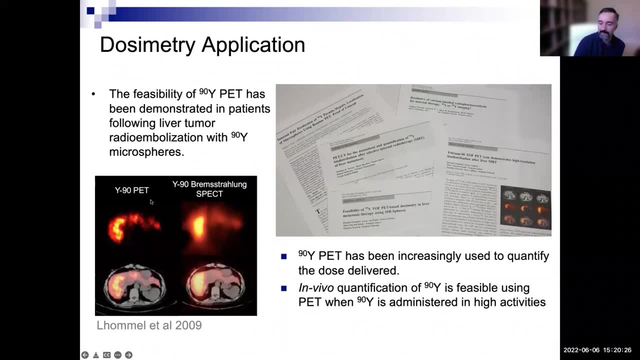 into the patient for therapy. there's sufficient positron emission that you can actually do PET imaging. So people started showing that, to the great surprise of many people. I remember the hesitations we all had in those years when we were like: are you kidding me? 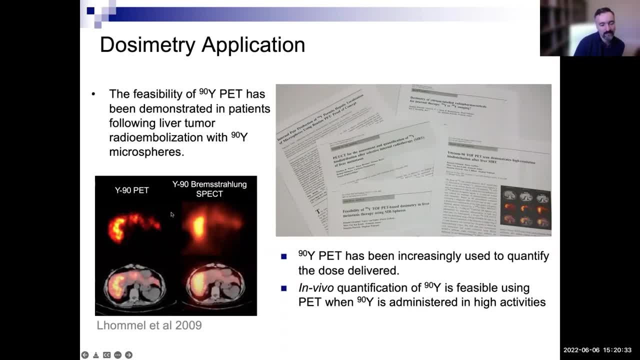 Are you really gonna be able to do PET imaging of 18.99?? And guess what? Look at the images: 18.99 PET compared to Bramstrahlung SPECT. Bramstrahlung SPECT is not really quantitative because it's very difficult to model in a detailed way. There are some attempts in making it quantitative, but you know there are some attempts in making it quantitative. but you know there are some attempts in making it quantitative, but you know there are some attempts in making it quantitative. 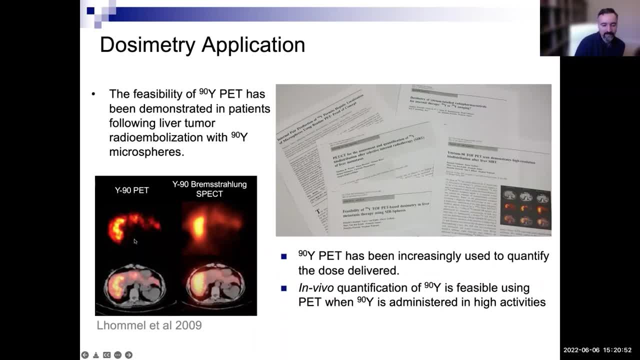 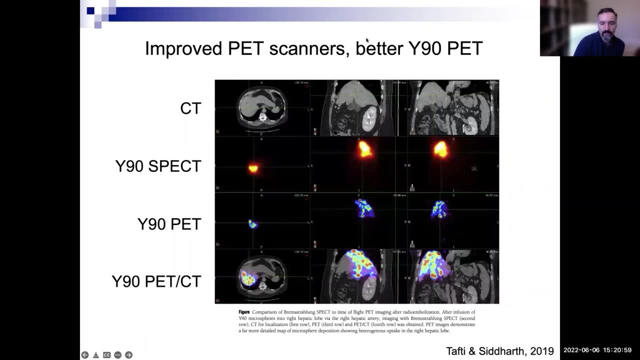 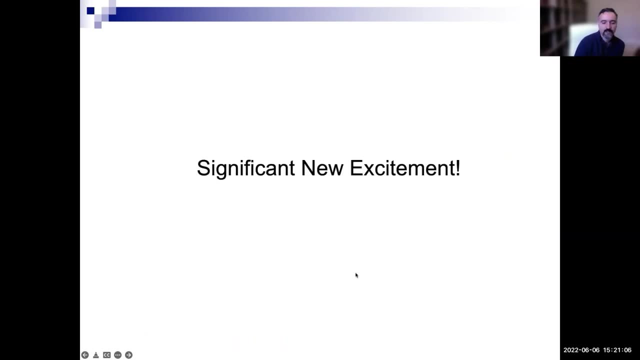 but it's very tough. But 18.99 PET can be more quantitative, But anyhow, both are options for imaging, And so- improved PET scanners, you can get better 18.99 images. So the significant new excitement, though, is okay. 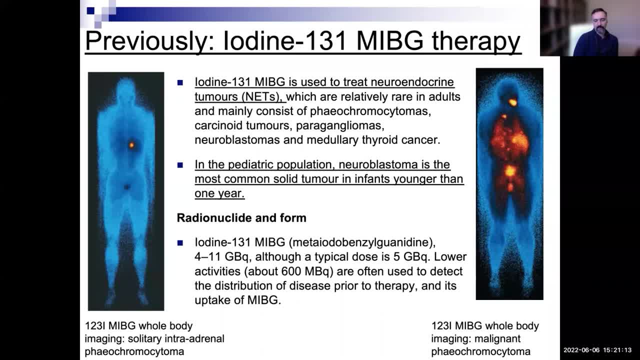 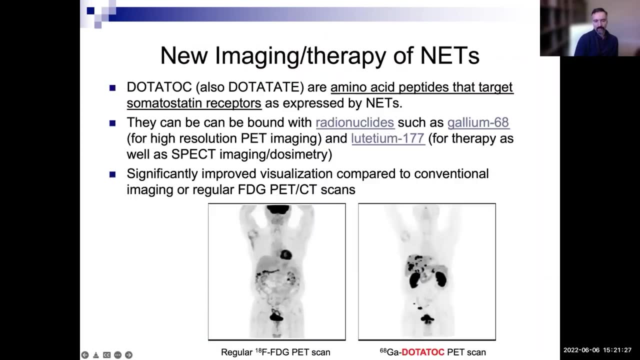 so in the past we were having, like, let's say, IDON1-31 therapy for neuroendocrine tumors, But then something happened, Okay. so just to show you before treatment, after treatment, that's great, But then people started really focusing on you know. 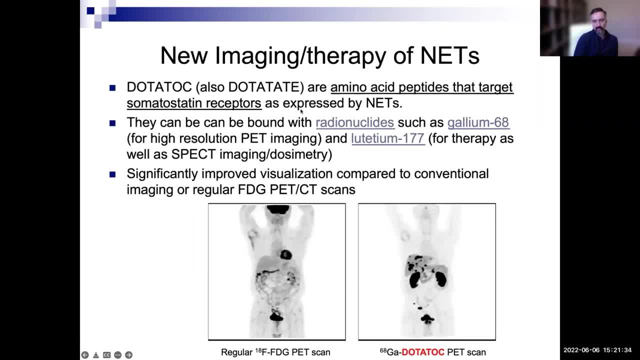 using amino acid peptides, these small molecule that really target the receptors that are being expressed on cancer cells, like for neuroendocrine tumors, for example, And so DOTA-TAC or DOTA-TATER are examples that do that, And you create a label with something like Gallium-68. 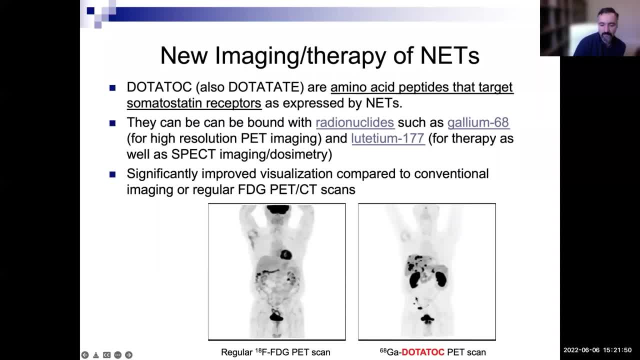 to do PET imaging. Okay, Which is here. And great label: Lutetium-177 for therapy. Notice how this image is so different than the floor. the conventional fluorine FDG PET scan. You see more things. There's the imaging side. 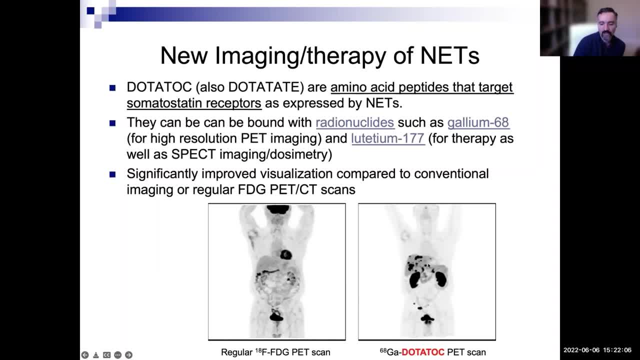 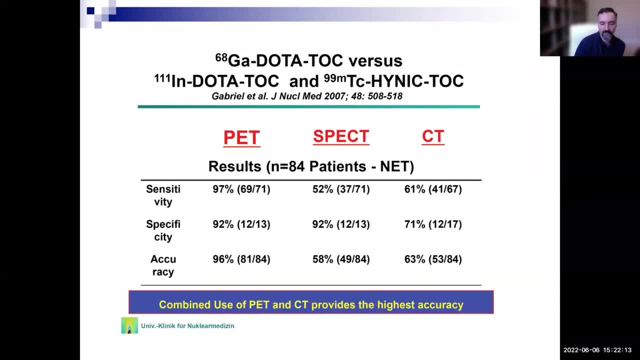 but the therapy side is pretty amazing too. So you get very high focal uptake with sparing of organs at risk, relative sparing, and you can really do better. So first of all, imaging-wise the PET: we saw a lot of things. 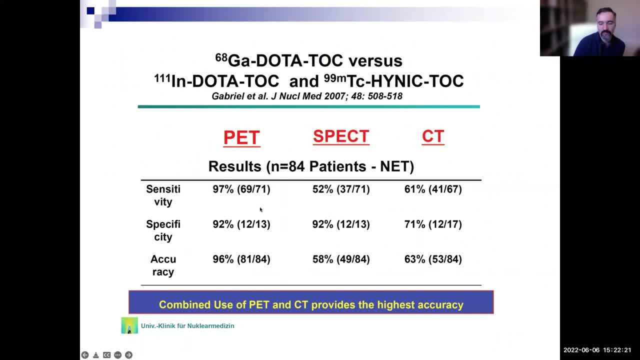 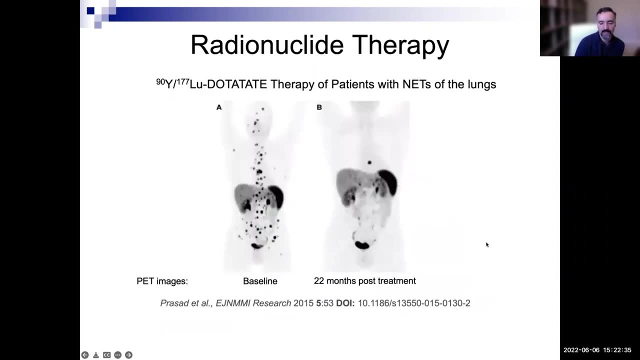 It's superb sensitivity-wise in detecting tumors compared to CT. and you know SPECT using other kinds of things, So Gallium-68, DOTA-TAC, But then again you're targeting the somatostatic receptors. They're sitting there for days and bombarding the heck. 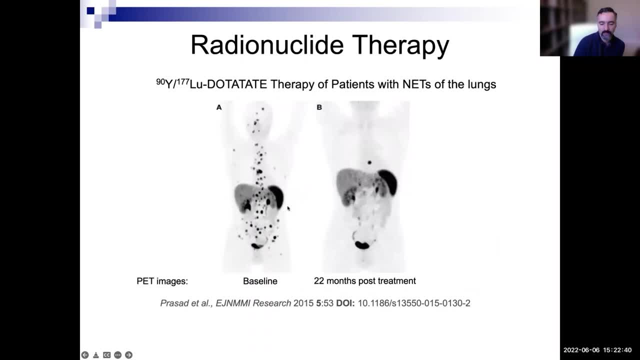 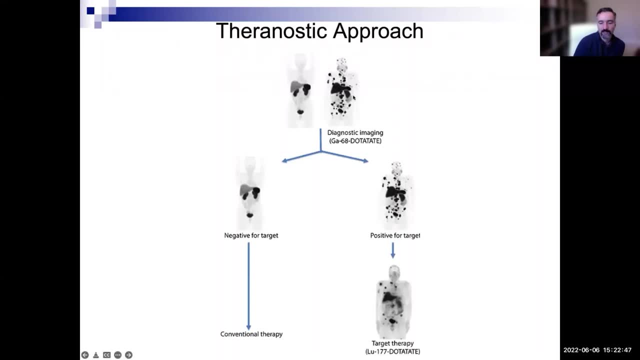 out of all these tumors that are spread through the body. So this is before, this is after, Right. So imaging is you identify which patients express those targets, put them on therapy and monitor them. So again, the idea is you have a molecule that targets. 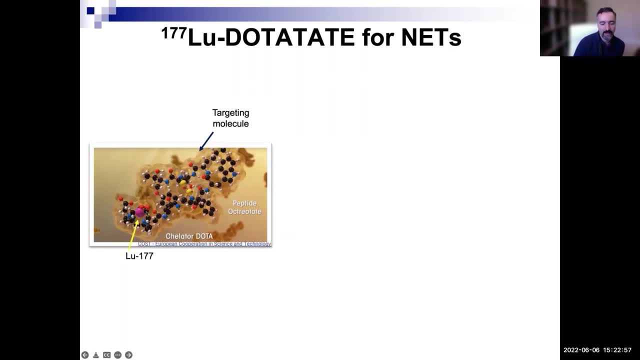 some kind of a protein that's being expressed. You have a chelator that encapsulates the kind of a radionuclide that emits the radiation, the beta radiation for killing and also possibly a gamma emission for imaging. Okay, so you image it. 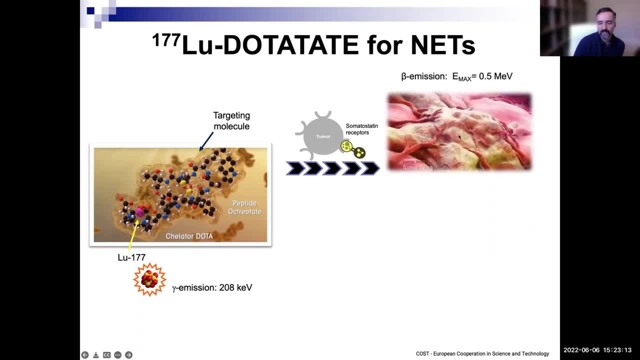 You're killing the tumor as you're sitting and binding, and binding to the cells that are expressing that protein. But also you're emitting some light, single photon light, for example from lutetium, And, if you do, SPECT imaging, because it's gamma imaging. 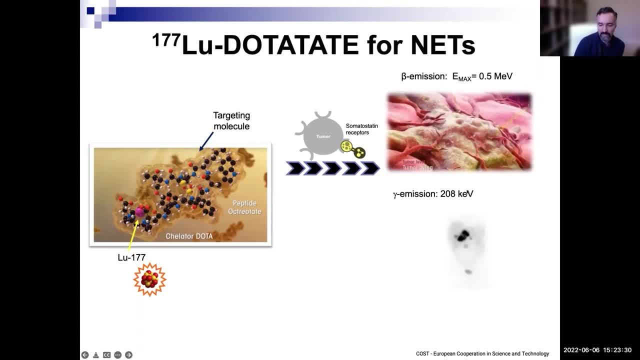 it's not positron, so it doesn't allow you to do PEP, but it allows you to do SPECT. You can actually measure how much dose you've delivered to the patient. So this is dosimetry. We should be doing dosimetry and we're pushing the community. 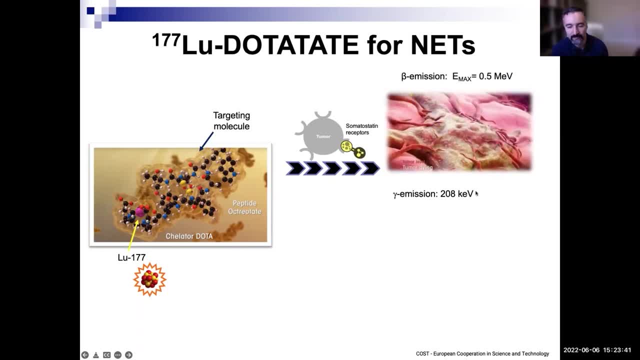 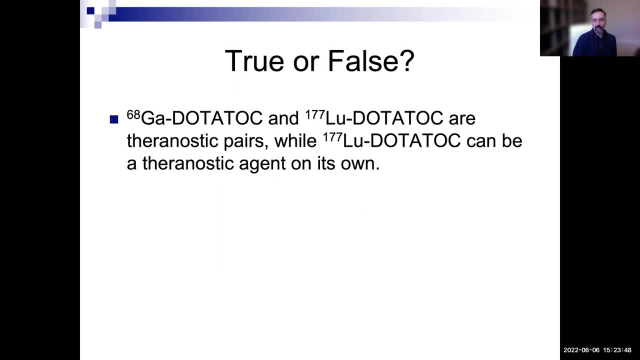 so that we're doing at least some kind of dosimetry, so we know how much we're actually delivering. So is it? quest Questions were false. Gallium-68-dotatog and lutetium-177-dotatog are theranostic pairs. 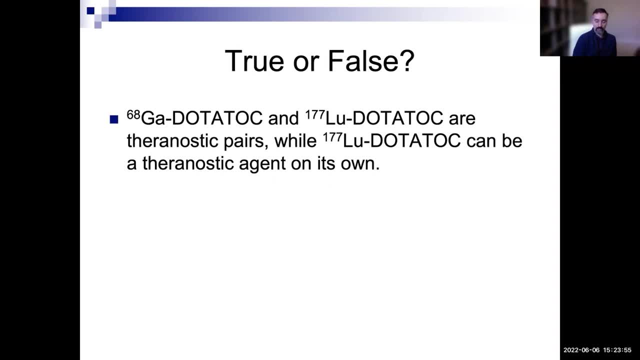 While lutetium-177-dotatog can be a theranostic agent on its own. The answer is that this is true. This is for PET imaging- gallium-68,. this is for therapy, While at the same time, the lutetium-177-dotatog 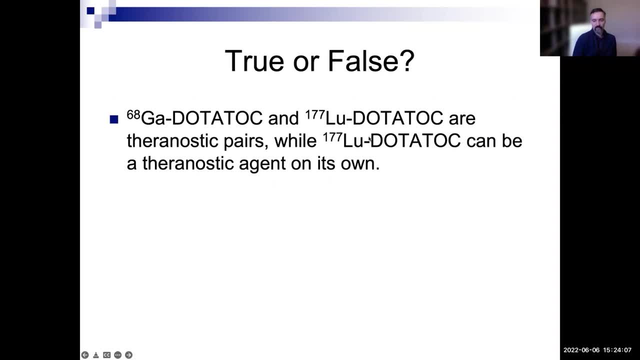 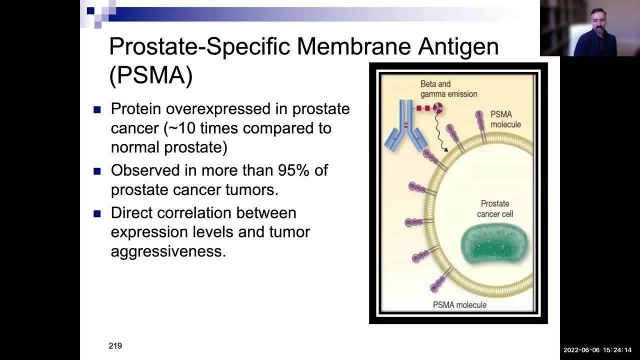 not only does it do therapy, but it also emits a single gamma ray so you can use SPECT to image it. So on its own too, it is theranostic. There's a lot of excitement in prostate cancer, So the so-called PSA you've all heard of. 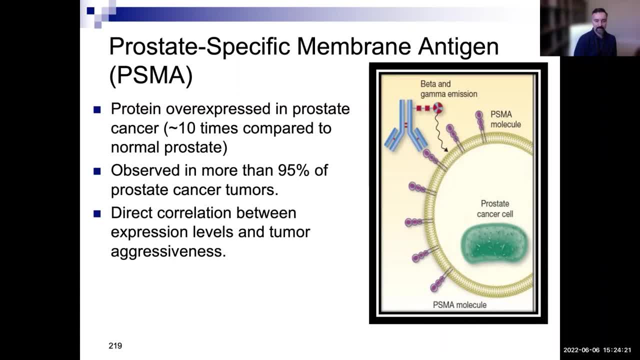 as we measure from the blood, but the PSMA process membrane antigen is this protein that is expressed and overexpressed. in prostate cancer correlates with aggressiveness. There have been molecules that have been designed to target it right. And then if you radio label those molecules, 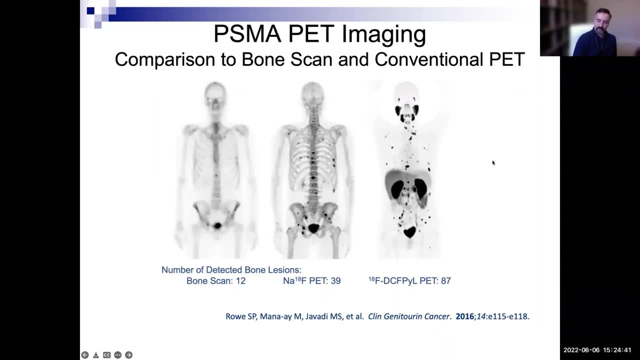 here's an example that was designed by Dr Martin Lodge and his lab at Johns Hopkins University, where I was in our division, And basically, you see, compared to conventional bone scans and PET scans, this one is more sensitive, finds a lot more things. 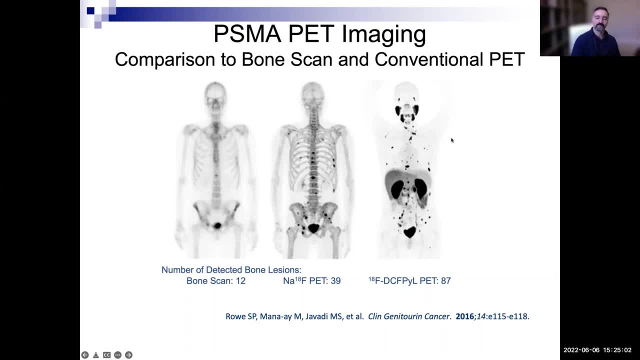 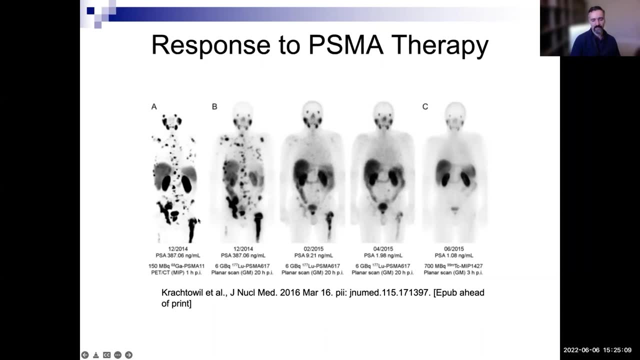 For example, it can find a lot more things. And that's the imaging side, but the therapy side too. So this is the pre-therapy PET scan. Many of these patients are unfortunately hopeless. Nothing is working. Hormone therapy is not working. 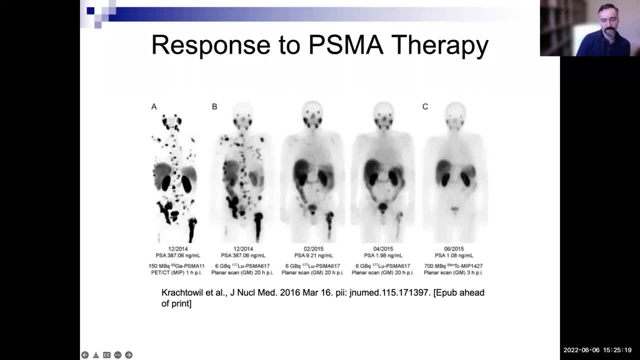 Nothing's working. Of course, external brain radiotherapy will not work here, But then you put them on these doses and you inject them with these PSMA radiopharmaceutical therapy doses and over time, as you're doing. these are SPECT images of Lutetium-177.. 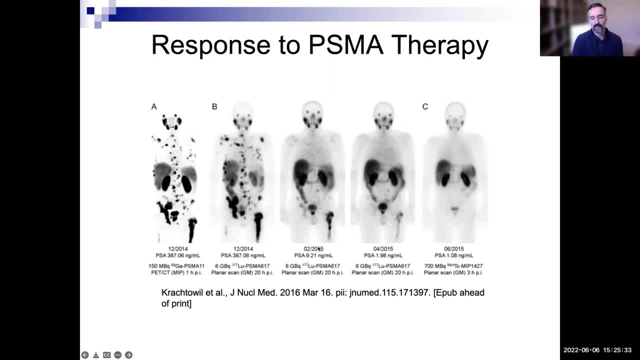 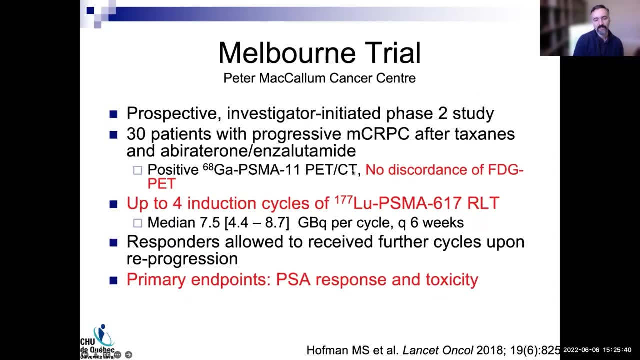 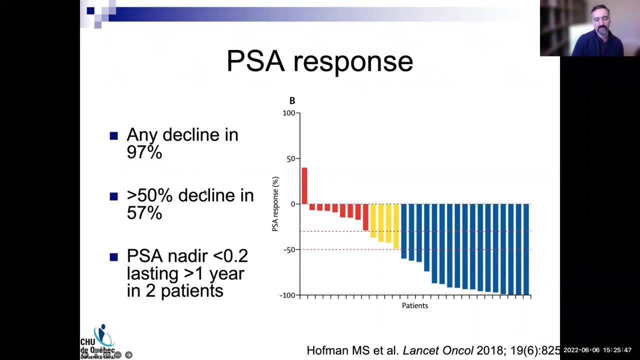 As Lutetium-177 is bombarding these tumors. you see how, over time, over multiple cycles, you see how the responses are mind-blowing. So there's a trial in Melbourne with 30 patients. These are the kind of there was significant decline. 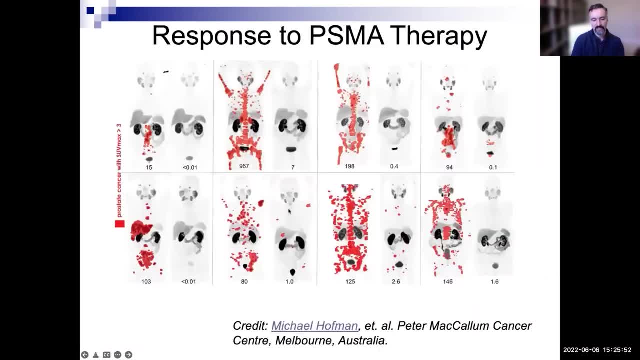 in PSA response. in many patients These are the kind of images you would get: Eight patients out of those 30 before, with tumors all over the body and after, Just miraculous responses. These are the PSA levels. See how much they've significantly changed. 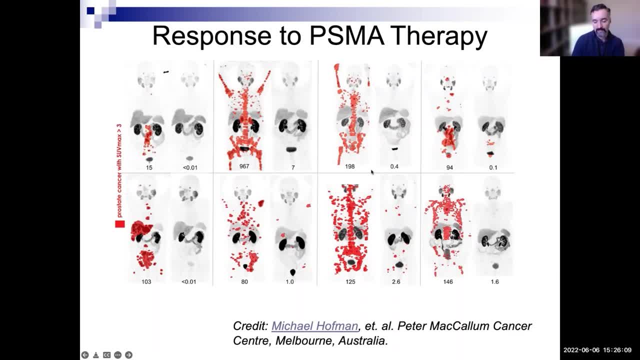 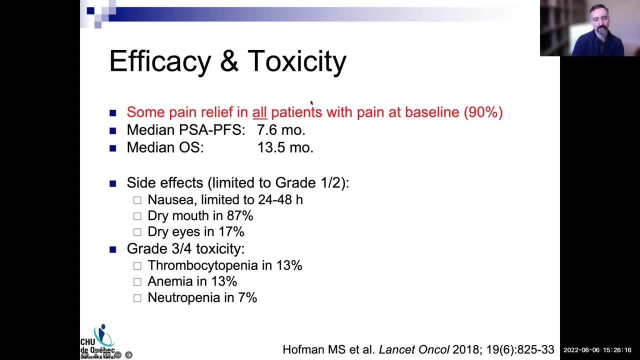 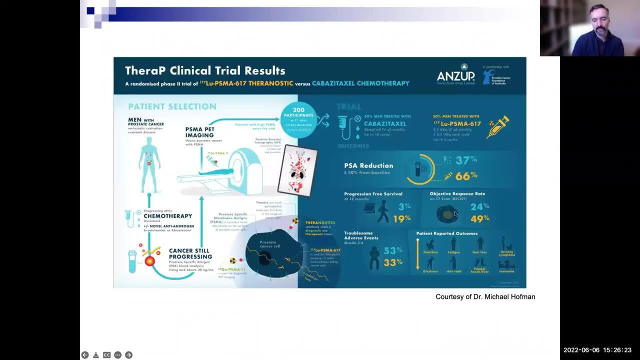 There's a paradigm shift in treatment of metastatic castration-resistant metastatic prostate cancer patients. So well-tolerated by patients- Some pain relief in all of them Well-tolerated. There are some studies, for example in Australia, that really showed that. 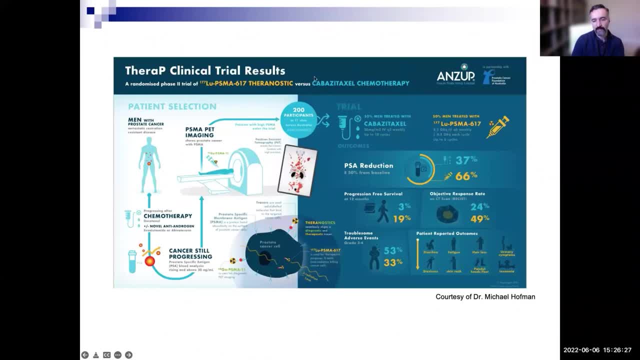 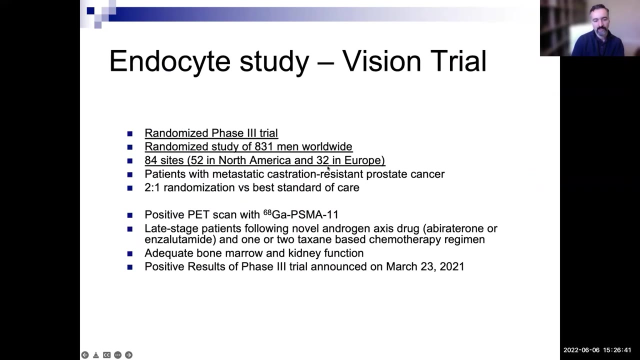 when you compared radiopharmaceutical therapy with chemotherapy- significant improvements to PSA reduction, to progression-free survival and to objective response rate based on resist criteria and CT. There's quite a larger North American study, or actually North American and European study. 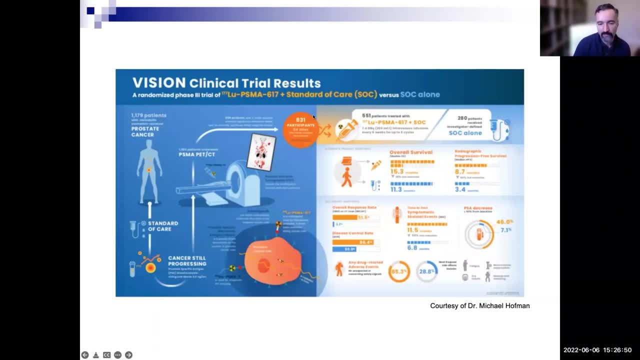 vision trial. that showed that overall survival. so this is comparing radiopharmaceutical therapy along with standard care, with standard care alone, And it showed that the overall survival increases by four months And that progression-free survival increases by five months. Now note: 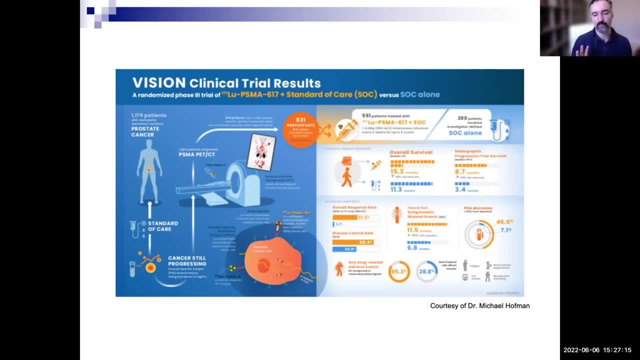 These were not personalized. Same dose, almost the same dose was given to everybody, And that needs to change. But even without that, even though it's uniform dose, non-personalized, no dosimetry, in a sense you're getting these significant improvements. 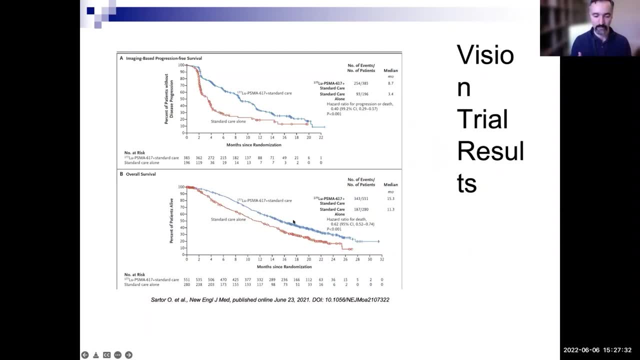 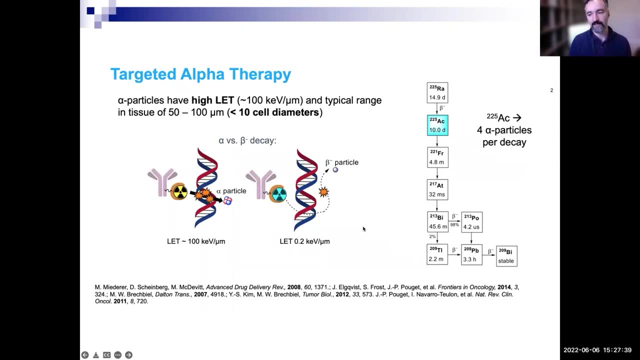 So it's been transformational. What the research community and what we're trying to push is to say: no, you gotta also personalize these and you might see more tremendous improvements. Those are beta therapies, meaning electrons, lutetium etriol-90, but you could also use, you know. 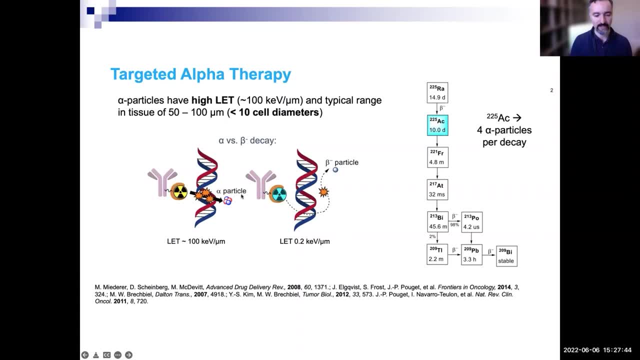 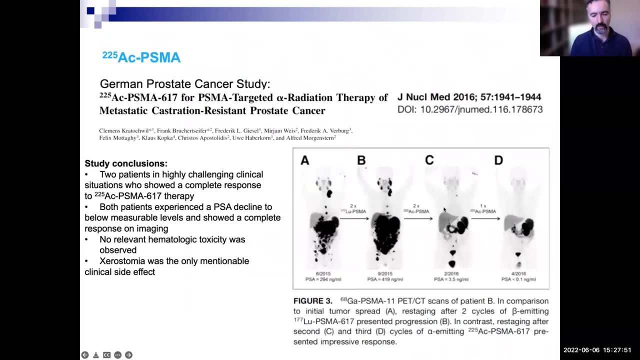 but you could also do alpha therapy towards, you know, double DNA strand break And there were some studies- anecdotal studies- showing that when lutetium does not work, alpha therapy might work beautifully. So there's a lot of research in this area. 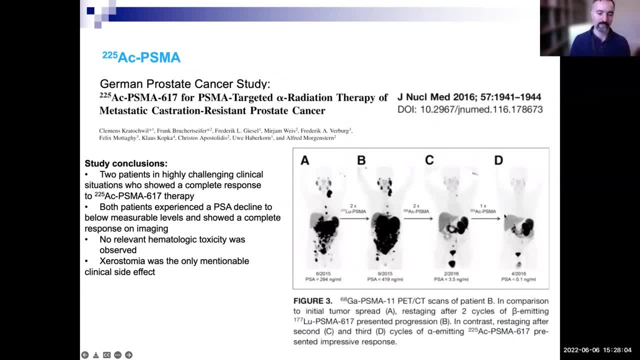 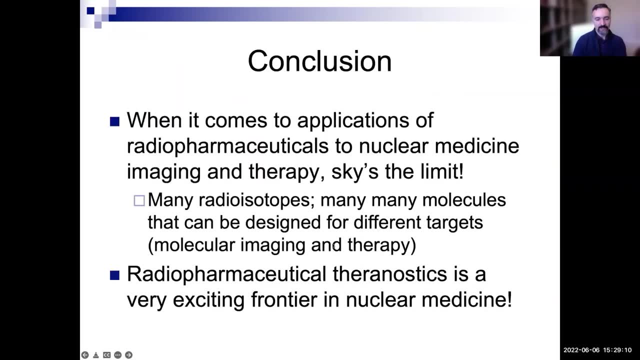 sort of mind blowing. you know images that were shown- that there's a lot of interest in this area, Perhaps a combination of alpha and beta therapy: beta for longer range, alpha for shorter range. So there's a lot of research in this area.